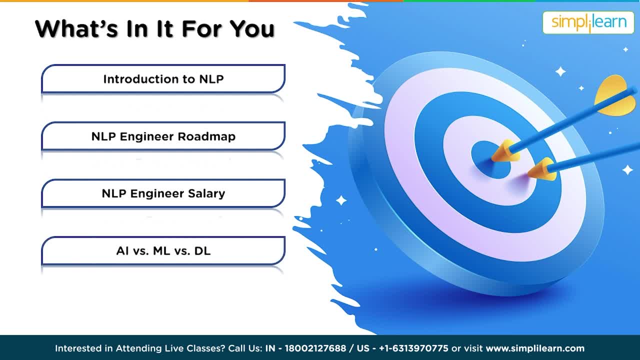 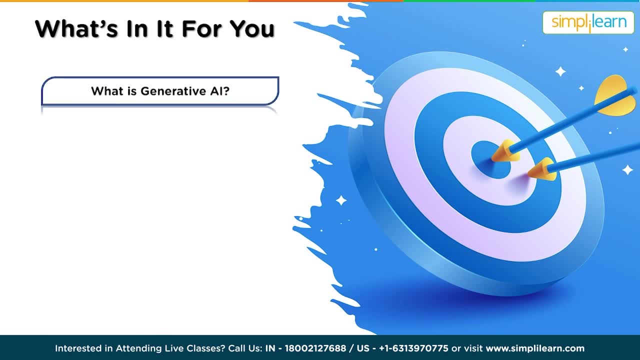 fantastic concepts like AI versus machine learning, versus deep learning, and after that we'll see text mining in NLP. Following that, we'll cover topics like what is generative AI and large language models in artificial intelligence. After covering all these topics, we'll see algorithms and projects like sentiment analysis. 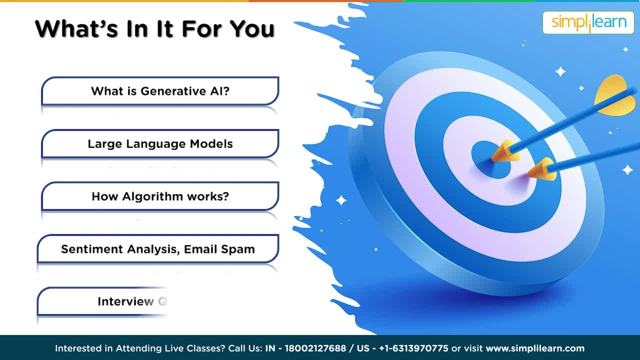 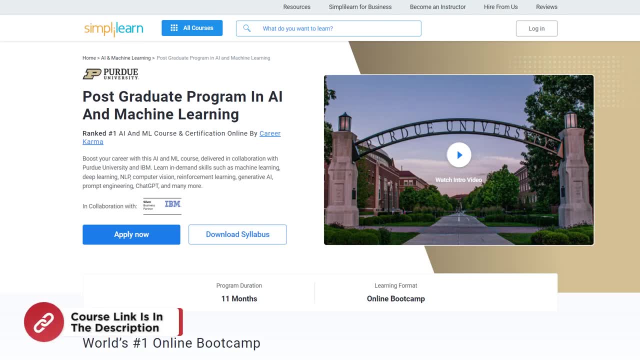 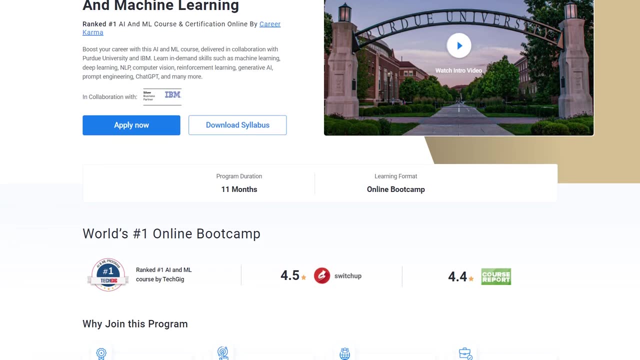 and email analysis. Speaking of interviews, we have covered you, along with the most frequently asked interview questions to help you crack the toughest interviews. But before we move on to what NLP is, if you are an aspiring AI and machine learning engineer, then there's no better time to train yourself in the exciting field of artificial intelligence. 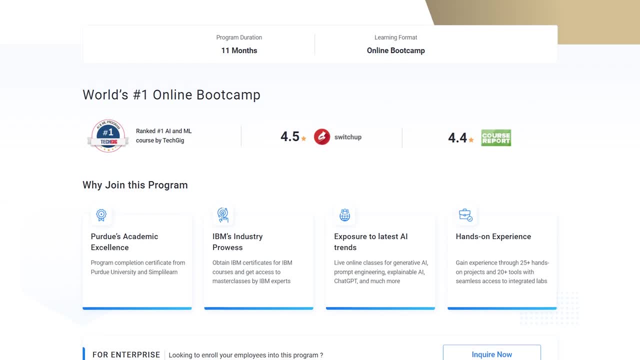 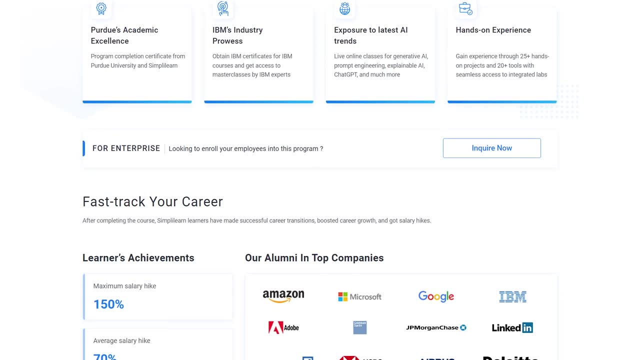 If you're looking for a course that covers everything from the fundamentals to advanced techniques, then accelerate your career in AI and machine learning with a comprehensive postgraduate program in AI and machine learning. Boost your career with this AI and machine learning course. Thank you for watching. 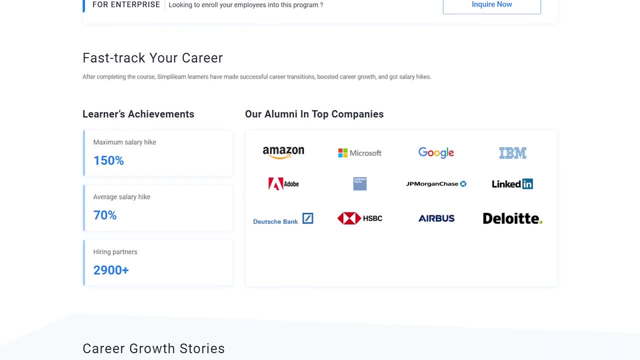 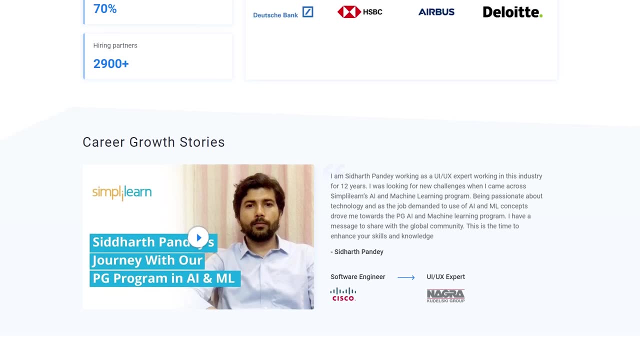 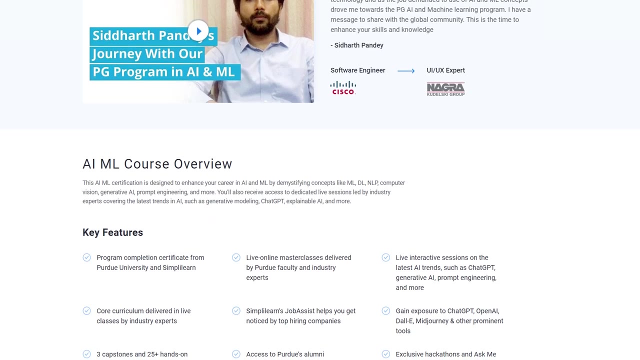 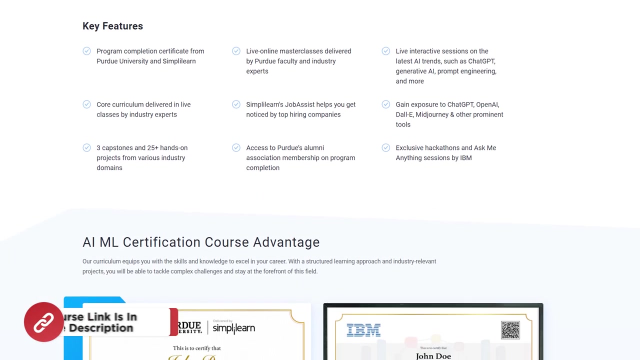 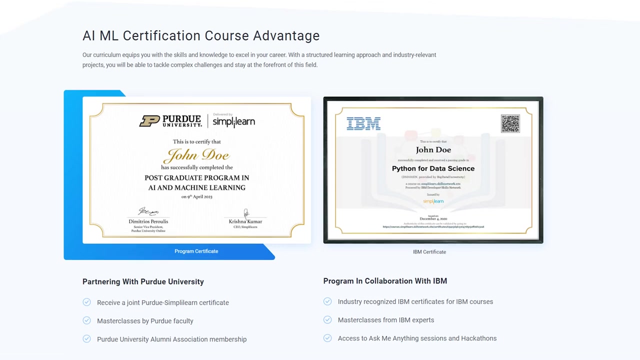 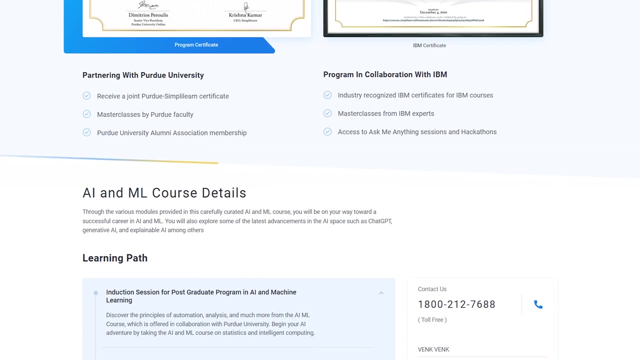 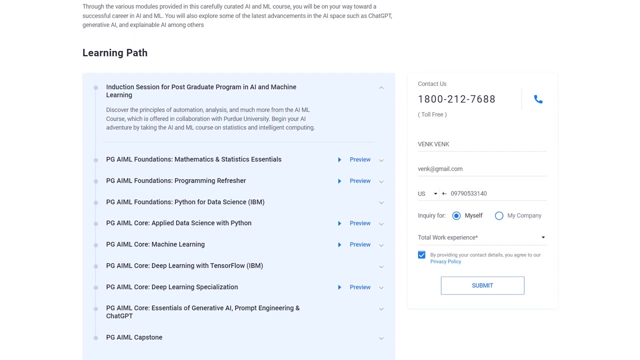 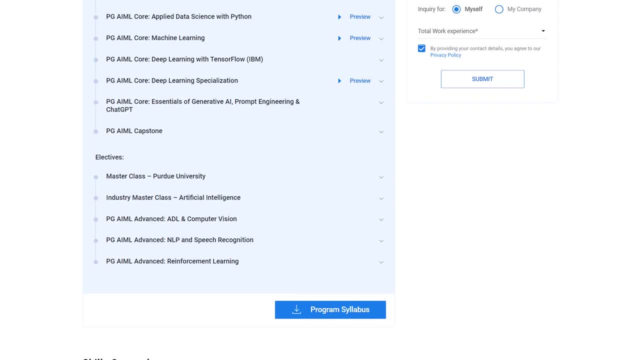 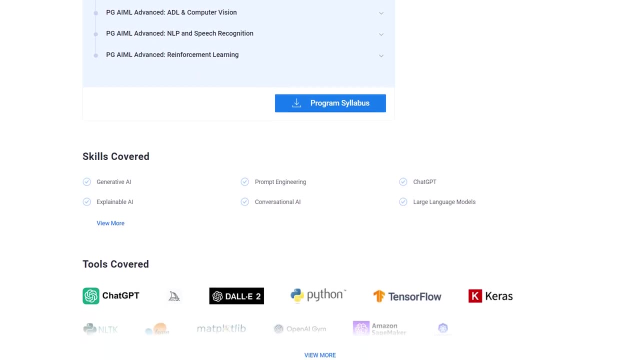 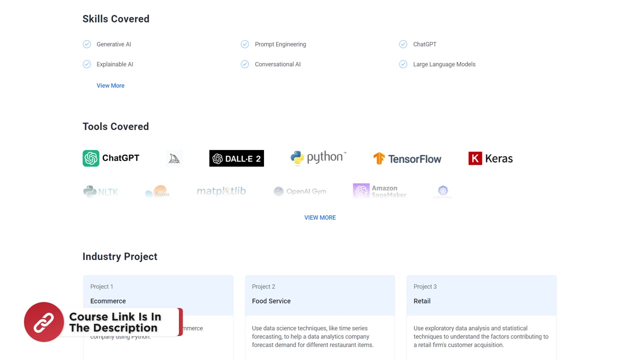 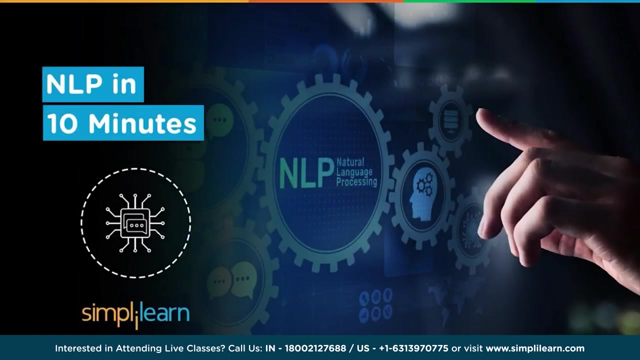 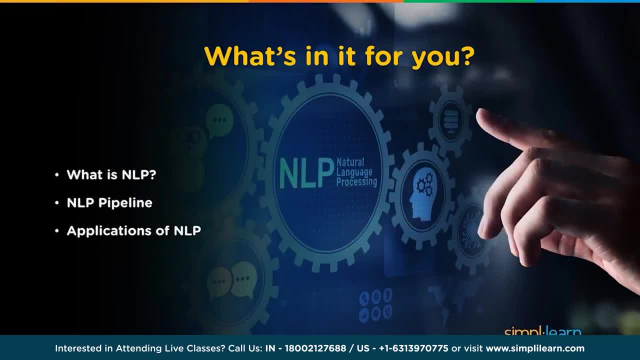 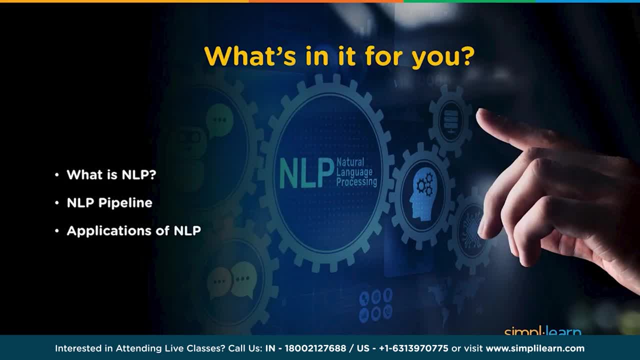 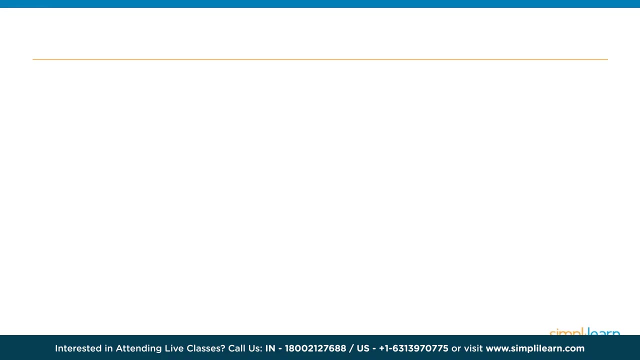 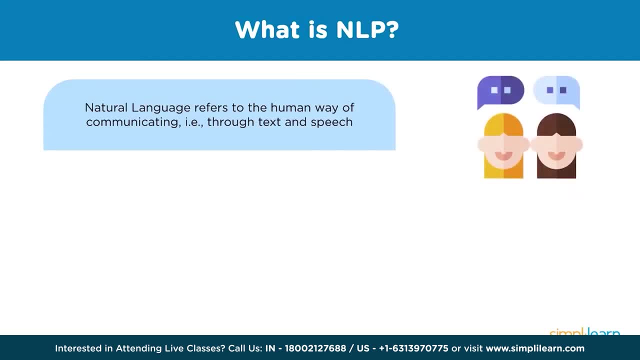 communicate with each other, mostly via speech or text. To convey your intent to someone, you may directly talk to them or send them a message. The human way of communicating is known as natural language. Around the globe, many languages are spoken and messages are. 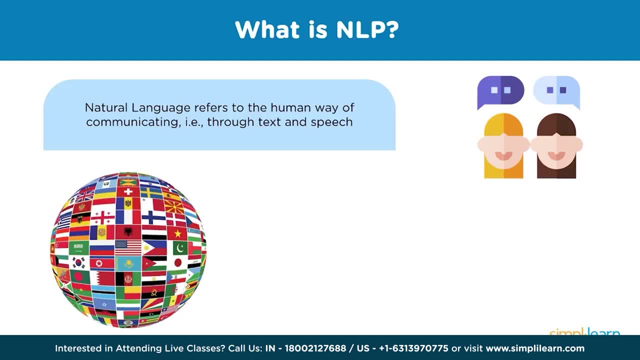 shared virtually every single day. All these conversations, feedbacks and messages are data in themselves. This data is extremely valuable as it can give us customer information and insight into human sentiment. However, this data is not useful to computers as it is not in a form that can be understood by machines. Machines communicate using ones. 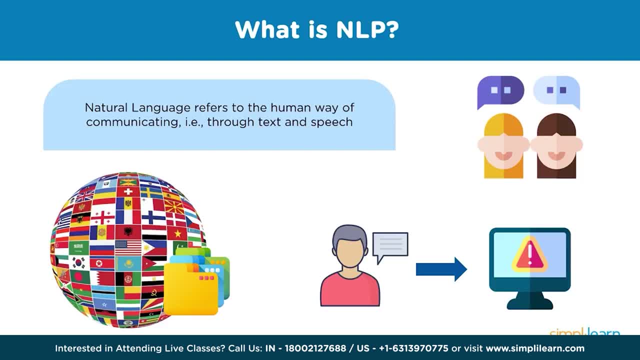 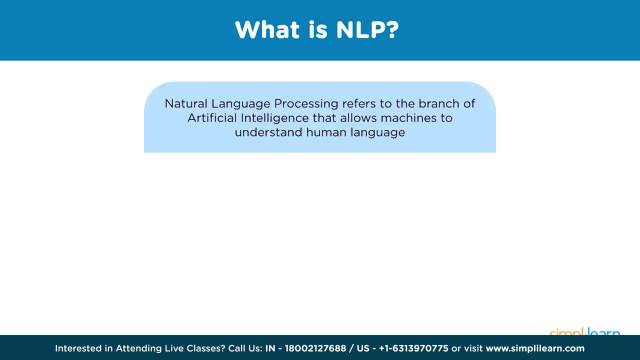 and zeros and not via words. They cannot understand English, French or Spanish, only binary. And this is where NLP comes into the picture. NLP stands for Natural Language Processing. NLP stands for Natural Language Processing. This is where NLP comes into the picture. 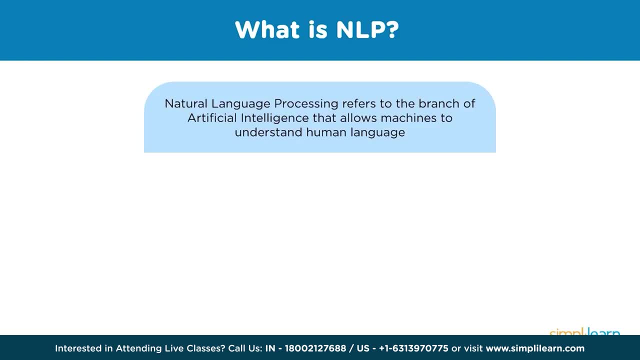 Natural Language Processing is a branch of artificial intelligence that deals with the interactions between humans and computers Using the natural language. the ultimate objective of NLP is to read, decipher, understand and make sense of human languages in a manner that is valuable, and to build systems that can make sense of text and perform tasks like 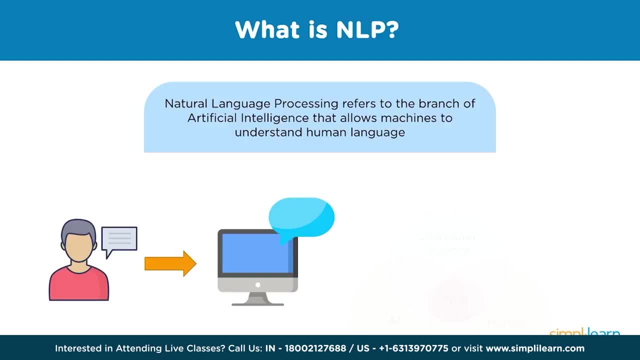 translation, grammar checking or topic classification. NLP basically is the task of processing and using written forms of languages and making a computer understand them. Companies are increasingly using NLP-equipped tools to gain insights from data and to automate routine tasks. A sentiment analyzer, for instance, can help brands detect emotions in text such 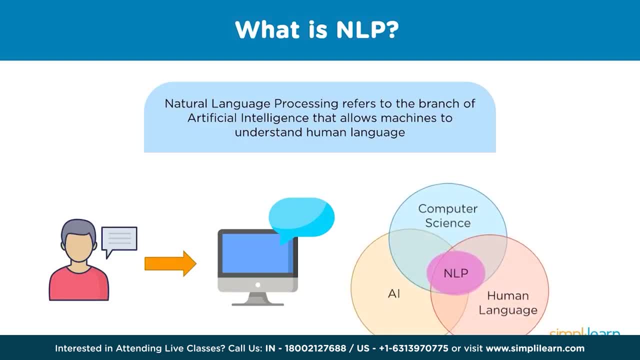 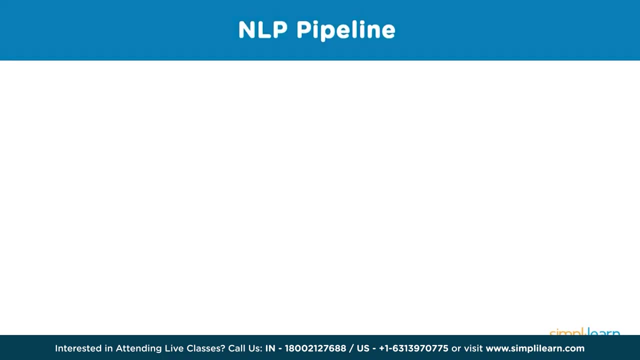 as negative comments on social media. NLP, at the end of the day, is nothing more than accumulation of artificial intelligence, computer science and the human language. The next topic that we'll be looking at are NLP pipelines. So what exactly are pipelines? A pipeline is a set of data processing elements. 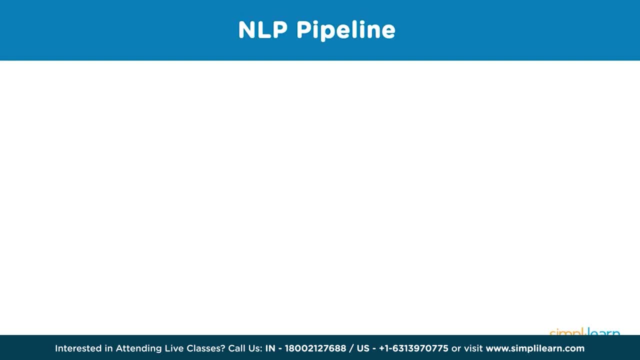 which are connected in series where the output of one element is the input of the next one. It basically represents the various steps which have to be taken in our computation and the order in which they occur In this pipeline we are going to be parsing. 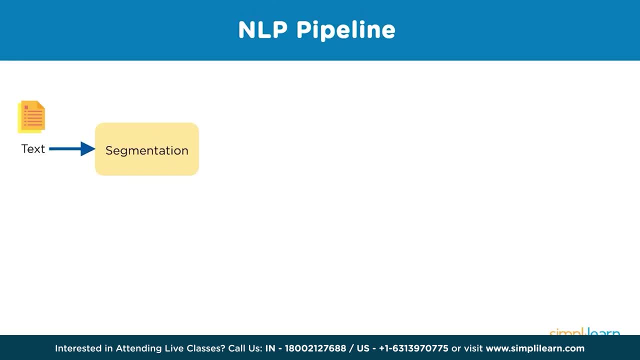 our data. Parsing means converting our data from one form to another. In this case, we are parsing our input text data to a file which can be understood by our computer. The text is first broken into segments, and the segments are then converted into even smaller tokens. The word stems of all of these tokens are: 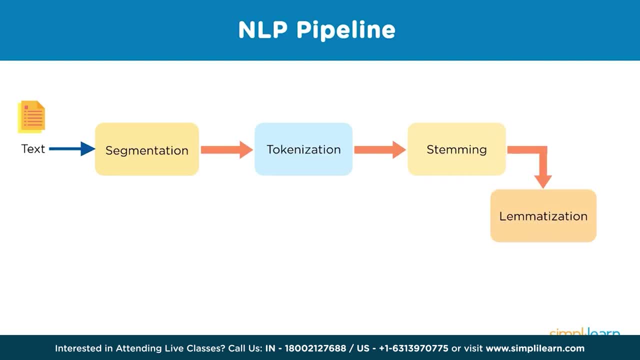 found, followed by finding the root words of these stems in a process known as lemmatization. We will then recognize which part of speech the word belongs to, Which means if the word is a verb, a noun or a pronoun. 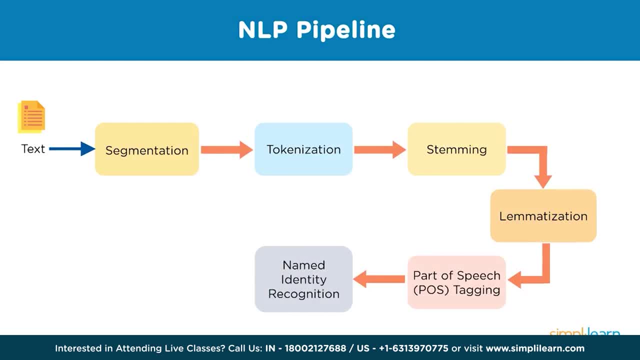 And finally, we will separate the instances of everyday popular entities from our words to better understand what the sentence is trying to convey. The final file that we'll get will be a file which will be understood by a computer Segmentation. The first process of a pipeline is segmentation. 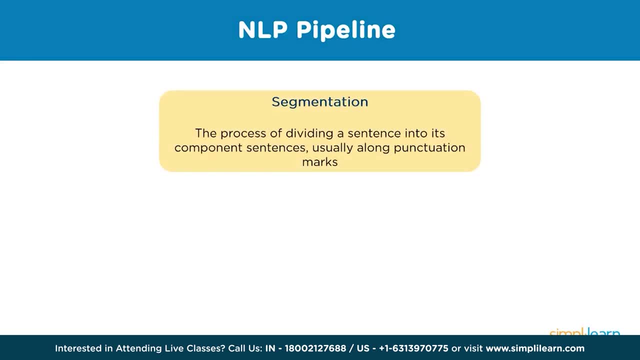 Now, what exactly is segmentation? Sentence segmentation or text segmentation is basically dividing the given text into logically decipherable units of information. We divide the sentence into its constituent sub-sentences, usually along the punctuations or along line breaks and page components for HTML files. 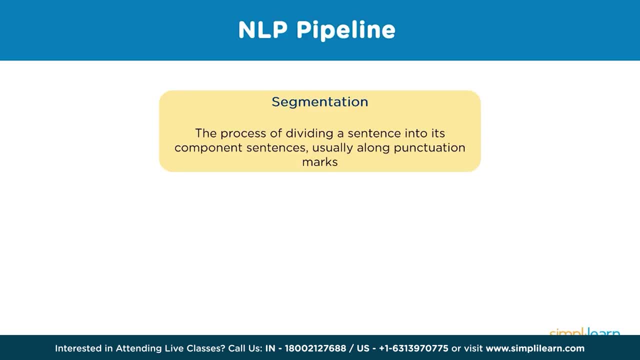 Dividing a document into its constituent sentences allows us to process it without losing its essence and the necessary information that it contains. In this case, let's consider a sentence. The lemonade quenched her thirst, but not her longing After sentence segmentation. we are going to divide this sentence into two. 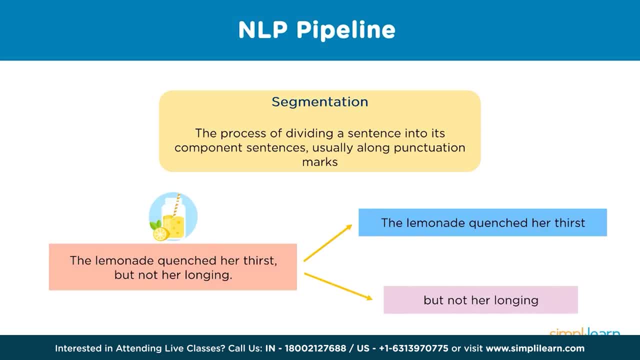 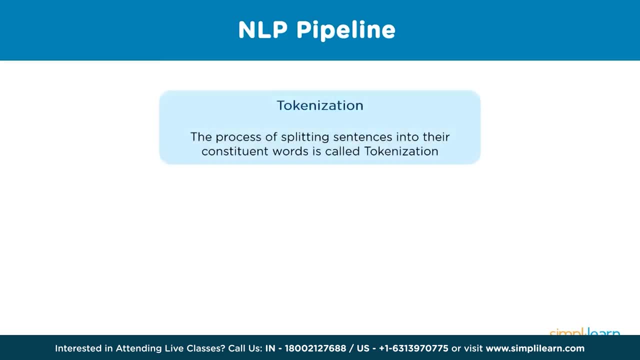 The first sentence is going to be: The lemonade quenched her thirst, And the second one is going to be: But not her longing. The next step of our pipeline is called tokenization. Tokenization is nothing but the process of dividing a sentence into its constituent words. 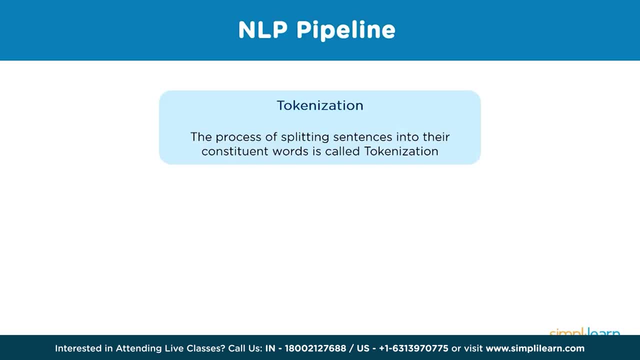 The sentence that is given to us will be separated and all the words in the sentence will be stored separately. This is done so we can understand the syntactic and semantic information contained in each sentence. Thus, we decipher the relevance of a sentence by analyzing it word by word, thereby making 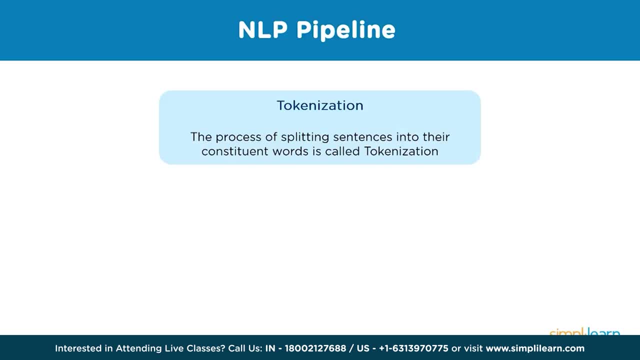 sure that no loss of information occurs. The computer does not understand punctuations and special characters. hence we can remove any punctuations and special characters which may occur. Let's take a look at the second part. Let's take a look at the third part. 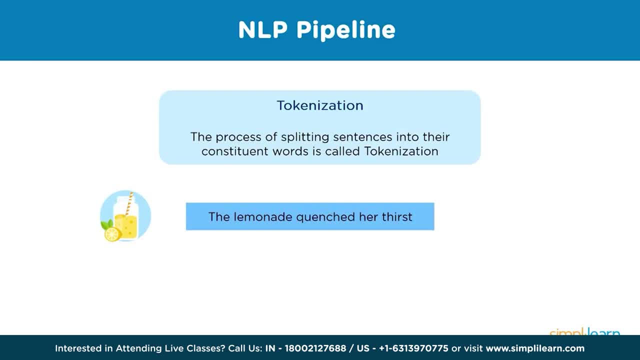 Let's take a look at the third part of our previously segmented sentence Over here. let's consider the lemonade quenched her thirst. After tokenization, we are going to separate every single word in the sentence. So after tokenization we are going to get five different tokens. 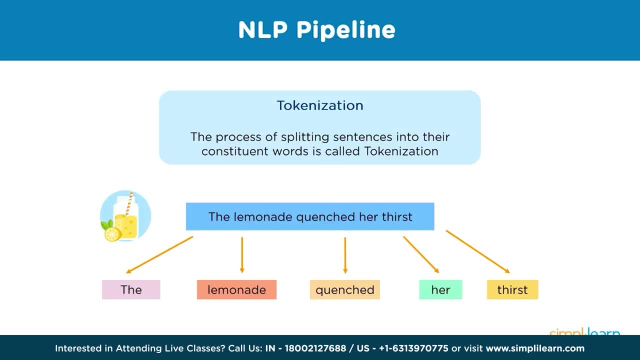 The lemonade quenched her and thirst. All of these are going to be treated as separate entities. After tokenization, we perform stemming. Stemming is the process of obtaining the word stems of a word. Stemming is the process of obtaining the word stems of a word. 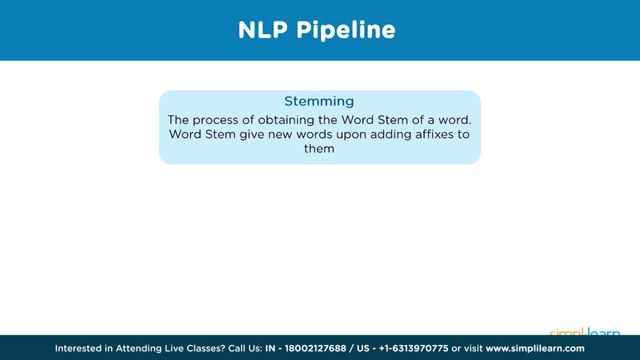 Word stems are also known as the base form of a word, and we can create new words by attaching affixes to them in a process known as inflection. Stemming is the process of recognizing the word stems of individual words. This is done by removing affixes such as ing, es, ed, etc. 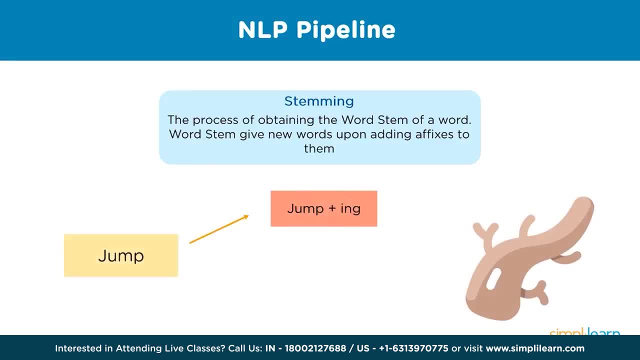 For example, consider our sentence: jump. Jump is the word stem of various different words like jumping, jumped and jumps. In this sentence, the word jump is the stem of various different words like jumping, jumped and jumps. In this sentence, the word jump is the stem of various different words like jumping, jumped. 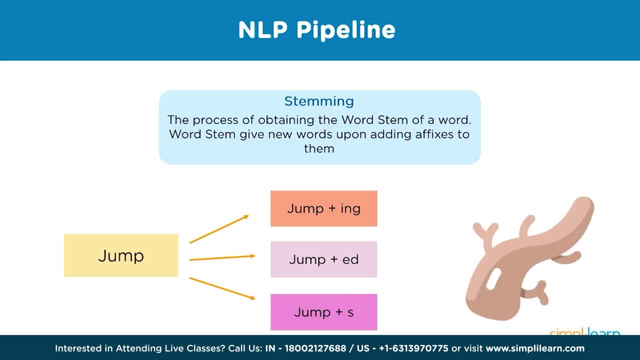 and jumps. If we remove all of these affixes, we will get our basic word, stem, which is jump. This is basically what we want at the end of stemming. The next process in our pipeline is called lemmatization. Lemmatization is the process of figuring out the root form or root word, which is nothing. 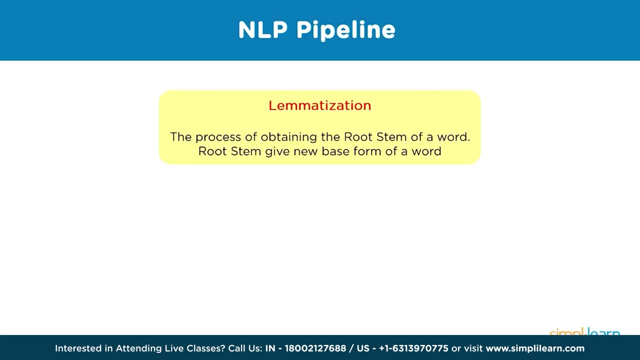 but the most basic form, also known as the lemma, of each word in the sentence. Lemmatization is very similar to stemming, where we remove word affixes to get the base form of a word. The difference is that the root word is always a word which is present in the dictionary. 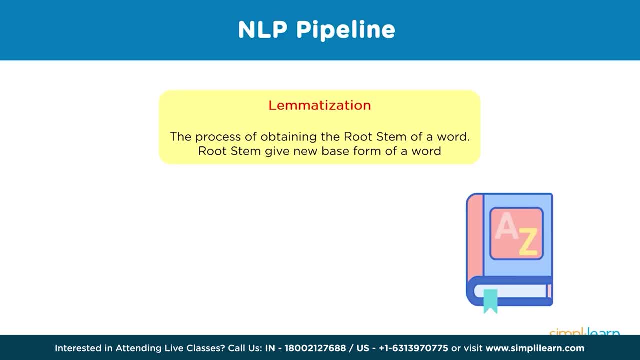 but the root stem may not be so. Lemmatization uses a knowledge base called WordNet. Let's consider three different words: went, going and gone. At the end of the day, all of these words have originated from a single word, which. 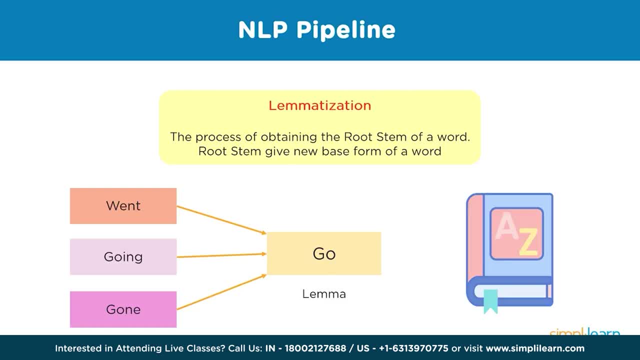 is go. In this case, go is our lemma. All the other words which are derived from go can be traced back to it. The next part of our pipeline is called part of speech tagging. Part of speech tagging is a process of converting a sentence to different forms. 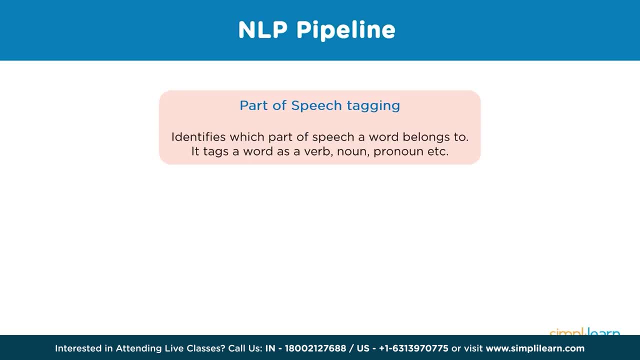 It can be a list of words or a list of tuples. The tag in case of is a part of speech tag and signifies whether the word is a noun, adjective verb and so on. We are basically splitting our verbs into their grammatical components. 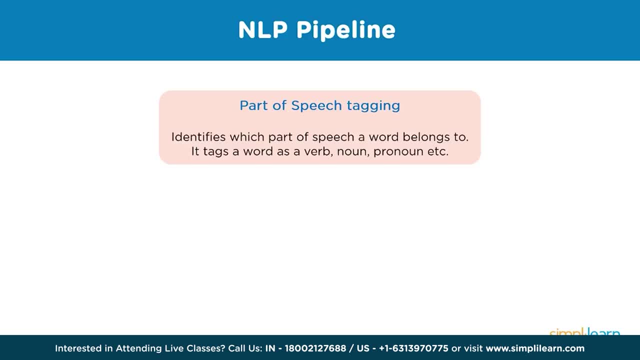 To understand the meaning of any sentence or to extract relationships and to build a knowledge graph, we need to know the meaning of the sentence Part of speech. tagging is a very important step, as the same word can have different part of speeches in different sentences. 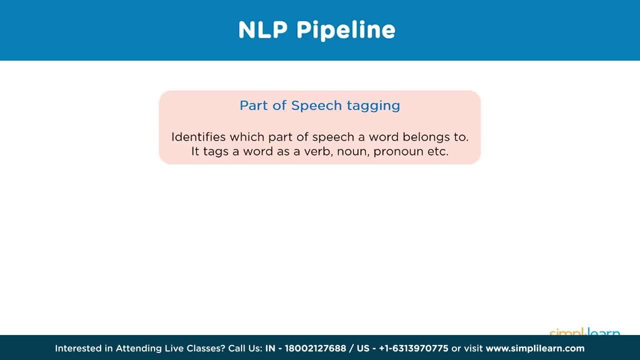 For example, let's consider the sentence: give me your answer. In this sentence, answer is a noun. But if we consider another sentence- answer the question over here- answer will be a verb. Using part of speech tagging, we can take our different tokens and find the different. 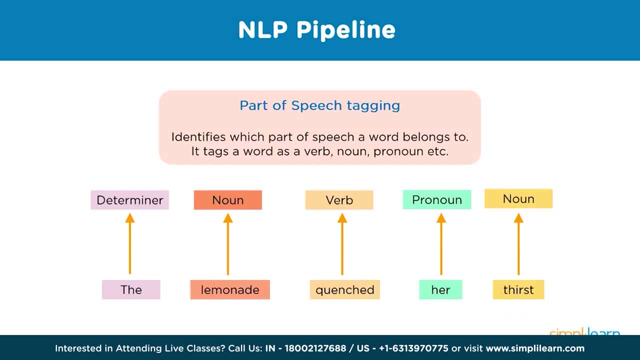 part of speech that it belongs to. In this case, the is a determiner, lemonade is a noun, quenched is a verb, her is a pronoun and thirst is a noun. The final step in our NLP pipeline that we are looking at here is nothing but named entity. 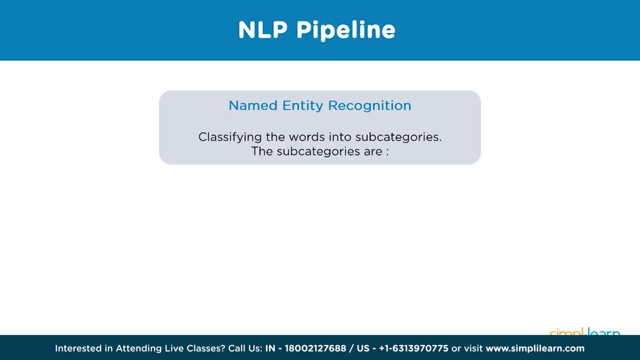 recognition. Named entity recognition, also known as named entity identification, entity chunking and entity extraction, is a sub-task of information extraction that seeks to locate and classify named entities, which are mentioned in unstructured text, into predefined categories. Extracting the main entities in a text helps us sort unstructured data and detect important 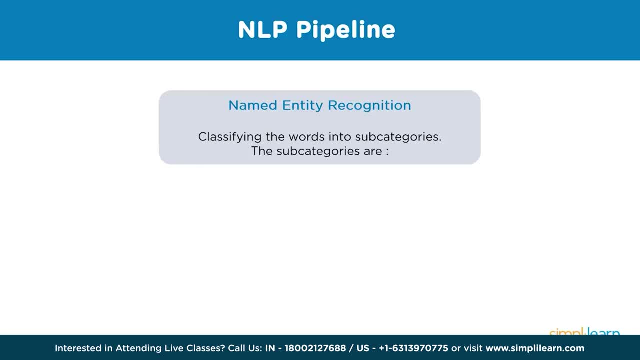 information, which is crucial if you have to deal with large data sets. The sub-categories that we are considering are person, whether the named entity is a person, whether it's a quantity like kilograms, a location or a number, An organization, the name of a movie, or whether it's a monetary value like dollars. 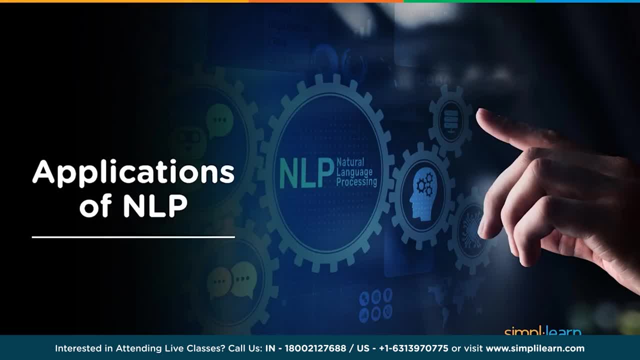 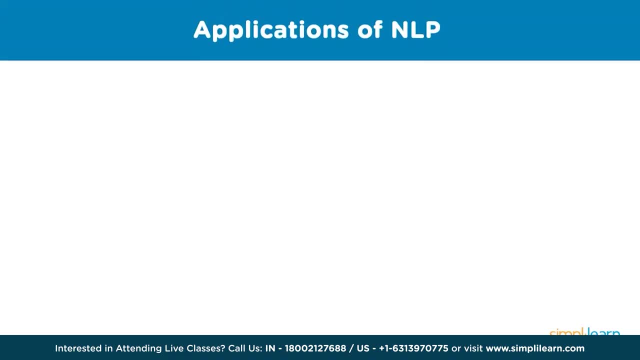 or euros. So far, we've looked at what NLP is and how we can perform natural language processing, But what are some applications of it and where is it used in the real world? One of the applications of NLP is in chatbots. 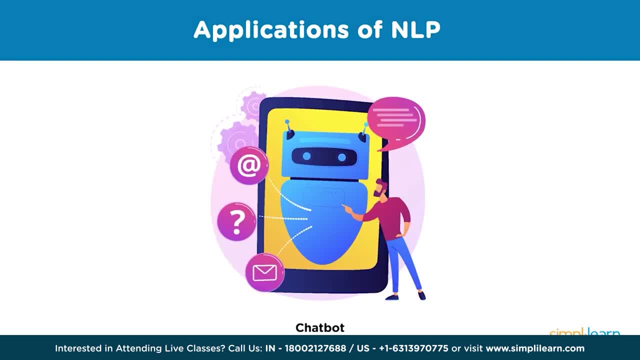 Chatbots can help you solve issues while performing natural language processing. In other words, they can hold a conversation in plain English. A chatbot is nothing but a software application which can be used to conduct an online chat conversation, either through text or speech, in place of providing direct contact with 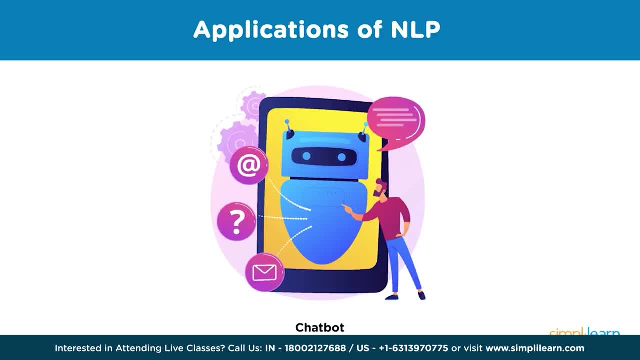 a live human agent. You might have seen those talk to one of our agents section. on websites Those are usually chatbots. A lot of companies also use WhatsApp chatbots to make the process seem less mechanical. So what are some of the applications of a chatbot? 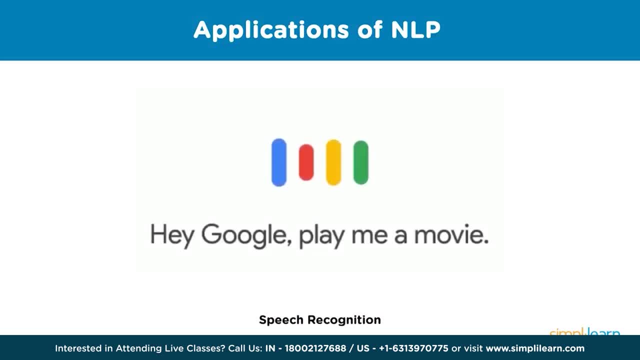 Let's take a look. Another application of NLP is speech recognition. Probably the most popular example of NLP in action are virtual assistants like Google Assist, Siri and Alexa. Natural language processing understands and translates the human language like Hey Siri, where is the nearest gas station? 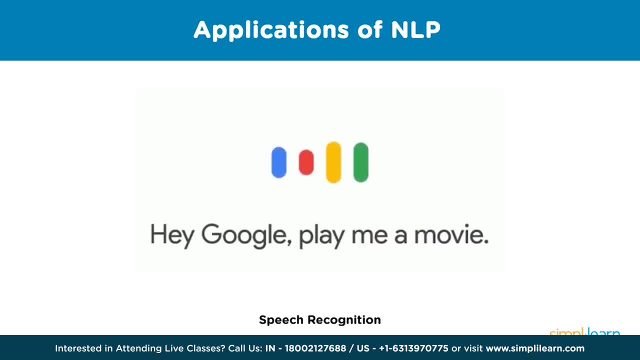 into numbers, making it easy for machines to understand. They recognize when you are talking, converting speech to text, and understand what you requested. After the years, virtual assistants have become streamlined enough to be able to emulate human speech patterns almost flawlessly. 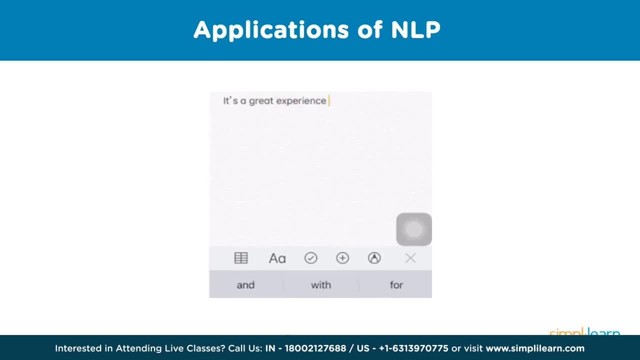 Another application of NLP is autocorrection. Autocorrection, also known as text replacement, replace as you type or simply autocorrect, is an automatic data validation function commonly found in word processors and text editing interfaces for smartphones and tablet computers. It acts as a spell check if you have a problem with the text. 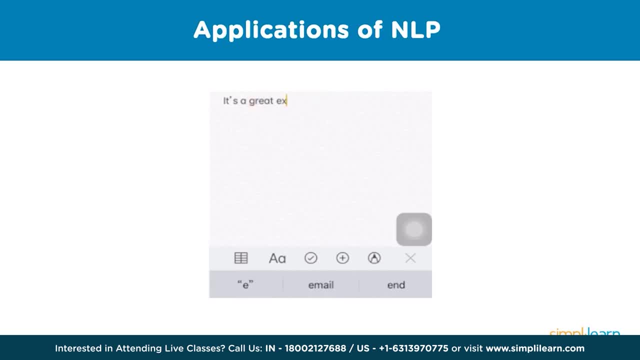 It checks and corrects any spellings or grammar mistakes which may arise as you are typing. Some language check. softwares like Grammarly, Paperator, Reverso and others can even check how unique and engaging your articles are, And all of this is done using NLP. 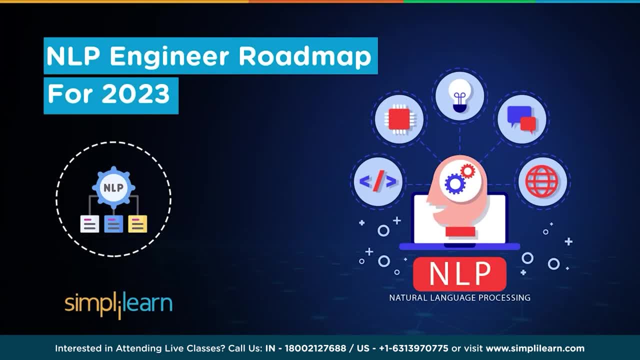 Hello everyone, welcome to this video on the Natural Language Processing NLP Engineer Roadmap by SimpliLearn. To stay updated with our content, make sure to subscribe to our YouTube channel and hit the bell icon. So in this video we will begin by example. 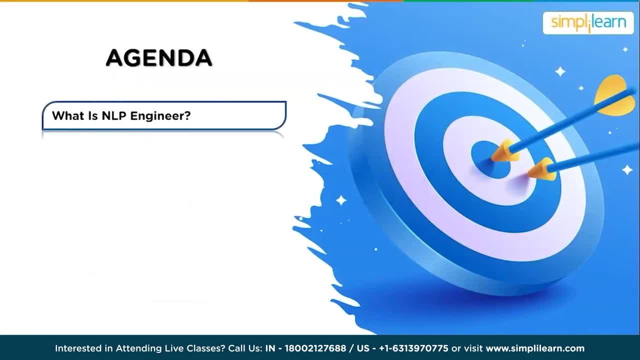 Let's start by examining the role of NLP Engineer. Progressing further, our focus will shift towards the essential knowledge and skills required to excel as an NLP Engineer. Having comprehensively explored these subjects, we will then proceed to explore the intricacies. 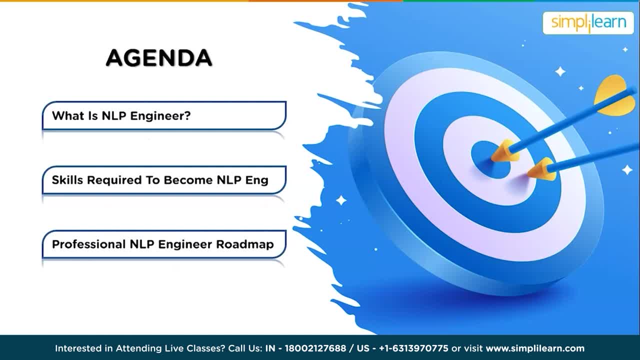 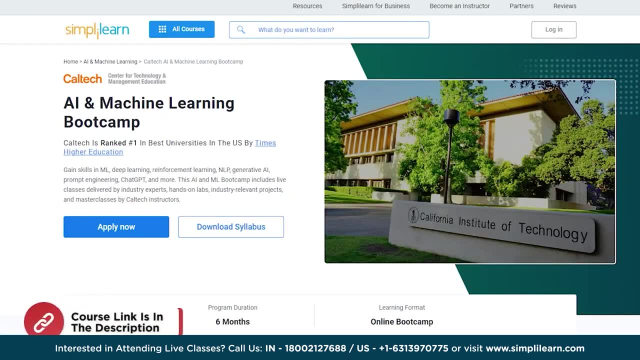 and construction of a professional career roadmap tailored specifically for individuals aspiring to become accomplished NLP Engineers. On that note, if you are an aspiring AI-ML Engineer, then there is no better time to train yourself in the exciting field of machine learning. If you are looking for a career in machine learning, then this is the time for you. 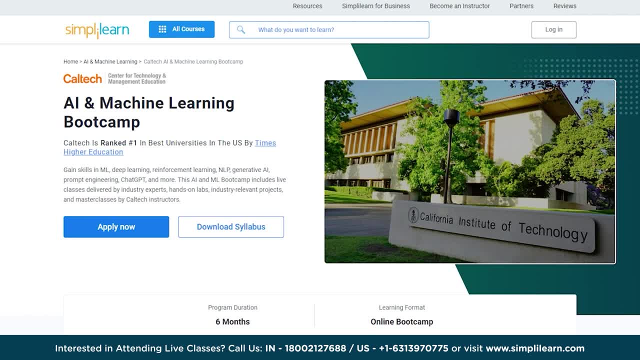 If you are looking for a course that covers everything from the fundamental to advanced techniques like machine learning, algorithm development and unsupervised learning, look no further than our Caltech program partnership with IBM. This AI-ML Bootcamp in collaboration with Caltech will help you advance your career as an AI-ML. 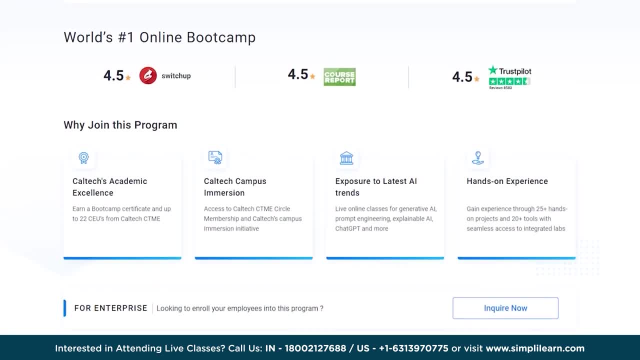 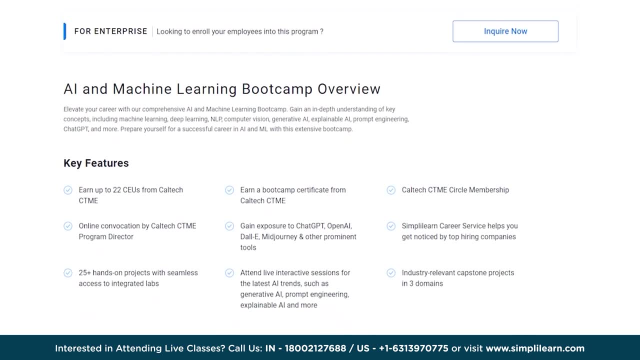 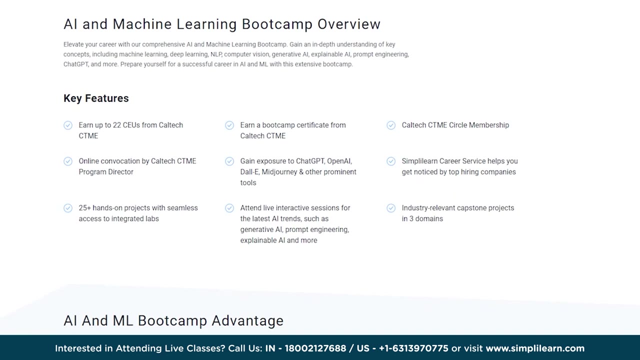 specialist. The AI-ML Bootcamp includes live classes delivered by industry experts, hands-on labs, industry-relevant projects and masterclasses by Caltech professors. Key features of this amazing machine learning course includes an up to twenty-two CUs from Caltech CTME. online convocation by Caltech CTME program director. simple and career service. 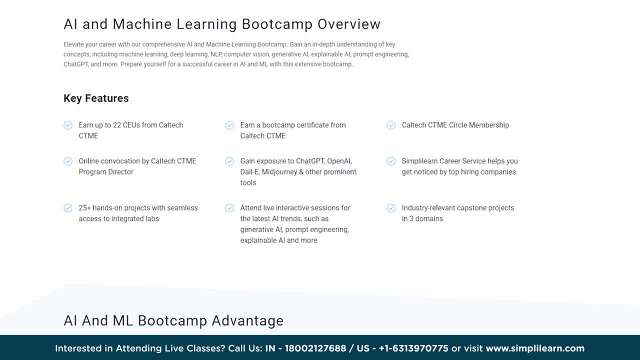 helps you get noticed by top hiring companies and a bootcamp certificate from Caltech CTME Industry-relevant project in three domains. Caltech CTME Circle membership. twenty-five plus hands-on projects across industry verticals with integrated labs. So why wait? 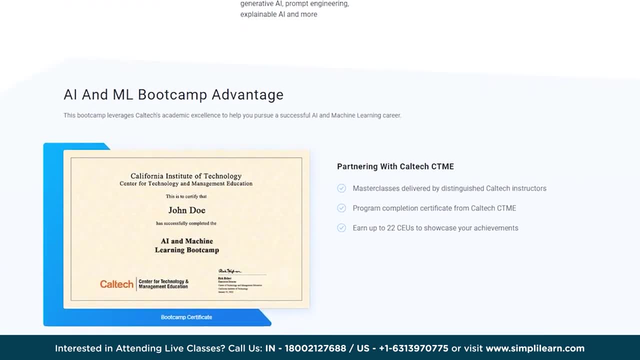 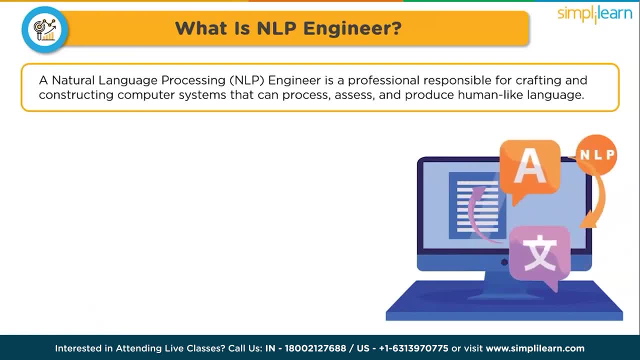 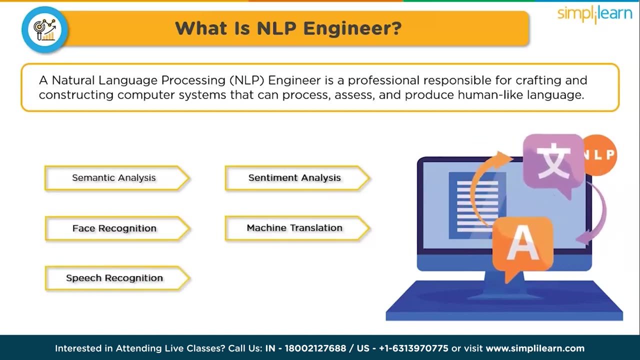 An Azure language processor When processing NLP. an engineer is a professional responsible for crafting and constructing computer systems that can process, assess and produce human-like language. NLP branches out into numerous captivating domains, including semantic analysis, sentiment analysis, face recognition, machine translation and speech recognition. 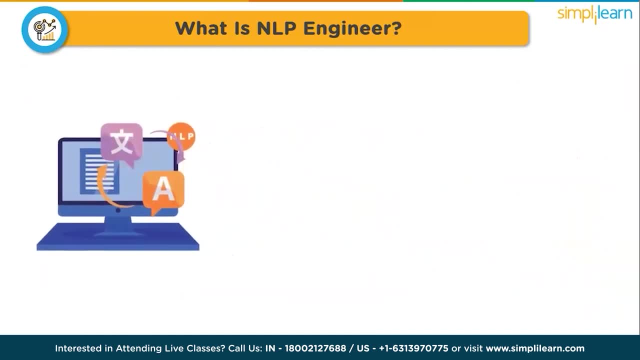 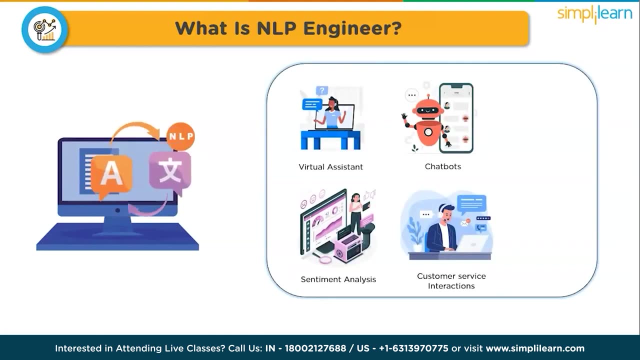 The reach of NLP extends across a diverse spectrum of applications, notably featuring virtual assistants, chatbots, sentiment analysis, customer service interaction and language translation. The task of NLP engineer involves erecting these innovative applications and seemingly embedding them into the existing framework. The average salary for NLP engineer: 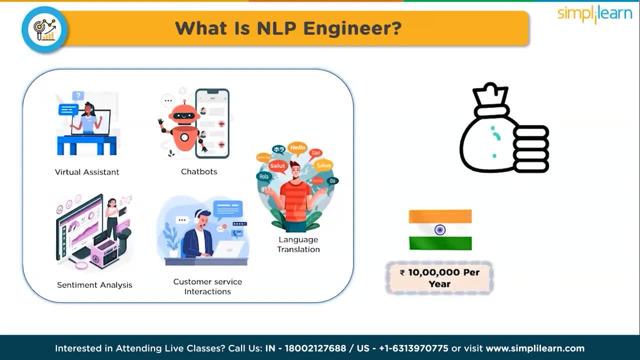 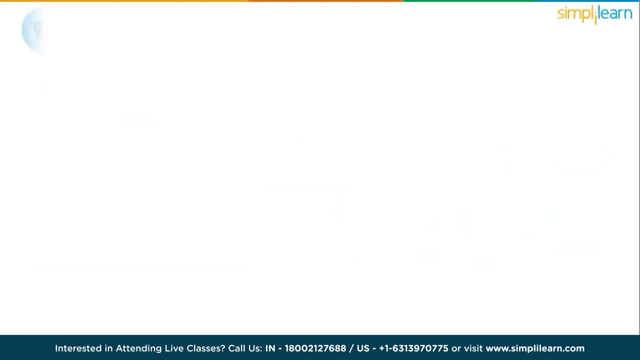 in India is 10 lakh per year, and in the US, average annual salary for NLP engineer is $120,000.. So, moving forward, let's see skills required as an NLP engineer. So becoming a NLP engineer entails the acquisition of a diverse set of applications and knowledge. 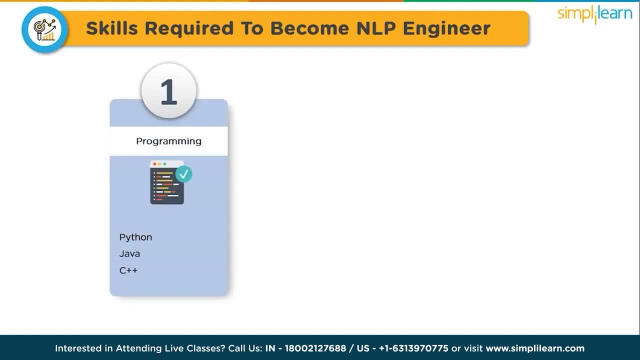 Some of these encompasses: proficiency in programming. mastery of at least one programming language, such as Python, Java or C++, coupled with a solid grasp of data structure, algorithm and principle of software engineering. grasp of machine learning: building a strong foundation in machine learning algorithm, encompassing both supervised and unsupervised learning. 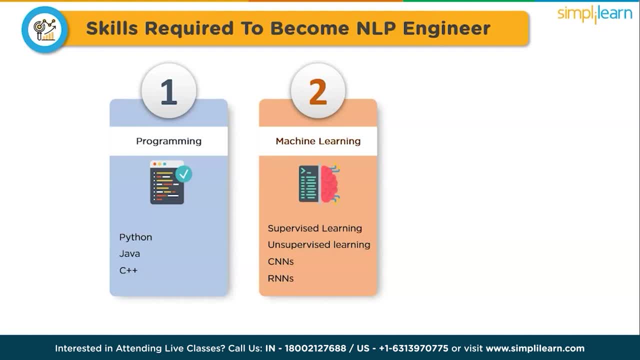 Familiarity with advanced techniques like CNN and RNN is vital. NLP techniques: cultivating a deep understanding of NLP techniques which encounter NLP programming. It encompasses facets like text preprocessing, sentencing and semantic analysis, and the intricate domain of sentiment analysis. 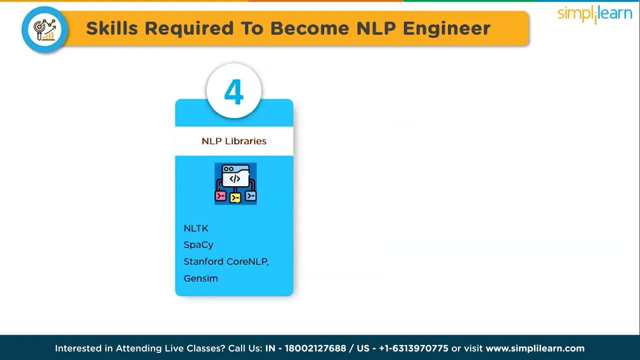 The fourth one is NLP Libraries and Frameworks. Navigate easily through NLP libraries and frameworks such as Natural Language Toolkit, NLTK, SPACE, Stanford Core, NLP and Gensim, harnessing their capabilities to streamline your NLP endeavors. The fifth one is Data Science Acumen: Developing a sound grasp of data science principles and 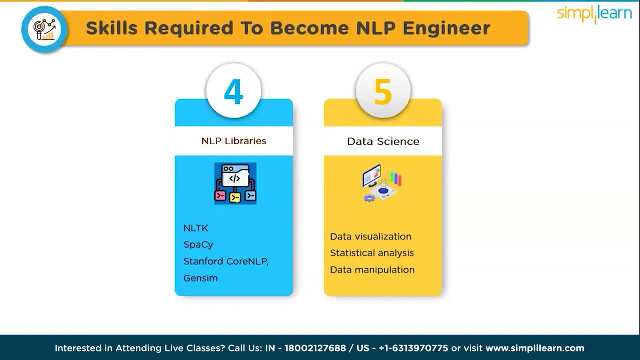 encompassing facets such as data visualization, statistical analysis and the art of data manipulation. Armed with these multi-faceted skill sets, you will be primed to embark on a journey as an accomplished NLP engineer, ready to navigate the complexity of natural language. 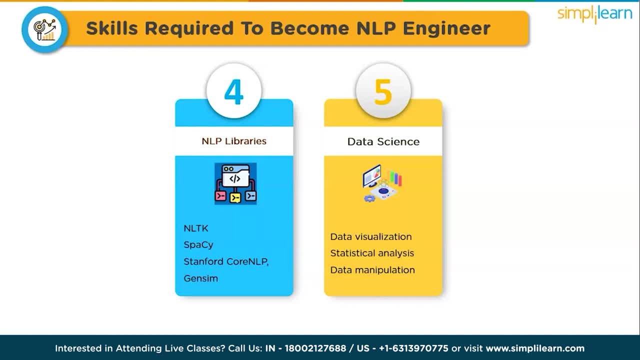 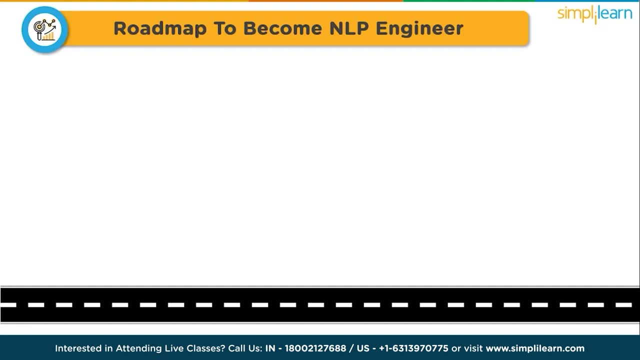 processing and contribute to the exciting world of NLP innovation Moving forward. let's see the professional NLP engineer roadmap. Here is a comprehensive professional strategy for those aspiring to become NLP engineers. The first one is Educational Foundation. Embark on your journey by pursuing a degree in competitive fields such as computer science. 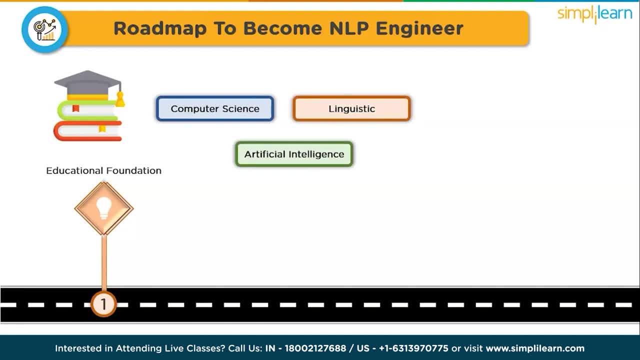 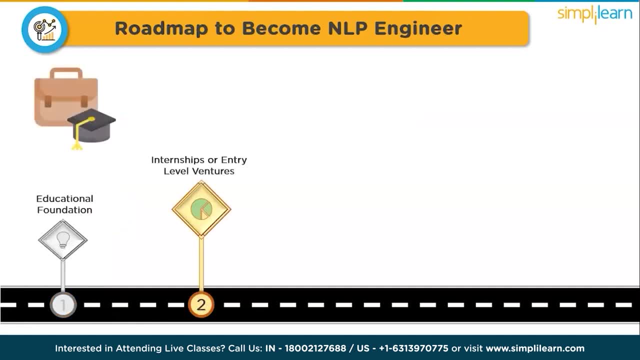 linguistics or artificial intelligence. Many accomplished NLP engineers hold advanced degrees, either a master or PhD, in these domains. The second one is Internship or Entry-level Ventures: considering immersing yourself in practical experience through internship or entry-level jobs within the industry. 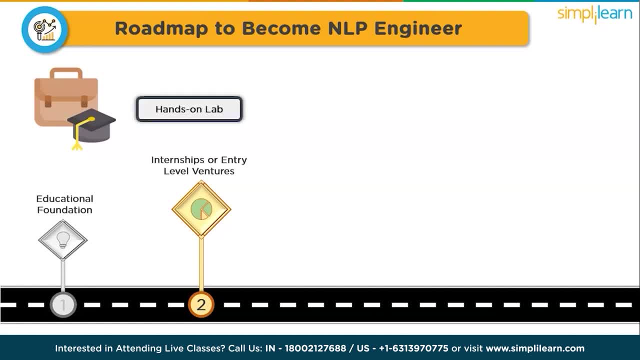 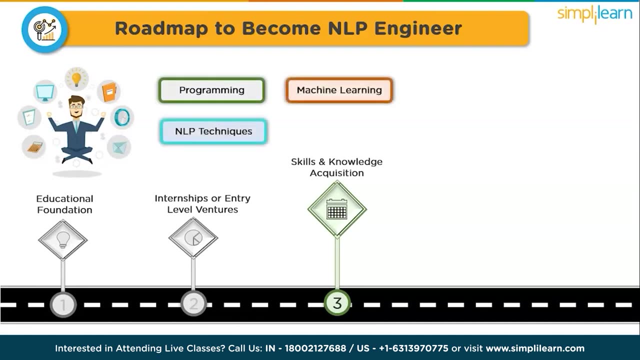 These opportunities not only equip with hands-on expertise, but also aid in constructing a robust portfolio. The third one on the list is Skills and Knowledge Acquisition. Develop a comprehensive grasp of essential proficiency requests of NLP engineers. This encompasses programming processes, machine learning, NLP techniques and data science. 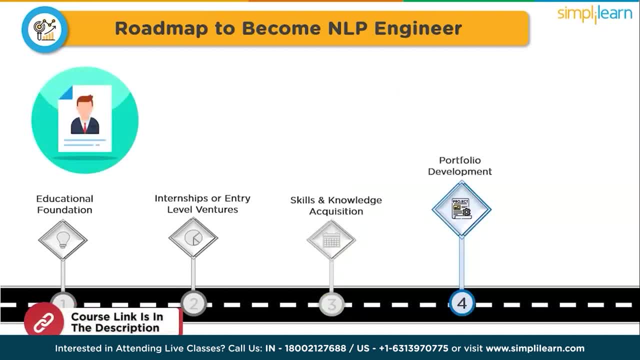 The fourth one is Portfolio Development. Curate a diverse portfolio teaming with projects that illuminate your capabilities and expertise. Projects like sophisticated chatbots, a sentiment analysis tool or a language model can sustain your aptitude for solving real-world NLP challenges and validate your skill set for potential. 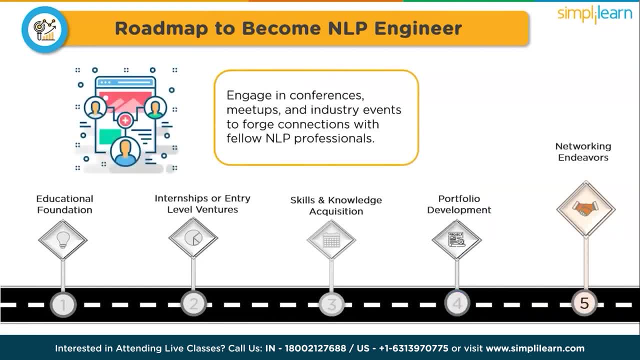 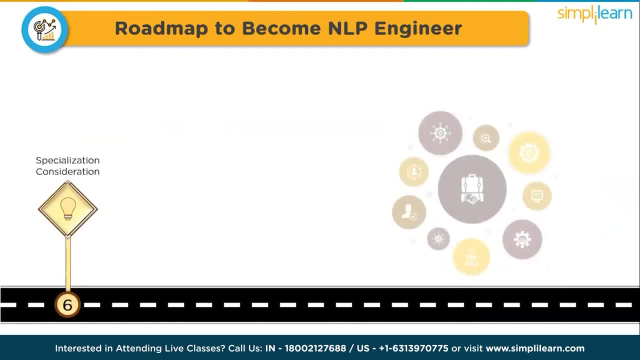 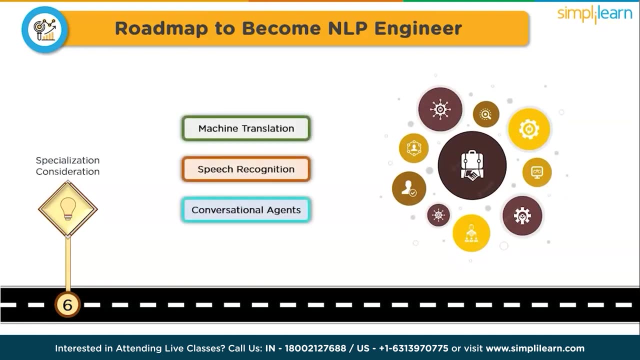 employers. The fifth one is Networking Endeavours: Engage in conference meetups and industries events to forge connections with fellow NLP professionals. The sixth one is Specialization Consideration: Ponder the prospect of specialization in a specific NLP realm, be it machine translation. 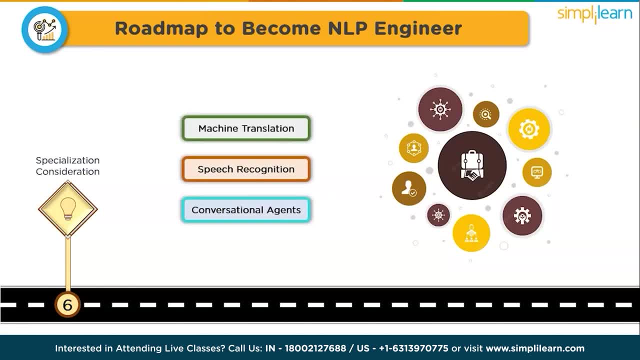 speech recognition or conversational agents. This specialization not only differentiates you in the job market, but also enables you to attain expertise within a particular niche. In summary, the part toward becoming an NLP engineer is as follows: 1. Becoming an NLP Engineer entails a fusion of educational attainment, hands-on experience. 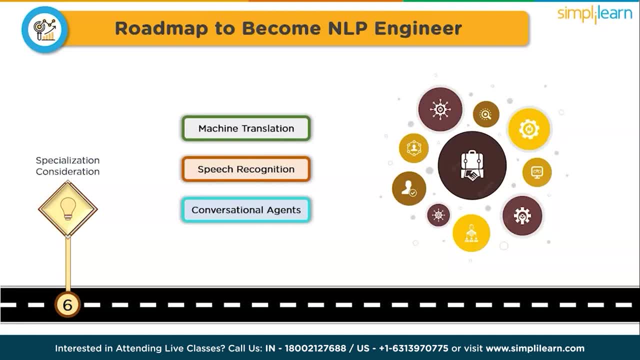 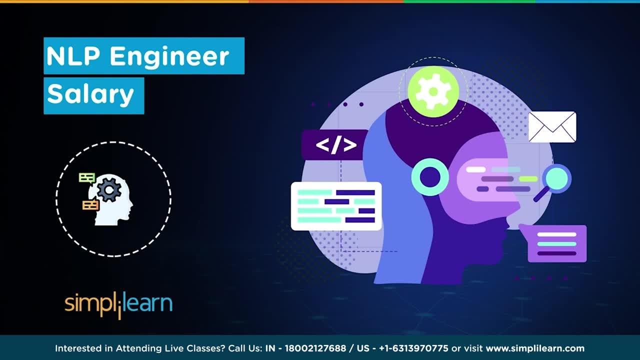 and the mastery of the lectric area of skills and knowledge domains. Hello everyone and welcome to this new video on NLP Engineer Salary. With the world advancing towards a more informed and database future, learning skills that help us to be relevant in the job market is crucial. 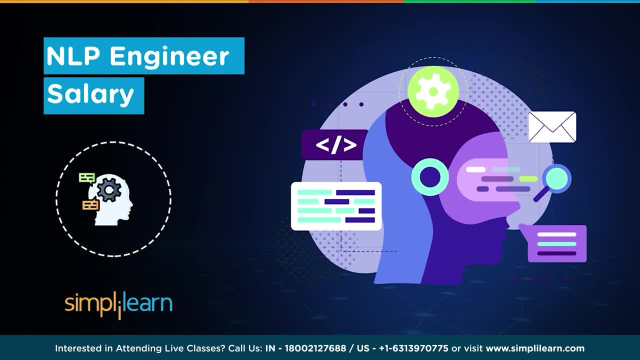 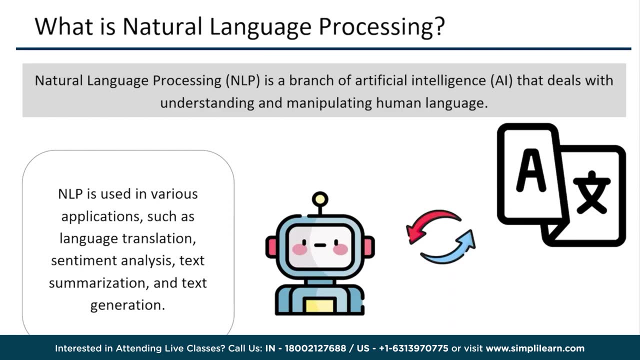 One such skill in the field of data and AI is Natural Language Processing. Let us start by understanding what NLP is. Natural Language Processing is the process in which NLP is processed. Natural Language Processing, or NLP, is a branch of Artificial Intelligence or AI that deals 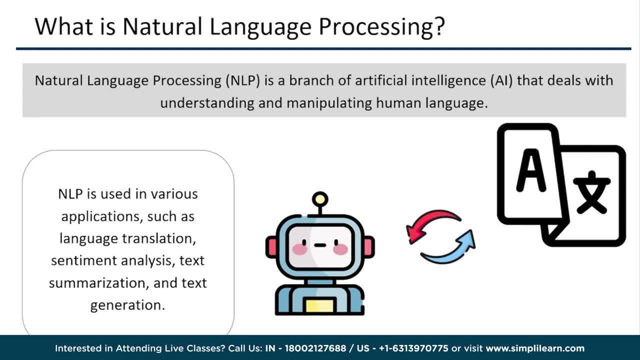 with understanding and manipulating human language. It seeks to develop algorithms and systems that can understand and process both structured and unstructured language data to support decision-making processes. NLP is a field that has been gaining momentum in recent years, thanks to advance in machine learning algorithms and the availability of large datasets such as software. software. 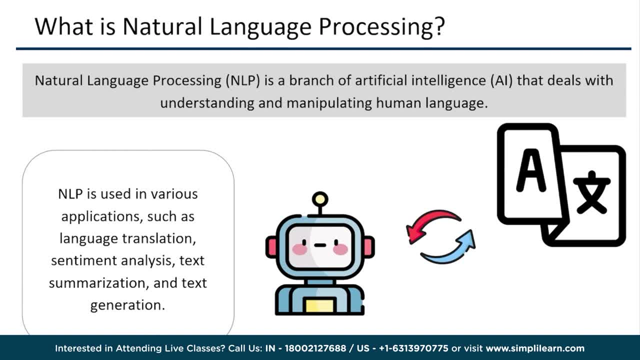 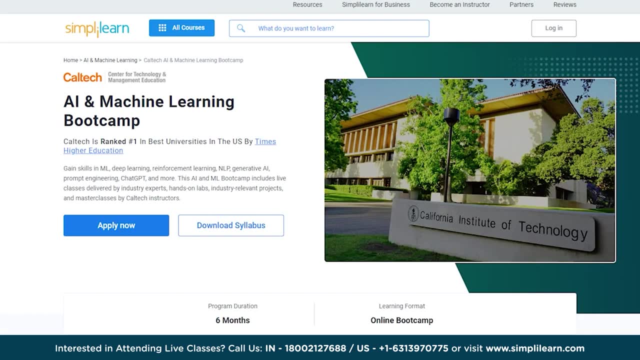 software and machine learning algorithms. NLP is used in various applications, such as social media conversations, customer reviews and medical records. NLP is used in various applications such as language translation, sentiment analysis, text summarization and text generation. If you want to master NLP and become an expert NLP Engineer, then you should enroll in amazing 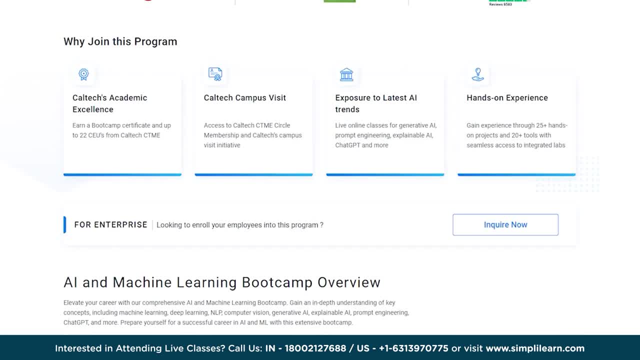 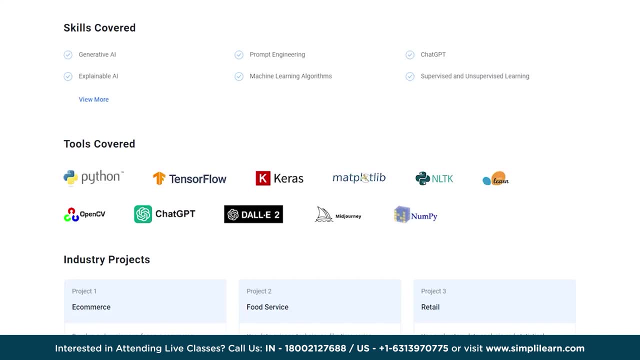 AI and Machine Learning program by Caltech CTME. You will gain skills like Machine Learning, Deep Learning, Reinforcement Learning, Generative AI Processing and Data Management, prompt engineering, chat, GPT and more. This AI and machine learning bootcamp includes. 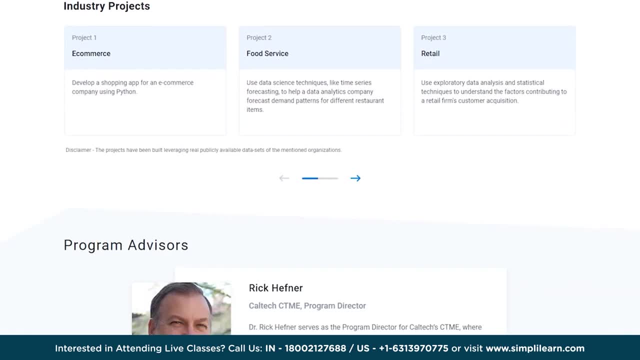 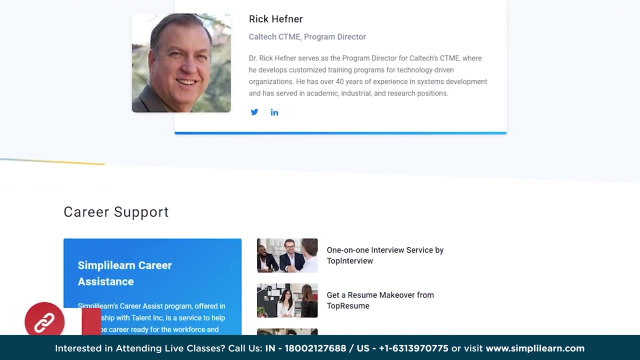 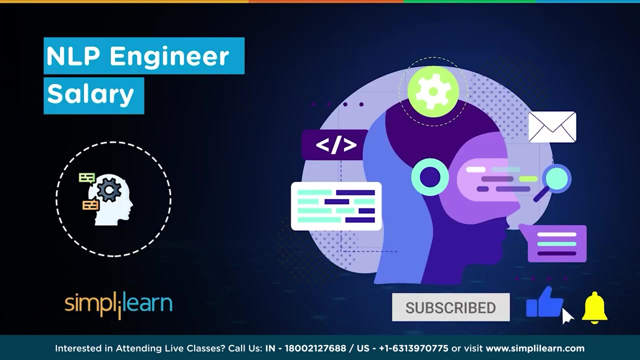 live classes delivered by industry experts, hands-on labs, industry relevant projects and masterclasses by Caltech instructors. So hurry up, what are you waiting for? Enroll the course now. find the course link in the description box. So, before we move ahead, consider subscribing to simply learn and hit the bell icon to never. 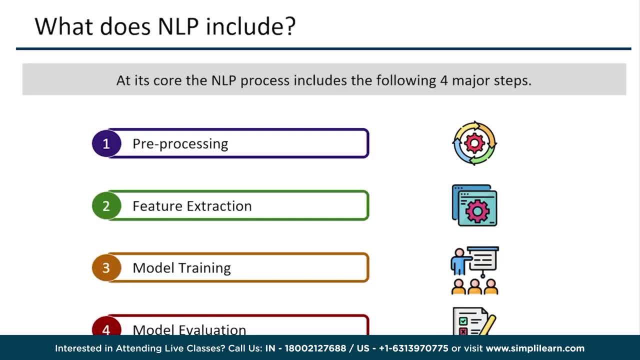 miss any updates from us. So let's move ahead by knowing. what does NLP include? At its core, NLP involves a series of steps. Number one is pre-processing. The first step in NLP is to prepare the language data for analysis. This involves activities such as: 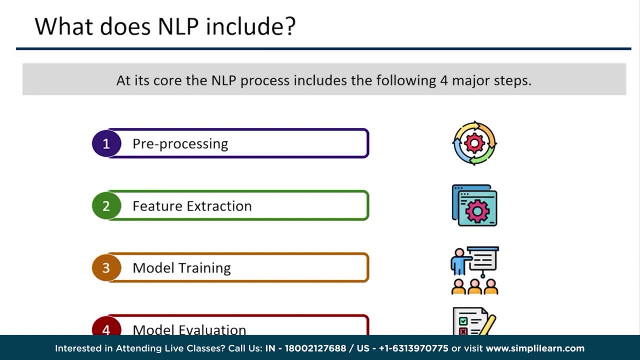 cleaning, tokenization and normalization of the text data. Step two involves feature extraction. The next step is to extract relevant features from the prepared data. This involves identifying keywords, stems and parts of speech tags that are important to be clear. Step three is to 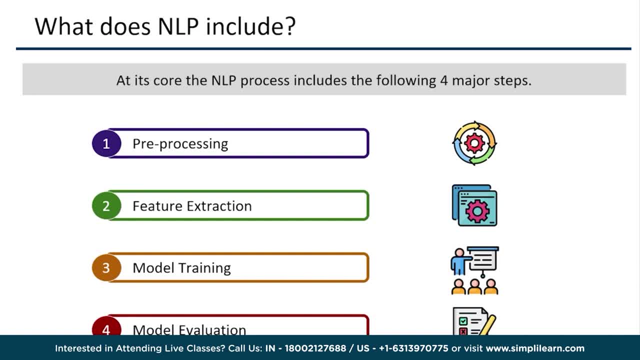 for the task at hand. step 3 involves model training. the extracted features are then used to train a machine learning model, such as neural networks or a support vector machine to predict the target variable. and the last step is model evaluation. once the model is trained, it needs to be evaluated to. 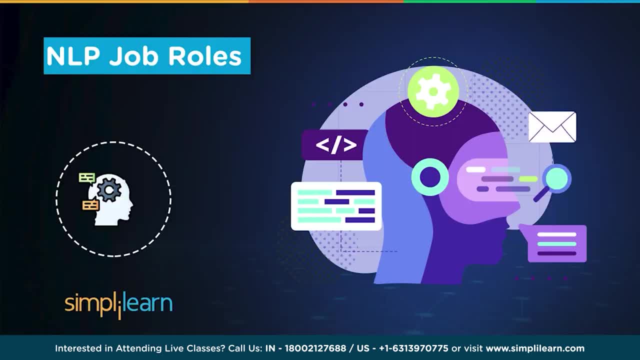 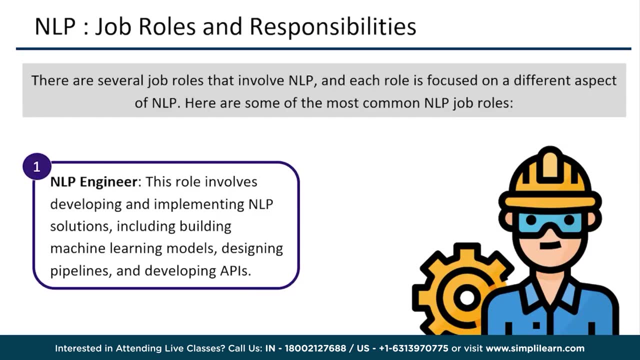 ensure it performs well on new data. now let's move ahead by knowing NLP job roles and responsibilities. several job roles that involves nlp and each role is focused on different aspects of nlp. here are some most common in LP job roles. the number one is an NLP engineer. this role involves developing and implementing. 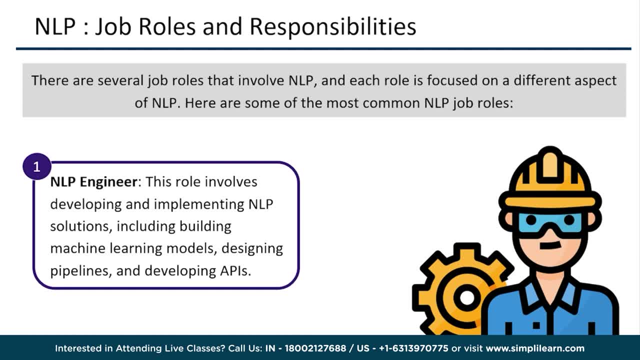 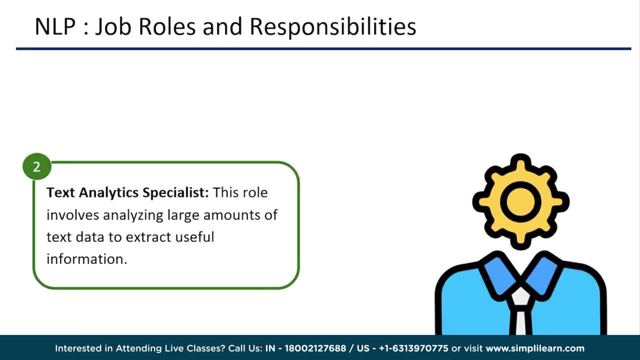 nlp solutions, including building machine learning models, designing pipelines and developing APIs. nlp engineers typically have a background in engineering or computer science and have knowledge of machine learning algorithms, software computing, people using software engineering equipment and management development and data structures. The next we have is text analytics specialist. This role involves 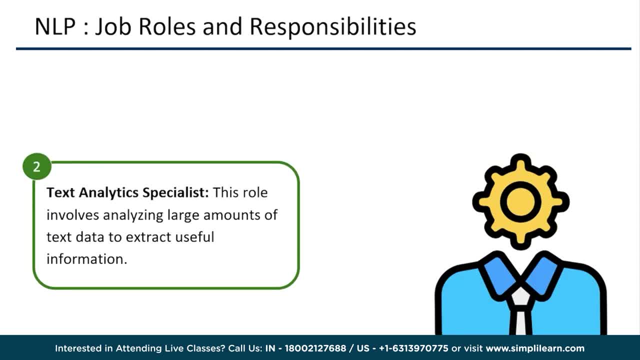 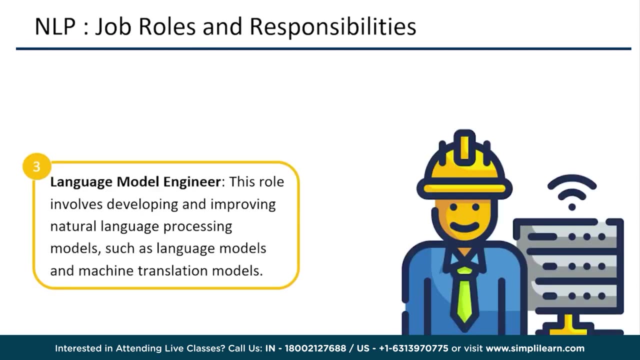 analyzing large amount of text data to extract useful information. Text analytics specialists typically have a background in data analysis, statistics and machine learning, and they use NLP tools and techniques to process and analyze text data. Language model engineer: This role involves developing and improving natural language processing models, such as language models and. 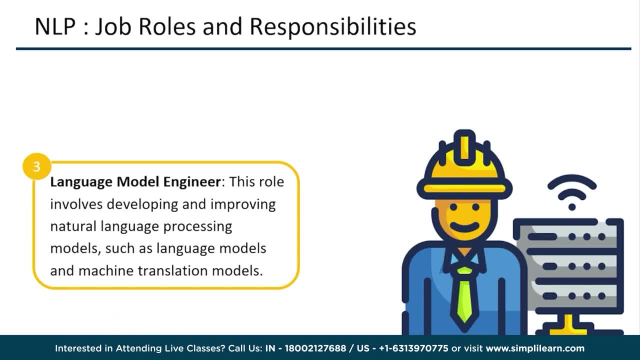 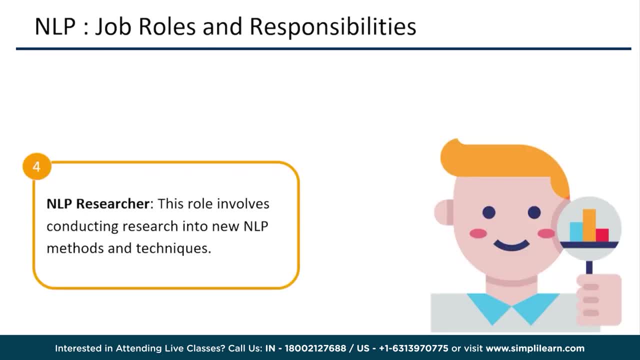 machine translation models. Language model engineers typically have a background in computer science, machine learning and natural language processing. On number four, we have NLP researcher. This role involves conducting research into new NLP methods and techniques. NLP researchers typically have a background in computer science, machine learning and natural language processing. 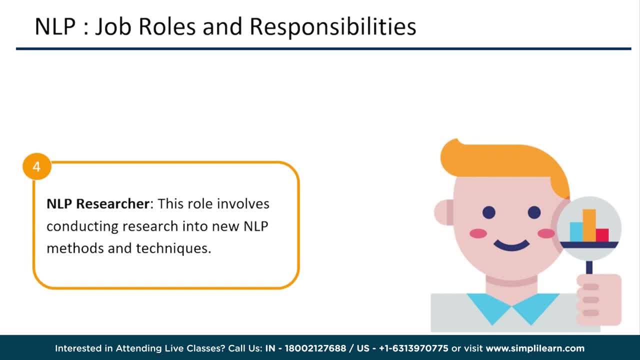 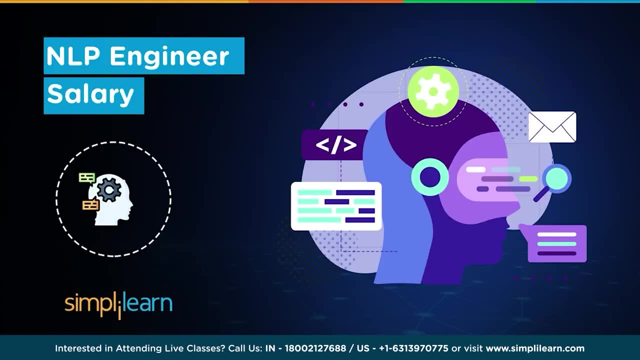 and they publish their research in various academic journals and conferences. And the most awaited. let's start with salary of NLP engineers. Let us now discuss the salary of NLP engineers in India and USA. For the sake of better understanding, we will split up the salary ranges based on the 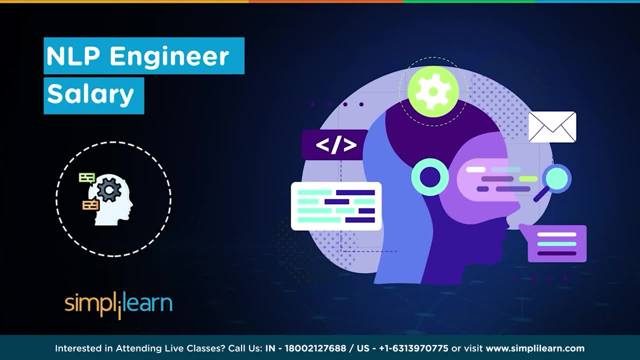 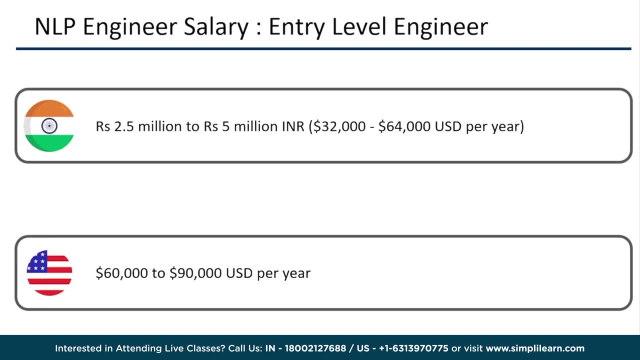 experience level of a professional. So let's start with entry-level NLP engineers. In India, the salary ranges from 2.5 million rupees to 5 million rupees. However, in USA, the salary ranges between $60,000 to $90,000 per year. 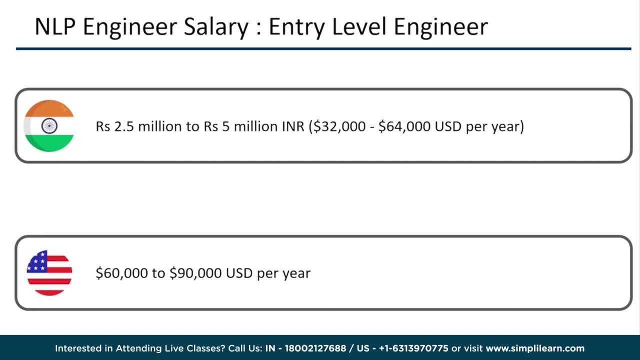 Entry-level NLP engineers typically have background in computer science, engineering or a related field and have some experience with NLP, but may not have yet worked on large scale enterprise projects Moving towards mid-level NLP engineers. these engineers earn 5 million to 8 million rupees per. 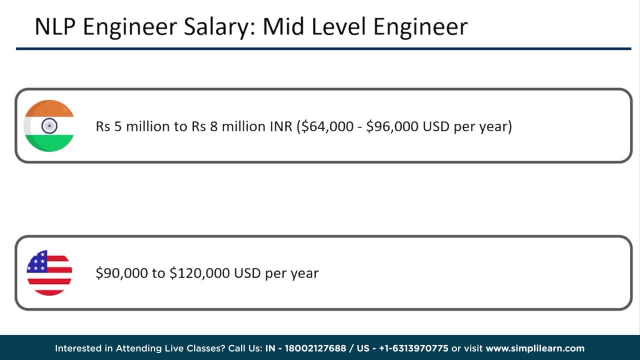 year In United States they earn between ninety thousand dollars to hundred and twenty thousand per year. Mid-level NLP engineers have few years of experience working on NLP projects and are typically comfortable working on both technical and business related aspects of NLP projects. 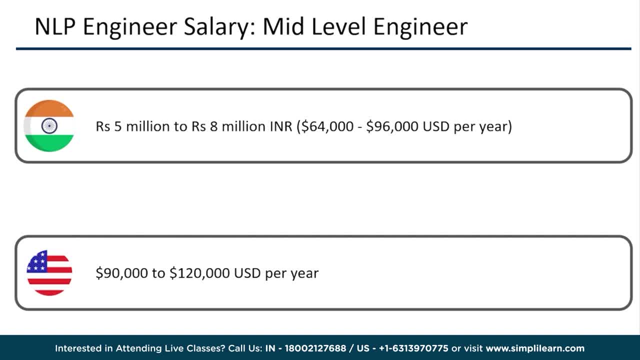 They may have some leadership responsibilities and are often responsible for ensuring that NLP projects are completed on time and to spec. Next, we have a senior level NLP engineers. These engineers earn up to 8 million rupees to 15 million rupees in India per year. 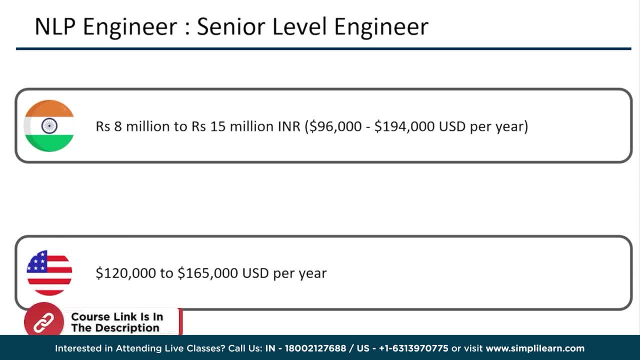 However, in the United States they earn between $120,000 to $165,000 per year. Senior level NLP engineers have extensive experience working on enterprise level NLP projects and are often considered authorities in NLP technologies, methods and tools. 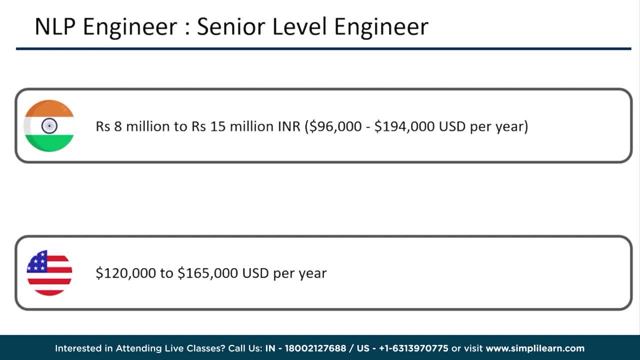 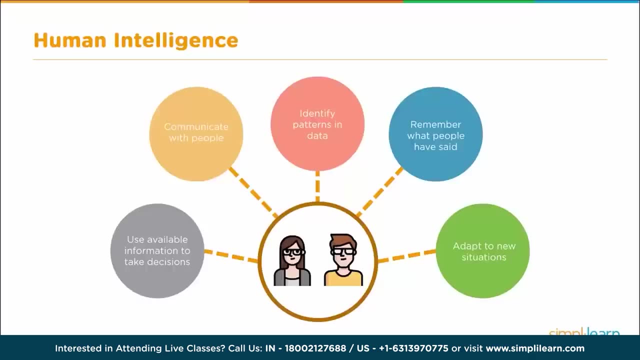 They may serve as subject matter experts, lead teams of engineers and other NLP professionals and be responsible for ensuring the long-term success of NLP projects. Human versus artificial intelligence: Humans are amazing. Let's just face it. We're amazing creatures. We're all over the planet. We're exploring every nook and cranny We've gone to. 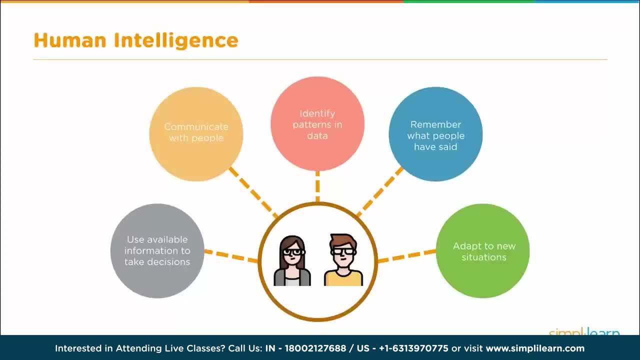 the moon. We've gone into outer space. We're just amazing creatures. We're able to use the available information to make decisions, to communicate with other people, identify patterns and data. remember what people have said: adapt to new situations. So let's take a look at the 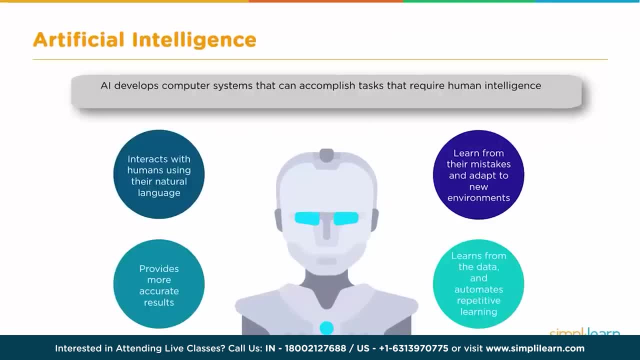 so you can get a picture. You're a human being, so you know what it's like to be human. Let's take a look at artificial intelligence versus the human. Artificial intelligence develops computer systems that can accomplish tasks that require human intelligence. So we're looking at this, One of the things that 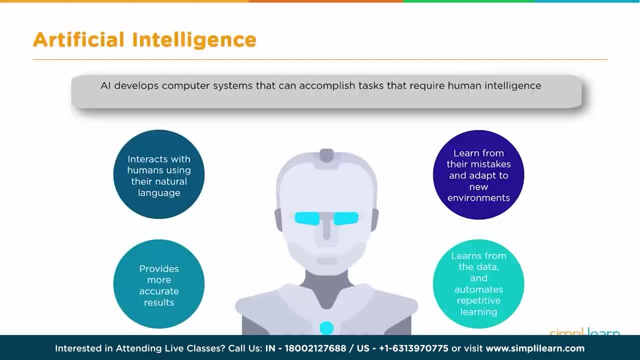 computers can do is they can provide more accurate results. This is very important. Recently I did a project on cancer where it's identifying markers And as a human being, you look at that and you might be looking at all the different images and the data that comes off of them and say I like this. 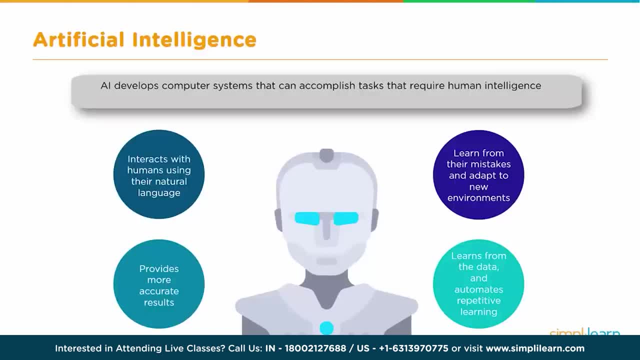 person, So I want to give them a very good outlook. And the next person you might not like, so you want to give them a bad outlook. Well, with artificial intelligence, you're going to get a consistent prediction of what's going to come out. It interacts with humans using their natural language. We've seen that as probably the biggest development feature right now. that's in the commercial market that everybody gets to use, as we saw with the example of Alexa. They learn from. 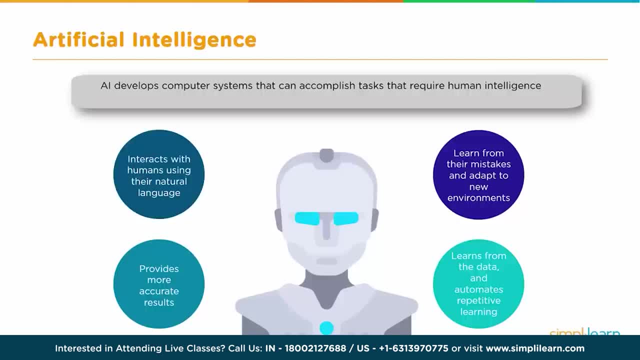 their mistakes and adapt to new environments. So we see this slowly coming in more and more And they learn from the data and automate repetitive learning. Repetitive learning has a lot to do with the neural networks. You have to program thousands upon thousands of pictures in there and it's all automated. So, as today's computers evolve, it's very quick and easy and affordable to do this. What is machine learning and deep learning all about? Imagine this. 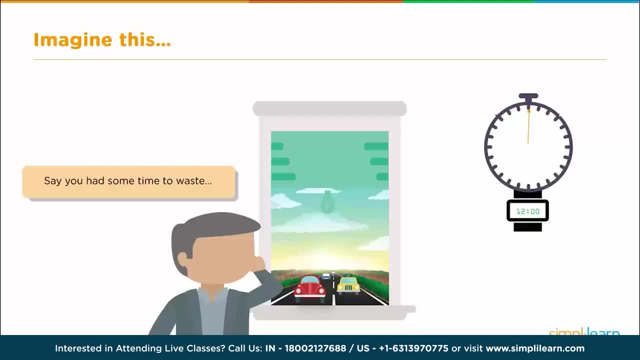 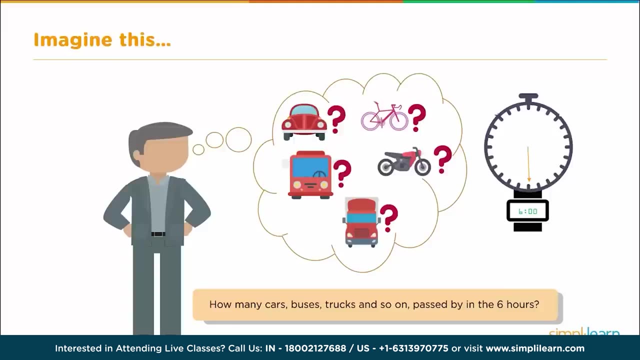 Say you had some time to waste- Not that any of us really have a lot of time anymore to just waste in today's world- And you're sitting by the road and a whole lot of time passes by. Here's a few hours And suddenly you wonder how many cars, buses, trucks and so on passed by in the six hours. Now, chances are you're not going to sit by the road for six hours and count buses, cars and trucks, unless you're working for the city and you're trying to do city planning And you want to know: hey, do we need to add a new truck route? 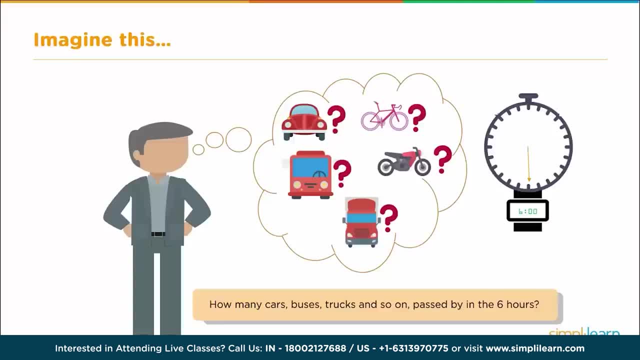 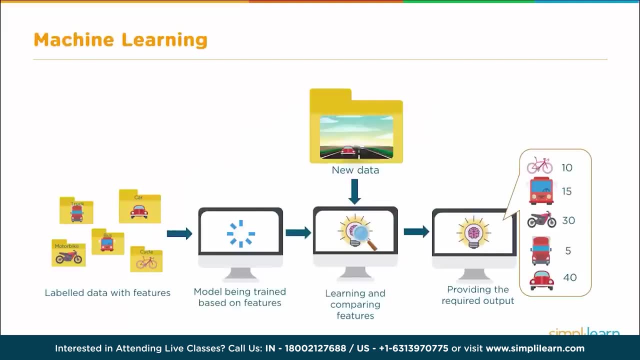 Maybe we need a bicycle lane because we have a lot of bicyclists here, That kind of thing. So maybe city planning would be great for this Machine learning. Well, the way machine learning works is we have labeled data with features. So you have a truck or a car, a motorcycle, a bus or a bicycle, and each one of those are labeled. 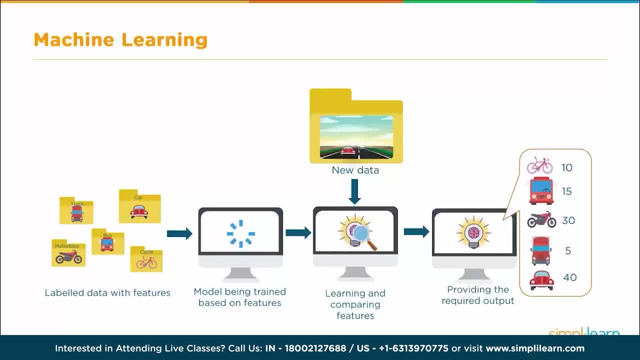 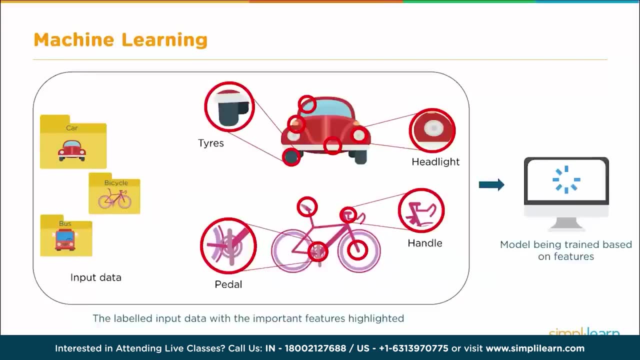 It comes in and, based on those labels and comparing those features, it gives you an answer: It's a bicycle, It's a truck, It's a motorcycle. Let's look a little bit more in depth on this. In the model here, it actually the features we're looking at would be like the tires. 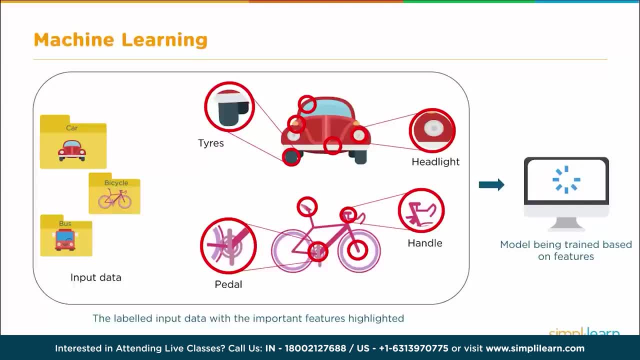 Someone sits there and figures out what a tire looks like. It takes a lot of work If you try to figure the difference between a car tire, a bicycle tire, a motorcycle tire. So in the machine learning field this could take a long time if you're going to do each individual aspect of a car and try to get a result on there. 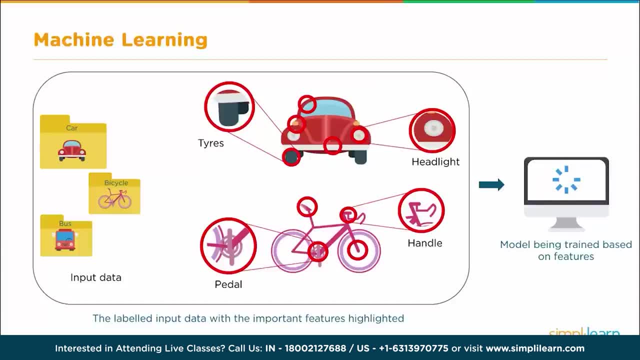 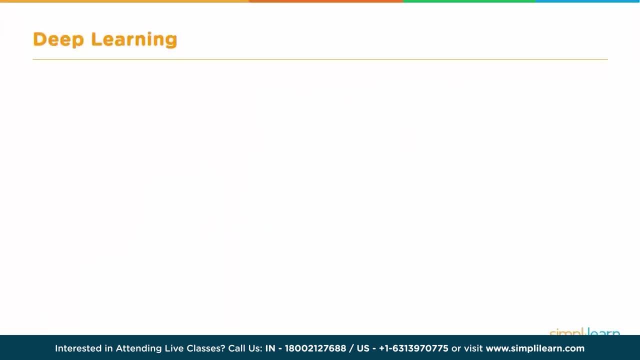 And that's what they did do. This is still used. We've used it for a number of reasons. It's probably a little more than a 10-year-old car, But what we found- and it would be useful to do a little more in depth for everybody- is that you can take small amounts of data, smaller amounts of data, and you figure out what those features are and then you label them. 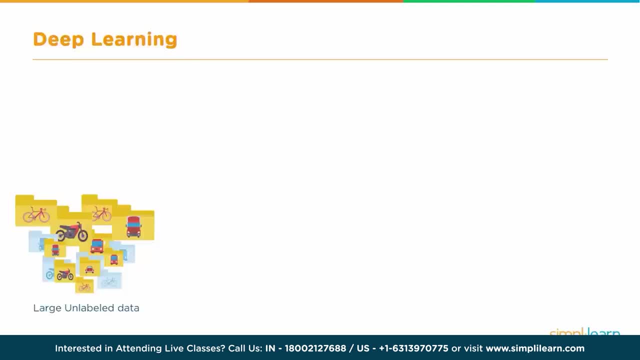 Deep learning. So with deep learning, one of our solutions is to take a very large unlabeled data set and we put that into a training model using artificial neural networks And then that goes into the neural network itself and we create a neural network. 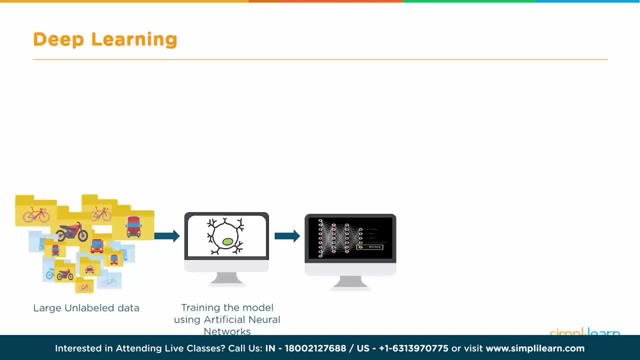 And you'll see, The arrows are actually kind of backward. the bicycle in and then it comes back and says if it's a truck? it comes back and says, well, you need to change that to bicycle. and then it changes all those weights going backward. they call it back. 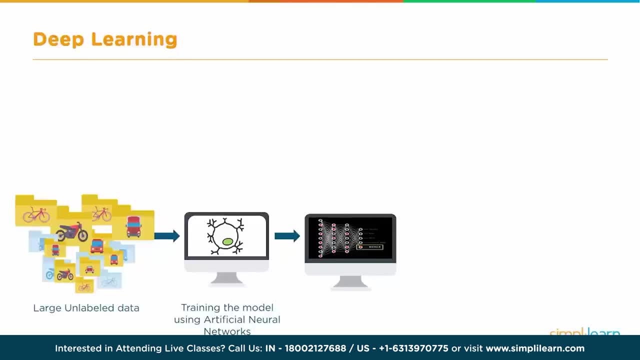 propagation and let it know it's a bicycle and that's how it learns. once you've trained the neural network, you then put the new data in and they call this testing the model. so you need to have some data you've kept off to the side where you know the answer to, and you take that and you 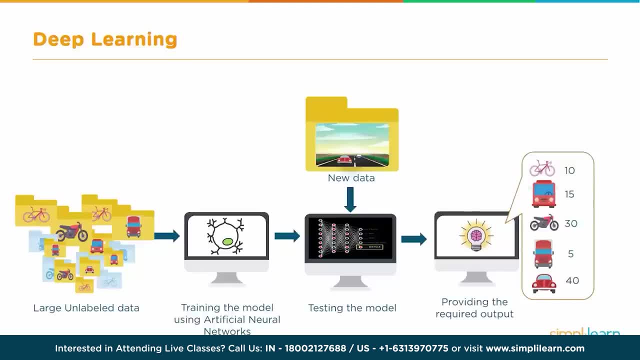 provide the required output and you say, okay, is this? is this neural network working correctly? did it identify a bike as a bike, a truck as a truck, a motorcycle as a motorcycle? let's just take a little closer look at that, determining what objects are present in the data. so how does deep learning 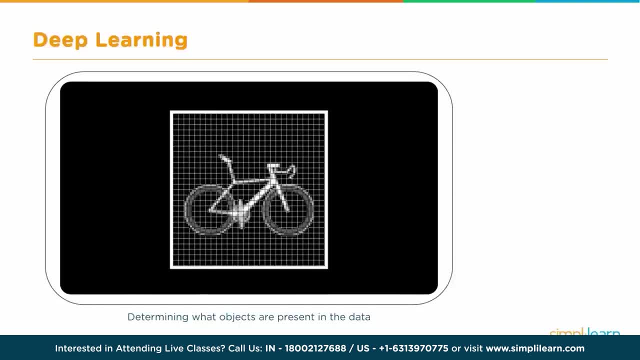 do this and here we have the image of the bike. it's 28 by 28 pixels. that's a lot of information there. could you imagine trying to guess that this is a bicycle image by looking at each one of those pixels and trying to figure out what's around it? and we actually do that as human beings. it's. 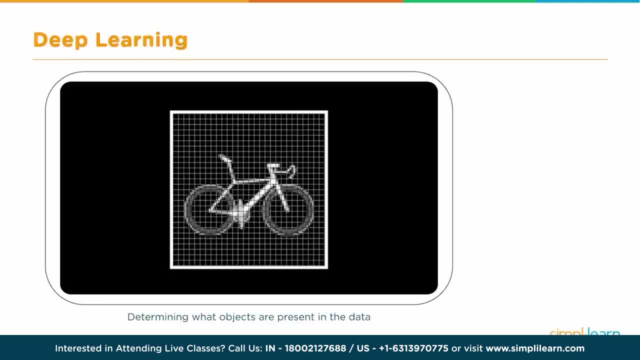 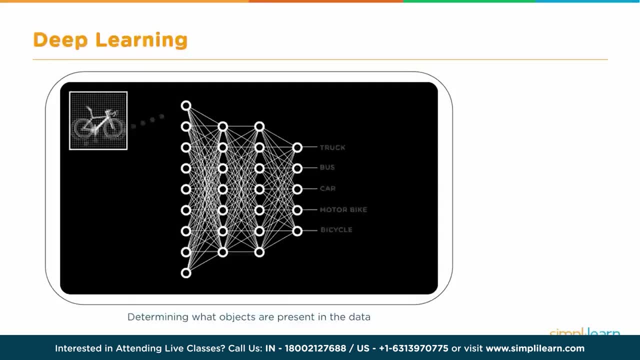 pretty amazing. we know what a bicycle is and even though it comes in as all this information and what this looks like is the image comes in, it converts it into a bunch of different nodes- in this case, there's a lot more than what they show here- and it goes through these different layers and outcomes and says, okay, this is a bicycle- a lot. 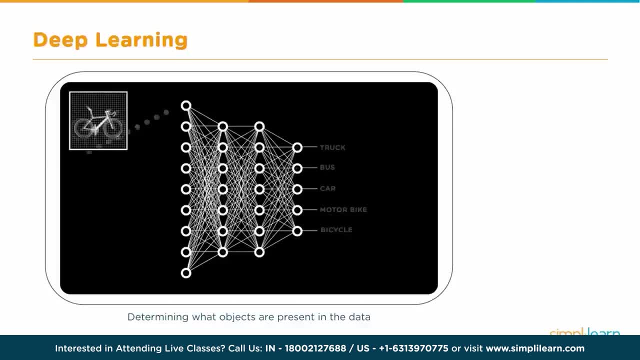 of times they call this the magic black box. why? because as we watch it go across here all these weights and all the math behind this, and it's not. it's a little complicated on the math side. you really don't need to know that when you're. 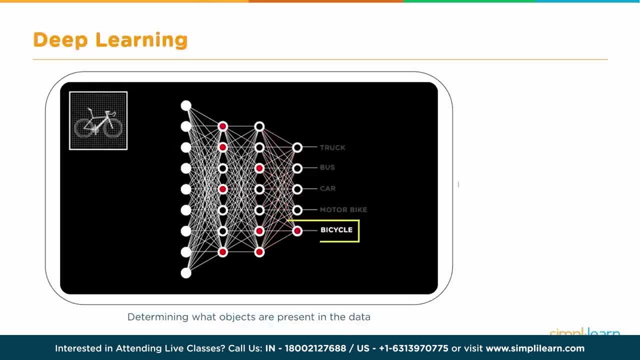 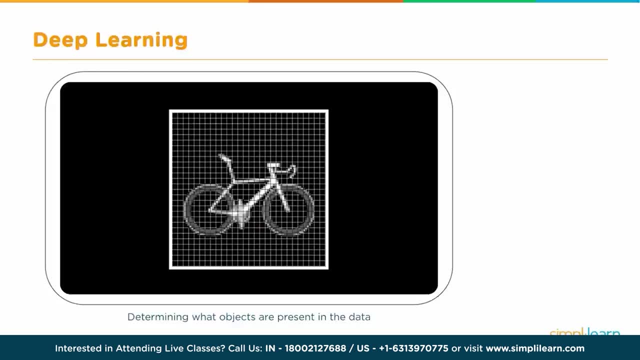 programming or doing working with the deep learning, but it's like magic. you don't know. you really can't figure out what's going to come out by looking, what's in each one of those dots and each one of those lines are firing and what's going in between them. so we like to call it the 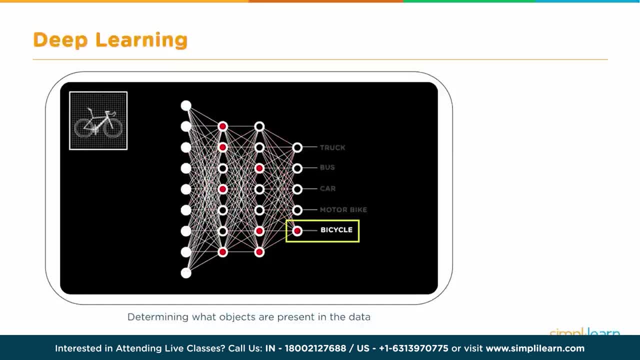 magic box. so that's where deep learning comes in. and in the end it comes up and you have this whole neural network. it comes up and it says, okay, we fire all these different pixels and we connects all these different dots and gives them different weights, and it says, okay, this is a bicycle and 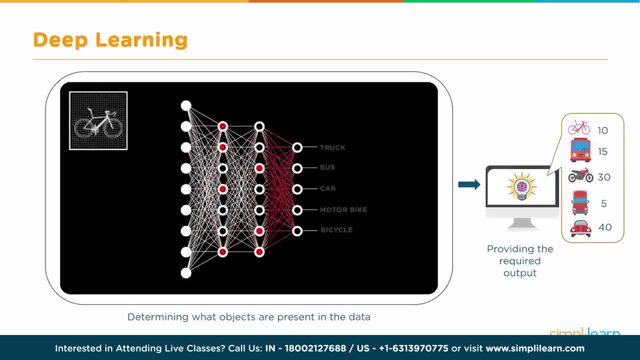 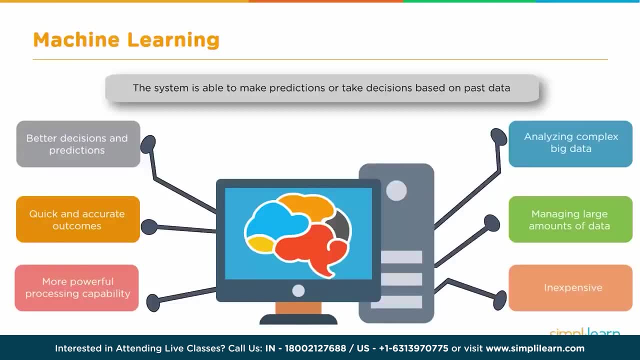 that's how we determine what the object is present in the data: machine learning. we're gonna take a step into machine learning here and you'll see how these fit together in a minute. the system is able to make predictions or take decisions based on past data, as very important for machine learning is that we're looking at stuff and based on what's. 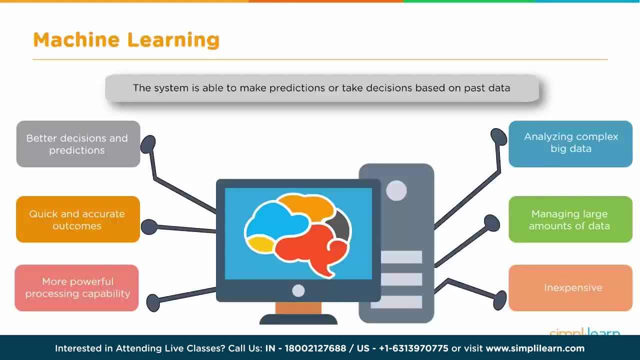 been there before. we're creating a decision on there, creating something out of their coloring a beach ball. we're telling you what the weather is in chicago. but it's nice about machine learning- a very powerful processing capability. It's quick and accurate outcomes, so you get results right. 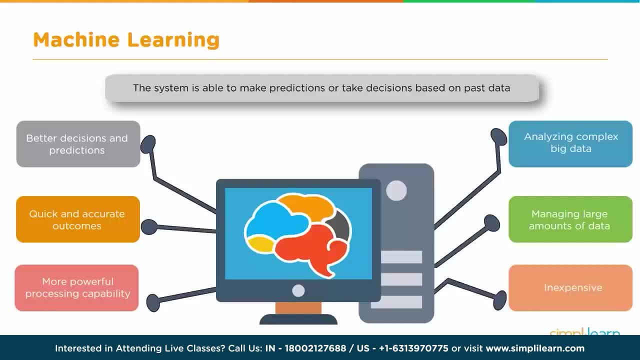 away. Once you program the system, the results are very fast and the decisions and predictions are better. They're more accurate. They're consistent. You can analyze very large amounts of data. Some of these data things that they're analyzing now are petabytes and terabytes of data. 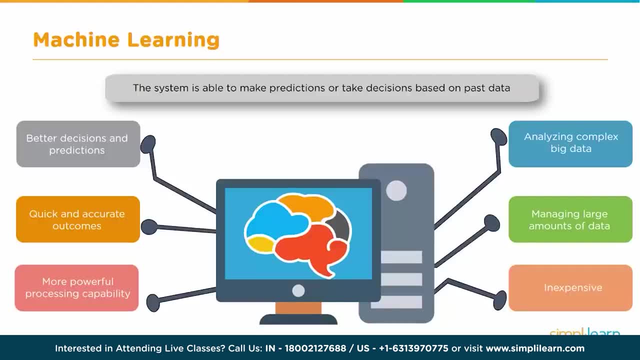 It would take hundreds of people, hundreds of years, to go through some of this data and do the same thing that the machine learning can do in a very short period of time, And it's inexpensive compared to hiring hundreds of people, So it becomes a very affordable way to move into the 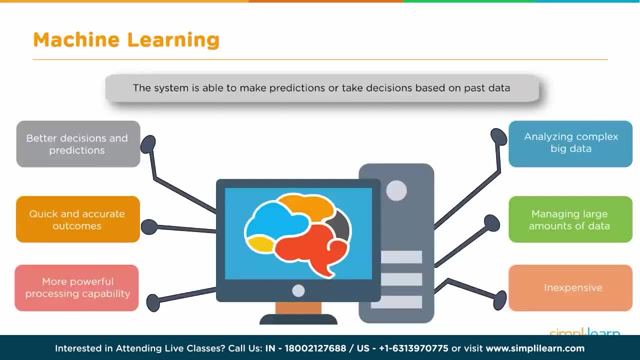 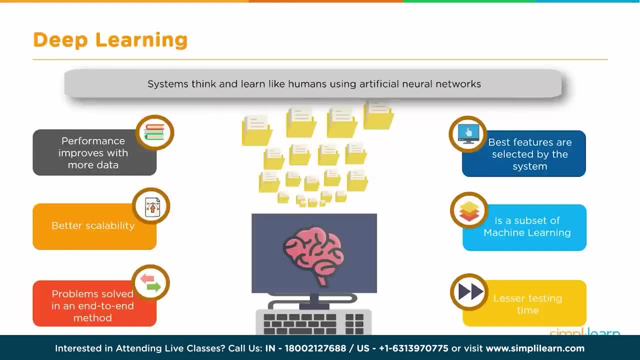 future is to apply the machine learning to whatever businesses you're working on, And deep learning Systems think and learn like humans using artificial neural networks. Again, it's like a magic box. Performance improves with more data, So the more data that deep learning. 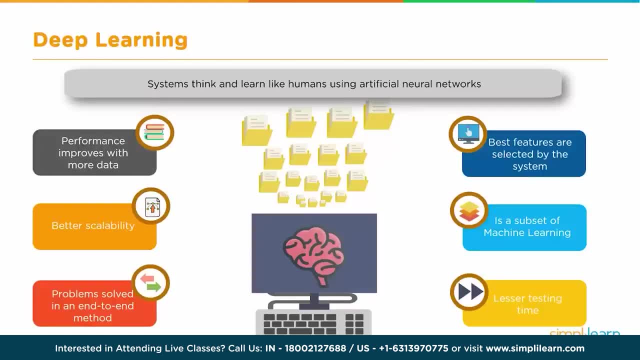 gets, the more it gives you better results. It's scalability, So you can scale it up, You can scale it down. You can increase what you're looking at Currently. you know we're limited by the amount of computer processing power as to how big that can get. 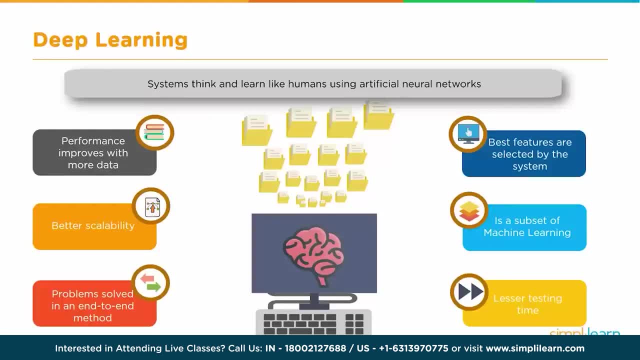 But that envelope continually gets pushed every day on what it can do. Problem solved in an end-to-end method. So instead of having to break it apart and you have the first piece coming in and you identify tires and the second piece is identifying labeling, handlebars, and then you bring that. 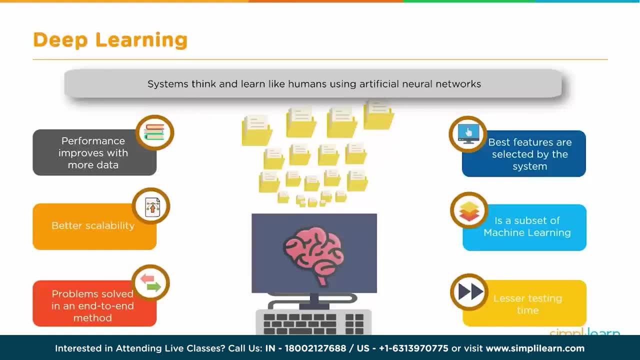 in, And if it has handlebars and tires, it's a bicycle, And if it has something that looks like a large square it's probably a truck. The neural networks does this all in one network. You don't really know what's going on in all those weights and all those little bubbles, But it does it pretty much in one. 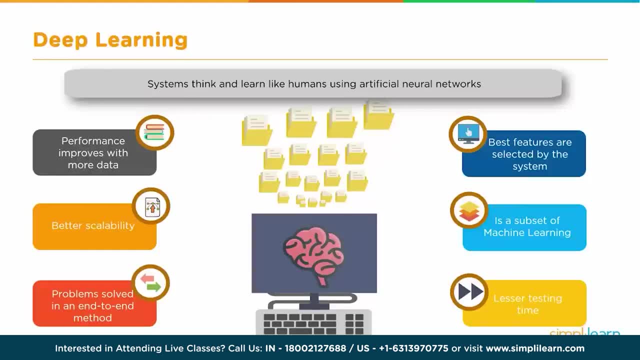 package. That's why the neural network systems are so big nowadays and coming into their own. Best features are selected by the system, And this is important. They kind of put it on a bullet on the side here. It's a subset of machine learning. It's a subset of machine learning. It's a subset of machine. 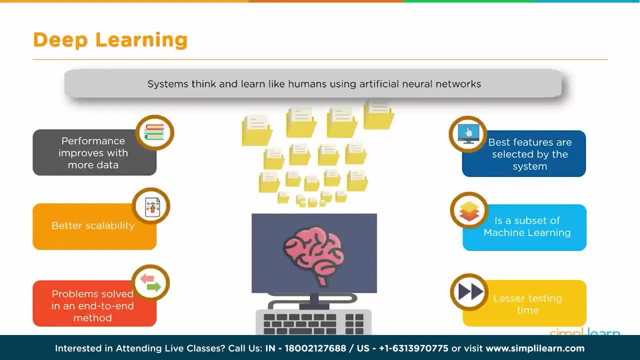 learning. This is important. We talk about deep learning. It is a form of machine learning. There's lots of other forms of machine learning- data analysis- But this is the newest and biggest thing: that they apply to a lot of different packages And they use all the other machine learning tools. 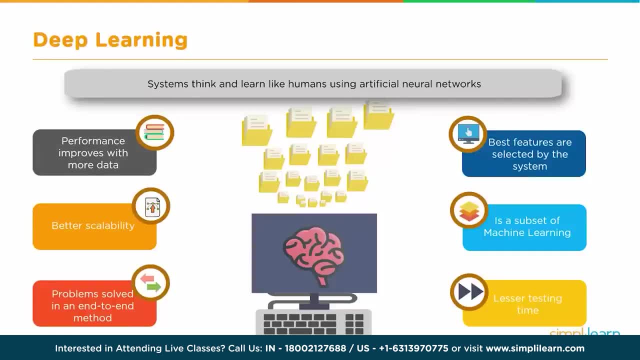 available to work with it And it's very fast to test. You put in your information, You then have your group of tests And then you held some aside. You see how does it do. It's very quick to test it and see what's going on with your deep learning and your neural networks. 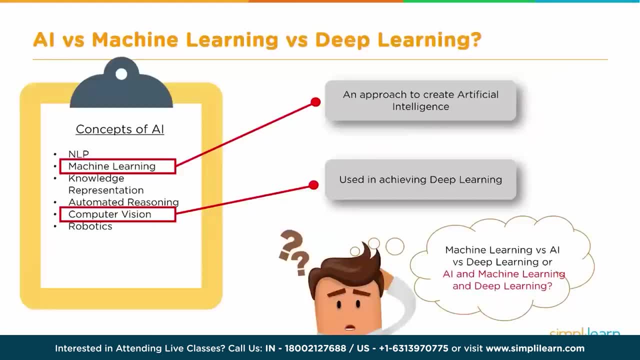 Are they really all that different- AI versus machine learning, versus deep learning, Concepts of AI. So we have concepts of AI. you'll see, Natural Language Processing, Machine learning, an approach to create artificial intelligence, so it's one of the subsets of artificial intelligence. 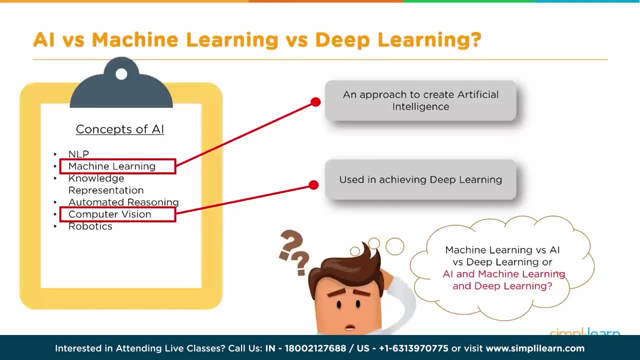 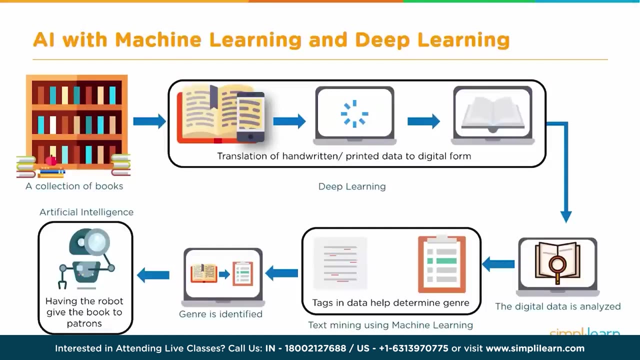 Knowledge representation, automated reasoning, computer vision, robotics, Machine learning versus AI versus deep learning or AI and machine learning, machine learning and deep learning. So, when we look at this, we have AI with machine learning and deep learning, And so we're gonna put them all together. 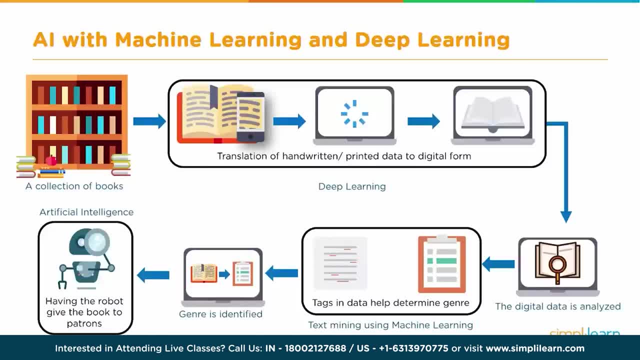 We find out that AI is the big picture. We have a collection of books that goes through some deep learning. the digital data is analyzed, text mining comes through the particular book you're looking for- maybe it's a genre of books- is identified and in this case we have a robot. 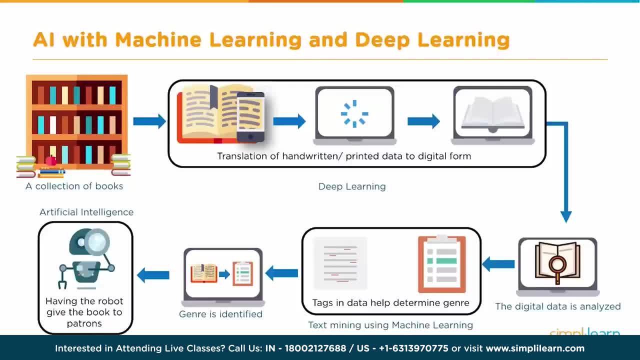 that goes and gives a book to the patron. I have yet to be at a library that has a robot: bring me a book, but that will be cool when it happens. So we'll look at some of the pieces here. This information goes into as far as this example. 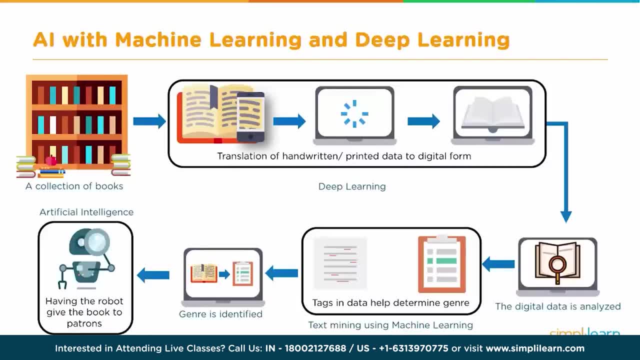 the translation of the handwritten, printed data to digital form. That's pretty hard to do. That's pretty hard to go in there and translate hundreds and hundreds of books and understand what they're trying to say if you've never read them. So in this case, we use the deep learning. 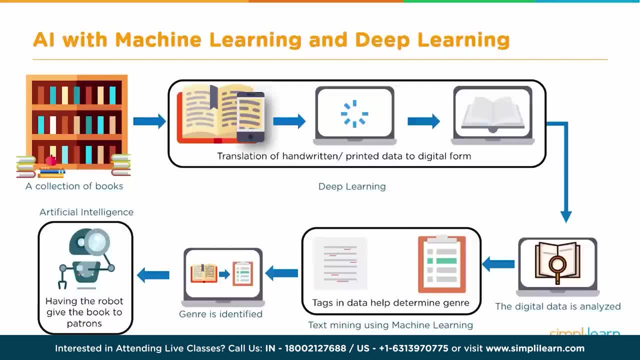 because you can already use examples where they've already classified a lot of books, and then they can compare those texts and say: oh okay, this is a book on automotive repair, this is a book on robotic building. The digital data is then analyzed, then we have more. 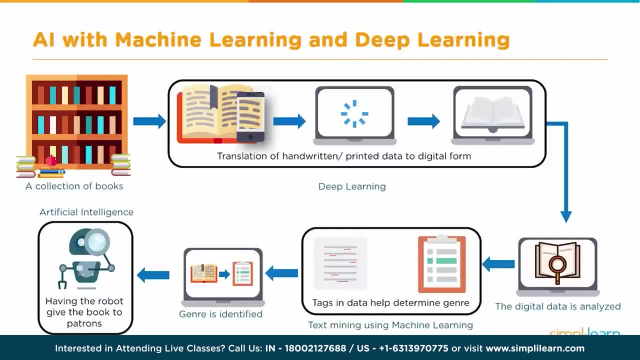 text mining using machine learning. so maybe we'd use a different program to do a basic: classify what you're looking for and say: oh, you're looking for auto repair and computers, so you're looking for automated cars. Once it's identified, then of course it brings. 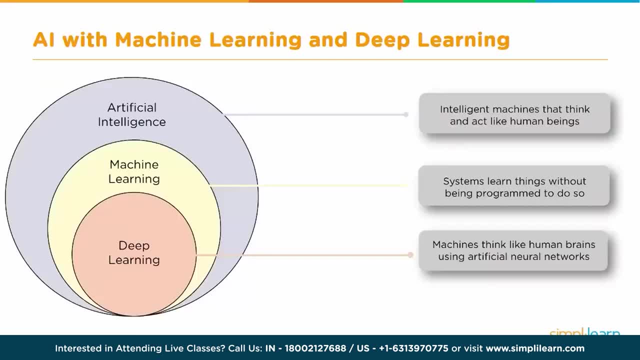 you the book. So here's a nice summation of what we were just talking about: AI with machine learning and deep learning. Deep learning is a subset of machine learning, which is a subset of artificial intelligence, So you can look at artificial intelligence as the big picture. 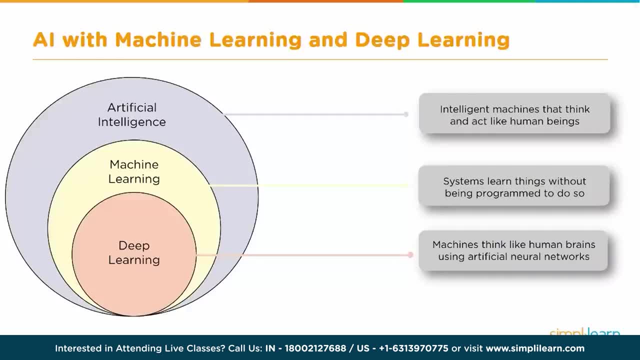 How does this compare to the human experience in either doing the same thing as a human? we do or does it better than us? And machine learning, which has a lot of tools, is something that learns from data, past experiences. It's programmed. 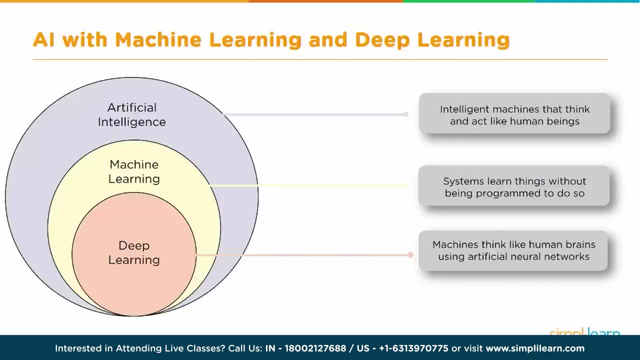 It comes in there and it says, hey, we already had these five things happen. The sixth one should be about the same. And then there's a lot of tools in machine learning, but deep learning, then, is a very specific tool in machine learning. 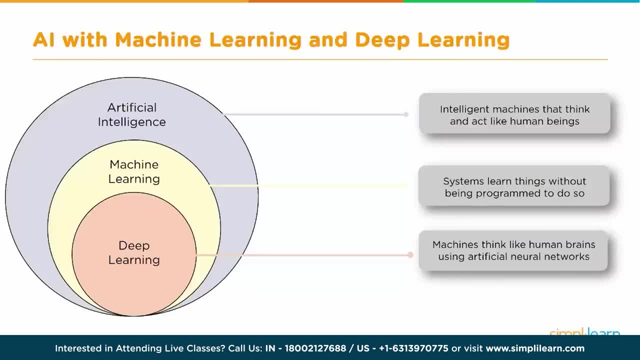 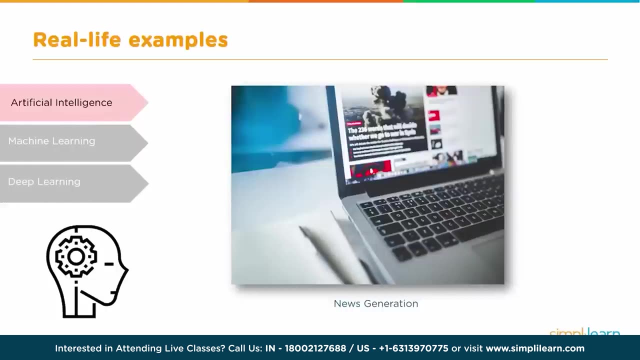 It's the artificial neural network which handles large amounts of data and is able to take huge pools of experiences, pictures and ideas and bring them together. Real life examples: Artificial intelligence: news generation- very common nowadays, as it goes through there and finds the news articles or 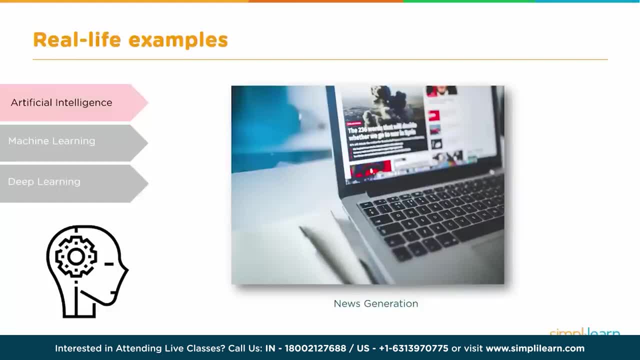 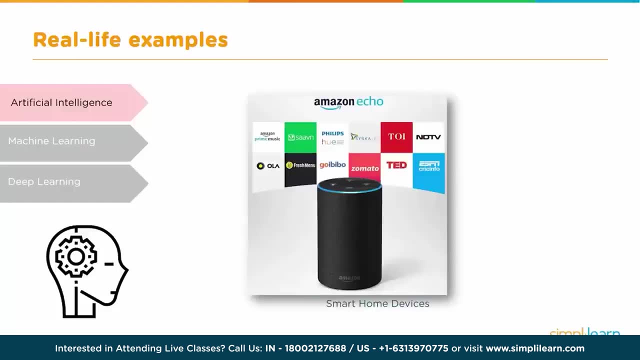 generates the news based upon the news feeds or the back end, coming in and says: OK, let's give you the actual news based on this. There's all the different things: Amazon Echo- They have a number of different Prime Music on there. 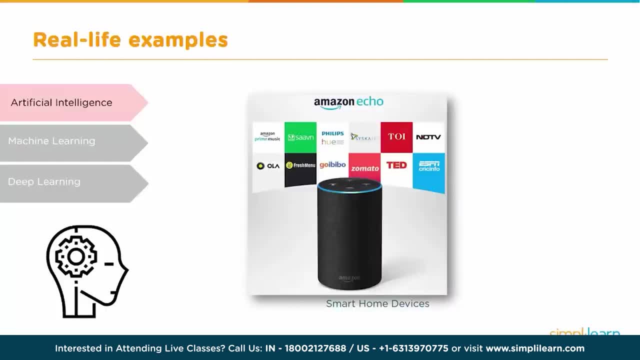 Of course, there's also the Google Command, and there's also Cortana. There's tons of smart home devices. Now we can ask it to turn the TV on or play music for us. That's all artificial intelligence From front to back. you're having a human experience. 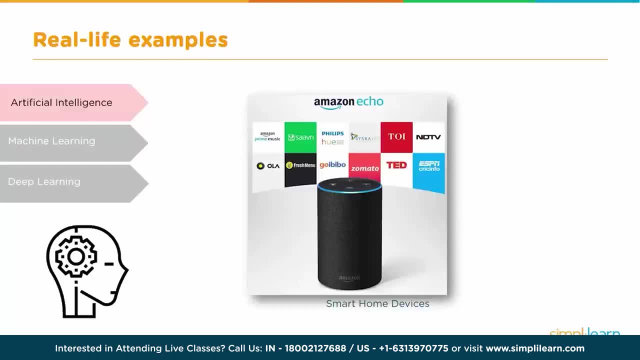 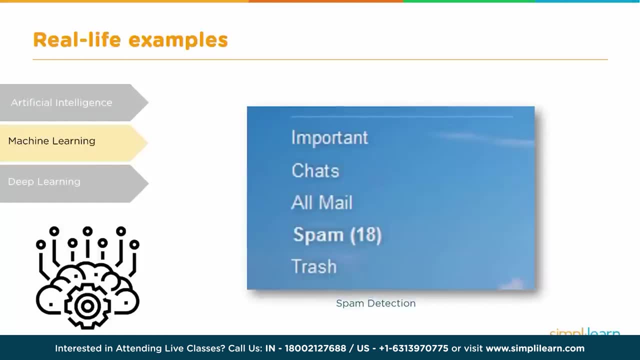 with these computers and these objects that are connected to the processing Machine learning, spam detection- very common. Machine learning doesn't really have the human interaction part, So this is the part where it goes and says: OK, that's a spam, that's not a spam. 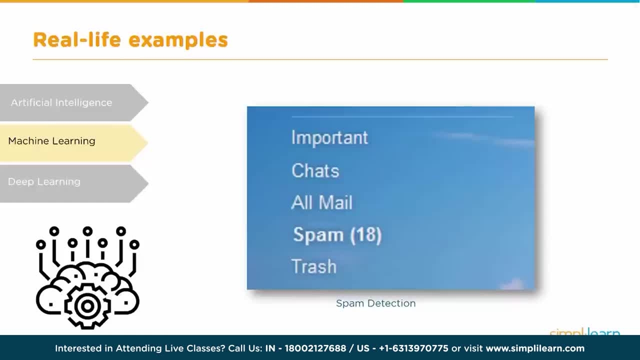 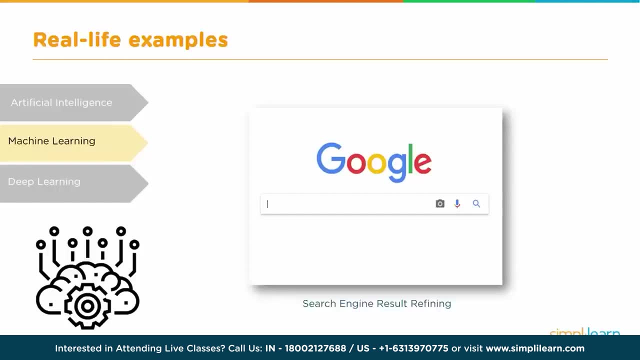 And it puts it in there. And that's it. It puts it in your spam folder. Search engine result refining- another example of machine learning, whereas it looks at your different results and it is able to categorize them. as far as this had the most hits, 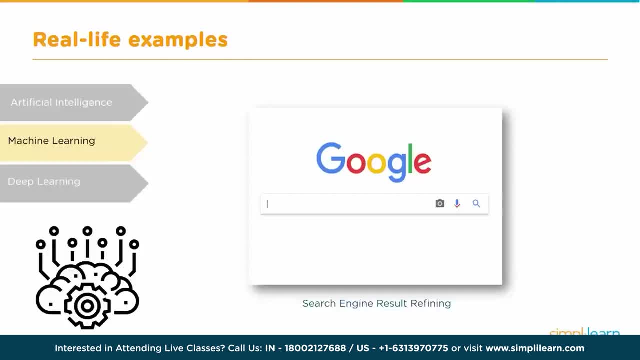 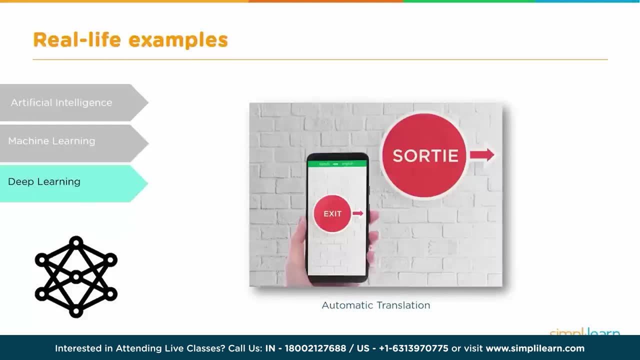 this is the least viewed. this has five stars. however, they want to weight it. All good examples of machine learning. And then the deep learning, Deep learning. another example is, as you have an exit sign, in this case it's translating it. 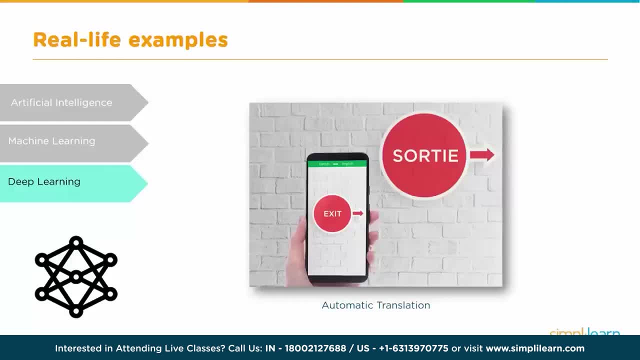 It's translating it into French: sortie. I hope I said that right. The neural network has been programmed with all these different words and images, and so it's able to look at the exit in the middle and it goes OK. we want to know what that is in. 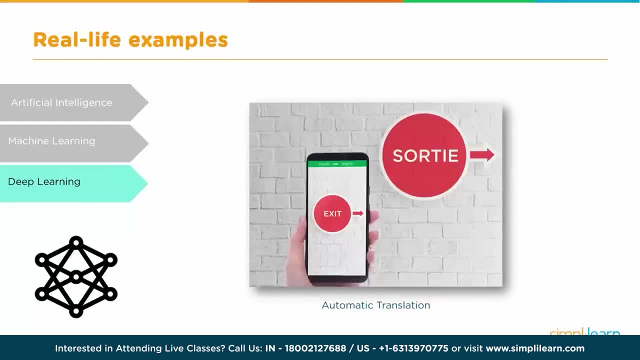 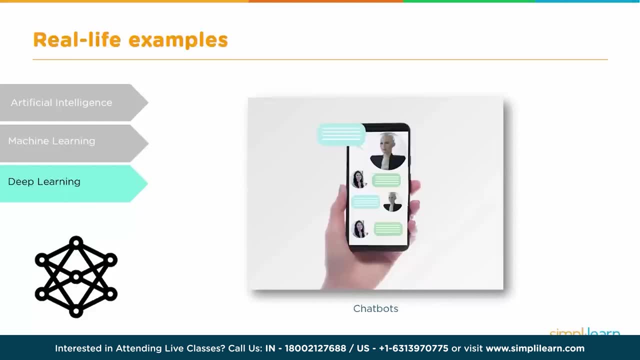 French and it's able to push that out in French and learn how to do that. And then we have chat bots. I remember when Microsoft first had their little paper clip boy. that was like a long time ago that came up and you would type: 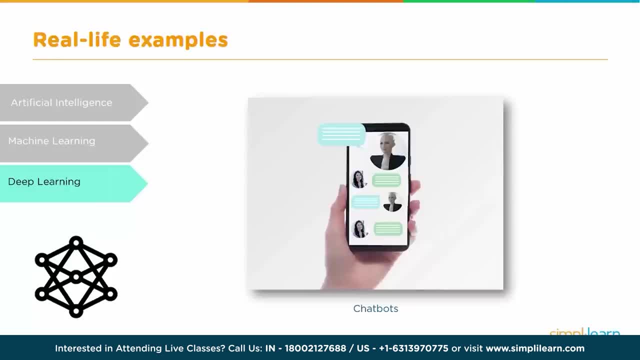 in there and chat with it. These are growing. you know, it's nice to just be able to ask a question and it comes up and gives you the answer And instead of it being where you're just doing a search on certain words. 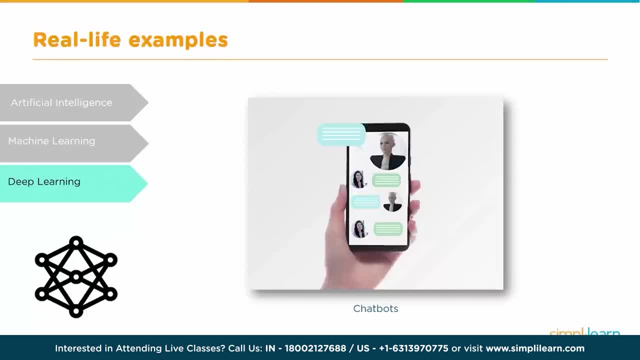 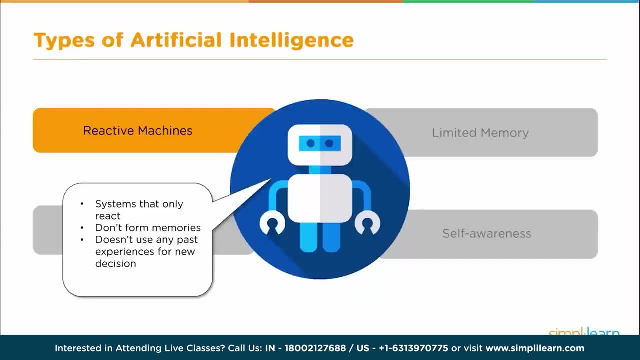 it's now able to start linking those words together and form a sentence in that chat box. Types of AI and machine learning- Types of artificial intelligence. This and the next few slides are really important. So one of the types of artificial intelligence is reactive machines. 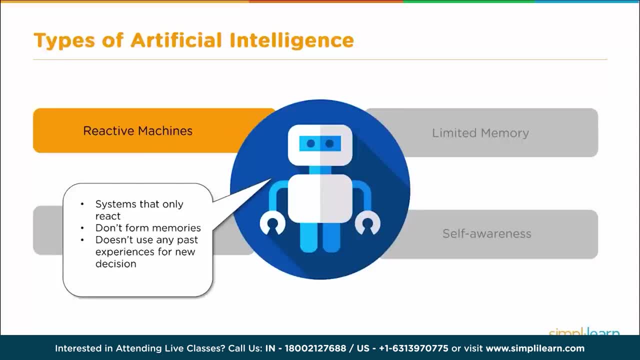 Systems that only react. They don't form memories, They don't have past experiences. They have something that happens to them and they react to it. My washing machine is one of those. If I put a ton of clothes in it and they get all clumped on one. 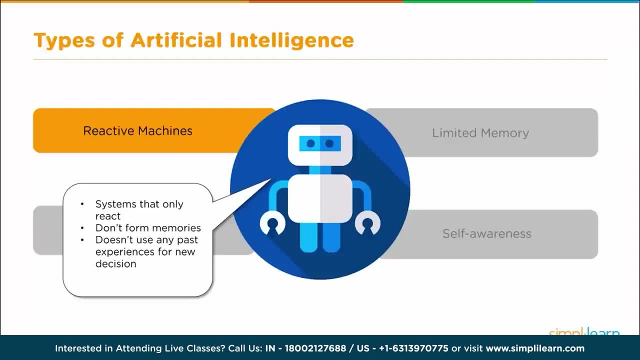 side, it automatically adds a weight to re-center it. So my washing machine is actually a reactive machine, working with whatever the load is and keeps it nice, And so when it spins it doesn't go thumping against the side. Limited memory. 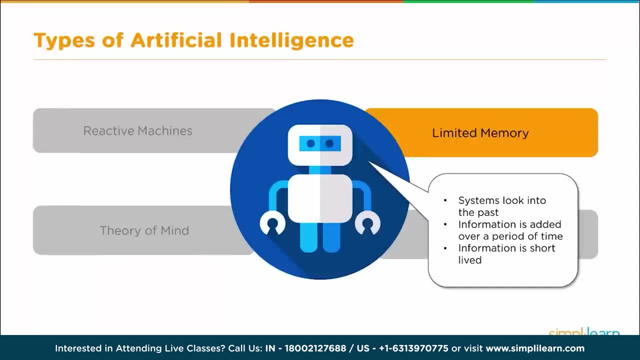 Another form of artificial intelligence Systems. look into the past. Information is added over a period of time And information is short-lived. When we're talking about this and you look at like a neural network that's been programmed to identify cars, it doesn't remember all those pictures. 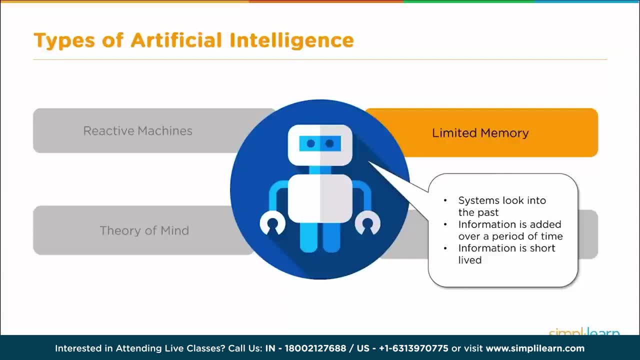 It has no memory as far as the hundreds of pictures you process through it. All it has is: this is the pattern I used to identify cars as the final output for that neural network we looked at. So when they talk about limited memory, this is what they're talking about. 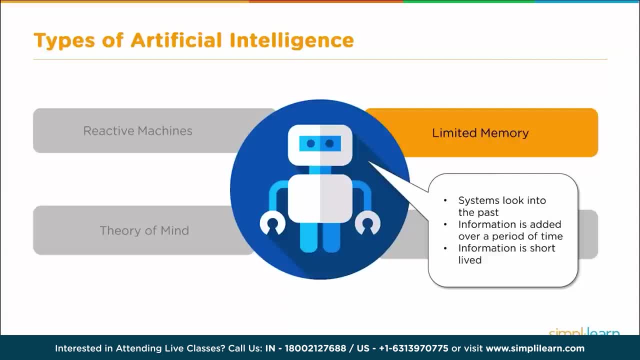 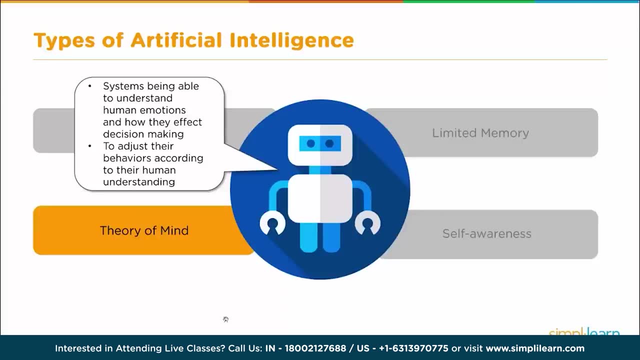 They're talking about. I've created this based on all these things, but I'm not going to remember any one. specifically Theory of mind Systems being able to understand human emotions and how they affect decision-making, to adjust their behaviors according to their human understanding. 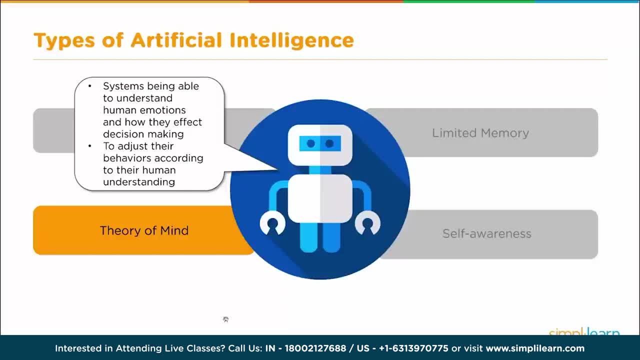 This is important because this is our page mark. This is how we know whether it is an artificial intelligence or not. Is it interacting with humans in a way that we can understand? Without that, interaction is just an object. So we talk about theory of mind. 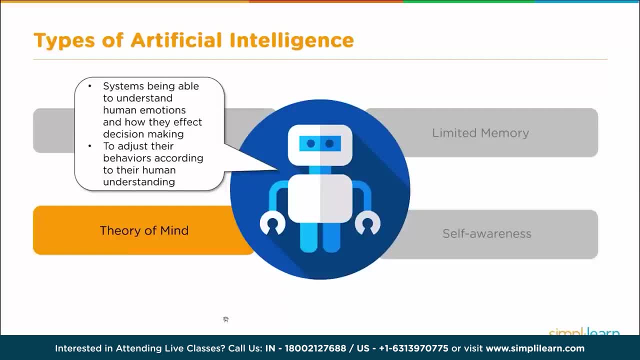 We really understand how it interfaces that whole. if you're in web development, user experience would be the term I would put in there. So the theory of mind would be user experience. How is the whole UI connected together? And one of the final things is, as we get into artificial intelligence, is systems being? 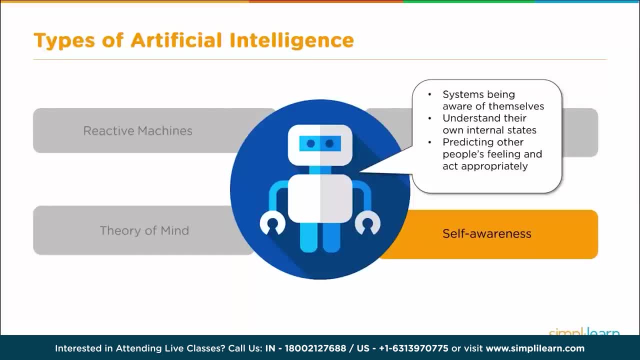 aware of themselves, understanding their internal states and predicting other people's feelings and act appropriately. So as artificial intelligence continues to progress, we see ones that are trying to understand well what makes people happy. How would they increase our happiness? How would they keep themselves from breaking down if something's broken inside? 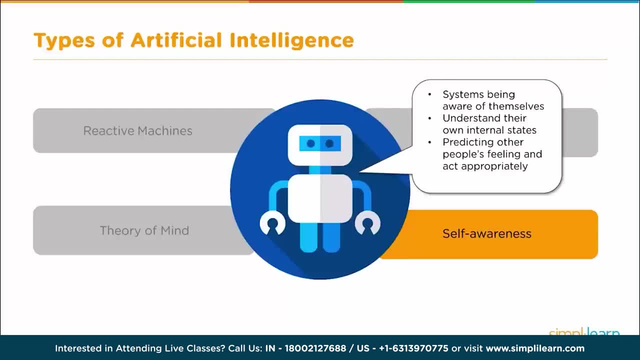 They have that self-awareness to be able to fix it And, just based on all that information, predicting which action would work the best. What would help people? If I know that you're having a cup of coffee first thing in the morning is what makes you. 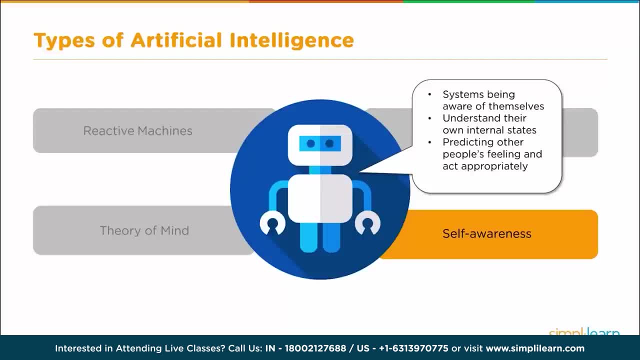 happy. as a robot, I might make you a cup of coffee every morning at the same time to help your life and help you grow. That would be the self-awareness It's being able to know all those different things. Types of machine learning. 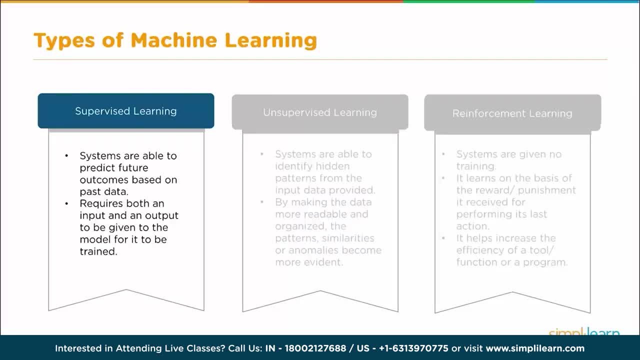 And, like I said on the last slide, this is very important. This is very important If you decide to go in and get certified in machine learning or know more about it. these are the three primary types of machine learning. The first one is supervised learning. 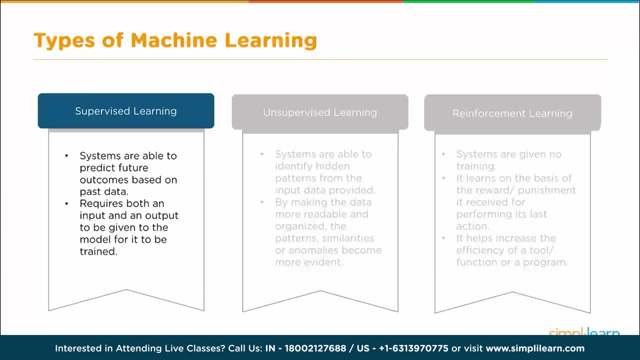 Systems are able to predict future outcome based on past data Requires both an input and an output to be given to the model for it to be trained. So in this case We're looking at anything where you have a hundred images of a bicycle and those hundred 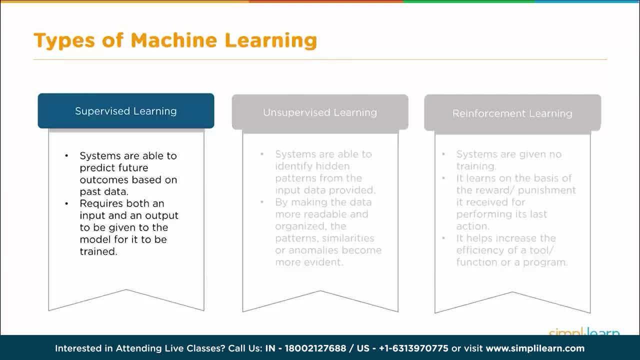 images you know are bicycle, So it's their preset. Someone already looked at all hundred images and said: these are pictures of bicycles And so the computer learns from those. and then it's given another picture and maybe the next picture is a bicycle and it says: oh, that resembles all these other bicycles. 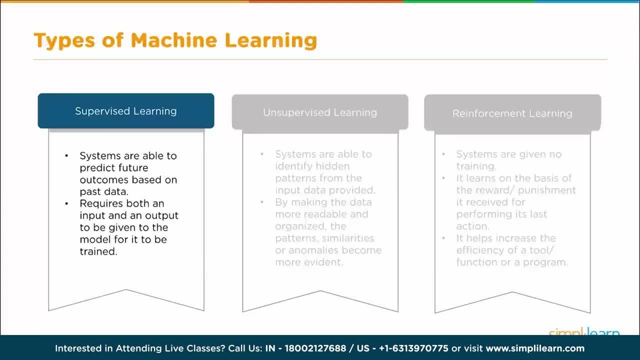 So it's a bicycle And the next one's a car and it says, eh, it's not a bicycle, That would be supervised learning, because we had to train it, We had to supervise it. So that's the third one: Unsupervised learning. 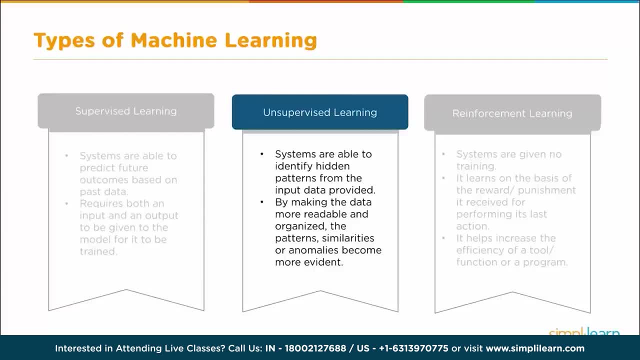 Systems are able to identify hidden patterns from the input data provided. by making the data more readable and organized, The patterns, similarities or anomalies become more evident. You'll heard the term cluster. How do you cluster things together? Some of these things go together. 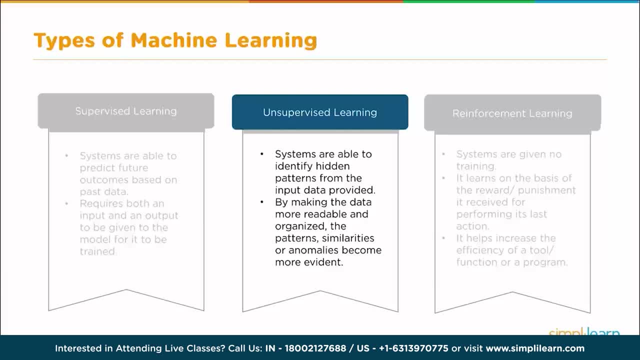 Some of these don't. This is unsupervised, where it can look at an image and start pulling the different pieces of the image out because they aren't the same. The human, all the parts of the human, are not the same as a fuzzy tree behind them, just. 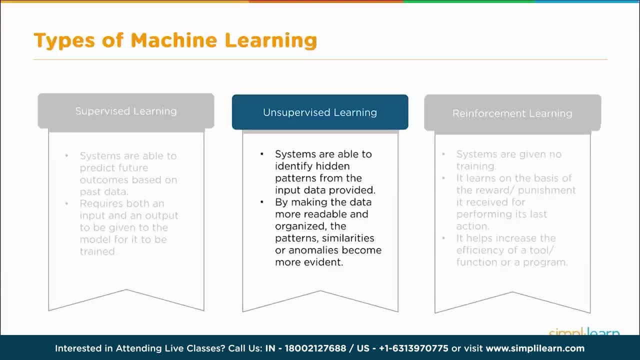 slightly out of focus, which is not the same as the beach ball. It's unsupervised, because we never told it what a beach ball was, We never told it what the human was and we never told it that those were trees. All we told it was: hey, separate this picture by things that don't match and things that 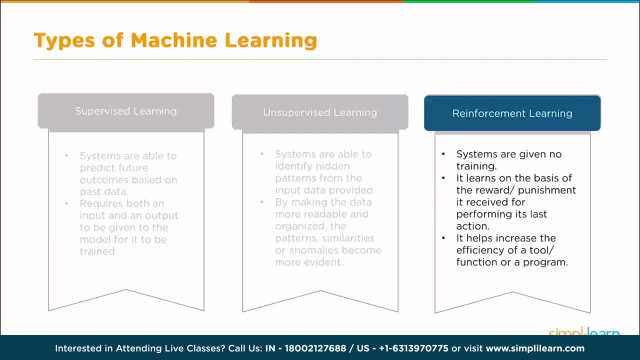 do match and come together. And finally there's reinforcement learning. Systems are given no training. It learns on the basis of the reward punishment it received for performing its last action. It helps increase the efficiency of a tool, function or a program. Reinforced learning or reinforcement learning is kind of you. give it a yes or no. 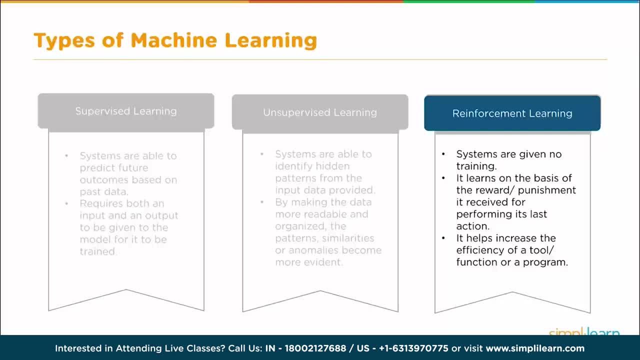 Yes, you gave me the right response, No, you didn't. And then it looks at that and says, oh, okay, so based on this data coming in, what I gave you was a wrong response, so next time I'll give you a different one. 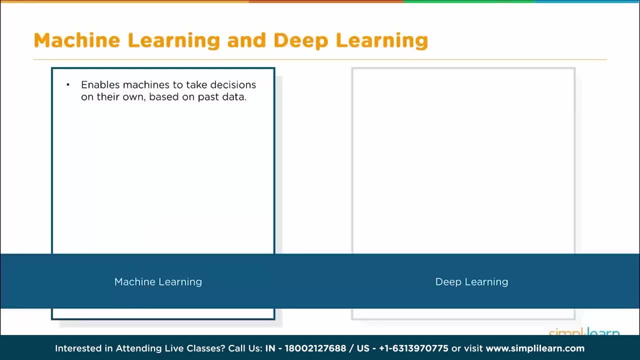 Comparing machine learning and deep learning. So remember that deep learning is a subcategory of machine learning, So it's one of the many tools, And so we're grouping a ton of machine learning tools all together. There's regression, k-means, clustering. 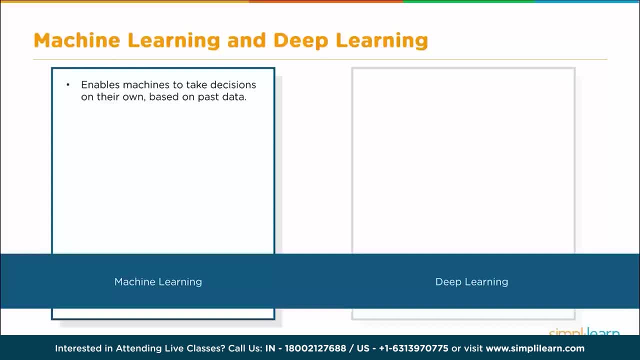 There's all kinds of cool tools out there you can use in machine learning. Enables machines to take decisions, to make decisions on their own based on past data. Enables machines to make decisions with the help of artificial neural networks. So it's doing the same thing, but we're using an artificial neural network as opposed to. 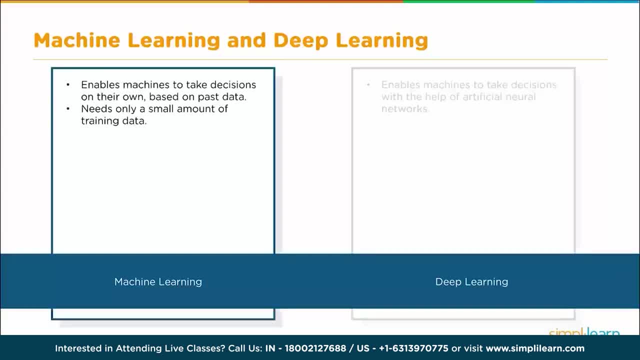 one of the more traditional machine learning tools Needs only a small amount of training data. This is very important. When you're talking about machine learning, they're usually not talking about training. They're talking about huge amounts of data. We're talking about, maybe, your spreadsheet from your business and your totals for the 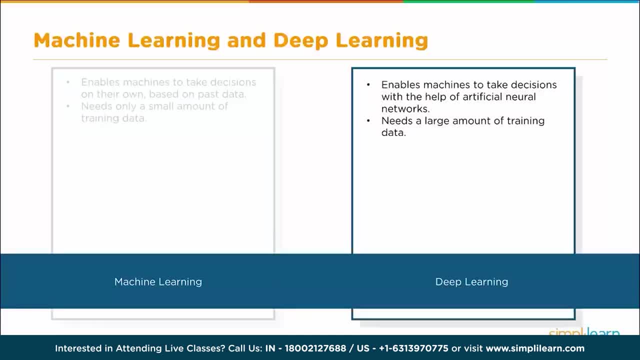 end of the year. When you're talking about neural networks, you usually need a large amount of data to train the data, So there's a lot of training involved. If you have under 500 points of data, that's probably not going to go into machine learning. 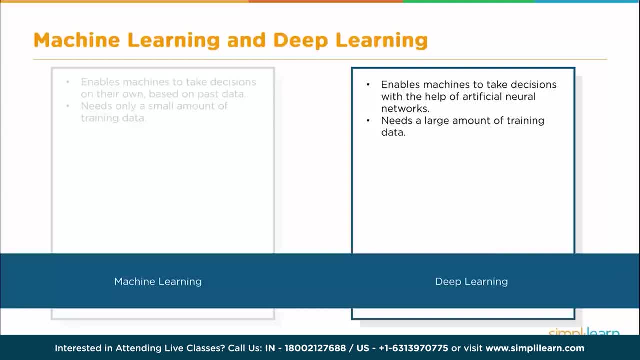 Or maybe you have, like in the case of one of the things, 500 points of data and 30 different fields. It starts getting really confusing there. in artificial intelligence or machine learning and the deep learning aspect, It really shines when you get to that larger data. that's really complex. 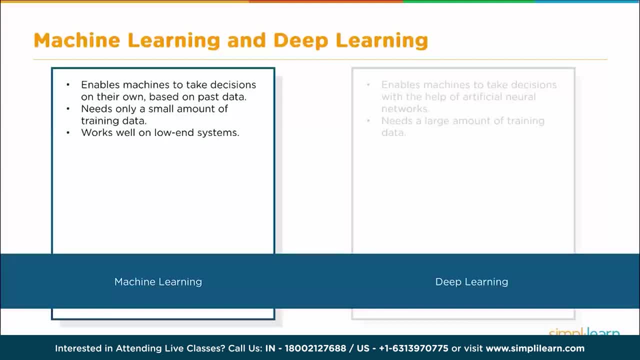 Works well on low-end systems. So a lot of the machine learning tools out there you can run on your laptop with no problem and do the calculations there. Where with the machine learning it usually needs a higher-end system to work, It takes a lot more processing power to build those neural networks and to train them. 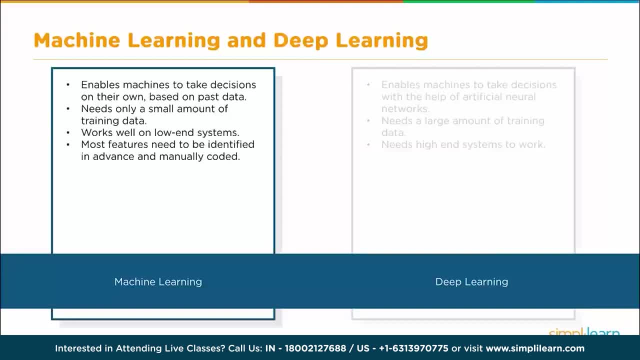 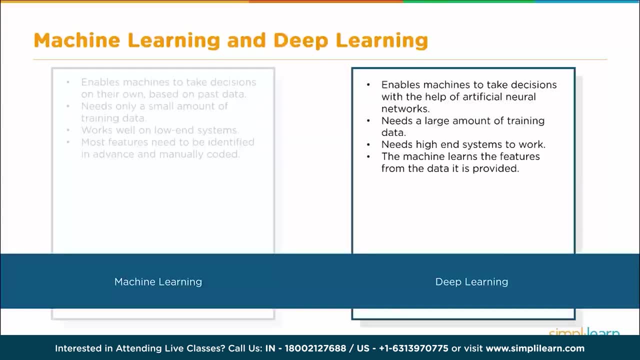 It goes through a lot of data. We're talking about the general machine learning tools. Most features need to be identified in advanced. It's manually coded, so there's a lot of human work on here. The machine learns the features from the data it is provided. 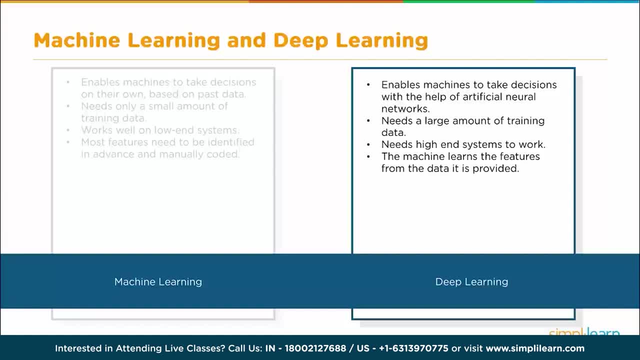 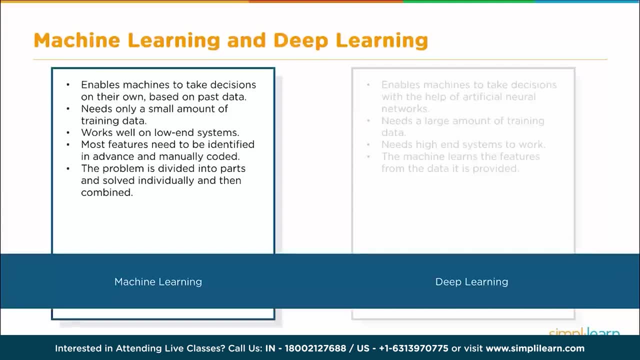 So again, it's like a magic box. You don't have to know what a tire is, It figures it out for you. The problem is divided into parts and solved individually and then combined. So in machine learning you usually have all these different tools and use different tools. 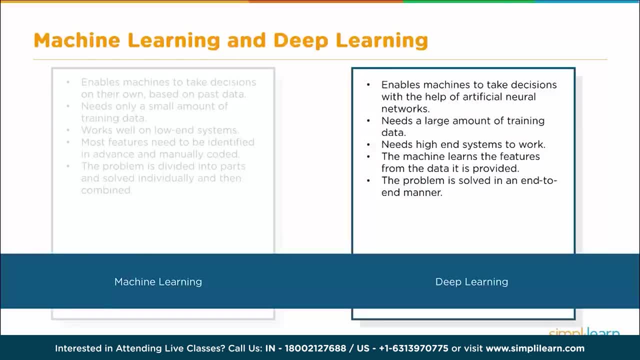 for different parts And the problem is solved in an end-to-end manner. So you only have one neural network or two neural networks. that is bringing the data in and putting it out. It's not going through a lot of different processes to get there. 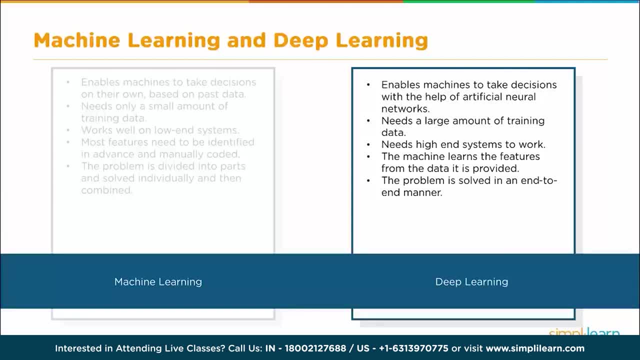 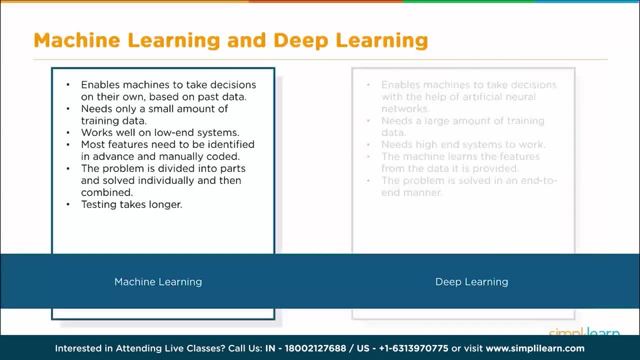 And remember you can put machine learning and deep learning together So you don't always have just the deep learning solving the problem. You might have it solving one piece of the puzzle With regular machine learning and most machine learning tools out there. they take longer. 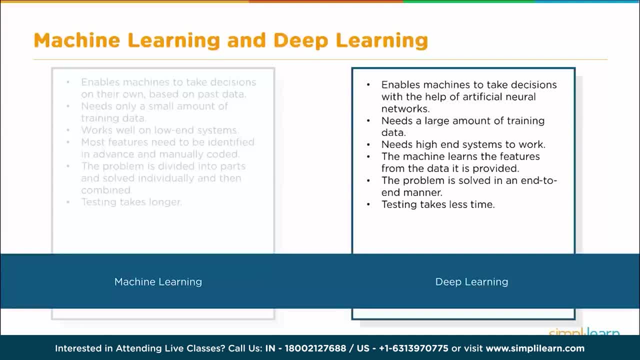 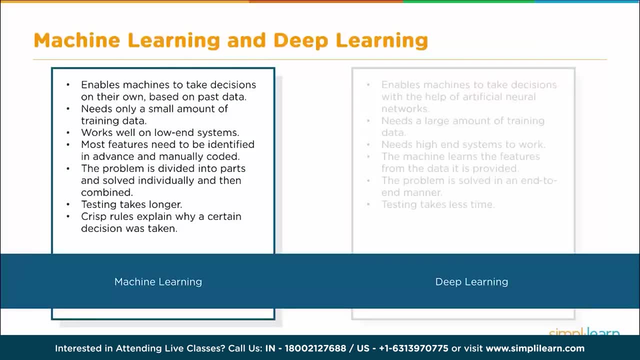 to test and understand how they work, And with the deep learning it's pretty quick. Once you build that neural network, you test it and you know. So we're dealing with very crisp rules, Limited resources: You have to really explain how the decision was made. when you use most machine learning. 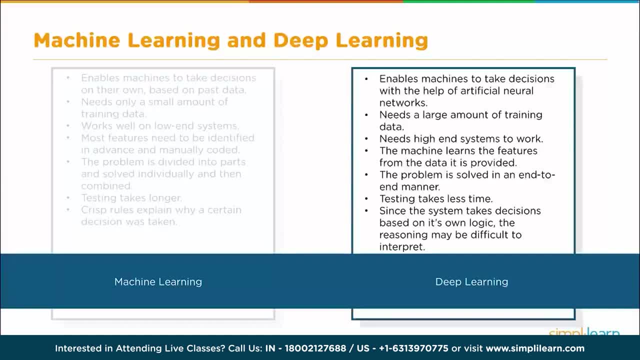 tools. But when you use the deep learning tool inside the machine learning tools, the system takes care of it based on its own logic and reasoning, And again, it's like a magic black box. You really don't know how it came up with the answer. 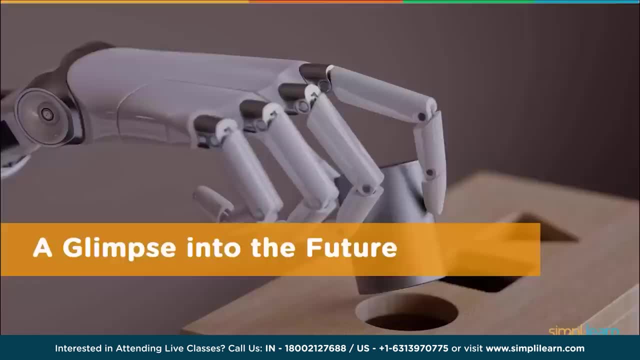 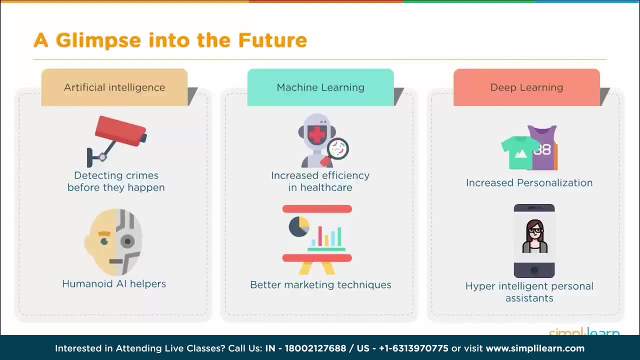 You just know it came up with the right answer: A glimpse into the future. So a quick glimpse into the future. Artificial intelligence: We'll be using it to detecting crimes before they happen. Humanoid AI helpers, Which we already have a lot of. 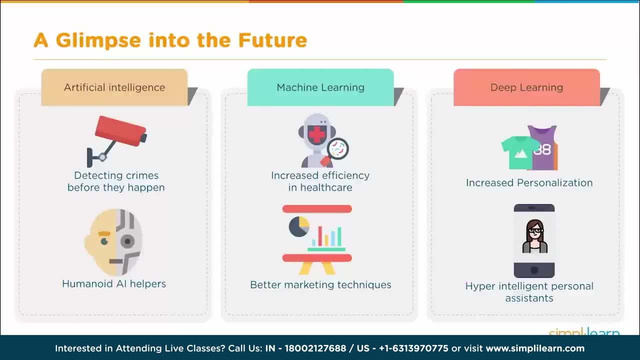 There'll be more and more. Maybe it'll actually be androids. That'd be cool to have an android that comes and gets stuff out of my fridge for me. Machine learning, Increasing efficiency in healthcare- That's really big in all the forms of machine learning. 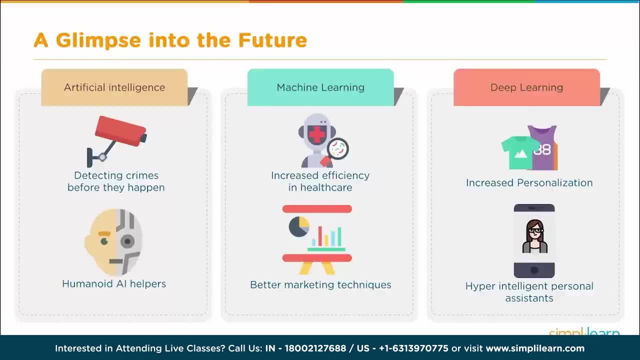 Better marketing techniques, Any of these things. if we get into the sciences it's just off the scale. Machine learning and artificial intelligence go everywhere. And then the subcategory deep learning Increased personalization. So what's really nice about the deep learning is it's going to start now. 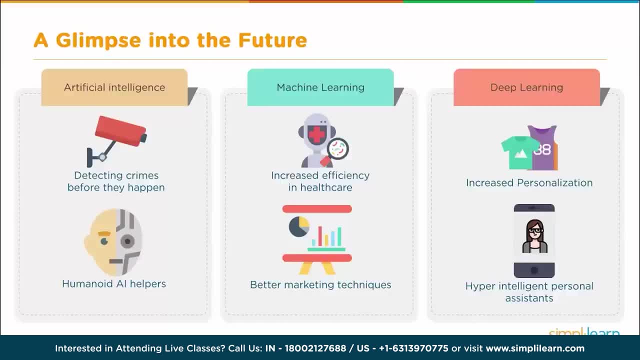 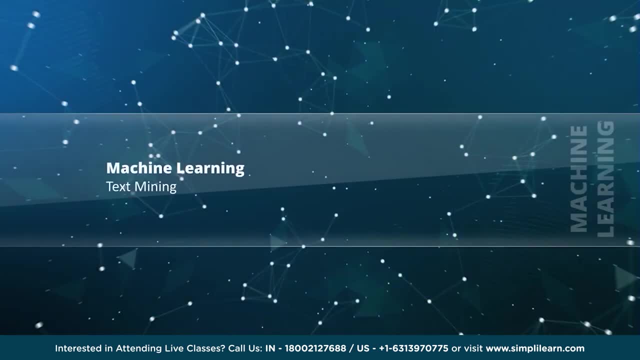 Catering to you. That'll be one of the things we see more and more of, And we'll have more of a hyper-intelligent personal assistant. I'm excited about that. In this lesson, you are going to understand the concept of text mining. 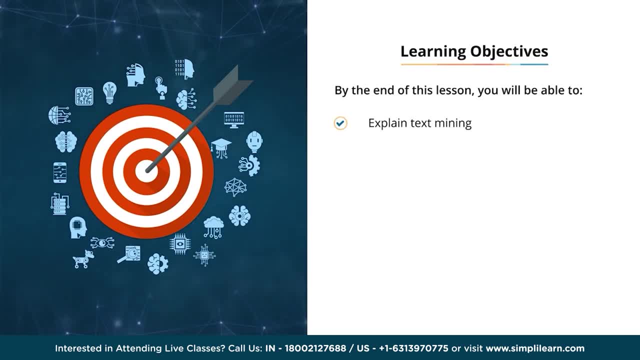 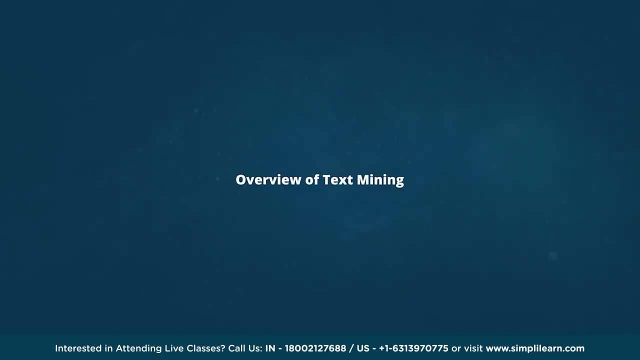 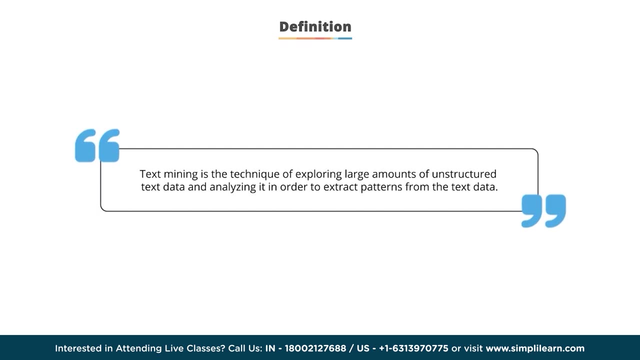 By the end of this lesson, you will be able to Explain text mining, Execute text processing tasks. So let's go ahead and understand text mining in detail. Let's first understand what text mining is. Text mining is the technique of exploring large amounts of unstructured text data and 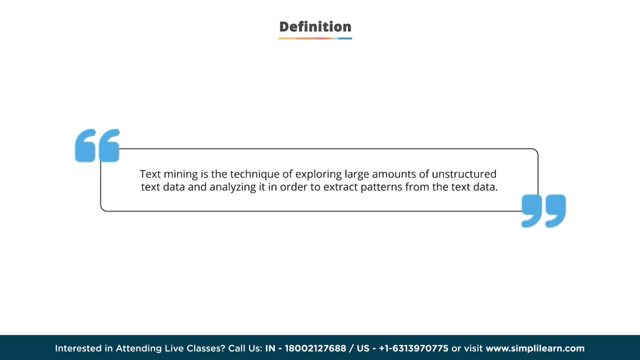 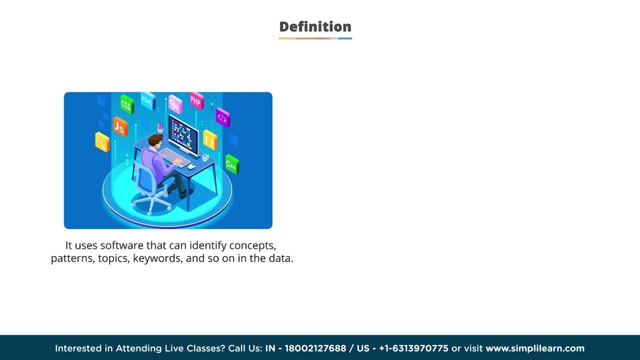 analyzing it in order to extract patterns from the text data. It is aided by software that can identify concepts, patterns, topics, keywords and other attributes in the data. It utilizes computational techniques to extract and summarize the high-quality information from unstructured textual resources. 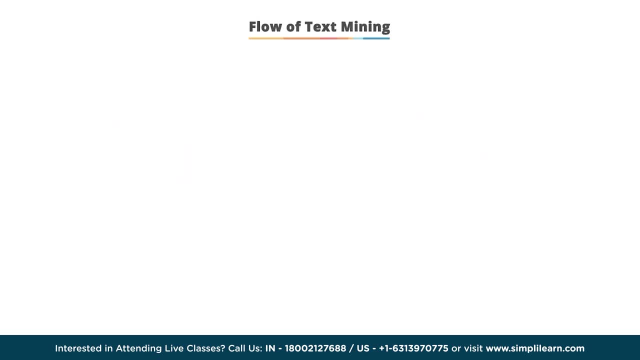 Let's understand the flow of text mining. There are five techniques used in text mining system. Information extraction or text pre-processing: This is used to examine the unstructured text by searching out the important words and finding the relationships between them. Categorization or text transformation. attribute generation. 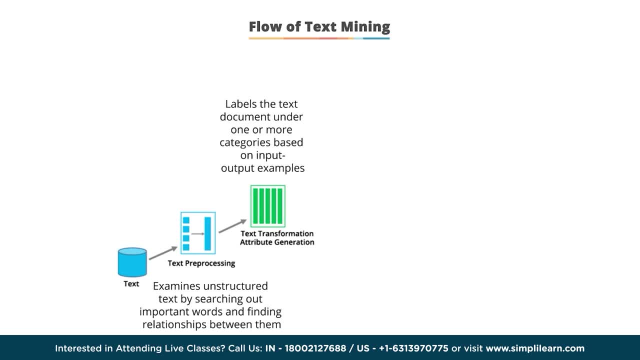 Categorization technique labels the text document under one or more categories. Classification of text data is done based on input-output. exactly Now you've drawn a picture of the text that was generated from theUBPcom presentation with categorization, Clustering or attribute selection. Clustering method is: 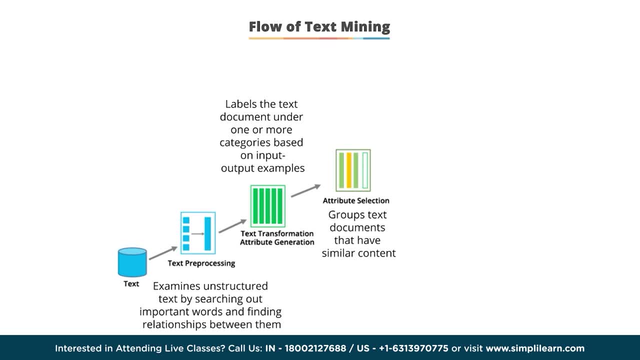 used to group text documents that have similar content. Clusters are the partitions, and each cluster will have a number of documents with similar content. Clustering makes sure that no document will be omitted from the search and it derives all the documents that have similar content. Visualization technique. 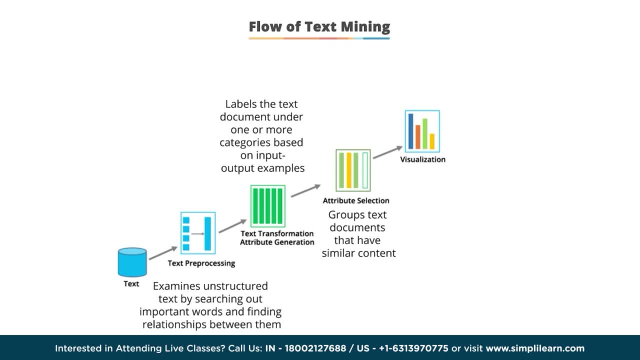 The process of finding relevant information is simplified by visualization technique. This technique uses text flags to represent a group of documents or a single document, and compactness is indicated using colors. Visualization technique helps to display textual information in a more attractive way. Summarization, or interpretation or evaluation. Summarization technique will 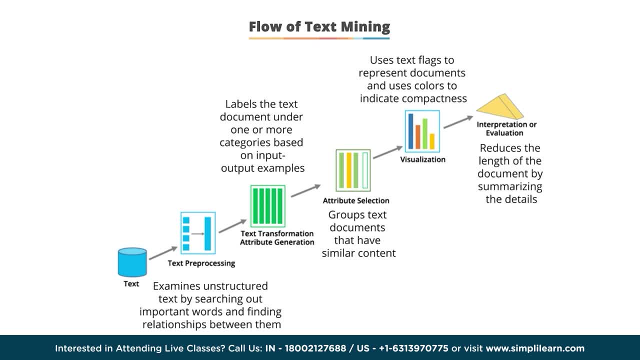 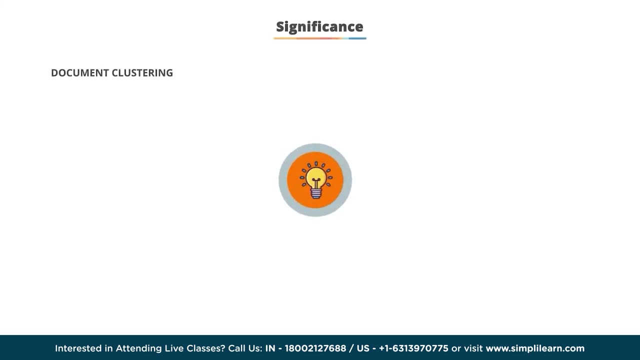 help to reduce the length of the document and summarize the text. Visualization technique helps to summarize the details of the documents. It makes the document easy to read for users and understand the content. at the moment, Let's understand the significance of text mining, Document clustering. Document clustering is an important part of text mining It. 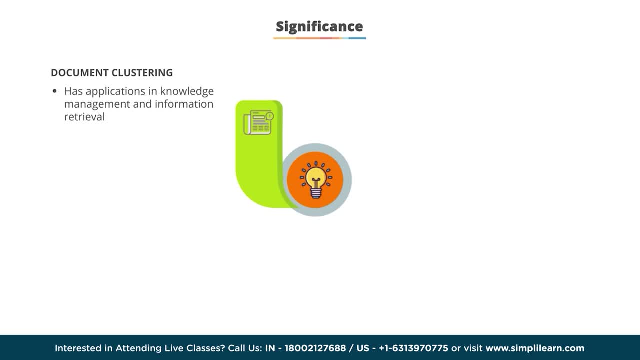 has many applications in knowledge management and information retrieval. Clustering makes it easy to group similar documents into meaningful groups, such as in newspapers, where sections are often grouped together. Text mining is the process of automatically searching large amount of text for text patterns and recognition of features. 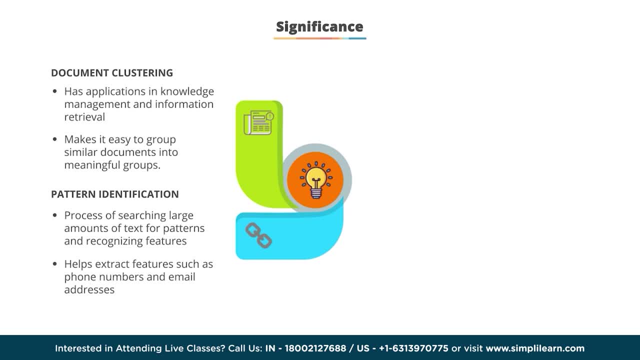 Features such as telephone numbers and email addresses can be extracted using pattern matches. Product insights: Text mining helps to extract large amounts of text, for example, customer reviews about the products. Mining consumer reviews can reveal insights like most loved feature, most hated feature, improvements required and reviews of competitors' products. 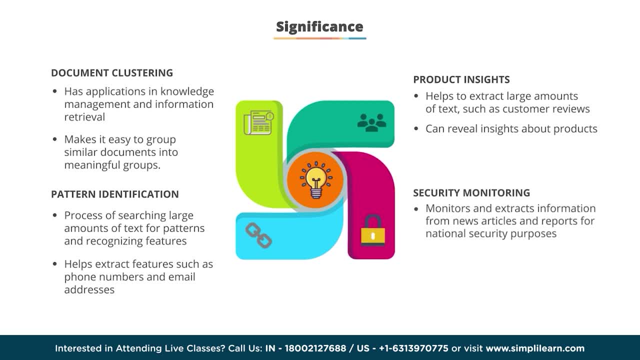 Security monitoring. Text mining helps in monitoring and extracting information from news articles and reports for national security purposes. Text mining makes sure to use all of your available information. It is a more effective and productive knowledge discovery that allows you to make better informed decisions, automate information-intensive processes and improve your 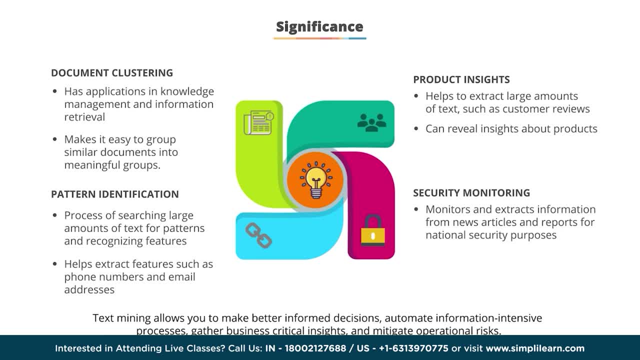 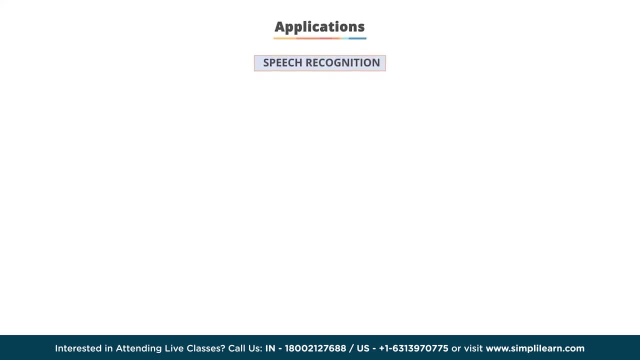 operational performance, Gather business-critical insights and mitigate operational risk. Let's look at the applications of text mining: Speech recognition. Speech recognition is the recognition and translation of spoken language into text and vice versa. Speech often provides valuable information about the topics, subjects. 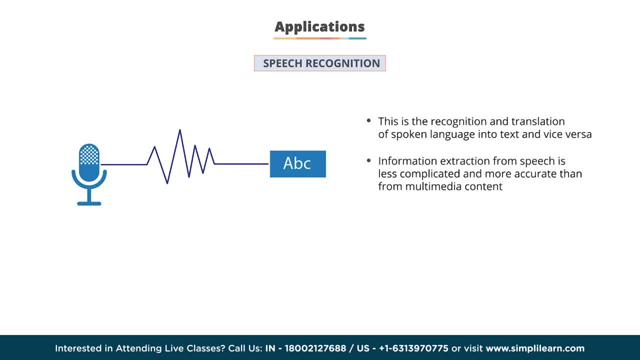 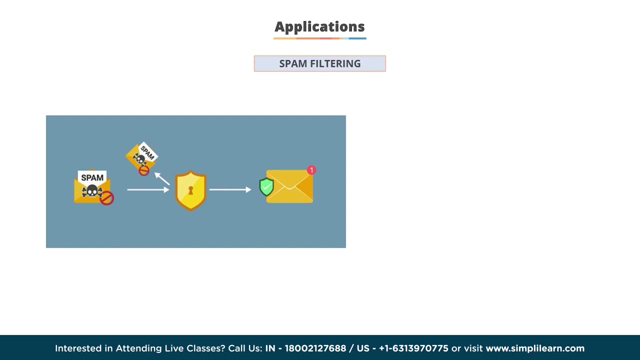 and concepts of multimedia content. Information extraction from speech is less complicated, yet more accurate and precise than multimedia content. this fact motivates content-based speech analysis for multimedia data mining and retrieval, where audio and speech processing is a key, enabling technology. spam filtering- spam detection- is an important method in 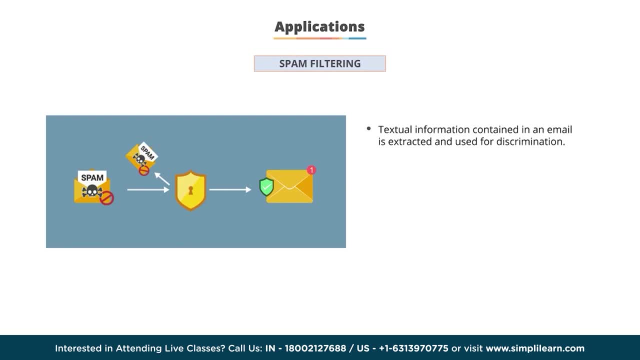 which textual information contained in an email is extracted and used for discrimination. text mining is useful in automatic detection of spam emails based on the filtering content. using text mining, an email service provider such as gmail or yahoo mail checks the content of an email and if some malicious text is found in the mail, then that email is marked as spam and sent. 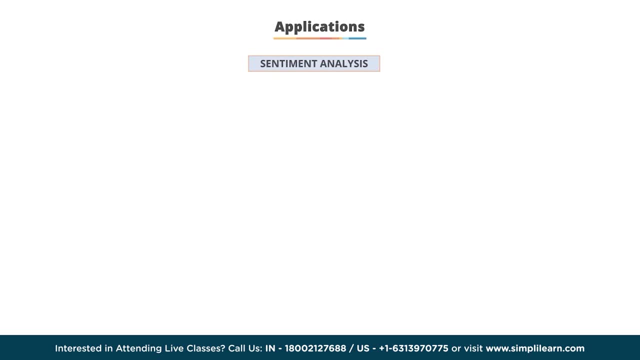 to the spam folder. sentiment analysis. it is done in order to determine if a given sentence expresses positive, neutral or negative sentiment. sentiment analysis is one of the most popular applications of text analytics. the primary aspect of sentiment analysis includes data analysis of the body of the text for understanding the opinion expressed by it and other key factors comprising modality and mood. 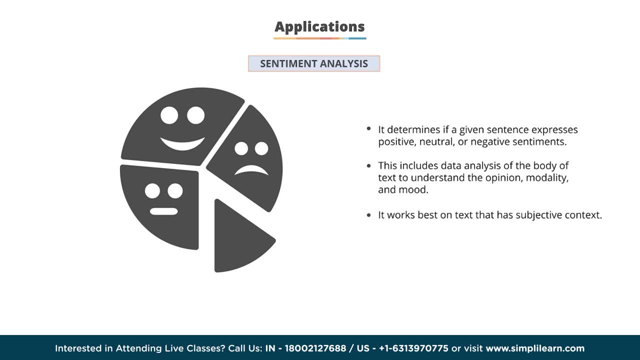 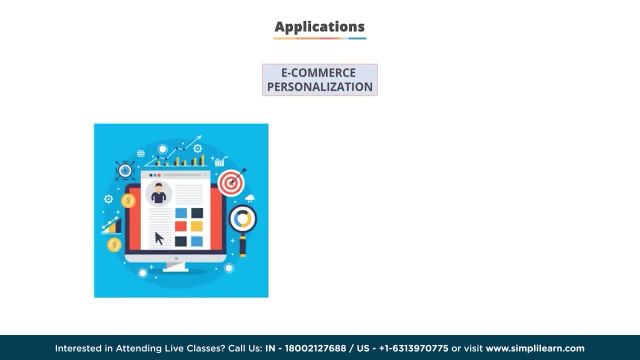 usually the process of sentiment analysis works best on text that has a subjective context than on that with only an objective context. e-commerce: the most important aspect of sentiment analysis is the use of text for personalization. text mining is used to suggest products that fit into a user's profile. text mining is increasingly 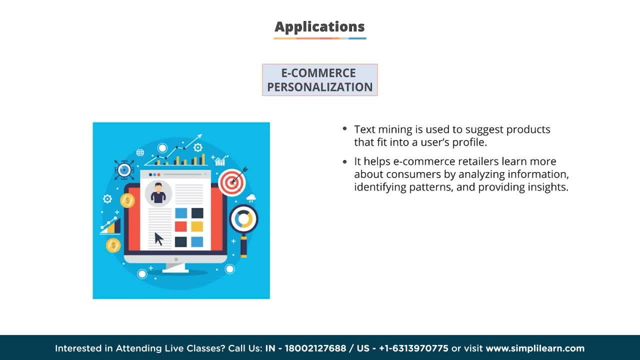 being used by e-commerce retailers to learn more about the consumers, as it is the process of analyzing textual information in order to identify patterns and gain insights. e-commerce retailers can target specific individuals or segments with personalized offers and discounts to boost sales by identifying customer purchase patterns and opinions on particular products. 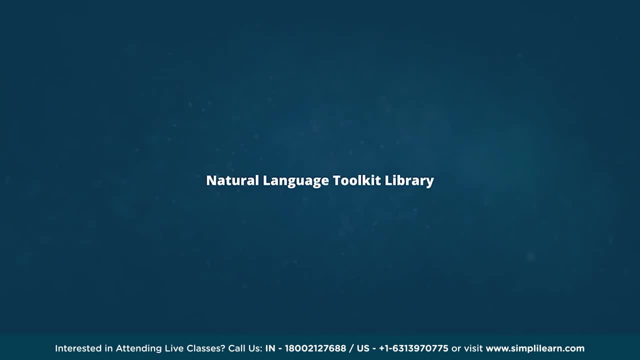 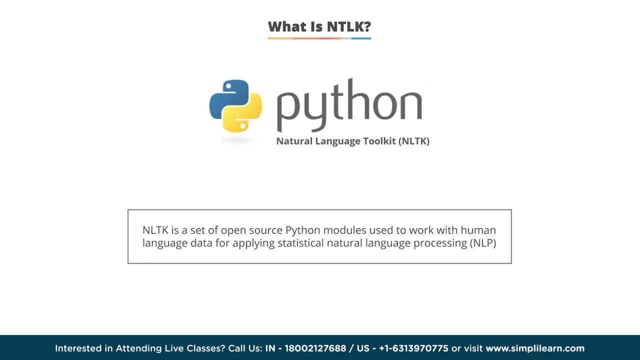 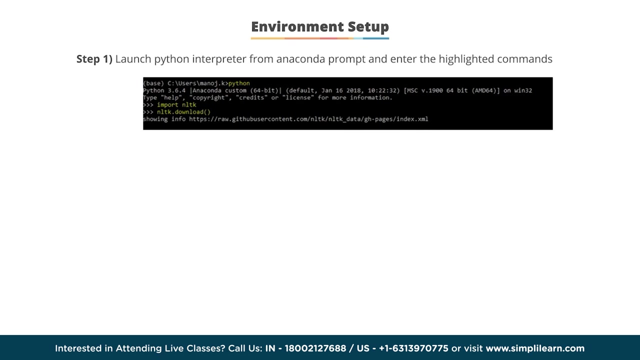 Let's look at Natural Language Toolkit library in detail. Natural Language Toolkit is a set of open-source Python models that are used to apply statistical natural language processing on human language data. Let's see how you can do environment setup of NLTK. Go to Windows start and launch Python interpreter from Anaconda prompt and enter the following commands: 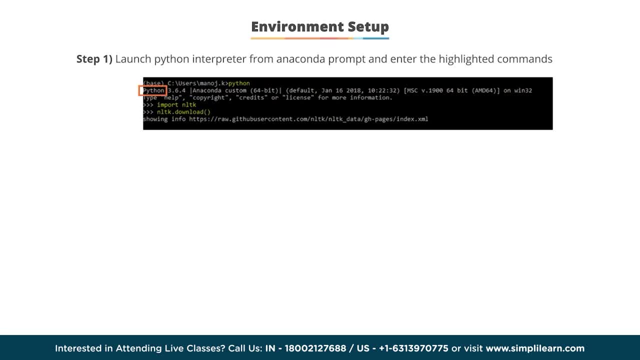 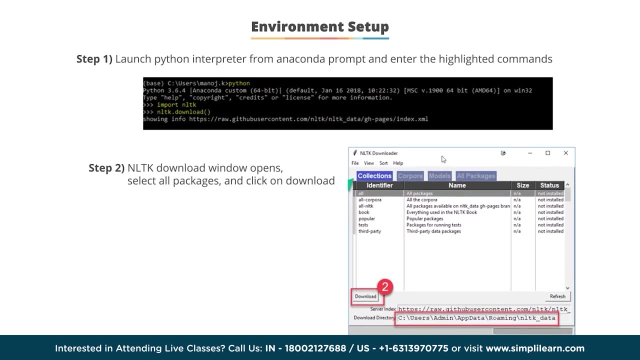 Enter command Python to check the version of Python installed on your system. Enter import NLTK to link you to the NLTK library available to download. Then enter nltkdownload function. that will open the NLTK download window. Check the download directory, select all packages and click on download. 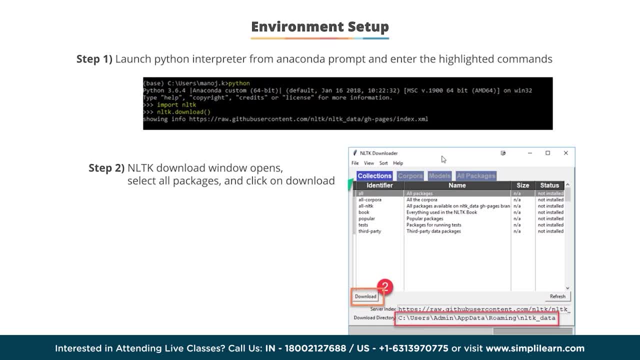 This will download NLTK onto your Python. Once you have downloaded the NLTK, you must check the working and functionality of it. In order to test the setup, enter the following command in Python: idle From nltkcorpus- import brown. The brown is an NLTK corpus that shows the systematic difference. 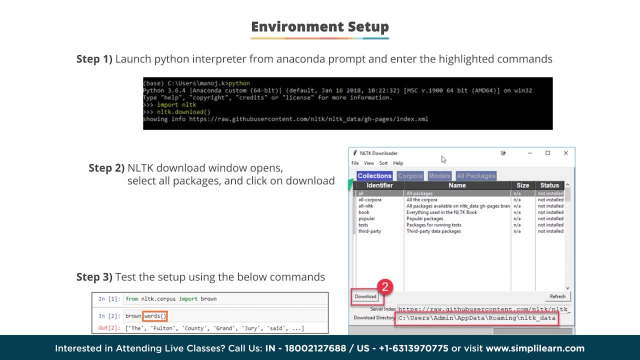 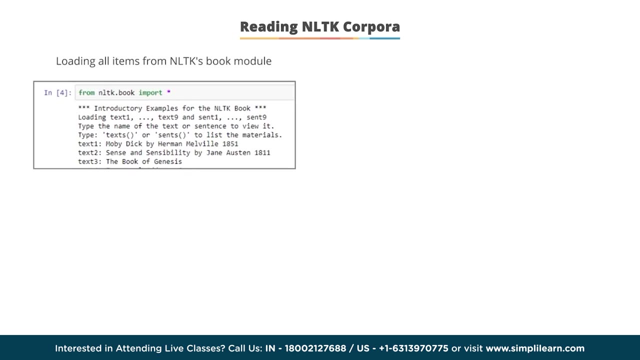 between different genres available in Python Words function will give you the list available words in the genre. The given output shows that we have successfully tested the NLTK installed on Python. Let's now understand how you can read a specific module from NLTK corpora. 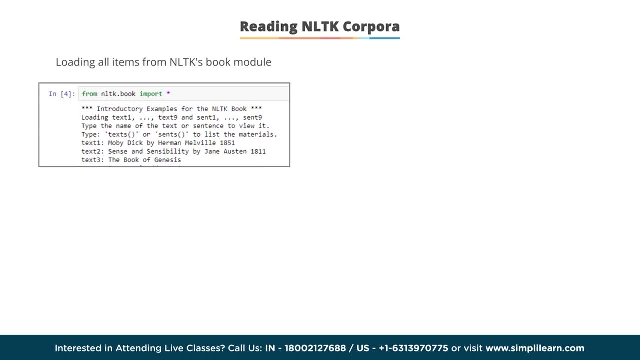 If you want to import an entire module from NLTK corpora, use asterisk symbol with that module name. import command. Enter the command from nltkbookmark. It will load all the items available in NLTK's book module. Now in order to explore brown corpus. 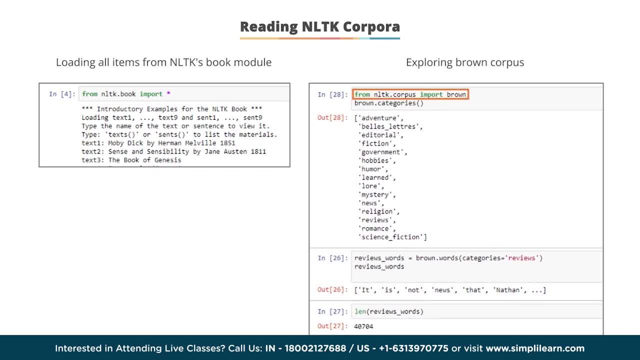 enter the command nltkcorpus- import brown. This will import brown corpus on the Python. Enter browncategories function to load the different genres available. Select a genre and assign that genre to a variable using the following syntax: Variable name. Variable name is equal to brownwords. 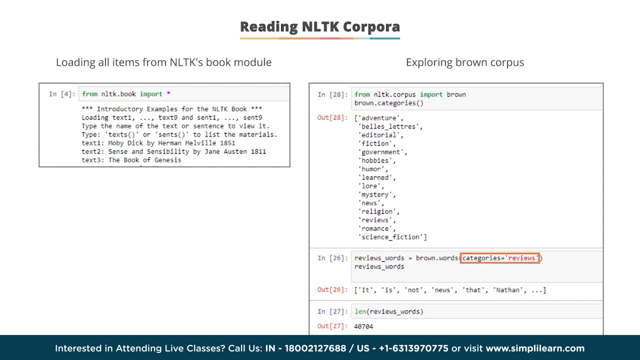 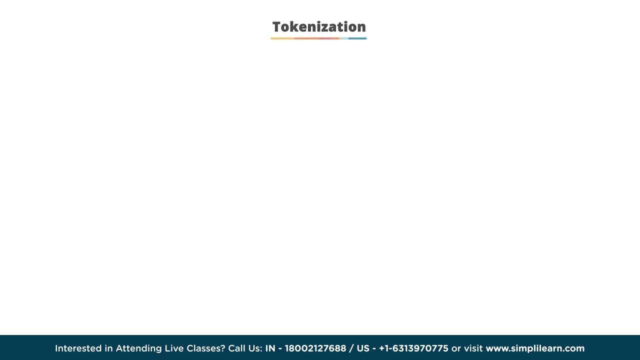 Categories is equal to genre name. Now, in order to see the available words inside the selected genre, just enter the defined variable name as a command. Let's understand text extraction and pre-processing in detail. So let's first understand the concept of tokenization. 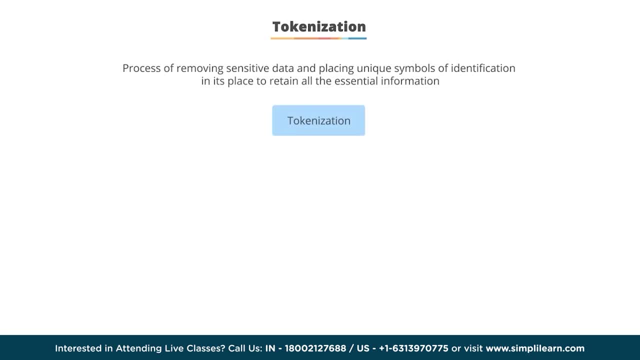 Tokenization is the process of removing sensitive data and placing unique symbols of identification in that place in order to retain all the essential information concerned with the data by its security. It is a process of breaking running streams of text into words and sentences. It works by segregating words using punctuation and spaces. 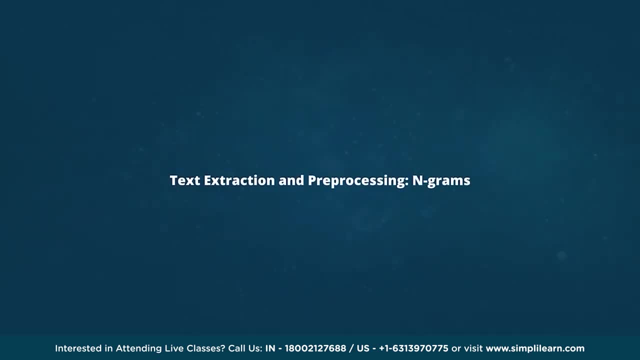 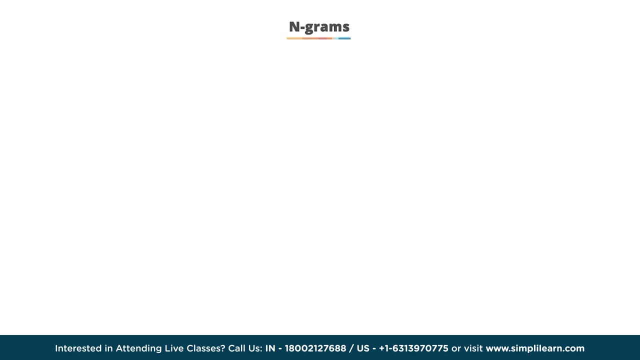 Text extraction and pre-processing engrams. Now let's look at what engram is and how it is helpful in text mining. Engram is the simplest model that assigns these probabilities to sequences of words or sentences. Engrams are combinations of adjacent words or letters of length n in the source text. 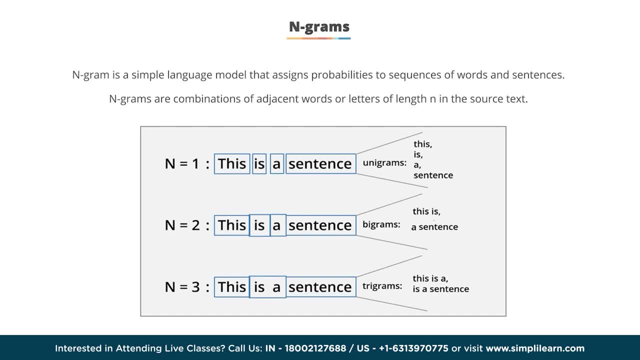 So engram is very helpful in text mining when it is required to extract patterns from the text, As in the given example. this is a sentence. All of these words are considered individual words and thus represent unigrams. A two-gram or bigram is a two-word sequence of words like this is: is a or a sentence. 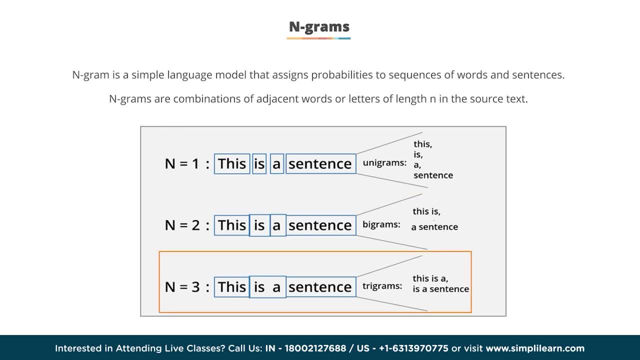 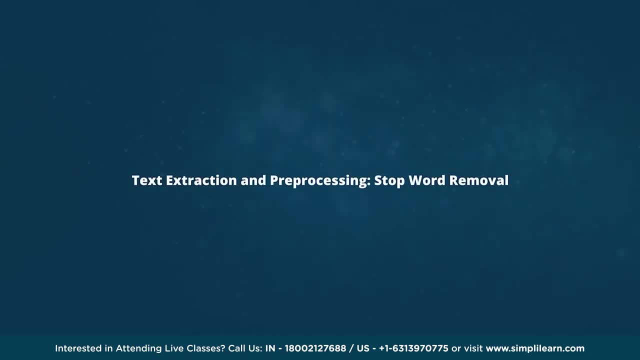 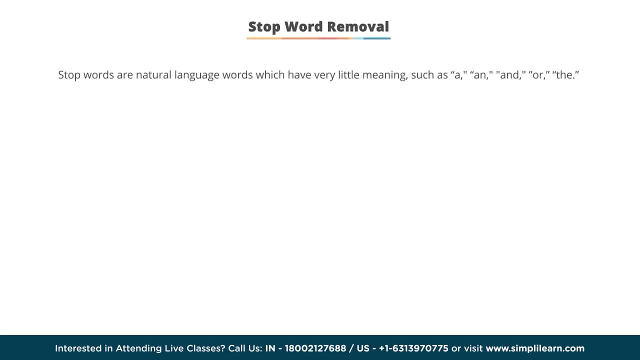 and a three-gram, or trigram, is a three-word sequence of words like this is a or is a sentence. Let's now understand what stop words are and how you can remove them. Stop words are natural language words that have negligible meanings, such as a, an and. 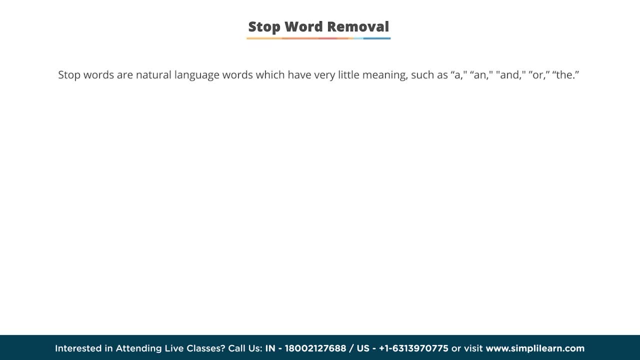 or the and other similar words. These words also will take up space in the database or increase the processing time, So it is better to remove such words by storing a list of stop words. You can find the list of stop words in the NLTK data directory. 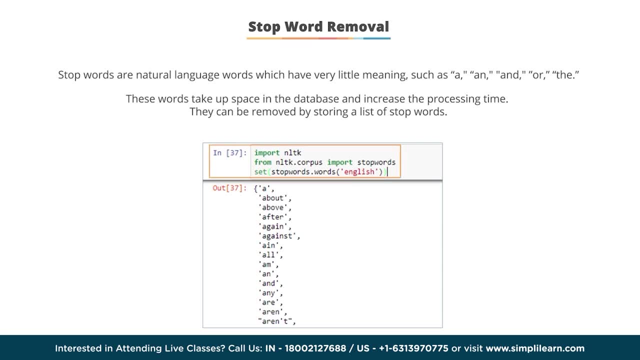 that is stored in 16 different languages. Use the following command to list the stop words of English language defined in NLTK corpus: Importing NLTK will import the NLTK corpus for that instance. Enter from nltkcorpus. import Stop words will import stop words from NLTK corpus. 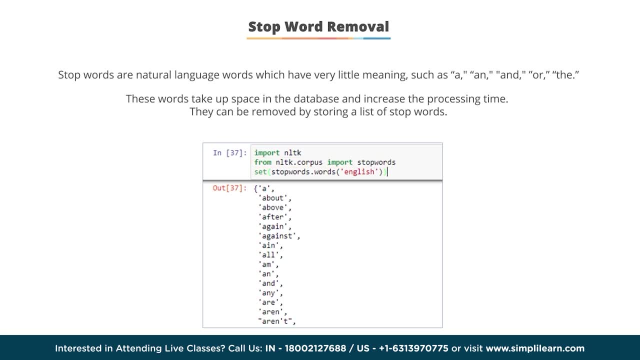 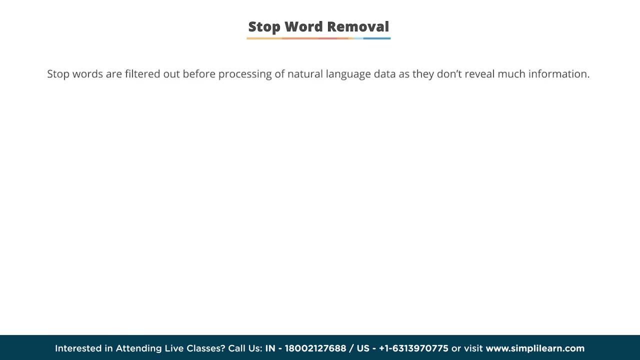 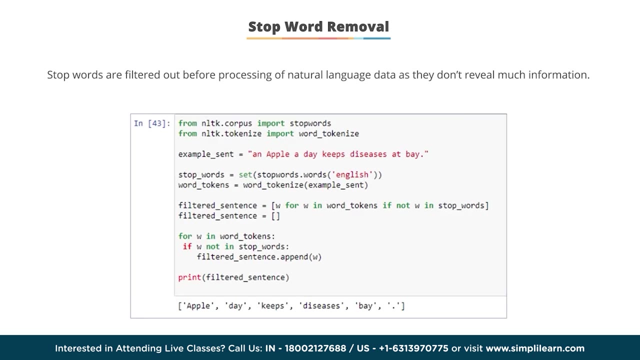 Now set the language as English, So use set function as set under braces stopwordswords. Set genre as English. Stop words are filtered out before processing of natural language data as they don't reveal much information. So, as you can see in the given example, before filtering the sentence: 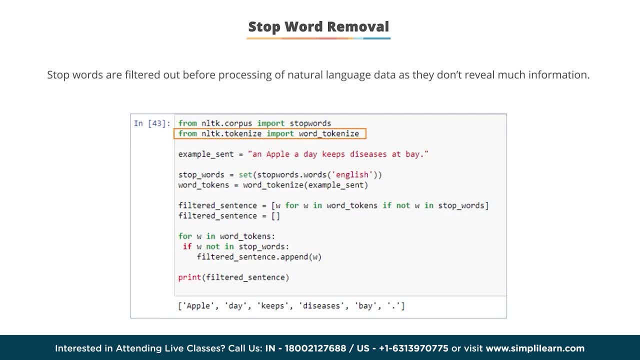 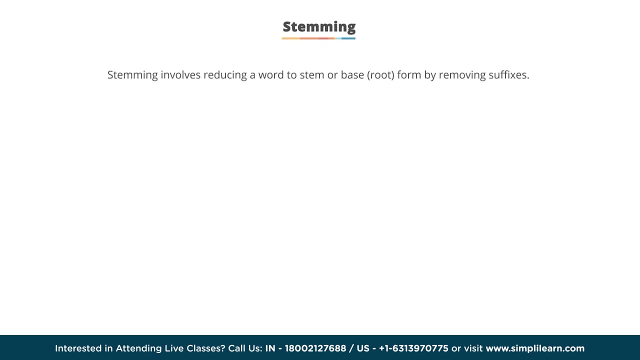 the tokenization of stop word is processed in order to remove these stop words and the filtering is applied in order to filter the sentence based on some criteria: Text extraction and pre-processing stemming. Stemming is used to reduce a word to stem or base word by removing suffixes. 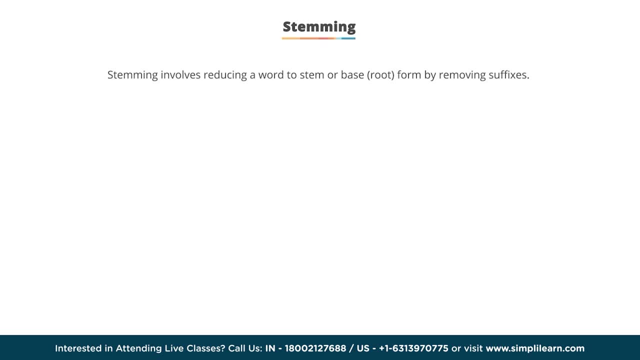 such as helps, helping, helped and helper to the root word help. The stemming process or algorithm is generally called a stemmer. There are various stemming algorithms, such as Porter stemmer, Lancaster stemmer, Snowball stemmer, etc. Use any of the stemmers defined under NLTK stem corpus. 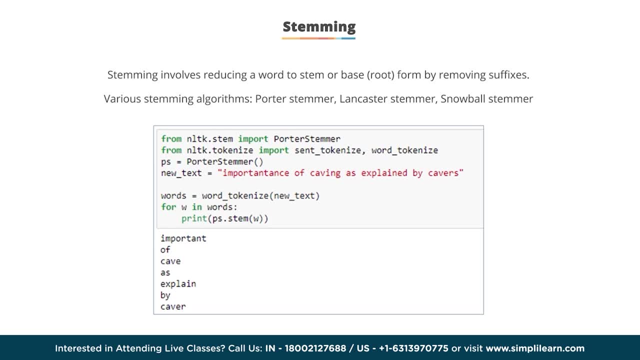 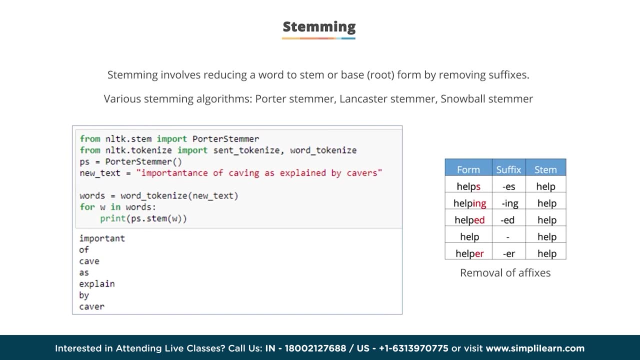 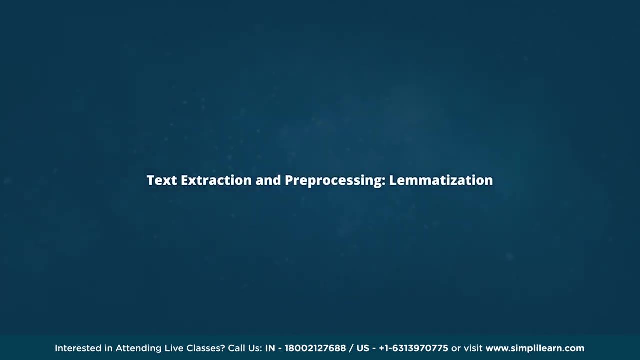 in order to perform stemming, as shown in the example Here, we have used Porter stemmer. When you observe the output, you will see that all of the words given have been reduced to their root word or stem. Text extraction and pre-processing lemmatization. 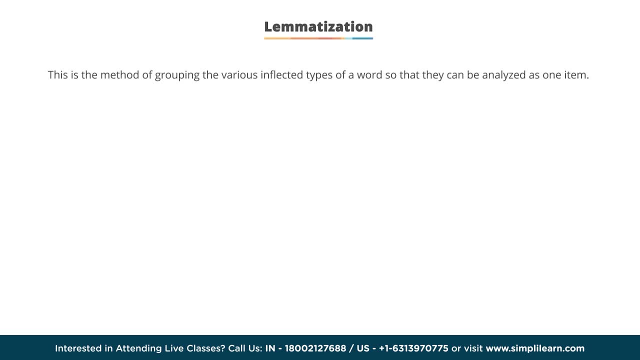 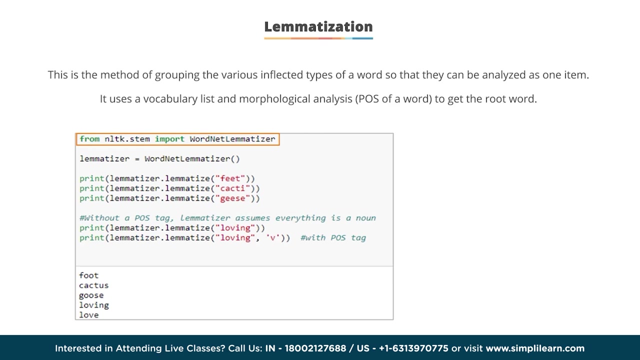 Lemmatization is the method of grouping the various inflected types of a word in order that they can be analyzed as one item. It uses vocabulary list or a morphological analysis to get the root word. It uses WordNet database that has English words linked together by their semantic relationship. 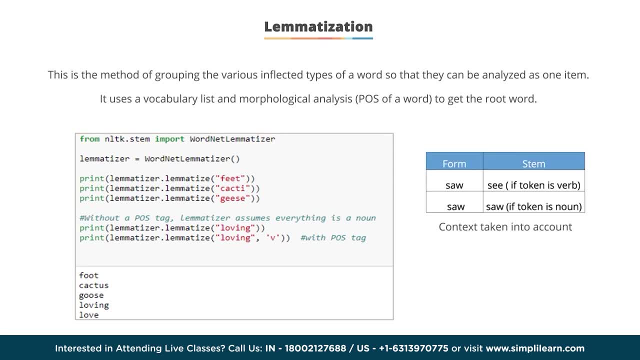 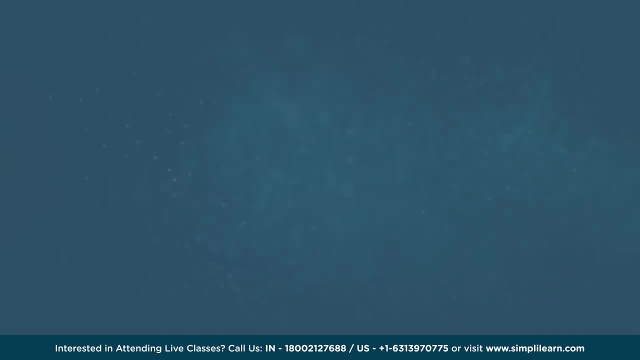 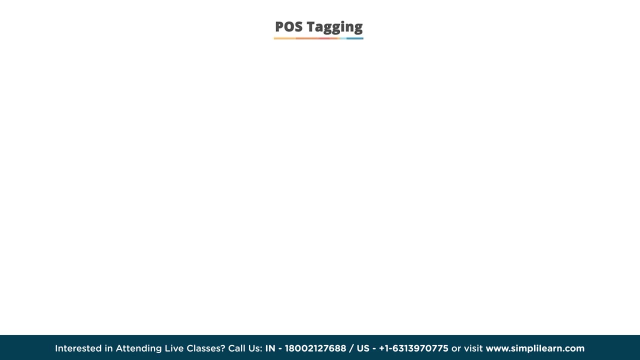 As you can observe the given example, the different words have been extracted to their relevant morphological word using lemmatization, Text extraction and pre-processing POS tagging. Let's now look at different part of speech tags available in the National Language Toolkit library. 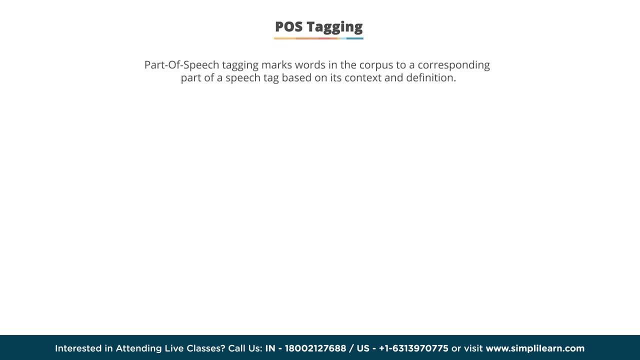 A POS tag is a special label assigned to each token or word in a text corpus to indicate the part of speech and often also other grammatical categories such as tense, number, case, etc. POS tags are used in text analysis tools and algorithms and also in corpus searches. 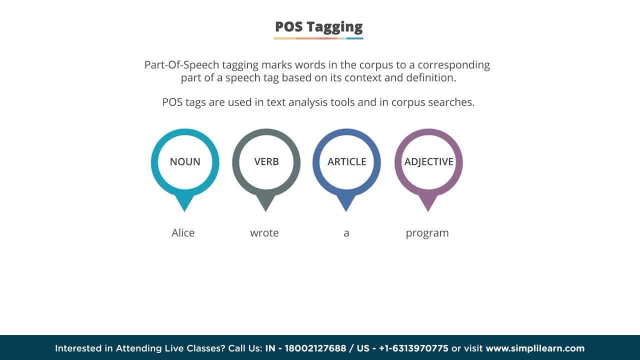 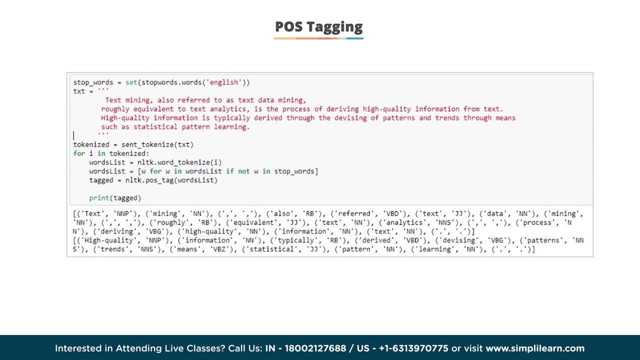 So look at the given example Here. Alice wrote a program is the source text given. The POS tags given are: Alice is a noun, wrote is a verb, a is an article and program is an adjective. Look at the given example to understand how POS tags are defined. 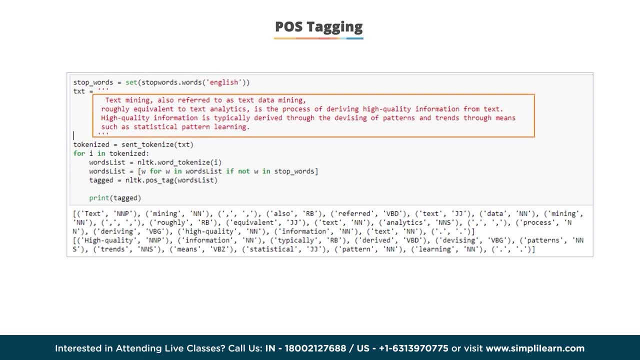 So the given sentence or paragraph contains different words that represent different parts of speech. We will first use tokenization and removal of stop words and then allocate the different POS tags. These are shown with different words in the given sentence. POS tags are useful for lemmatization. 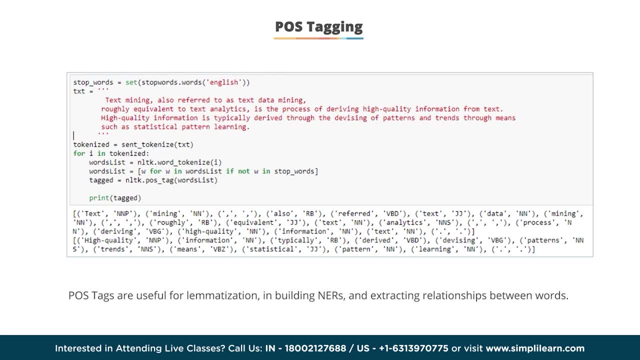 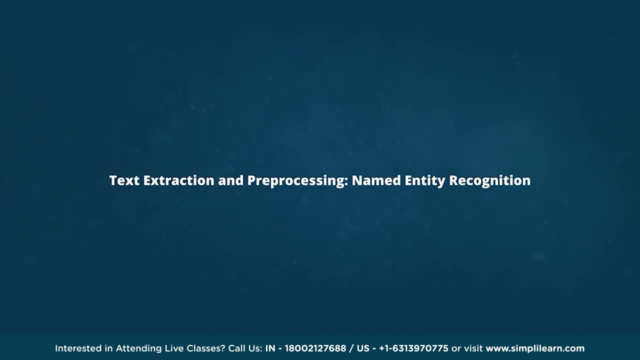 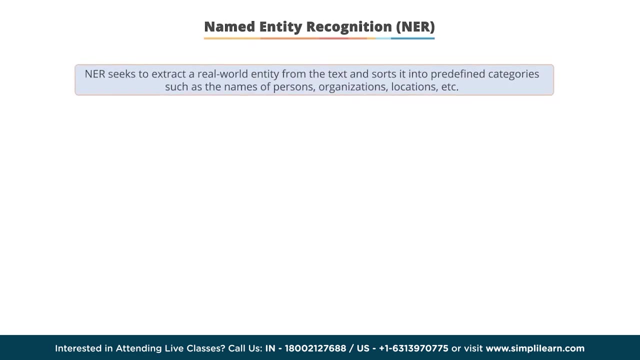 in building named entity recognition and extracting relationships between words, Text extraction and pre-processing. named entity recognition. Now let's understand what named entity recognition is all about. NER seeks to extract a real-world entity from the text and sorts it into pre-defined categories. 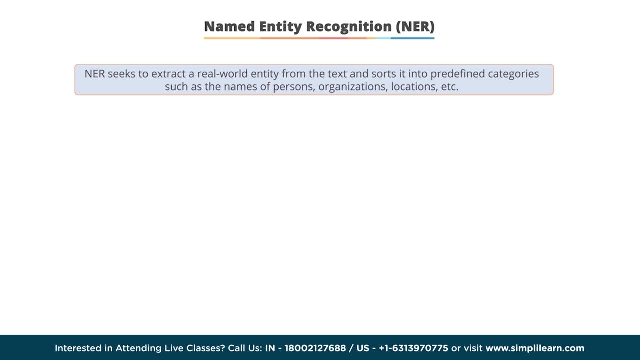 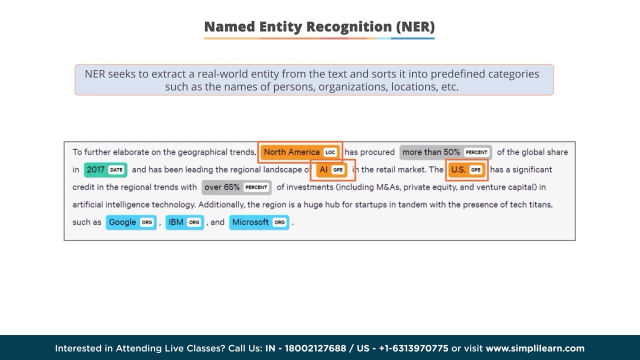 such as names of people, organizations, locations, etc. Many real-world questions can be answered with the help of name entity recognition. Were specified products mentioned in complaints or reviews. Does the tweet contain the name of a person? Does the tweet contain the person's address? 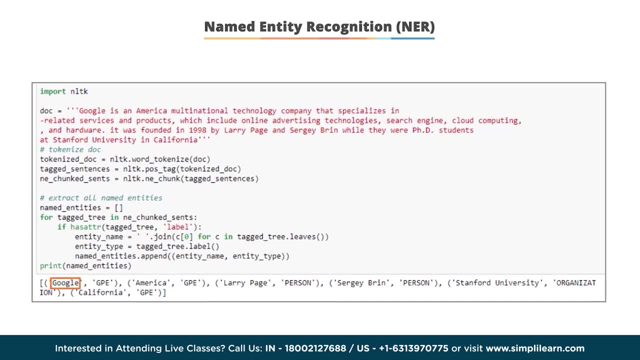 As you can see in the given example, Google America, Larry Page, etc. are the names of a person, place or an organization, So these are considered named entities and have different tags, such as person, organization, GPE or geopolitical entity, etc. 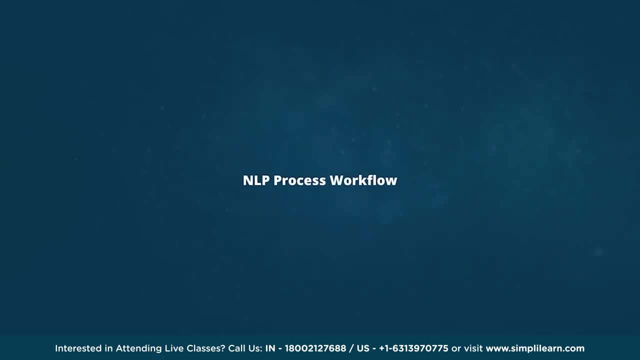 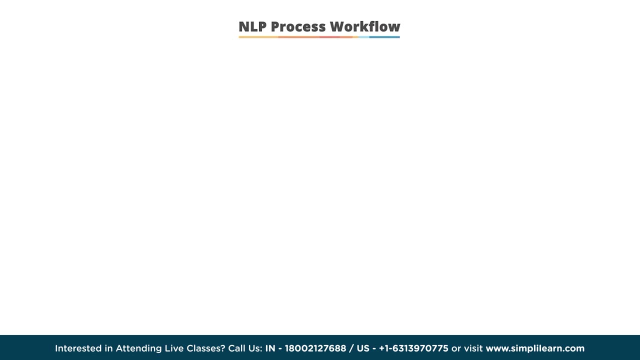 NLP process workflow. Now you have an understanding of all NLTK tools, so now let's understand the natural language processing workflow. Step 1. Tokenization: It splits text into pieces, tokens or words, and removes punctuation. Step 2. Stop-word removal. 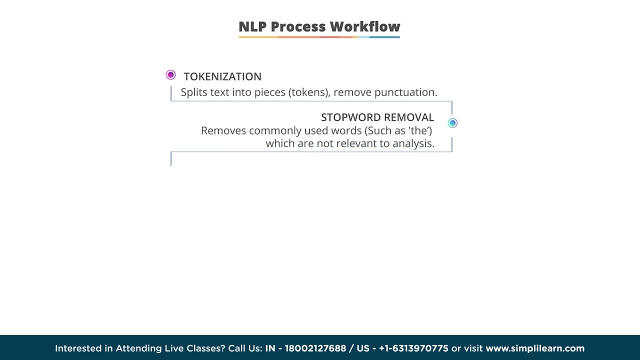 It removes commonly used words such as the is, are, etc. which are not relevant to the analysis. Step 3. Stemming and lemmatization. It reduces words to base form in order to be analyzed as a single item. 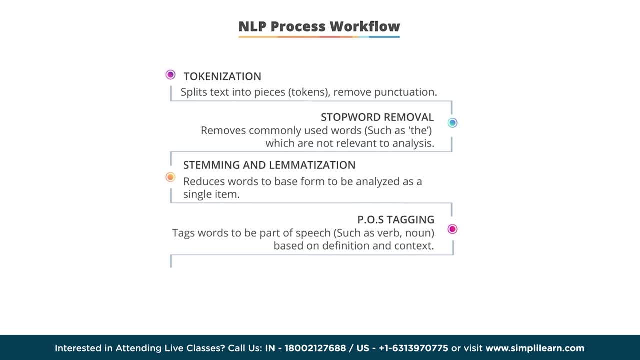 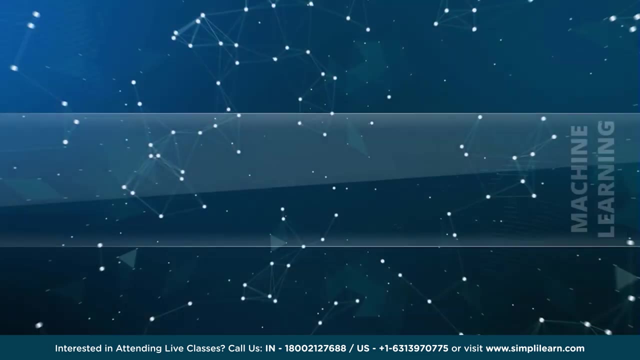 Step 4. POS tagging: It tags words to be part of speech, such as noun, verb, adjective, etc. based on the definition and context. Step 5. Information retrieval: It extracts relevant information from the source: M01. Brown Corpus. 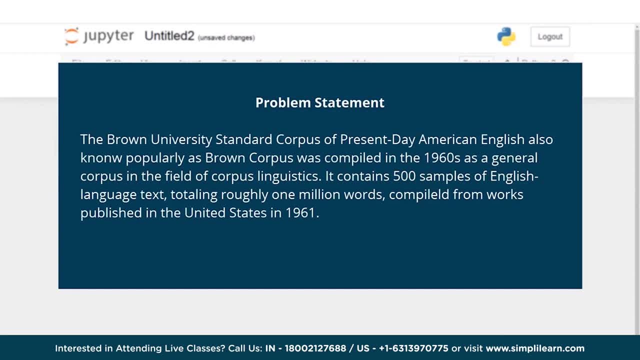 Problem statement. The Brown University Standard Corpus of present-day American English, also known popularly as Brown Corpus, was compiled in the 1960s as a general corpus in the field of corpus linguistics. It contains 500 samples of English language text. 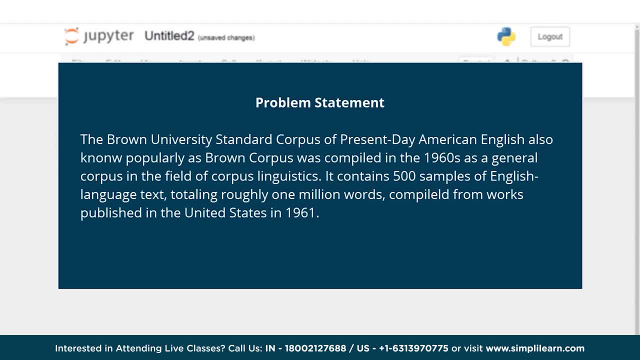 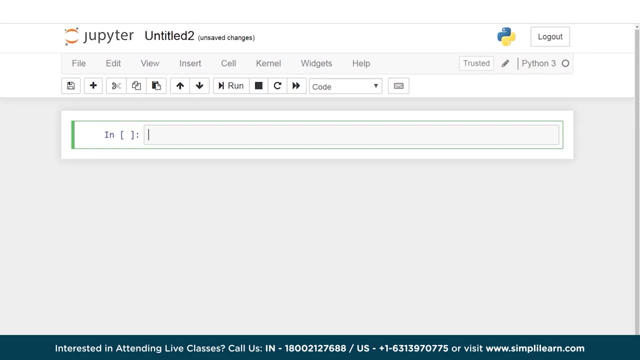 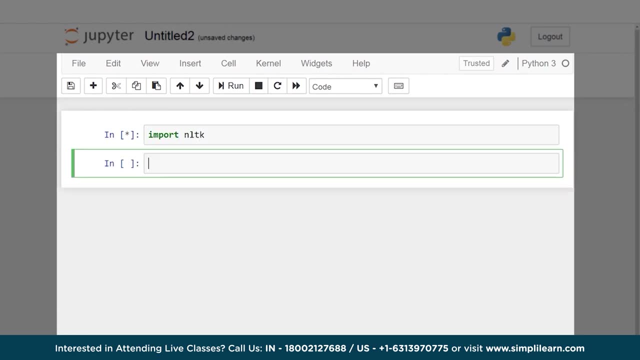 totaling roughly one million words compiled from works published in the United States in 1961.. We will be working on one of the subset data set and perform text processing tasks. Let us import the NLTK library and read the CA underscore 10A. 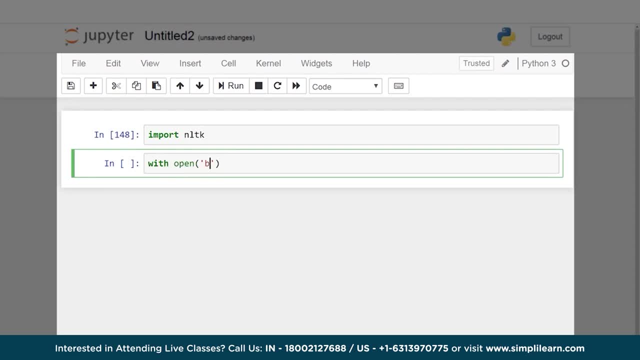 Import NLTK, We will have to make sure that there are no slashes in between. hence, we will use the replace function within pandas. for the same, Let's have a look at the data once. Let's have a look at the data once. 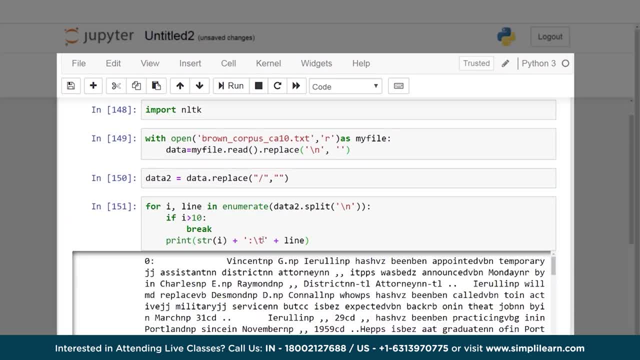 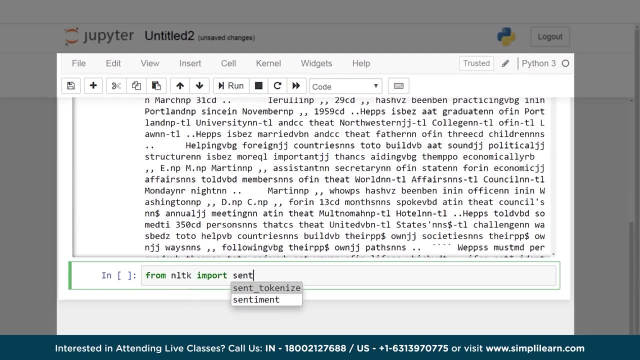 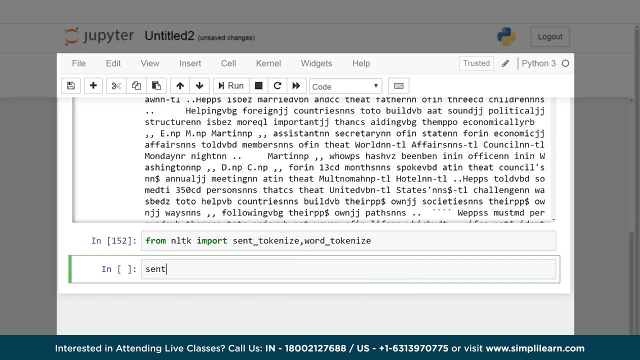 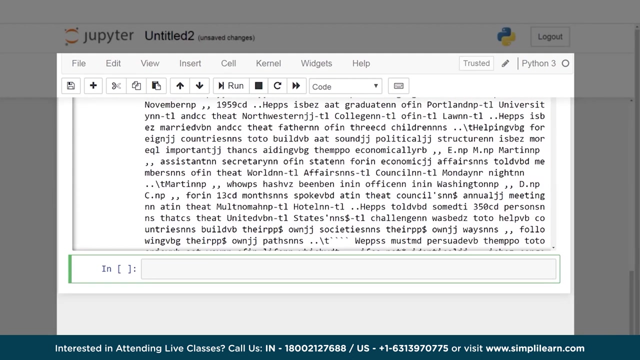 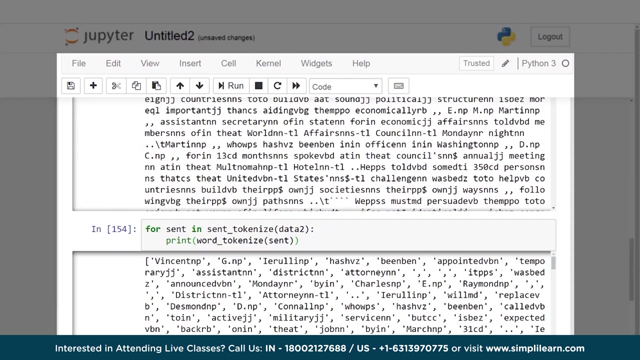 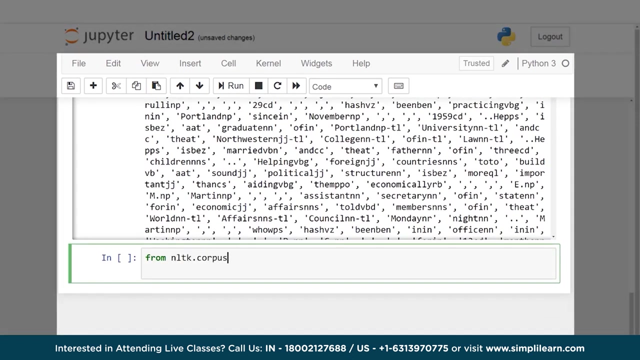 Tokenization. After performing sentence tokenization on the data we obtained. Similarly, after applying sentence tokenizer, the resulting output shows all individual words. Stopword Removal: Let's import the stopword library From nltkcorpus: import stopwords. We also need to ensure that the text is in the same case. 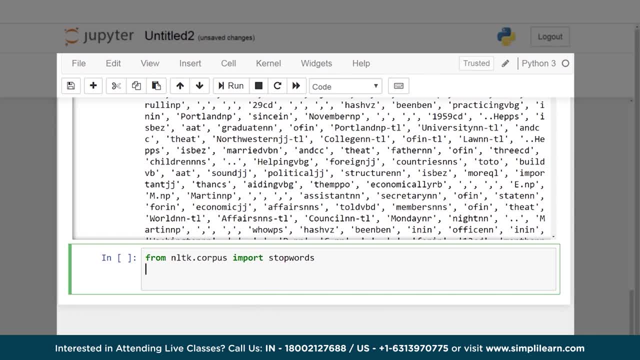 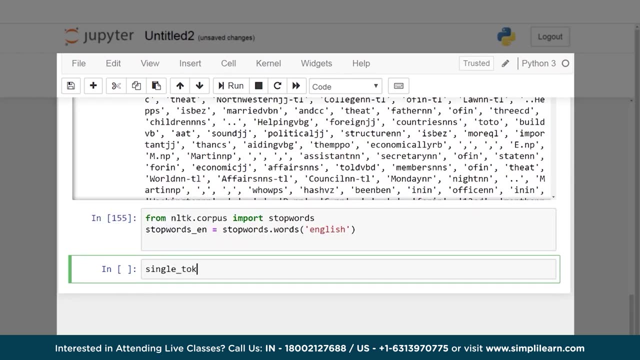 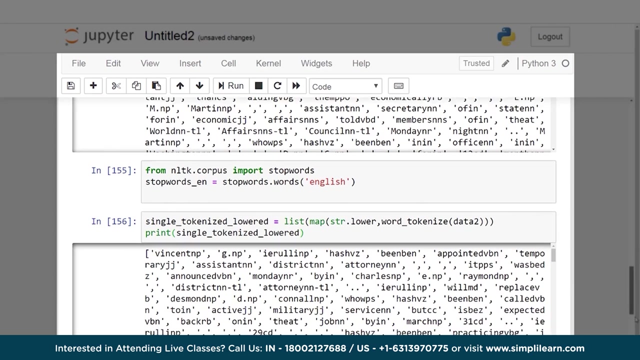 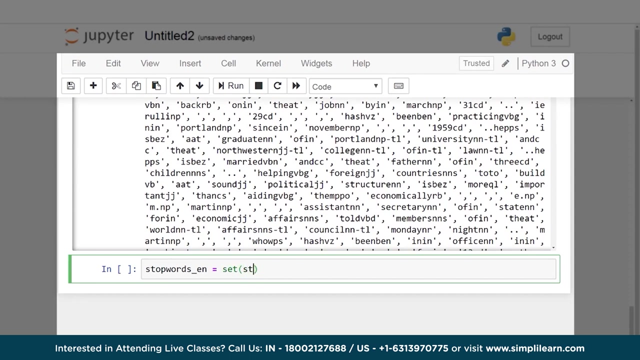 NLTK has its own list of stopwords. We can check the list of stopwords using stopwordswords and English. inside the parenthesis Map, the lowercase string with our list of word tokens. Let's remove the stopwords using the English stopwords list. in NLTK We will be using set checking, as it is faster in Python than a list. 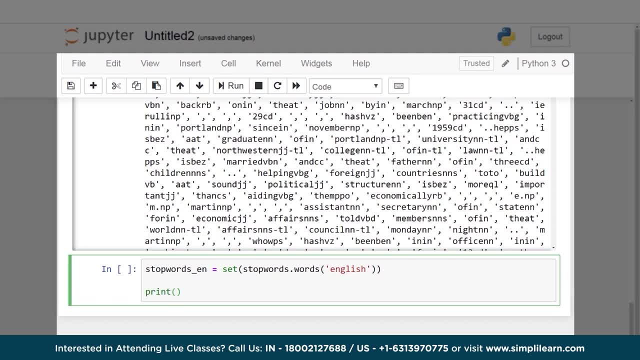 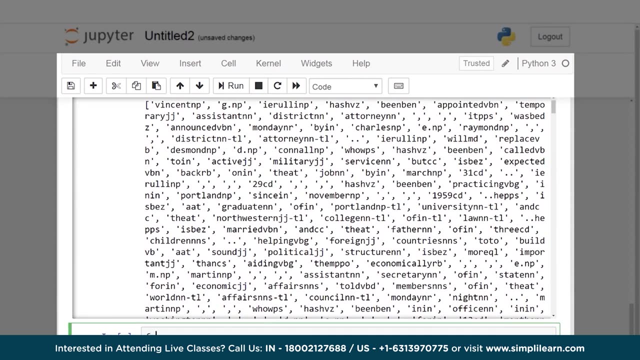 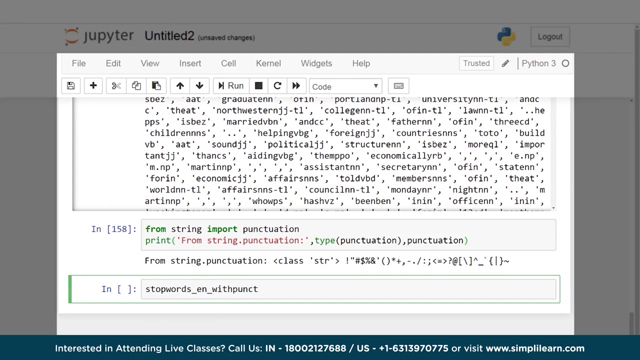 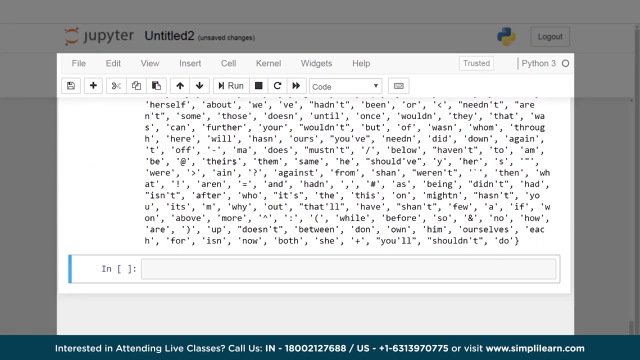 By removing all stopwords from the text we obtain. Often, we want to remove the punctuations from the documents too, Since Python comes with batteries included. we have Stringpunctuation From string import punctuation, Punctuation with the stop words from NLTK. Removing stop words with punctuation. 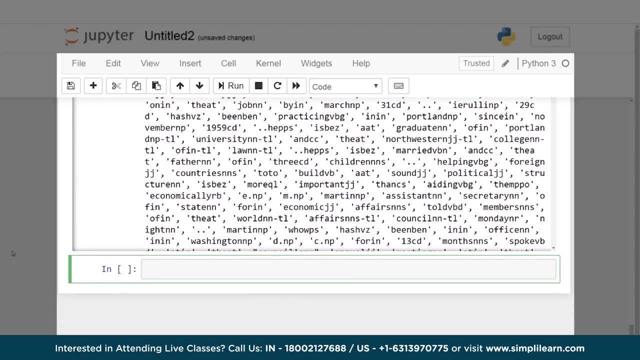 Stemming and lemmatization. We will be using stemming and lemmatization to reduce words to their root form, For example, walks. walking, walked will be reduced to their root word: walk. Importing Porter stemmer as the stemming library. 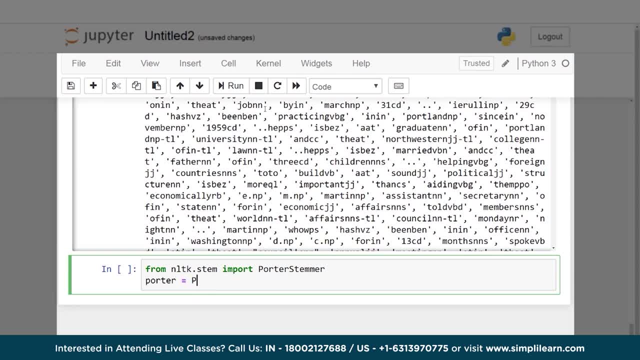 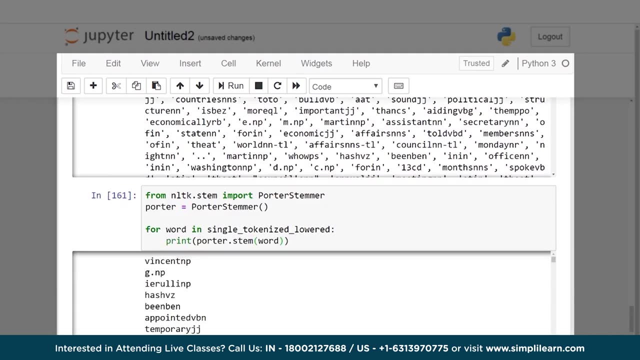 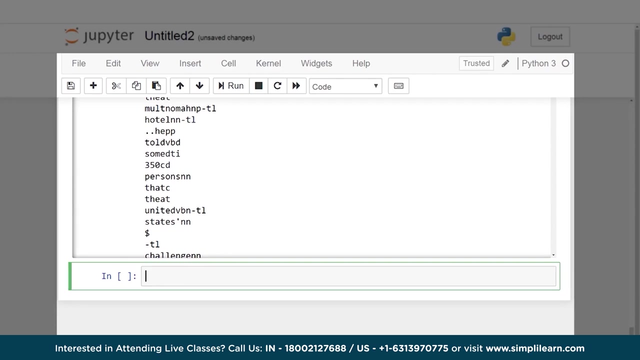 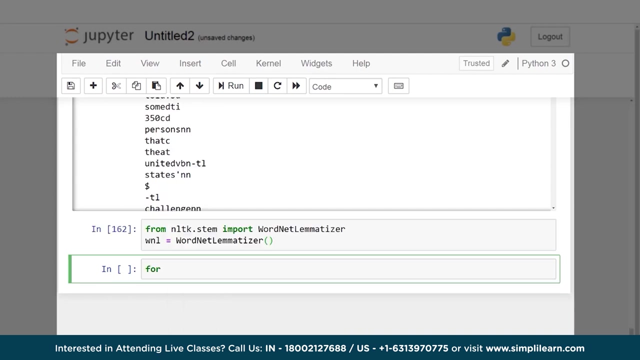 From NLTKSTEM: import Porter stemmer. Printing the stem words. Import the WordNet lemmatizer from NLTKSTEM Printing the root words. We also need to evaluate the POS tags for each token. From NLTKSTEM. import Porter stemmer. 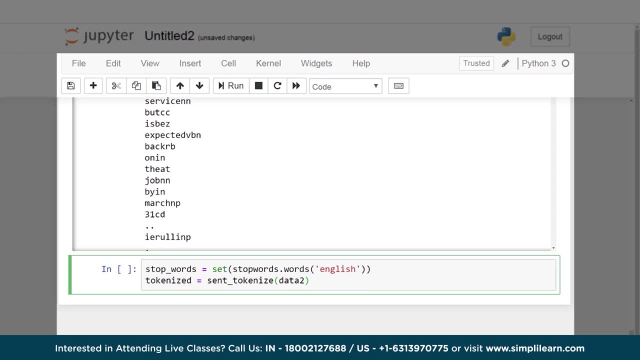 Create a new word list and store the list of word tokens against each of the sentence tokens in data2.. For I in tokenized. Also, we will check if there were any tokens in the text. Also, we will check if there were any tokens in the text. 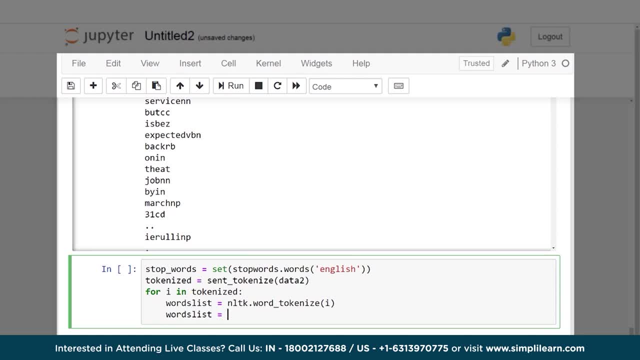 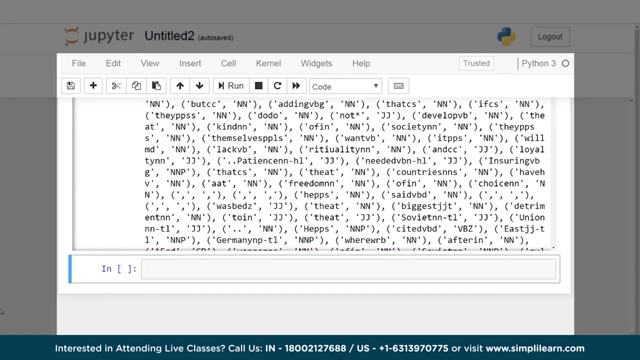 Also, we will check if there were any stop words in the recently created word list. We will now tag the word tokens accordingly using the POS tags and print the tagged output. For our final text processing task, we will be applying Named Entity Recognition to classify named entities in text into predefined categories. 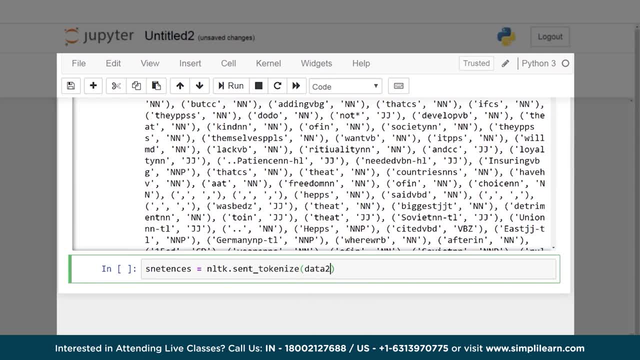 such as the names of persons, organizations, locations, expressions of times, quantities, monetary values, percentages, etc. Named Entity Recognition: If we set the parameter binary equals true, then named entities are just tagged as NE. Otherwise, the classifier adds category labels such as person, organization and GPE. 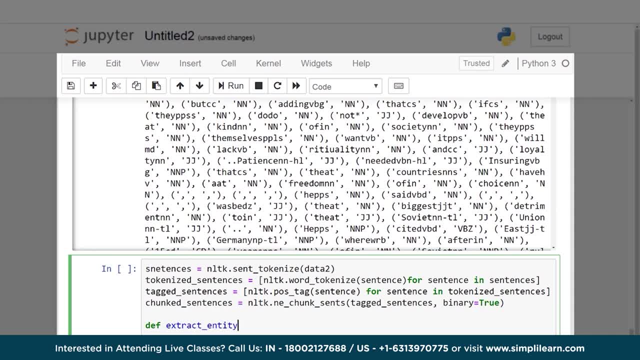 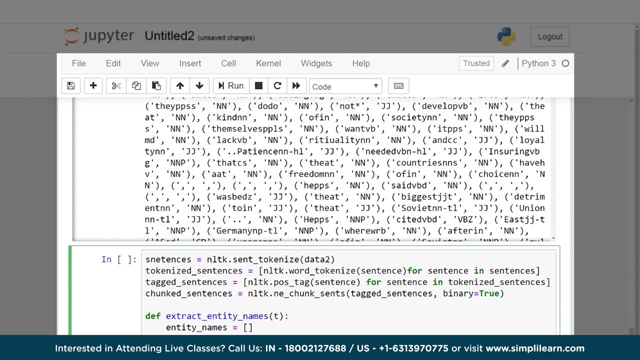 Create a function named as Extract Entity Names along with an empty list named as Entity Names. We will now extract named entities from a NLTK chunked expression and store them in the empty created above. Create a function named as Extract Entity Names, along with an empty list named as Entity Names. 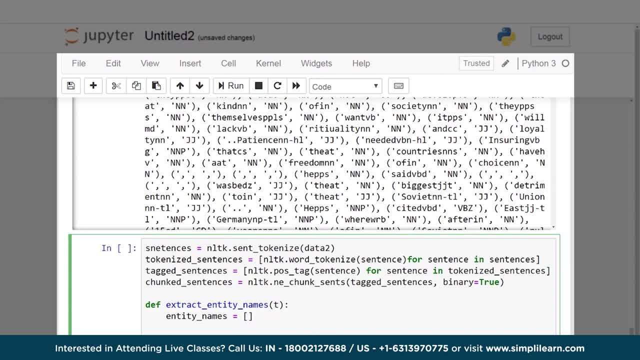 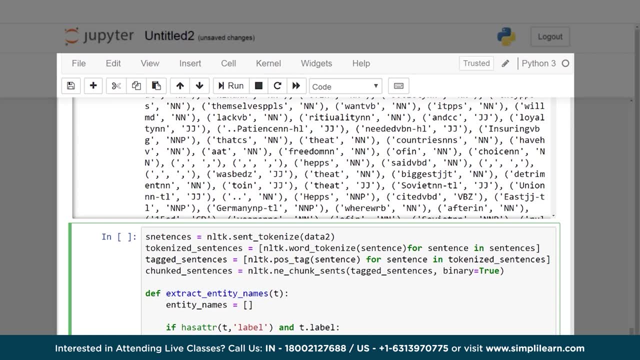 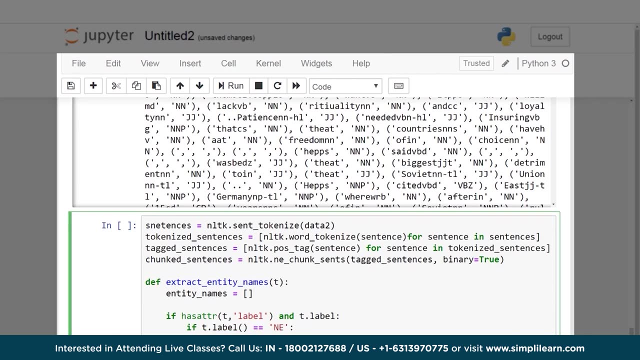 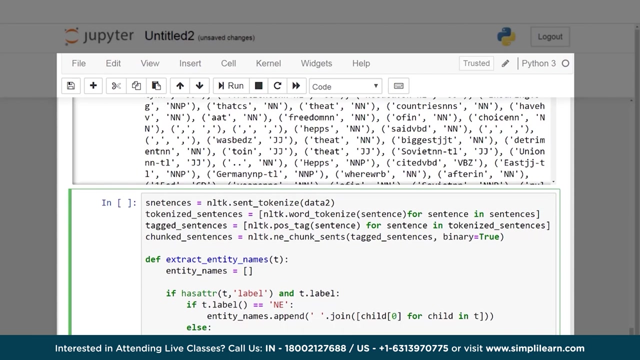 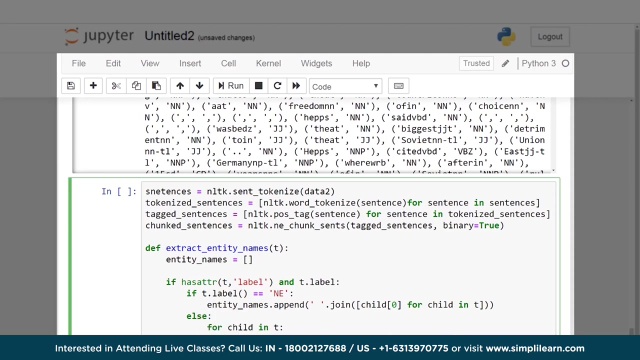 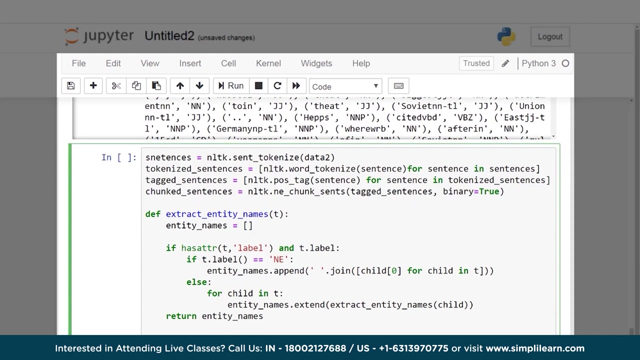 Create a function named as Extract Entity Names along with an empty list named as Entity Names. Again, we will set the Entity Names list as an empty list and will extract the Entity Names by iterating over each tree in chunked sentences. Create a function named as Extract Entity Names along with an empty list named as Entity Names. 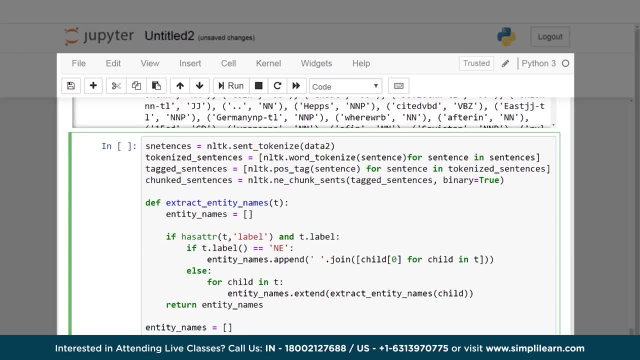 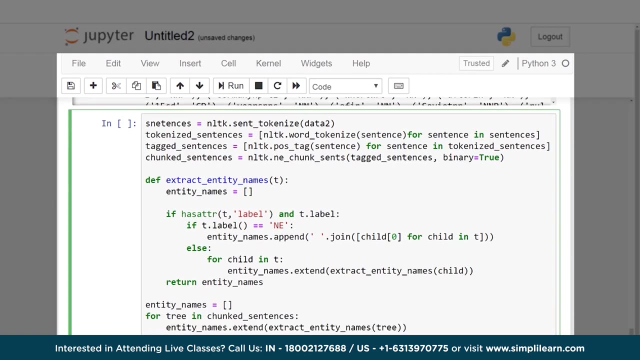 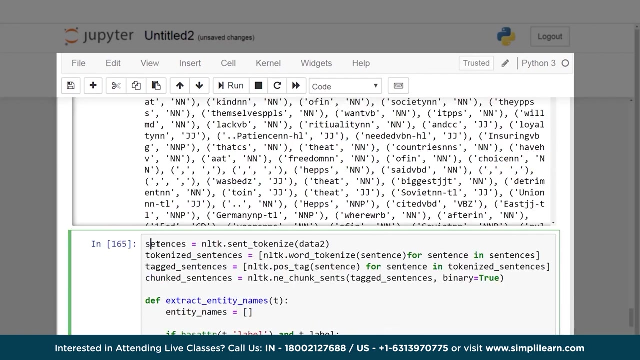 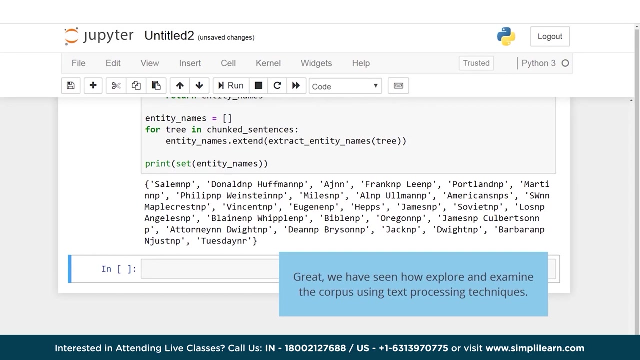 Create a function named as Extract Entity Names along with an empty list named as Entity Names. Create a function named as Extract Entity Names along with an empty list named as Entity Names. Great, we have seen how to explore and examine the corpus using text processing techniques. 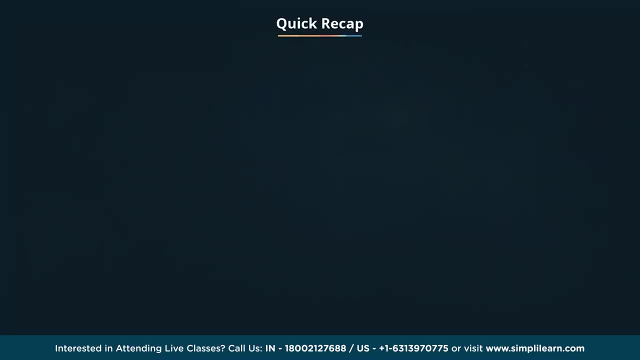 Let's quickly recap the steps we've covered so far: 1. Import the text. 2. Import the NLTK library. 3. Perform tokenization. 4. Perform stemming and lemmatization. 5. Perform named entity recognition. 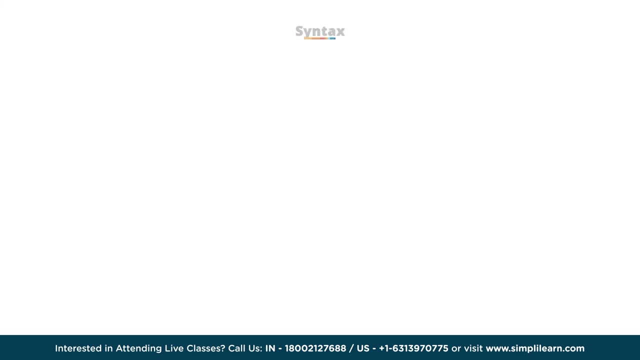 Structuring Sentences – Syntax. Let's first understand what syntax is. Syntax is the grammatical structure of sentences. In the given example, this can be interpreted as syntax and it is similar to the ones you use while writing. Knowing a language includes the power to construct phrases and sentences out of morphemes and words. 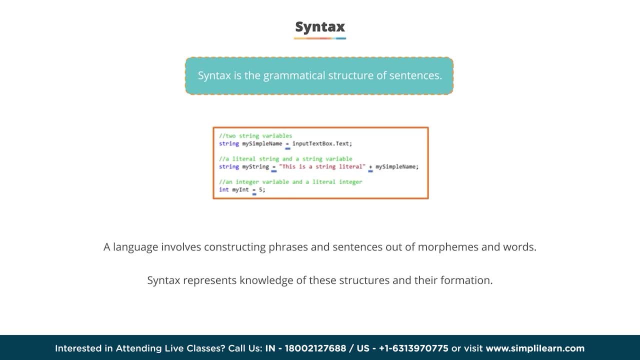 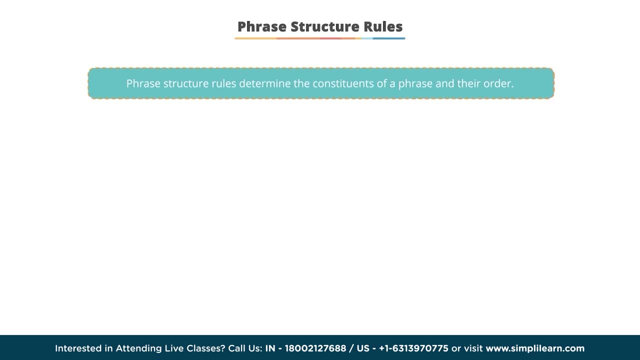 The part of the grammar that represents a speaker's knowledge of these structures and their formation is called syntax. Phrase. structure rules are rules that determine what goes into a phrase, that is, constituents of a phrase, and how the constituents are ordered. Constituent is a word or group of words that operate as a unit and can be used to frame larger grammatical units. 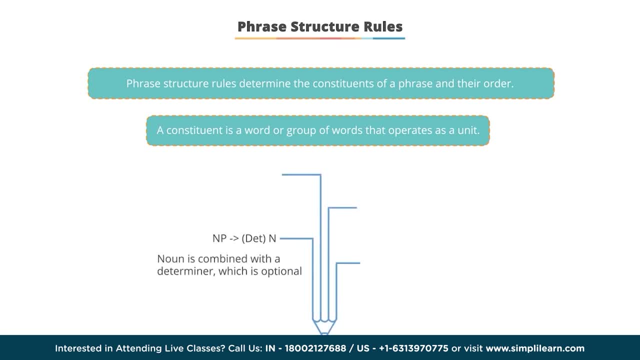 The given diagram represents that is determined when a noun is combined with a determiner and the determiner, an be optional. is determined when a noun phrase is combined with a verb phrase. is determined when a verb is combined optionally with the noun phrase and propositional phrase. 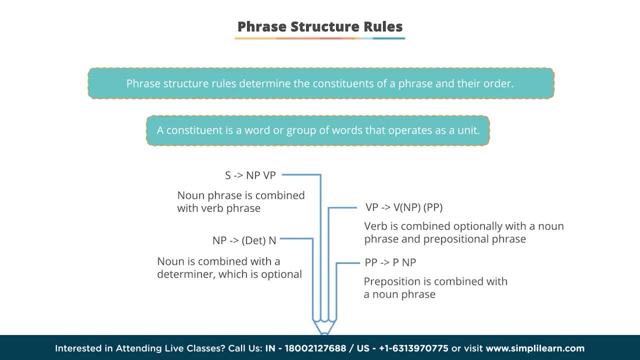 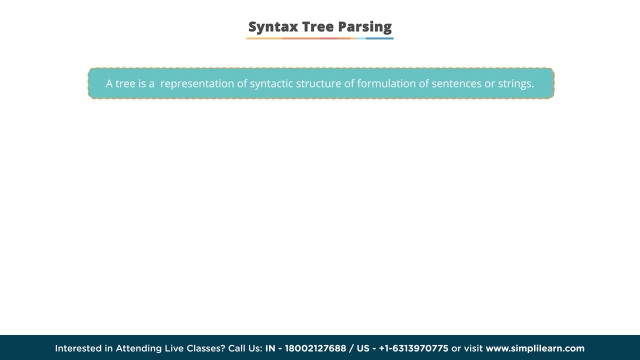 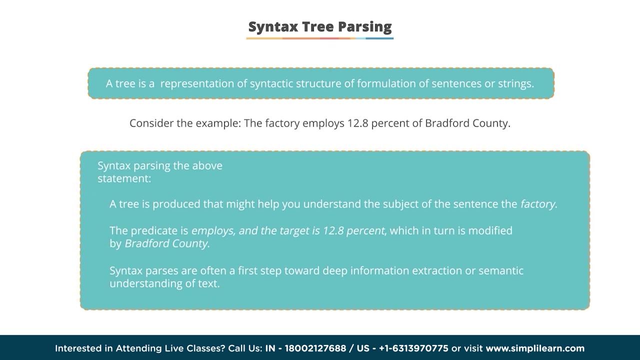 is determined when a preposition is combined with a noun phrase. a tree is a representation of syntax board text dialect. okay, structure of formulation of sentences or strings. consider the given sentence: the factory employs 12.8 percent of bradford county. what can be the syntax for pairing this statement? 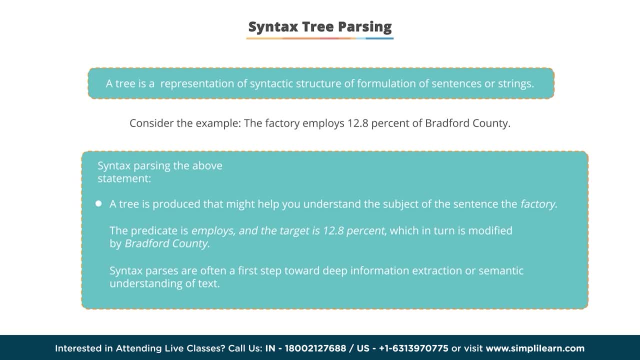 let's understand this: a tree is produced. that might help you understand that the subject of the sentence is the factory, the predicate is employs and the target is 12.8 percent, which in turn is modified by bradford county. syntax parses are often a first step toward deep 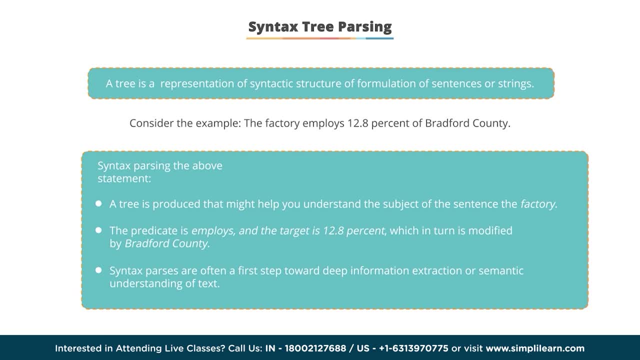 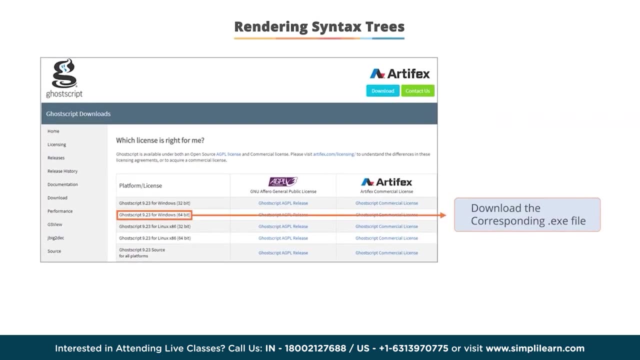 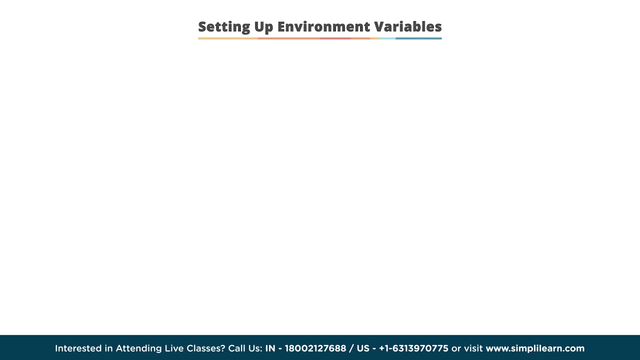 information extraction or semantic understanding of text. rendering syntax trees. download the correspondingexe file to install the ghost script rendering engine, based on your system configuration, in order to render syntax trees in your notebook. let's understand how you can set up the environment very variable. once you have downloaded and installed the file, go to the folder where it is installed. 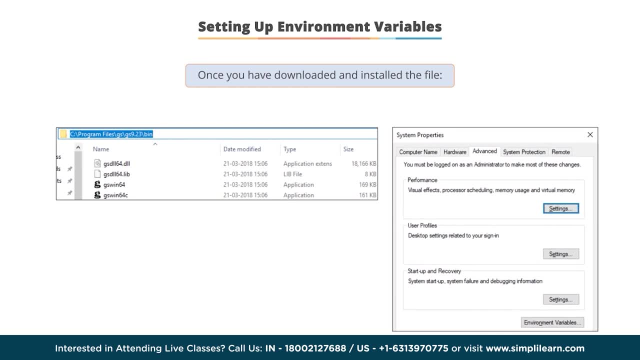 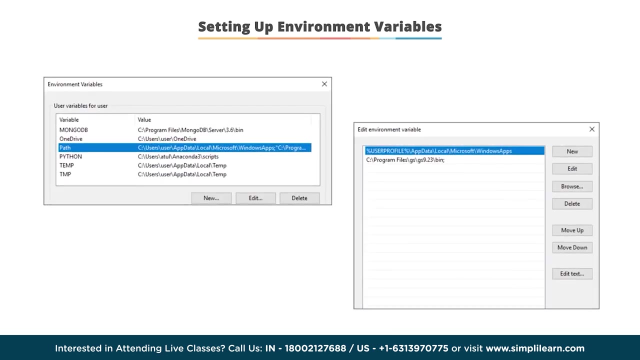 and copy the path of the file. now go to system properties and under advanced properties you will find the environment variable button. click on that to open the pop-up box tab of the environment. now open the bin folder and add the path to the bin folder in your environment variables. 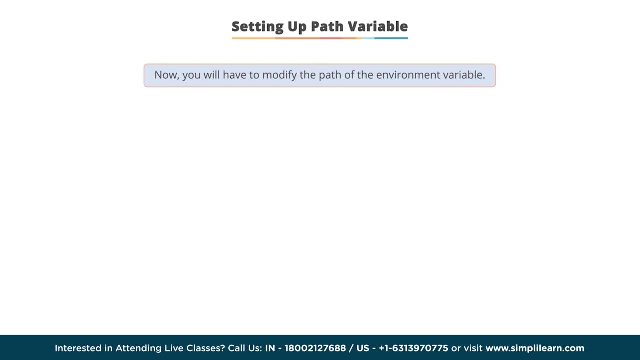 now you will have to modify the path of the environment variable and then select the path trove button. that you have done already. to make it比 from the configuration volume, we're going to create the path to the bin, then set up the bin folder with a raw code and in the bin folder to create the text. 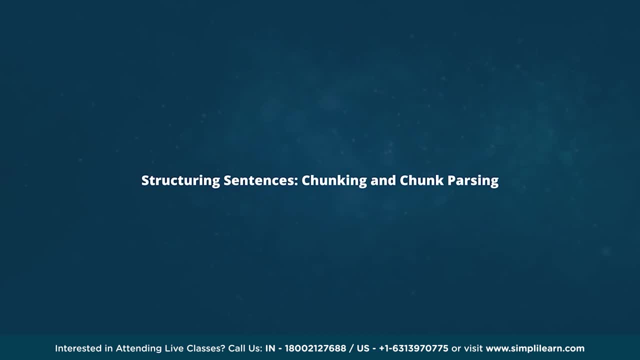 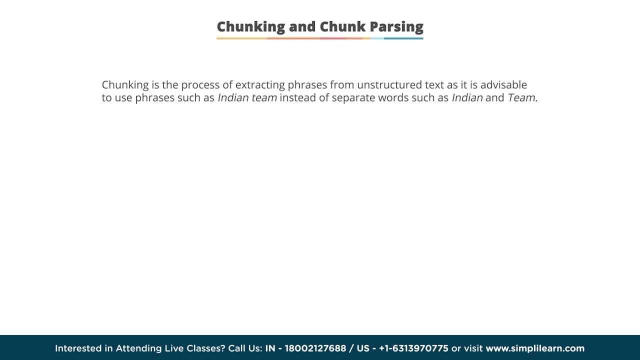 tree. use the given code to test the working of syntax tree after the setup is successfully installed. structuring sentences, chunking and chunk parsing. the process of extraction of phrases from unstructured text is called chunking. instead of using just simple tokens which may not represent the actual meaning of the text, it is advisable to use phrases such as indian team as a single word. 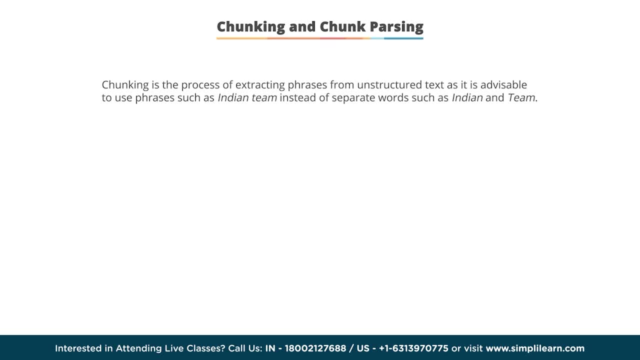 instead of Indian and team as separate words. The chunking segmentation refers to identifying tokens and labeling refers to identifying the correct tag. These chunks correspond to mixed patterns. in some way To extract patterns from chunks we need chunk parsing. The chunk parsing segment refers to identifying strings of tokens. 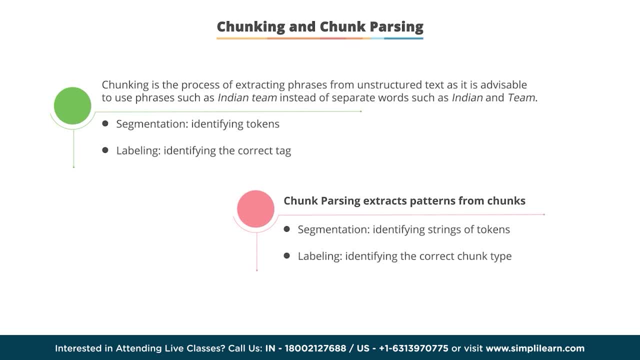 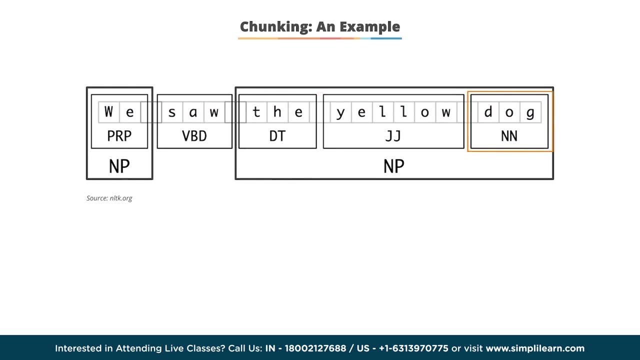 and labeling refers to identifying the correct chunk type. Let's look at the given example. You can see here that yellow is an adjective, dog is a noun and the is the determiner, which are chunked together into a noun phrase. Similarly, chunk parsing is used to extract patterns. 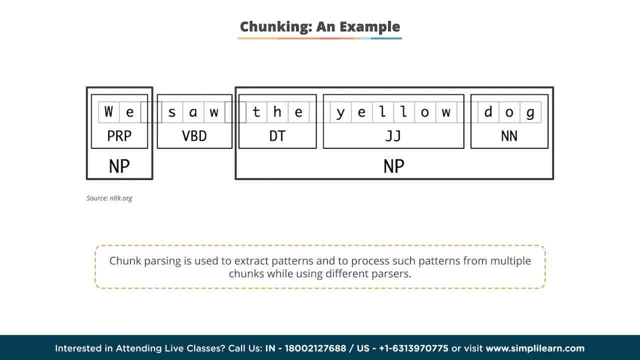 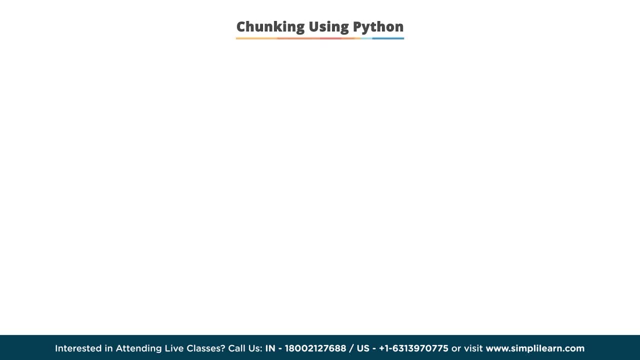 and to process such patterns from multiple chunks while using different parsers. Let's take an example and try to understand how chunking is performed in Python. Let's consider the sentence: The little mouse ate the fresh cheese assigned to a variable named cinch. 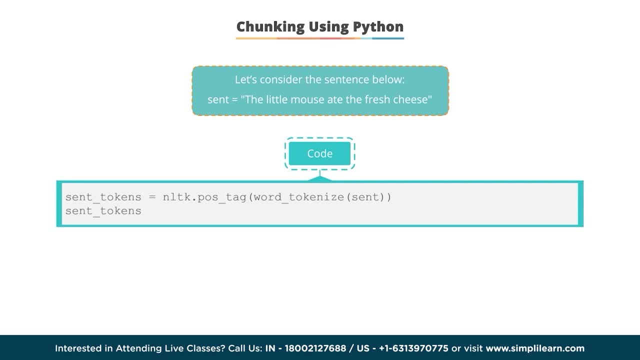 Using the word tokenize function under NLTK corpora, you can find out the different tags associated with the sentence provided. So, as you can see in the output, different tags have been allocated against each of the words from the given sentence using chunking. 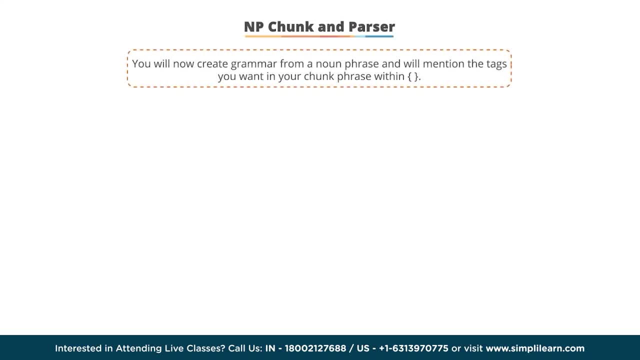 NP chunk and parser. You will now create grammar from a noun phrase and will mention the tags you want in your chunk phrase within the function. Here you have created a new function and you have created a regular expression matching the string The given regular expression indicates. 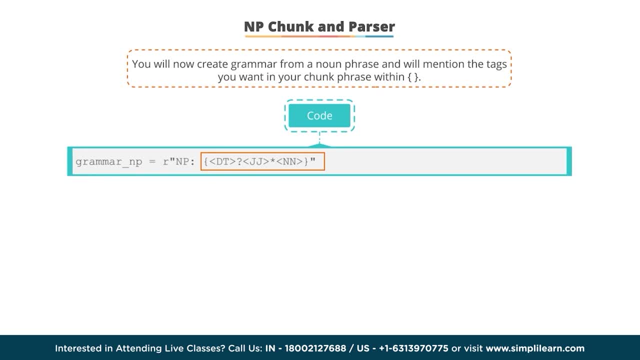 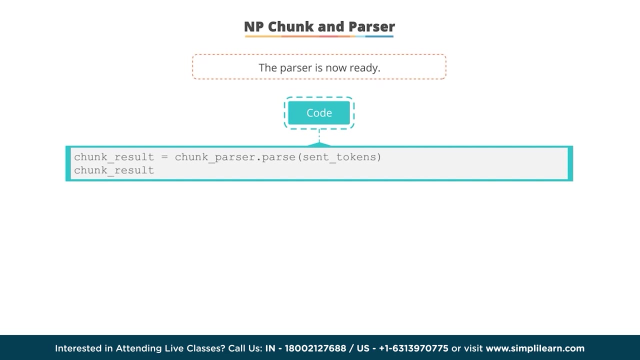 optional determiner, followed by optional number of adjective, followed by a noun. You will now have to parse the chunk. therefore, you will create a chunk parser and pass your noun phrase string to it. The parser is now ready. You will use the parse within your chunk parser to parse your sentence. 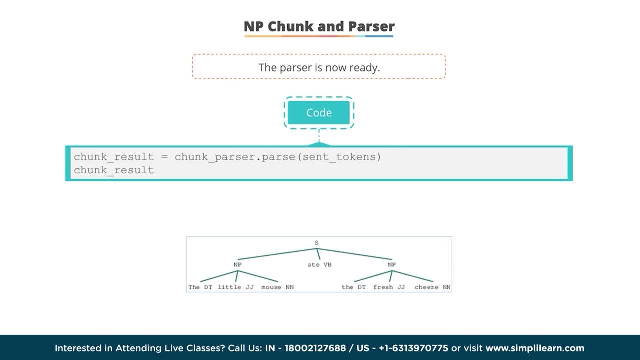 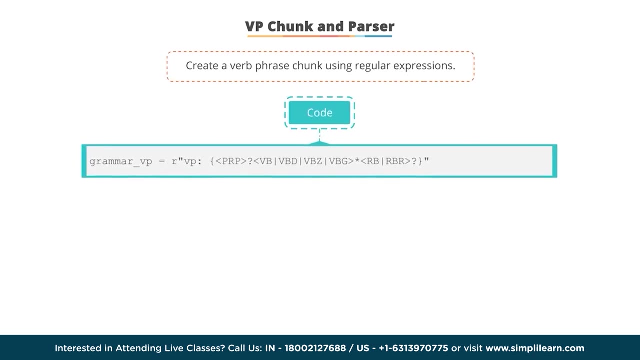 The sentence provided is: the little mouse ate the fresh cheese. This sentence has been parsed and the tokens that match the regular expressions are chunked together into noun phrases. NP: Create a verb phrase chunk using regular expressions. The regular expression has been defined as optional personal pronoun. 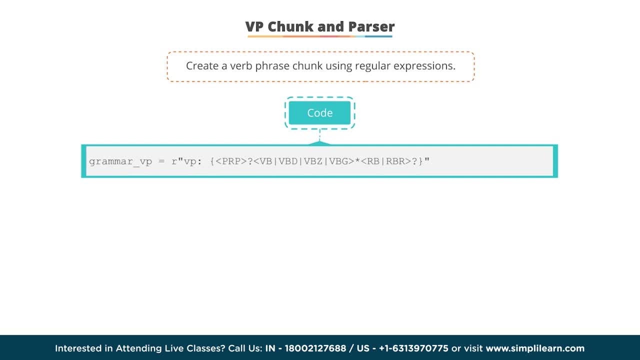 followed by zero or more verbs with any of its type, followed by any type of adverb. You will now create another chunk parser and pass the verb phrase string to it. Create another sentence with any of its type, followed by any type of adverb. 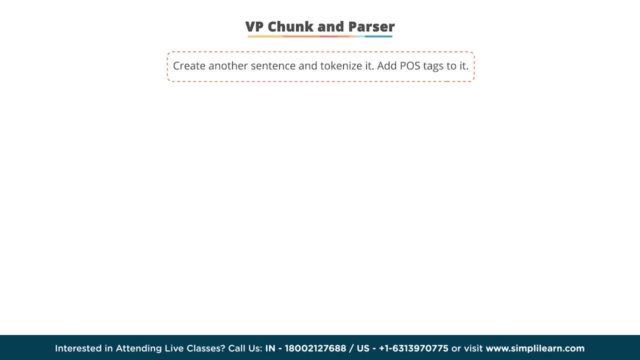 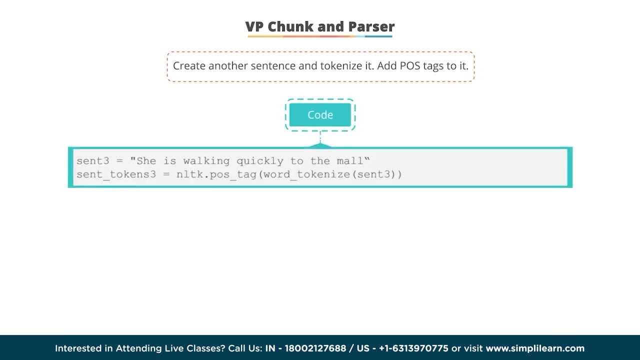 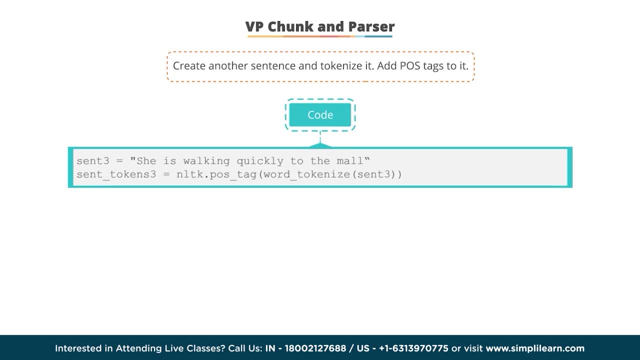 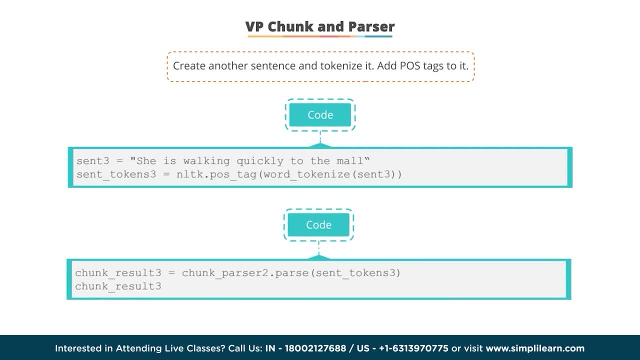 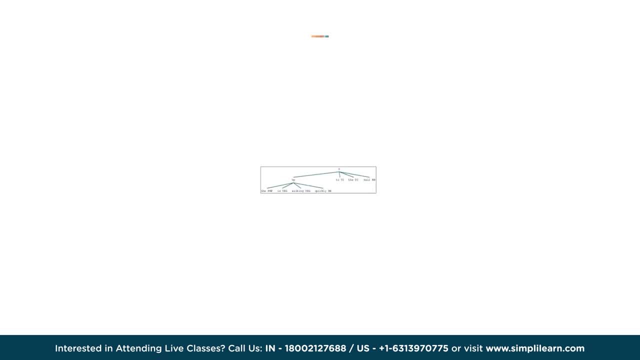 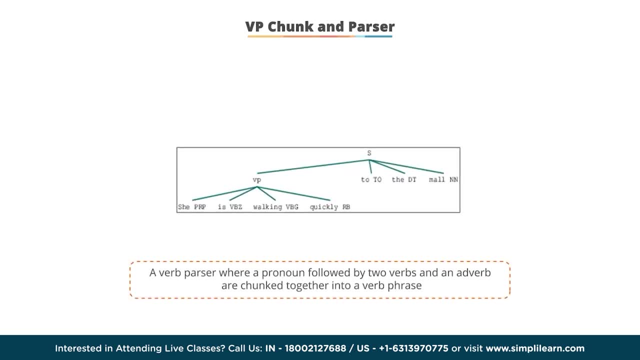 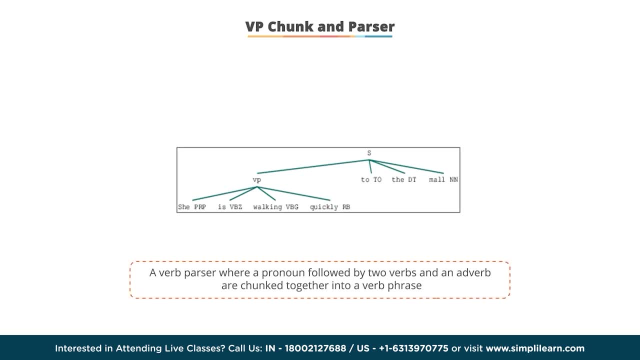 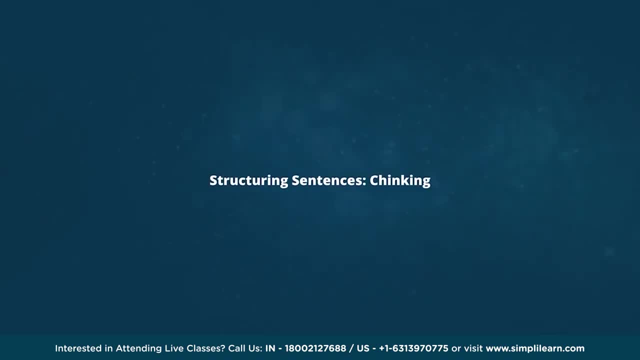 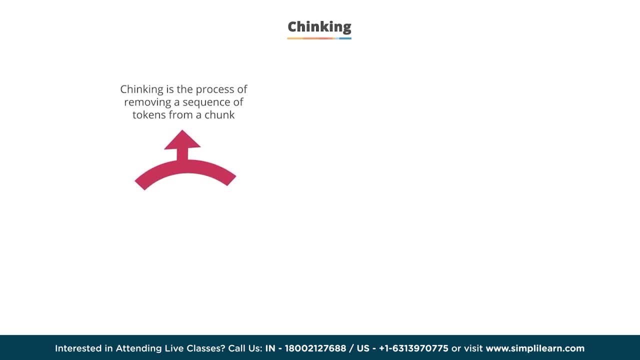 You will now create another chunk parser and pass the verb phrase string to it. You will now create another chunk parser and pass the verb phrase string to it. Chunking is the process of removing a sequence of tokens from a chunk. How does chunking work? 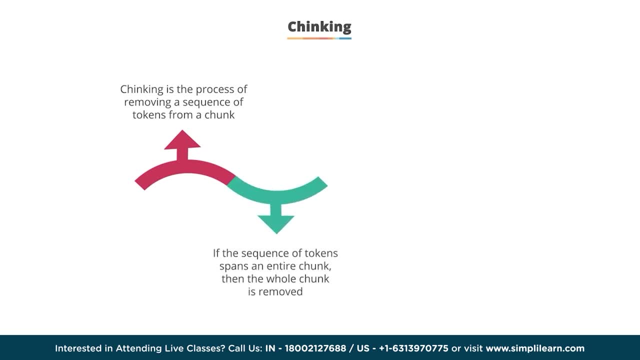 The whole chunk is removed when the sequence of tokens spans an entire chunk. If the sequence is at the start or the end of the chunk, the tokens are removed from the start and end and a smaller chunk is retained. If the sequence of tokens appears in the middle of the chunk, these tokens are removed, leaving. 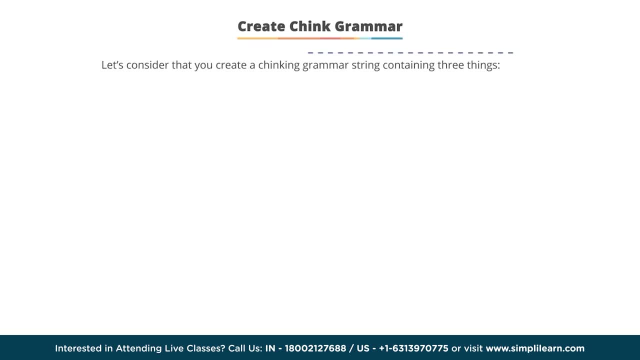 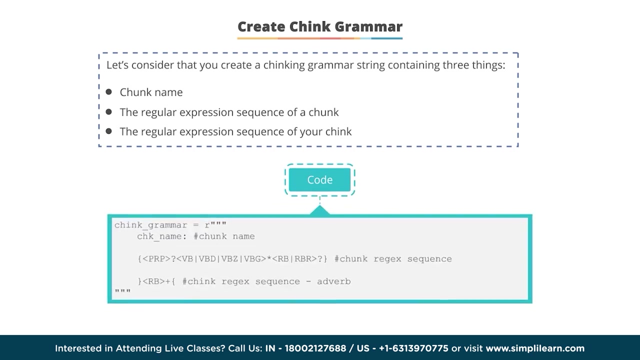 two chunks where there was only one before. Here you create a chinking grammar string containing three things: chunk name. the regular expression sequence of a chunk. the regular expression sequence of your chink. Here in the given code we have the chunk regular expression as optional personal pronoun followed. 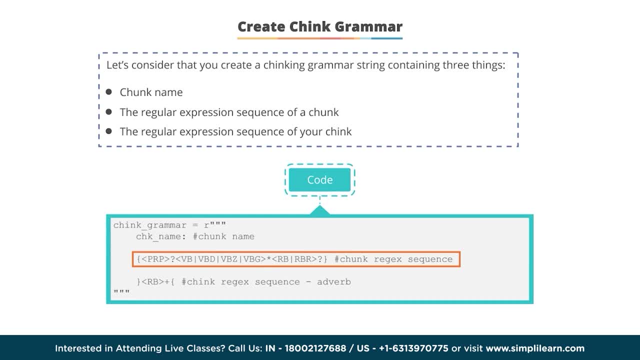 by zero or more occurrences of any type of the verb type, followed by zero or more occurrences of any of the adverb types. The chink regular expression says that it needs to check for the adverb in the extracted chunk and remove it from the chunk. 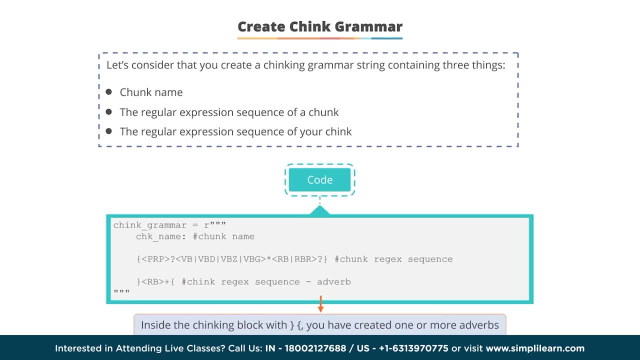 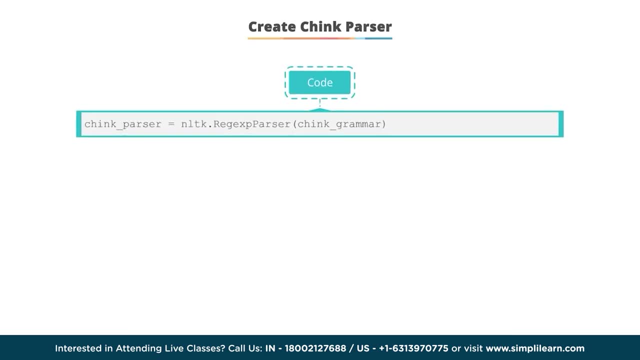 Inside the chinking block with open curly braces and closing curly braces. you have created one or more adverbs. You will now create a parser from nltkregexpparser and pass the chink grammar to it. Now use the new chink parser to parse the tokens sent3 and run the results. 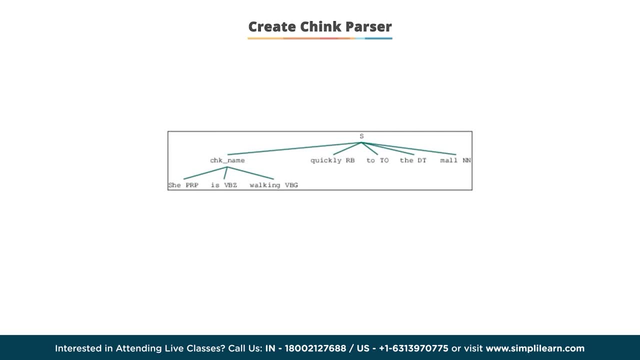 As you can see, the parse tree is generated. While comparing the syntax tree of the chink parser with that of the original chunk, you can see that the token is quickly chinked out of the chunk. Let's understand how to use context-free grammar. 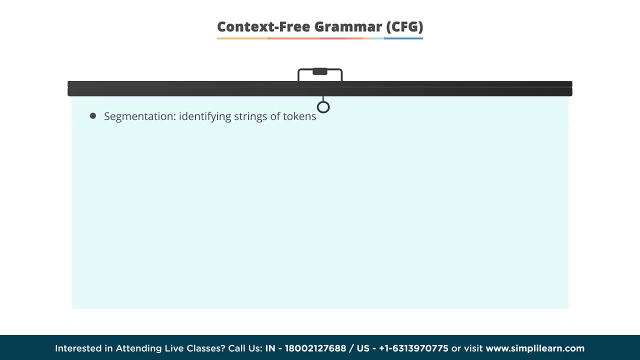 A context-free grammar is a four-tuple sum-n-t-r-s, where sum is an alphabet and each character in sum is called a terminal, nt is a set and each element in nt is called a non-terminal r. the set of rules is a subset of nt times. the set of sum u and t s the start. 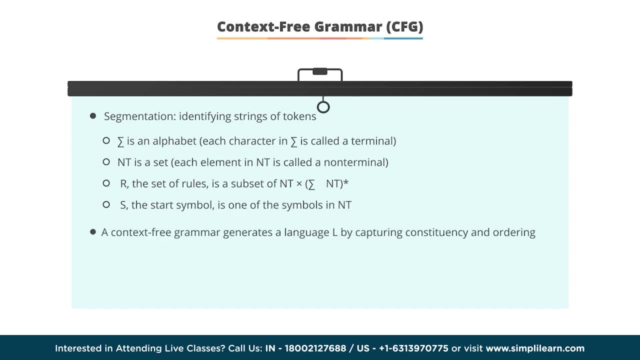 symbol is one of the symbols in nt. A context-free grammar generates a language, l capturing constituency and ordering. In cfg, the start symbol is used to derive the string. You can derive the string by repeatedly replacing a non-terminal on the right-hand side of the. 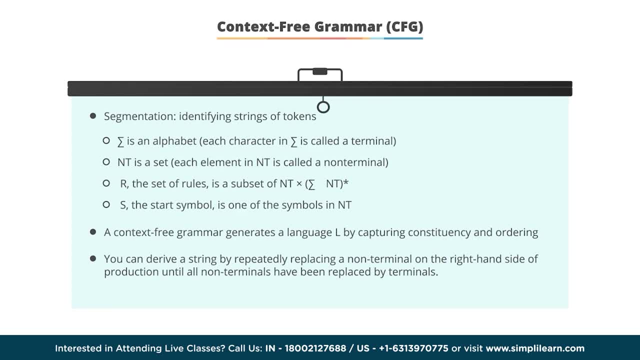 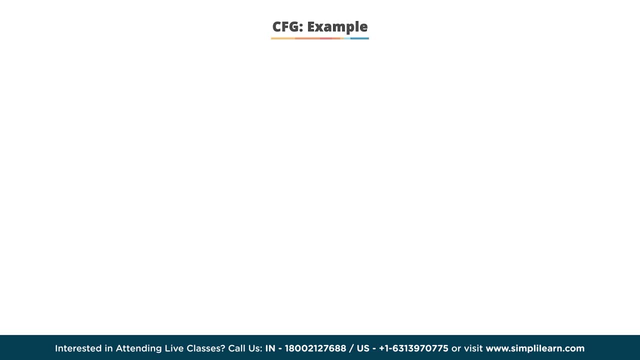 production Until all non-terminals have been replaced by terminal symbols. Let's understand the representation of context-free grammar through an example. in context-free grammar, A sentence can be represented as a noun phrase followed by a verb phrase. Noun phrase can be a determiner nominal. a nominal can be a noun. vp represents the. 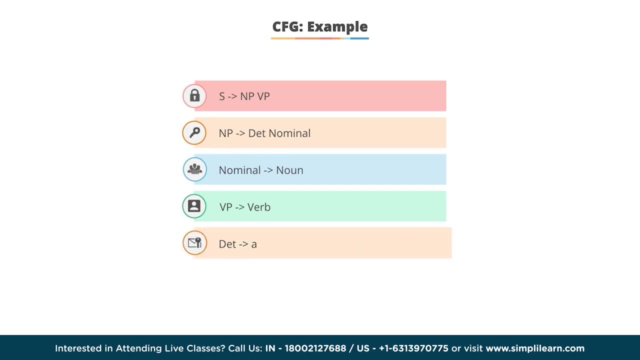 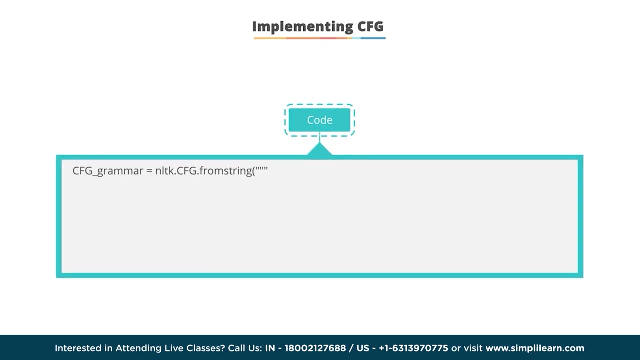 verb phrase. a can be called a determiner, flight can be called a noun. Consider the string below, where you have certain rules. When you look at the given context-free grammar, a sentence should have a noun phrase followed by a verb phrase. 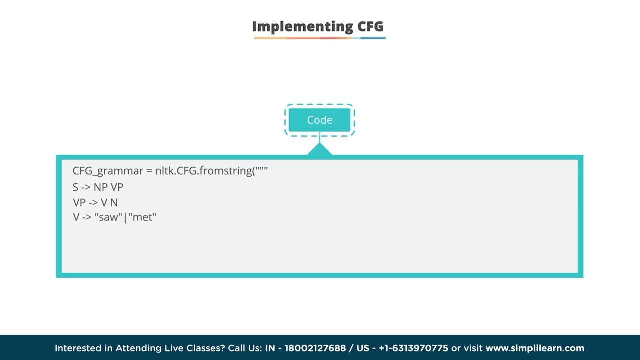 A verb phrase is a verb followed by a noun. A verb can either be saw or met, Noun phrases can either be John or Jim, and a noun can either be a dog or a cat. Check the possible list of sentences that can be generated using the rules. 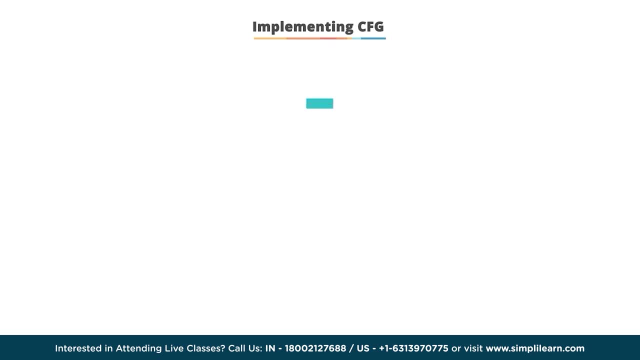 Use the join function to create the possible list of sentences. You can check the different rules of grammar for sentences. You can also use the join function to create the possible list of sentences. If you want a definition of the word, use the join function to create the possible list. 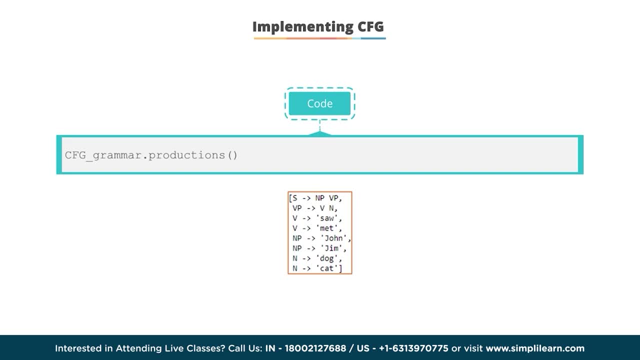 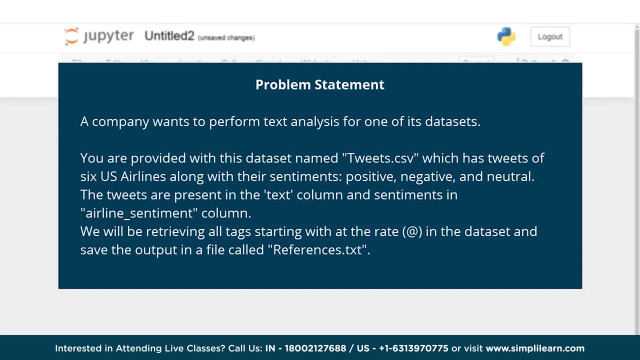 of sentences. Try out the new code to create the following code: Demo 2 – Structuring sentences. Problem statement – a company wants to perform text analysis for one of its datasets. You are provided with this dataset named tweetscsv, which has tweets of 6 US airlines, along with 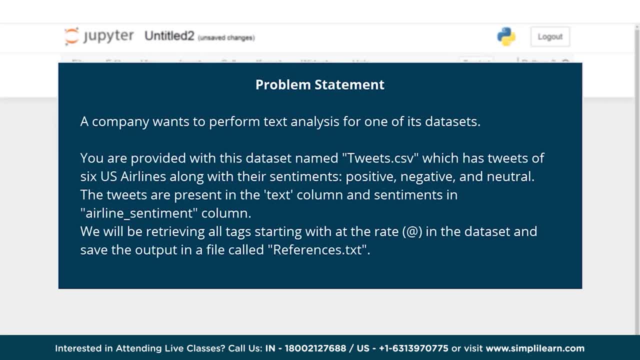 their sentiments: positive, negative and neutral. The tweets are present in the text field. When you open the text field, you can create a text-free grammar, the text column and sentiments in airline underscore sentiment column. We will be retrieving all tags, starting with at the rate in the dataset and save the output. 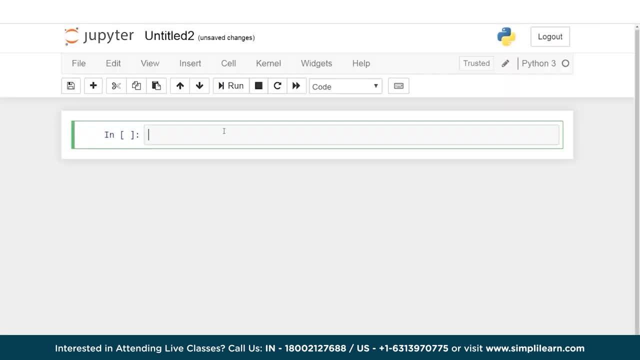 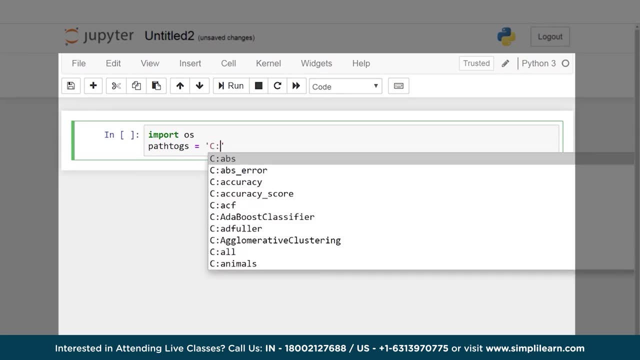 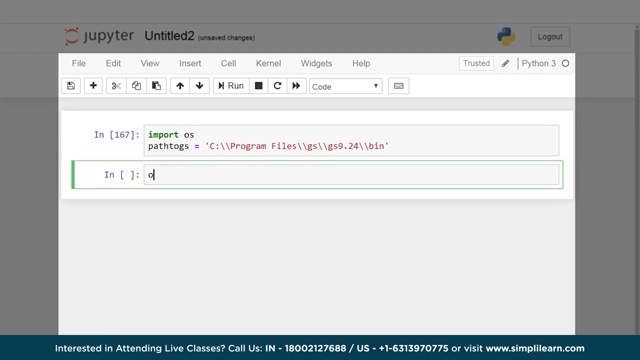 in a file called references dot txt. Let us first import the pandas library and read the tweets dataset. Let us first import the pandas library and read the tweets dataset. Let us first import the pandas library and read the tweets dataset. Extract the features, text and airline sentiment. 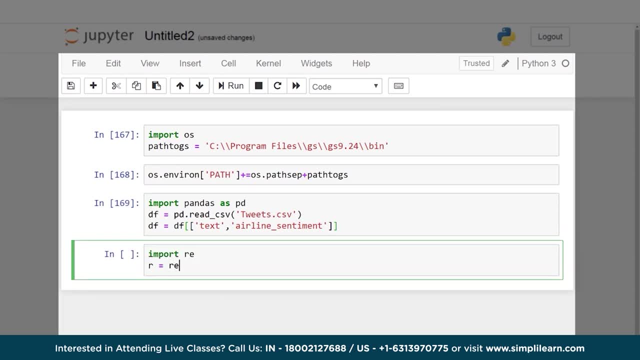 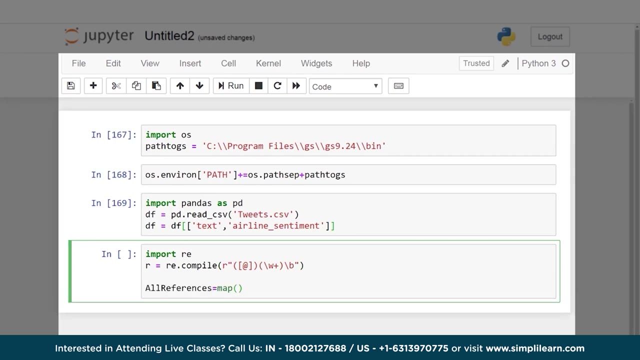 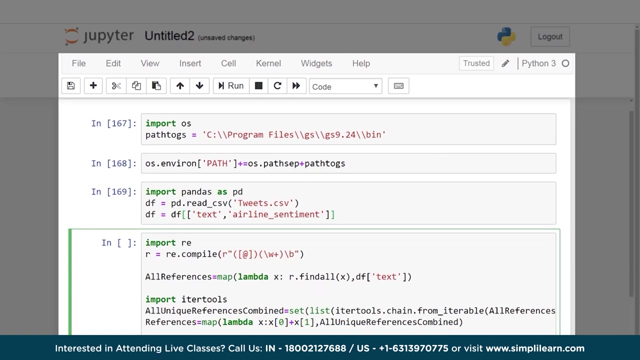 We will iterate through the dataset using reg x: find the relevant tweets. We will iterate through the dataset using reg x: find the relevant tweets. Now we will import the iter tools module. it returns efficient iterators. The result is stored in a file named referencestxt. 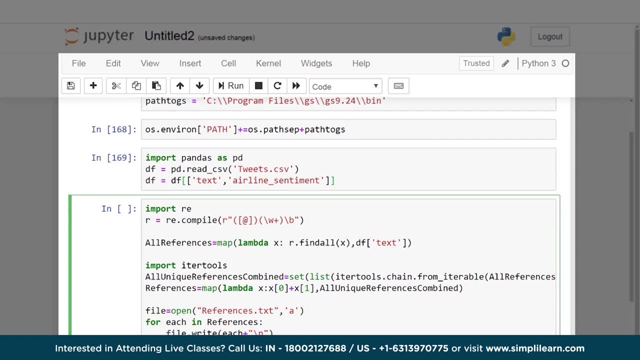 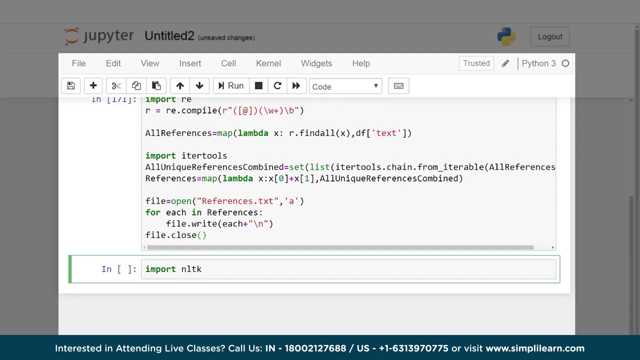 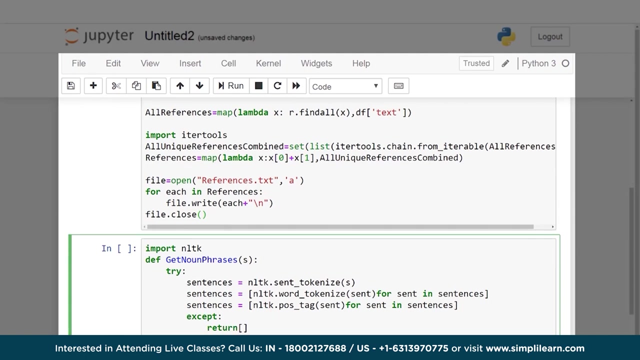 Let's extract all noun phrases and save them in a file named noun phrases for left caret- airline underscore, sentiment. right caret review dot txt. Thank you for watching Here. left caret- airline underscore, sentiment. right caret has three different values: positive, negative and neutral. so three files will be created. 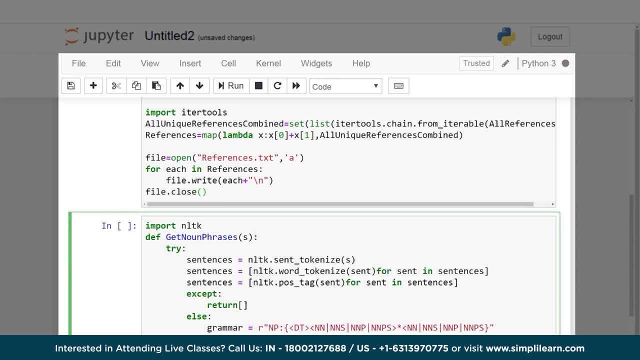 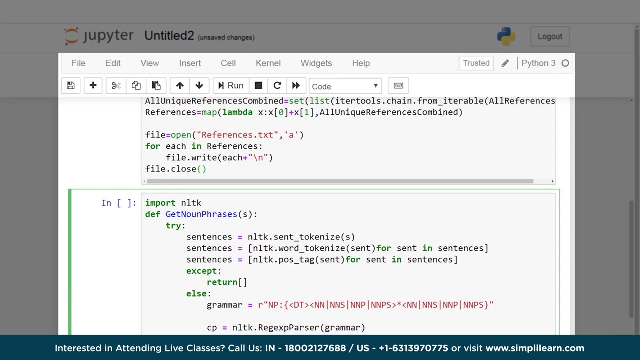 Now we will iterate all the leaf nodes and assign them to noun phrases: variable. Here left caret airline underscore sentiment. right caret has three different values: positive, negative and neutral. Here left caret, airline underscore sentiment. right caret has three different values: positive: 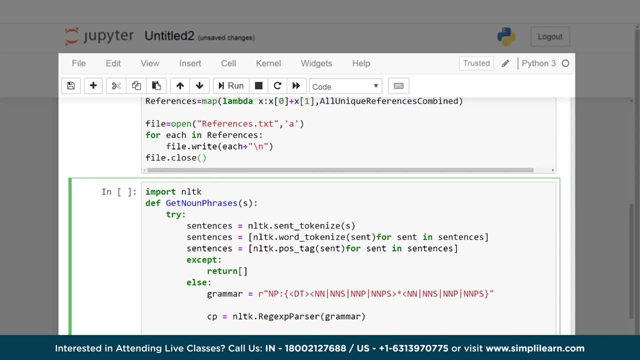 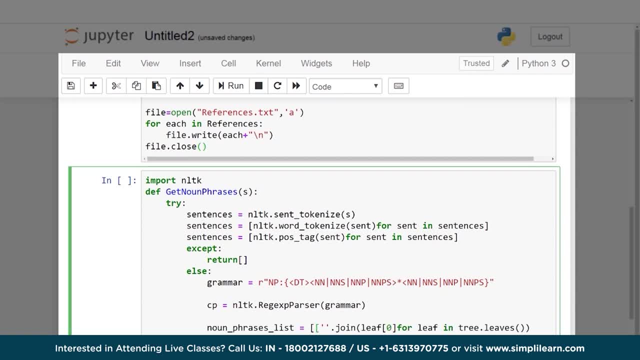 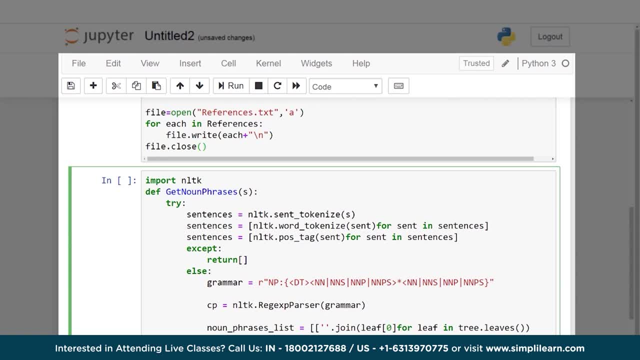 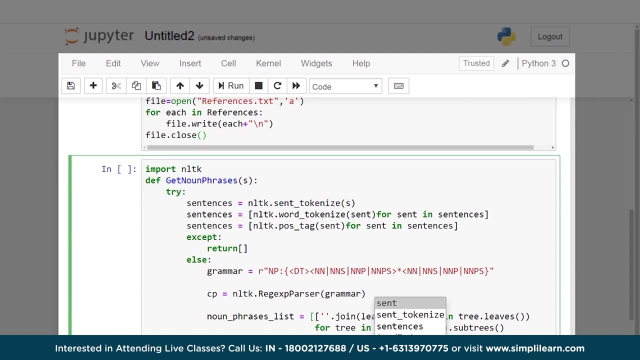 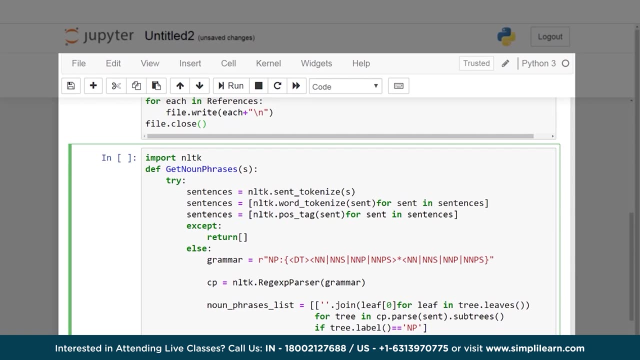 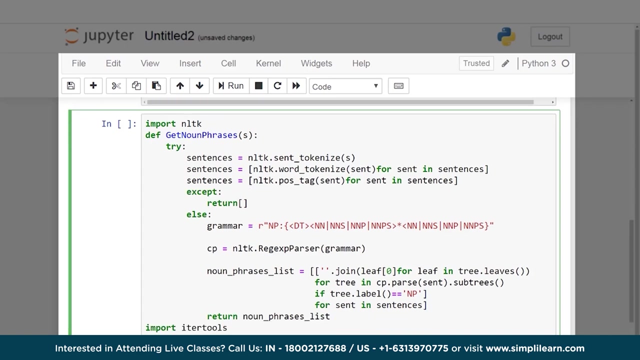 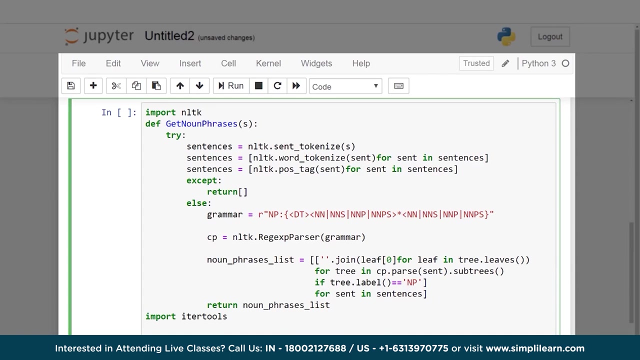 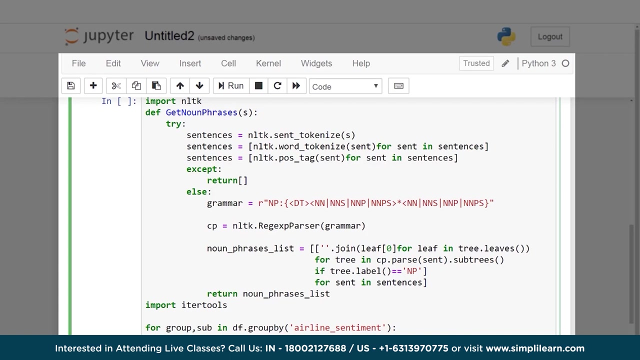 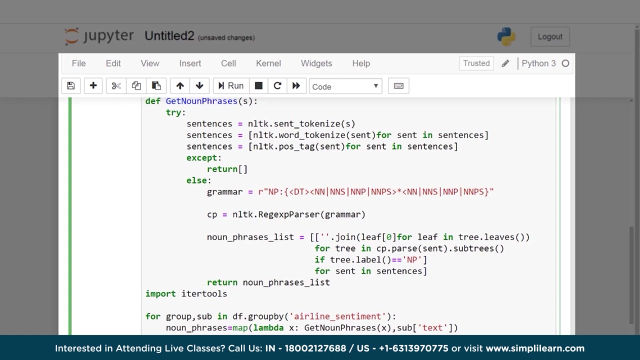 negative and neutral Here. left caret airline underscore sentiment, right caret still survives. This means that the functions in iter tools operate on iterators. to produce more complex iterators Using the map function, we will get all the noun phrases from the text, Putting it into list. 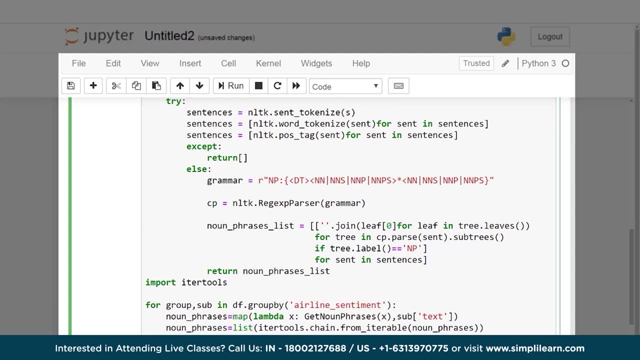 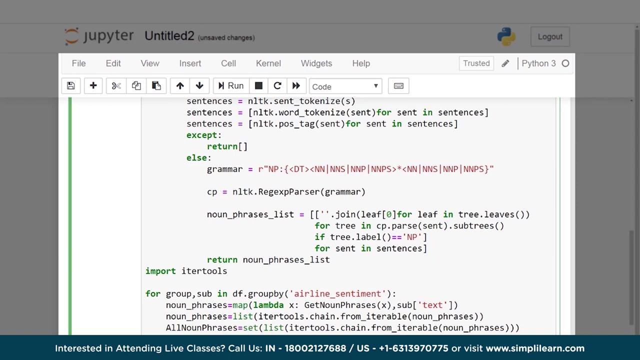 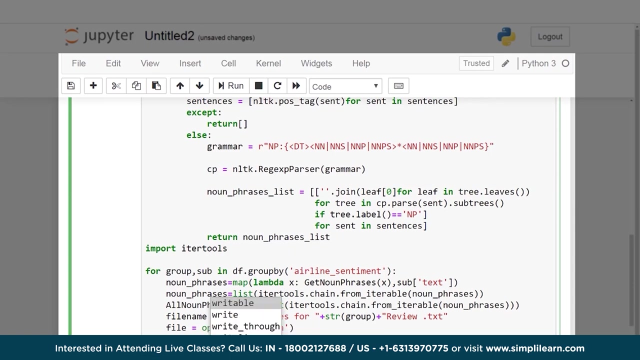 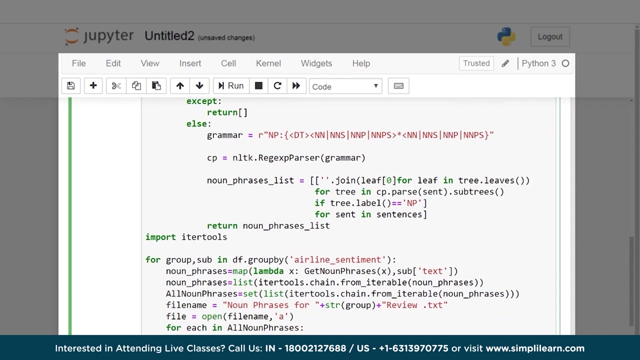 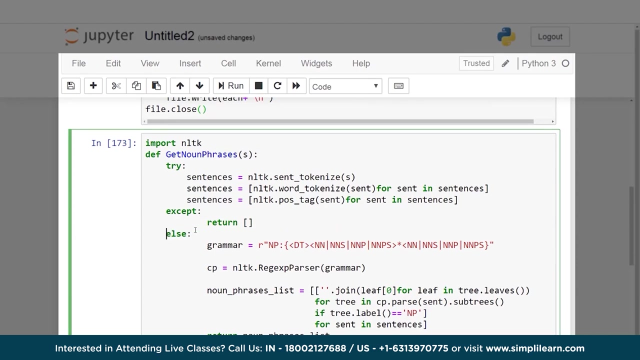 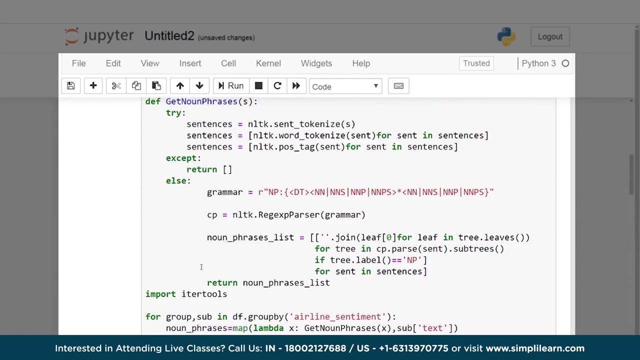 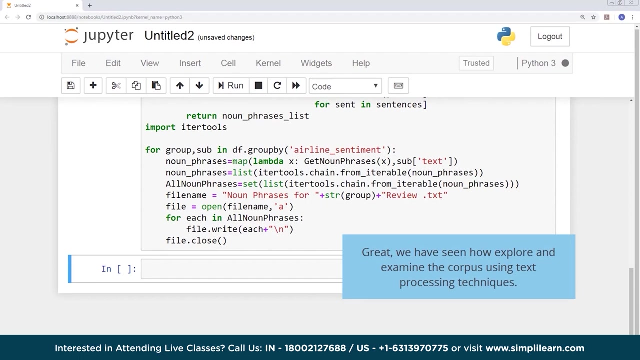 Creating a file name in the name of reviewtxt. making a abel file name. creating a abel file name. Click on Save etwd. Select the project language to choose from. Great, We have now seen how to explore and examine the corpus using text processing techniques. 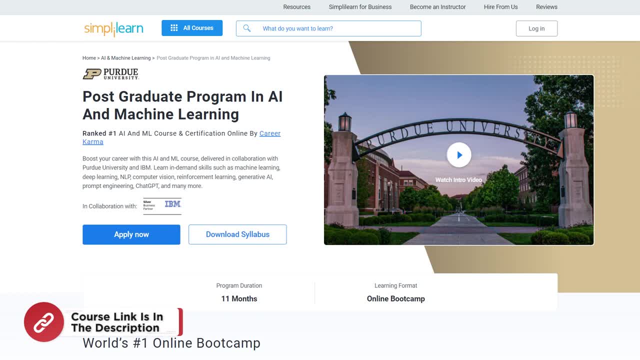 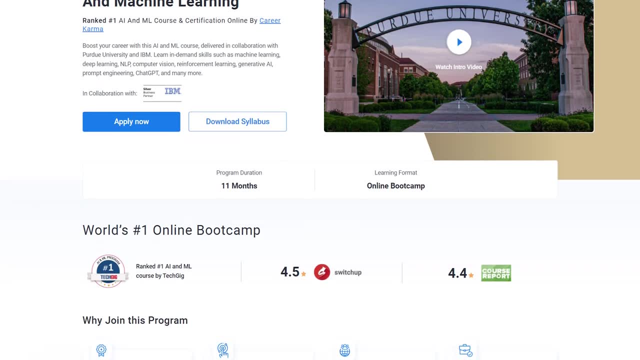 If you are looking for a course that covers everything from the fundamentals to advanced techniques, then accelerate your career in AI and Machine Learning with a comprehensive postgraduate program in AI and Machine Learning. Boost your career with this AI and ML course, delivered in collaboration with Purdue University and IBM. 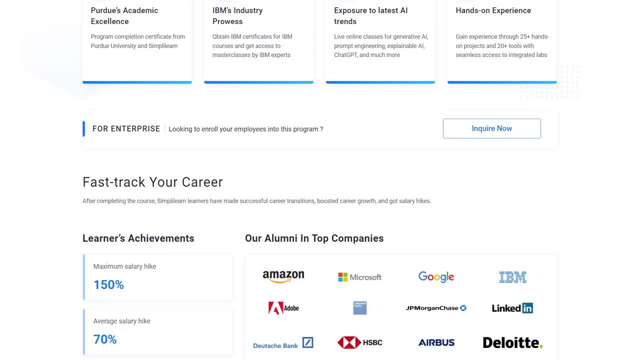 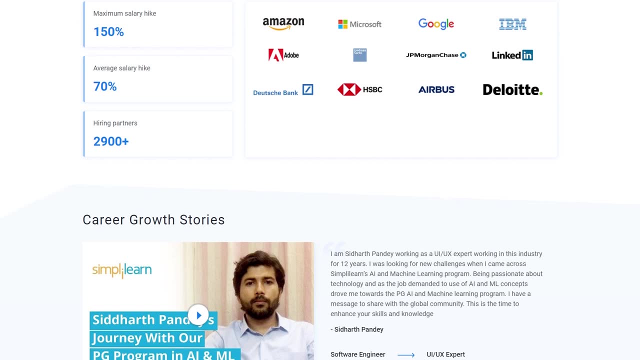 Learn in-demand skills such as Machine Learning, Deep Learning, NLP, Computer Vision, Reinforcement Learning, Generative AI, Prompt Engineering, ChatGPT and many more. You'll receive a prestigious certificate and Ask Me Anything. sessions by IBM. 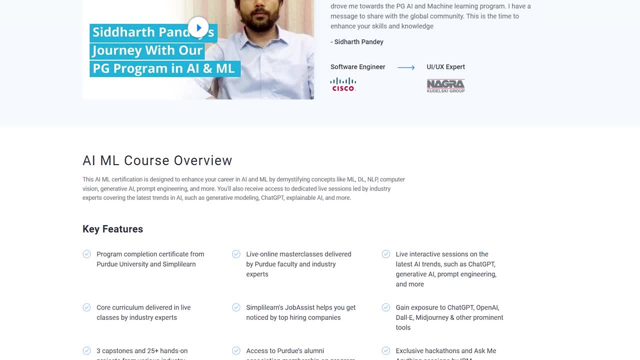 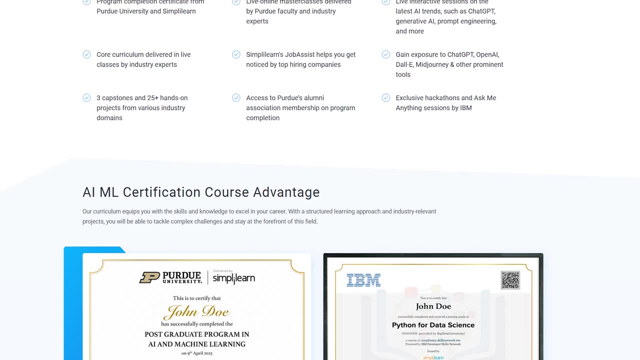 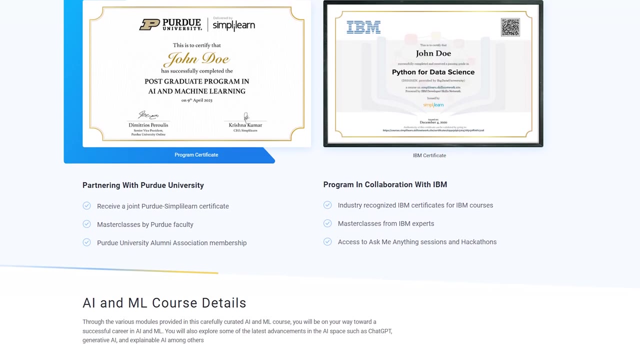 With five capstones in different domains, using real datasets. you'll gain practical experience. Masterclasses by Purdue faculty and IBM experts ensure top-notch education. Simply Learn's Job Assist helps you get noticed by leading companies. This program covers Statistics, Python, Supervised and Unsupervised Learning. 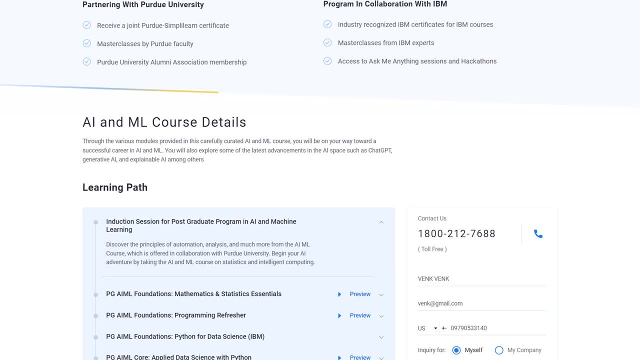 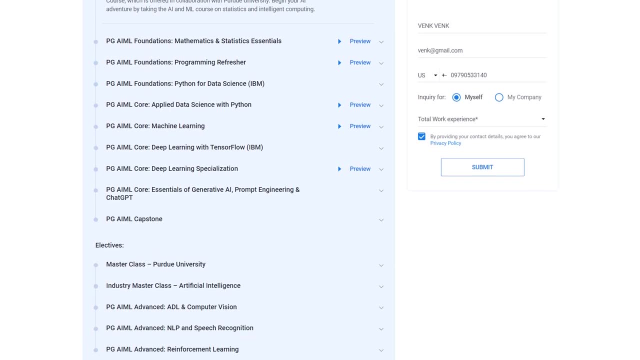 NLP, Neural Networks, Computer Vision, GANs, Keras, TensorFlow and many more such skills. Admission to this postgraduate program in AI and Machine Learning requires a bachelor's degree with an average of 50% or higher marks. 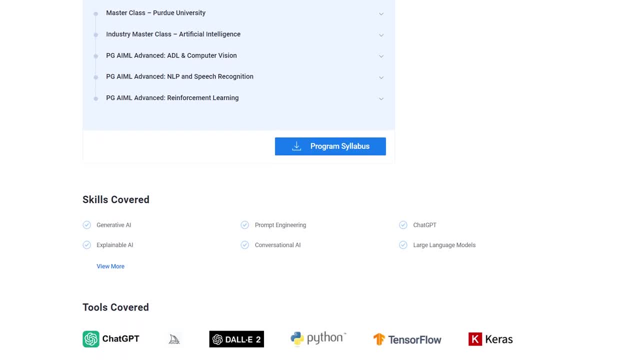 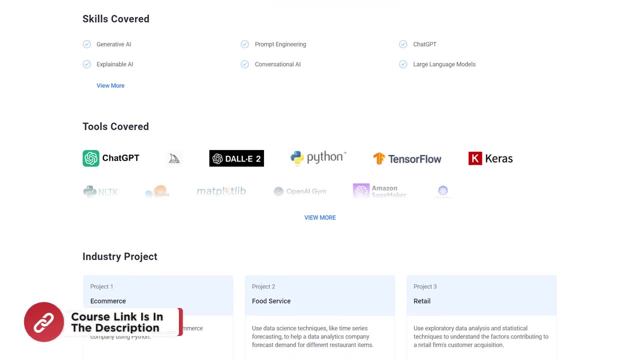 along with a basic understanding of programming concepts and mathematics, And candidates with 2 plus years of work experience are preferred to enroll in this school. So enroll now and unlock exciting AI and Machine Learning opportunities. The link is mentioned in the description box below. 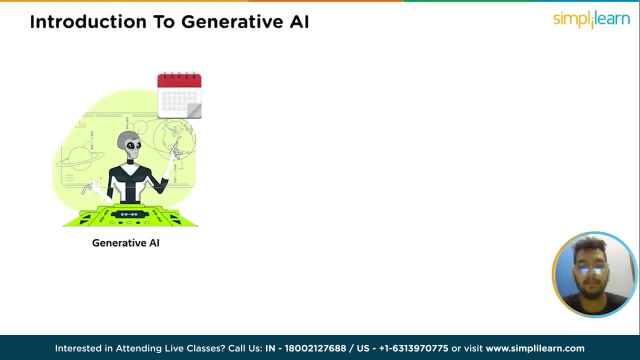 As you can see, Generative AI has emerged seemingly out of nowhere in recent months, With a notable surge in interest, according to Google Trends, even within the past year. The spike in curiosity can be attributed to the introduction of generative models such as Jale-2, BART and ChairGPT. 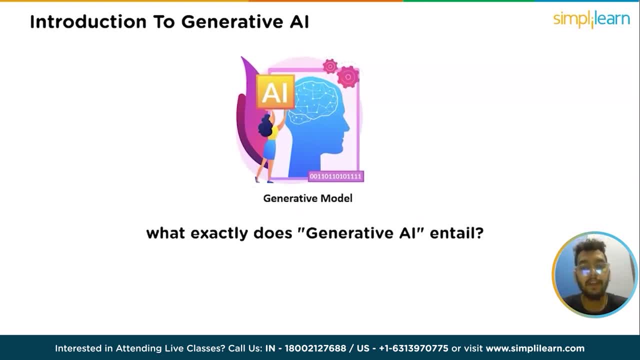 However, what does Generative AI entail? As a part of our introductory series on Generative AI, this video will provide a comprehensive overview of a subject starting from the basics. The explanation will cater to all levels of familiarity, ensuring that you are familiar with it. 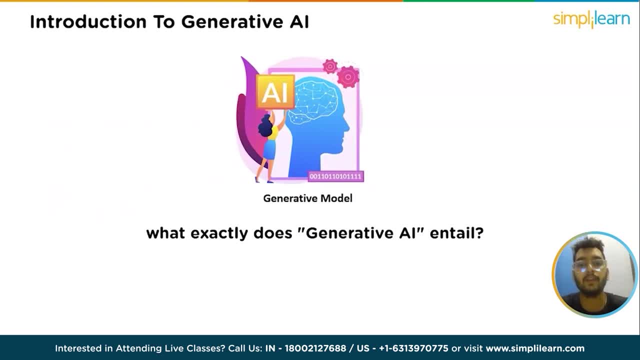 We hope this video will help you to gain a better understanding of how this technology operates and its growing integration to our daily lives. Generative AI is, after all, a tool that is based on artificial intelligence- A professional who elicits to switch careers with AI by learning from the experts. 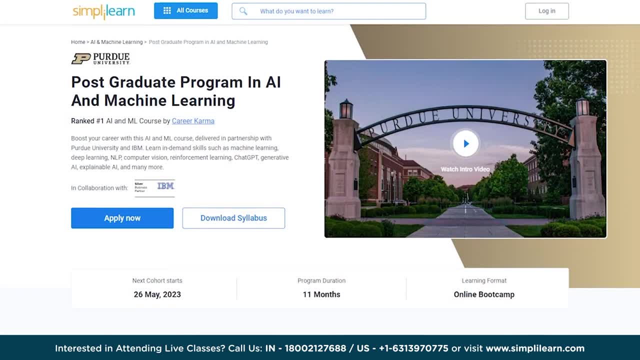 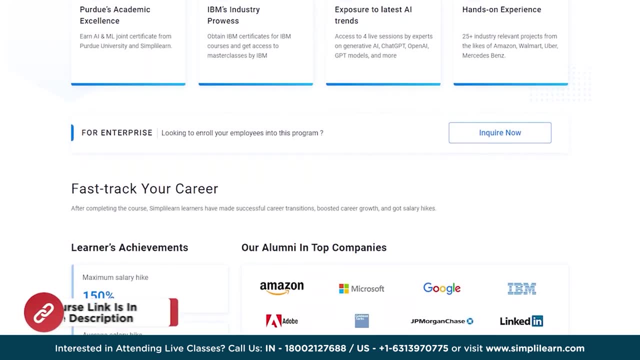 Then try giving a short, simple and postgraduate program in AI and Machine Learning from Purdue University in collaboration with IBM. The link in the description box should navigate to the home page, where you can find a complete overview of the program being offered. Take action, upskill and learn. 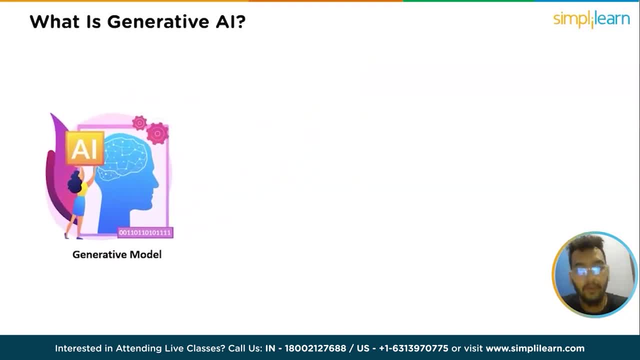 What is Generative AI? Generative AI is a form of artificial intelligence that possesses the capability to generate a wide range of content, including text, visual, audio and synthetic data. The recent excitement surrounding Generative AI stems from user-friendly interfaces that allow users to effortlessly create high-quality text, graphics and video within seconds. 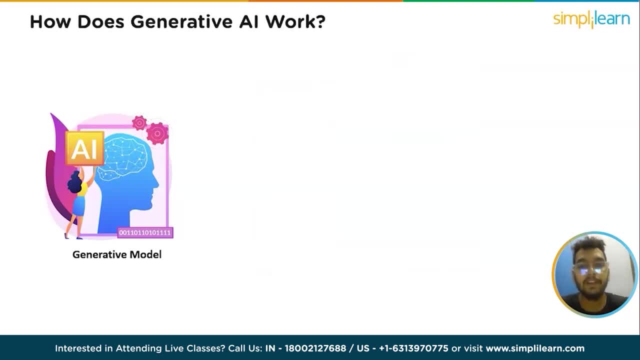 Now moving forward. let's see how does Generative AI work. Generative AI begins a prompt which can take the form of a video. It is a prompt which can take the form of text, image, video, design, audio, musical notes or any input that AI systems can process. 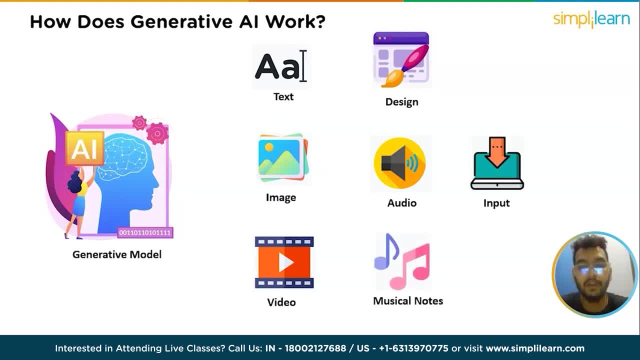 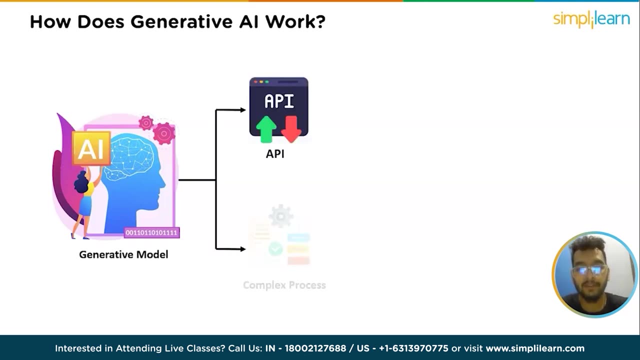 Various AI algorithms that generate new content in response to the given prompt. This content can range from essay and problem solution to realistic, created using images or audio of a person In the early stages of Generative AI utilizing the technology involved submitting data through an API or a complex process. 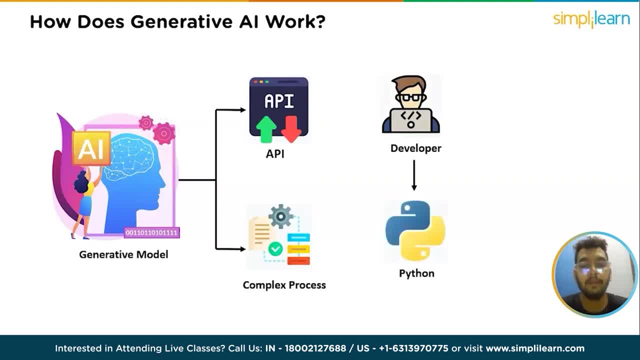 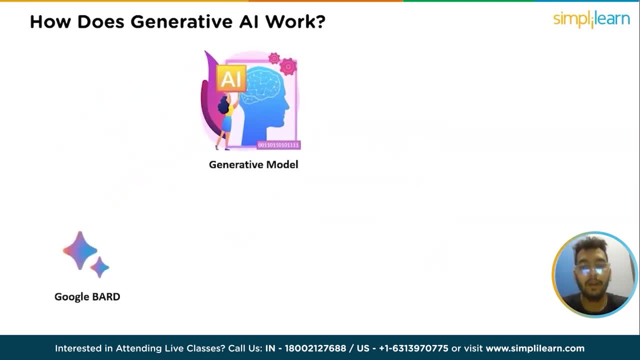 developers need to acquaint themselves with a specialized tool and writing application using programming language like Python. Some of the recent and fully operational Generative AIs are Googlebot, Dale, OpenAI, ChatGPT, Microsoft Bing and many more. So now let's discuss ChatGPT, Dale and BART, which are the most popular Generative AI interfaces. 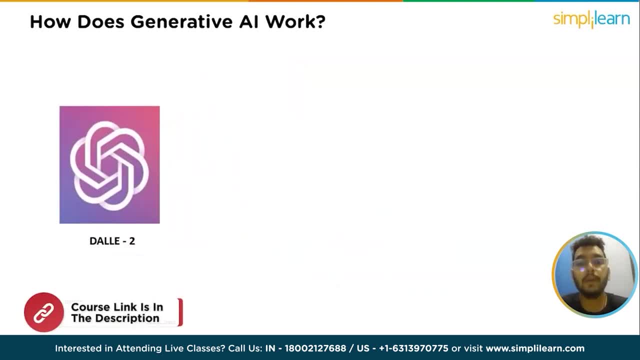 So first is Dale 2, which was developed using OpenAI, GPT implementation in 2021.. Exemplify: OpenAI is a multi-modal AI application. It has been trained on a vast dataset of images and their corresponding textual description. Dale is capable of establishing connection between various media forms, such as vision, text, audio. 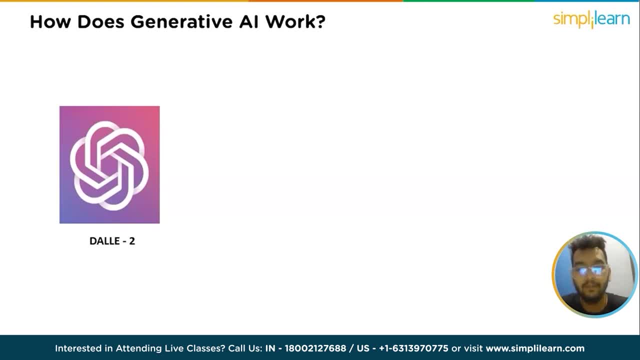 It specifically links the meaning of words to visual elements. OpenAI introduced an enhanced version called Dale 2 in 2022, which empowers users to generate imagery in multiple styles based on their prompts, And the next one is ChatGPT. In November 2022, ChatGPT, an AI-powered chatbot built on OpenAI GPT 3.5 implementation, gained immense popularity worldwide. 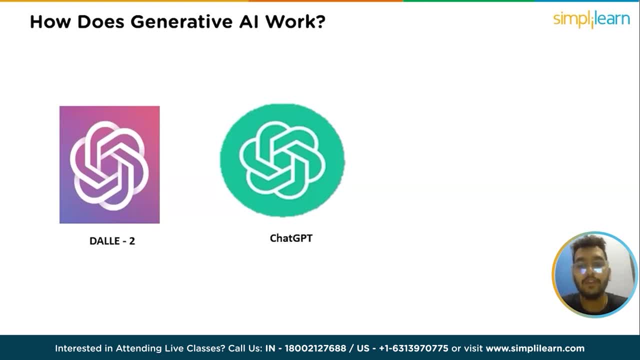 OpenAI enabled users to interact with and fine-tune the chatbot's text response through a chat interface with interactive feedback. Unlike earlier versions of GPT that were solely accessible via an API, ChatGPT brought a more interactive experience. On March 14, 2023, OpenAI released ChatGPT 4.. 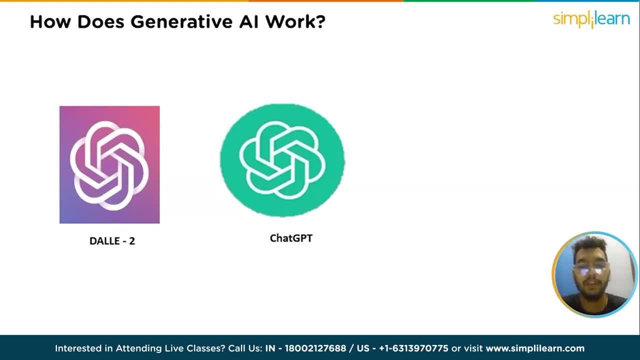 ChatGPT integrates the conversational history with the user, making a genuine dialogue. Microsoft, impressed by the success of the new ChatGPT interface, announced a substantial investment in OpenAI and integrated a version of GPT into its Bing search engine, And the next one is BARD. 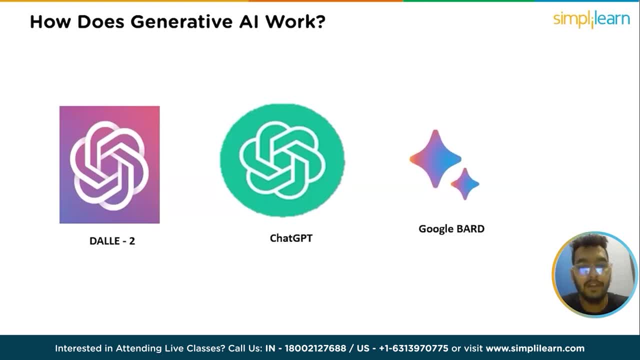 Google BARD. Google was also an earlier fortuner in advancing Transformer AI techniques for language processing, protein analysis and other content types. It made some of these models open-source for researchers but were not made available through a public interface. In response to Microsoft's integration of GPT into Bing, Google hurriedly launched a public-facing chatbot named Google BARD. 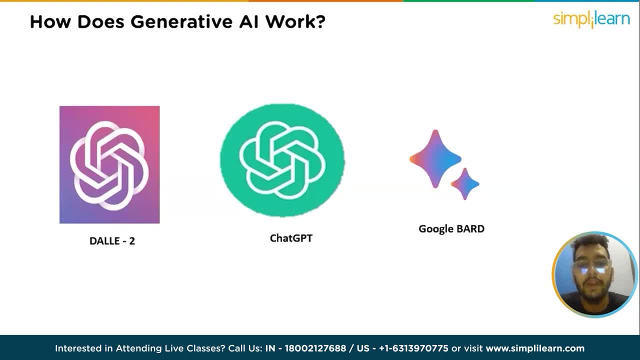 BARD's debut was met by an error, when the language model incorrectly claimed that the Webb Telescope was the first to discover a planet in a foreign solar system. As a consequence, Google's stock price suffered a significant decline. Meanwhile, Microsoft's implementation of ChatGPT and GPT 3.5 were also successful. 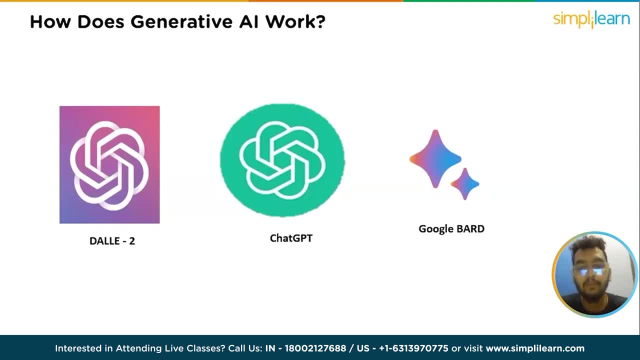 In addition, Google BARD and the BARD-GPT-powered system also faced criticism for producing inaccurate results and displaying erratic behavior in their early editions. So, moving forward, let's see what are the use cases of Generative AI. Generative AI has broad applicability and can be employed across a wide range of use cases to generate diverse forms of content. 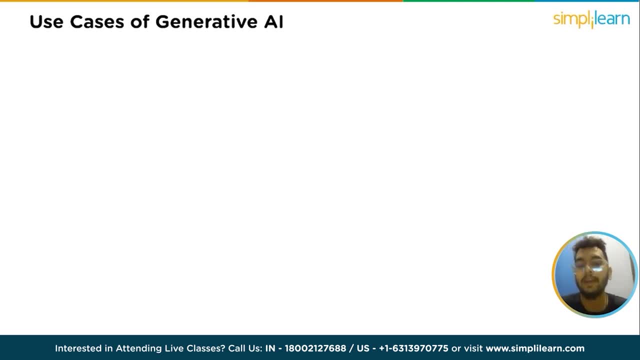 Recent advancements, like GPT, have made this technology more accessible and customizable for various applications. Some notable use cases for Generative AI are as follows: Chatbot Implementation. Generative AI can be utilized to develop chatbots for customer service and technical support, enhancing interaction with users and providing efficient assistance. 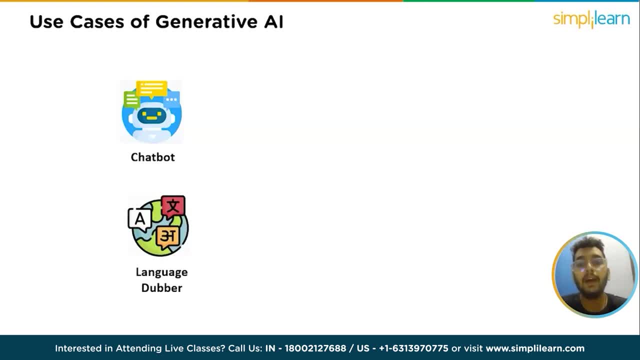 Language Dubbing: Enhancement In the realm of movies and educational content. Generative AI can contribute to improving dubbing in different languages, ensuring accurate and high-quality translation. Content Writing: Generative AI can assist in writing, email responses, dating profiles, results and more. 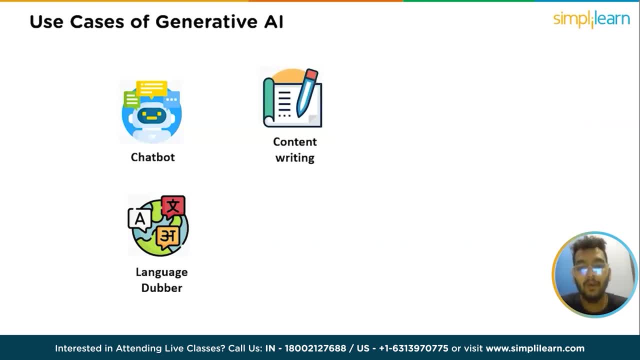 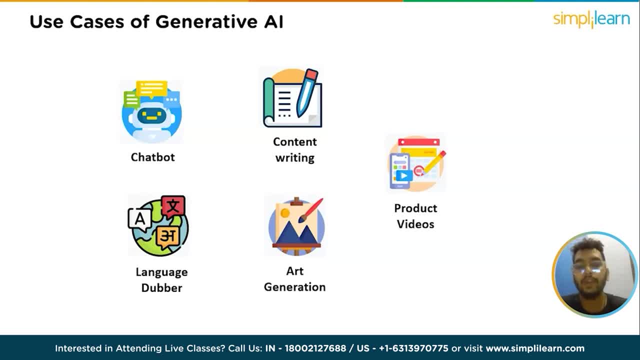 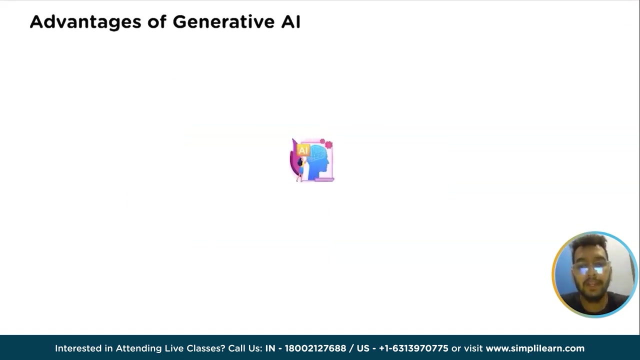 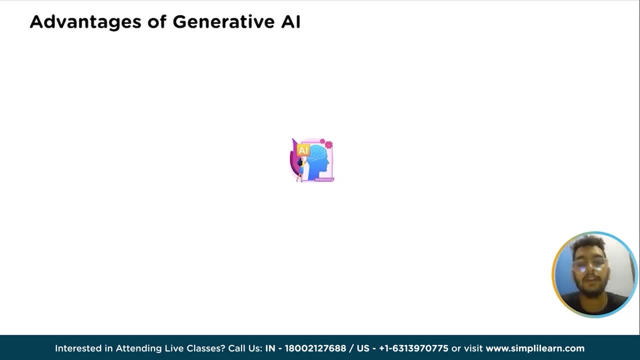 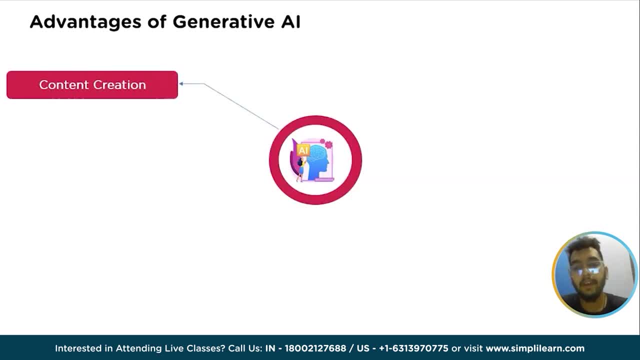 • Automated content creation. Generative AI can automate the manual process of writing content, saving time and effort by generating text or other form of content. 2. Efficient Email Responds. Responding to emails can be made more efficient with Generative AI, reducing the effort required and improving response. 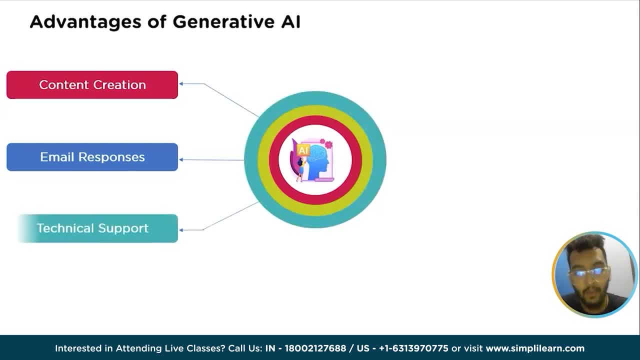 time. • Enhanced Technical Support. Generative AI can improve responses to specific technical queries, providing accurate and helpful information to users or customers. 4. Realistic Person Generation. By leveraging Generative AI, it becomes possible to create realistic representation of people and resources. 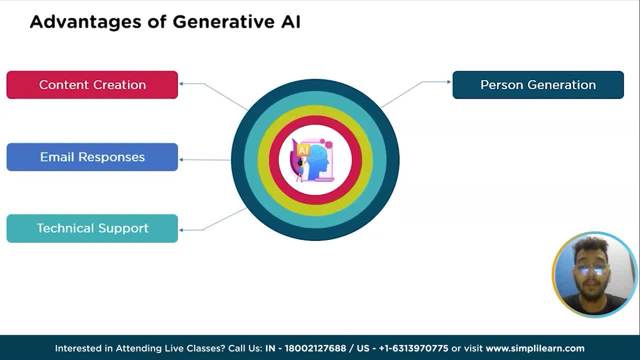 enabling applications like virtual characters or avatars. and the fifth one is coherent information summarization. Generative AI can summarize complex information into a coherent narrative, Distilling key points and making it easier to understand and communicate complex concept. The implementation of generative AI offers a range of potential benefits: streamingly process and announcing content creation in various areas of business. 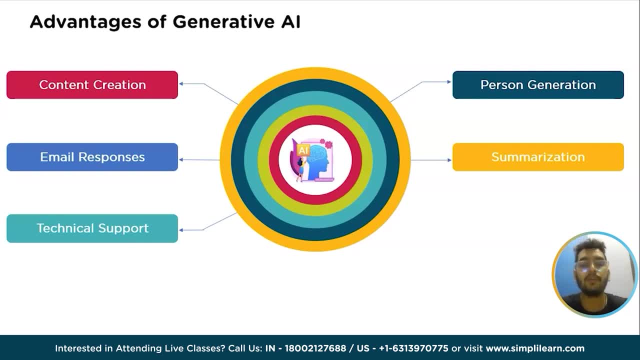 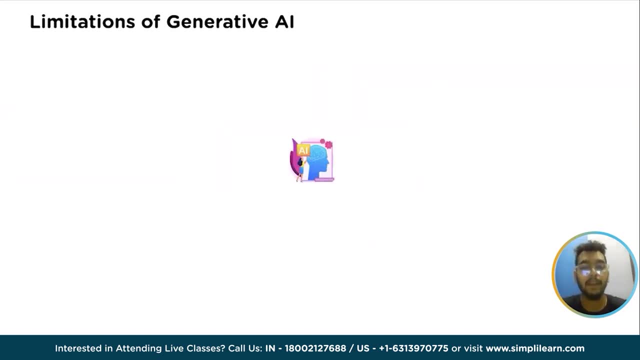 Operation. so, after seeing advantages of generative AI, let's move forward and see what are the limitations of generative AI. Early implementation of generative AI serve as vivid examples highlighting the numerous limitation associated with this technology. Several challenges arise from the specific approaches employed to implement various use case, for instance: 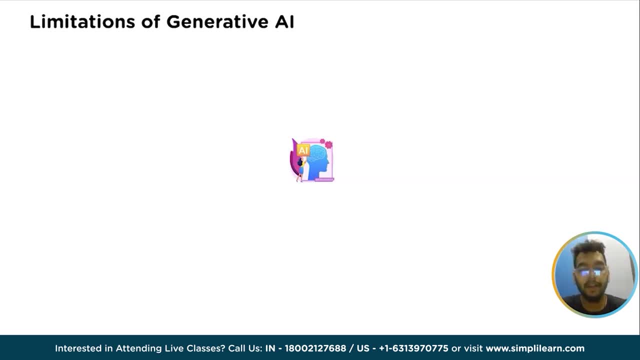 While a summary of a complex topic may more reader friendly than explanation incorporating multiple supporting sources, the ease of readability comes at the expense of 10 Transparent, identifying the information sources. So the first one is: when implementing or utilizing a generative AI application, It is important to consider the following limitation. I repeat: the first one is lack of source. 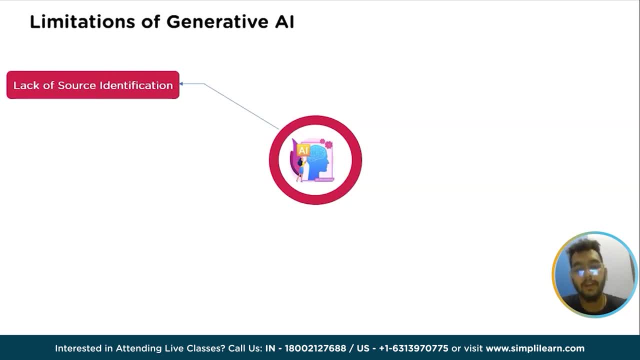 Identification: generative AI does not always provide clear identification of content source, Making it difficult to trace and verify origin of the information. The second one is assessment of bias. Assessing the bias of original sources used generative AI can be challenging, as it may be difficult to determine the underlying perspective or agendas of the data utilized in the training process. 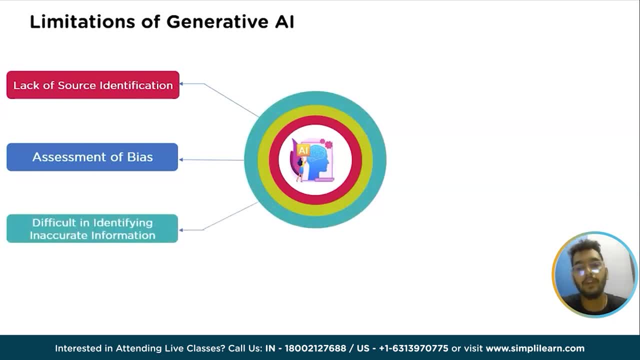 The third one is difficulty in identifying inaccurate information. Generative AI can generate realistic content, making identifying inaccuracy or falsehoods within the generated output harder. and the fourth one is adaptability to a new circumstances. Understanding how to fine-tune generative AI for a new circumstances or specific context can be complex. 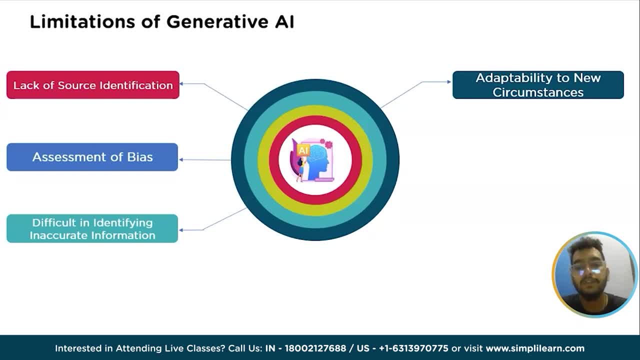 Requiring careful consideration and expertise to achieve desired result. and the fifth one is glossing over bias, Prejudice and hatred. generative AI research may amplify or Preparatory biases, prejudices or hateful content present in the training data. Require vigilant scrutiny to prevent such issues. 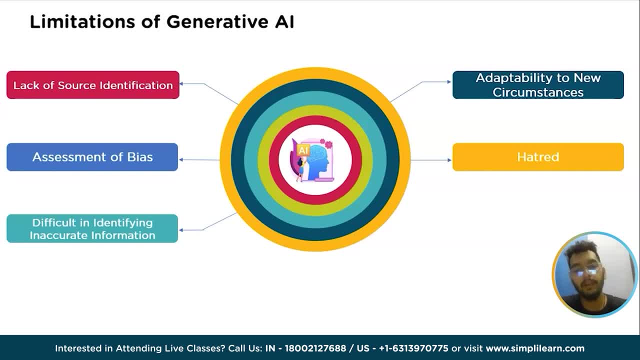 So awareness of these limitation is crucial when implementing of utilizing generative AI, as it helps users and developers critically evaluate and mitigate the risk of bias and hatred in the training process. It also helps to mitigate potential risks and challenges associated with the technology. So future of generative AI. furthermore, advances in AI development platforms will contribute to the accelerated progress of research and development in the realm of. 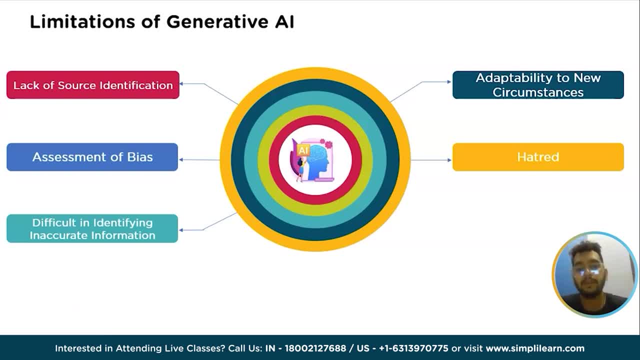 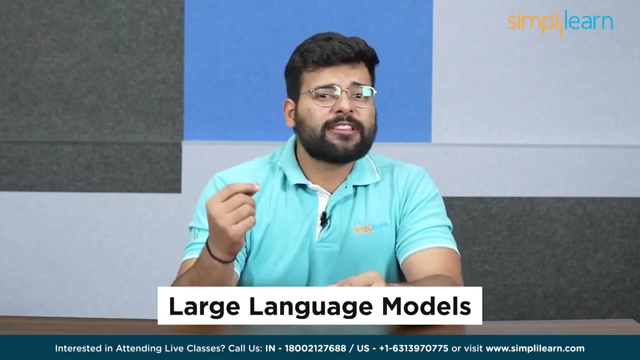 Generative AI. the development will encompass various domains such as text, images, videos, 3d contact, drugs, supply chains, Logistic and business processes. while the current standalone tools are impressive, the true transformative impact generative AI will realize while these capabilities are seemingly integrated into the existing Tools with regular use. hello everyone and welcome to the video on large language models. large language models are basically very advanced. 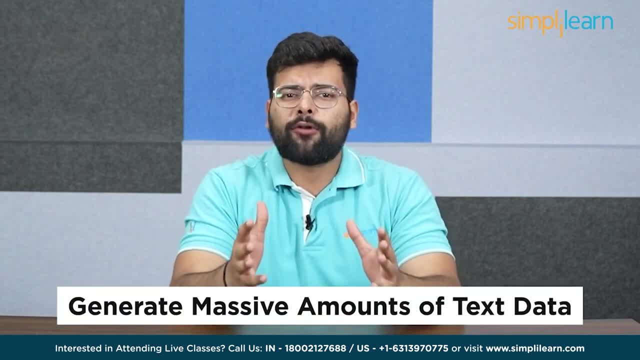 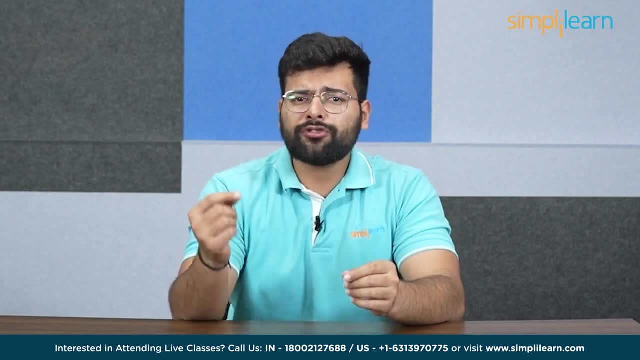 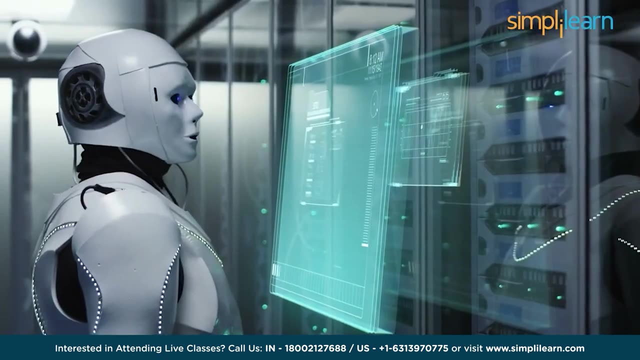 Artificial intelligence systems that can process and generate massive amounts of text data. They are designed to learn from and understand natural human language and can be used to perform a wide range of language related tasks, such as translation, speech recognition and automatic summary generation. one of the key advantages of large language models is their ability to learn from vast amounts of data, which allows them to 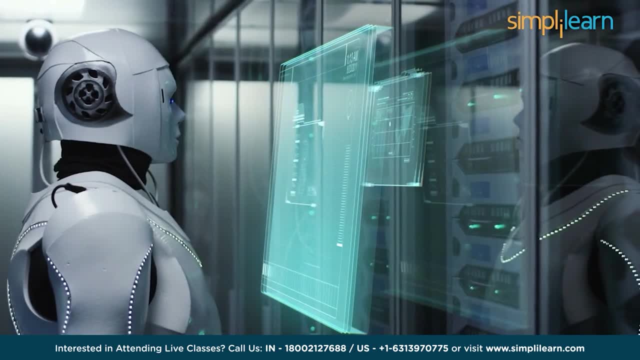 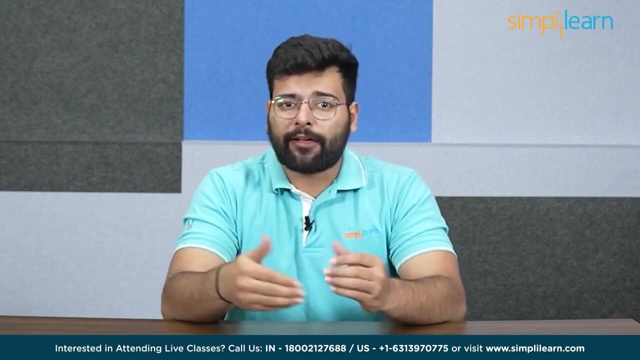 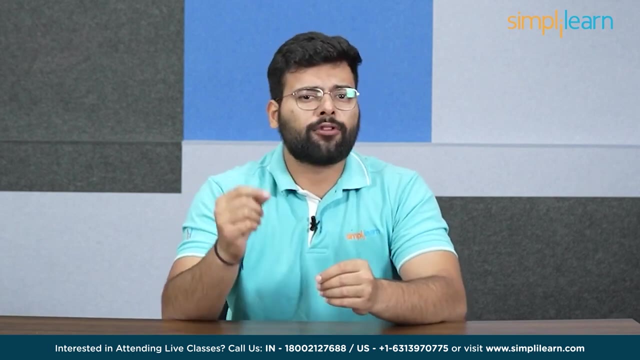 Generate highly accurate and realistic responses to complex natural language prompts. Additionally, they can be trained on multiple languages simultaneously, Which means they can be used to perform language translation between different pairs of languages, making them an invaluable tool for businesses and Organizations that work with people from diverse cultural backgrounds, not just language related tasks. 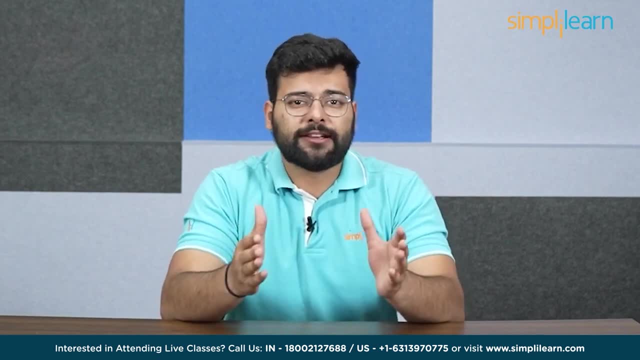 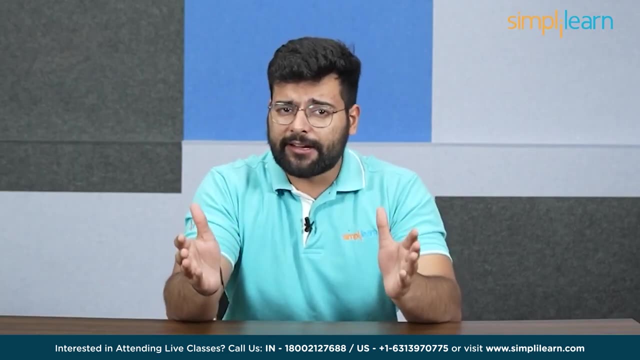 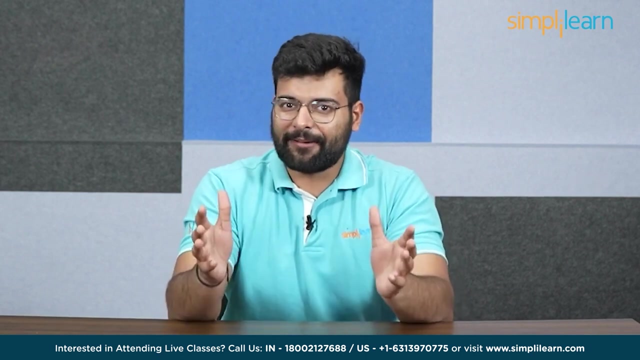 But LLMs can also have the potential to revolutionize fields such as research, science and healthcare. by allowing researchers to quickly analyze And process vast amounts of complex text data, They can accelerate progress in areas such as drug discovery, healthcare diagnostics and AI development. That being said, large language models also present some challenges, for instance, 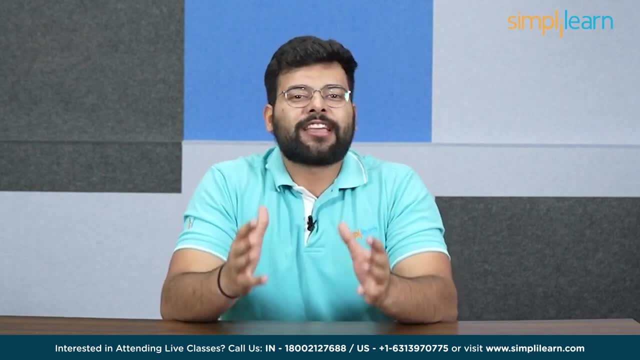 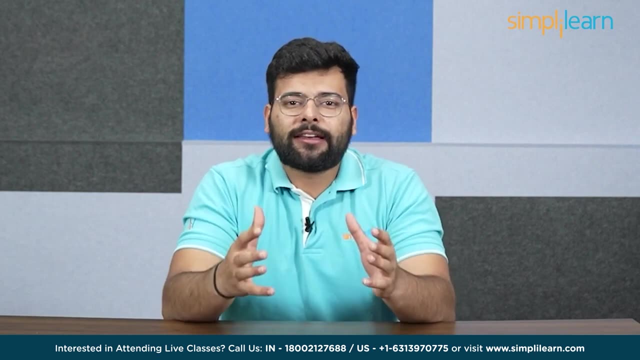 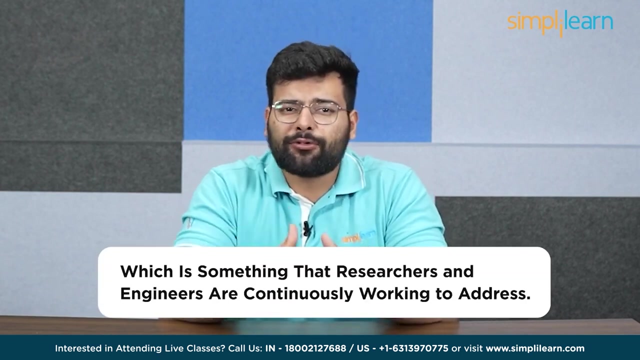 They require a significant amount of compute resources, which can be prohibitively expensive for some organizations. Additionally, because they are trained on huge amounts of data, They may inadvertently reinforce biased or discriminatory patterns in language use, which is something that researchers and engineers Are continuously working to address. 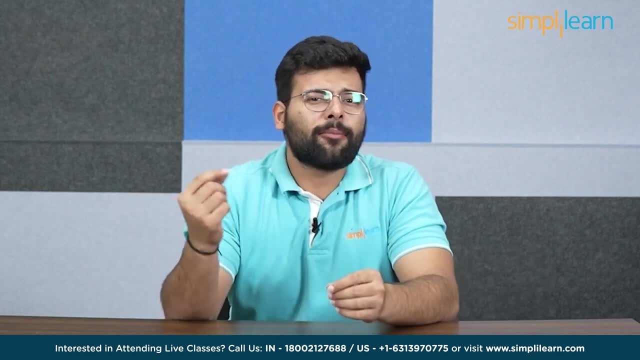 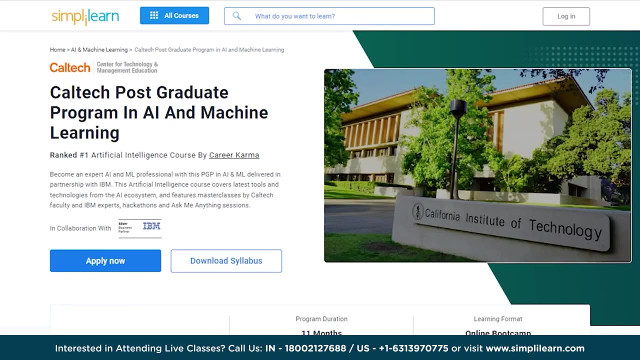 overall, large language models are an exciting and rapidly developing field with tremendous potential to transform the way we live, work and communicate. So if you want to embark on a journey of AI and ML, then try giving a short tour post graduate program in AI and ML That is in partnership with IBM. 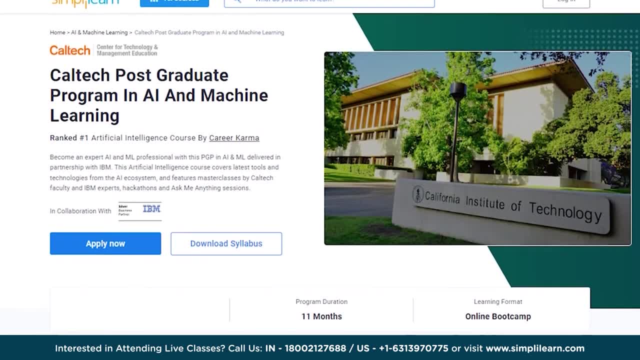 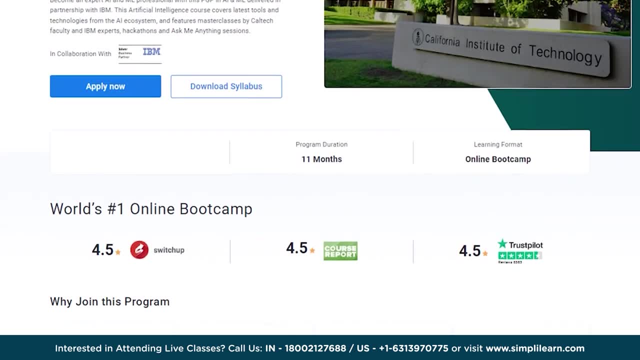 This artificial intelligence course covers the latest tools and technologies from the AI ecosystem and features master classes by Caltech faculty and IBM Experts, hackathons and- ask me anything- sessions. this program Showcases Caltech CTM is excellence and IBM's industry progress. the artificial intelligence course. 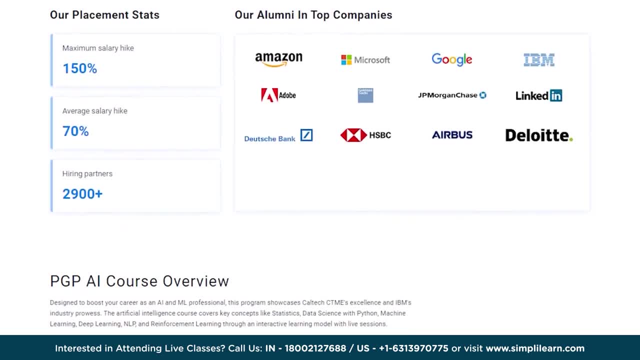 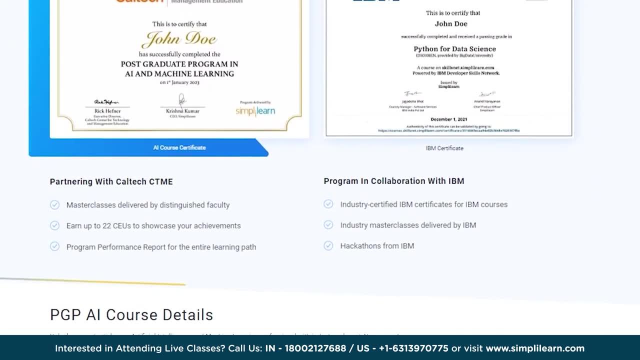 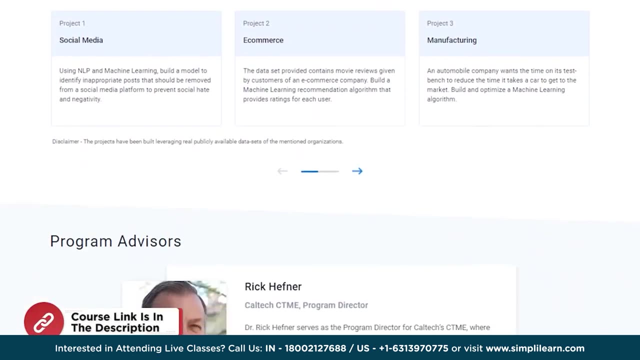 Covers key concepts like statistics, data sense with Python, machine learning, deep learning, NLP and reinforcement learning Through an interactive learning model with live sessions and roll now and unlock exciting AI and ML opportunities. The link is mentioned in the description box below and, with that having said, hey, everyone welcome to simply learns YouTube channel. 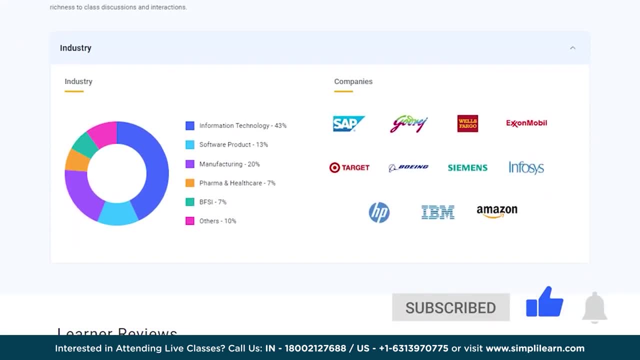 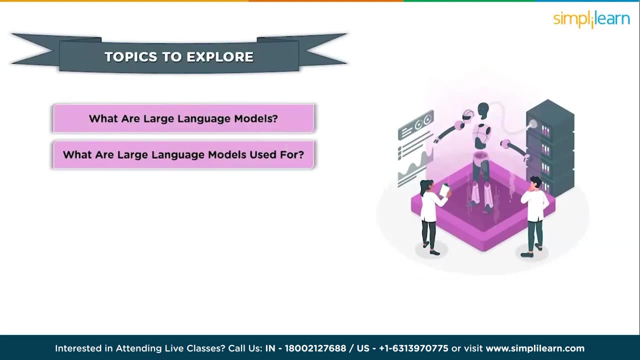 But before we dive into that, don't forget to Like, subscribe and share. In this video we will cover topics like what are large language models? after that We'll look at what large language models used for, and after that We'll cover how our large language models trained. after this: 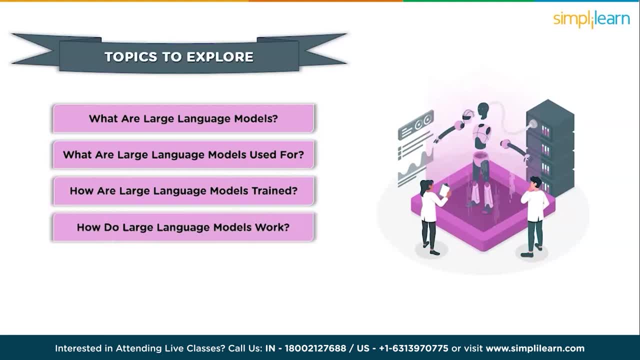 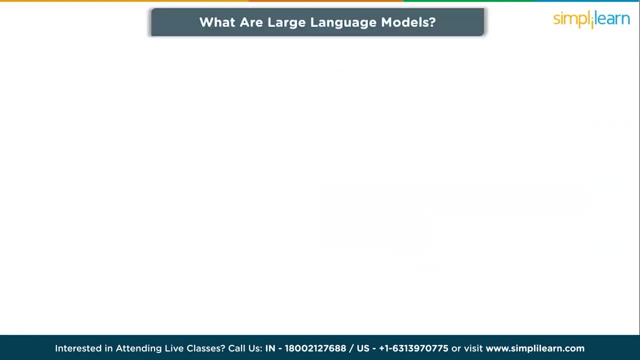 We'll look at how do large language models work and at the last we'll see some applications of large language models. So, without any further ado, let's get started. So we'll start with. what are the large language models? large language models such as GPT-3. 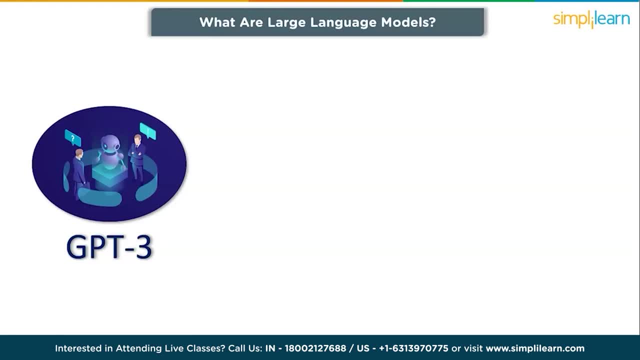 generative, pre-trained transformer-3, Advanced artificial intelligence systems designed to understand and generate human-like text. These models are built using deep learning techniques and have been trained on vast amounts of text data from the Internet. These models use self-attention mechanisms to analyze the relationships between words or tokens in a text. 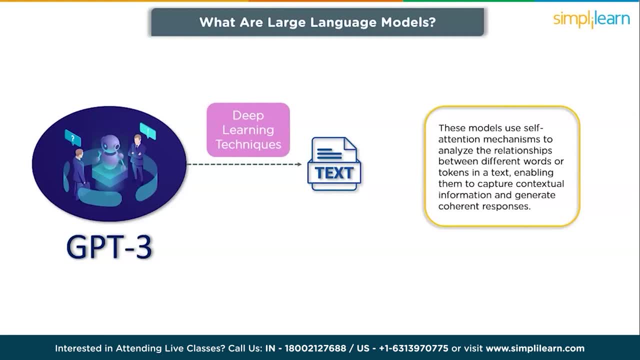 enabling them to capture contextual information and Generate core and responses. these models use self-attention mechanisms To analyze the relationship between different words or tokens in the text, enabling them to capture contextual information and generate core and responses. These models have significant implications for a wide range of applications. 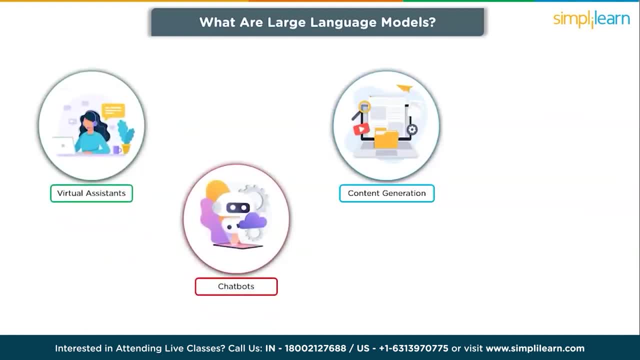 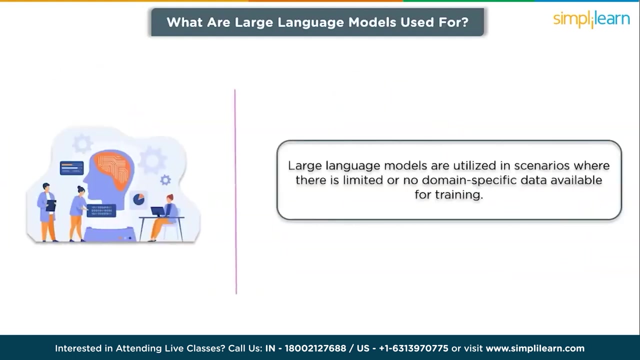 including virtual assistants, shared boards, content generation, Language translation and aiding in research and decision making processes. their ability to generate coherent and contextually appropriate text has led to advancement in natural language understanding and human-computer interaction. Now we'll see what our language models used for. So large language models are utilized in scenarios where there is limited or no domain specific data available for training. 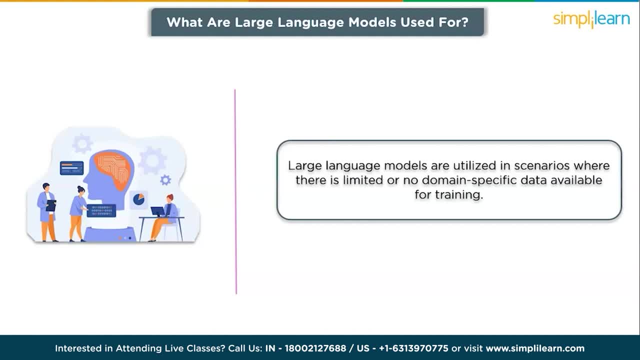 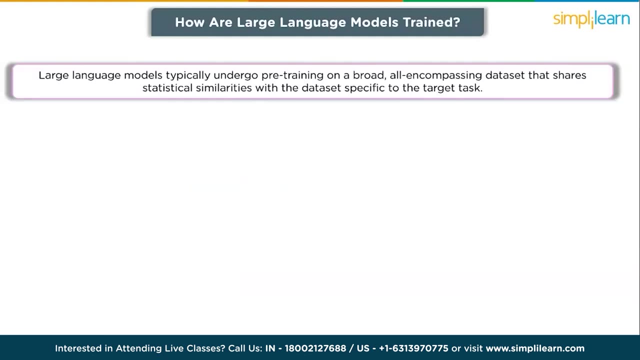 These scenarios include both few short and zero short learning approaches, Which rely on the models, strong inductive bias and its capability to derive meaningful representations from a small amount of data, or even no data at all. Now we'll see how our large language models trained. Large language models typically undergo pre-training on a broad, all-encompassing. 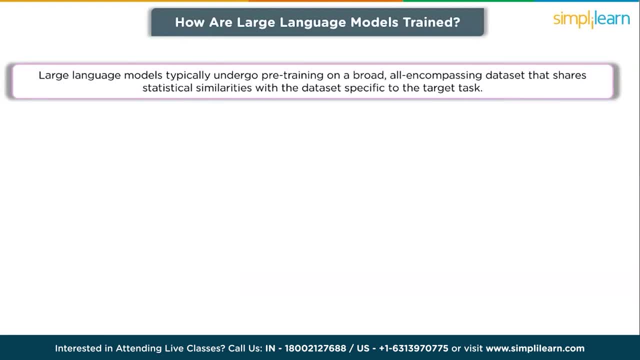 Dataset that shares statistical similarities with the data set specific to the target task. The objective of pre-training is to enable the model to acquire high-level features that can later be applied during the fine-tuning phase for specific tasks, and the training process of a large language model involves several steps. 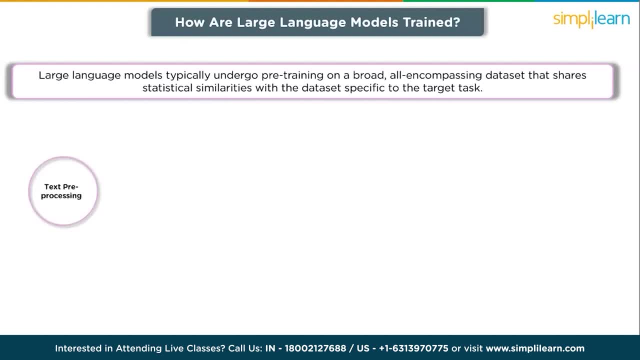 The first is text pre-processing. the textual data is transformed into a numerical representation that can be effectively processed By the model. this conversion may involve techniques like tokenization and coding and creating input sequences. The next we have is random parameter initialization. The models parameters are initialized randomly before the training process begins. 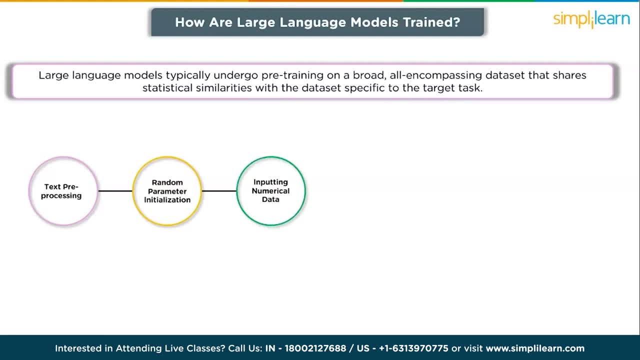 The next is inputting numerical data. The numerical representation of text data is fed into the model for processing the models architecture, typically based on transformers, Allows it to capture the contextual relationships between the words And tokens in the text. and the next is loss function calculation. a loss function is employed to measure the 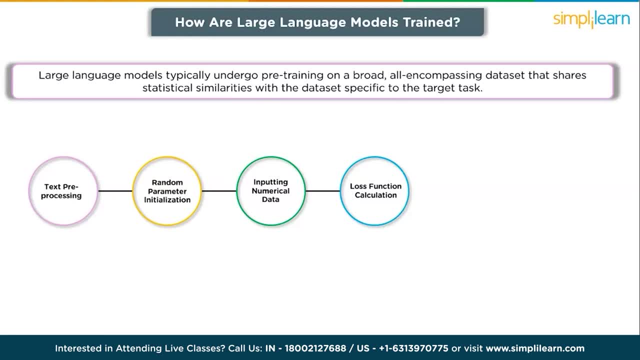 discrepancy between the model's predictions and the actual next word or token in a sentence. The model aims to minimize this loss during training, and the next is parameter optimization. The models parameters are adjusted through optimization techniques, such as gradient descent, to reduce the loss. This involves calculating gradients and updating the parameters accordingly, gradually improving the model's performance. 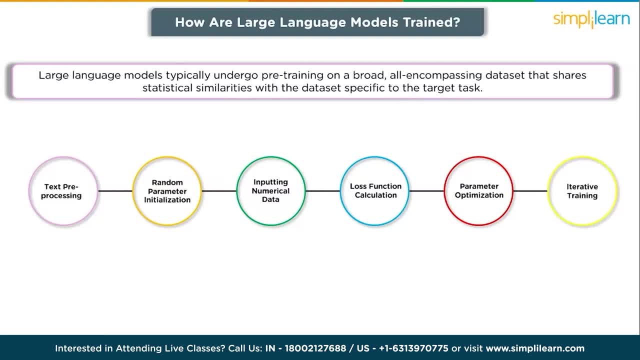 And the next is iterative training. The training process is repeated over multiple iterations or epochs until the model's outputs achieve a satisfactory level of accuracy on the given task or data set. By following this training process, large language models learn to capture linguistic patterns, understand context and generate coherent responses, enabling them to excel at a wide range of language related tasks. 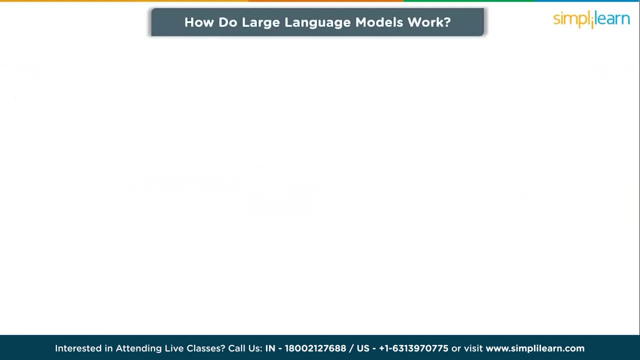 And now we will see. how do large language models work? So large language models Leverage deep neural networks to generate outputs based on patterns learned from the training data. typically, a large language model adopts a transformer architecture Which enables the model to identify relationships between both in a sentence. 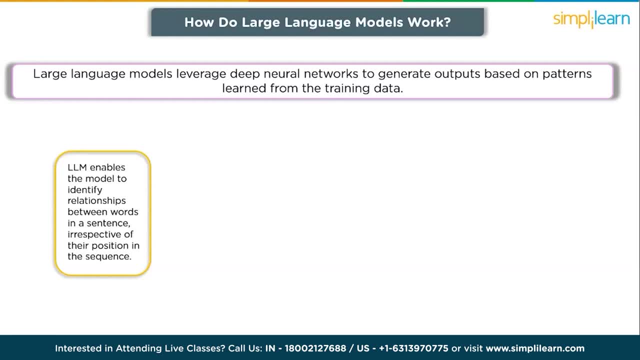 Irrespective of the position in the sequence. in contrast to recurrent neural networks- that is our enhance- that rely on requirements to capture token relationships, Transformer neural networks employee self-attention as their primary mechanism, self-attentionhhhhhh attention scores- that determines the importance of each token with respect to. 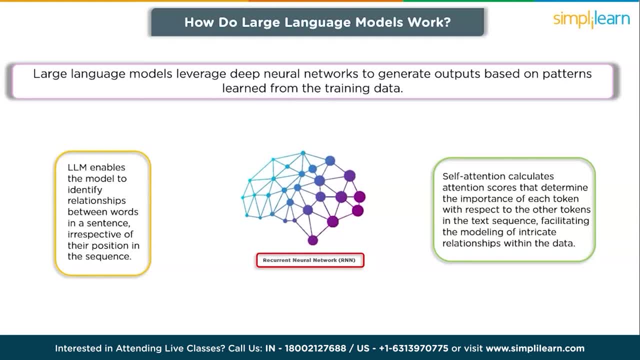 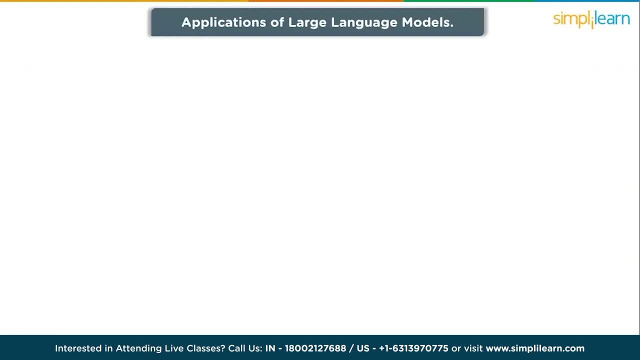 other tokens in the text sequence, facilitating the modeling of intricate relationships within the data. now we'll see applications of large language models. large language models have wide range of applications across various domains. here are some notable applications. the first one is natural language processing. large language models are used to improve natural 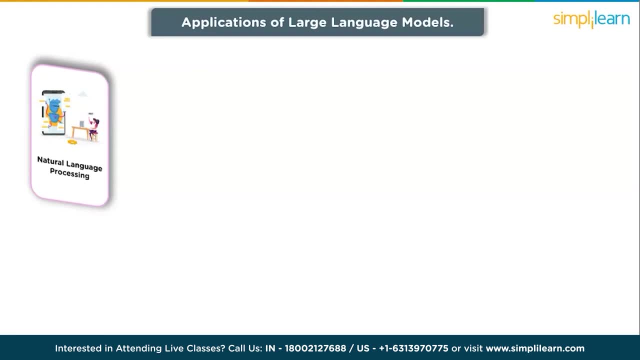 language understanding tasks such as sentiment analysis, named entity recognition, text classification and language modeling. the next is chat boards and virtual assistants: large language models. power conversational agents, chat boards and virtual assistants providing more interactive and human-like interactions with users. and the next is machine translation- large language. 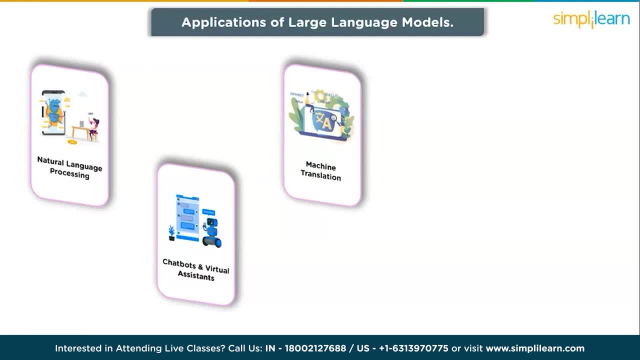 models have been used for automatic language translation, enabling the translation of text between different languages with improved accuracy. and the next we have is sentiment analysis. large language models can analyze and classify the sentiment or emotion expressed in a piece of text, which is valuable for market research, brand monitoring and social media. 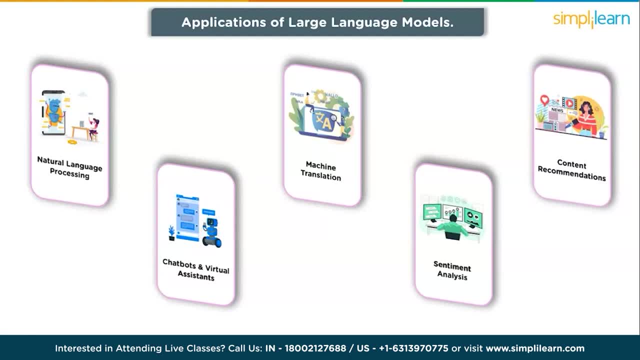 analysis, and the next we have is content recommendation. these models can be employed to provide personalized content recommendations, enhancing user experience and engagement on platforms such as news websites or streaming services. these applications highlight the versatility and potential impact of large language models in various domains: improving language understanding, automation and interaction between humans and computers. everyone. 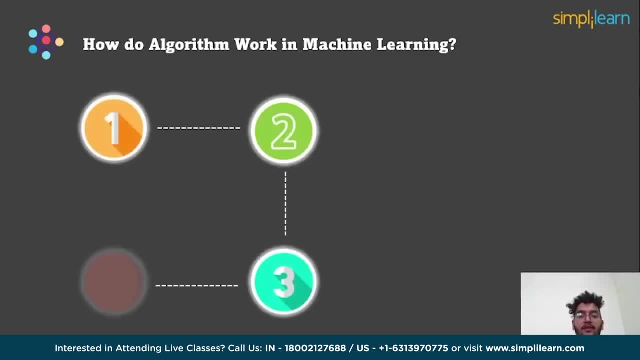 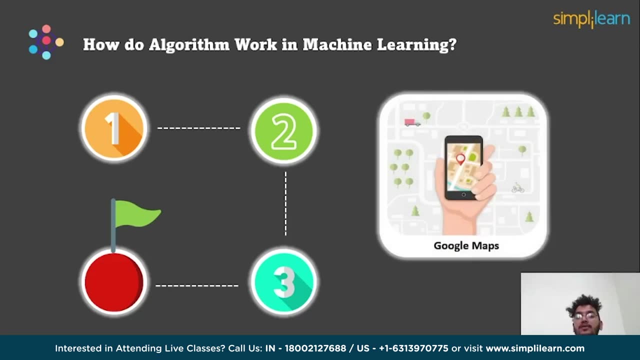 knows, the algorithm is a step by step process to approach a particular problem. there are numerous examples of algorithm, from figuring out sets of number to finding roots, through maps, to showing data on a screen. let's understand this is by using an example. every algorithm is built on inputs and outputs. Google search analysis by Google Search audio website如 stalker. 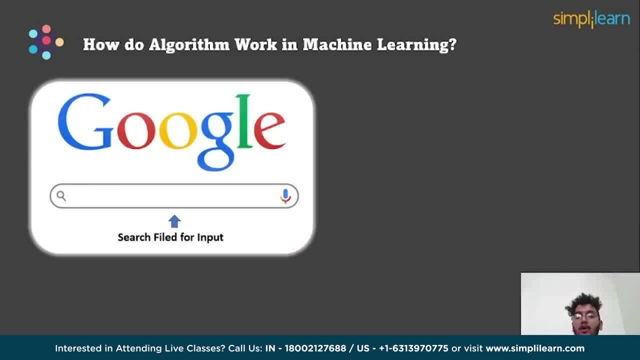 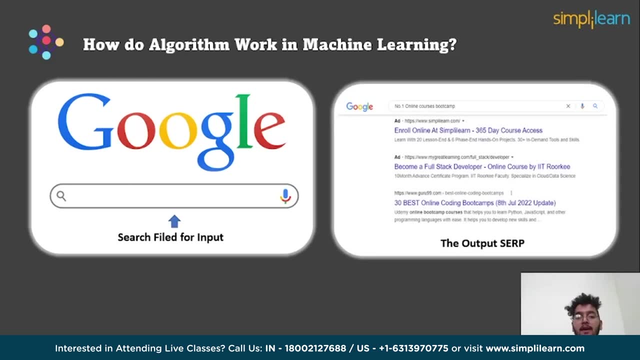 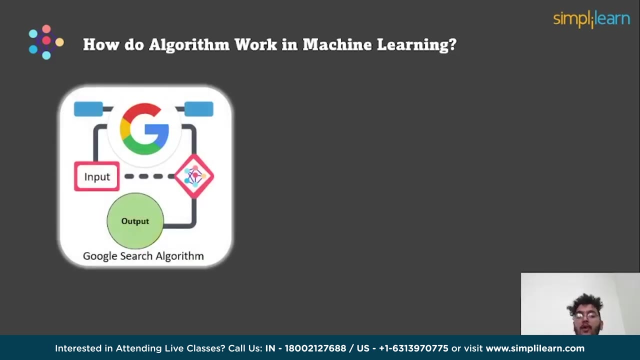 algorithm is no different. The input is the search field and the output is the page of result that appears when you enter a particular phrase or keyword, also known as SERP or Search Engine Result Page. Google has a search algorithm so it can sort results from various websites. 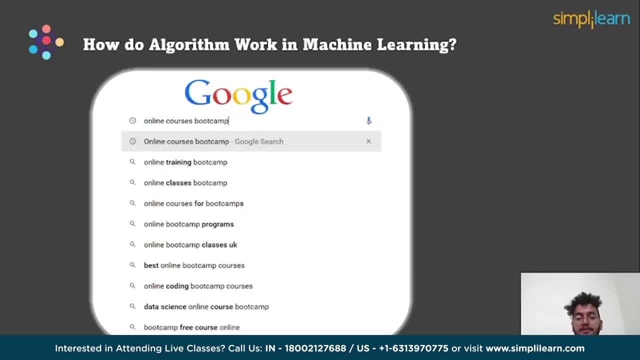 and provides the users the best results. When you start a search, you will see the search box will attempt to guess what you are looking for. In order to better understand what the user is looking for, the algorithm is trying to gather as many as suggestions from them. 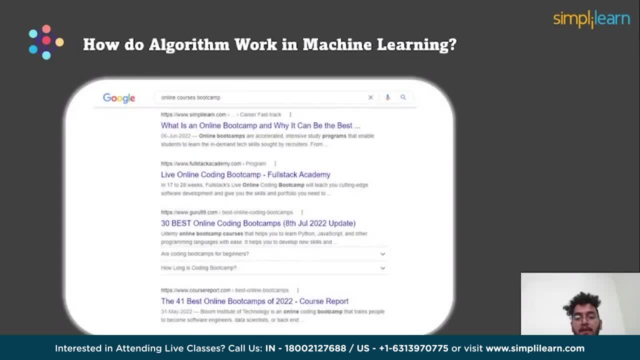 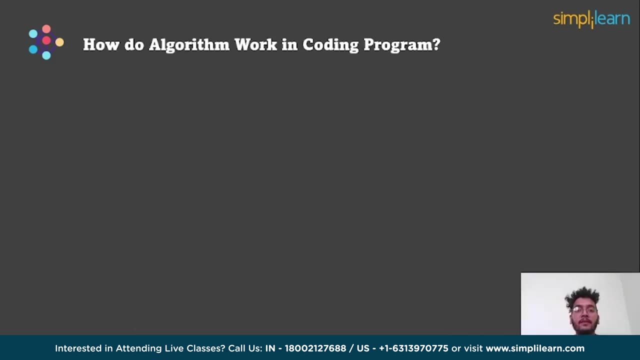 as possible. The results from the search field that best matches the query will be ranked. The choose 5th website will rank, and in what position, using more than 200 ranking variables. Now let's take an example of coding program and see how the algorithm works. Here we will. 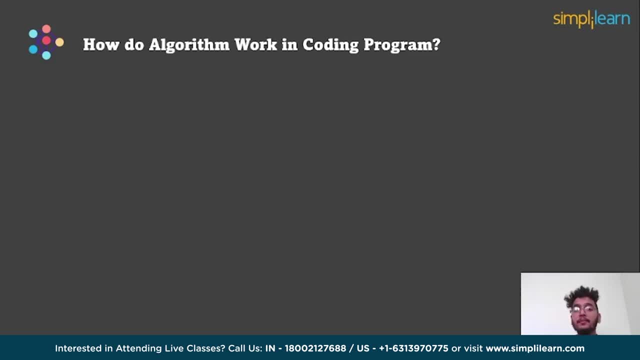 use a case of computer program wherein we want to print the multiplication table of any number. Let's take 2.. The algorithm starts here and then it assigns a value to a variable. The variable i is having an initial value of 1. The system will read the number, The number. 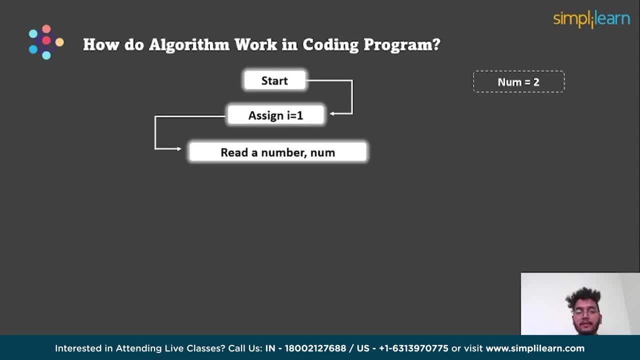 in case is 2.. Now the system has a condition. A condition can now either be true or false. If the value of i reaches 11,, then the loop will end. Otherwise, value of i will multiply by the number. The initial value of i is 1.. 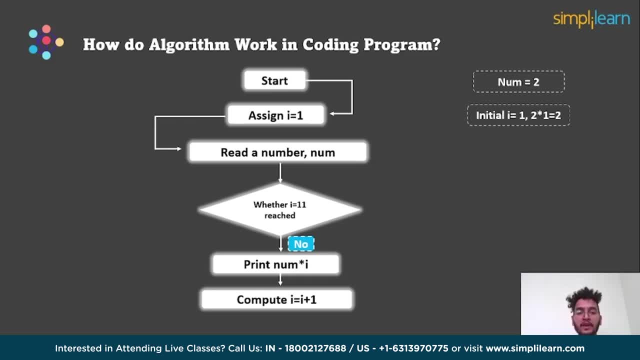 So for the first time the system output will be 2.. Now value of i will be increased by 1. According to the loop condition. the system will then move back and check for the condition again. The new value of i is 2,, which is still less than 11.. The system will 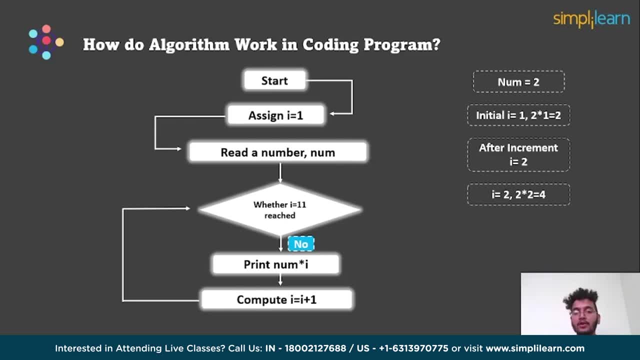 again print 2 into i, which is 2 into 2 on the screen. The new output result will be 4.. The system will keep following the same procedure repeatedly until the value of i becomes 11.. Once the value of i becomes 11,, then only the algorithm will terminate. 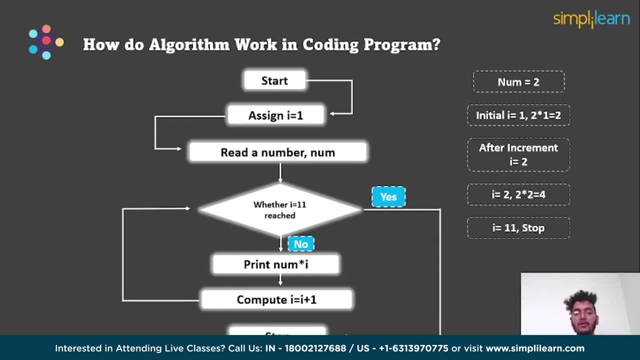 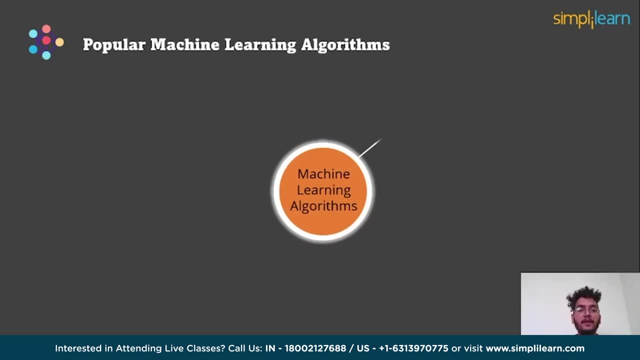 After discussing how an algorithm works, let's move forward and see some popular machine learning algorithms. Some popular machine learning algorithms are: Linear Regression Algorithm, Logistic Regression, Algorithm, Decision Tree, Support Factor Machine Algorithm, SV Algorithm. And the fifth one is KNN- K-Nearest Neighbor Algorithm. 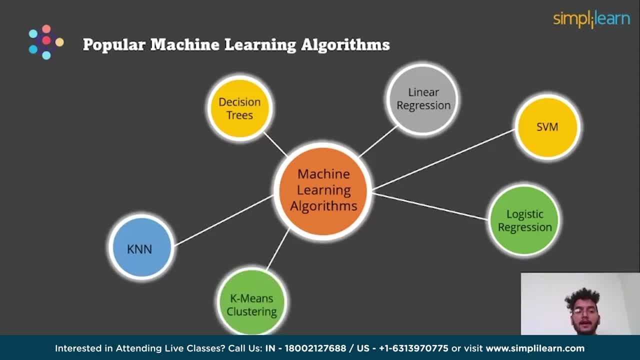 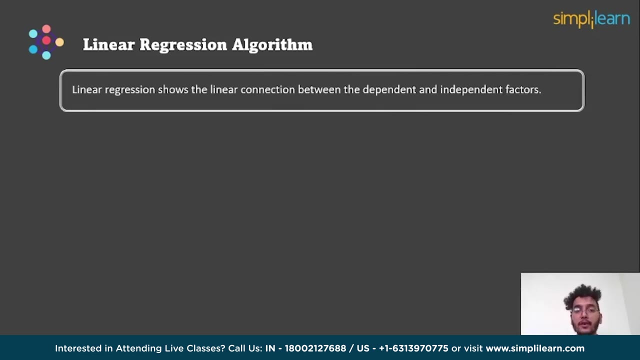 The sixth one is K-Means Clustering Algorithm, And the seventh one is Random Forest Algorithm. And the last but not the least algorithm is Apriori Algorithm. Let's go through them in detail, one by one. Linear Regression is one of the most famous. 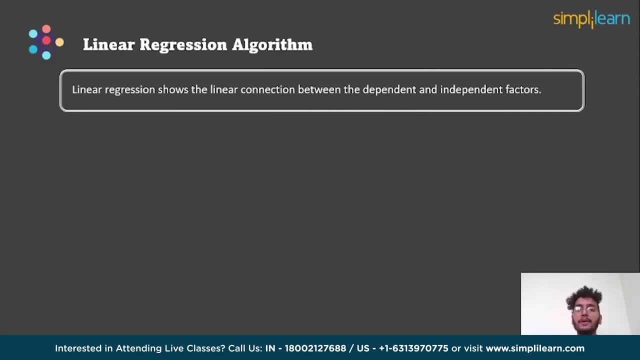 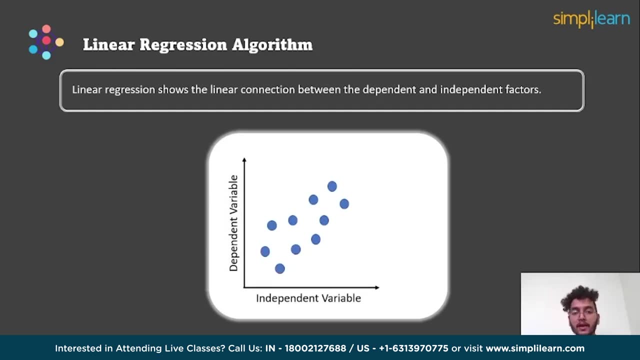 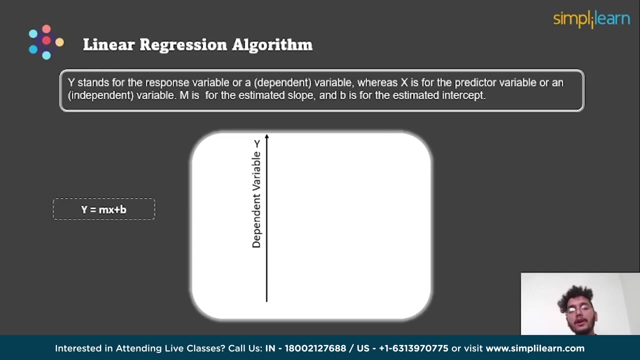 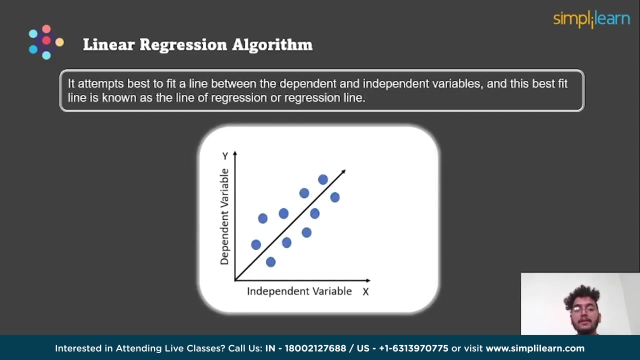 and straightforward machine learning algorithms utilized for predictive analysis. Linear Regression shows the linear connection between the dependent and the independent factors. The equation of line is: y equals to mx plus b. Here y stands for the response variable or a dependent variable, whereas x is for the predator variable or an independent variable. It attempts best. 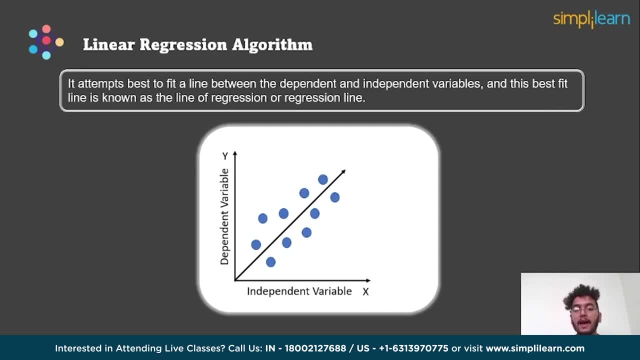 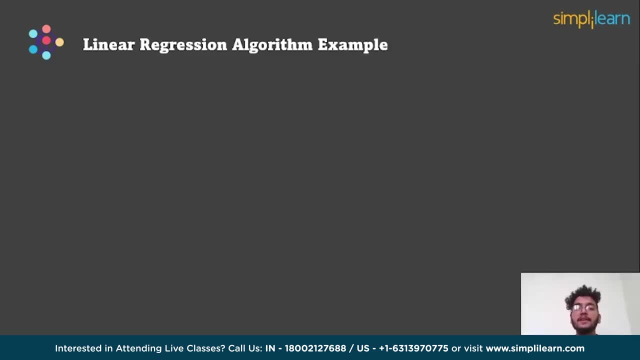 to fit line between dependent and independent variables, And this best-fit line is known as line of regression or regression line. Let's take a real example of Linear Regression. Let's start with Linear Regression. This is the line of regression. Let's take a real 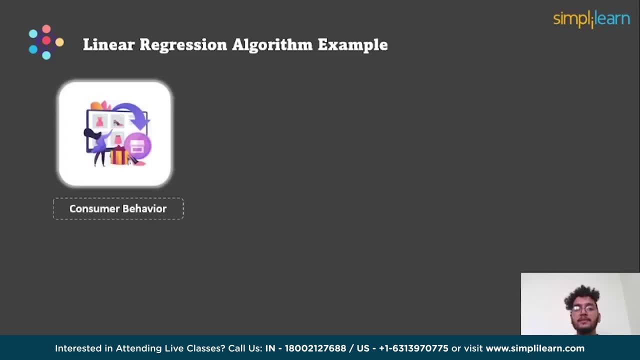 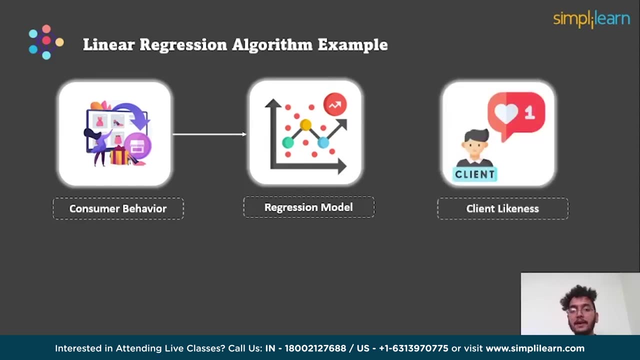 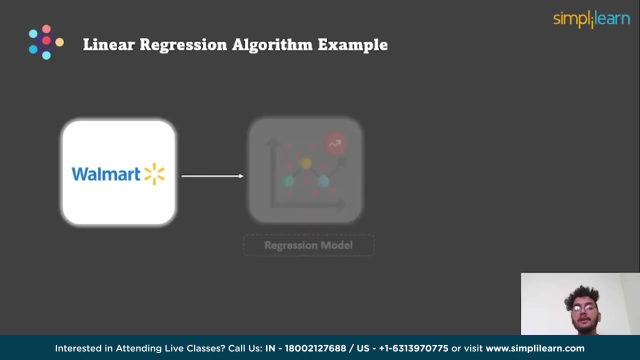 The real application example. in predicting consumer behavior, businesses use linear regression to forecast things like how much a client is likely to spend. Things like targeted marketing and product development may benefit from this. Walmart, for instance, used linear regression to forecast which goods would be in high demand. 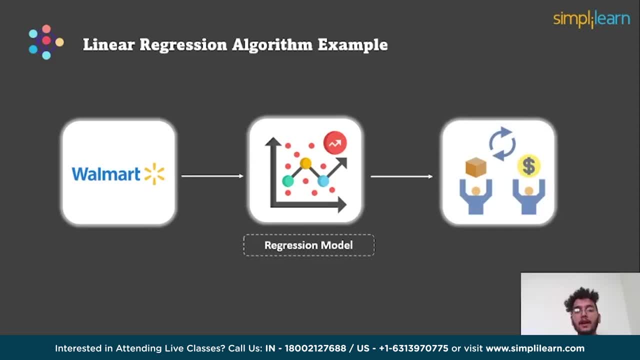 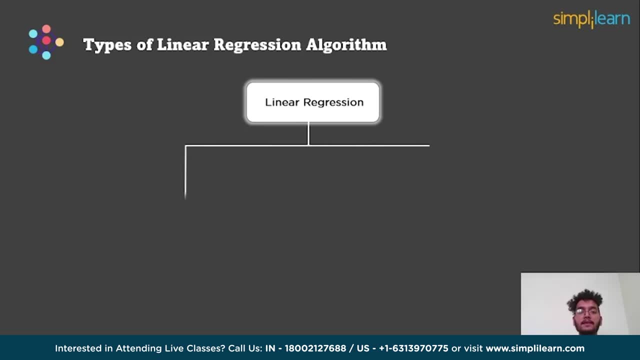 across the nation. Moving forward, let's see types of linear regression. There are two types of linear regression algorithm. The first one is simple linear regression and the second one is multiple linear regression. In simple linear regression, if an independent variable is utilized to forecast the worth. 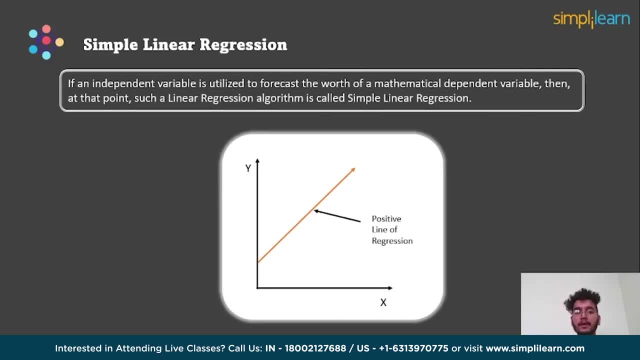 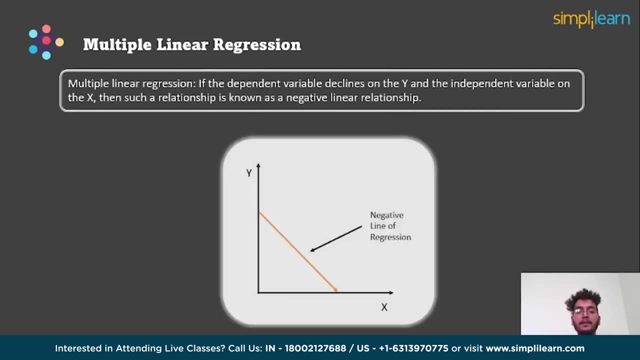 of a mathematical dependent variable, then at that point such a linear regression algorithm is called simple linear regression. The equation of line will be: y equals to a0 plus a1x. If the dependent variables are declined on the y and the independent variables on x. 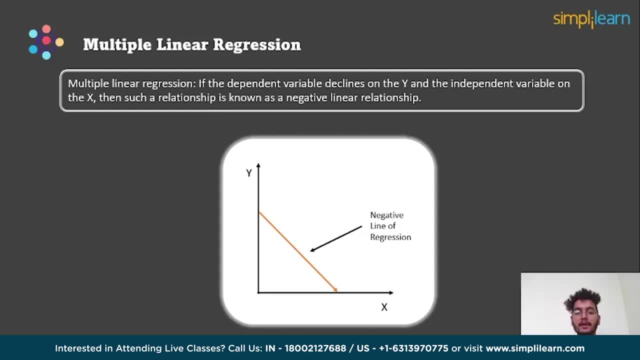 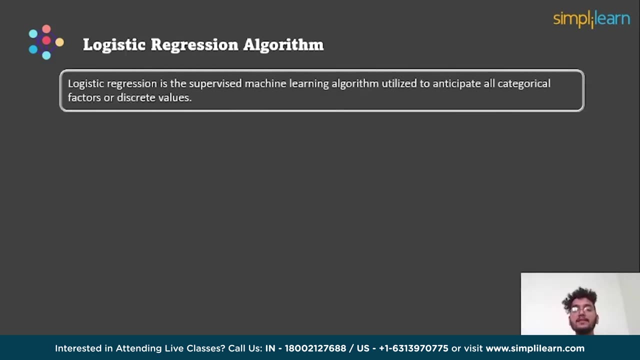 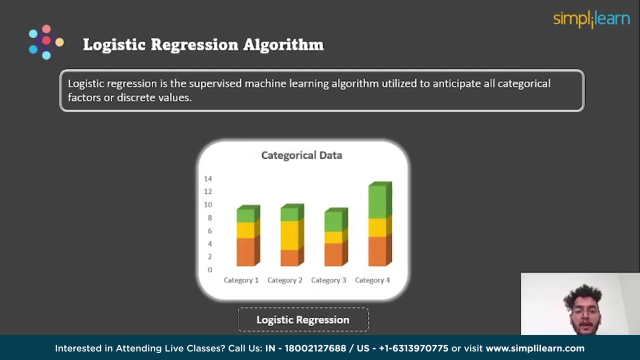 then such a relationship is called negative linear regression. The line of equation will be: minus of a0 plus a1x. Moving forward, let's see Logistic linear regression. Logistic regression is the supervised machine learning algorithm utilized to anticipate all the categories, factors or discrete values. It could be very well used for the grouping issues in machine. 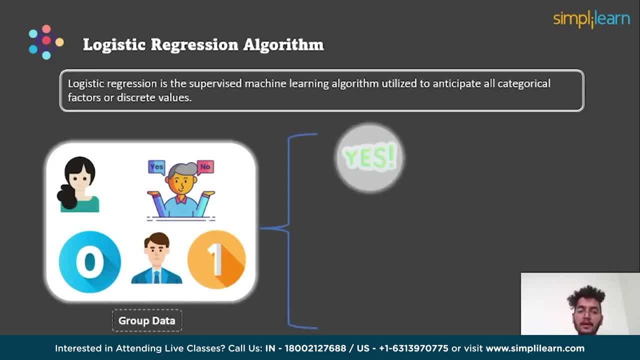 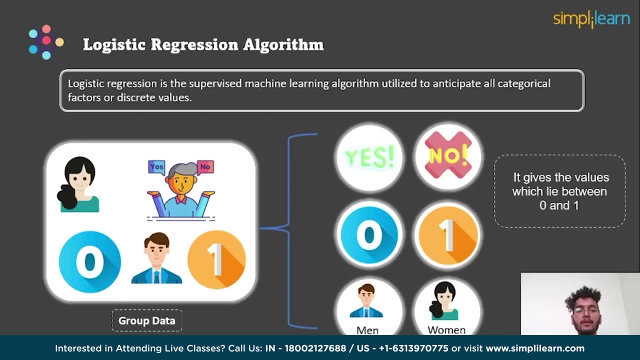 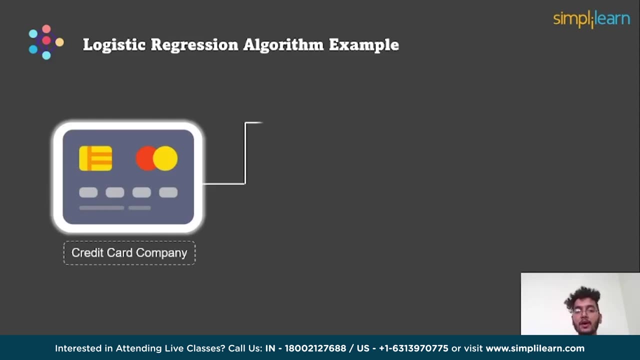 learning And the result of the logistic regression can be either yes or no, 0 or 1, men or women, and so on. It gives the values which lies between 0 and 1.. For example, a credit card business is interested in knowing whether the transaction amount and the credit scope 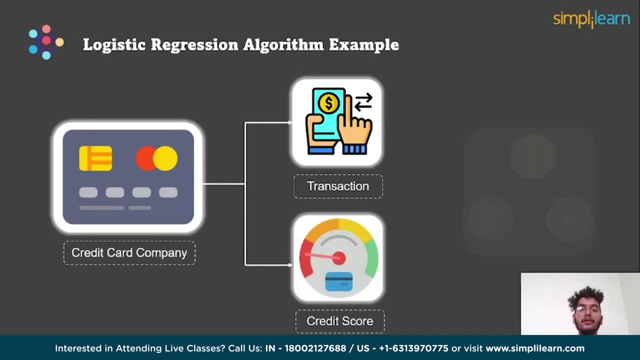 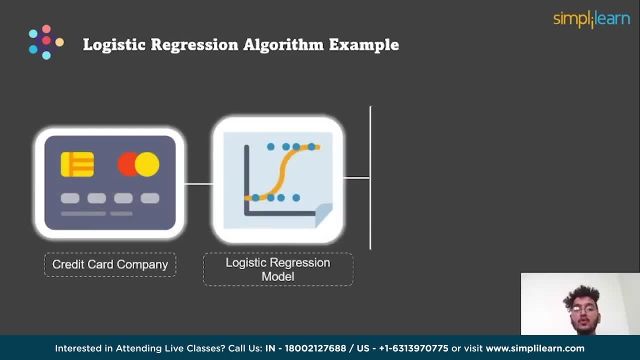 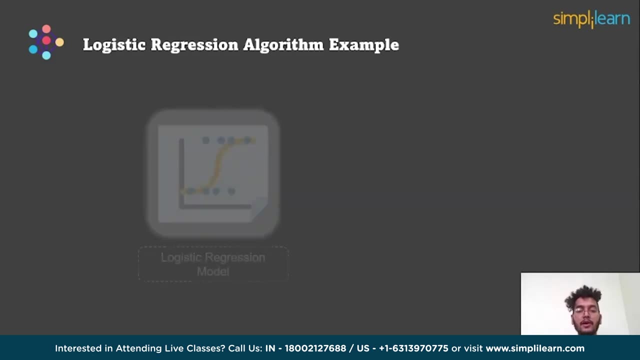 have an impact on the probability that a particular transaction would be fraudulent. The business can use logistic regression to determine how these 2 creditor values can relate the probability that our transaction is fraudulent. The response variable in the model has two possible outcomes. First one is the transaction is fraudulent and the second 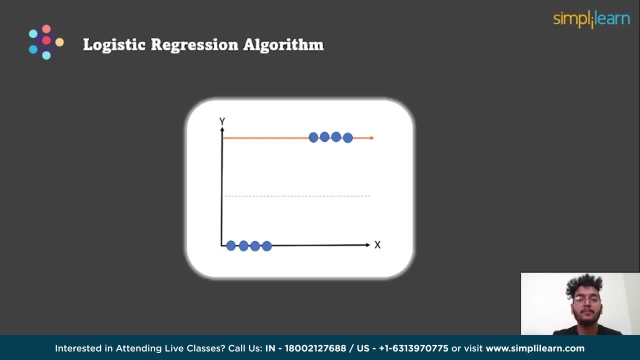 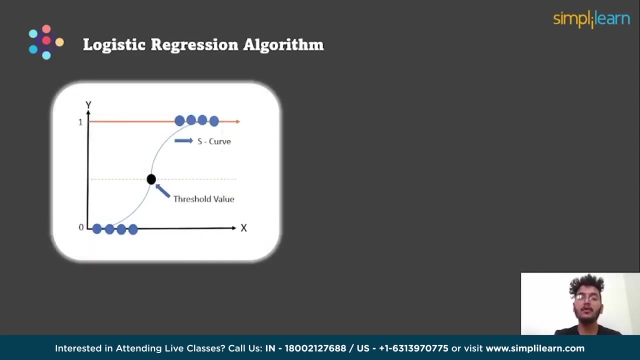 one is the transaction is not fraudulent. In logistic regression, rather than fitting a regression line, we fit an as-formed logistic capability which predicts 2 credit cards per greatest value, 0 or 1.. The logistic regression equation can be calculated from linear regression equation. The steps to get logistic regression equations are the equation of straight line. 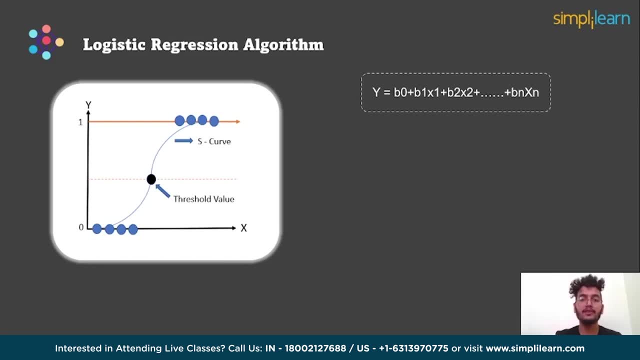 can be written as: y equals to b0 plus b1, x1 plus b2, x2 till bn, xn. In logistic regression, y can be between 0 and 1 only, So for that let's divide the above equation by 1 minus. 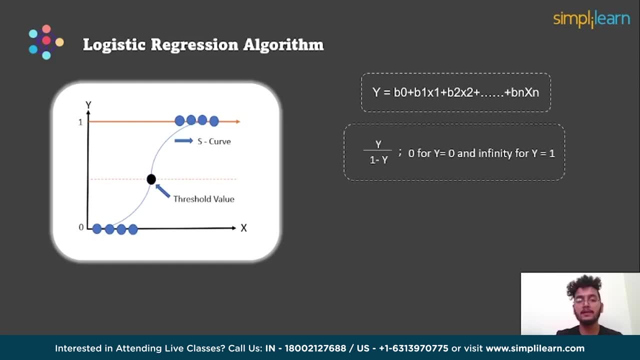 y, Then the equation will be y upon 1 minus y, that is 0 for y0 and infinity for y equals to 1.. But range between minus infinity to plus infinity. then we have to take the logarithm of equation and now it will become log of y upon 1 minus y equals to b0 plus b1, x1 plus. 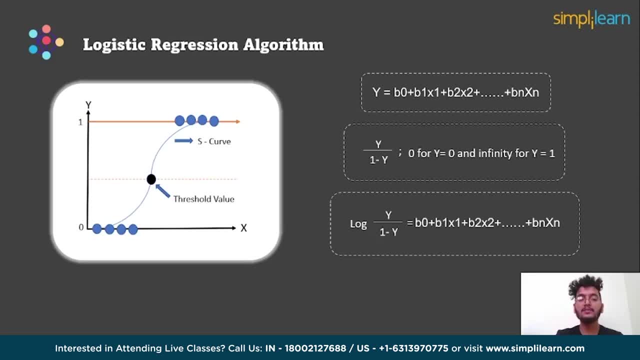 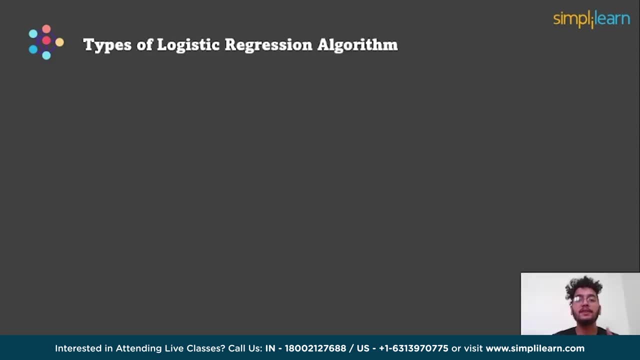 b2, x2, so on till bn, xn. Let's move forward and see types of logistic regression. There are three types of logistic regression that can be classified. First one is binomial. In binomial logistic regression there can be only two possible types of dependent variables. 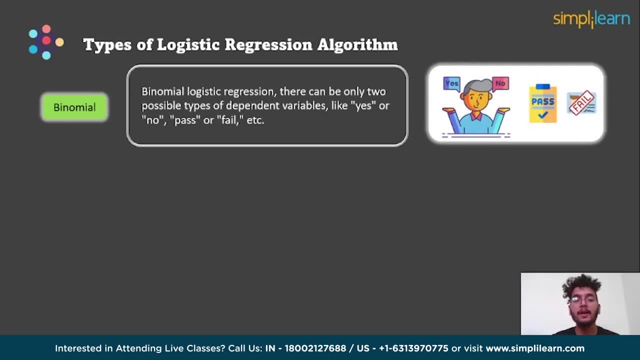 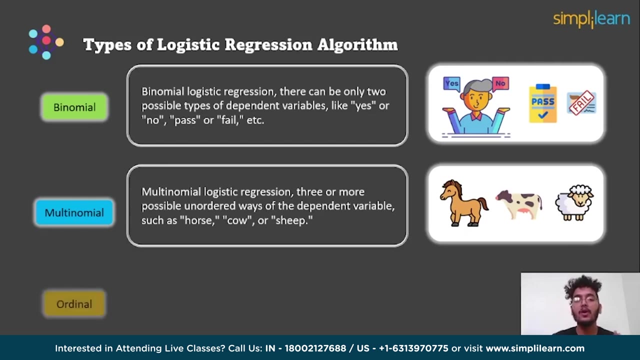 like yes or no, pass or fail, man, woman and many more. And the second one is multinomial. In multinomial logistic regression there can be three or more possible unordered ways of dependent variable, such as horse, cow and sheep. And the last one is ordinal In binomial. 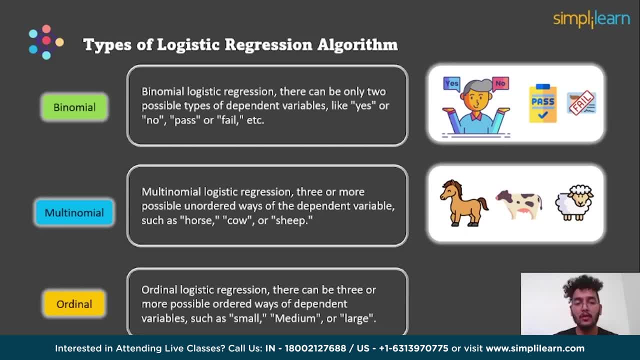 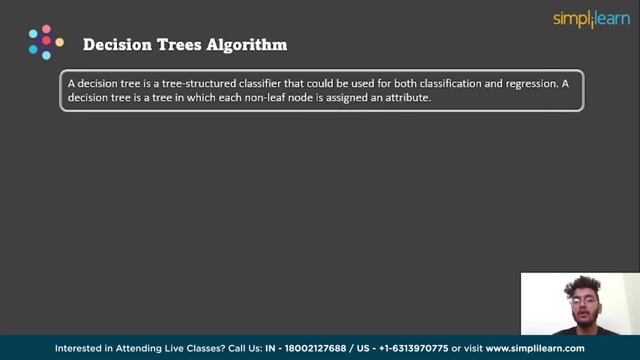 in ordinal logistic regression there can be three or more possible ordered ways of dependent variable, such as small, medium or large, Moving forward. let's see decision trees in detail. A decision tree is a tree structured classifier that could be used for classification and regression. A decision tree is a tree in which each non-leaf node 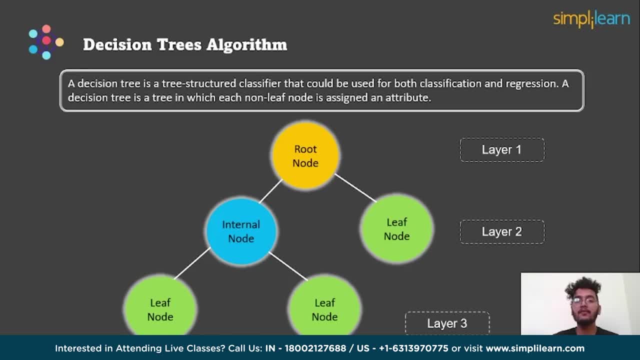 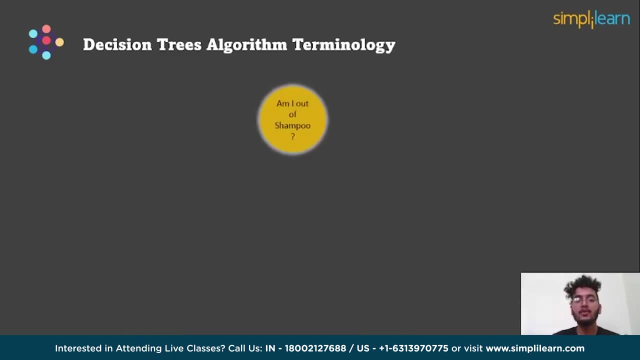 is assigned to an attribute. Additionally, each arc contains one of the available values for its parent node, Which is associated with each leaf node. that is the node from where the arc is directed. Let's see some decision tree terminology. First one is root. that contains the entire. 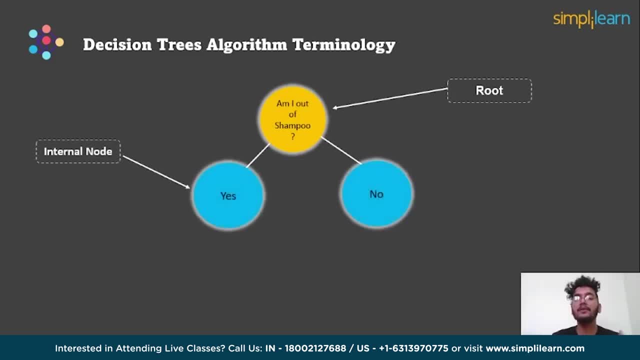 data set. The next one is node attached for the data of a certain attribute. And the third one is branch, which connects the node to internal node or the internal node to leaf node. And the fourth one is leaf node, the terminal node that predicts the outcome. Let's 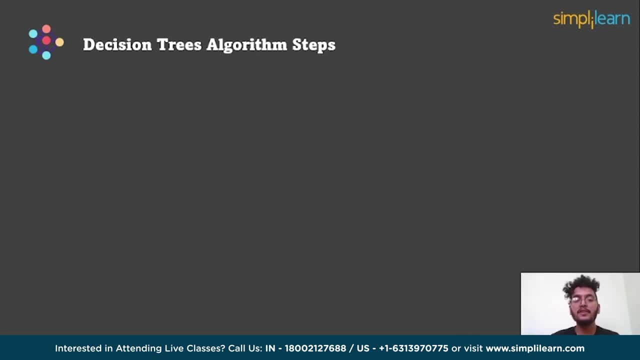 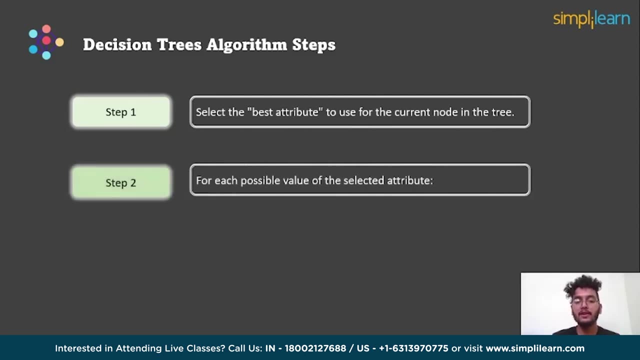 move forward and see decision tree algorithms. The first one is select the best attribute to use the current node in the tree. The second one is, for each possible values, select the attributes. The third one is partition the examples using the possible values of this. 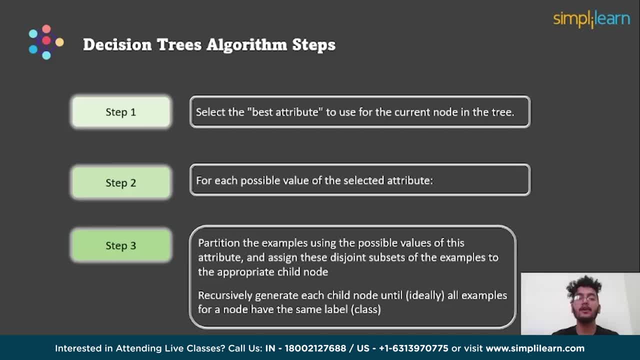 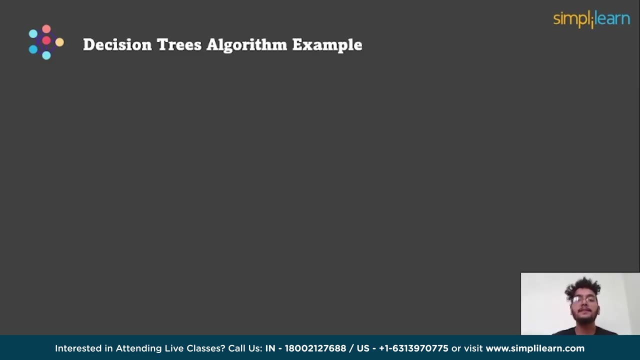 attribute and assign these disjoint subset or the example to the appropriate child node. Recursively generate each child node until, ideally, all examples for a node have the same label class. Moving forward, let's understand the decision tree, For building a decision tree. 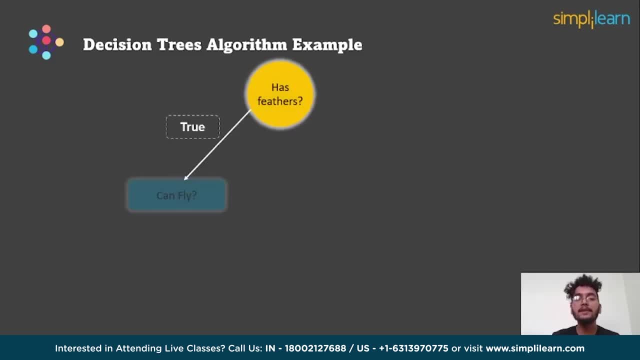 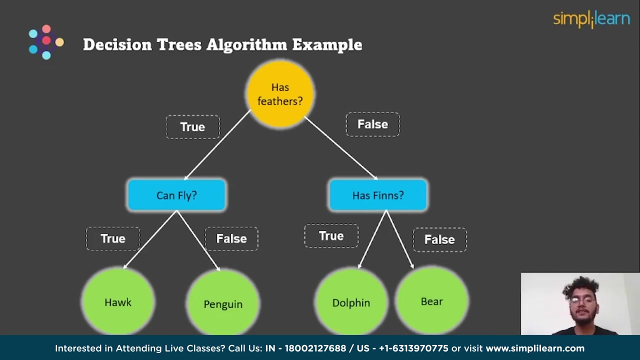 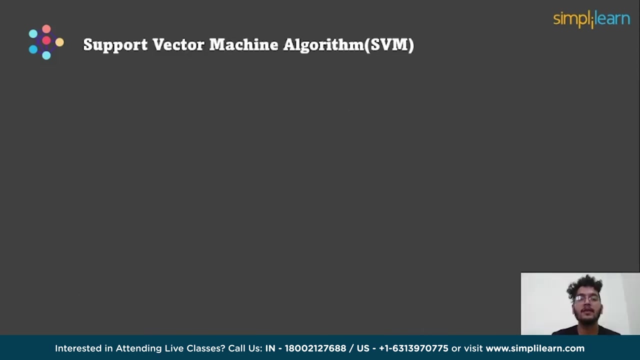 step one is select an attribute, then split the data into its children in a tree, Continue splitting with the available attributes and keep splitting until leaf nodes are pure, like only one class remains. a maximum depth is reached. a performance metric is achieved. Let's move forward and see SVM Algorithm Support Vector Machine Algorithms. 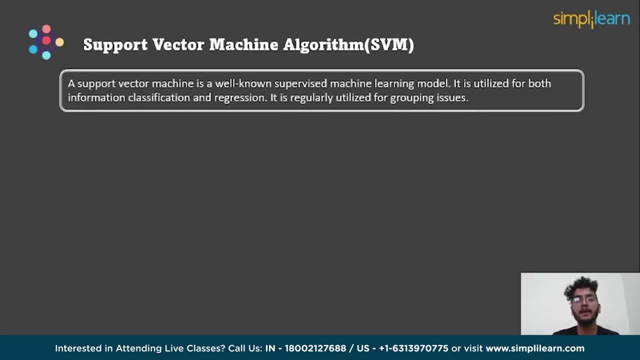 A support vector machine is a well-known supervised machine learning model. It is utilized for both information classification and regression. It is regularly utilized for the grouping issues. We can involve it in different life care system and we can involve it in typically happy or sad look arrangement. We can involve it in filters if we make specific looks. 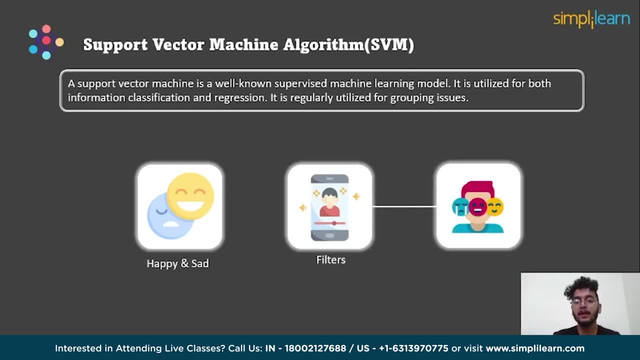 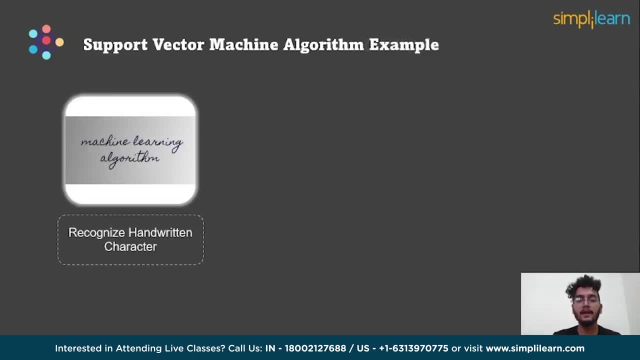 It would add the particular filter. according to the expression, The scope of articulation lies between happy and sad. Support Vector Machine helps him to recognize handwritten characters used widely like. checks continue to be a significant part of the majority of non-cash transactions and are frequently written by the pupil. The current check processing 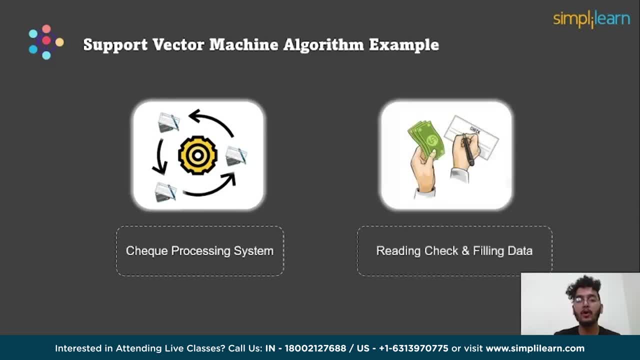 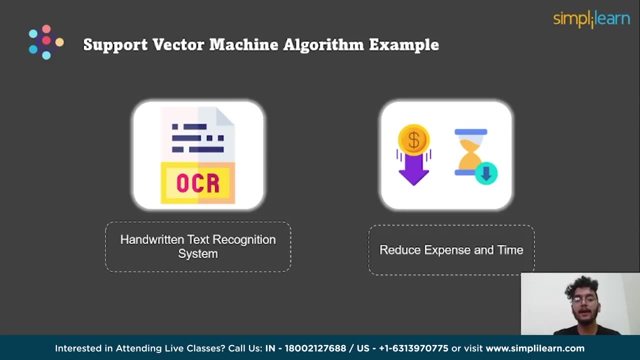 system in many developing nations involves a bank employee to read and manually enter the information in a check, While also verifying the data like signature and date. A handwritten text recognition system can reduce expenses and labor hours because a bank must handle several checks each day. 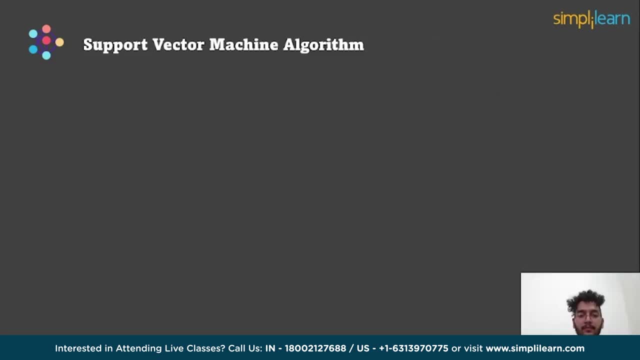 Moving forward. let's see the algorithm of SVM. The objective of support vector machine is to make the best line or choice limit that can isolate n-dimensional space into classes. So we can undoubtedly put the new data into classes. So we can undoubtedly put the new data into classes. 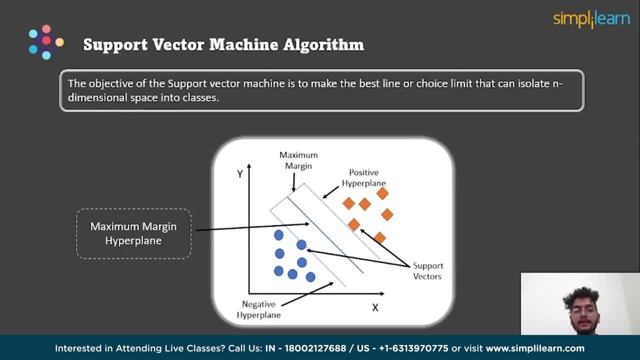 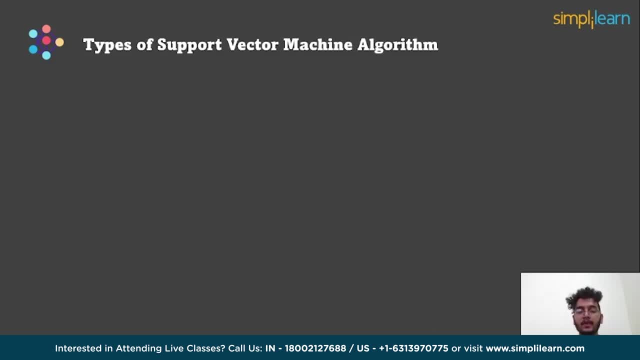 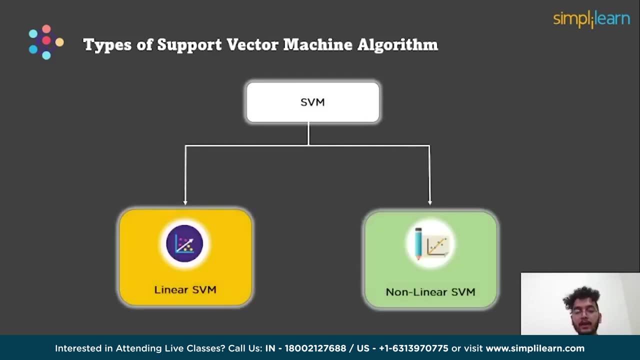 Let's move forward and these types of support vector machine. Support vector machine can be of two types. This 1 is linear SVM And the 2 is nonlinear SVM. Let's move forward and see That's work. and see linear SVM is utilized for linear leave. detachable information. 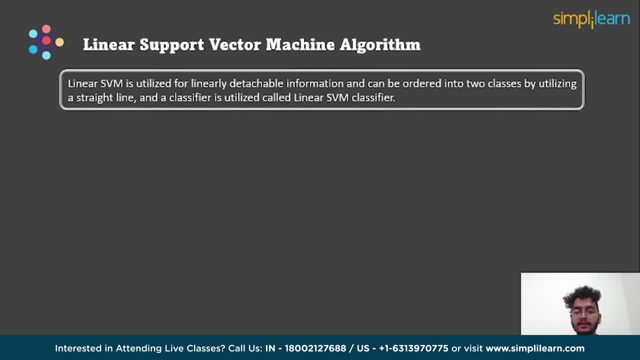 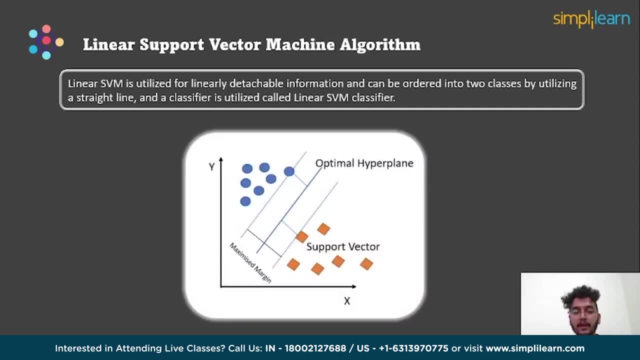 We can most simplify if a dataset is ordered into two classes by utilizing Iceberg hacker. and Então私 n вы можете Buy Attack Dark 둘러레. The soft rock was again saying a straight line. then such information are named linearly separable information and. 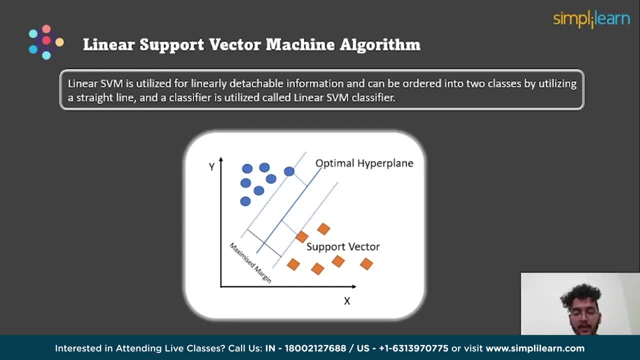 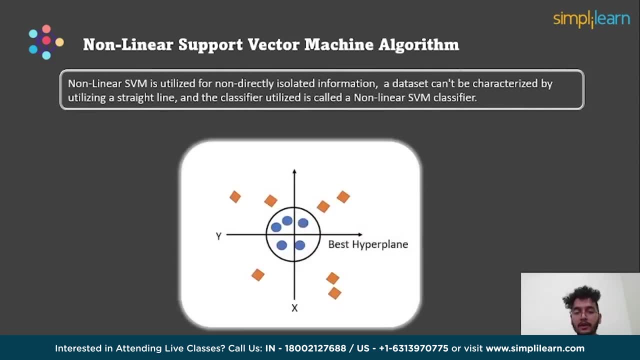 a classifier is utilized, called linear SVM classifier. Moving forward, let's see nonlinear SVM. Nonlinear SVM is utilized for non-directly isolated information and that implies, in the event that a dataset can't be categorized by utilizing a straight line, such information. 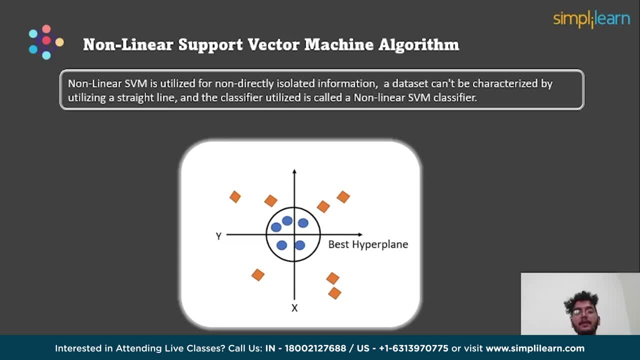 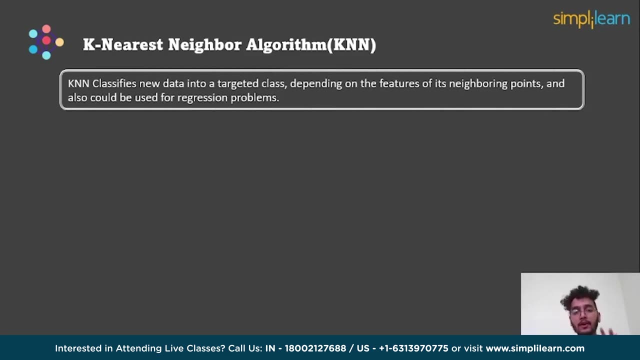 is named non-directed information and the classifier utilized is called a non-linear SVM classifier. Moving forward, let's see K-NN algorithm in detail. K-NN is a supervised learning technique. K-NN classifies new data into a targeted classes depending on the features of its neighboring. 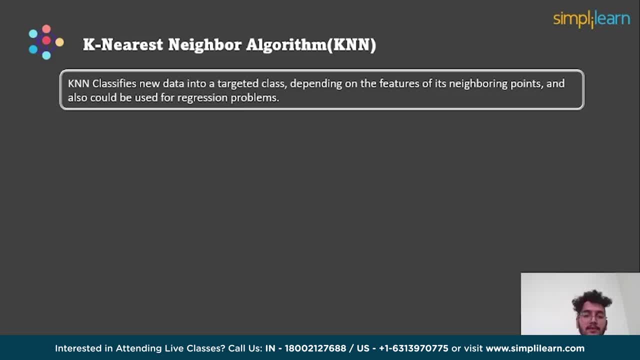 points and also be used for the regression problems. It is an instance-based learning algorithm and a bit-lazy learning algorithm. K-NN can also be used for regression problems. K-NN calculation stores every one of its accessible information and orders another information. 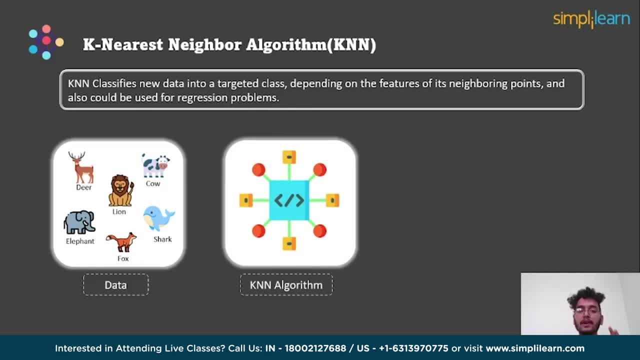 point based on the likeness. This means that when new data information appears, it usually tends to be successfully categorized into a good-suit classes using the K-NN algorithm. Let's imagine we have an image of animal that resembles a cow or ox. 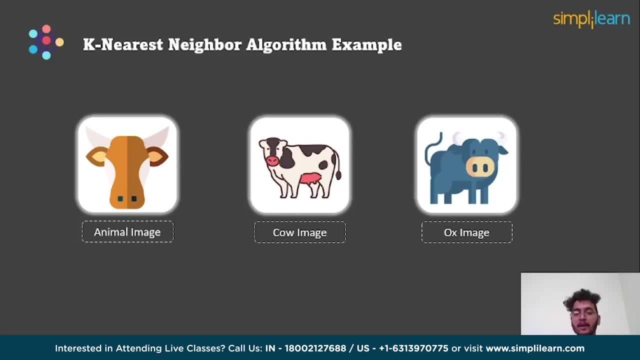 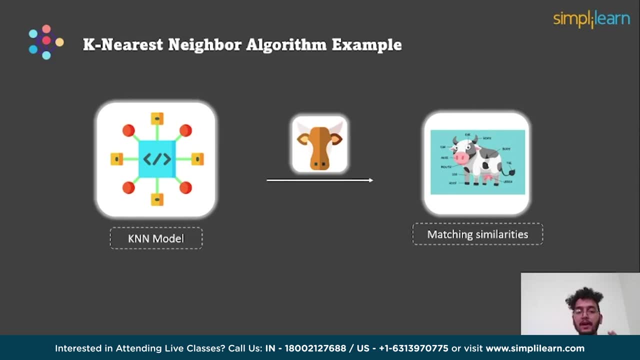 However, here we are not sure if it is a cow or ox, as K-NN method is based on a likeness matrix, It will identify the properties of new data that are related to the image of cow or ox And, based on those qualities, it will classify the data as belonging to either cow or ox. 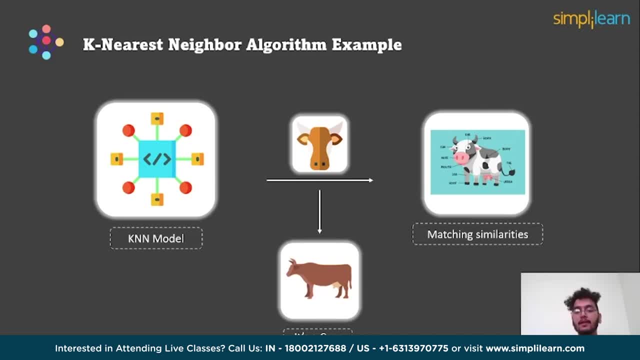 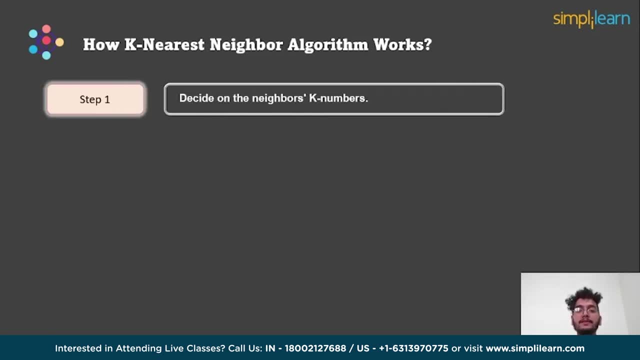 group Moving forward. let's see how does K-NN work. The steps to implement K-NN algorithms are: Step 1. Decide on the neighbors' k-numbers. Step 2. Calculate the Euclidian distance between k-neighbors in step 2.. 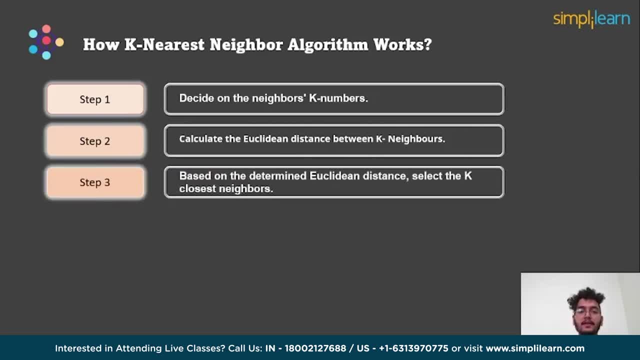 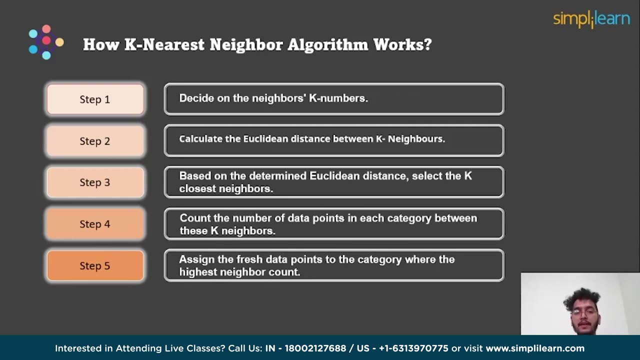 Step 3. And one is based on the determined Euclidian distance. select the k-closest neighbors. Step 4. Count the numbers of data points in each category between these k-neighbors. Step 5. Assign the fresh data points in the category where the highest neighbors count. 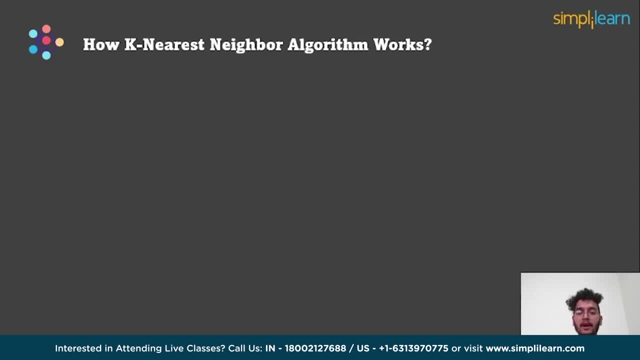 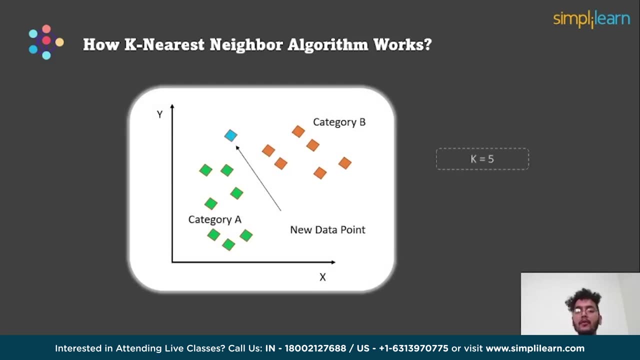 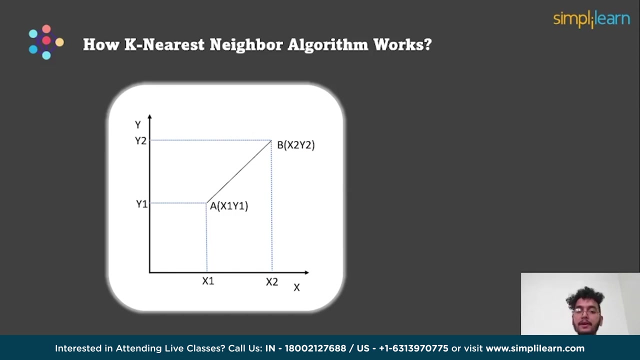 And then K-NN model is ready. Let's say we need to add a new data point to the vital category. At first we will decide on the numbers of neighbors. therefore we will pick k equals 1. Then the Euclidian distance between the data points, and then can be determined. 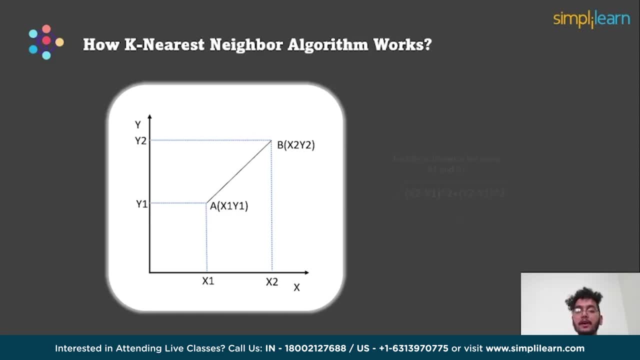 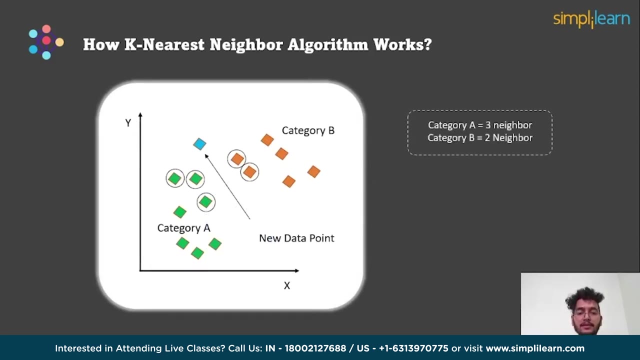 The distance between two points, known as the Euclidian distance, can be determined by Under root of x2 minus x1 ka whole square, plus y2 minus y1 whole square. Then we determine the closest neighbors by calculating the Euclidian distance. There are three closest neighbors in category A and two closest neighbors in category B. 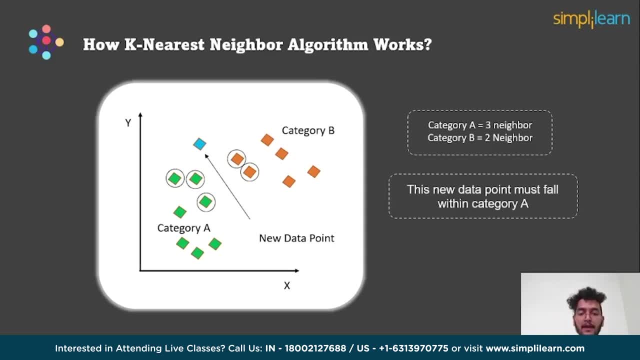 Step 6.. Each new data point must fall with category A Because, as we can see, its three closest neighbors are also from group A. After understanding the K-NN algorithm, let's move forward and see the k-means algorithms in detail. 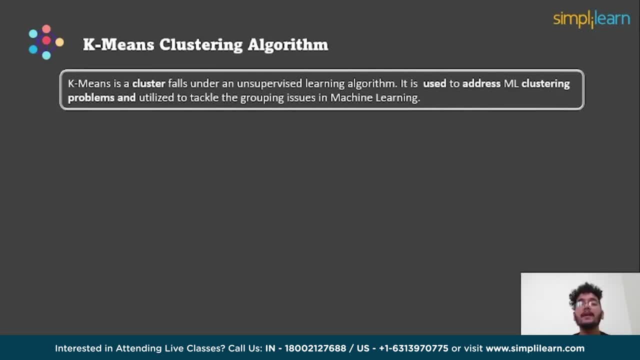 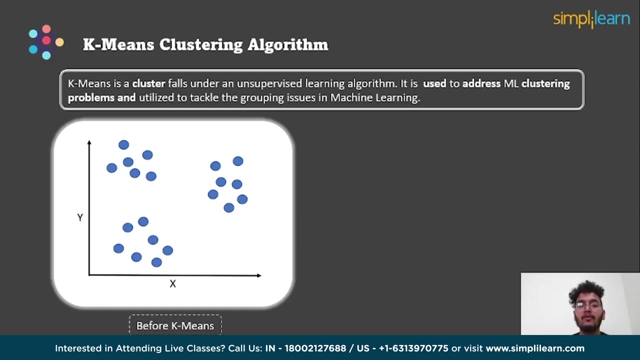 The k-means is a cluster pulse under that is an unsupervised learning algorithm. It is used to address machine learning clustering problems and utilized to tackle the grouping issues in machine learning. It permits us to bunch the information into various gatherings. It is a helpful method for finding the classification of groups in the unlabeled dataset without 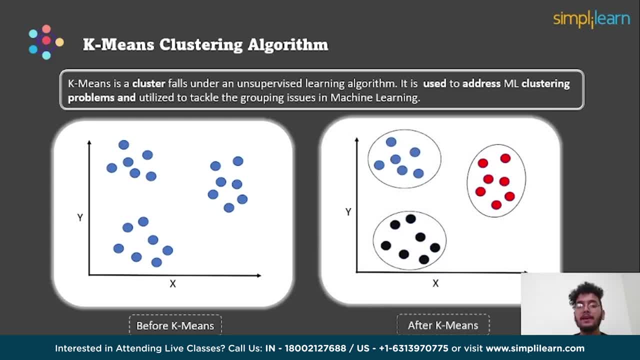 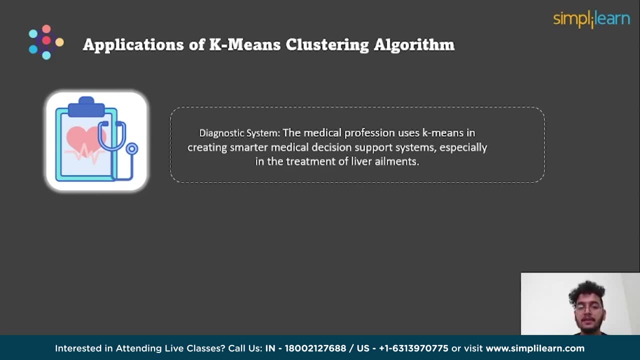 the requirement of any training. This k-means algorithm groups the data into similar classes. Let's see some applications of k-means clustering. Let's see some applications of k-means clustering Diagnostic system. The medical profession uses k-means clustering in creating smarter medical decisions. 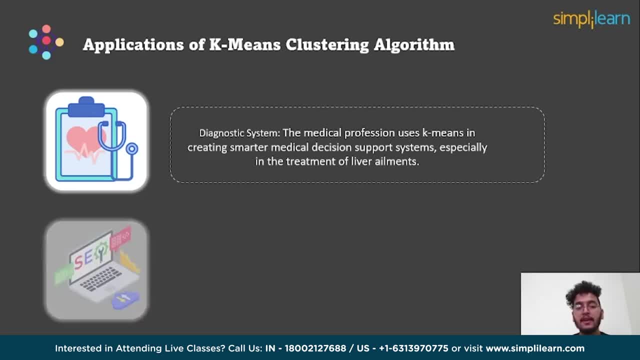 Support system, especially in the treatment of liver alignment. The second one is search engine. Clustering forms the backbone of search engine. When a search engine is performed, the search results need to be grouped, and the search engines very often use clustering to do this. 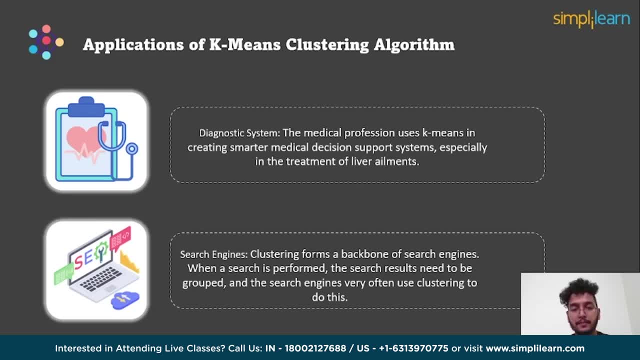 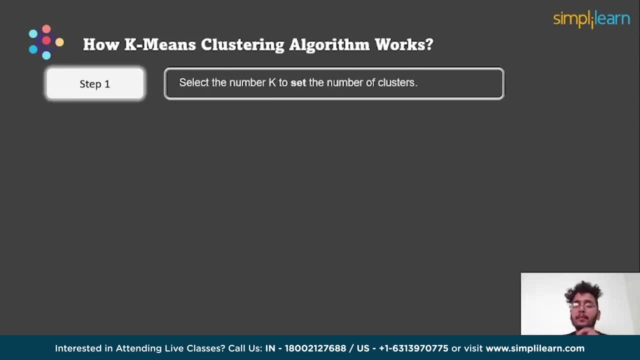 Moving forward, let's see how k-means algorithm works. The steps to implement k-means algorithms are: Step 1. Select the number k to set the number of clusters. Step 2. Select a random k-point or centroid: Step 3.. 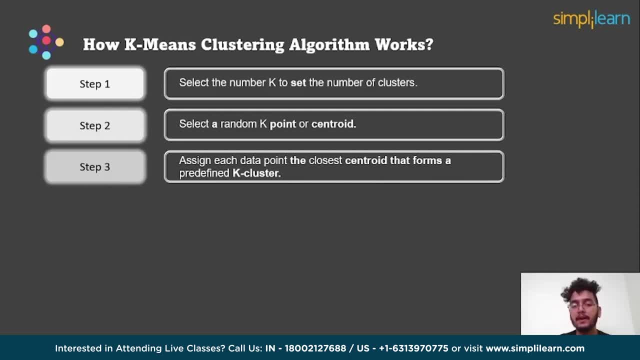 Assign each data point: the closest centroid- Step 4.. Determine the variance and set new gravity points for each cluster- Step 5.. Repeat the third step. This means reallocating each data point to the new closest centroid cluster- Step 6.. 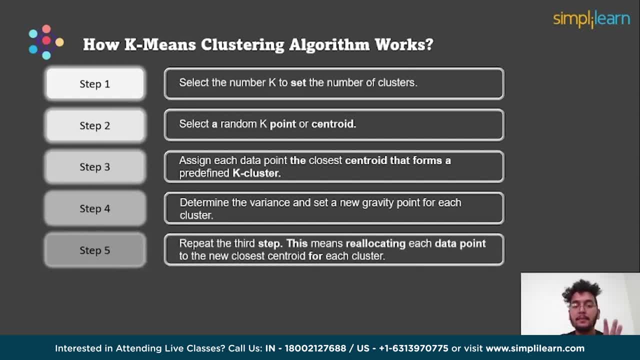 If a reassignment occurs, go to step 4.. Otherwise, go to exit Step 7.. The model is ready to use. So now we have an clear understanding of how k-means algorithm works. Let's move forward to see how k-means algorithm works. 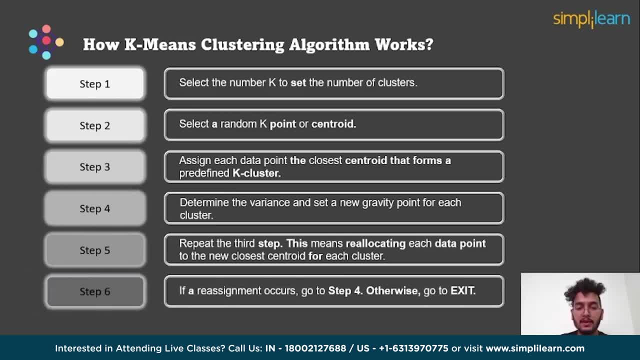 Step 7.. The model is ready to use Step 8.. The model is ready to use Step 9.. The model is ready to use Step 10.. The model is ready to use Step 11.. The model is ready to use. 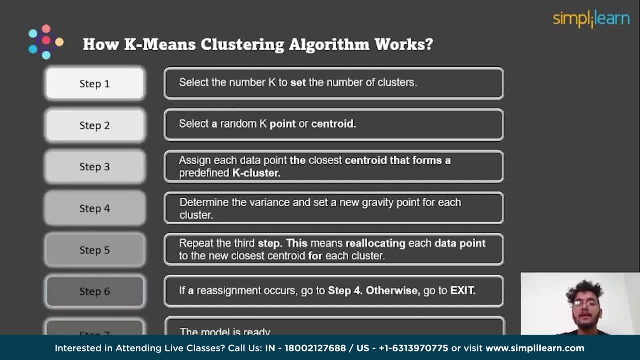 Step 12.. The model is ready to use. Step 13.. The model is ready to use. Now we have an clear understanding of how k-means algorithm works. let's move forward to see the graphical representation of k-means algorithm. 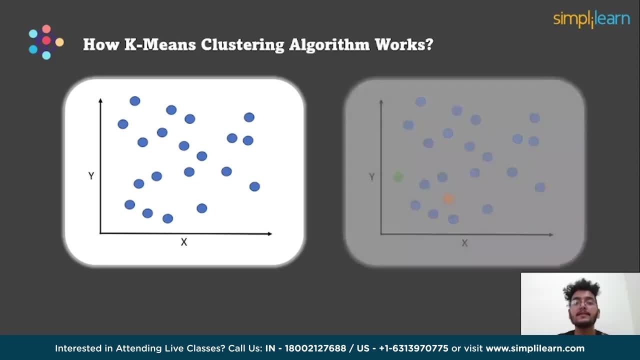 Consider that there are two variables, m1 and m2.. This is a scatter plot of these two variables along the x and y-axis. We should accept the number of k of bunches, that is, k equals to 2, to recognize the dataset and to place them into various groups. 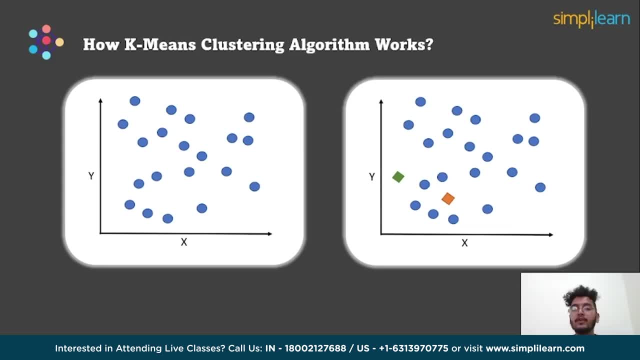 It implies here we will attempt to bunch these dataset into two unique groups. We will really want to pick an irregular k-point or centroid to frame this group. These centroids can be either the focus of the dataset or some of other points. Thus, here we are choosing under two points as k-points which are not the piece of our. 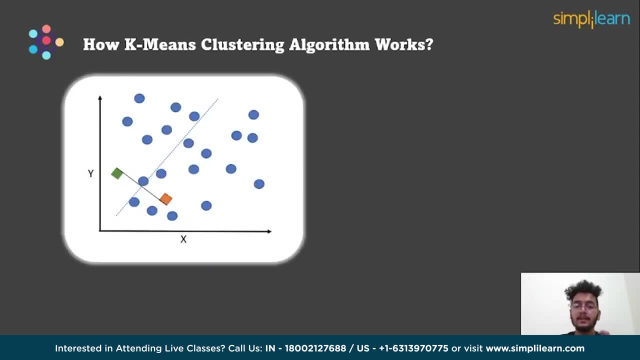 dataset. We will assign every data of interest in the scatterplot to the nearest k-point or centroid. We will register it by applying some math that we consider to find the distance between two points, ie Euclidian distance. Thus we will draw a median between both the centroids. 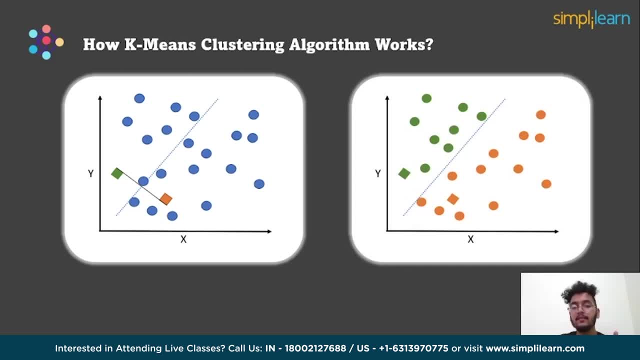 From the graph, the left half of the line are close points to the right and the k1 centroid Green is near the orange centroid. We should variety them as green and orange for clear representation. As a need might arise to track down the nearest group, we will repeat the cycle by picking. 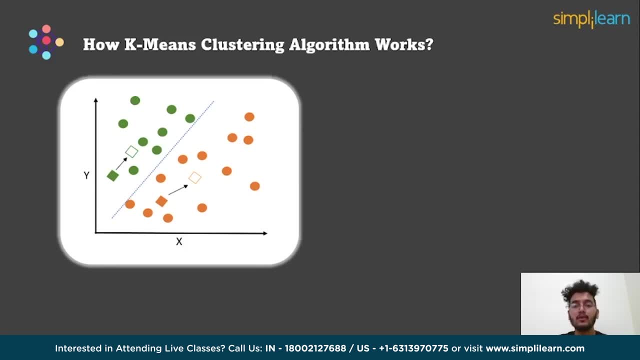 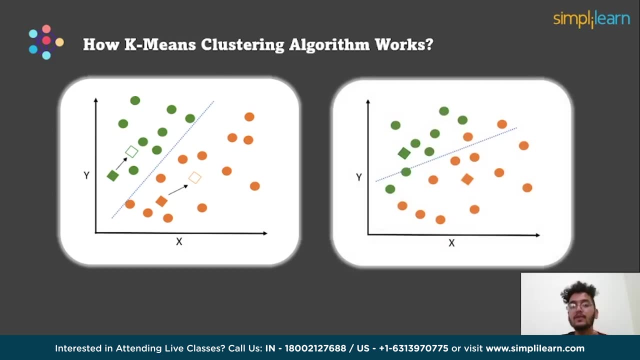 another centroid To pick the new centroid. we will figure out the center point of gravity of these centroids and will track down new centroid. Then we will reassign every piece of information to highlight new centroid. For this we will repeat a similar course of tracking down a middle line. 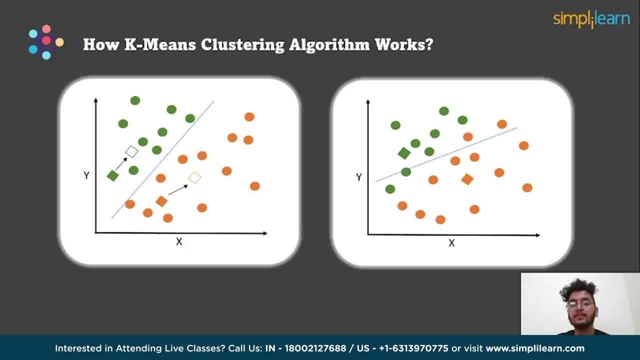 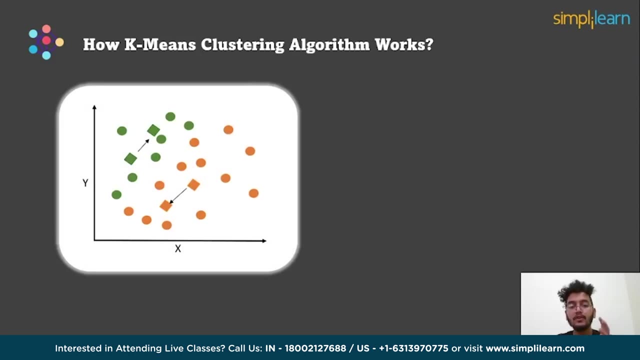 The middle will be like as seen in the picture: One orange point is on the left half of the line and two green points are on the right. Thus, these three points will be appointed to the new centroid. As reassignment has occurred, we will again go to step 4, tracking down new centroid or. 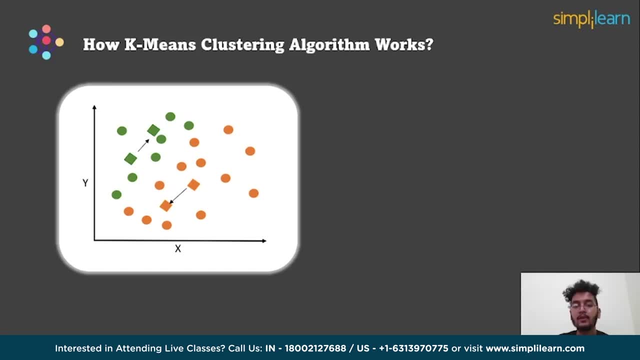 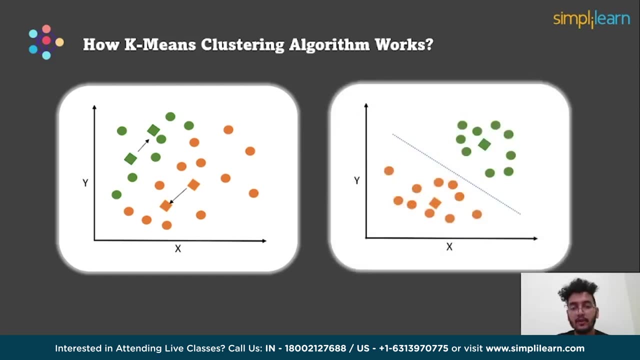 k points. We will repeat the cycle by tracking down the center point of gravity of centroid. So the new centroid will be displayed as like this: We now have new centroid, So once more, define the middle boundary and reassign the data of interest. 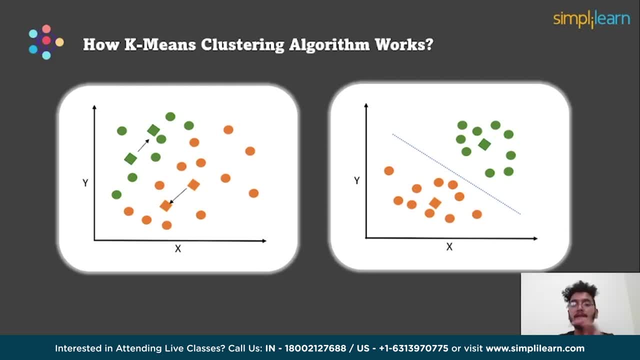 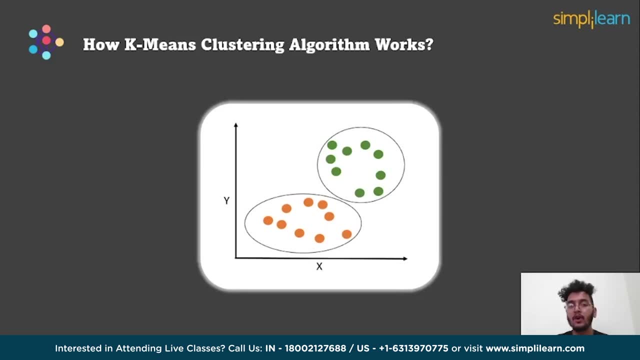 By this graph. there are no unique pieces of information on one or the other side of the line implying our model is shaped By the previous graph. there are no unique pieces of information on one or the other line Supplying our model is shaped. 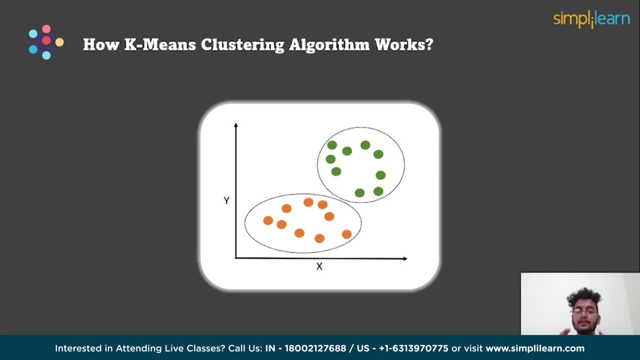 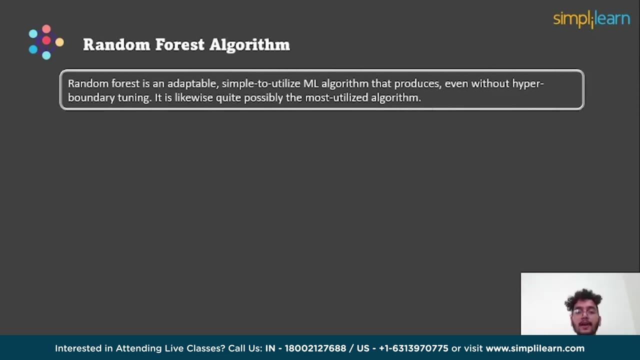 As our k-means model is ready, and the two last groups will be displayed as like these: Now we have a clear understanding of how k-means clustering algorithm works. Now let's move forward to understand random forest algorithm. Random forest is an adaptable, simple to utilize machine learning algorithm that produces even. 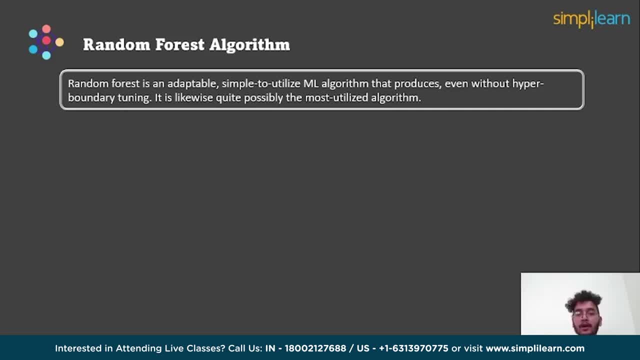 without the hyperboundary tuning, An extraordinary outcome. more often than not, It is like what we have seen in the previous graph. It is like what we have seen in the previous graph. It also identifies quite possibly the most utilized algorithm because of its effortness. 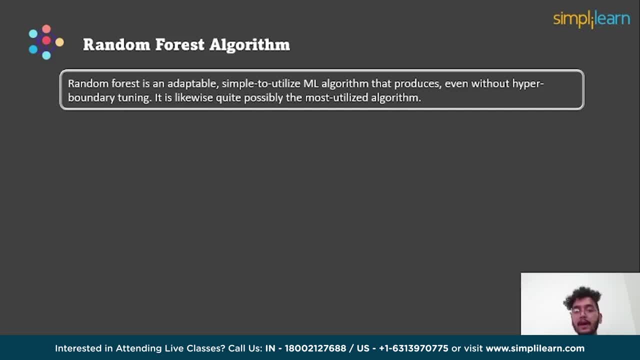 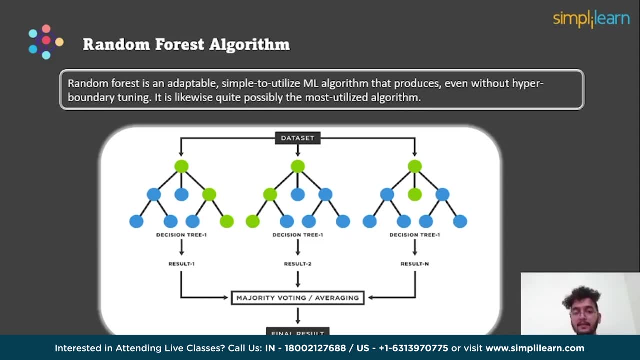 and variety. like it tends to be utilized for both grouping and classification tasks. Random forest is a classifier that contains various choice trees on different subsets of the given dataset and takes the normal to work on the present exactness of the dataset. Instead of depending on the choice tree, the random forest takes the forecast from each. 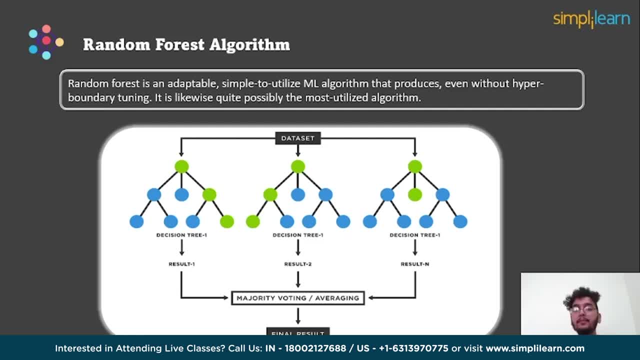 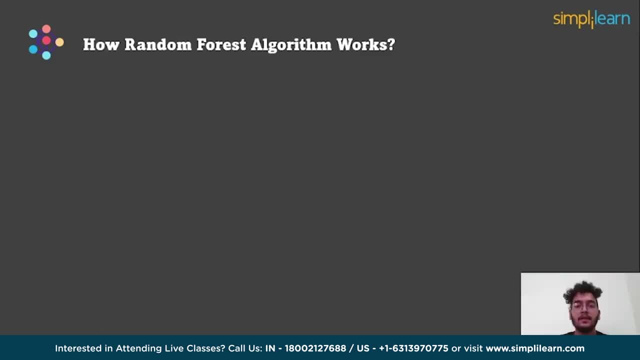 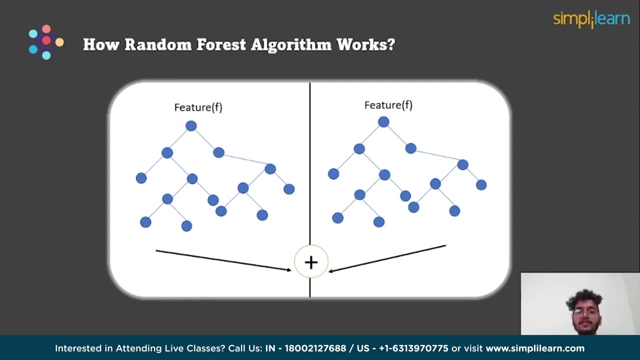 tree of the larger part of watts of expectation. it predicts the final result. Now let's move forward and see how does random forest work? We should see the random forest in order, since the arrangement is now and again thought to be the structured block of machine learning. 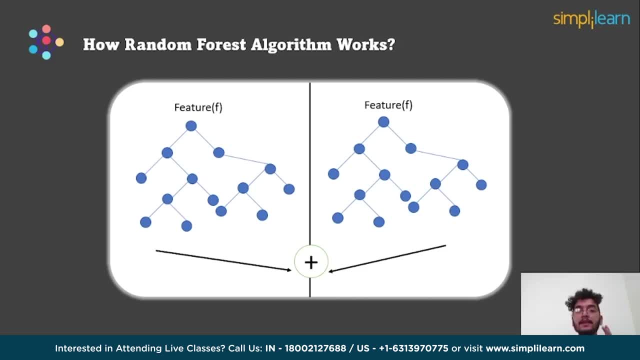 This is what a random forest would look like with two trees. The random forest has a similar hypermeter to our decision tree or a paging classifier. Luckily, there is a compelling reason: need to consolidate a decision tree with a paging classifier, Since you can undoubtedly utilize the classifier classes of random forest with random forest. 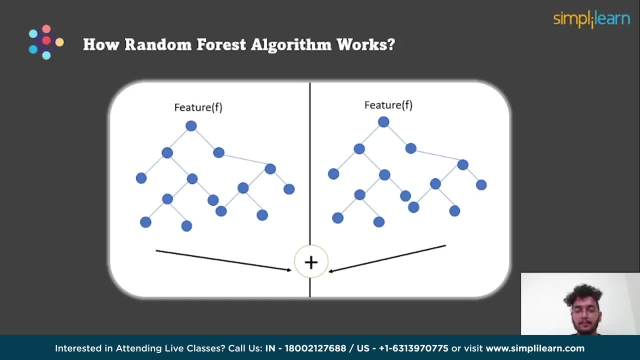 you can likewise manage tasks using the algorithm regressor Random forest. add extra arbitrage to the model while developing the trees. rather than looking for the main element while parting a node, It looks to the best component among an irregular subset. These outcomes in a wide variety often result in a superior model. 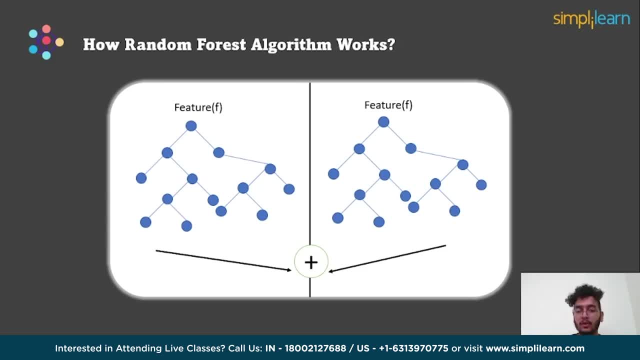 Subsequently, in a random forest, just a random subset of the element is thought about the algorithm. You might make trees more random by involving random edges for each component, instead of looking for the most ideal limits like a typical choice tree does. Let's move forward and see some application of random forest algorithms. 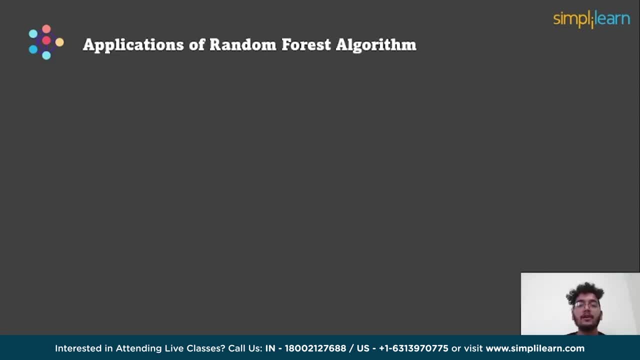 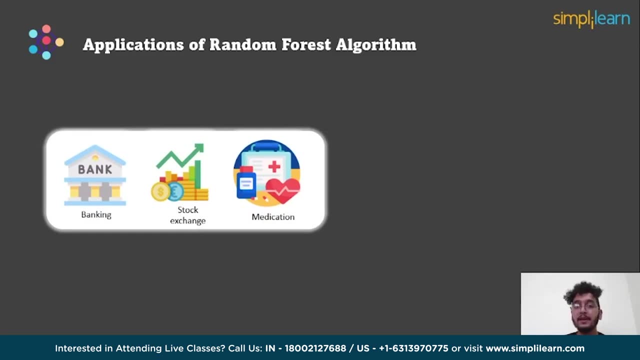 Random forest is in this. Let's move forward. Random forest is involved at work by researchers in numerous ventures, including banking stock exchanging, mitigation and many more. It is utilized to predict things which assist these businesses with running productively, like client activity, patient history and safety. 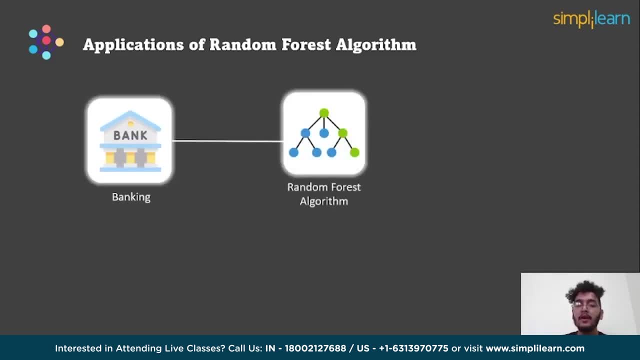 In banking, random forest is used to identify clients who are more likely to pay back their debts on schedule. Additionally, it is utilized to forecast who will make more frequent use of bank services. even fraud detection uses it- The Robin Hood of algorithms. indeed, Random forest is a tool used by stock traders to forecast future stock behavior. 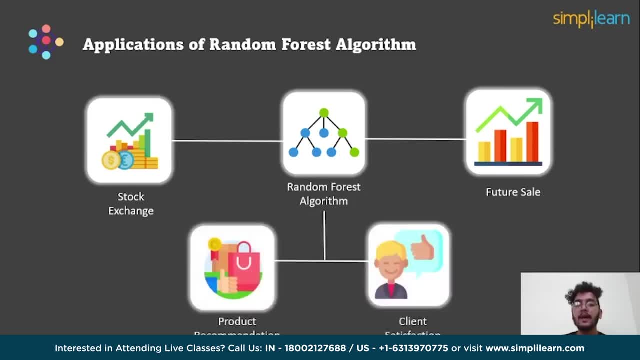 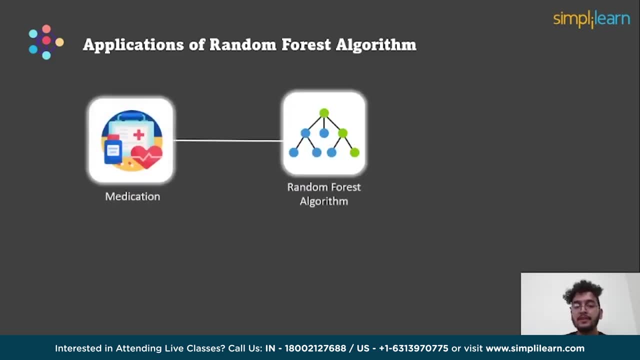 Retail businesses utilize it to make product recommendations and forecast client satisfaction. Random forest can be used in the healthcare industry to examine a patient's medical history and detect disorders. Random forest is a tool used by pharmaceutical experts to determine the ideal mix of ingredients in treatment or to forecast drug sensitivity. 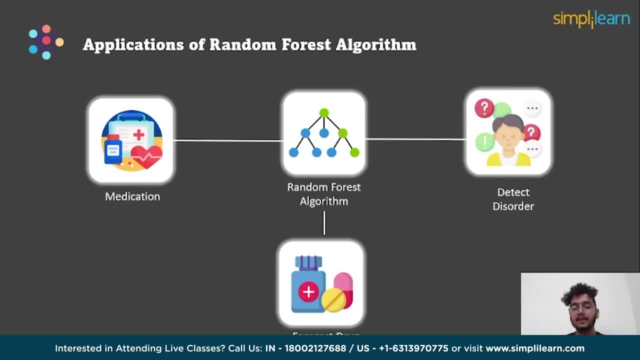 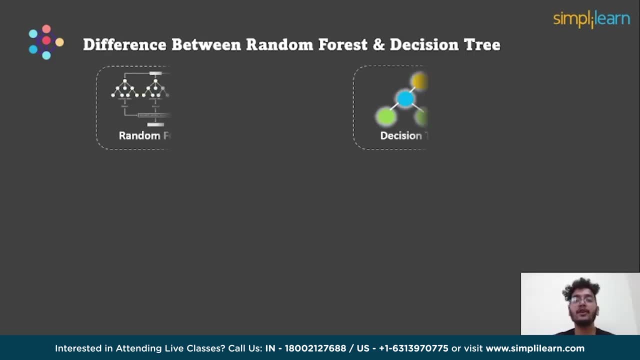 By seeing application of random forest algorithm, let's move forward and see some difference between decision trees and random forest. Let's see the difference between random forest and decision tree. The first one is: while building a random forest, the number of rows is selected randomly. 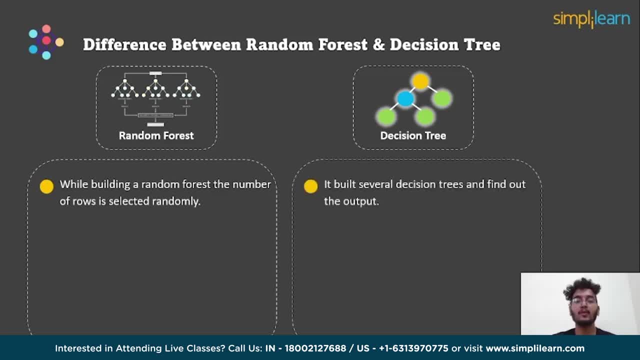 In decision trees. it builds several decision trees and find out the output. The second one is It combines two or more decision trees together In decision trees, whereas the decision is a collection of variables or datasets or attributes. The third one is: 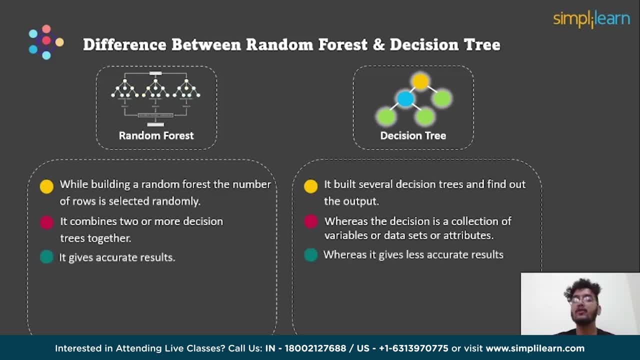 It gives accurate results, whereas it gives less accurate results. The fourth one is: By using random forest, it reduces the chance of overlifting, whereas decision trees it has the possibility of overlifting. The fifth one is: Random forest is more complicated to interpreters, whereas the decision tree is more complicated. 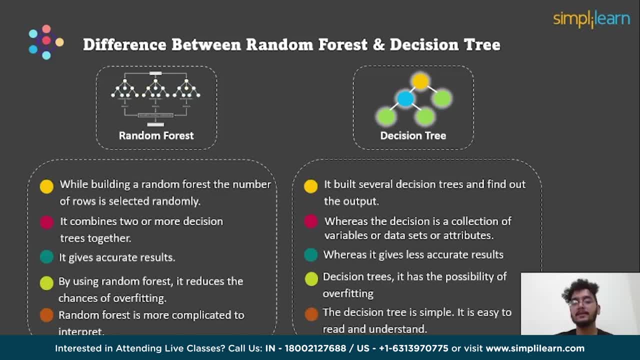 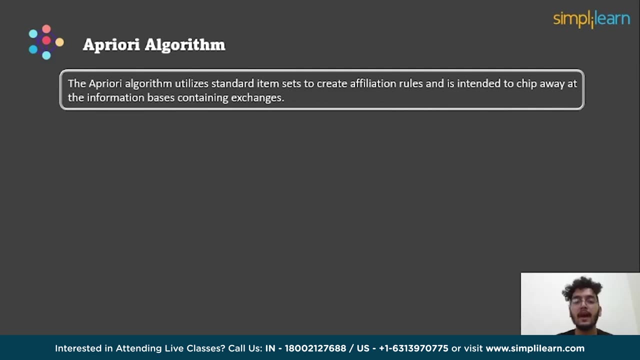 to interpret. The decision tree is simple. It is easy to read and understand. After seeing what is random forest how it works, let's move forward to see a priori algorithm in detail. The a priori algorithm utilizes standard item sets to create affiliation rules and is intended: 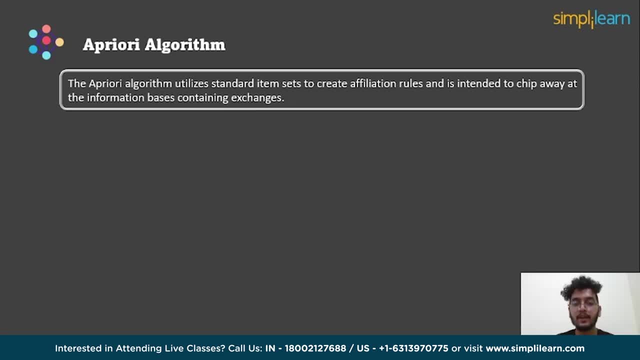 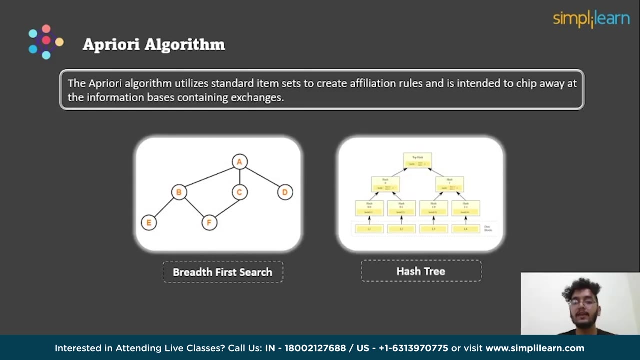 to chip away the information bases containing exchanges. With the assistance of these affiliation rules, it decides how firmly or feebly two objects are associated. This algorithm utilizes a breadth-first search and hash tree to work out the item set association effectively. It is the iterative interaction for finding out the successive item sets from the huge 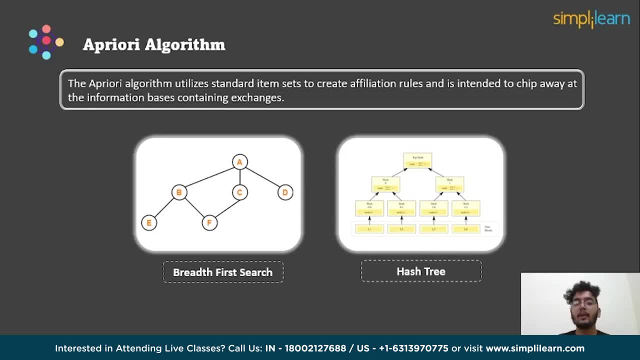 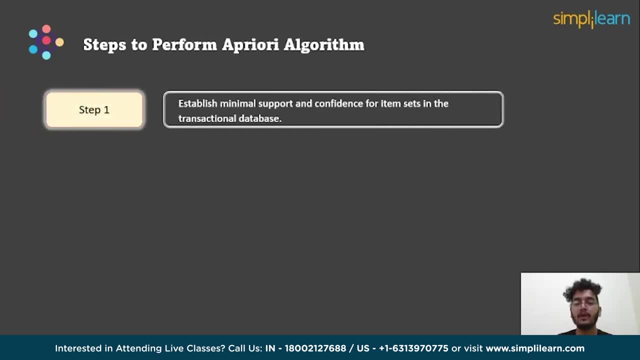 dataset. Let's move forward and see steps for a priori algorithms. The steps for a priori algorithms are: Step one is Establish minimal support and confidence for item sets in the transactional database. The second one is Take all transaction supports with a greater confidence. 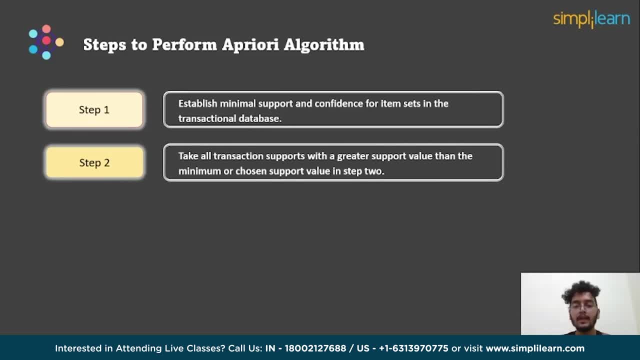 The second one is: Take all transaction supports with a greater confidence. The second one is: Take all transaction supports with a greater confidence. The third one is Tracking down all the roles in these subsets with confidence value greater than the threshold value: Allation and reservation. 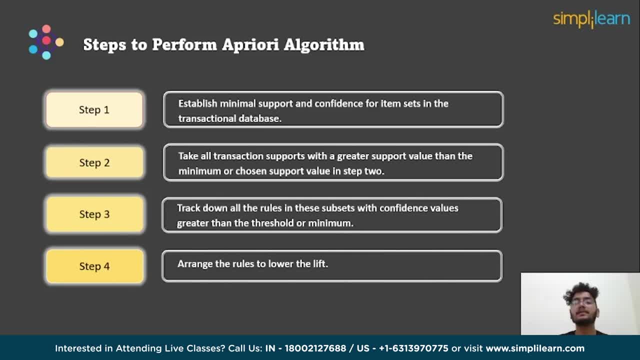 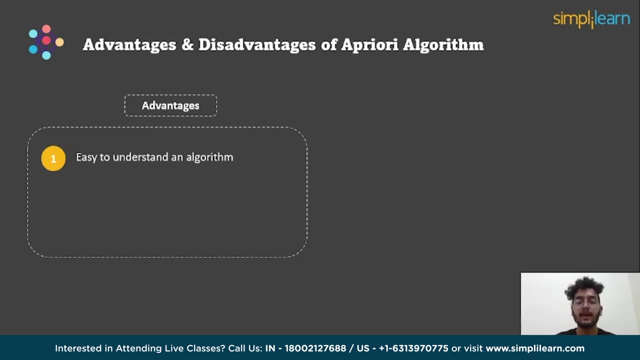 The fourth one is: Arrange the roles to lower the LIPT. At last we will see some advantage and disadvantage of a priori algorithms. The advantages of a priori algorithms are Easy to understand algorithm and are single line Colleges. The second one is: 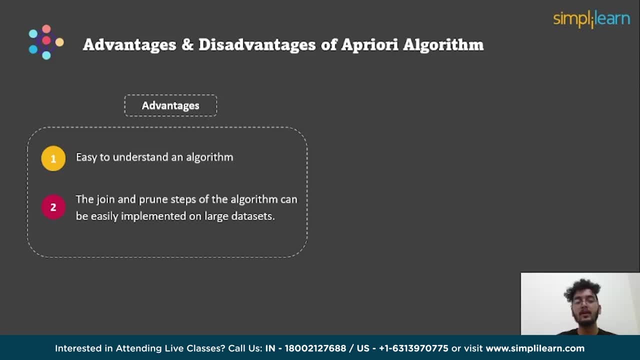 algorithms can be easily tuned. This will Vous cleverly see A priori may include even fewer Projects easily implemented on the large data set. The disadvantages of Apriori algorithms are: the Apriori algorithms work slowly as compared to the other algorithms and the second one. 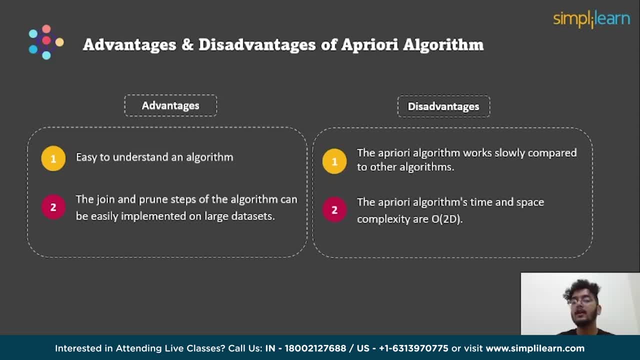 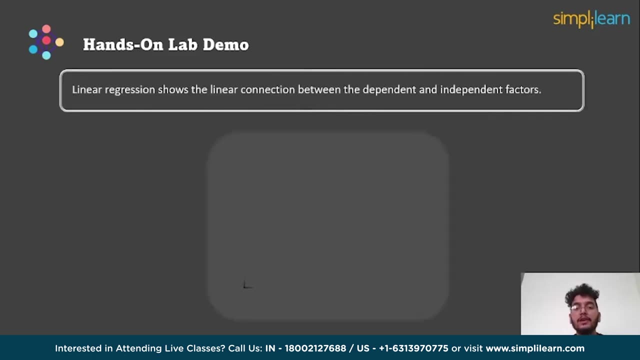 is the Apriori algorithms. times and space complexity are O of 2D, which is very low compared to the other ones. Let's move forward and see some hands-on lab demo. So we will see a hands-on lab demo on linear regression. As we know, linear regression is a way to find 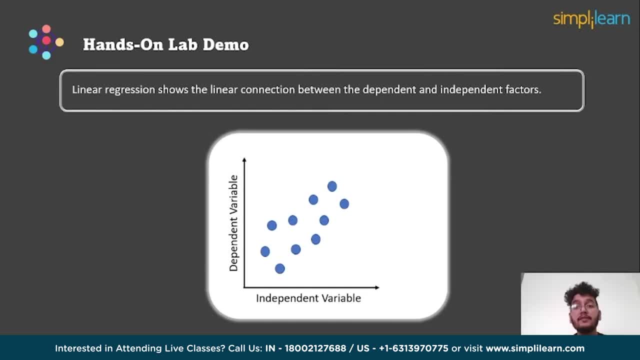 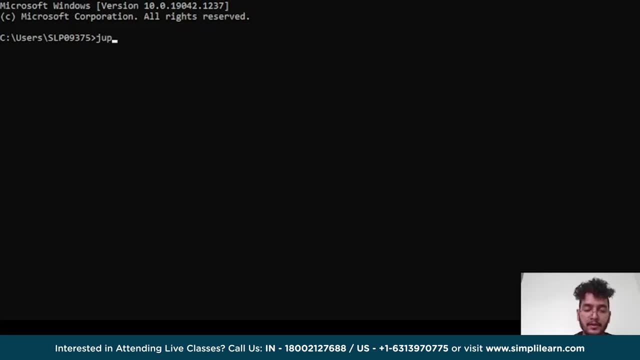 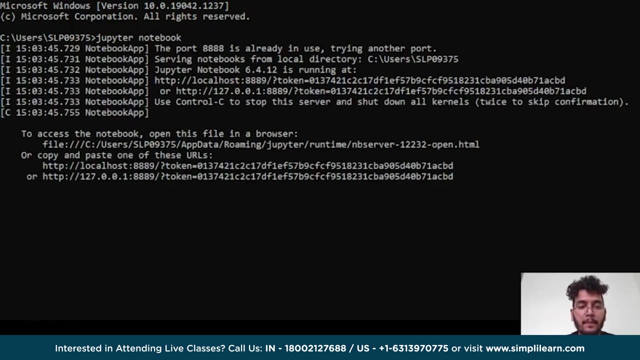 or to predict the relationship between two variables. Generally we use X and Y. So first we will open command prompt to write command to open Jupyter Notebook. So we will write Jupyter Notebook and then press enter. So this is the landing page of Jupyter Notebook. 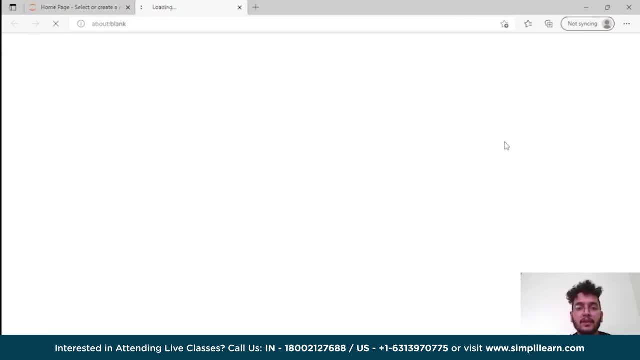 and select open new Python file. So this is how Jupyter Notebook UI looks like. So at first we will import some major libraries of Python which will help us in mathematical functioning. So the first one is NumPy. NumPy is a Python library used for working with 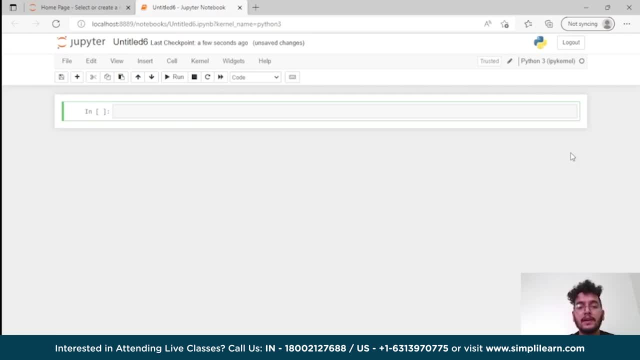 arrays. It also has functions for working in domains like linear algebra and matrices. It is an open source project and you can use it freely. NumPy stand for numerical Python, So we will write like: import NumPy as numpy. Here Np is used for denoting NumPy, So we will import the next library, Pandas, Pandas. 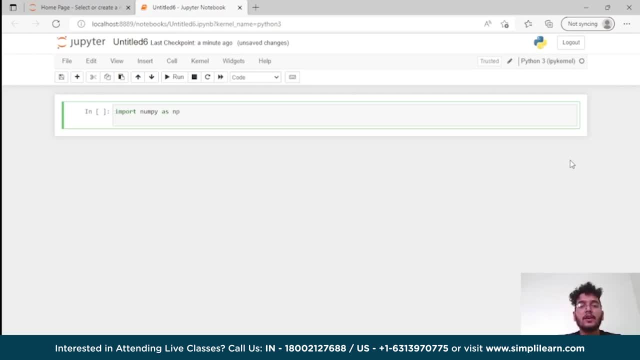 is a software library written for Python programming For like data manipulation and analysis. In particular it offers data structures and operation for manipulating numerical labels and time series. So we will write import Pandas as pd. Here pd is used for denoting NumPy, So we will write import Pandas as pd. Here pd is used for denoting NumPy, So we will write import Pandas as pd. Here pd is used for denoting NumPy, So we will write import Pandas as pd and a dd We will write import anakadep φ11.. 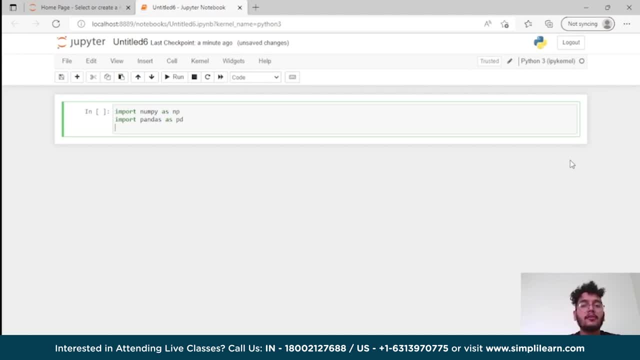 And here we will write: import esquiri ph VaVa. This willandoot is known as a symbol forнос, So we will divorce its points, so like pd to have it. and then next library we will visit AdvaTable, And this site is matplotlib, which is a. 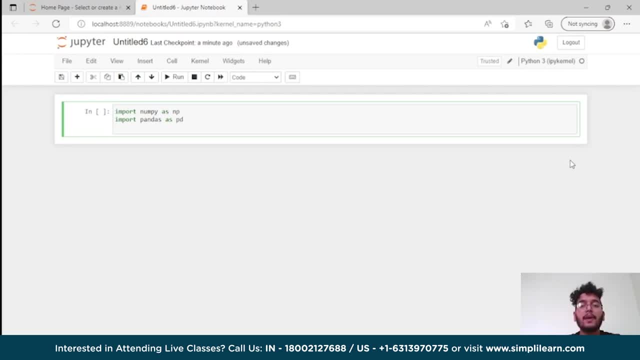 �� candidate without us for users so very small memory compared to the site of our model. We will create a stable divide take a node client module and select slash static, Java squad, and we need to input the code pull a— alguém home. 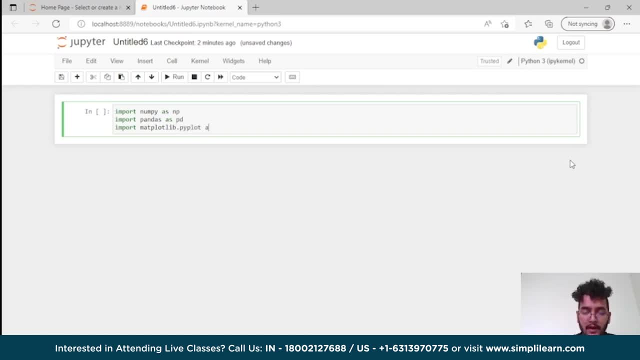 And power. next, if we take Matplotlib, is capabilities rather than the standard, or So after importing the libraries we will move ahead and import dataset. So for importing dataset we have to write: dataset equals to pd, dot, read underscore csv. And here we have to give the path of the file: dataset, dot, csv. 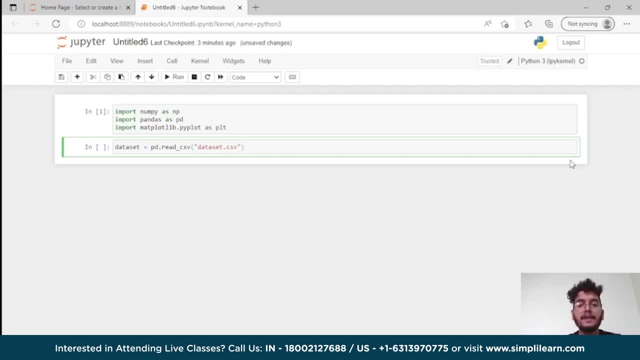 Here, pd is for pandas library, and read is used for reading the dataset from the machine And csv. csv is used for the type of file which you want to read. So after reading, let's see our data. So we will write dataset dot head and press enter. 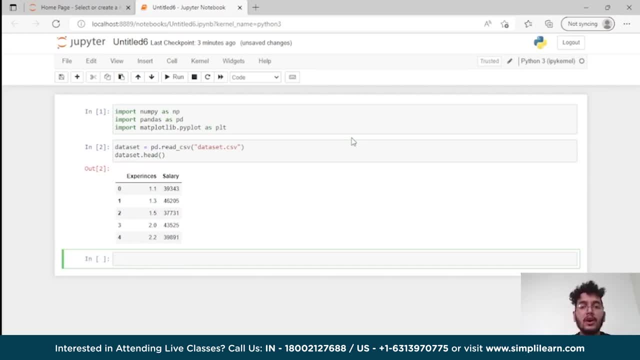 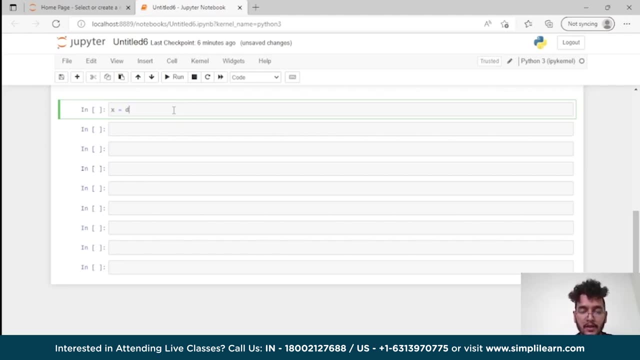 Here head is used for retrieving the first five lines from the data. So our data is coming properly. So moving ahead now, let's first define x and y axis. For x we have to write: x equals to dataset, dot, iloc, bracket, colon, comma, colon, again minus. 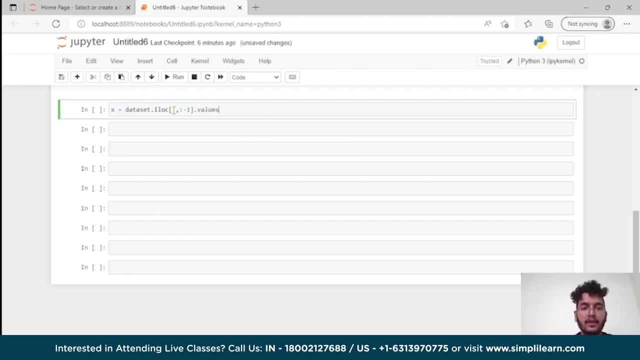 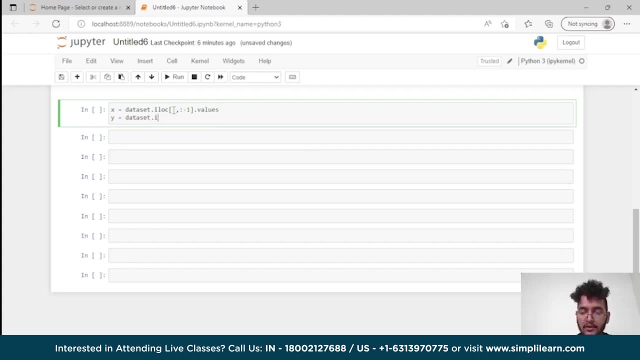 one dot values For x axis and for y axis we have to write: y equals to dataset dot iloc bracket colon comma one dot values. So if we will use dataset dot iloc bracket, colon, comma one dot values, Then we will use dataset dot iloc values for minus one values for x axis. 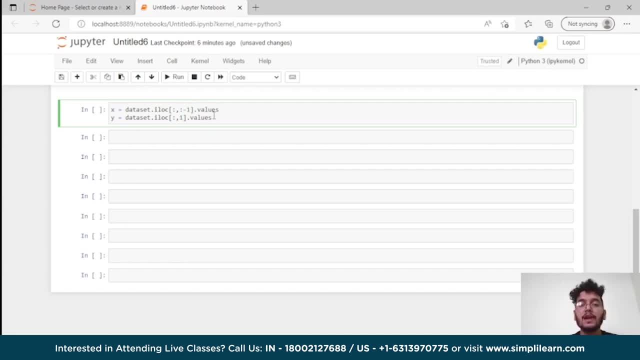 It will select till the second last column of the data frame instead of the last column, And I know this is as the second last column value and the last column value for the row is different, Whereas if we will use for the y axis values return a series vector. 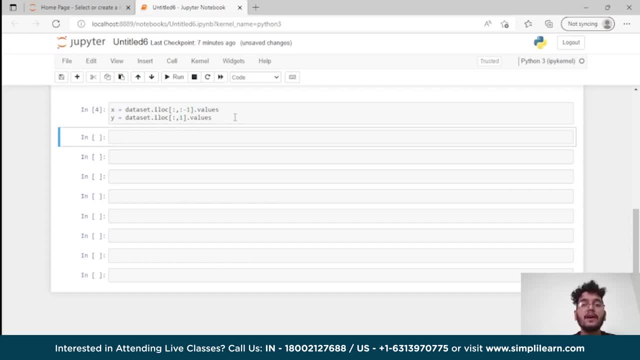 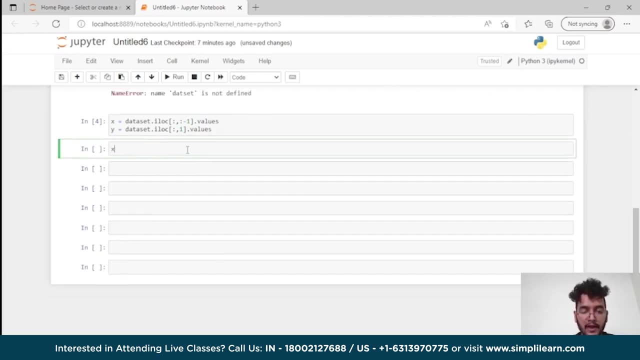 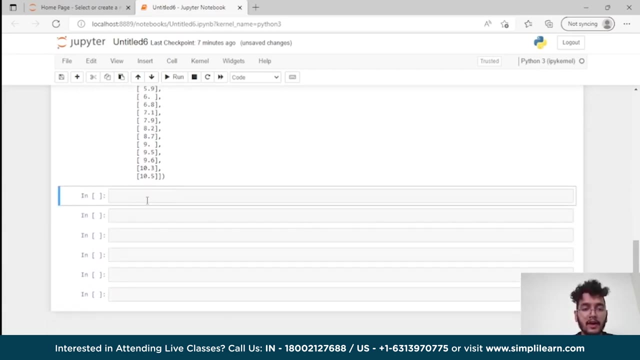 A vector does not have a column size. So, moving ahead, let's see the value for x and y axis. First we will see the value for x Like this: You have to write x equals to dataset, dot, iloc and press enter. So these are the arrays value for X and for Y axis you have to type Y and. 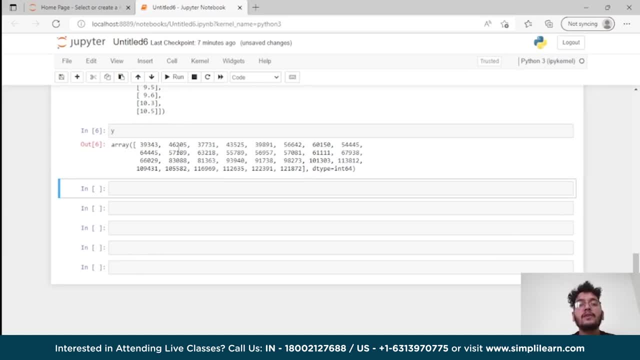 then enter. So these are arrays. value for Y axis. So after this, now let's split the data set into training and testing. Separating data into training and testing set is an important part for evaluating data mining models. Typically, when you separate a data set into a training. 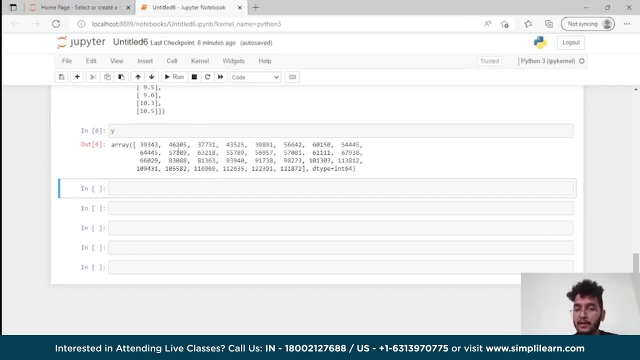 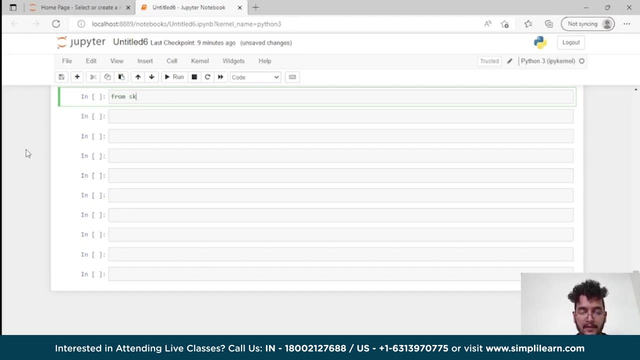 set and a testing set. most of the data set is used for training and a similar portion of data set is used for testing. So we will split it into 70 and 30 ratio. So for splitting we need to import some more libraries for this process, So we will write from sklearnmodel. 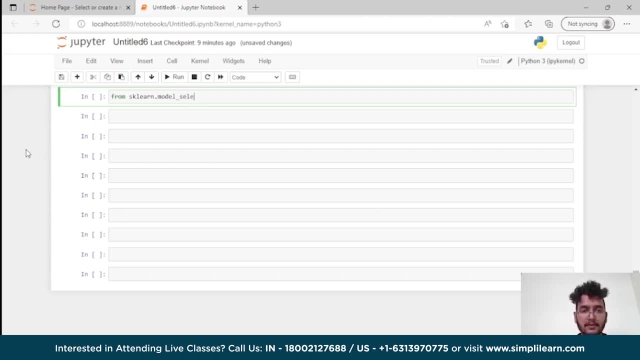 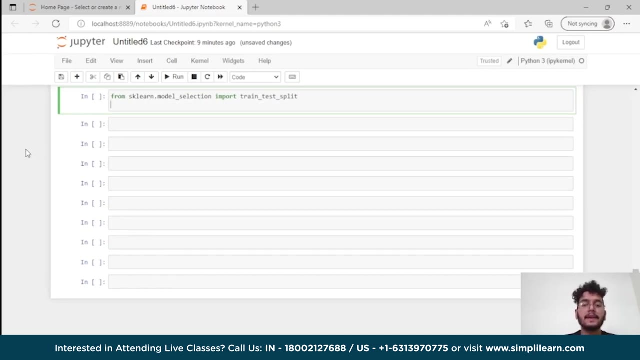 underscore selection, selection, import, train, Underscore test, underscore split. Scikit-learn, like sklearn, is most useful and robust library for machine learning in Python. It provides a selection of efficient tools for machine learning and statistical modeling, including classification, regression and clustering. 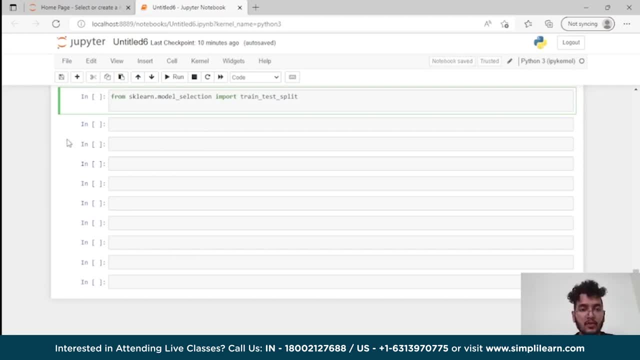 So after importing let's write code for the splitting data. So we will write here: X- underscore test. comma X underscore test. comma Y underscore train comma Y- underscore test. First, to train underscore test underscore split In brackets, we have to write X comma. 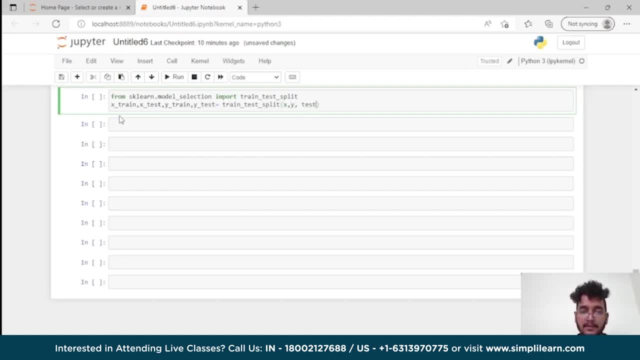 Y comma test underscores underscore split. So we have to write X comma. Y comma. test size equals to 0.3, comma random underscore state equals to zero. With random state equals to zero, we get the same train and test sets across different execution. So after this: 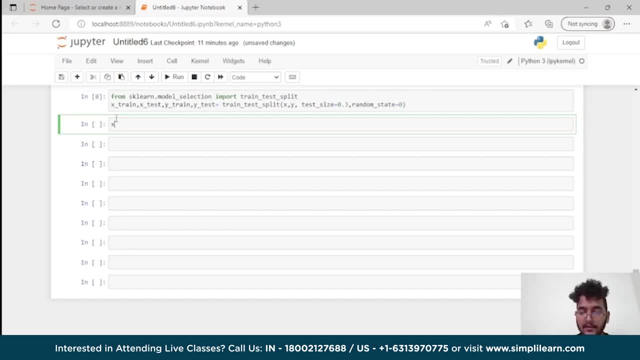 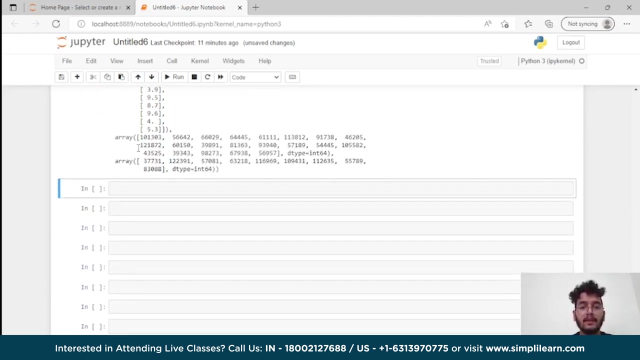 let's see the values together. So we will write X- underscore train. comma X underscore test. comma Y underscore train, comma Y underscore test. So these are the values of array X and array Y together. Moving ahead now let's work with. 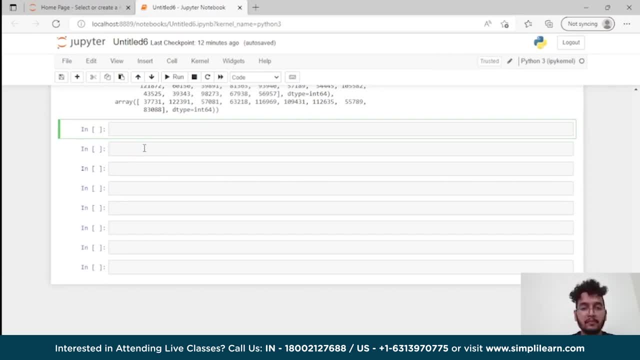 regression. First we need to import the library for regression. So we will use from, let's say, sklearn dot linear underscore model model. import linear regression. We already discussed sklearn is used for machine learning and linear regression. It's a major part of 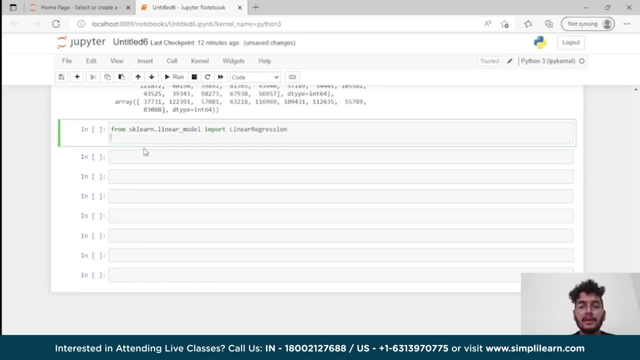 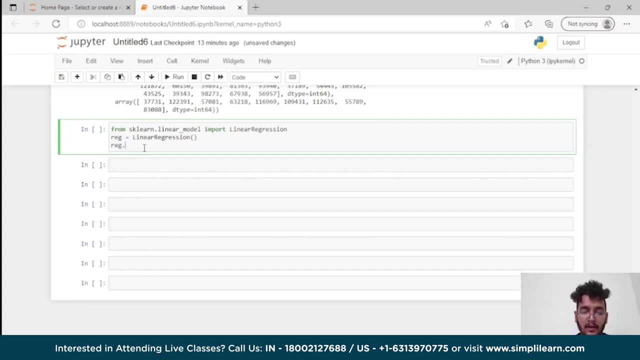 machine learning. So after this let's make a function for regression as rag, for easy use. So let's write: reg equals to linear regression and brackets. First we try to train and then test and compare. So we will write here: reg dot bit, bracket X, underscore train comma. 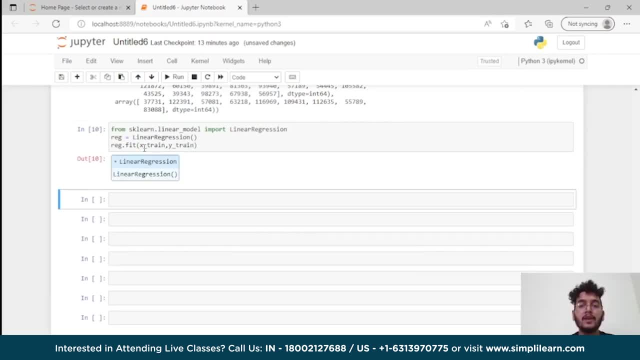 Y underscore train. Okay, Now let's predict values. but prediction values are always different, So we will predict values for Y first. So we will write Y underscore: predict equals to reg, dot predict. Sorry, predict X underscore test. So like Y underscore predict, dot predict, So we will write Y underscore. 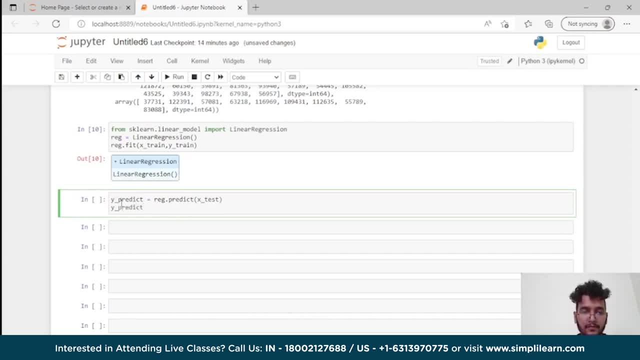 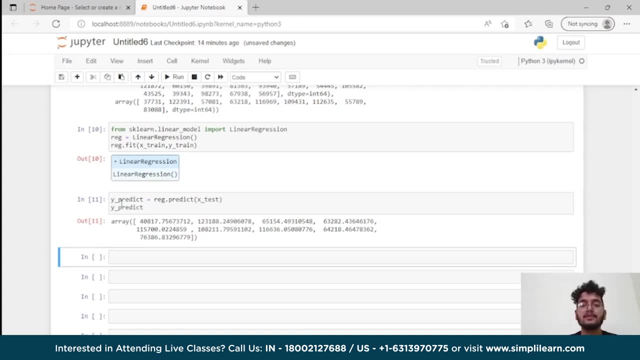 test. This is when the predict functions come into the picture. Python predict function enables us to predict the labels of the data values on the basis of training model. The predict function accept only a single argument, which is X underscore test here usually the data. 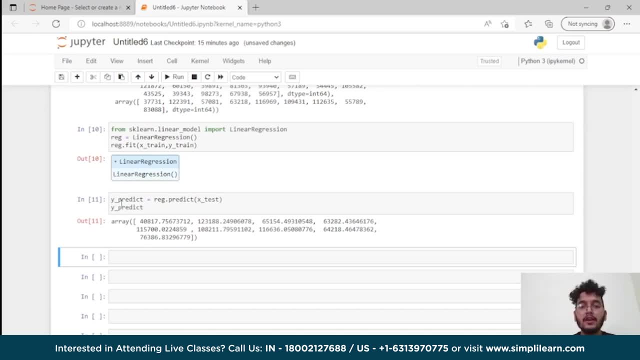 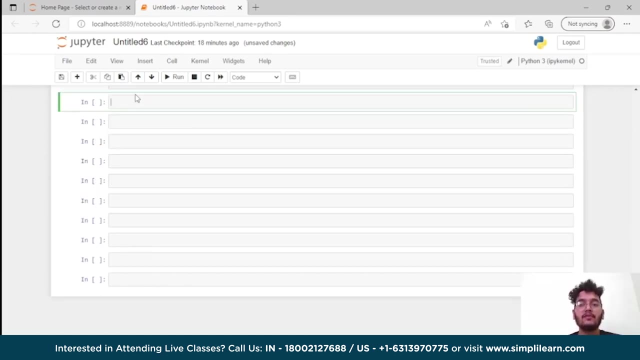 to be tested. So when you will check the value for Y test, you will see the different values like Y underscore test. Okay, Okay, Okay. So you can see there are totally different values from X axis. Now let's display on graph: 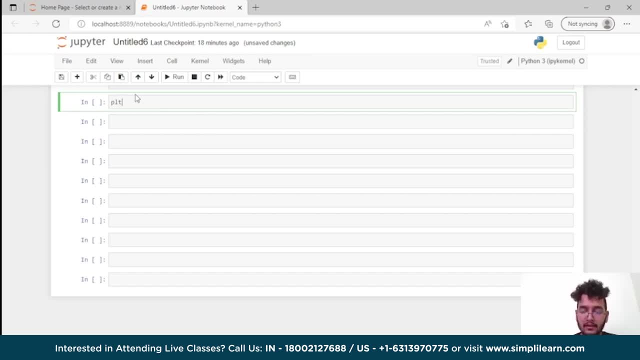 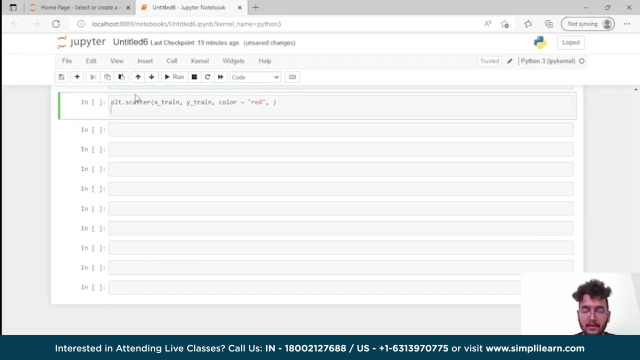 for training dataset. So we have to write PLT dot scatter X underscore train comma. Y underscore train comma. color equals to: you can choose by yourself. I will choose red, Okay, Okay, Okay, Okay, Okay. And then we have PLT dot plot X underscore train comma. regression point for predicting. 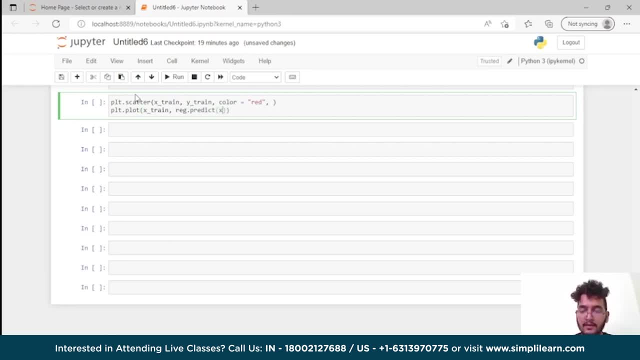 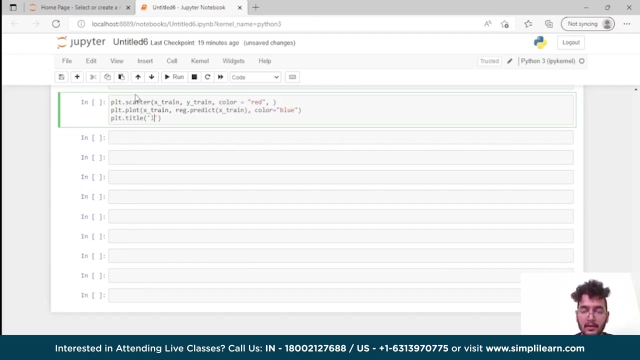 values for X underscore train. comma color equals to blue, So predict value. here we will say this is X underscore train. Okay, Okay, Okay, Okay. so this color is for the regression line and the plt dot title: linear regression: salary versus experience. 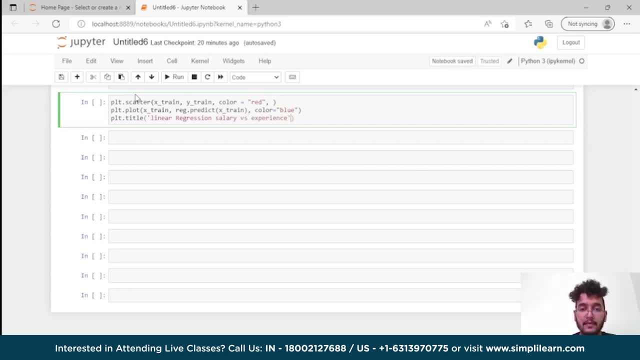 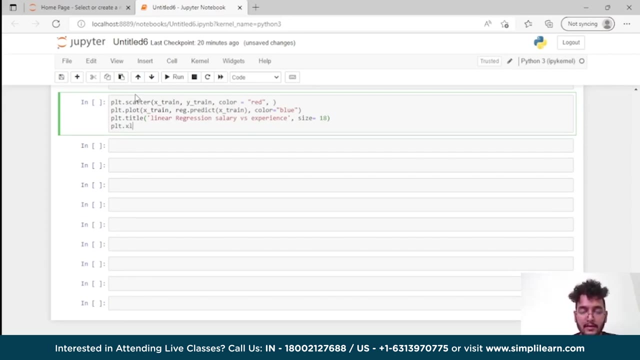 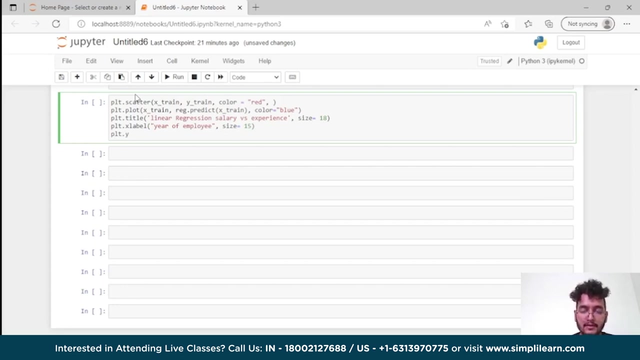 and i will prefer this size would be 18.. so let's set the labels for x and y axis. so x label- year of employee of employee, comma size will be. i will prefer size will be 50.. then for y-axis, we will write here: 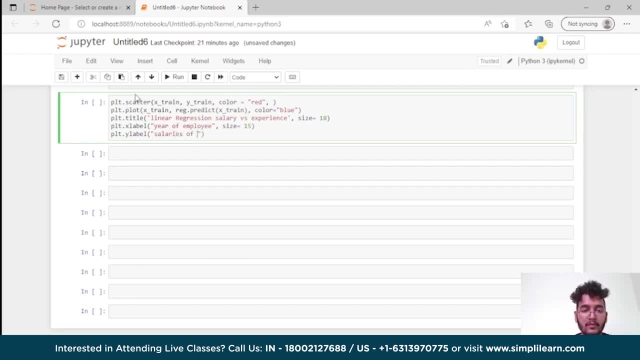 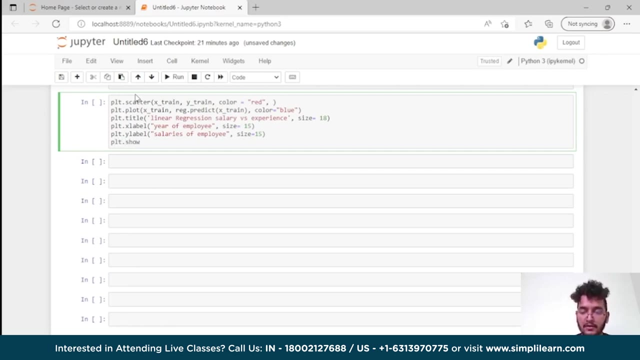 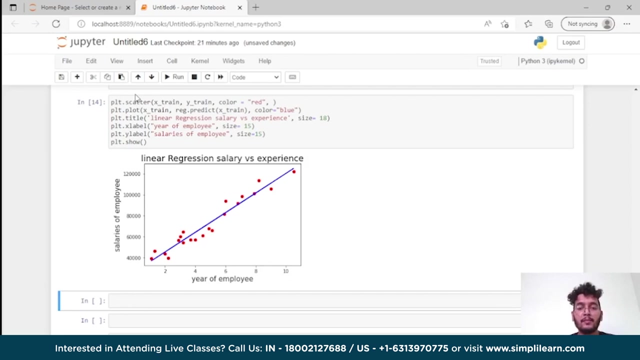 write salaries of, and i will prefer this same size, 15.. let's show the plot by writing pltshow. then hopefully we are fortunate, everything is going to be fine, perfect. so you can see we have linear regression line fitting through our data set. so this is how the linear regression work for training data set. 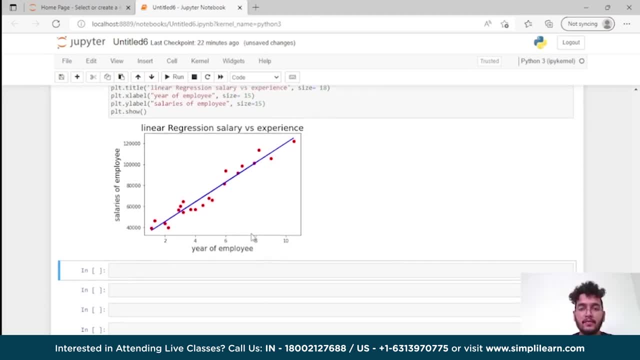 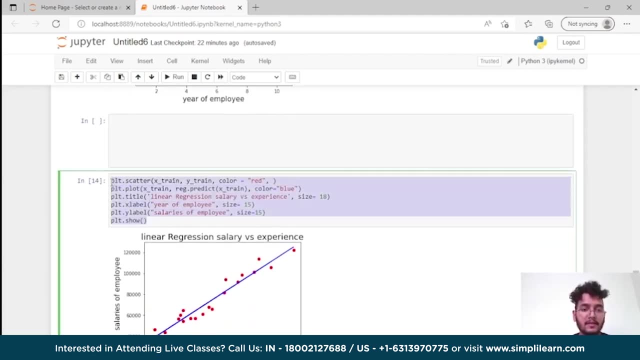 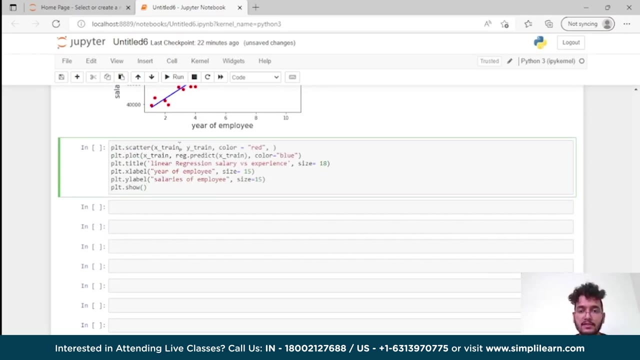 let's see how it will work for testing data set. now let's predict what test data set you can copy for the same and like you can change it. so we can copy here, so we can paste here, so we have to just change here: train to test data set. 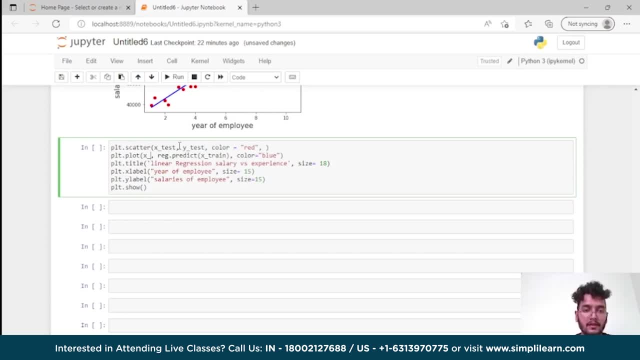 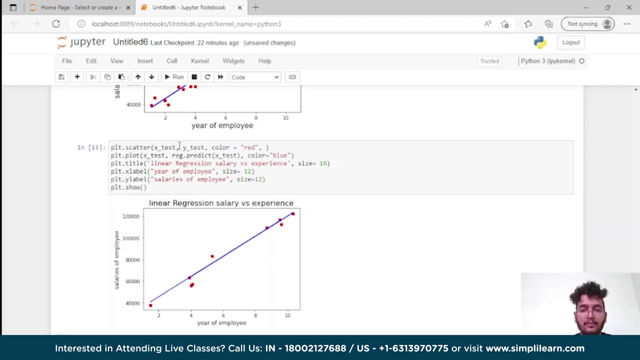 test here, then again test here, then again test here, everything, everything. we will reduce some size to 16, let's see. then it will reduce 12 and so perfect. so you can see, we have linear regression line fitting through our data set. so this is how the linear regression works for testing data set. 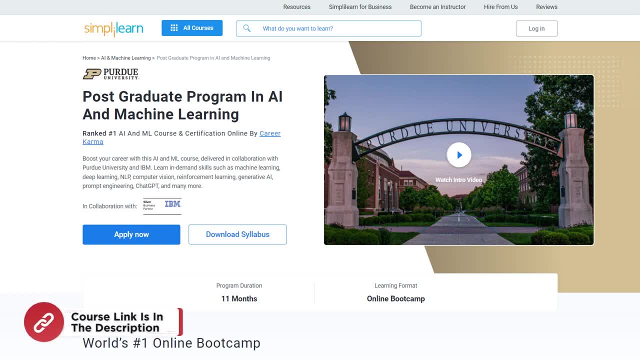 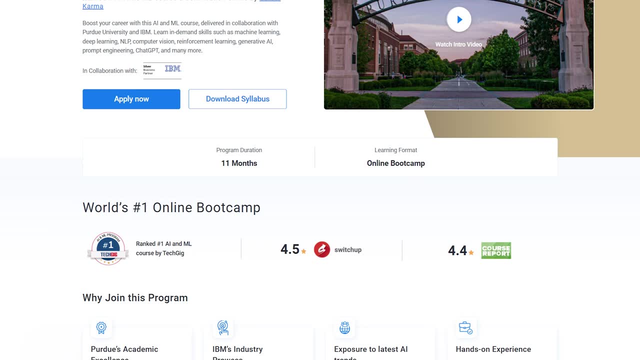 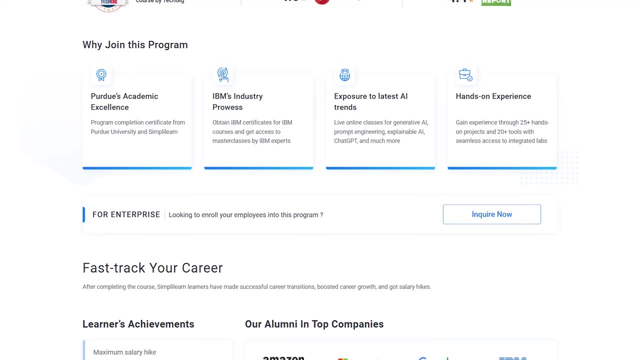 if you're looking for a course that covers everything from the fundamentals to advanced techniques, then accelerate your career in ai and machine learning with a comprehensive postgraduate program in ai and machine learning. boost your career with this ai and ml course, delivered in collaboration with the purview university and ibm. learn in demand skills such as machine learning. 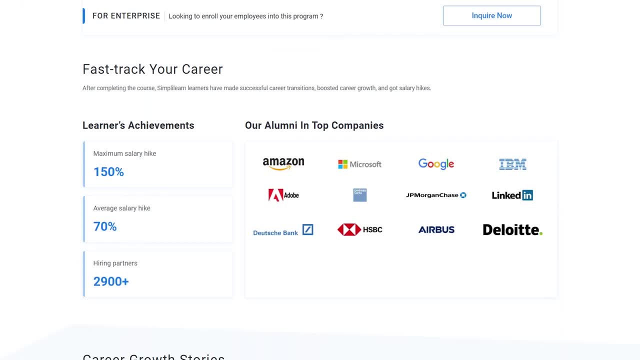 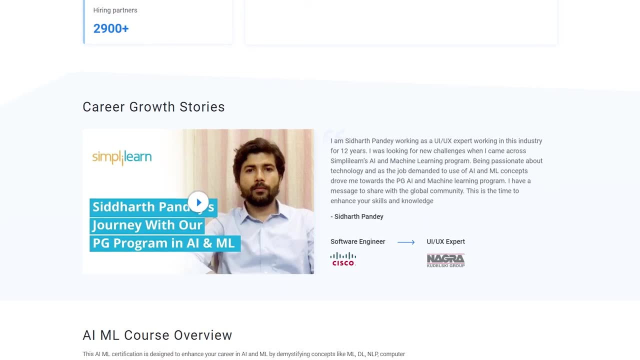 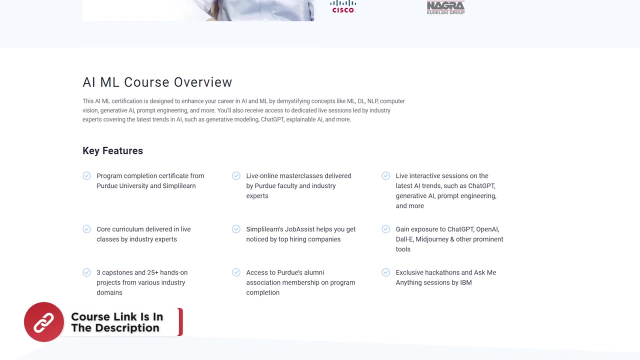 deep learning, nlp, computer vision, reinforcement learning, generative, ai, prompt, engineering, chat, gpt and many more. you'll receive a prestigious certificate and ask me anything. sessions by ibm with five capstones in different domains, using real data sets. you will gain practical experience. master classes by purdy faculty and ibm. 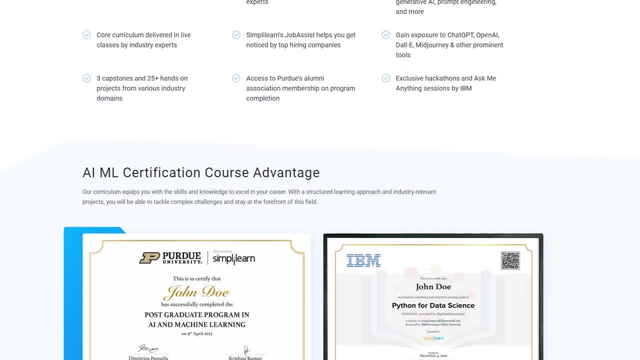 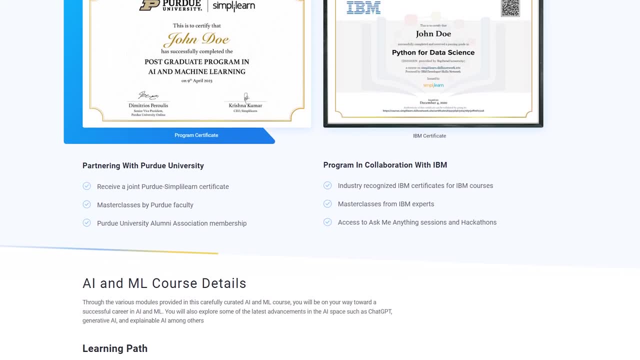 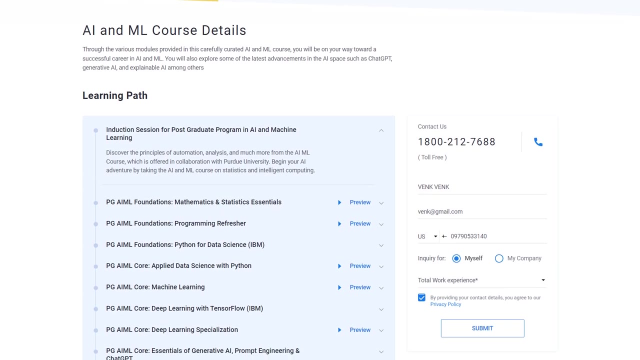 experts ensure top-notch education. Simply Learn's job assist: help you get noticed by leading companies. This program covers statistics, Python, supervised and unsupervised learning, NLP, neural networks, computer vision, GANs, Keras, TensorFlow and many more such skills. Admission to this postgraduate. 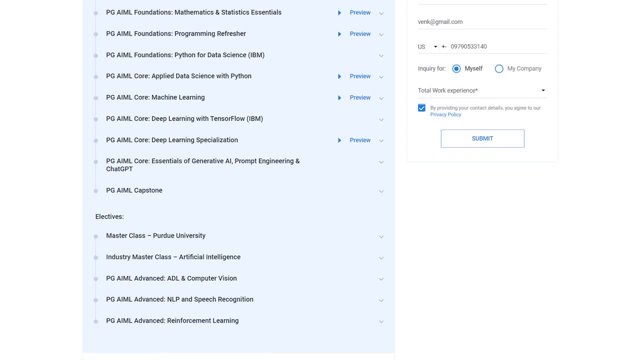 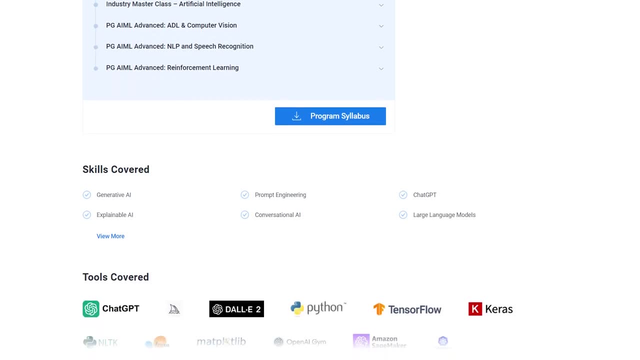 program in AI and machine learning requires a bachelor's degree with an average of 50% or higher marks, along with the basic understanding of programming concepts and mathematics, And candidates with two plus years of work experience are preferred to enroll in this school. So enroll now and unlock. 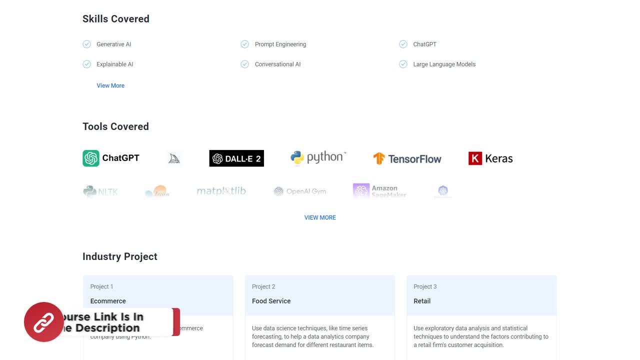 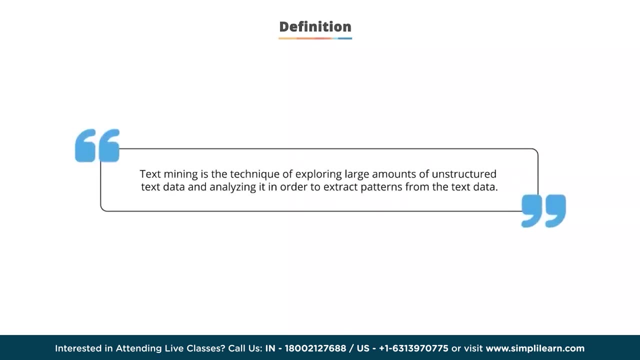 exciting AI and machine learning opportunities. The link is mentioned in the description box below. Let's first understand what text mining is. Text mining is the technique of exploring large amounts of unstructured text data and analyzing it in order to extract patterns from the text data. It is aided. 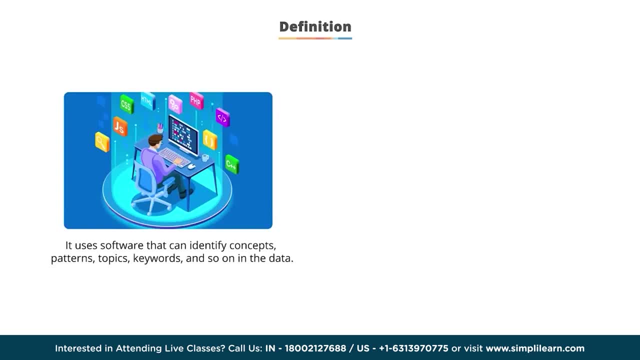 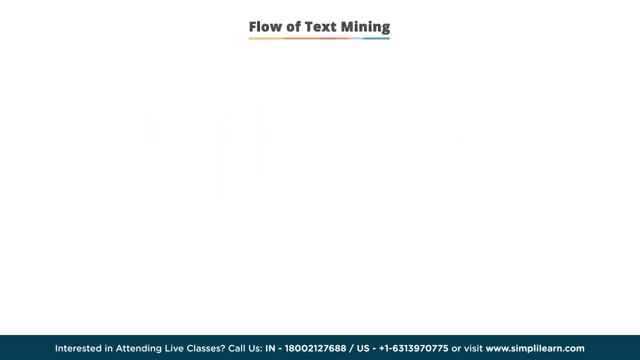 by software that can identify concepts, patterns, topics, keywords and other attributes in the data. It utilizes computational techniques to extract and summarize the high-quality information from unstructured textual resources. Let's understand the flow of text mining. There are five techniques used in text mining system: Information extraction or text. 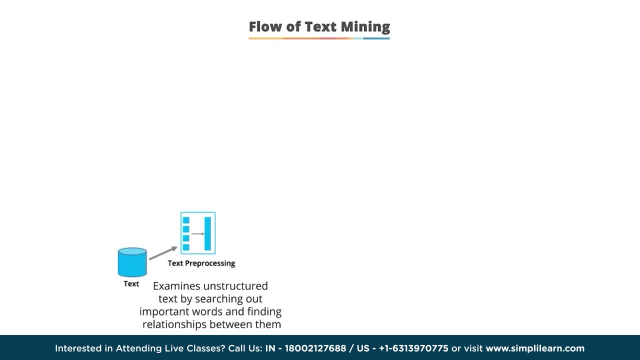 pre-processing. This is used to examine the unstructured text by searching out the important words and finding the relationships between the text and the words used to implement it. çocuklar-lovak alakali between them. Categorization or text transformation, attribute generation, Categorization technique. 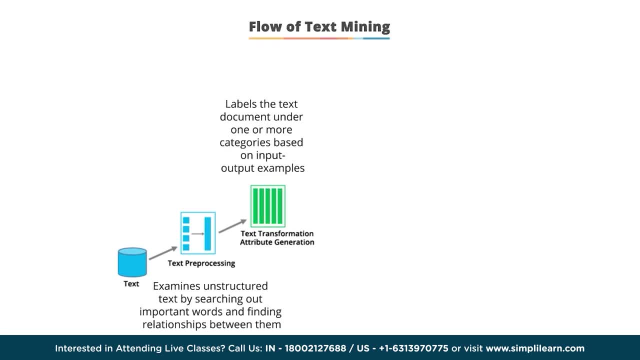 labels the text document under one or more categories. Classification of text data is done based on input-output examples, with categorization, Clustering or attribute selection. Clustering method is used to group text documents that have similar content. Clusters are the partitions and: 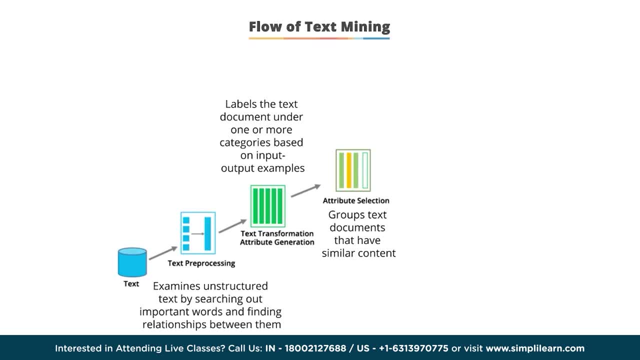 each cluster will have a number of documents with similar content. Clustering makes sure that no document will be omitted from the search and it derives all the documents that have similar content. Visualization technique: The process of finding relevant information is simplified by visualization technique. This technique uses text flags to represent a group of documents. 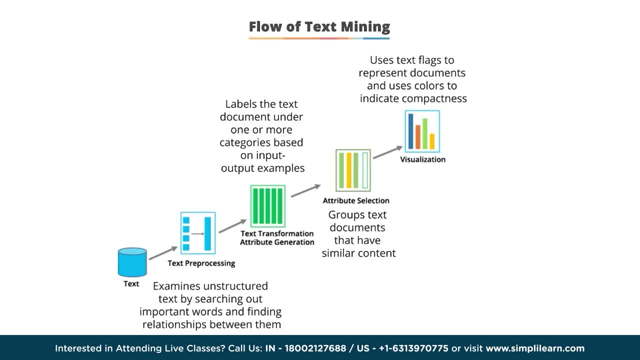 or a single document, and compactness is indicated using colors. Visualization technique: Visualization technique helps to display textual information in a more attractive way. Summarization or interpretation or evaluation: Summarization technique will help to reduce the length of the document and summarize the details of the documents. It makes the document easy to 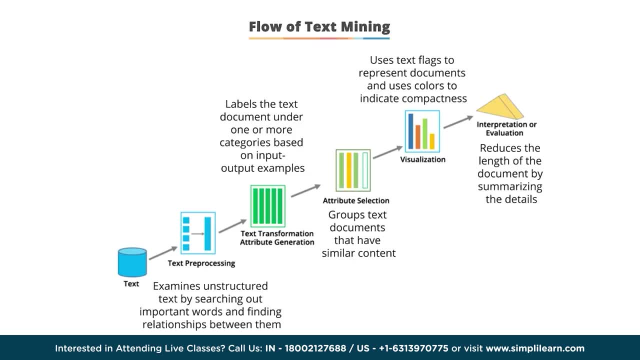 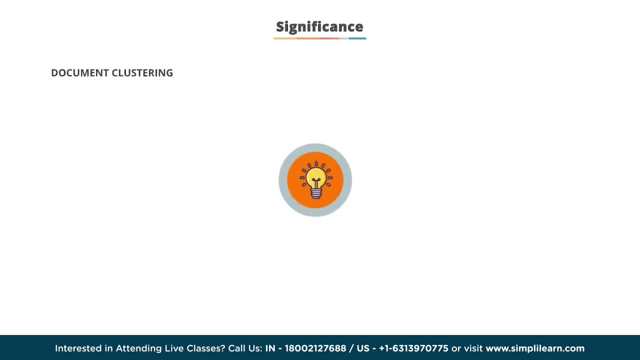 read for users and understand the content at the moment. Let's understand the significance of text mining, Document clustering. Document clustering is an important part of text mining. It has many applications in knowledge management and information retrieval. Clustering makes it easy to group similar documents into meaningful groups. 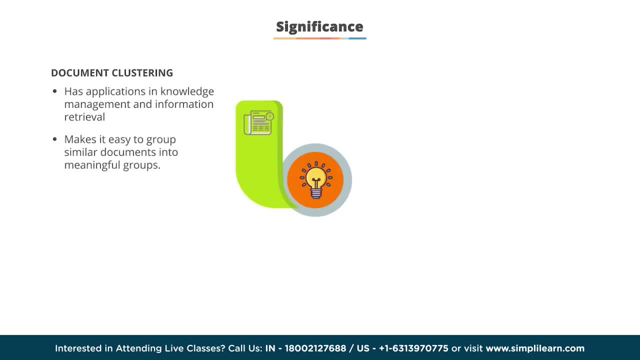 such as in newspapers, where sections are often grouped as business, sports, politics and so on. Pattern identification- Text mining is the process of automatically searching large amount of text for text, patterns and recognition of features. Features such as telephone numbers and email addresses can be extracted from text mining. Text mining is the process of automatically searching large amount of text for text, patterns and recognition of features. Features such as telephone numbers and email addresses can be extracted from text mining. 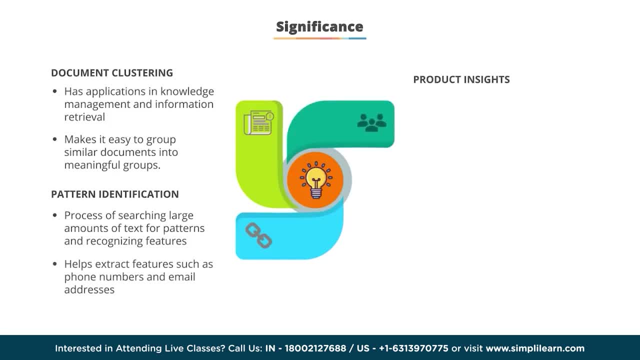 using pattern matches, Product insights. Text mining helps to extract large amounts of text, for example, customer reviews about the products. Mining consumer reviews can reveal insights like most loved feature, most hated feature, improvements required and reviews of competitors' products. 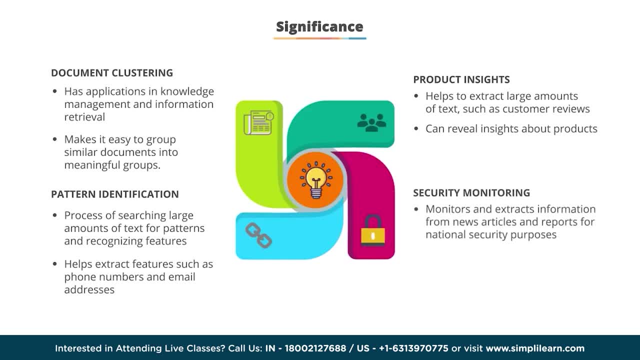 Security monitoring. Text mining helps in monitoring and extracting information from news articles and reports for national security purposes. Text mining makes sure to use all of your available information. It is a more effective and productive knowledge discovery that allows you to make better informed decisions. automate information-intensive processes. 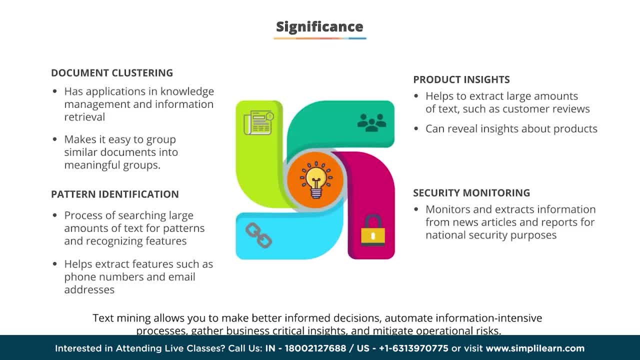 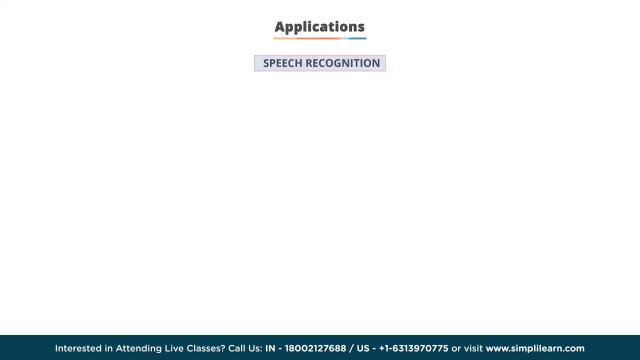 gather business-critical insights and mitigate operational risk. Let's look at the applications of text mining, Speech recognition. Speech recognition is a tool that allows you to identify and identify and identify information. Speech recognition is a tool that allows you to identify and identify and identify information. 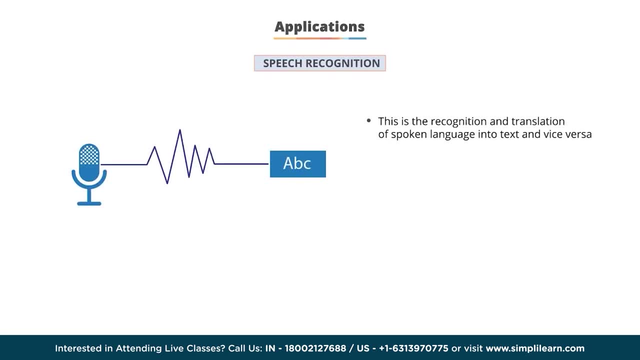 Speech recognition is the recognition and translation of spoken language into text and vice versa. Speech often provides valuable information about the topics, subjects and concepts of multimedia content. Information extraction from speech is less complicated, yet more accurate and precise than multimedia content. This fact motivates content-based speech analysis for multimedia. 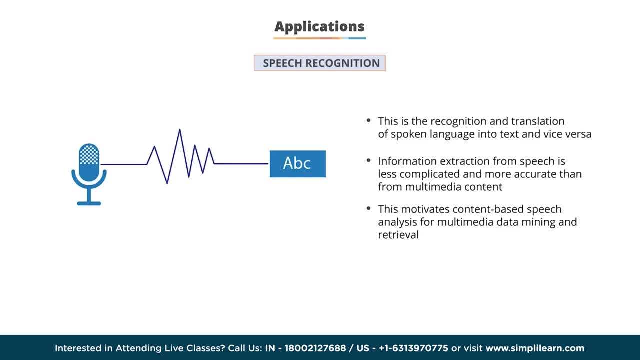 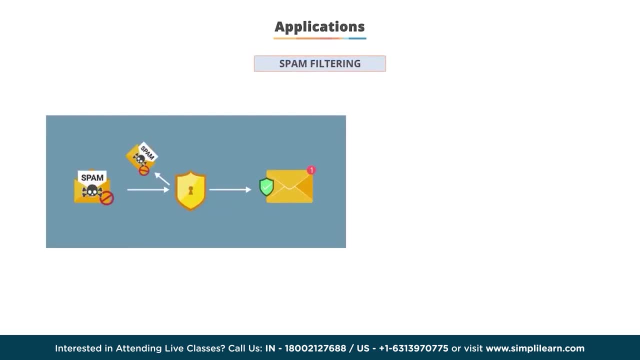 data mining and retrieval, where audio and speech processing is a key enabling technology. Spam filtering: Spam detection is an important method in which textual information contained in an email is extracted and used for discrimination. Text mining is useful in automatic detection of spam emails based on the filtering content Using text mining an email service provider such as Gmail. 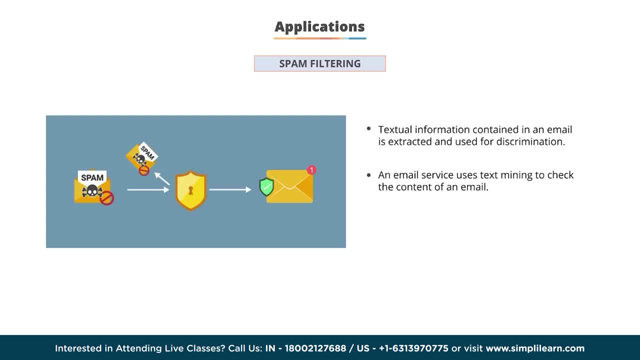 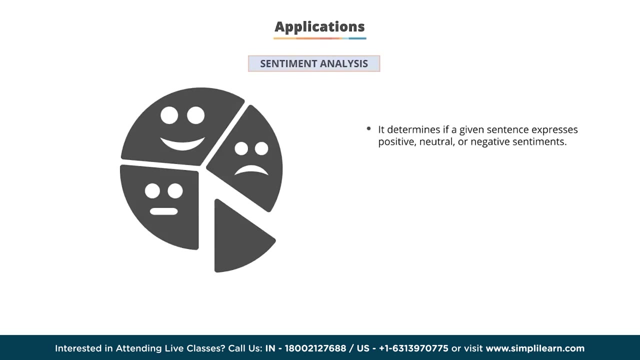 or Yahoo Mail checks the content of an email and if some malicious text is found in the mail, then that email is is marked as spam and sent to the spam folder. Sentiment Analysis: It is done in order to determine if a given sentence expresses positive, neutral or negative sentiments. 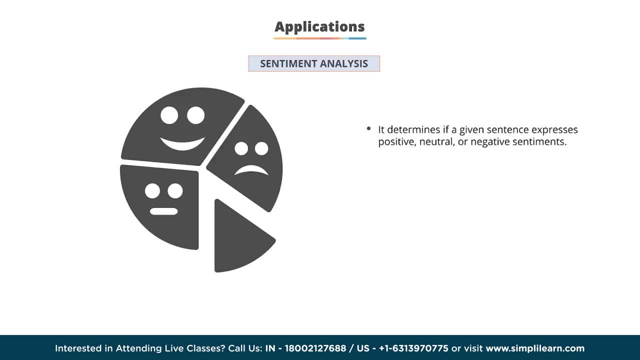 Sentiment analysis is one of the most popular applications of text analytics. The primary aspect of sentiment analysis includes data analysis of the body of the text for understanding the opinion expressed by it, and other key factors comprising modality and mood. Usually, the process of sentiment analysis works best. 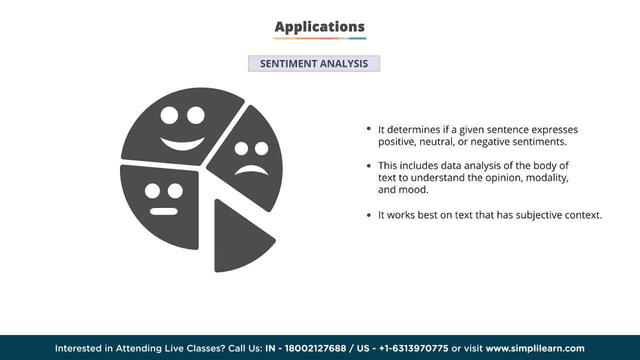 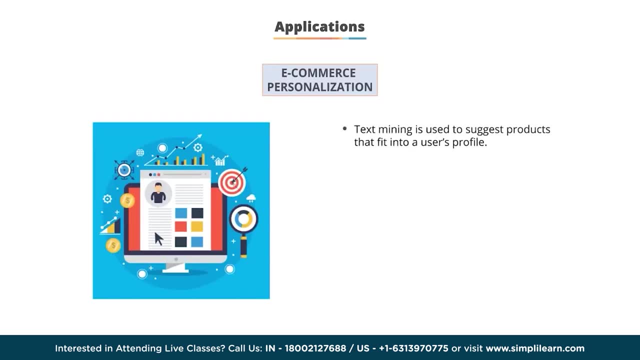 on text that has a subjective context than on that with only an objective context. E-commerce Personalization: Text mining is used to suggest products that fit into a user's profile. Text mining is increasingly being used by e-commerce retailers to learn more about the consumers. 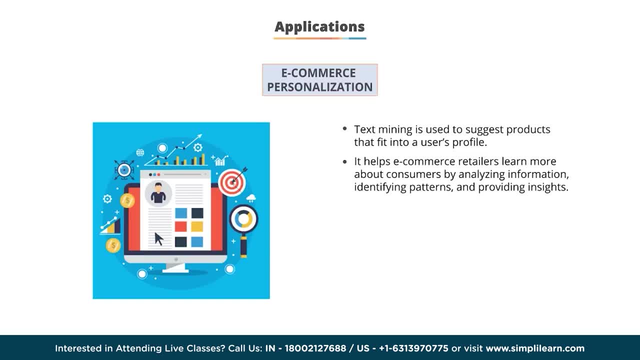 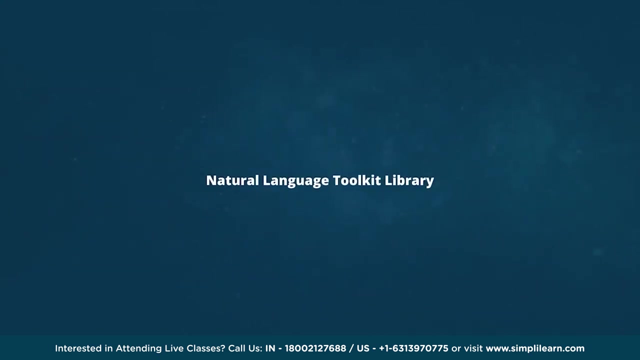 as it is the process of analyzing textual information in order to identify patterns and gain information. E-commerce retailers can target specific individuals or segments with personalized offers and discounts to boost sales and increase customer loyalty by identifying customer purchase patterns and opinions on particular products. Let's look at Natural Language Toolkit library in detail. 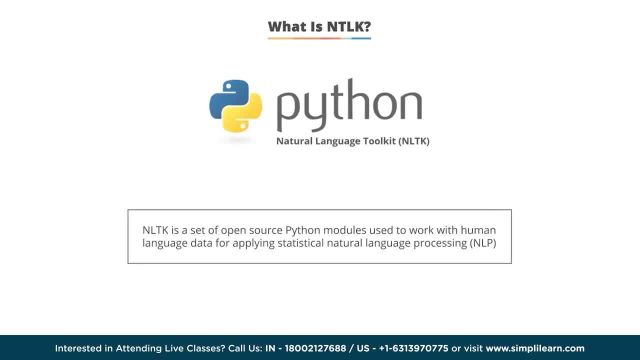 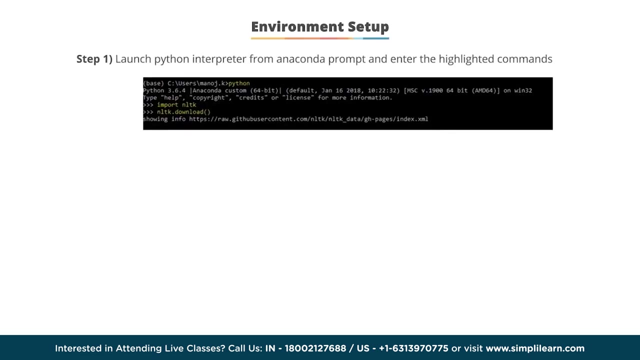 Natural Language Toolkit is a set of open-source Python models that are used to apply statistical natural language processing on human language data. Let's see how you can do. environment setup of NLTK. Go to Windows Start and launch Python interpreter from Anaconda prompt and enter the following commands: 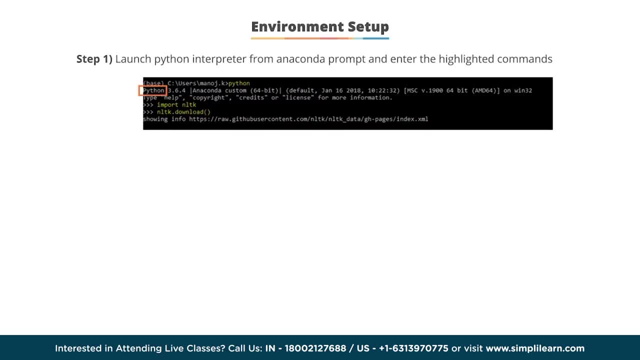 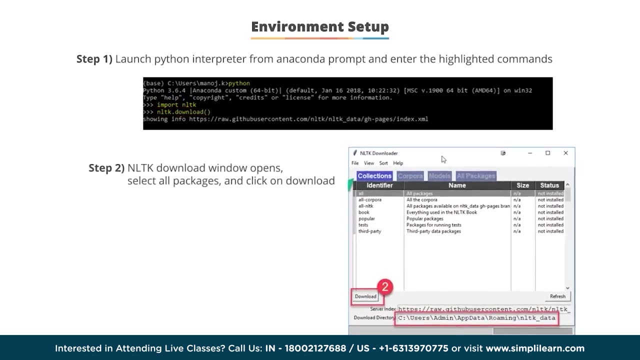 Enter command Python to check the version of Python installed on your system. Enter import NLTK to link you to the NLTK library available to download. Then enter nltkdownload function that will allow you to download the NLTK library. Open the NLTK download window. check the download directory. 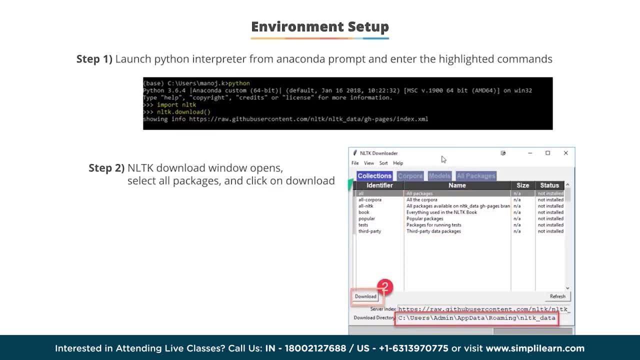 select all packages and click on download. This will download NLTK onto your Python. Once you have downloaded the NLTK, you must check the working and functionality of it. In order to test the setup, enter the following command in Python: idle From nltkcorpus import brown- brownwordcorpusbrown. 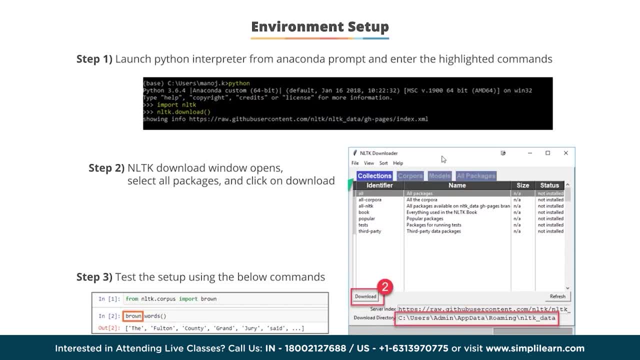 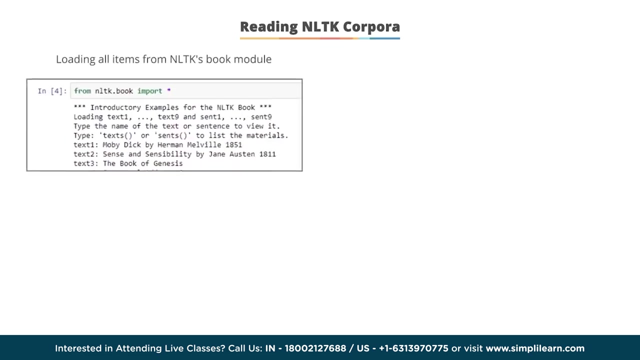 The brown is an NLTK corpus that shows the systematic difference between different genres. available Words function will give you the list of available words in the genre. The given output shows that we have successfully tested the NLTK installed on Python. Let's now understand how you can read a specific module from NLTK corpora. 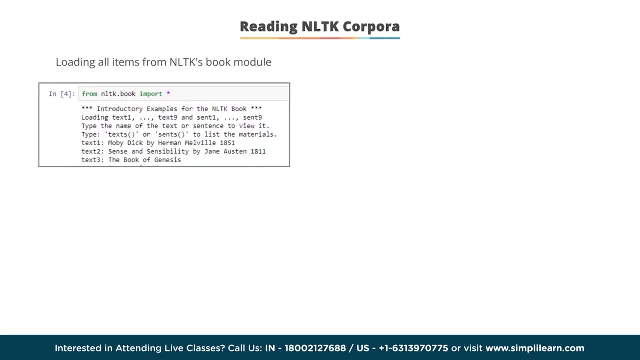 If you want to import an entire module from NLTK corpora, you must import a specific module from NLTK corpora. Use asterisk symbol with that module name: import command. Enter the command from nltkbookimport- asterisk. It will load all the items available in NLTK's book module. 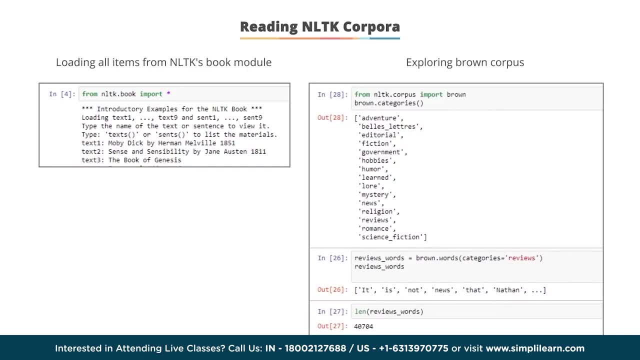 Now, in order to explore brown corpus, enter the command nltkcorpus- import brown. This will import brown corpus on the Python, Enter browncategories function to load all the items available in NLTK's book module. Select a genre and assign that genre to a variable using the following syntax: 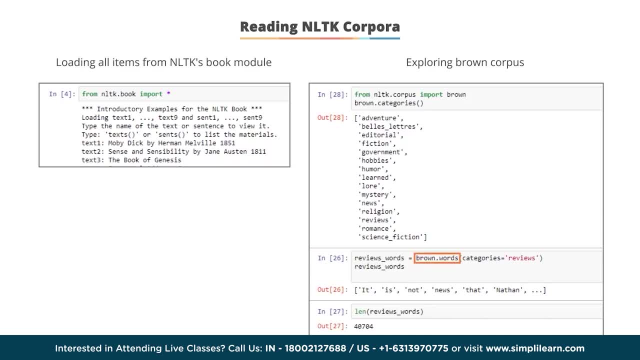 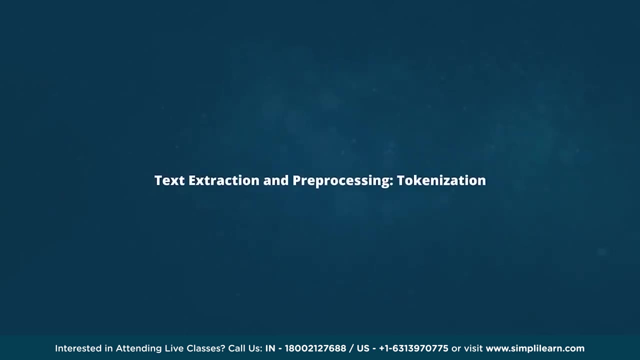 Variable name is equal to brownwords. Categories is equal to genre name. Now, in order to see the available words inside the selected genre, just enter the defined variable name as a command. Let's understand text extraction and pre-processing in detail. So let's first understand the context. 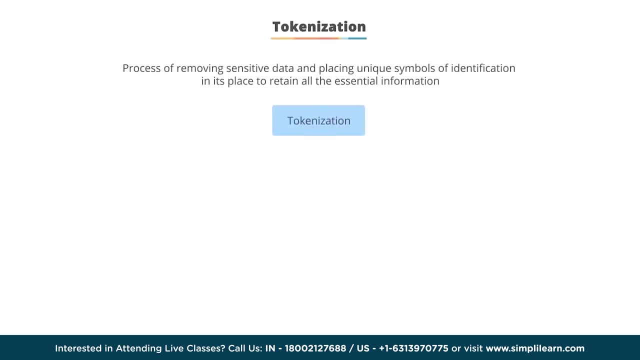 Concept of tokenization. Tokenization is the process of removing sensitive data and placing unique symbols of identification in that place in order to retain all the essential information concerned with the data by its security. It is a process of breaking running streams of text into words and sentences. 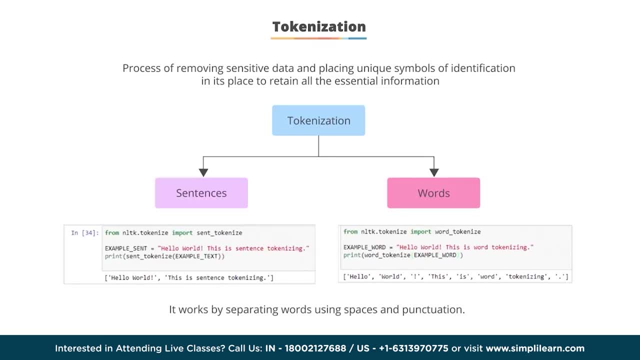 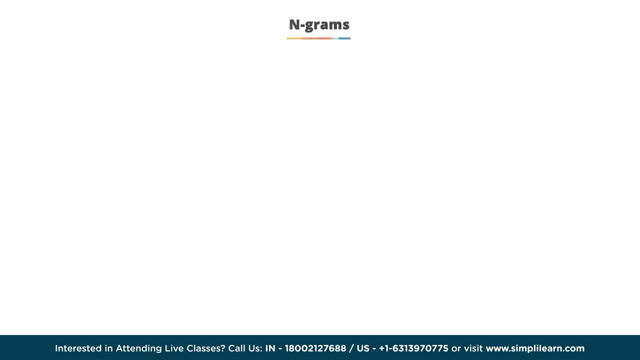 It works by segregating words, using punctuation and spaces. Text extraction and pre-processing Ngrams. Text extraction and pre-processing Ngrams. Text extraction and pre-processing Ngrams. Now let's look at what n-gram is and how it is helpful in text mining. 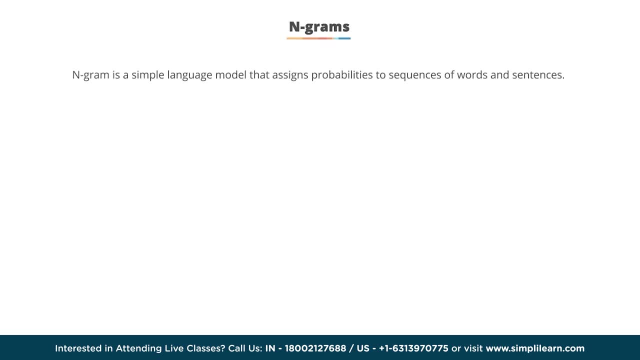 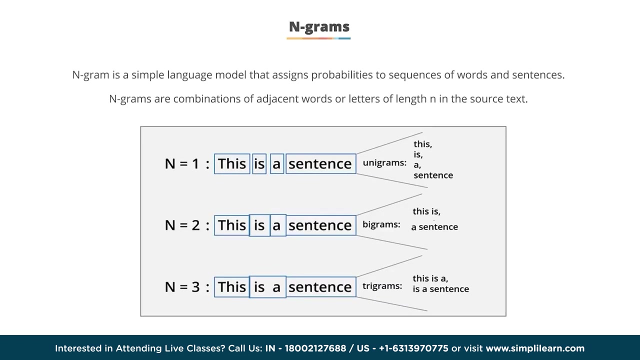 N-gram is the simplest model that assigns these probabilities to sequences of words or sentences. N-grams are combinations of adjacent words or letters of length n in the source text. So n-gram is very helpful in text mining when it is required to extract patterns from the 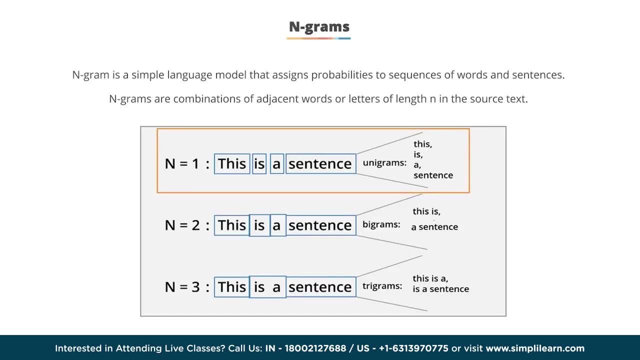 text, As in the given example, this is a sentence. All of these words are considered individual words and thus represent unigrams. A two-gram or bigram is a two-word sequence of words like this is: is a or a sentence. 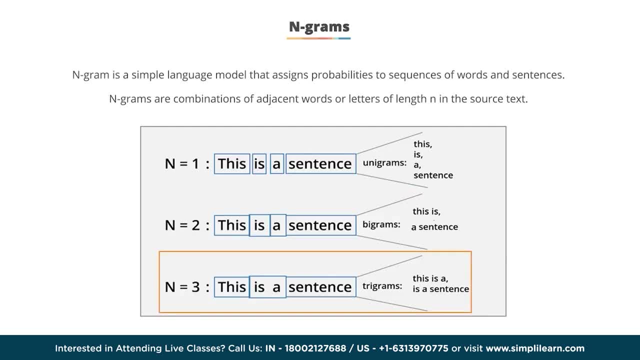 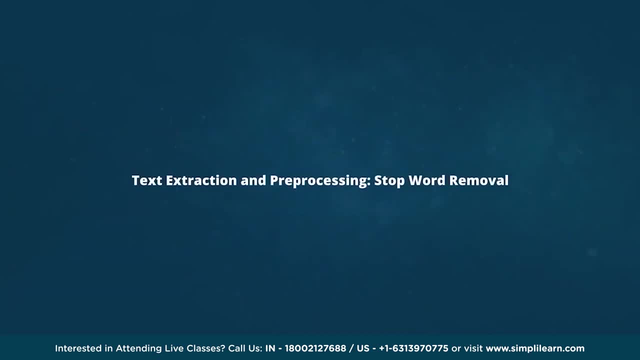 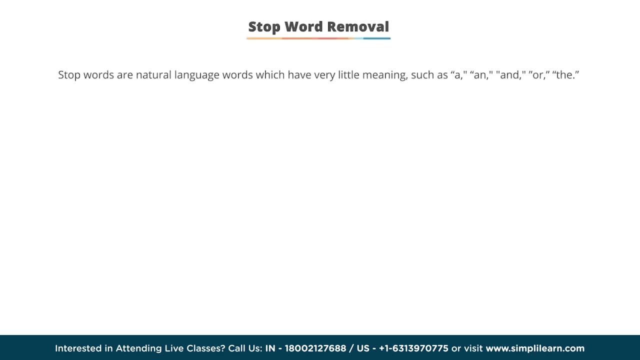 and a three-gram, or trigram, is a three-word sequence of words like this is a or is a sentence. Let's now understand what stop words are and how you can remove them. Stop words are natural language words that have negligible meanings, such as a, an and. 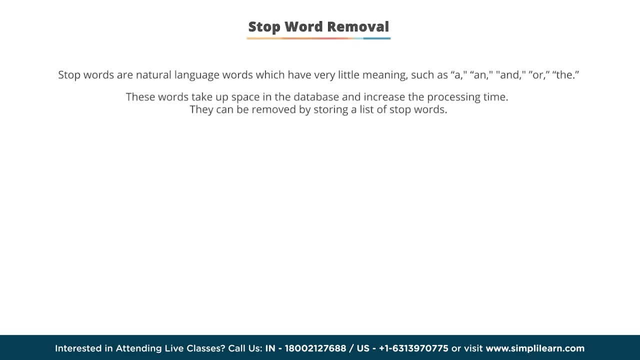 or the and other similar words. These words also will take up space in the database or increase the processing time, so it is better to remove such words by storing a list of stop words. You can find the list of stop words in the NLTK data directory that is stored in 16 different 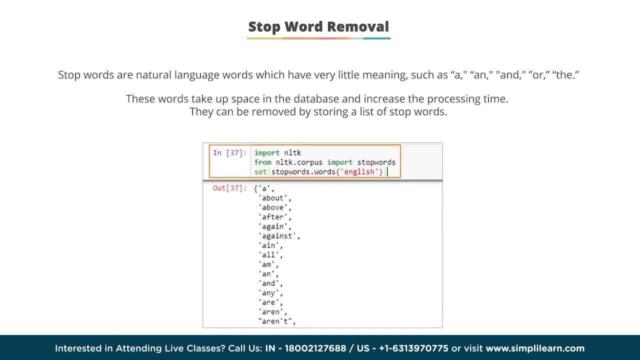 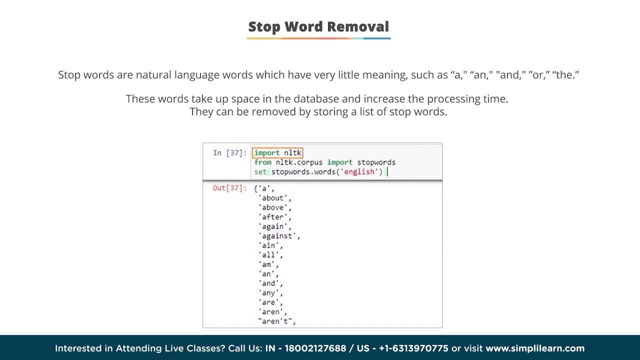 in NLTK corpus. importing NLTK will import the NLTK corpus for that instance. Enter from nltkcorpus. import Stop words will import stop words from NLTK corpus. Now set the language as English, so use set function as set under braces: stop wordswords. 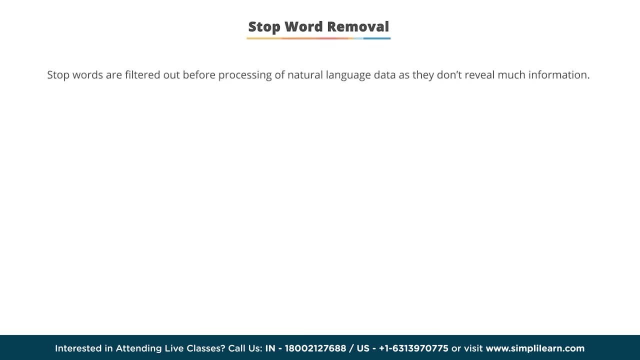 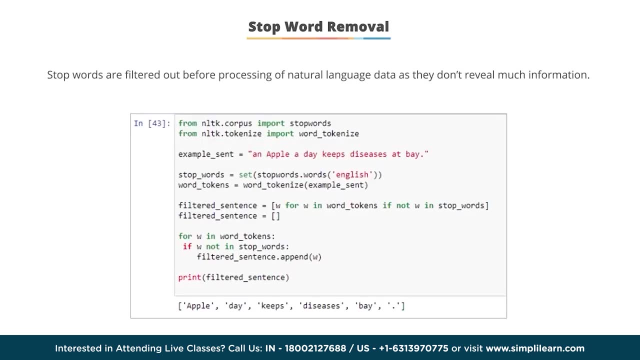 Set genre as English. Stop words are filtered out before processing of natural language data, as they don't reveal much information. So, as you can see in the given example, before filtering the sentence, the tokenization of stop word is processed in order to remove these stop words and the filtering is applied. 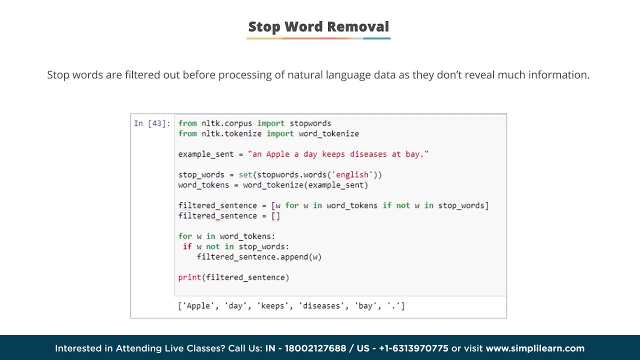 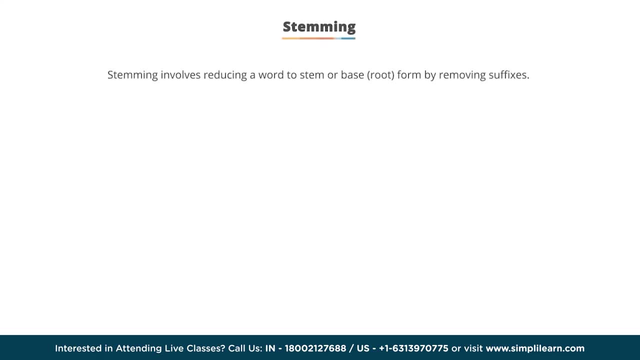 in order to filter the sentence based on some criteria: Text extraction and pre-processing stemming. Stemming is used to reduce a word to stem or base word by removing suffixes such as helps, helping, helped and helper to the root word help. The stemming process or algorithm is generally called a stemmer. 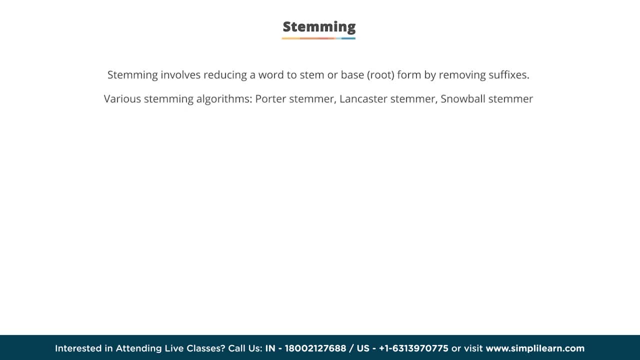 There are various stemming algorithms, such as Porter stemmer, Lancaster stemmer, Snowball stemmer, etc. Use any of the stemmers defined under NLTK stem corpus in order to perform stemming as shown in the example. Here, we have used Porter stemmer. 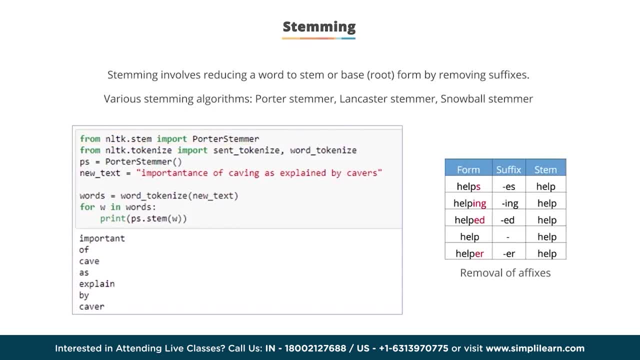 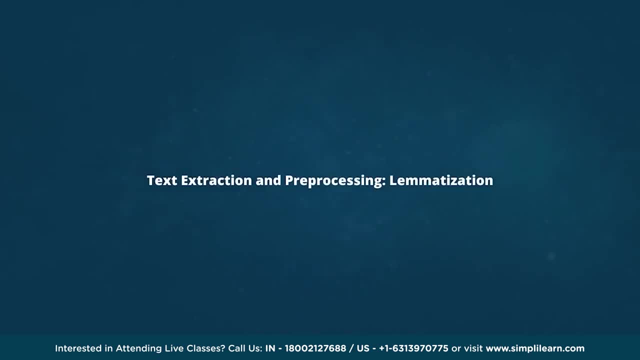 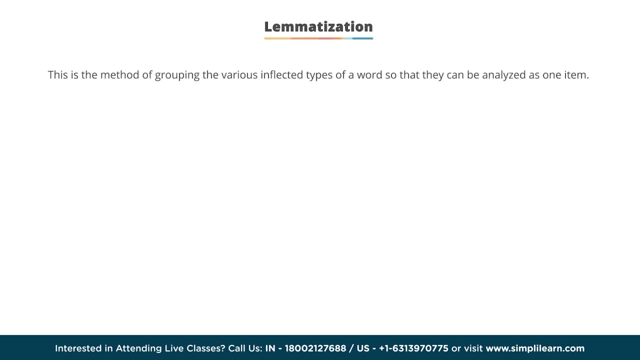 When you observe the output, you will see that all of the words given have been reduced to their root word or stem. Text extraction and pre-processing lemmatization: Lemmatization is the method of grouping the various inflected types of a word in order. 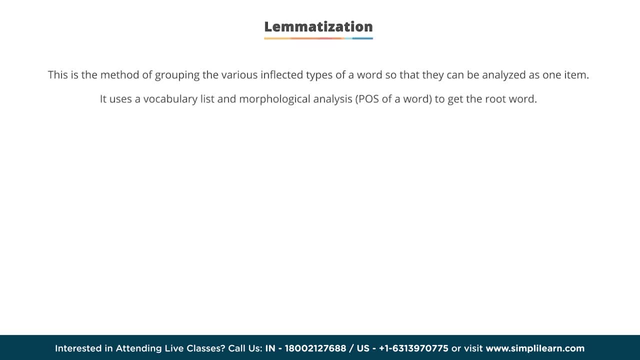 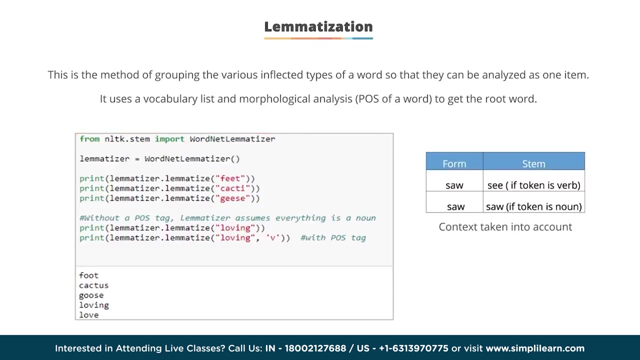 that they can be analyzed as one item. It uses vocabulary list or a morphological analysis to get the root word. It uses WordNetData, The WordNet database that has English words linked together by their semantic relationship. As you can observe the given example, the different words have been extracted to their 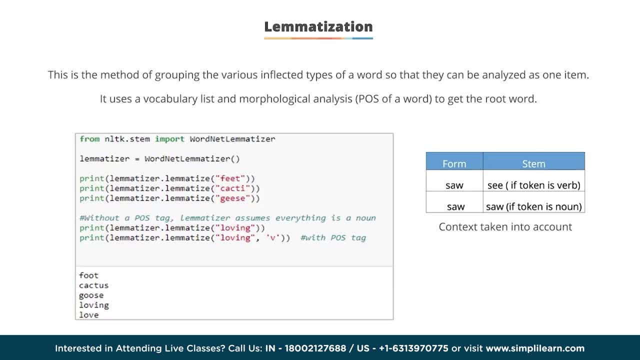 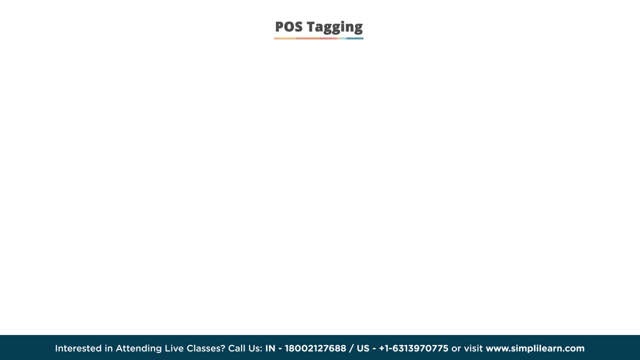 relevant morphological word using lemmatization, Text extraction and pre-processing POS tagging. Let's now look at different part of speech tags available in the National Language Toolkit library. A POS tag. What is a POS tag? POS tag is a special label assigned to each token or word in general. 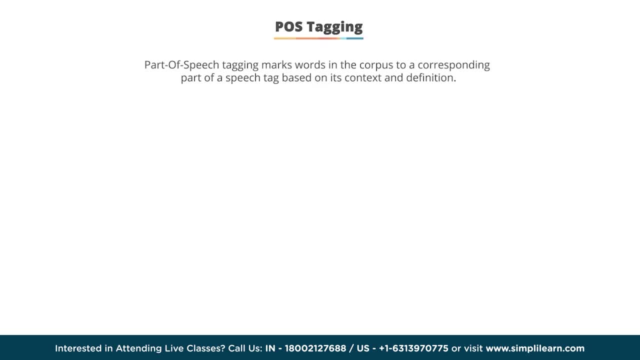 What is a POS tag or word in a text corpus to indicate the part of speech and often also other grammatical categories such as tense, number, case, etc. POS tags are used in text analysis tools and algorithms and also in corpus searches. 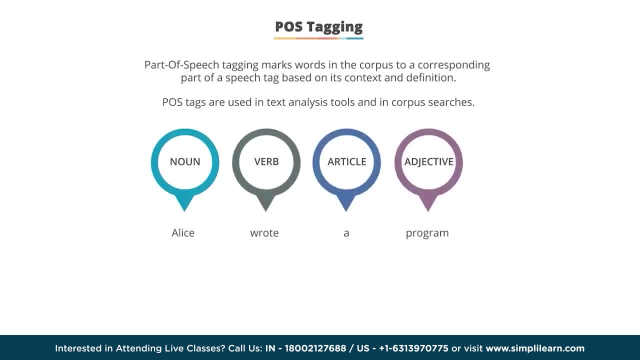 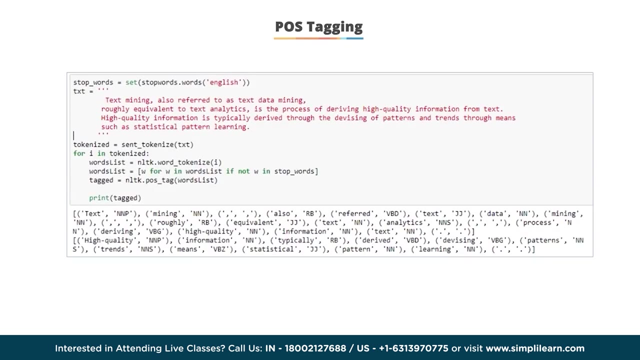 So look at the given example Here. Alice wrote a program is the source text given. The POS tags given are: Alice is a noun, wrote is a verb, a is an article and program is an adjective. Look at the given example to understand how POS tags are defined. 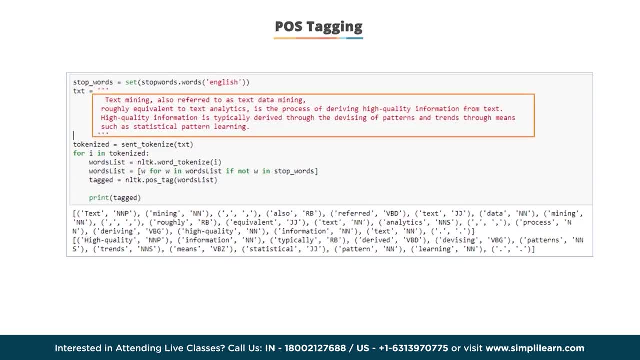 So the given sentence or paragraph contains different words that represent different parts of speech. We will first use tokenization and removal of stop words and then allocate the different POS tags. These are shown with different words in the given sentence. POS tags are useful. 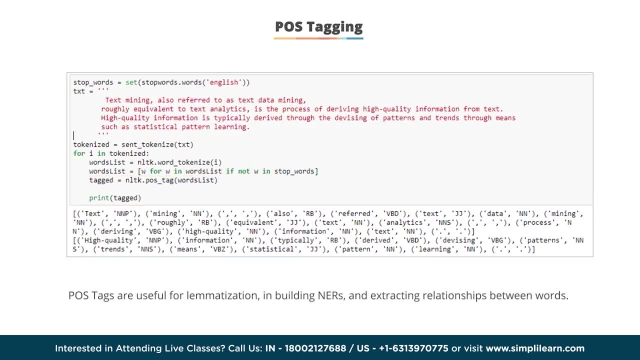 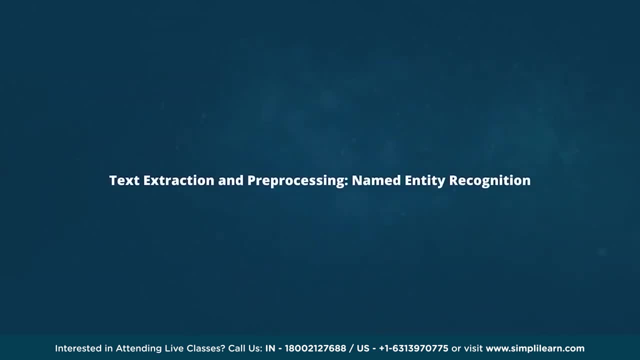 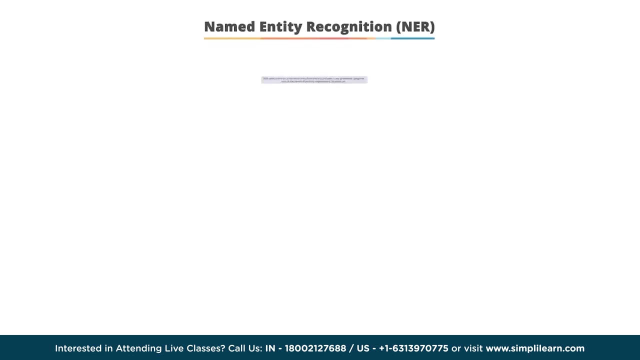 For example, for lemmatization in building named entity recognition and extracting relationships between words, Text extraction and pre-processing named entity recognition. Now let's understand what named entity recognition is all about. NER seeks to extract a real-world entity from the text and sorts it into predefined categories. 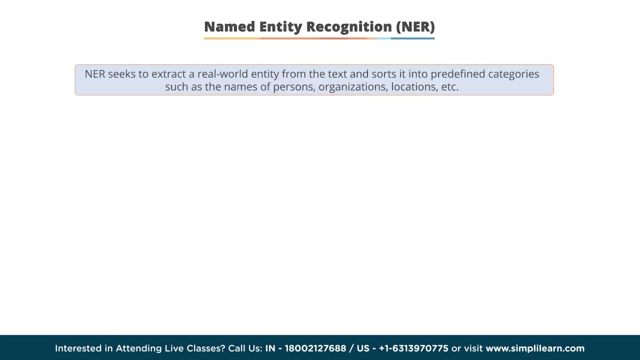 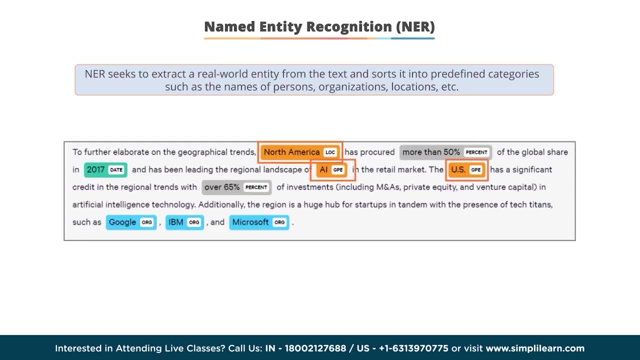 such as names of people, organizations, locations, etc. Many real-world questions are not defined. They can be answered with the help of named entity recognition. Were specified products mentioned in complaints or reviews. Does the tweet contain the name of a person? 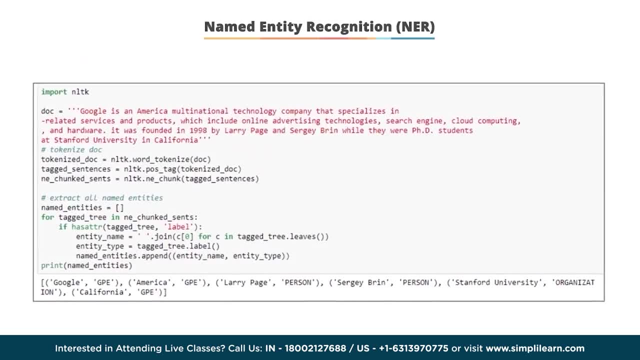 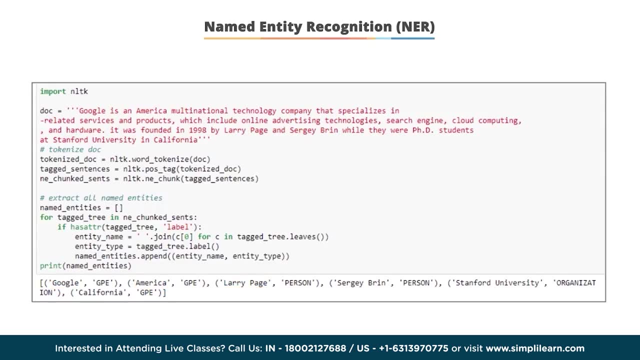 Does the tweet contain the person's address? As you can see in the given example, Google, America, Larry Page, etc. are the names of a person, place or an organization, So these are considered named entities and have different tags such as person, organization. 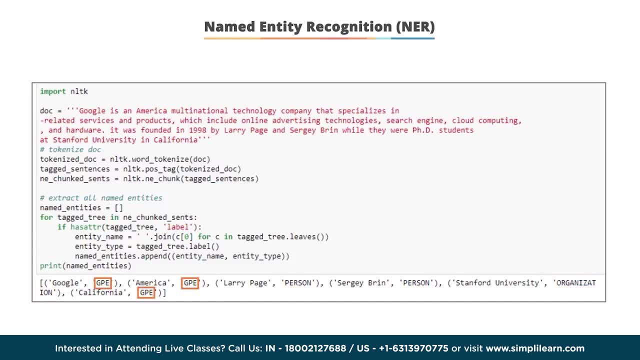 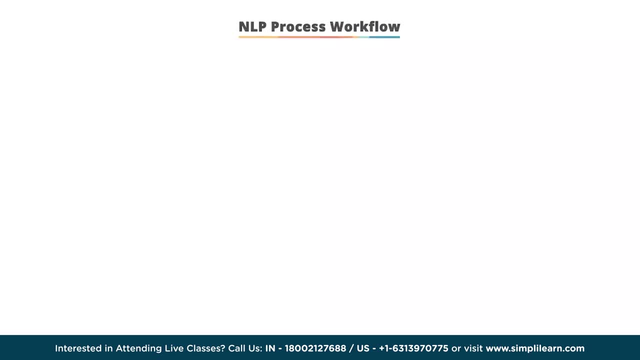 GPE or geoscience, NLP process workflow. Now you have an understanding of all NLTK tools, So now let's understand the natural language processing workflow. Step 1. Tokenization: It splits text into pieces, tokens or words and removes punctuation. 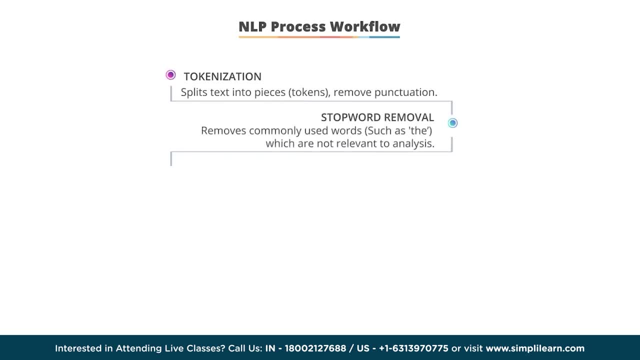 Step 2. Stop word removal. It removes commonly used words such as the is, are, etc. which are not relevant to the analysis. Step 3. Stemming and Limitization: It reduces words to base form in order to be analyzed as a single item. 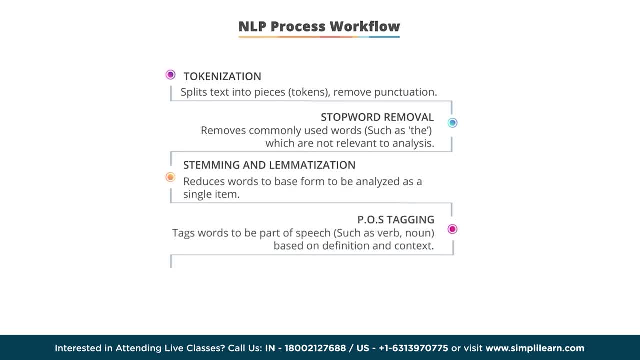 Step 4. POS Tagging: It tags words to be part of speech, such as noun, verb, adjective, etc. based on the definition and context. Step 5. Information Retrieval: It extracts relevant information from the source. Step 5.. 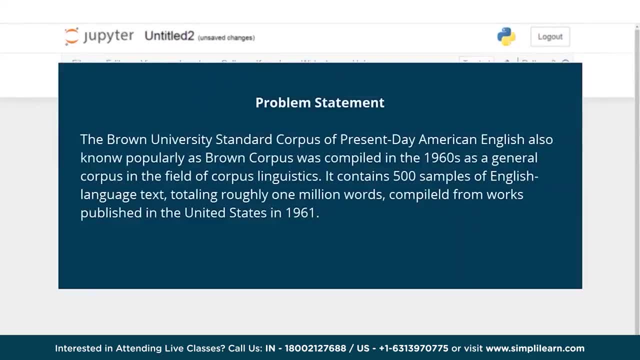 Formatting and Formatting: Step 1. Problem Statement: The Brown University Standard Corpus of present-day American English, also known popularly as Brown Corpus, was compiled in the 1960s as a general corpus in the field of corpus linguistics. It contains 500 samples of English-language text totaling roughly 1 million words compiled. 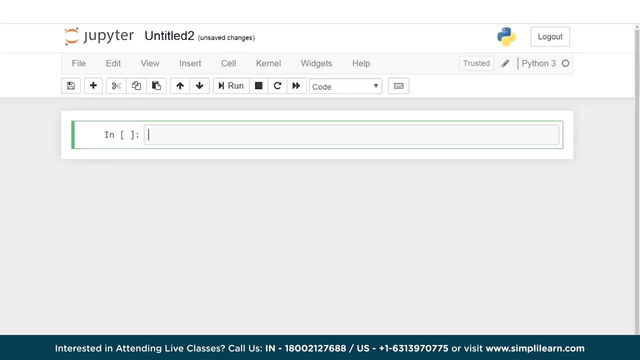 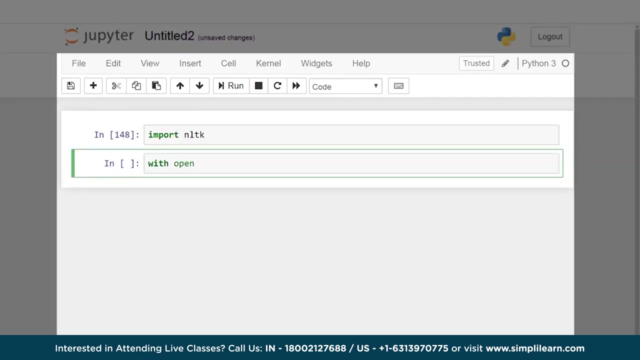 from works published in the United States in 1961.. We will be working on one of the subset data set, Step 2. Text Processing: Let us import the NLTK library and read the CA underscore 10: corpus: Import NLTK. We will have to make sure that there are no slashes in between. hence we will use the 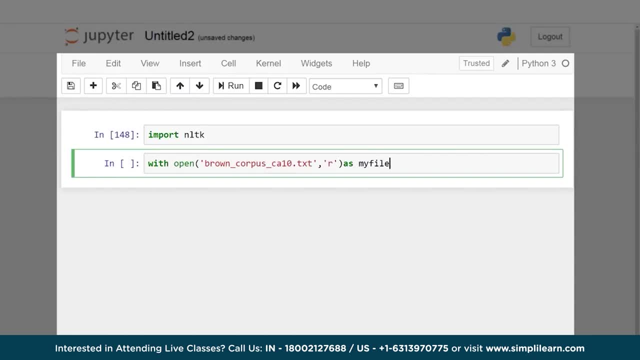 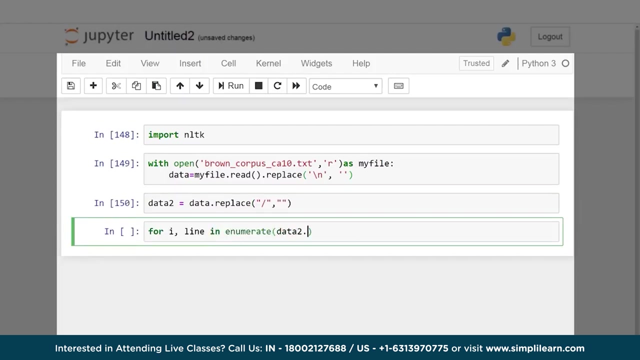 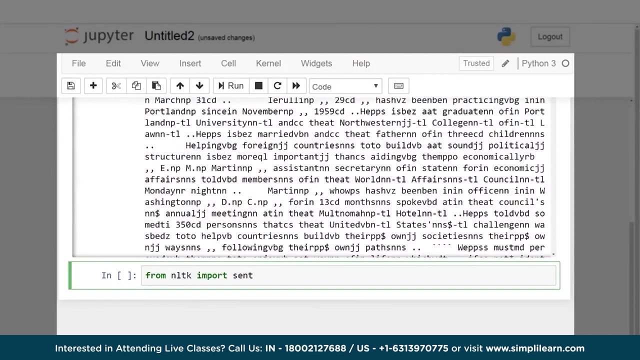 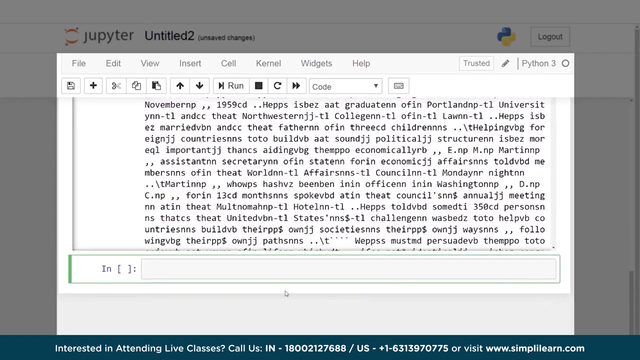 replace function within pandas for the same. Let us have a look at the data once. Step 3. Tokenization: After performing sentence tokenization on the data we obtain…. Step 4. Tape Mapping: Step 5. Tokenization: After applying Sentence Tokenizer. the resulting output shows all individual words: tokens. 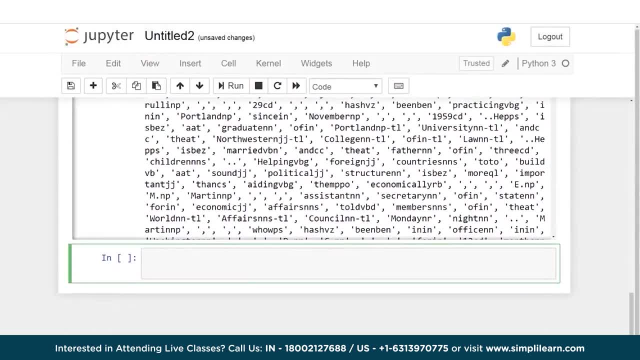 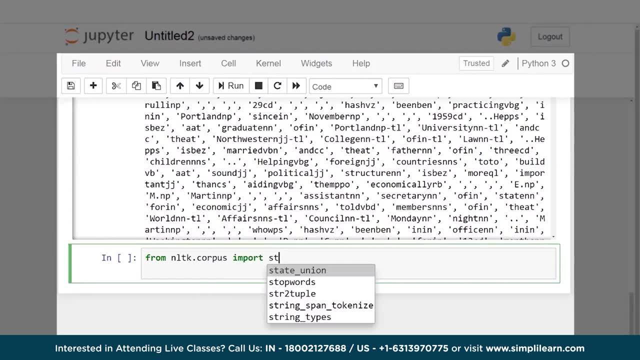 Stop Word Removal. Let's import the stop word library From nltkcorpus: import stop words. We also need to ensure that the text is in the same case. NLTK has its own list of stop words. We can check the list of stop words using stopwordswords and English inside the parenthesis. 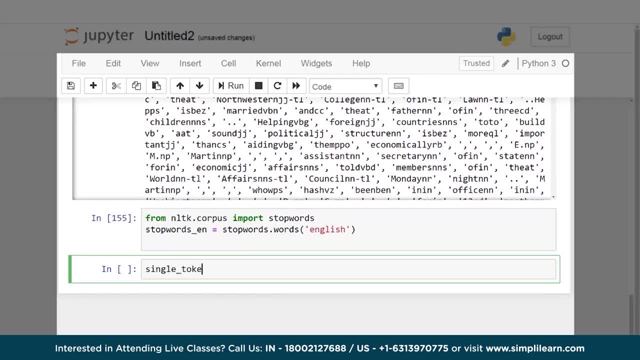 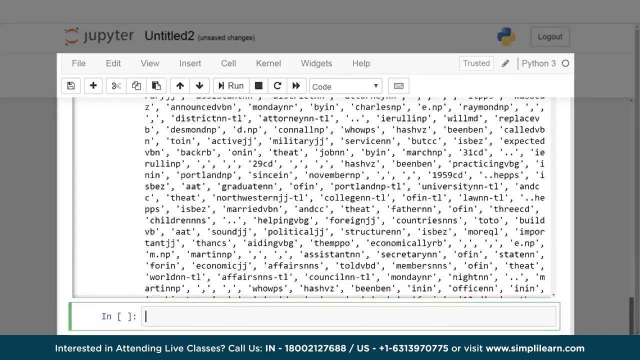 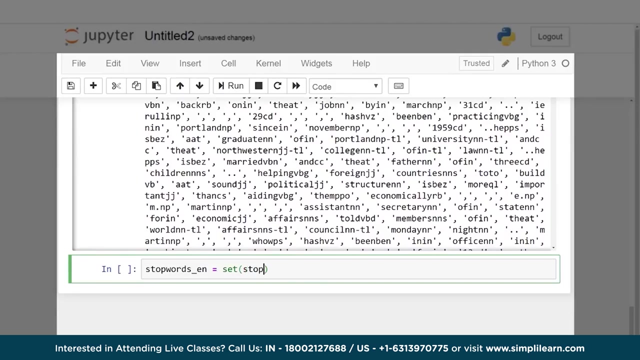 Map the lowercase string with our list of word tokens. Let's remove the stop words using the English stop words list in NLTK. We will be using set checking, as it is faster in Python than a list. By removing all stop words from the text, we obtain. 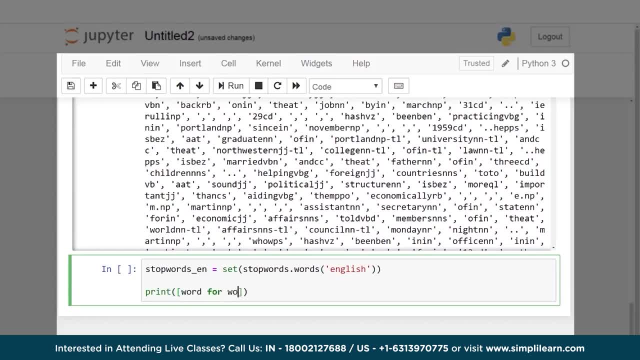 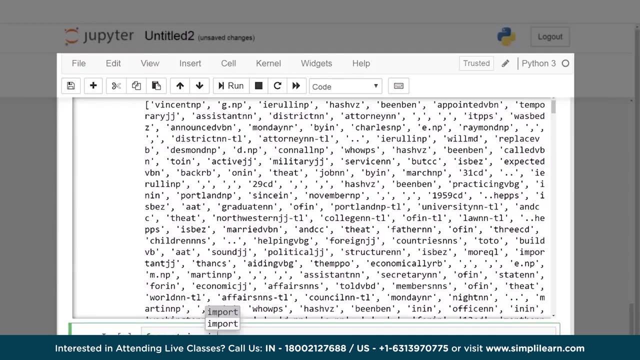 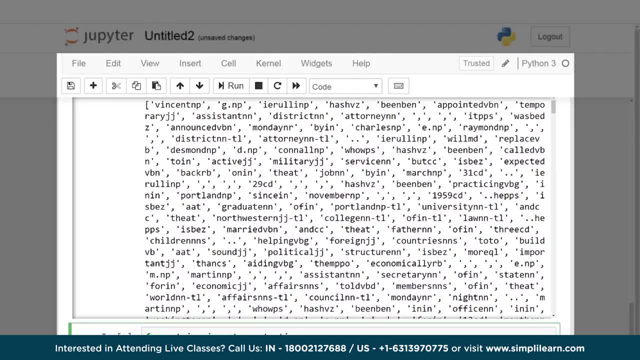 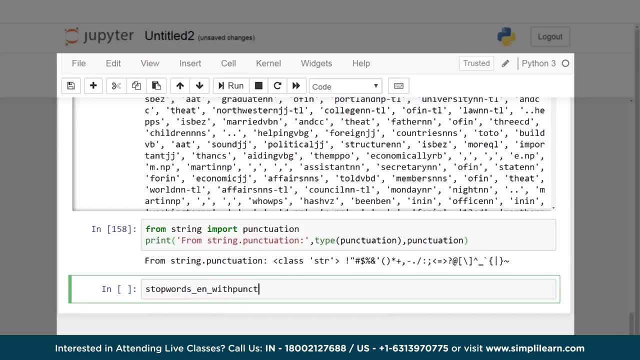 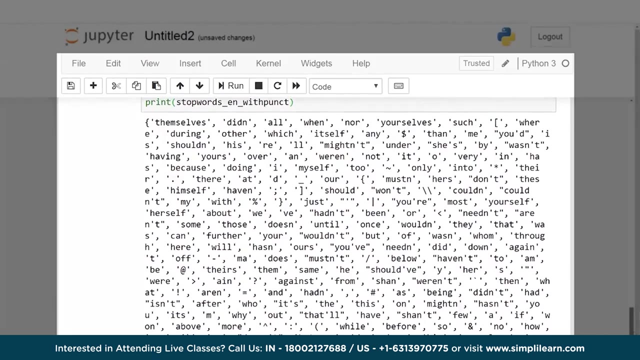 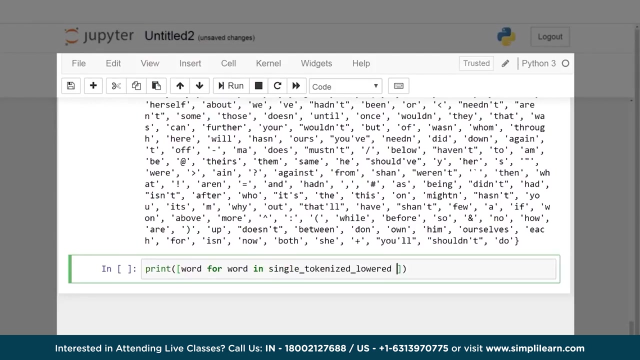 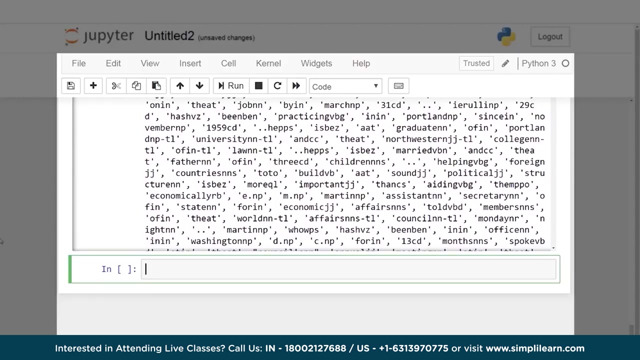 Combining the punctuation with the stop words from NLTK: Removing stop words with punctuation, Stemming and lemmatization. We will be using stemming and lemmatization to reduce words to their root form. For example, walks, walking, walked, will be reduced to their root word, walk. 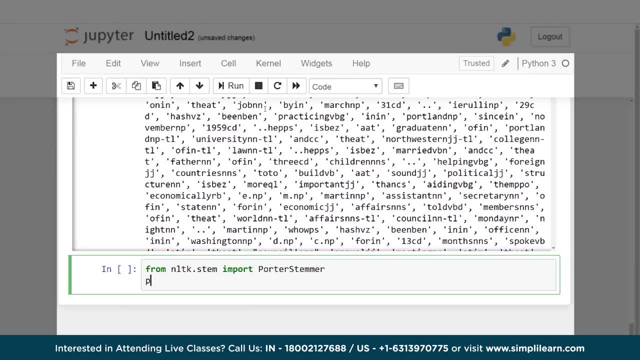 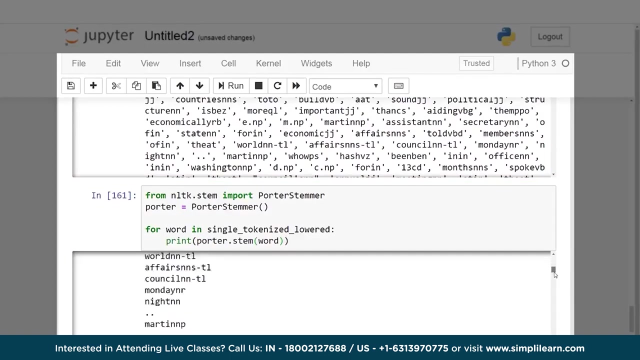 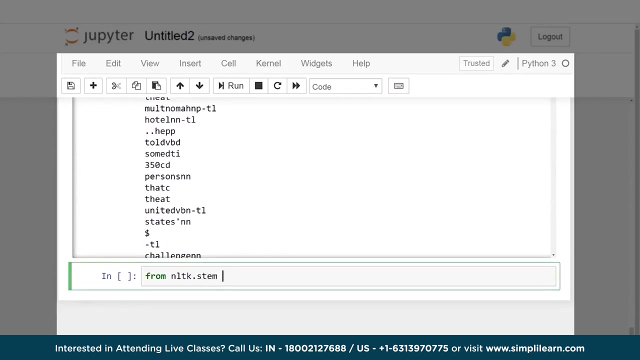 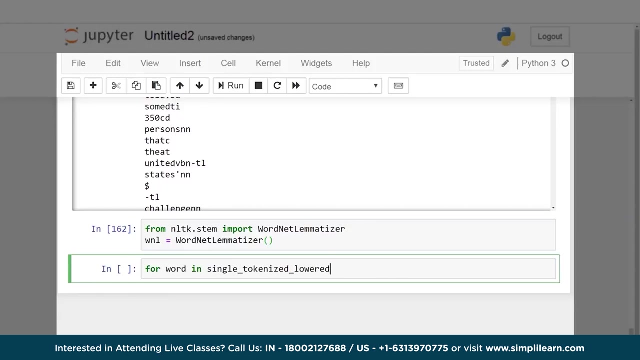 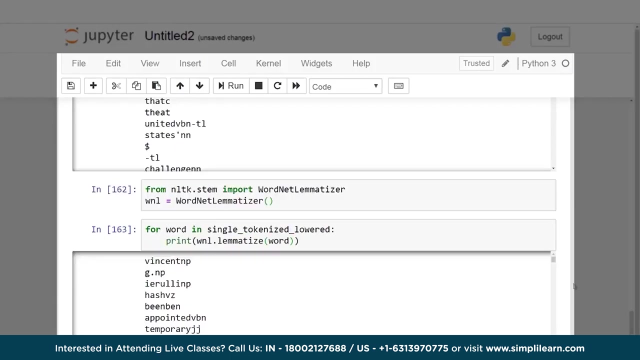 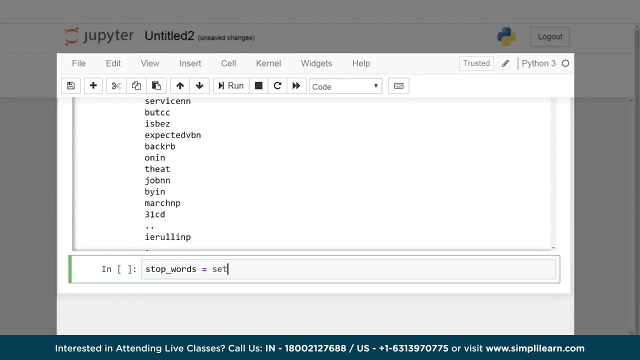 Importing porter stemmer as the stemming library From NLTKSTEM. import porter stemmer Printing the stem words. Import the WordNet lemmatizer from NLTK. From NLTKSTEM, Printing the root words. We also need to evaluate the POS tags for each token. 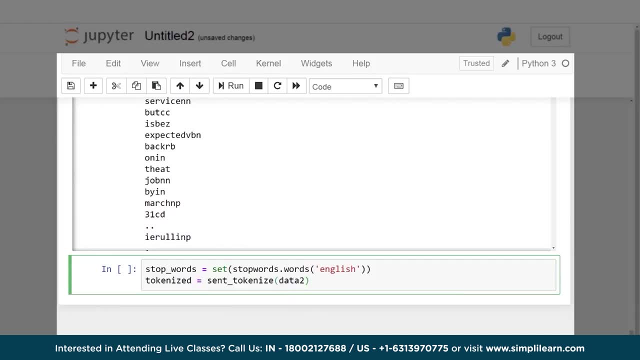 Create a new word list and store the list of word tokens against each of the sentence tokens in data2.. For I in tokenized. Also, we will check if there were any stop words in the recently created word list. We will now tag the word tokens accordingly using the POS tags and print the tagged output. 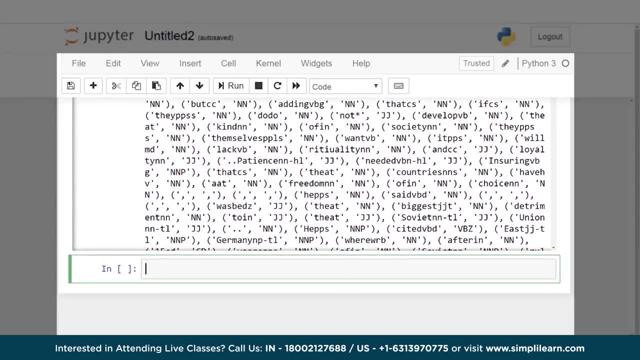 For our final text processing task. we will be applying Named Entity Recognition to classify named entities in text into pre-defined categories such as the names of persons, organizations, locations, expressions of times, quantities, monetary values, percentages, etc. Thank you. 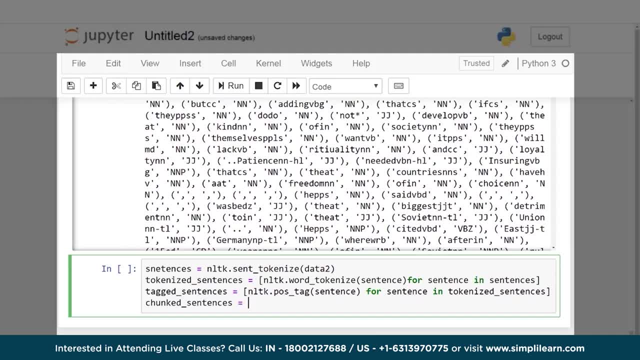 Now press the tagged sentences under the chunk parser. If we set the parameter binary equals true, then named entities are just tagged as NE. Otherwise, the classifier adds category labels such as person, organization and GPE. Create a function named as extractEntityNames along with an empty list named as EntityNames. 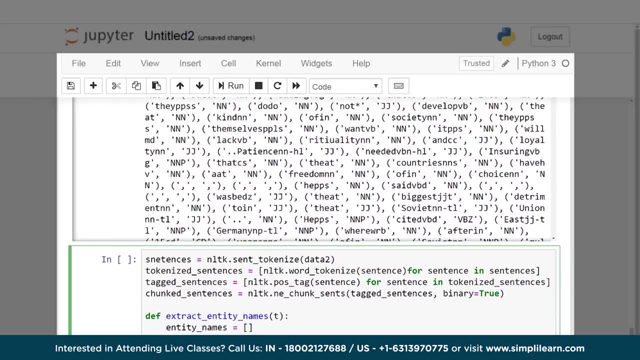 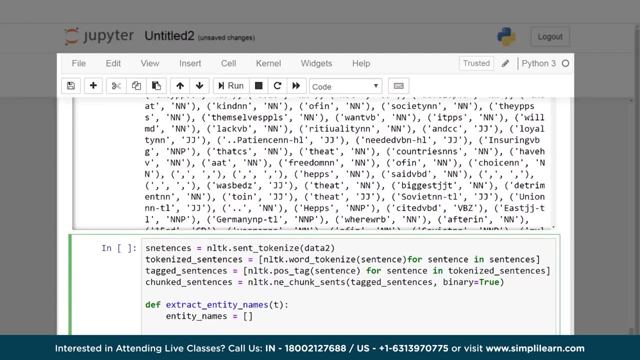 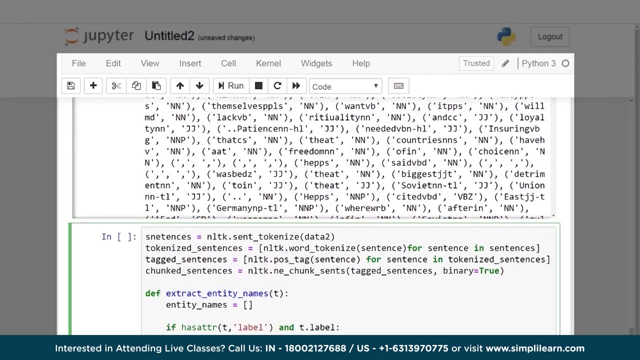 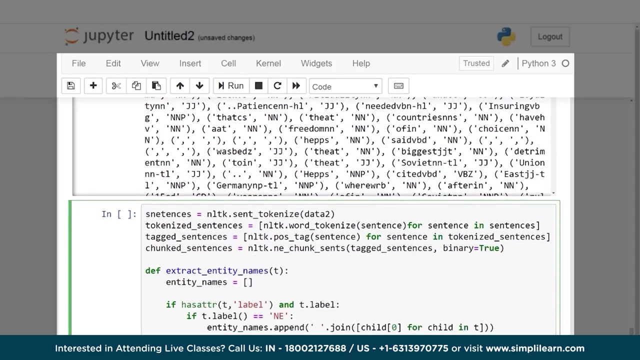 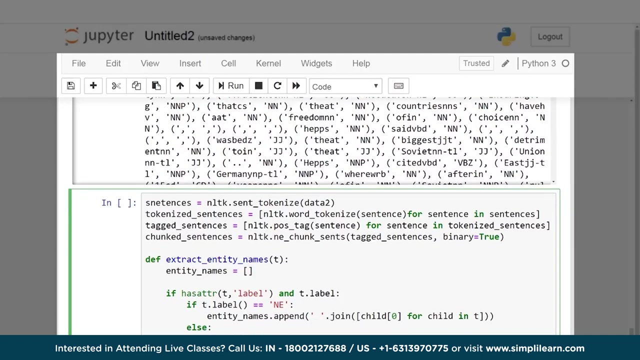 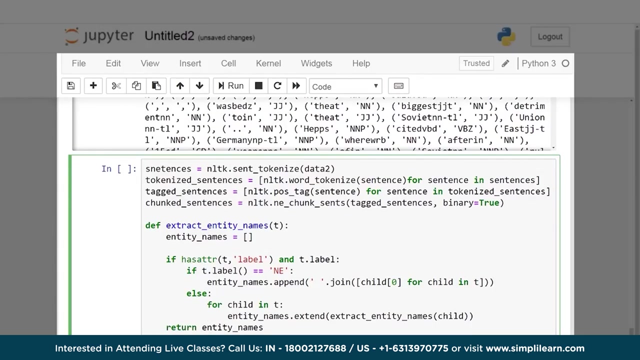 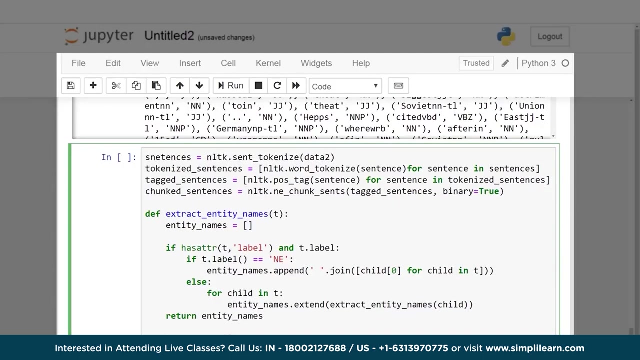 We will now extract named entities from a NLTK chunked expression and store them in the empty created above. Again, we will set the EntityNames list as an empty list and will extract the EntityNames by iterating over each tree in chunked sentences. 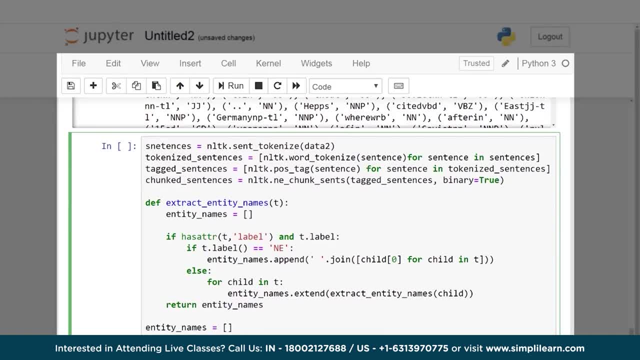 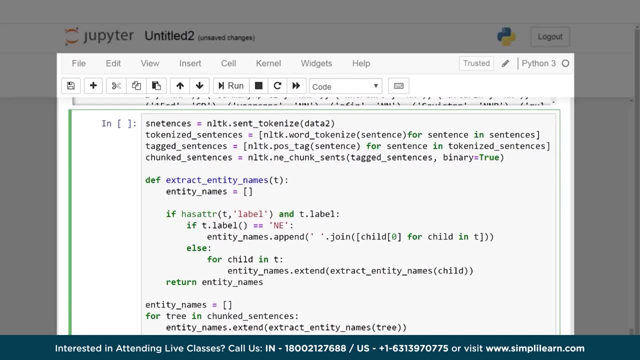 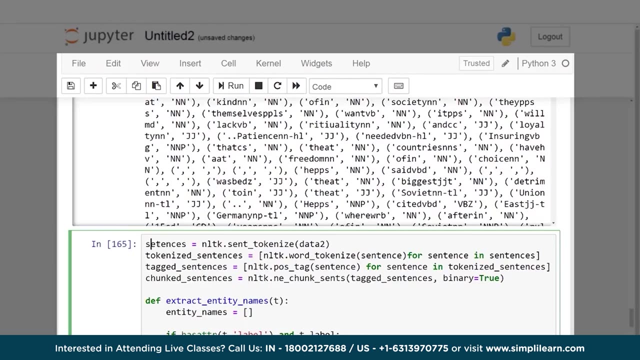 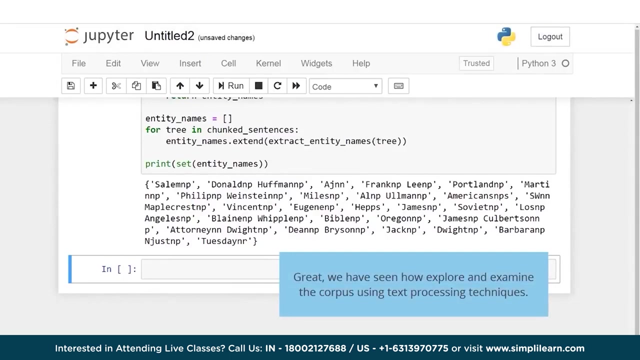 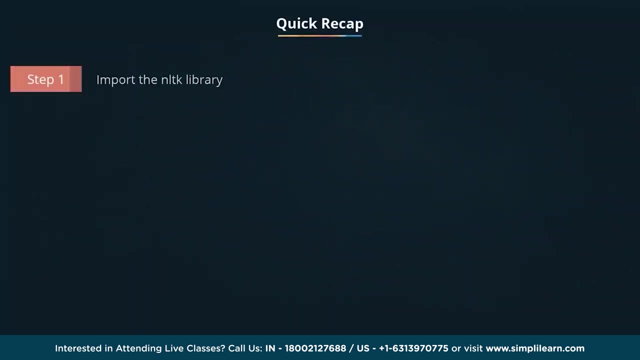 Great. we have seen how to explore and examine the corpus using text processing techniques. Let's quickly recap the steps we've covered so far: 1. Import the NLTK library. 2. Perform tokenization. 3. Perform stemming and delimitization. 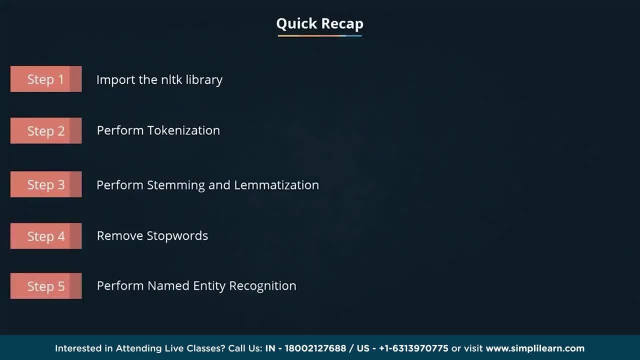 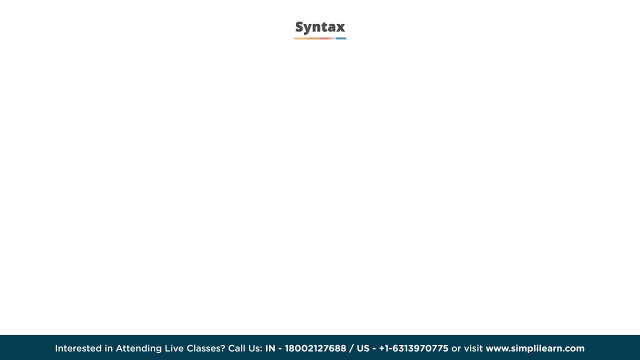 4. Remove stop words. 5. Perform named entity recognition. Structuring sentences- syntax. Let's first understand what syntax is. Syntax is the grammatical structure of sentences. In the given example, this can be interpreted as syntax and it is similar to the ones you use while writing codes. 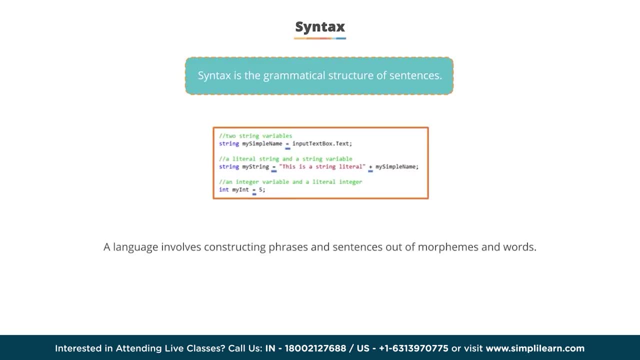 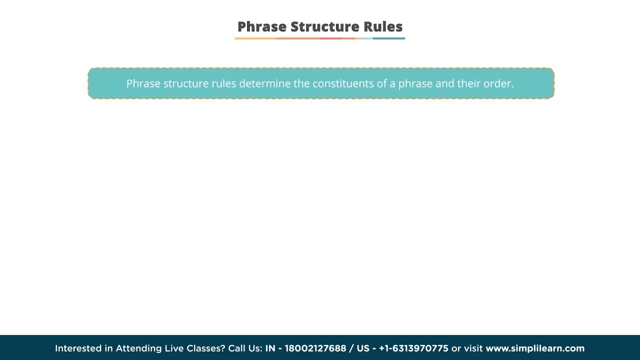 Knowing a language includes the power to construct phrases and sentences out of morphemes and words. The part of the grammar that represents a speaker's knowledge of these structures and their formation is called syntax. Phrase structure rules are rules that determine what goes into a phrase. 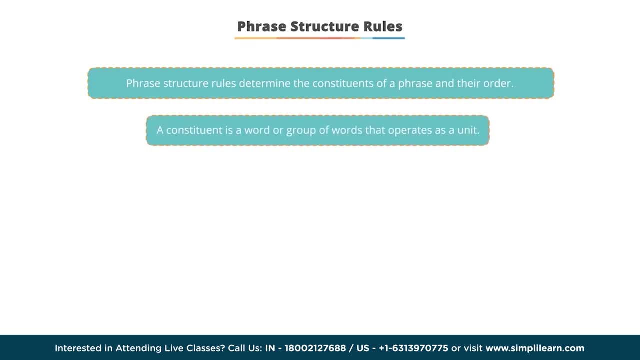 that is, constituents of a phrase and how the constituents are ordered. Constituent is a word or group of words that operate as a unit and can be used to frame larger grammatical units. The given diagram represents that A Noun phrase is determined when a noun is combined with a determiner and the determiner can be optional. 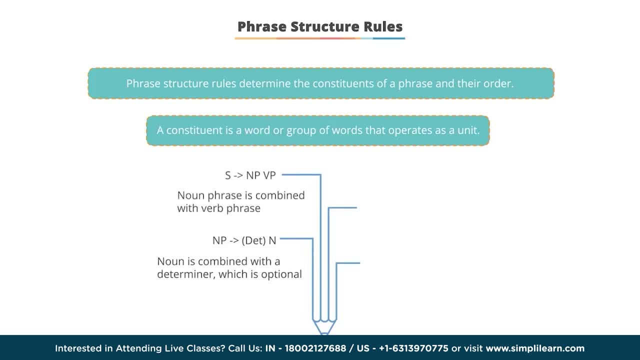 A sentence is determined when a noun phrase is combined with a verb phrase. A verb phrase is determined when a verb is combined optionally with the noun phrase and prepositional phrase, and a prepositional phrase is determined when a preposition is combined with a noun phrase. 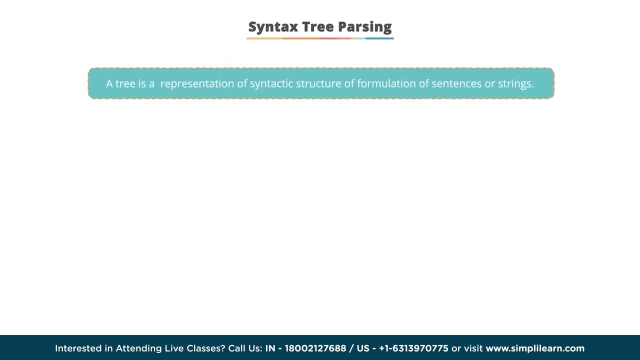 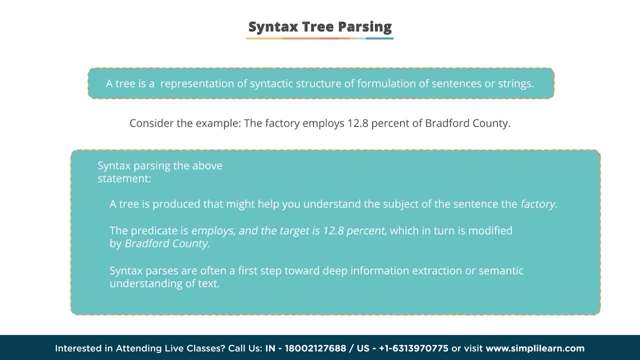 A tree is a representation of syntactics, structure of formulation of sentences or strings. Consider the given sentence. The factory employs 12.8% of Bradford County. What can be the syntax for pairing this statement? Let's understand this. A tree is produced. that might help you understand that the subject of the sentence is the factory. 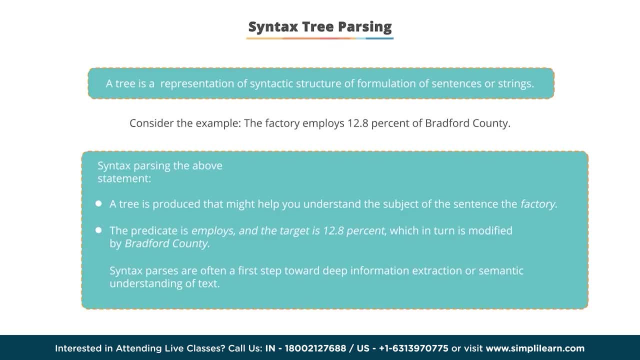 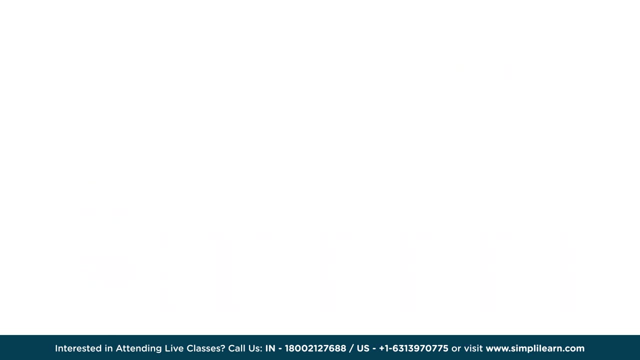 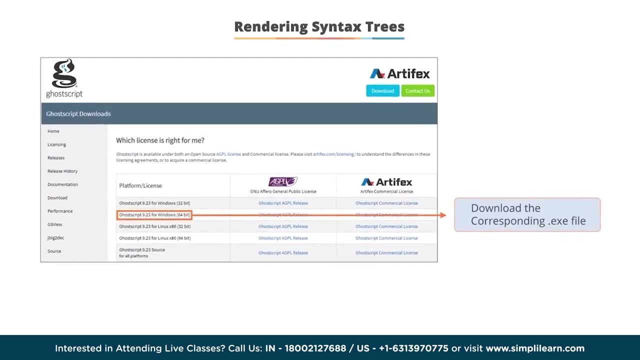 The predicate is employs and the target is 12.8%, which in turn is modified by Bradford County. Syntax parses are often a first step toward deep information extraction or semantic understanding of text Rendering Syntax Trees. Download the corresponding exe file to install the GhostScript rendering engine. 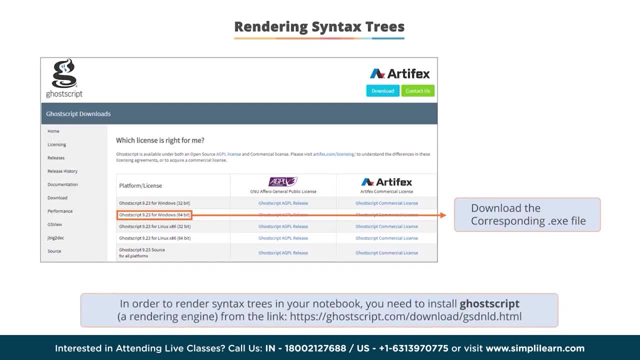 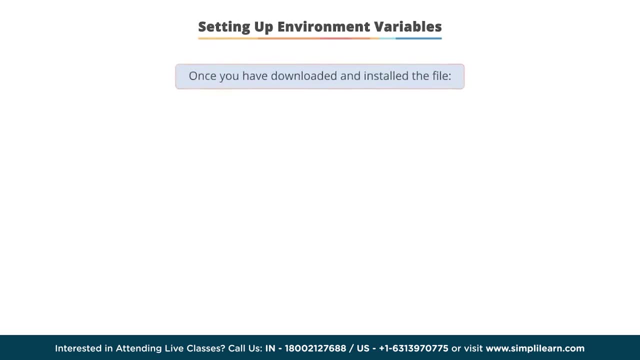 based on your system configuration, in order to install the GhostScript rendering engine, In order to render Syntax Trees in your notebook. Let's understand how you can set up the environment variable. Once you have downloaded and installed the file, go to the folder where it is installed and copy the path of the file. 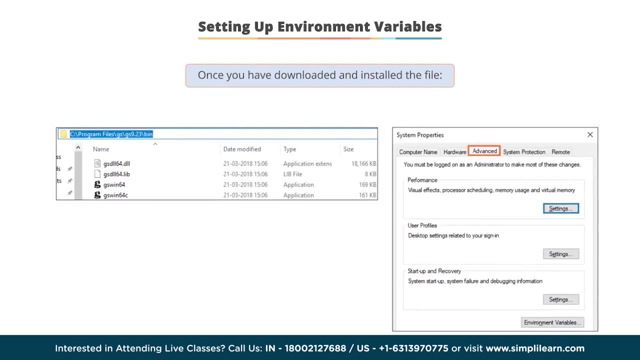 Now go to System Properties and under Advanced Properties you will find the Environment Variable button. Click on that to open the pop-up box tab of the environment. Now open the bin folder and add the path to the bin folder in your environment. This may be the path of the environment variables. 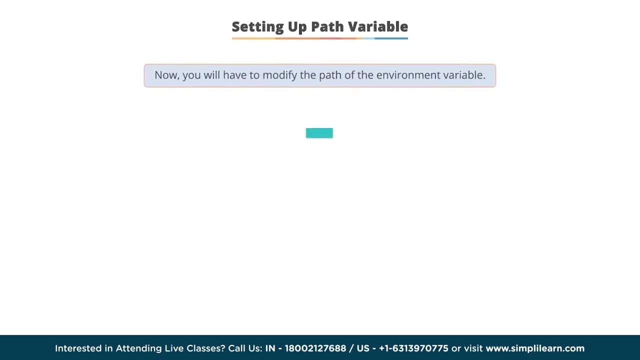 Now you will have to modify the path of the environment variable. Use the given code to test the working of Syntax Tree after the setup is successfully installed. Structuring Sentences. Chunking & Chunk. Parsing- The process of extraction of phrases from unstructured text is called chunking. 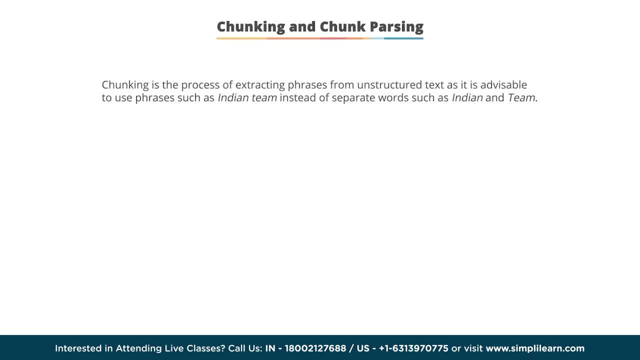 Instead of using just simple tokens, which may not represent the actual meaning of the text, it is advisable to use the text as a directory. advisable to use phrases such as indian team as a single word instead of indian and team as separate words. the chunking segmentation refers to identifying tokens and labeling refers to. 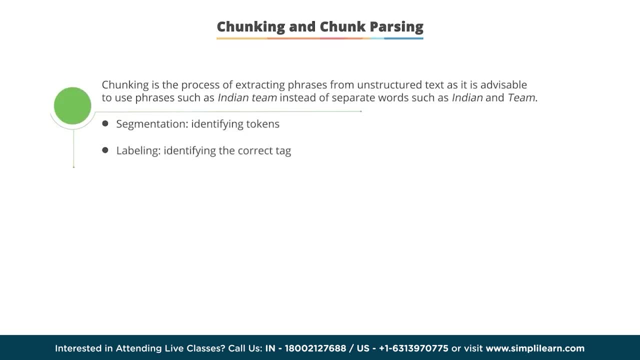 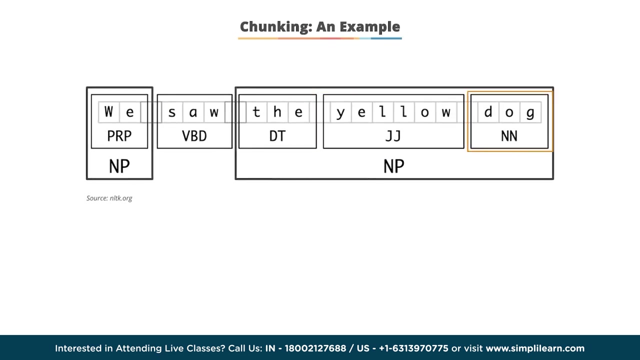 identifying the correct tag. these chunks correspond to mixed patterns. in some way to extract patterns from chunks, we need chunk parsing. the chunk parsing segment refers to identifying strings of tokens and labeling refers to identifying the correct chunk type. let's look at the given example. you can see here that yellow is an adjective, dog is a noun. 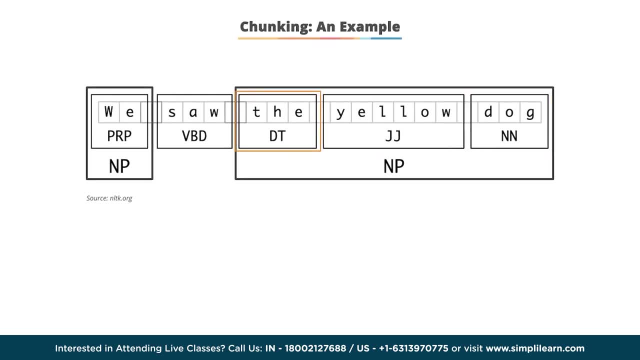 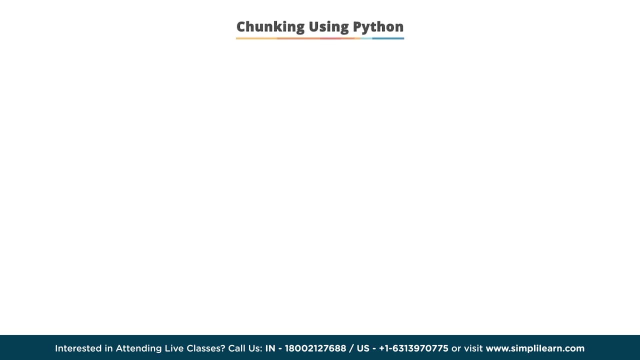 and the is the determiner, which are chunked together into a noun phrase. similarly, chunk parsing is used to extract patterns and to process such patterns from multiple chunks while using different parsers. let's take an example and try to understand how chunking is performed in python. let's consider the sentence: the little mouse ate the fresh cheese assigned to. 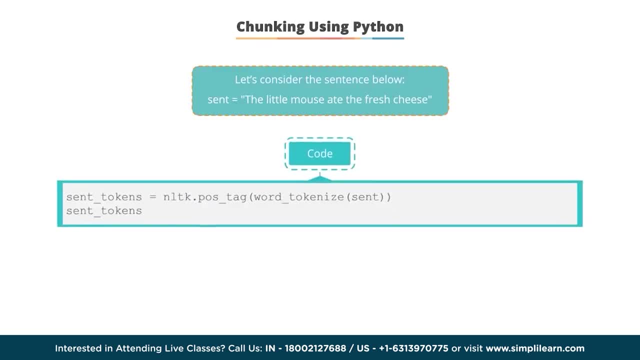 a variable named sent using the word tokenize function under nltk corpora. you can find out the different tags associated with the sentence provided. so, as you can see in the output, different tags have been allocated against each of the words from the given sentence using chunking, np chunk and parser. 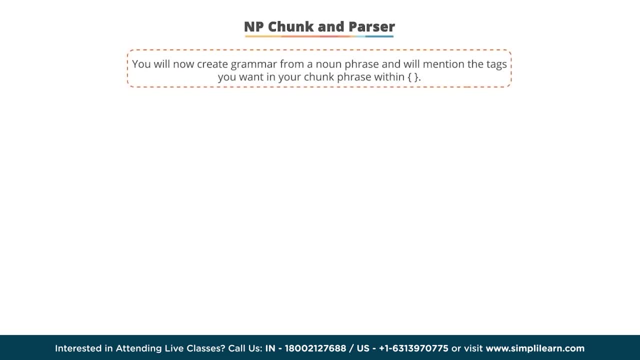 you will now create grammar from a noun phrase and will mention the tags you want in your chunk phrase within the function. here you have created a regular expression matching the string. the given regular expression indicates optional determiner followed by optional number of adjective followed by a noun. you will now have to parse the chunk. therefore, you will create a chunk. 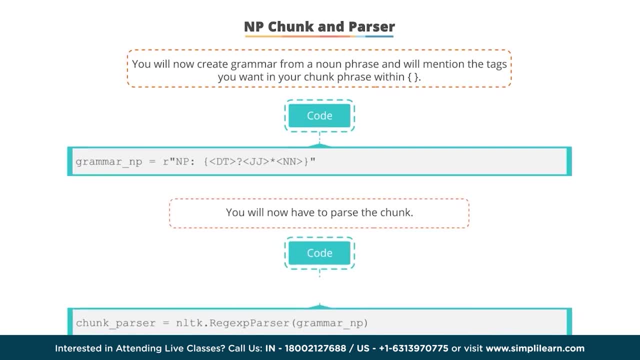 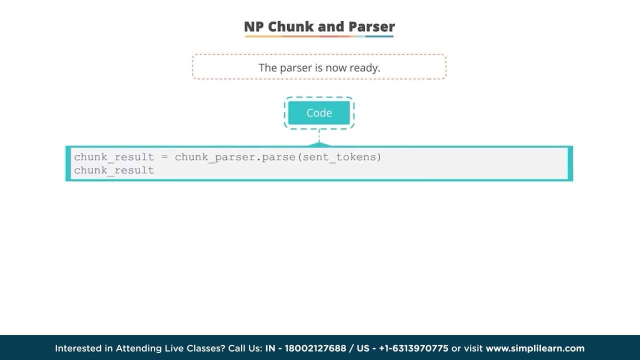 parser and pass your noun phrase string to it. the parser is now ready. you will use the parse parenthesis- parenthesis within your chunk parser to parse your sentence. the sentence provided is: the little mouse ate the fresh cheese. this sentence has been parsed and the tokens that match the 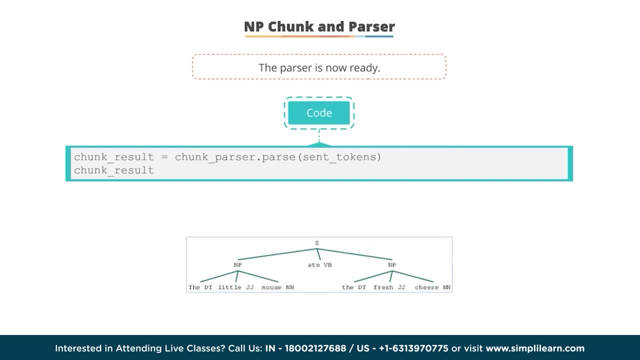 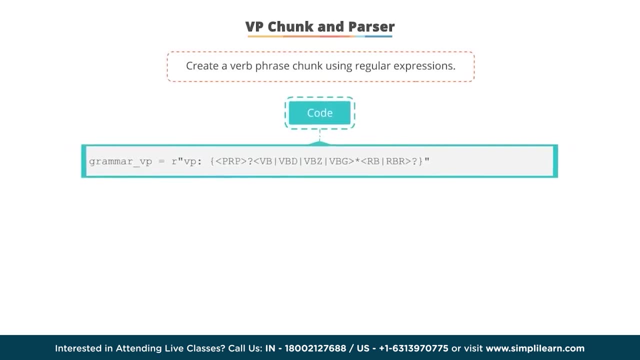 regular expressions are chunked together into noun phrases and p. create a verb phrase chunk using regular expressions. the regular expression has been defined as optional personal pronoun followed by zero or more verbs with any of its type, followed by any type of adverb. you'll now create another chunk, parser, and pass the verb phrase string to it. create another. 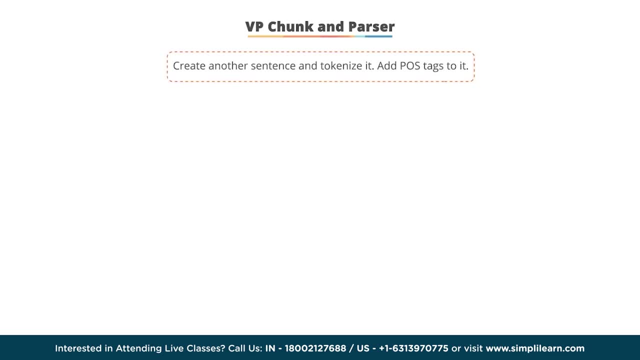 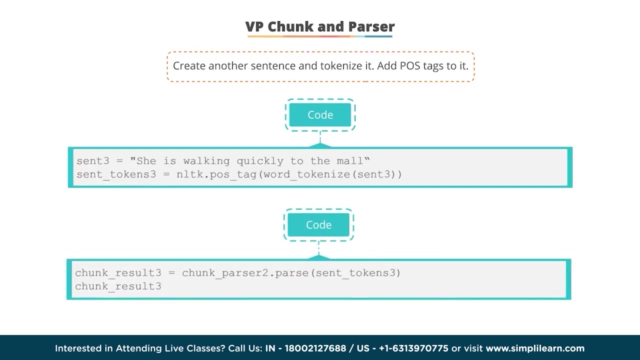 sentence and tokenize it. add pos tags to it. so the new sentence is: she is walking quickly to the mall and the pos tag has been allocated from nltk corpora. now use the new verb phrase parser to parse the tokens and run the results. you can look at the given tree diagram, which shows a verb parser. 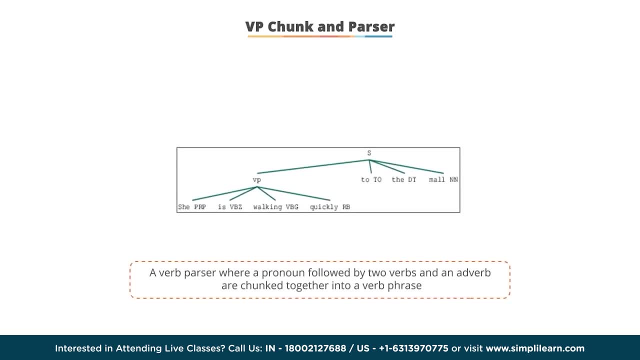 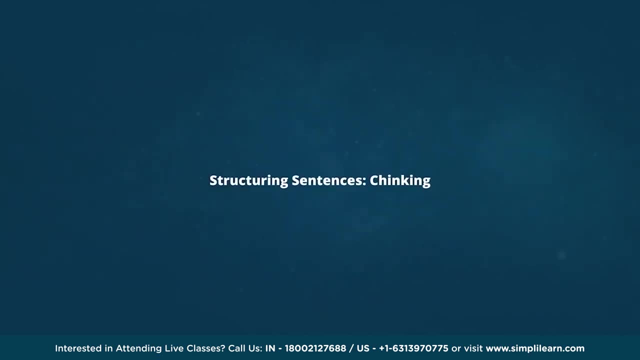 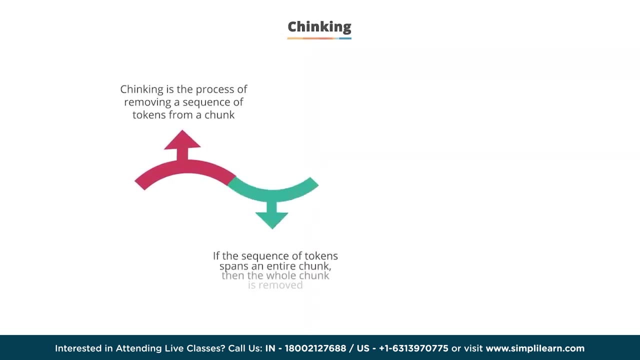 where a problem is solved. you can see that the pronoun followed by two verbs and an adverb are chunked together into a verb. parse structuring sentences: chinking. chinking is the process of removing a sequence of tokens from a chunk. how does chunking work? the whole chunk is removed when the sequence of tokens spans an. 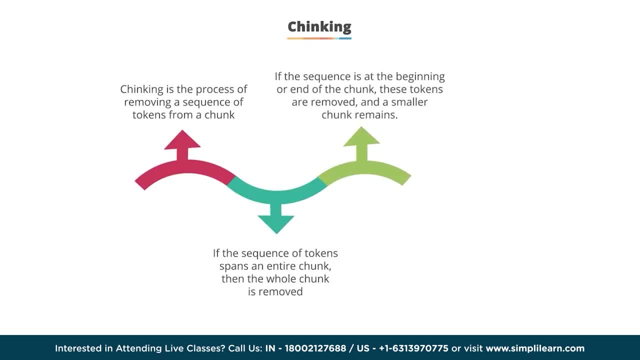 entire chunk. if the sequence is at the start or the end of the chunk, the tokens are removed from the start and end and a smaller chunk is retained. if the sequence of tokens appears in the middle of the chunk, these tokens are removed, leaving two chunks where there was only one before. consider you create a chinking grammar string containing 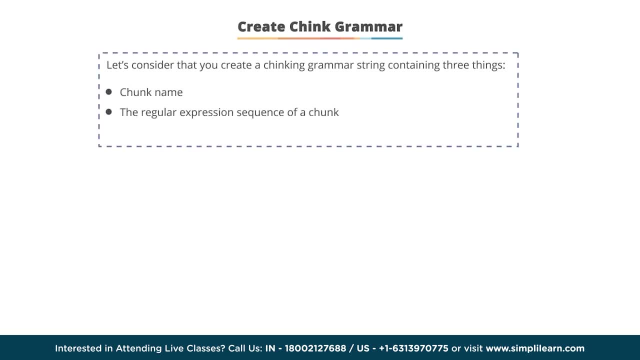 three things: chunk name: the regular expression sequence of a chunk. the regular expression sequence of your chink. here in the given code, we have the chunk regular expression as optional personal pronoun, followed by zero or more occurrences of any type of the adverb type, followed by zero or more occurrences of any of the adverb types: the chink regular. 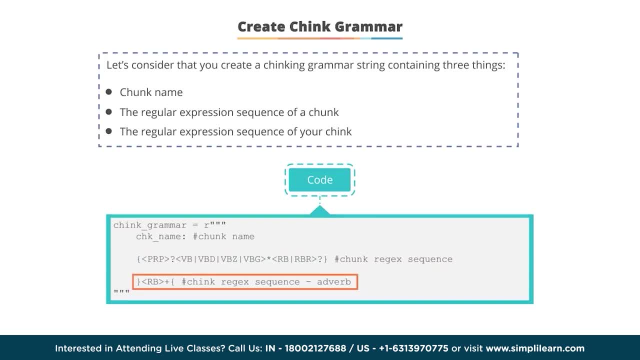 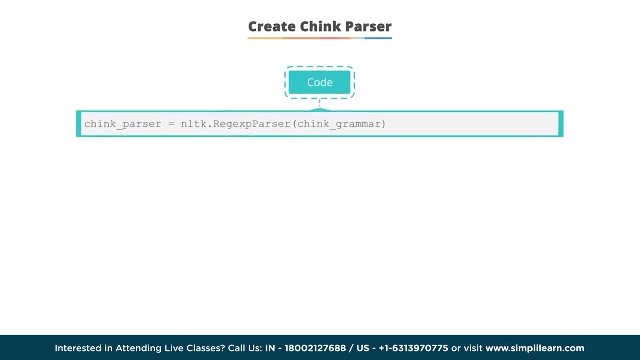 expression says that it needs to check for the adverb in the extracted chunk and remove it from the chunk inside the chinking block with open curly braces and closing curly braces. you have created one or more adverbs. you will now create a parser from nltk dot reg exp parser and pass the. 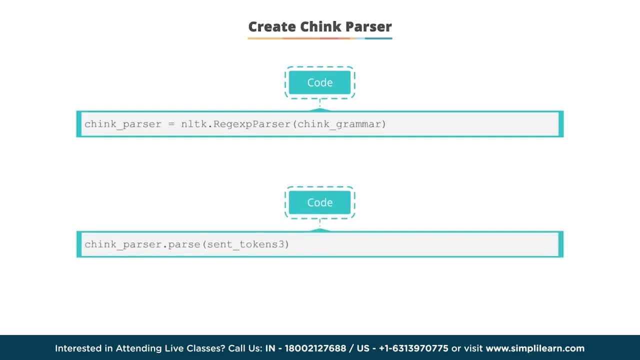 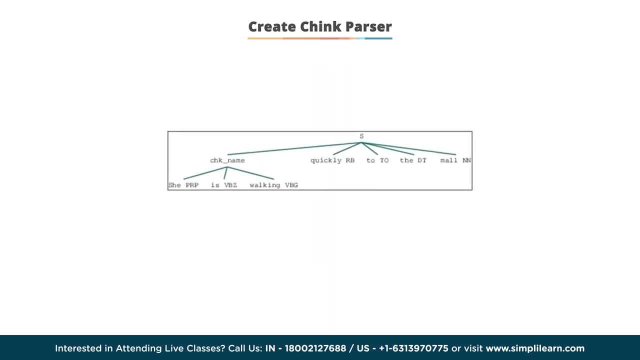 chink grammar to it. now use the new chink parser to parse the tokens sent three and run the results. as you can see, the parse tree is generated. while comparing the syntax tree of the chink parser with that of the original chunk, you can see that the token is quickly adverb chinked out of the chunk. 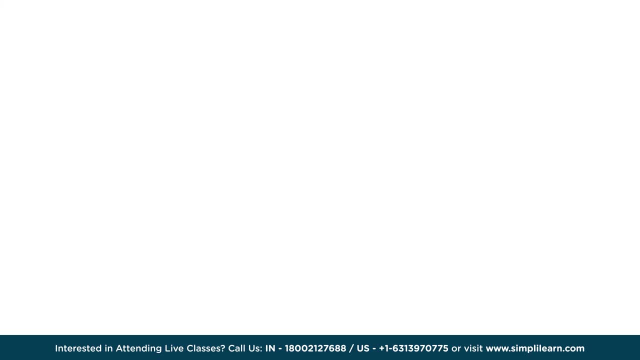 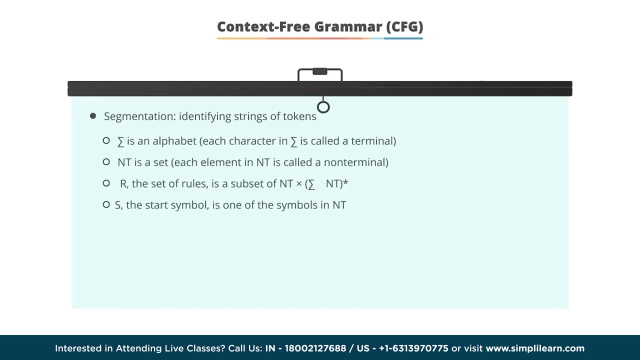 let's understand how to use context-free grammar. a context-free grammar is a four tuple sum ntrs, where sum is an alphabet and each character in sum is called a terminal. nt is a set and each element in nt is called a non-terminal r. the set of rules is a subset of nt times. the set of sum u and t. 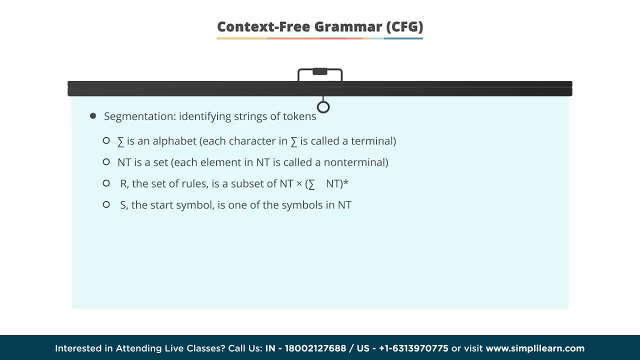 s. the start symbol is one of the symbols in nt. a context-free grammar generates a language, l capturing constituency and ordering. in cfg, the start symbol is used to derive the string. you can derive the string by repeatedly replacing a non-terminal on the right-hand side of the production until all non-terminals have been replaced by terminal symbols. 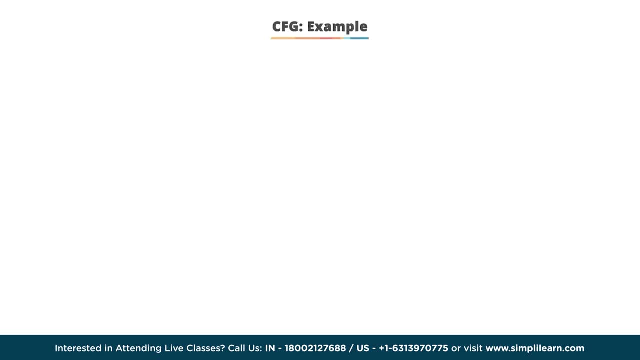 let's understand the representation of context-free grammar through an example. in context-free grammar, a sentence can be represented as a noun phrase followed by a verb phrase. noun phrase can be a determiner nominal. a nominal can be a noun. vp represents the verb phrase. a can be called a determiner. flight can be called a noun. consider the string below, where you have: 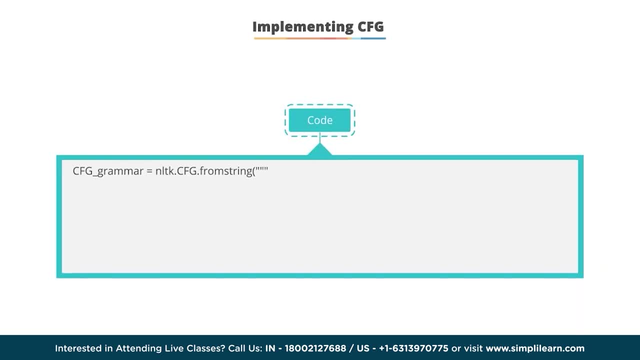 certain rules. when you look at the given context-free grammar, a sentence should have a noun phrase followed by a verb phrase. a verb phrase is a verb followed by a noun. a verb can either be saw or met. noun phrases can either be john or jim and a noun can either be a dog or a cat. check the. 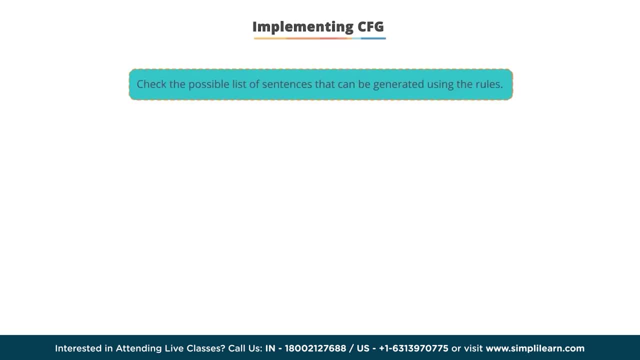 possible list of sentences that can be generated using the sentence-free grammar in context-free grammar using the rules. use the join function to create the possible list of sentences. you can check the different rules of grammar for sentence formation using the production function. it will show you the different tags used and the defined context-free grammar for the given. 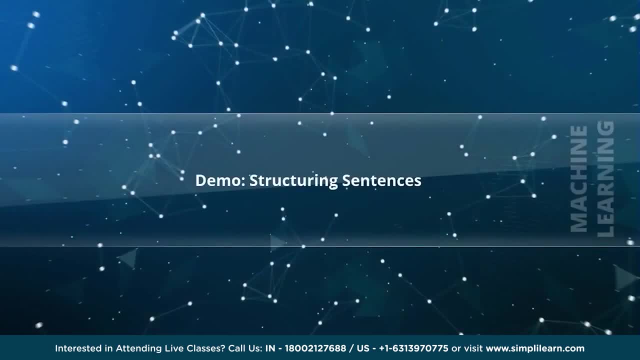 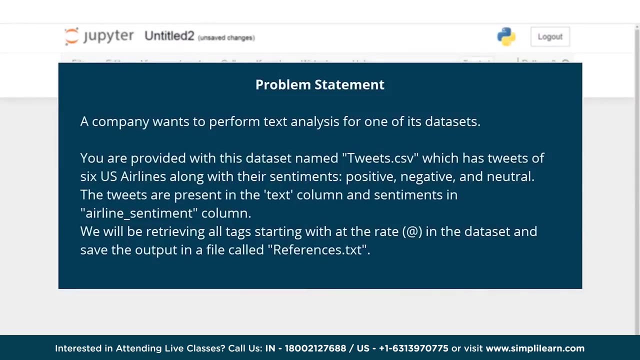 sentence: demo 2: structuring sentences. problem statement: a company wants to perform text analysis for one of its data sets. you are provided with this data set, named tweetscsv, which has three tags. the first tag is a column of text along with the second tag is the column of text. 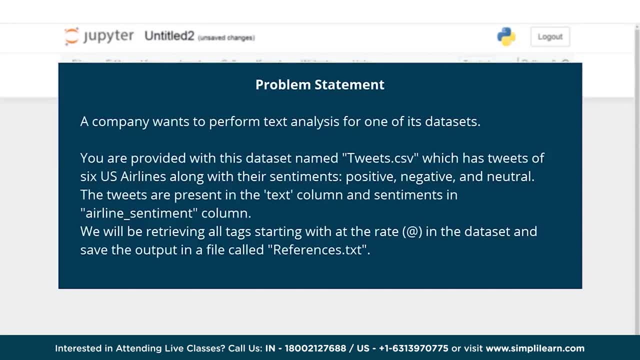 which is followed by a second tag on the top. the first image of the second column of the second image is an image showing the type of the text and the type of the text. as you see here you can see the different colors in the text on the left side and the text on the right side. 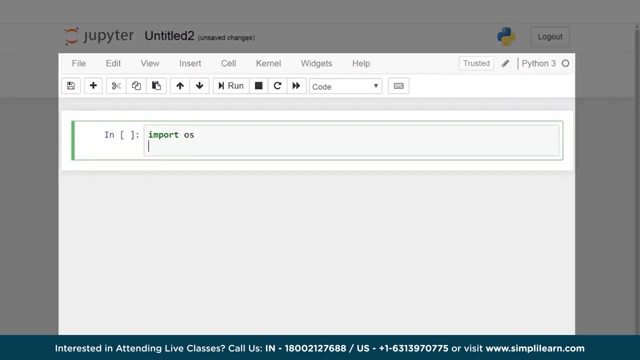 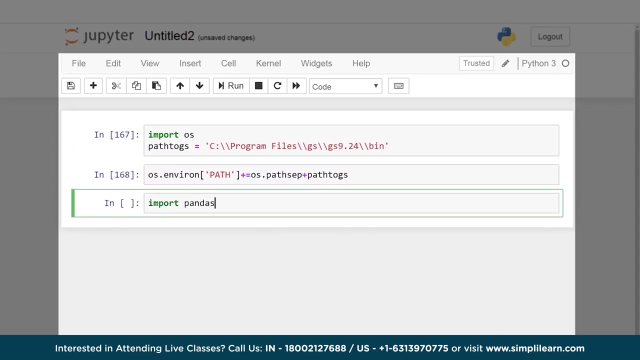 and on the right side you will see the content that is highlighted on this color bar, which is the. you Extract the features, text and airline sentiment. We will iterate through the dataset using regx. find the relevant tweets. Now we will import the iter tools module. 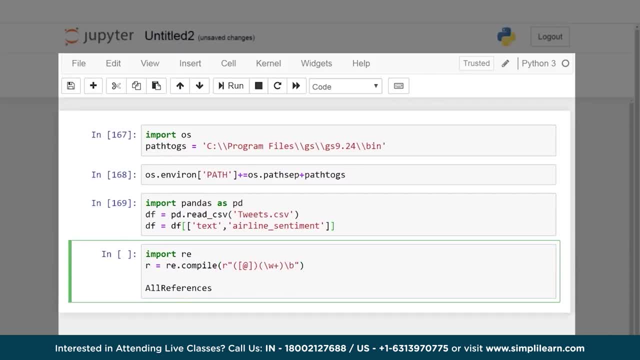 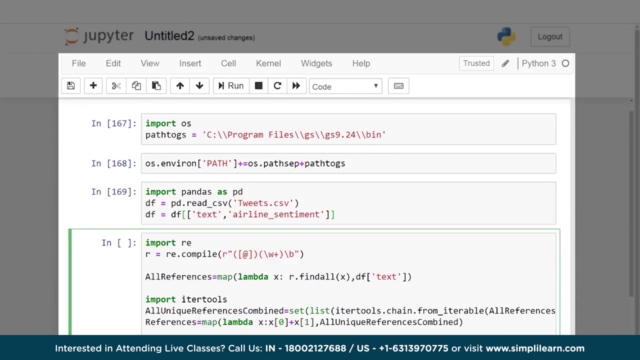 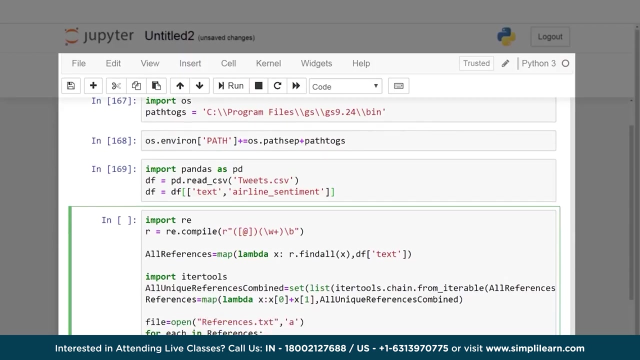 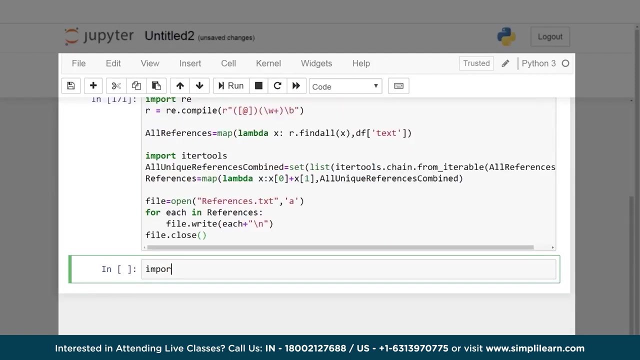 It returns efficient iterators, We will importuru update the concept for iter-tools from the table. Our result is stored in a file named referencestxt. Let's extract all noun phrases and save them in a file named Noun Phrases for left caret airline underscore sentiment right caret review dot txt. 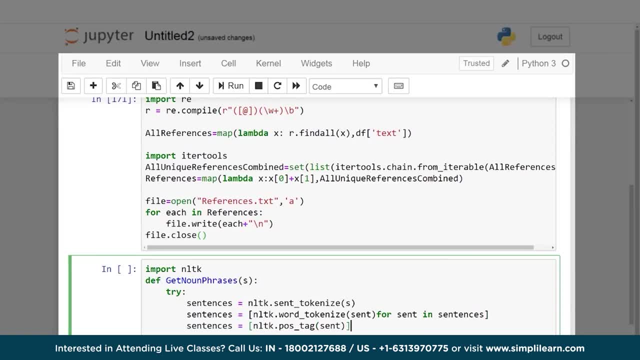 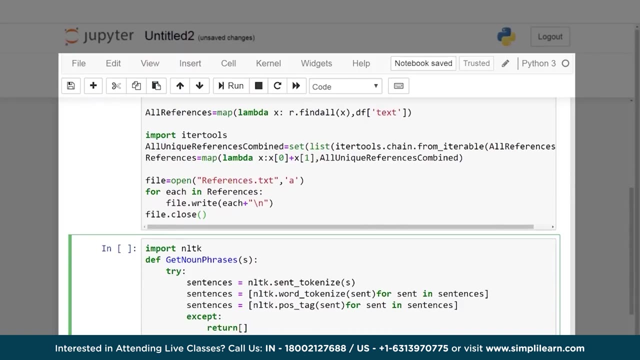 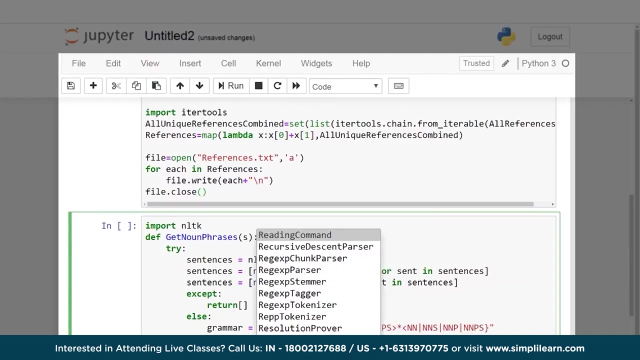 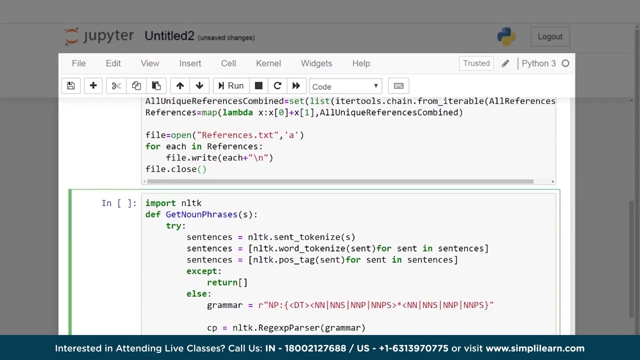 Here left caret, airline underscore sentiment right caret has three different values: positive, negative and neutral. so three files will be created Now we will iterate all the leaf nodes and assign them to Noun Phrases. Here: left caret- airline underscore sentiment right caret. 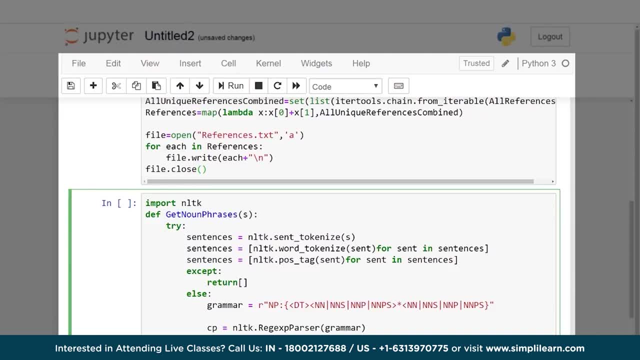 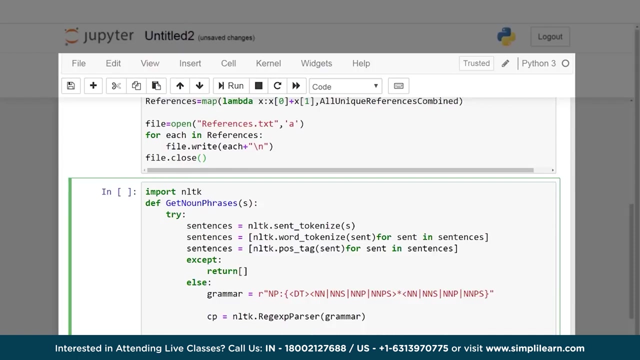 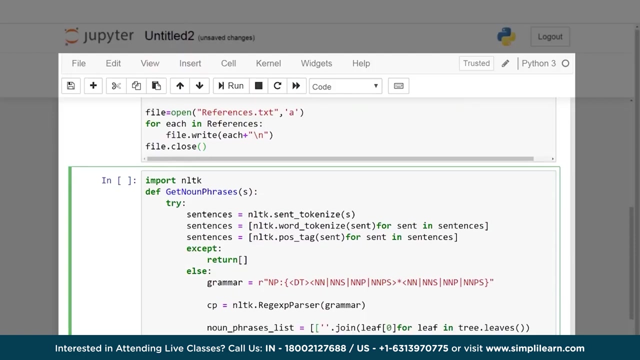 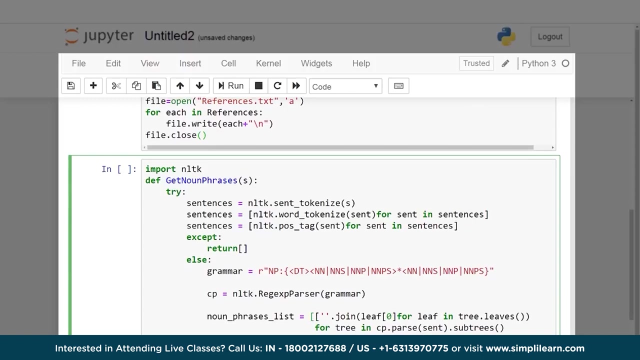 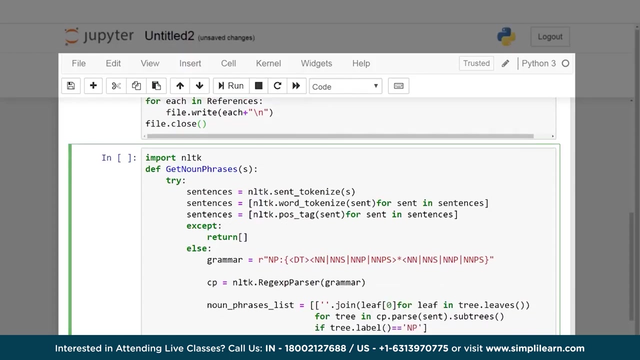 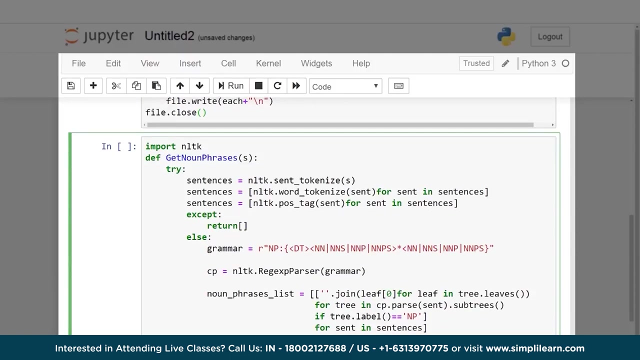 assign them to Noun Phrases. variable Here: left caret airline underscore sentiment: right caret- assign them to Noun Phrases. This means that the functions in iter tools operate on iterators to produce more complex iterators. This means that the functions in iter tools operate on iterators to produce more complex iterators. 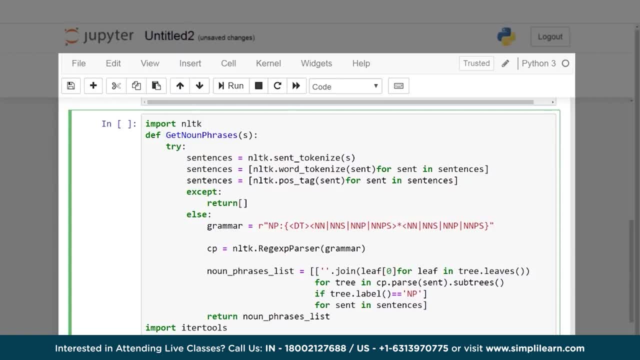 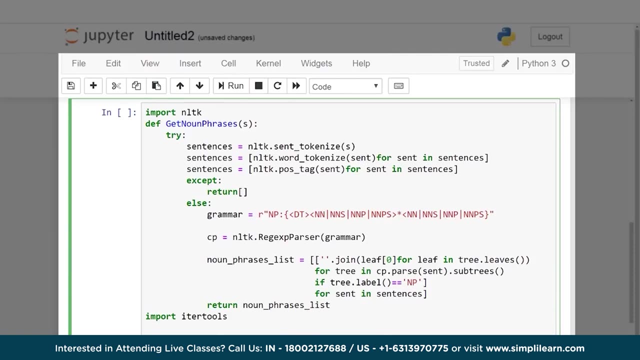 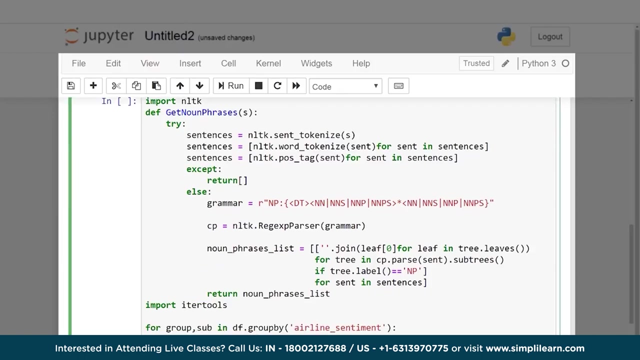 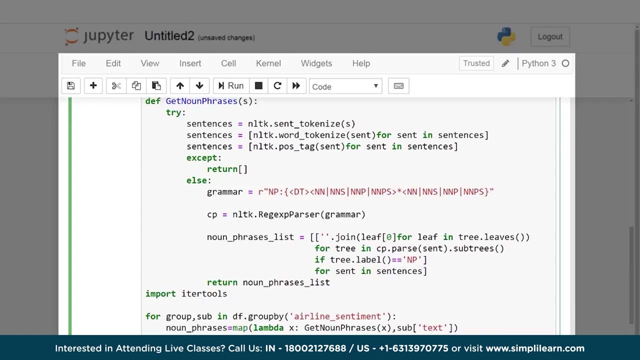 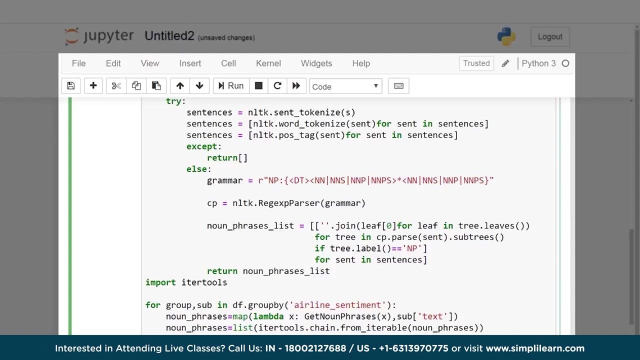 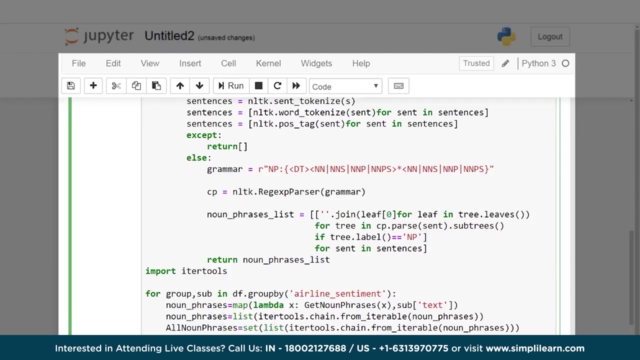 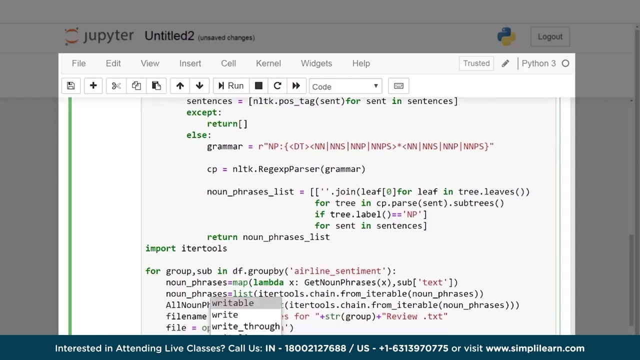 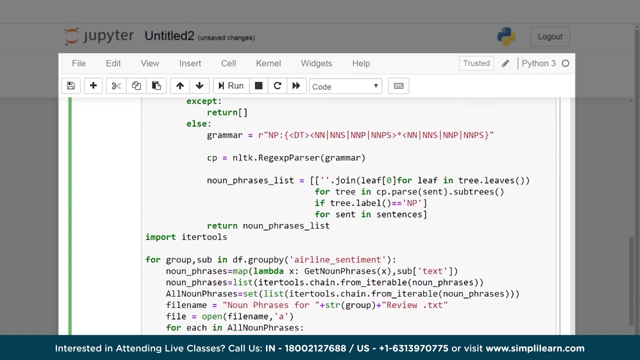 Using the map function, we will get all the noun phrases from the text, Putting it into list, Creating a file name in the name of reviewtxt, connecting, if necessary, touch to the name of the organization and saying data to be found By our system. it has some. 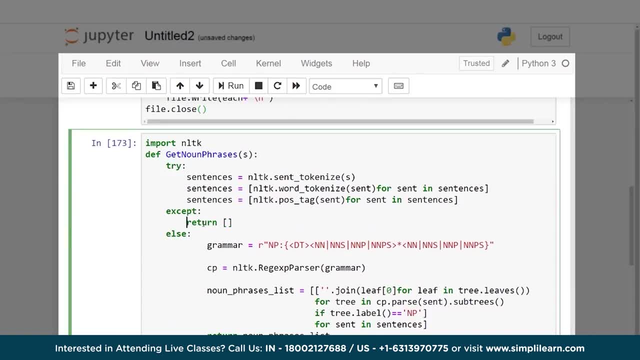 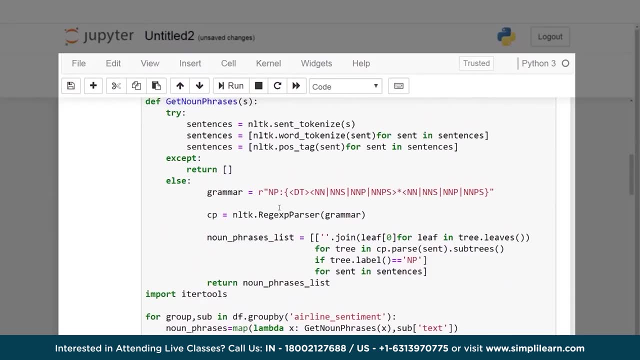 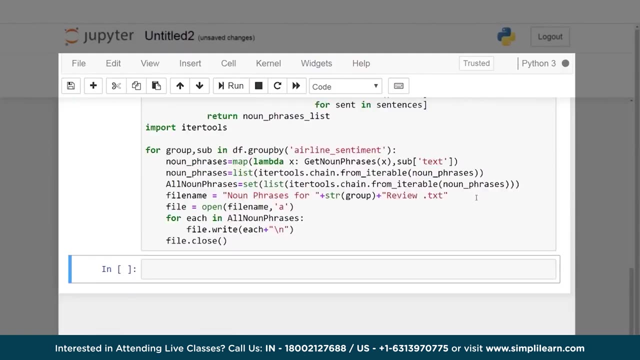 useful functions. it's they can provide you with code tracking Allugh animal that is. firstly, that is related to one another. After I going through the policies, I will change the that monocular. In a world where email is crucial, spam messages plague our inboxes, disrupting our digital. 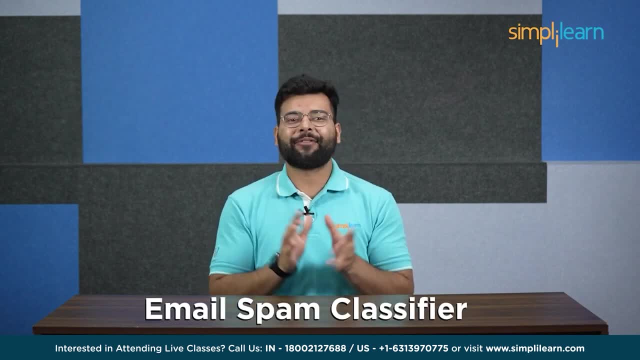 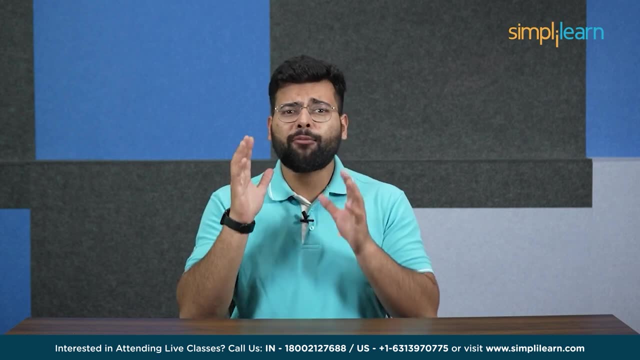 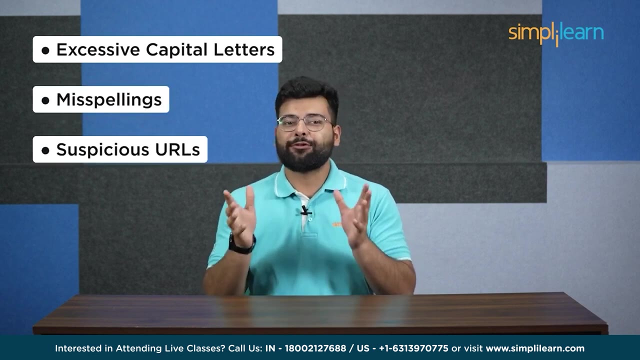 lives. But fear not. a hero emerges: the email spam classifier. This intelligent system learns from past encounters, uncovering the tricks employed by spammers: Deceitful subject lines, promising reaches, unreasonable low prices. It sports signs like excessive capital letters, misspellings and suspicious URLs. 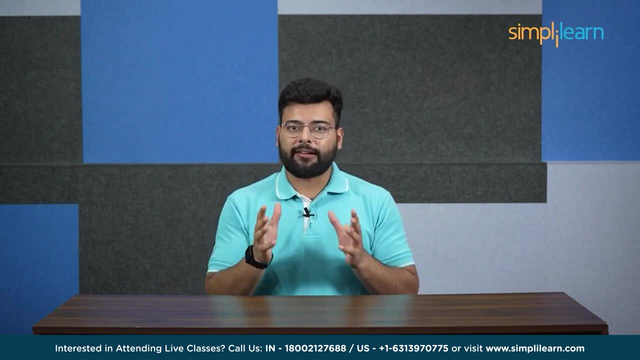 Yet the battle doesn't end here. Spammers constantly evolve their tactics, but the email spam classifier doesn't flinch. It adapts, refining its knowledge and staying up to date with the latest tricks. Every new spam email it encounters, it provides insights, enhancing its accuracy and ensuring 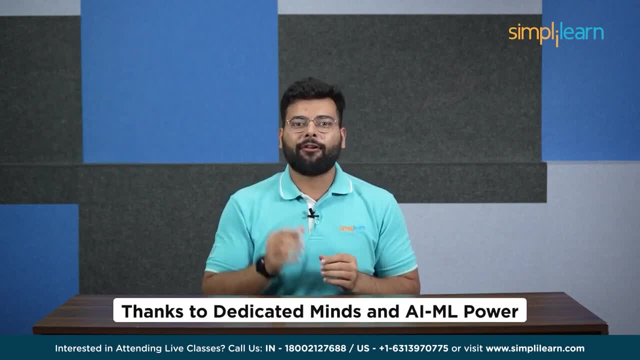 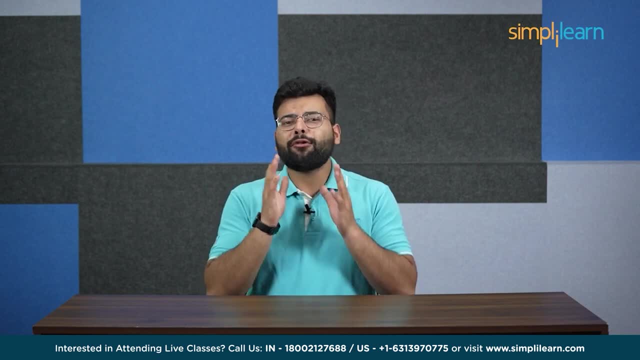 our protection. Thanks to dedicated minds and AI and ML power, the fight against email spam continues. The email spam classifier stands as our faithful guardian, a symbol of technology's victory over digital adversaries. It reclaims our inboxes and restores our privacy. 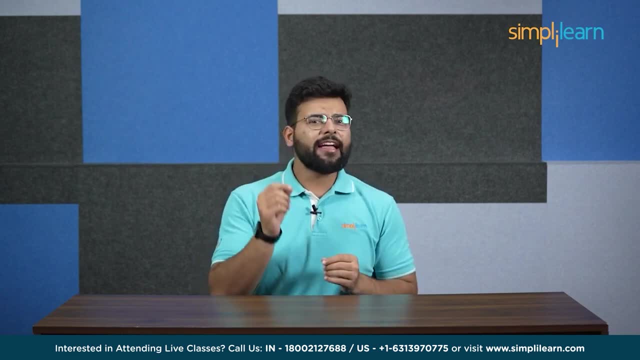 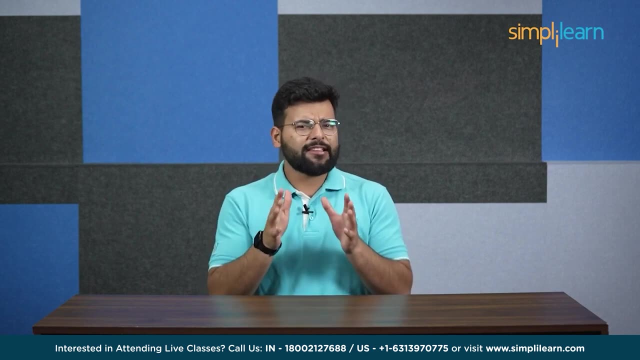 It is our future, for all of us. According to recent studies, AI and ML related job postings have increased by a staggering 344% in the past 5 years. Companies across the globe are actively seeking professionals who can harness the power of data and build intelligent systems. The average salary is $150,000 in the US and 15 lakhs per annum in India. Accelerate your career in AI and ML with our comprehensive postgraduate program in AI and ML: expertise in machine learning, deep learning, NLP, computer vision and reinforcement learning. 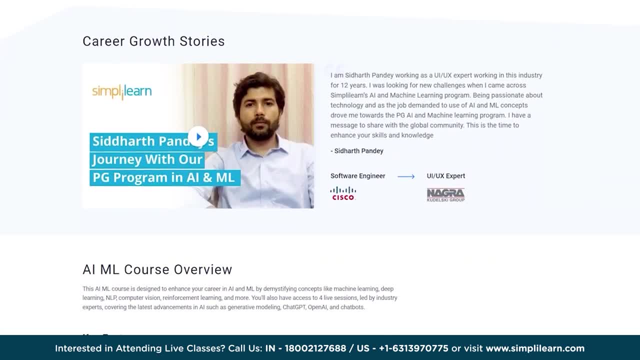 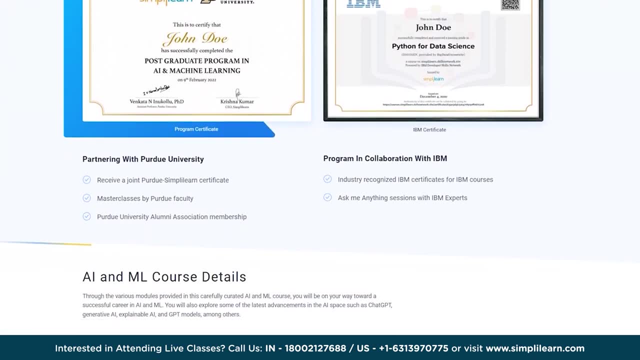 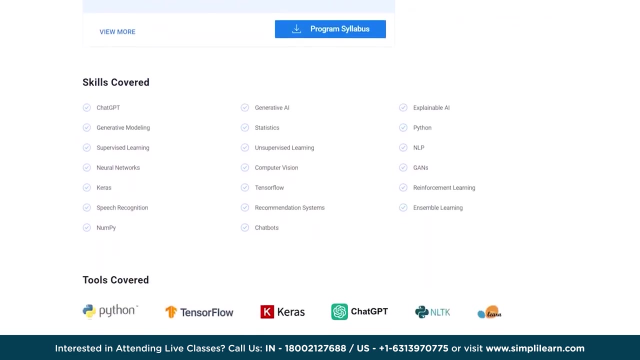 You will receive a prestigious certificate, exclusive alumni membership and hackathons and ask-me-anything sessions by IBM, With 3 capstones and 25-plus industry projects using real datasets from Twitter, Uber and more. you will gain practical experience, masterclasses by Purdue faculty and IBM experts. 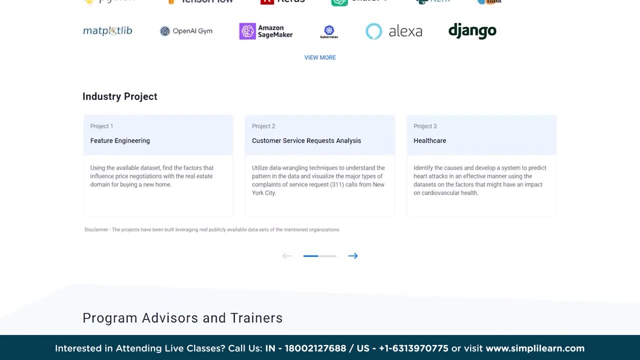 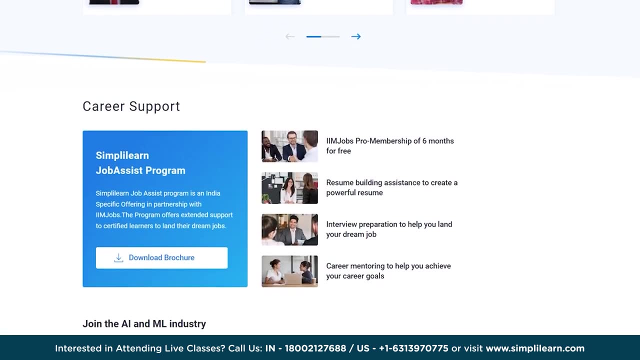 ensure top-notch education. SimpliLens Job Assist helps you notice by leading companies, live sessions on AI trends like ChatGPT, Generative AI and Explainable AI. This program calls statistics, Python, supervised and unsupervised learning, NLP, neural networks. 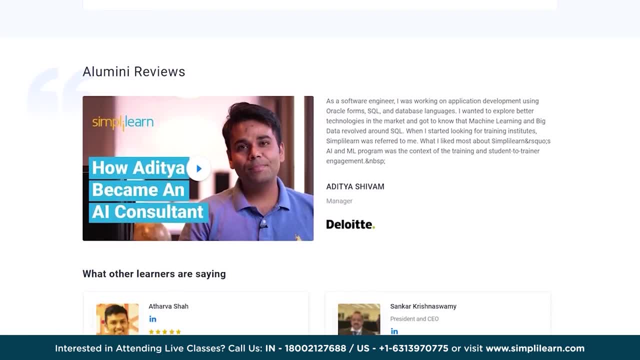 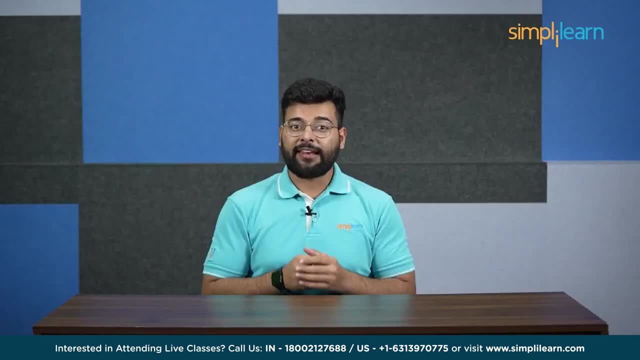 computer vision, GANs, Keras, TensorFlow and many more skills And roll now and unlock exciting AI and ML opportunities. The link is mentioned in the description box below. Let's take a minute to hear from our learners who have experienced massive success in their 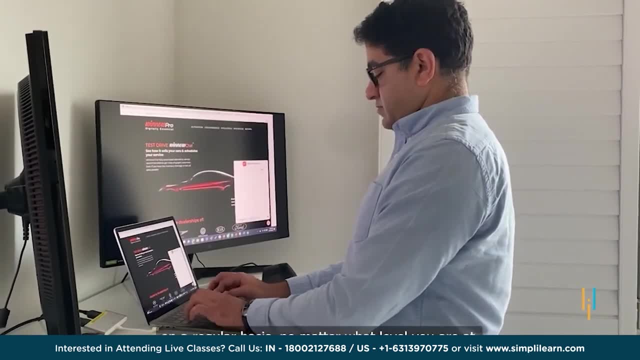 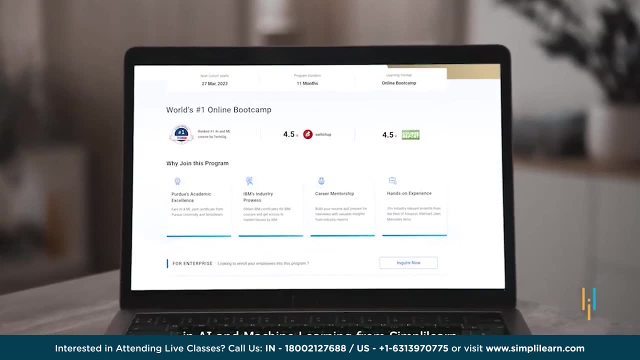 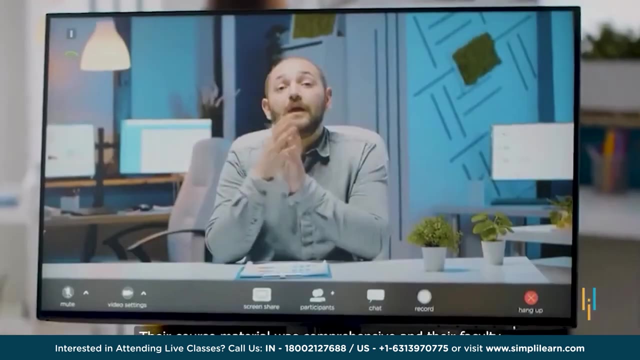 career, You need to keep updating your skills on a regular basis, no matter what level you are at. I recently completed the professional certificate program in AI and machine learning from SimpliLens in partnership with Purdue University. The course material was comprehensive and the faculty was extremely experienced. 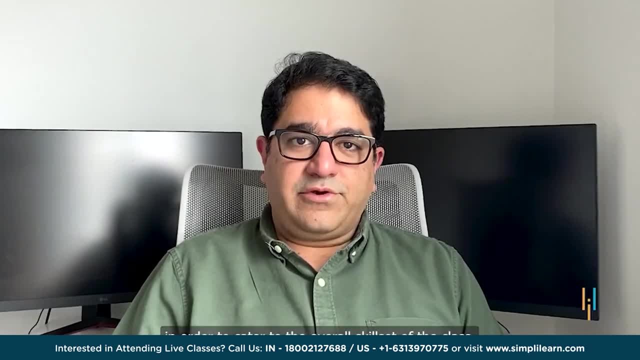 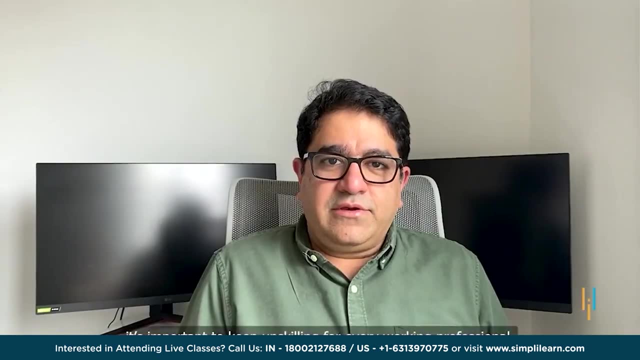 The faculty was able to adjust their teaching style in order to cater to the overall skill set of the class. In the rapidly evolving world of technology, It's important to keep upskilling for every working professional Stay relevant. Continue With that. having said, 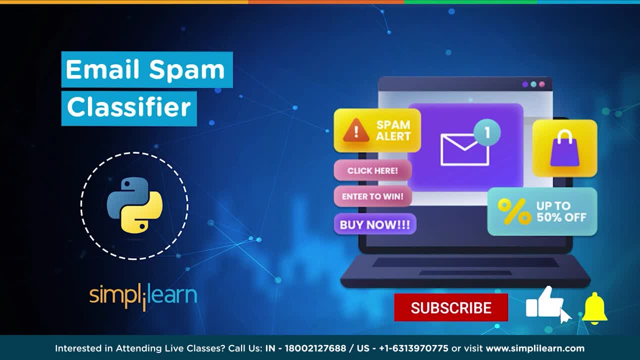 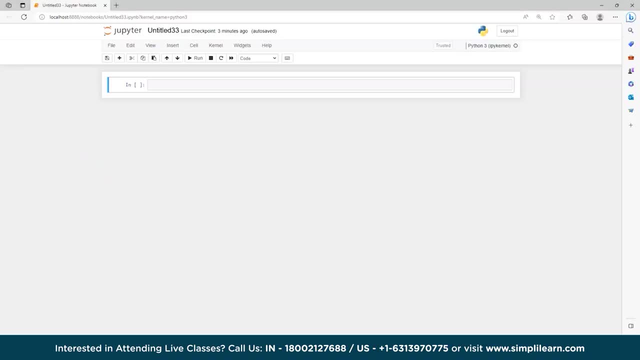 Hey everyone, welcome to SimpliLens YouTube channel. But before we dive into that, don't forget to like, subscribe and share. And now over to our training experts. So hello and welcome to this new video by SimpliLens email spam classifier. 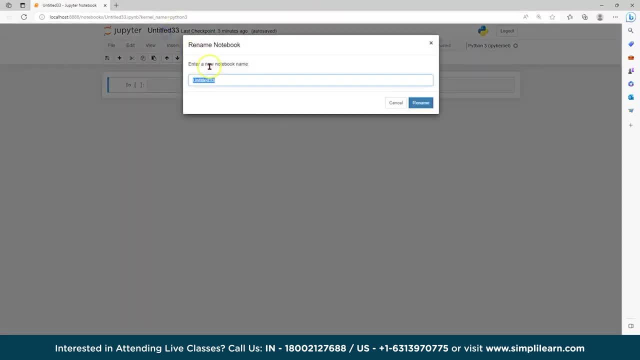 Okay, So first we will change this name to email spam classifier. Okay, So first we will change this name to email spam classifier. Okay, So first we will change this name to email spam classifier. Okay, That's it. That's it. 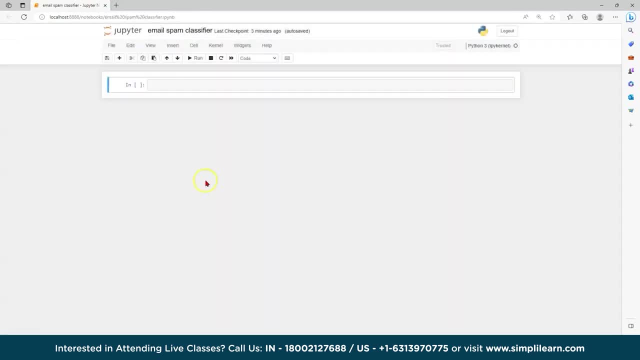 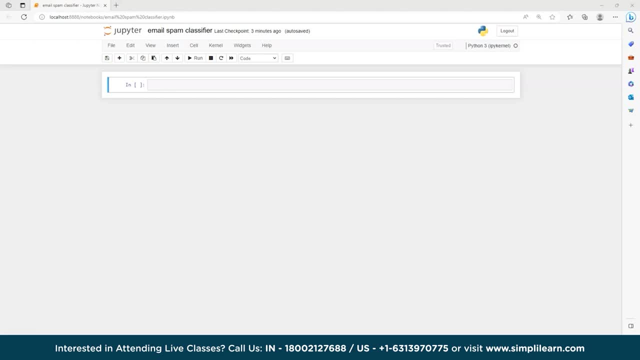 and logistic regression algorithm And then we will move on to this importing of data set of spam mail and ham mail. Ham is known as like, which is not spam spam. okay, so we will do some categorization of spam email and ham email. then we will split into the training, test and testing of the data. 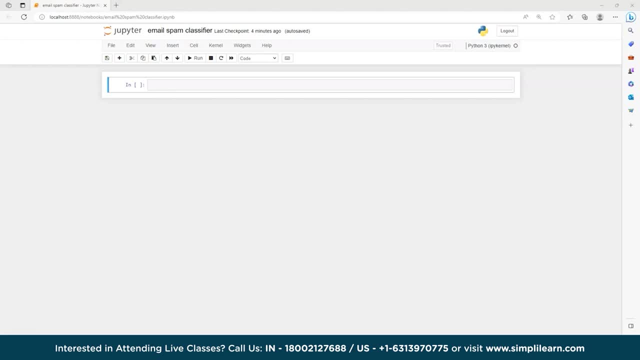 set okay, then we will transform the text data to feature vectors that can be used as input to the logistic regression and then we will convert the white train and the white test values as integers and then, moving forward, we will some see the features, the model extractions, and then we will train the model using logistic. 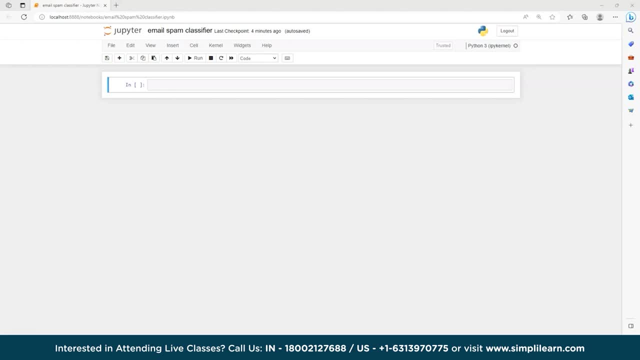 regression and after that we will predict the accuracy- how was the training data is giving, how much the testing data is giving, and at the end we will build a predictive system which will tell whether a particular email is spam or not spam. okay, cool, so let's move on to the coding part then. okay, so first. 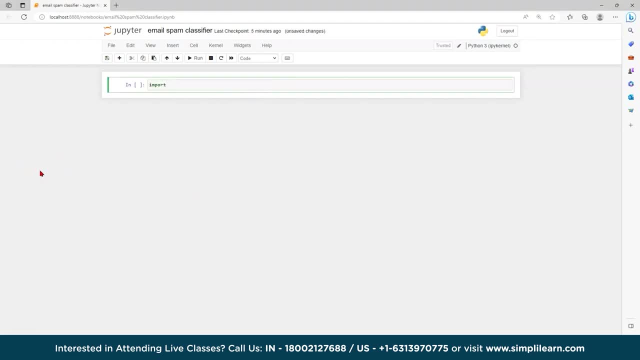 I will import some major lab is like import some major lab is like import some major lab is like import some major, important languages. like import some major languages. like import some major port numpy as np. okay then numpy. so numpy is a powerful python library for numerical computing. 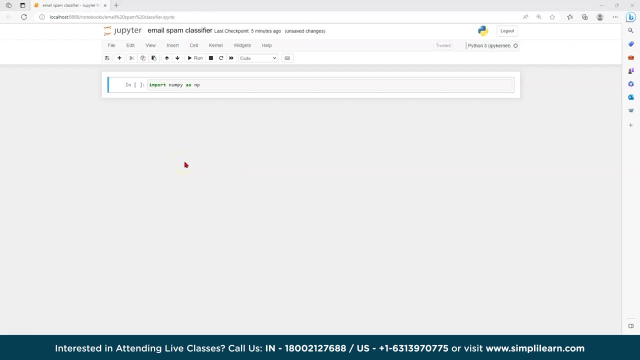 so it stands for numerical python and provides support for efficient array operations and mathematical function, linear algebra, random number generation and more. with numpy, you can work with the multi-dimensional array known as nders, and these arrays are highly optimized for performance and allow you to perform mathematical and logical operations on large data set efficiently. 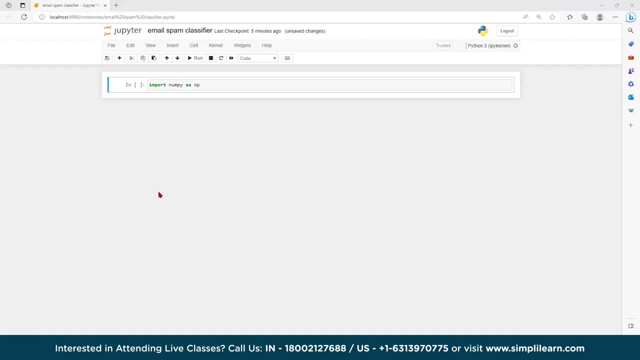 so numpy provides a wide range of function and methods to manipulate and analyze these areas. and the second one is import pandas as pd. okay, this pd and np is nothing. We don't want to write again and again pandas and numpy. So what is pandas? So pandas is a powerful Python library used for data manipulation and analysis. 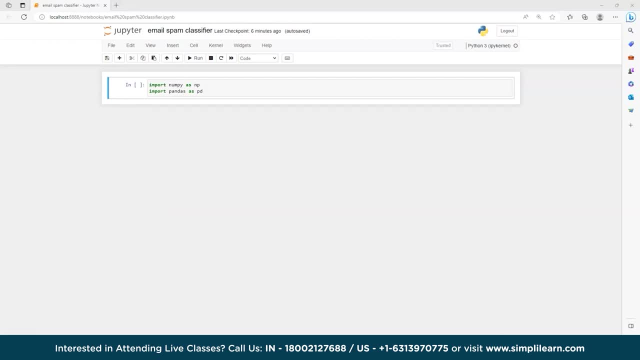 It provides easy to use data structure and data analysis tool, making it essential tool for working with structured data. So the third one is scikit-learn. So I will write here from scikit-learnmodel selection report: train test split. So what is scikit-learn? model selection and the train test split. 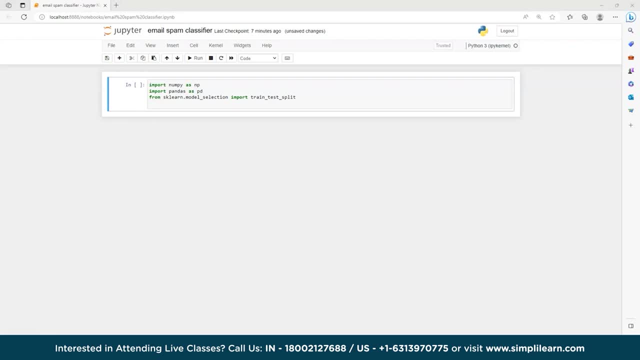 So scikit-learn. So? scikit-learn is a popular Python library for machine learning. It provides a wide range of tools and algorithms for various machine learning tasks, including classification, regression and that, clustering, dimensionally reduction and the model evaluation. 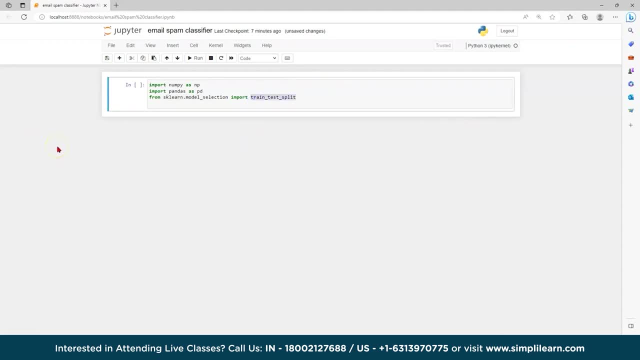 And this train test split this one. So the train test split function is a utility in scikit-learn that helps in splitting the data set into training and the testing subset. Later we will split the data into training and the testing subset, So this function is commonly used in machine learning tasks to assess the performance of. 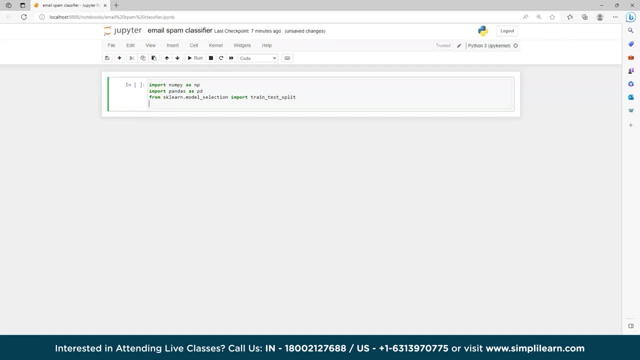 a model on unseen data. Okay, so move on to the next algorithm we will write from. we will write here from scikit-learnfeatureextensiontest. So this function is commonly used in machine learning tasks to assess the performance of a model on unseen data. 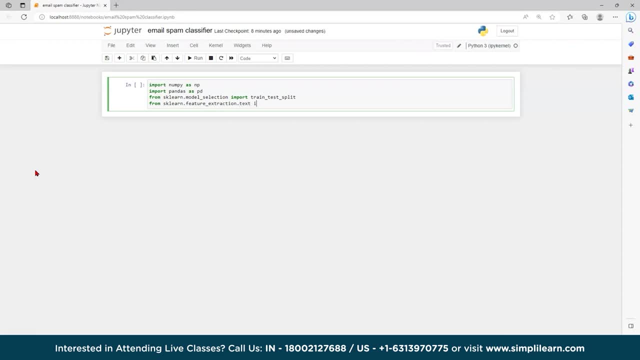 Okay, So move on to the next algorithm. This is called tfid-vectorizer. tfid-vectorizer- Text import- tfid-vectorizer- Text import- tfid-vectorizer. Okay, So what is tfid-vectorizer? So tfid-vectorizer is a feature of extraction technique commonly used in natural language. 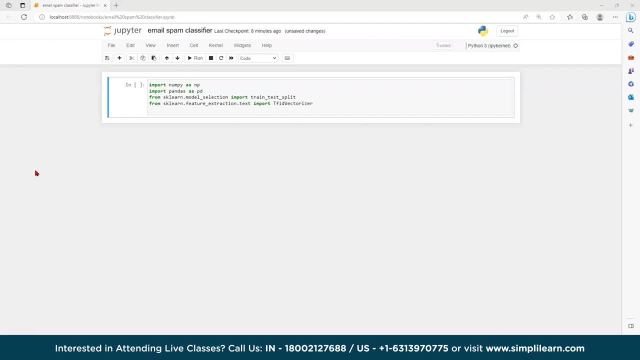 processing and text mining task. So it is a part of scikit-learn library. in python, so tfid vectorizer transform a collection of text document into a numerical representation that machine learning algorithm can work with. So move on to: we will import from a scikit-learn dot linear model import logistic regression. 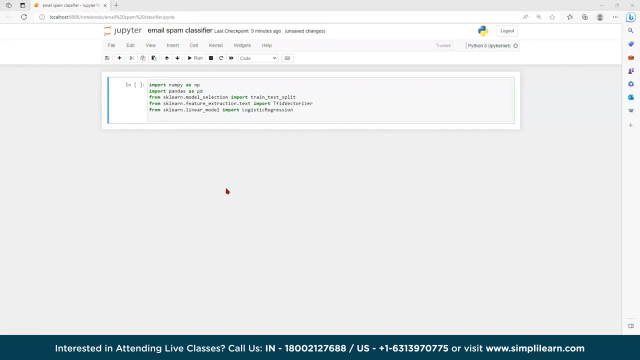 So what is logistic regression? So logistic regression is a popular classification algorithm Used in machine learning. it is a part of the scikit-learn library in python, Logistic learn, and the regression is suitable for binary classification problems where the target variable has the two classes. 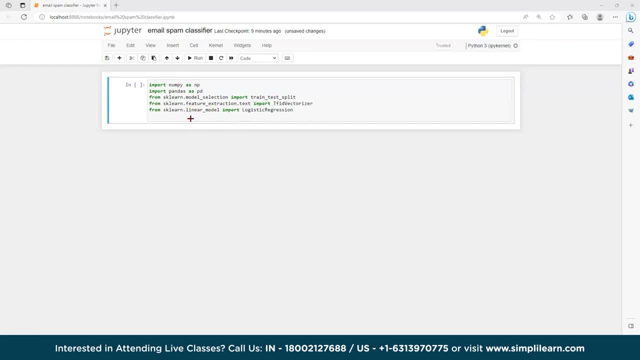 And the last, we will import accuracy score. So here I will write from sklearn dot metrics. So let me tell you first what is accuracy score. the accuracy score function is a performance metric provided by the scikit-learn library in python. It is commonly used to evaluate the performance of a classification model by measuring the 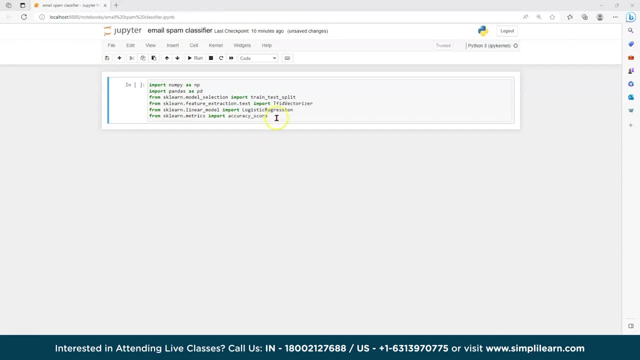 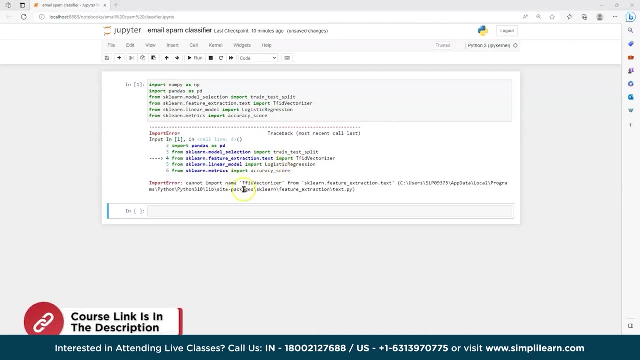 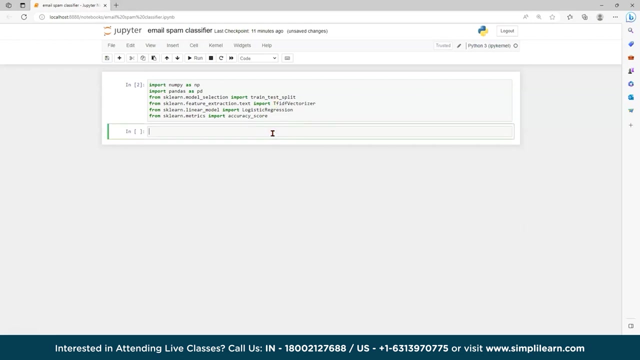 accuracy of the predictions. So let me run it. So let me run it. Okay, there is some error, maybe the spelling mistake. okay, what I will do, I will write it again. running it again. yeah, it's working. So now what I will do, I will import the data set. 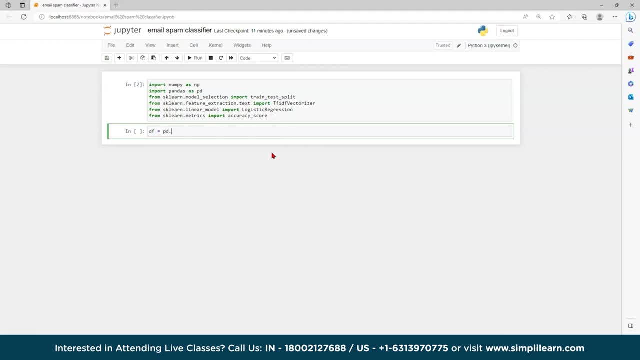 So I will write here: df equals to data frame. equals to pd dot. read underscore c: Okay, CSV mail underscore data dot- CSV. You can find this data set link in the description box below. okay, I will run it. yeah, So let's see the data frame. what's in it for us? 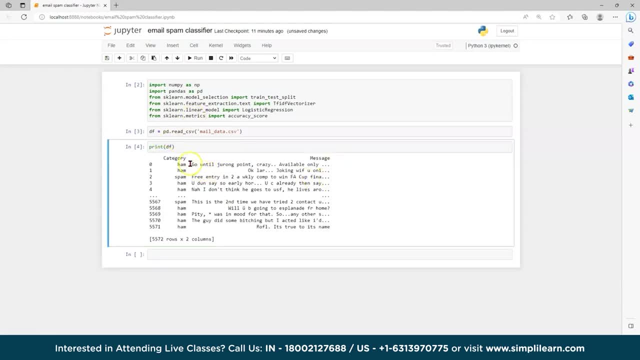 So, as you can see, here is category, then message. so these are the you know the mails. ham means not spam and spam is spam. okay, Those mails which are not spam known as ham. So there are two columns, five, five, seven, two rows. 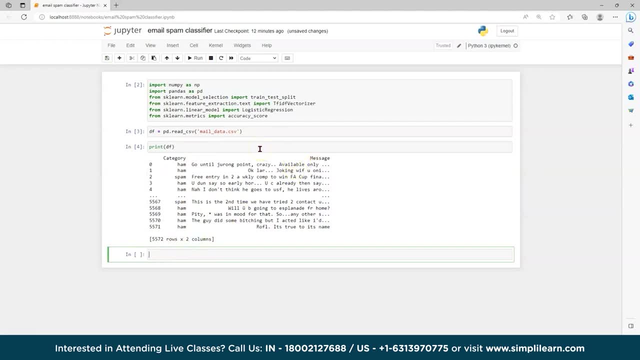 So, moving forward, what I will do? I will convert this mail data okay to not null. So I will write here: data equals to raw, not raw Data. equals to raw, not raw Data. equals to df dot, where pd dot not null, not null is df. 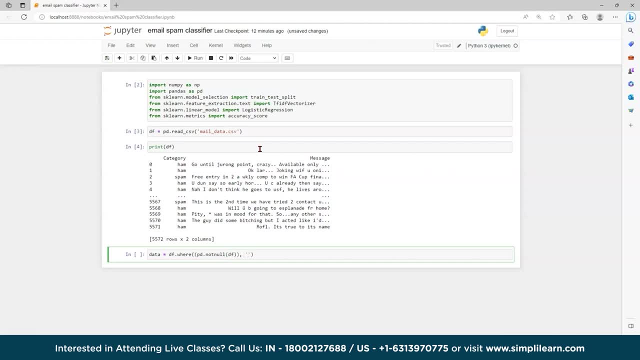 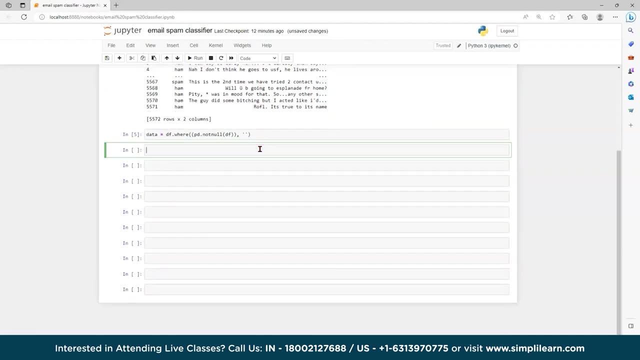 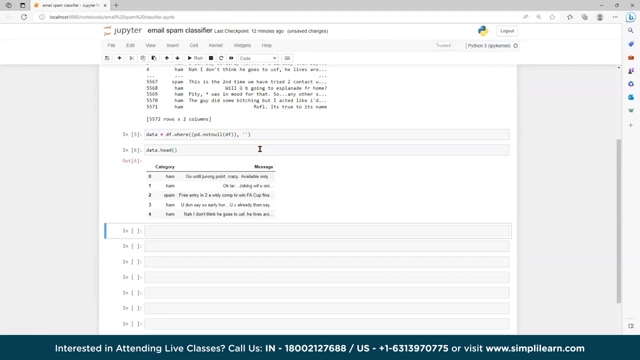 Okay, Then. okay, let me give you some spaces for the better visual. yeah, So now I will print data dot. Okay, Okay. So what is the meaning of head here? head means if you want to print the top five lines of the particular data set it is, you can use the head. 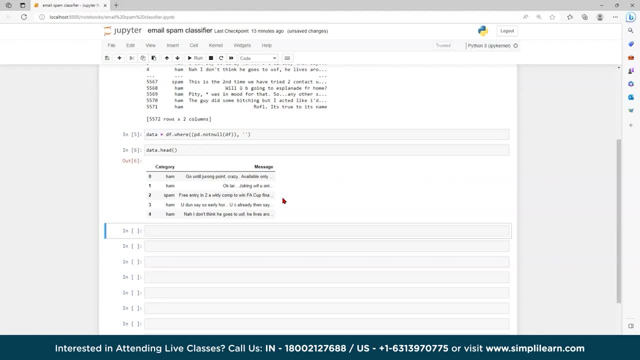 And if you want to print the last five rows of the data set so you can use the tail instead, If you will write here 10, instead of giving it blank, then run it So it will give you the top 10 rows of the particular data set. 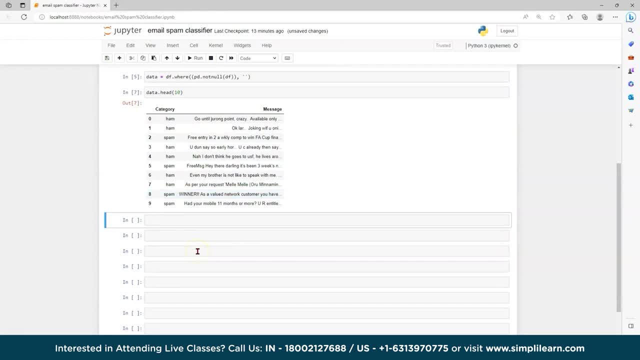 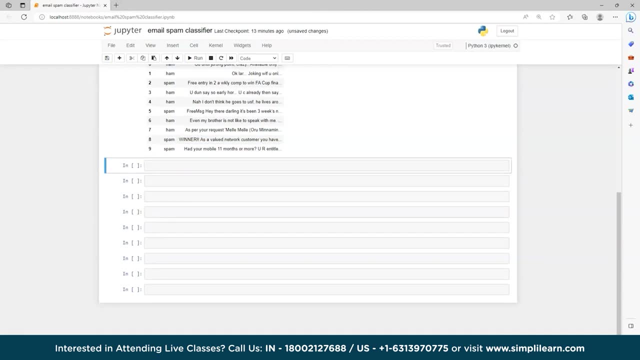 Okay, So that's it. Okay, So that's it for this spam mail, this ham mails. So later on, what we will do, we will train this data set using this particular data set. Okay, So let's move on to and see the info. okay, of the data set. so data dot info. 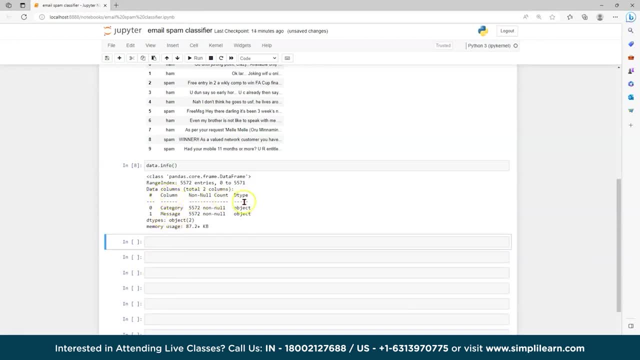 So info: you can see there are columns this null, null, count, this data type. So there are two columns like categories, See, and the message and the particular rows are the 5572 on the both and the data type is object. 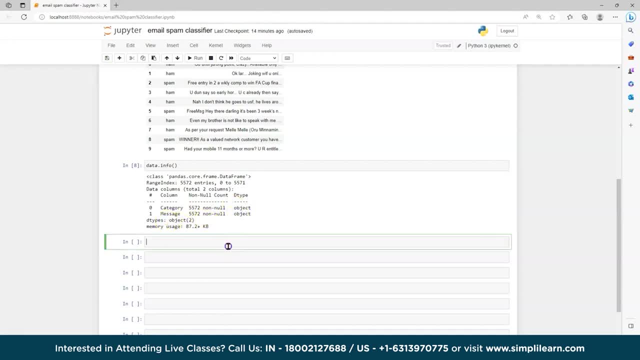 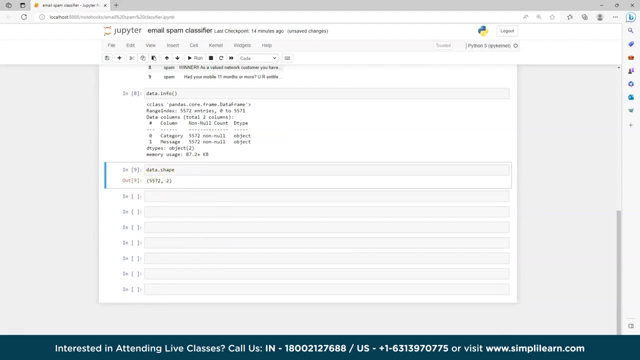 Okay, See the memory usage and you can see everything. And there is one more. you can see that it shape is 5572, comma two. these are the rows and these are the columns: two columns and 5572 rows. Okay. 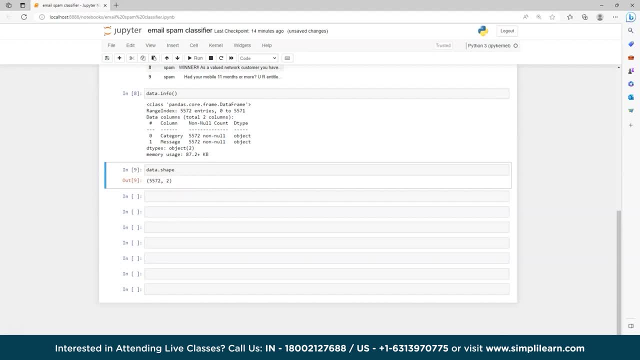 So now what I will do. I will assign the category to spam. Okay, So I will assign the category to spam am and ham mail. Okay, So what I will do here. I will write here: data dot loc. than data versus category equals. 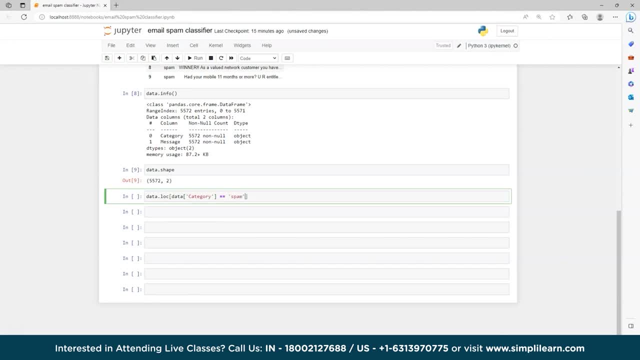 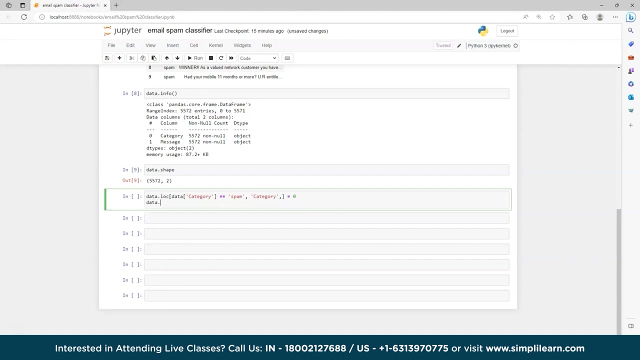 to equals to spam comma category. Okay, So, that's it. Okay, So, that's it, Okay. So I now Everything will be floor ette. So if the zero will show, it is known at this spam, And if one will show it is known as the ham mail. 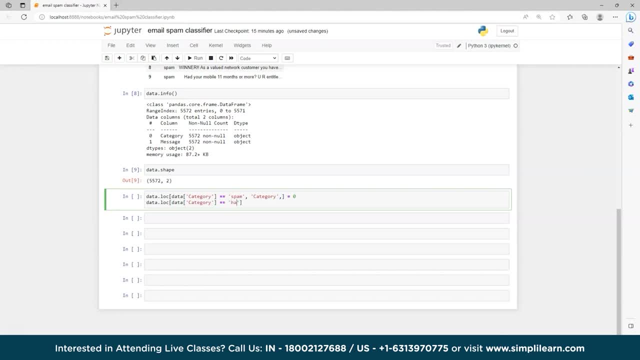 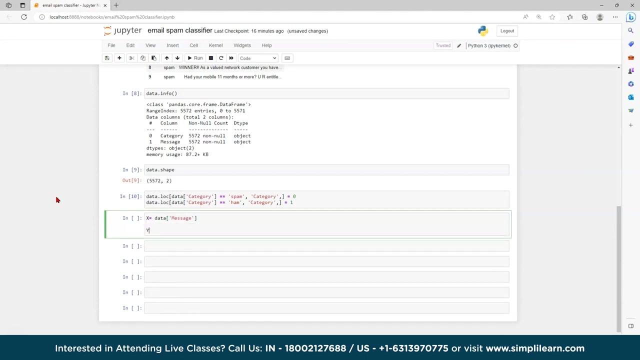 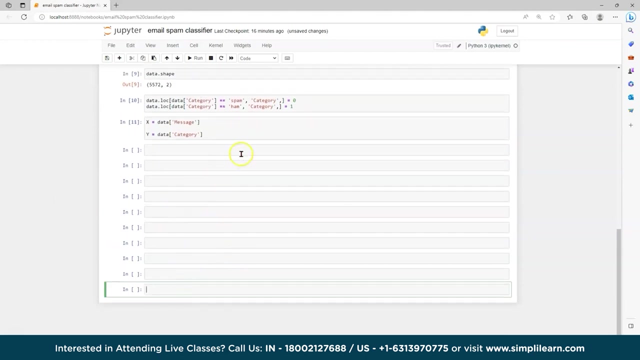 Okay, I will write here. okay, then let me run it. okay, it's running smoothly, so I will write here: X equals to data, then message, and the Y value will be data, then category. okay, then let me run it. so now what I will do first. so now what I will do. I will write a print: X, okay, so 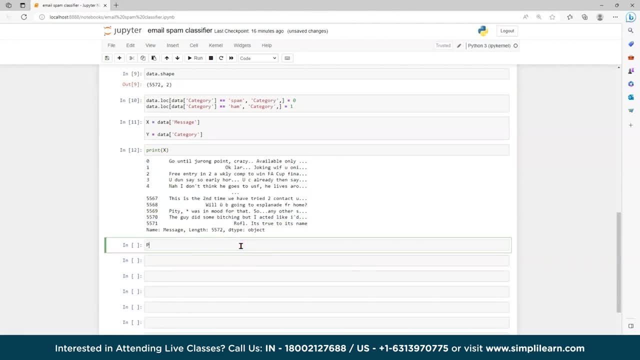 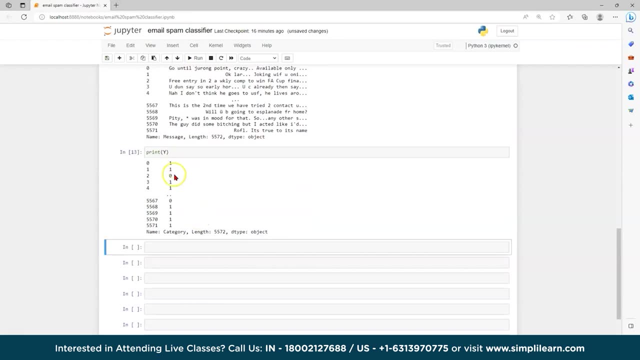 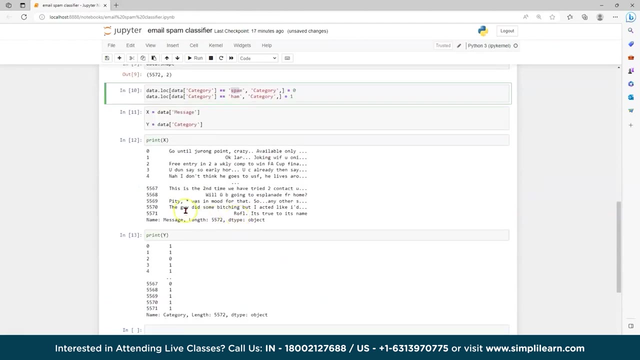 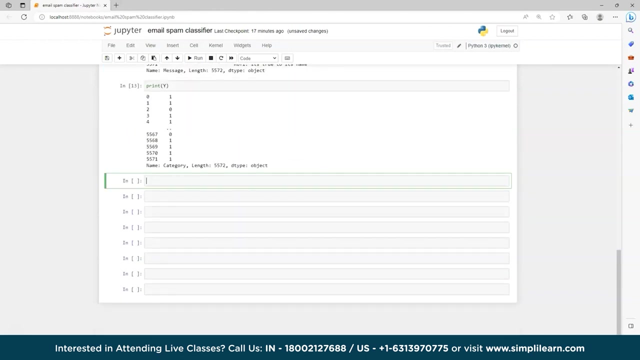 these are only the messages and category print Y. so now, as you can see, one one zero, one one zero. so here, zero means what is the zero means? zero means is spam and the one means it's hamlet. okay, so moving forward, what I will do, I will. 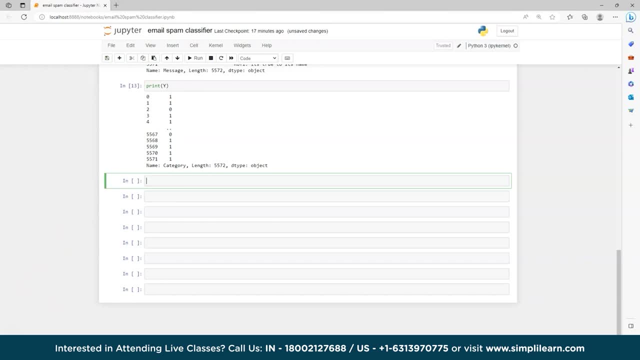 split this data set into testing and the training. okay, so I will write here: X train- this is the most important part- and the X test. okay, then Y train, then Y train, use string 100 words. then Y train is higher than X train, then Y train is lower than X train and Y train is order1. so all words come first. 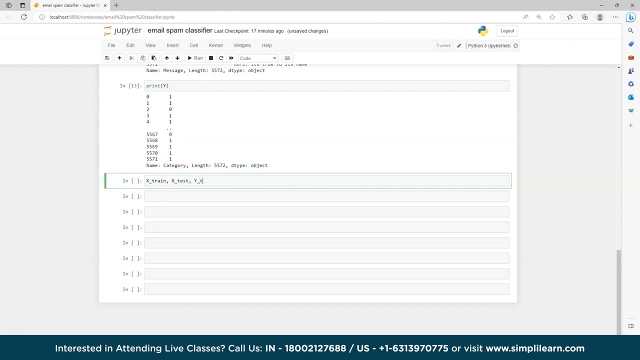 okay then why train? then why, okay, because you train test X comma, Y comma. test size equals to 0.2, then random: okay, random state equals to 3. okay, I will run. so this is. test size equals to 0.2, then random state equals to 3. okay, I will run. so this is. 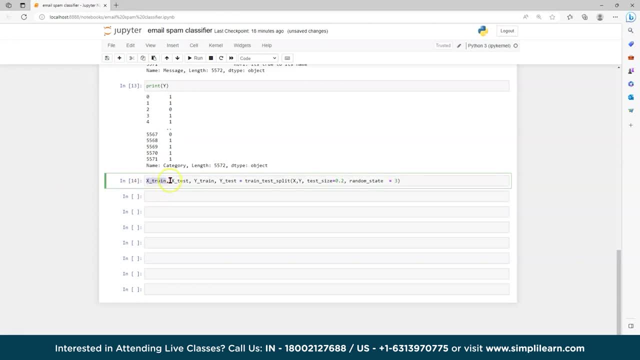 X train for the training set and X test is the testing. okay, then the same Y. you know the. what is the X and Y here? and here we are the splitting using train test display. then X comma Y test size is equal to 0.2. okay, 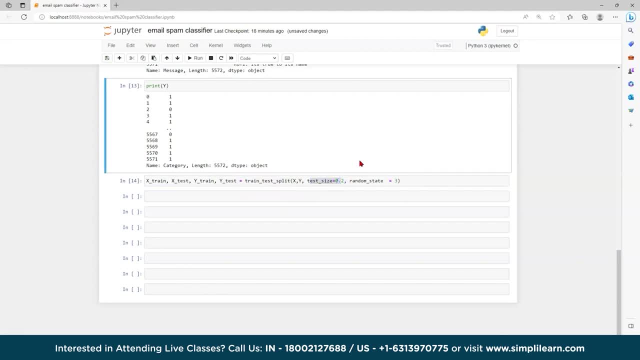 0.2 means it will be 80 and 20 percent, and 80 percent will be training and the testing will be 20 percent. okay, we will train data. 80 percent of data using this data set will be trained and the for the test, the 20. 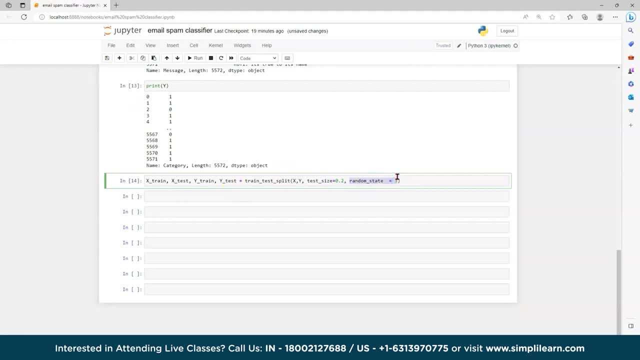 percent will data? okay, the random state equals to 3 and the random state is a hyper parameter is used to control any such randomness involved in machine learning model to get consistent result. okay, when splitting a data set is splitting a node in a decision tree or a, you know, logistic regression in 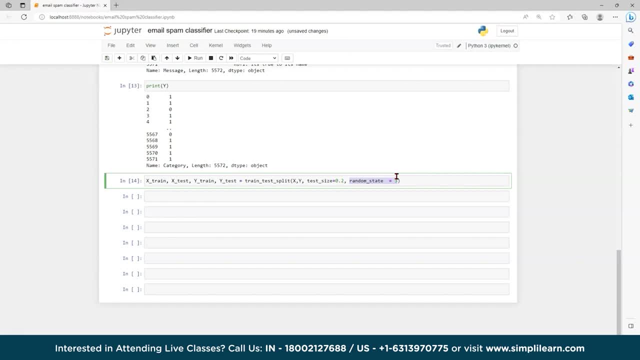 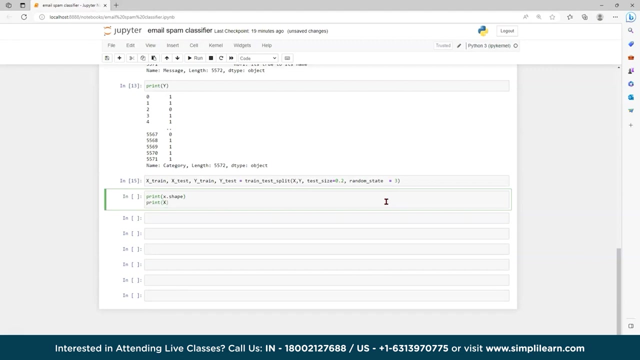 analyzing centroids in clustering takes place, so that is why we use random state. okay, so let me run it. it's working fine. so now I will show print X- dot ship. okay, then print X- underscore- train- dot ship. I will show you about the. I'm talking about a. 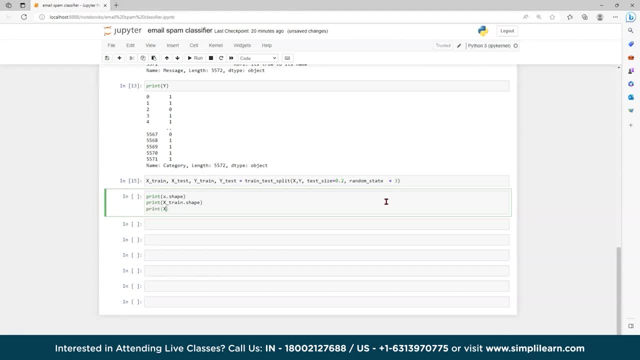 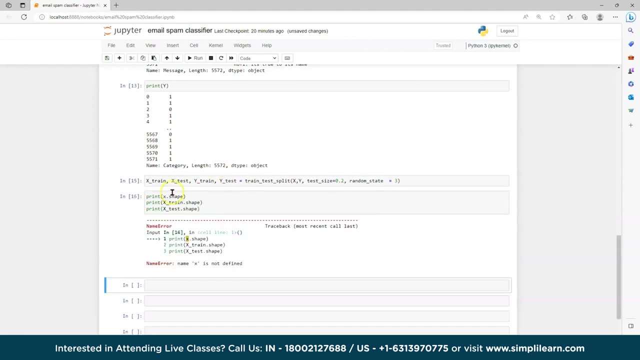 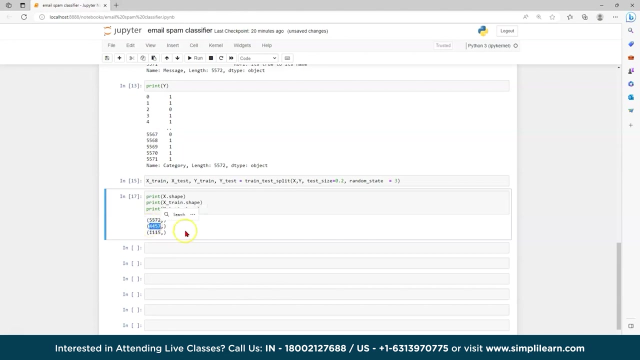 test size of the mind that I just has no print X underscore test. now see carefully. okay, so, as you can see, total rows are 5, 5, 7, 2. total row of 80 percent is four, four, five, seven, or else you can calculate, and the 20% is for the testing. 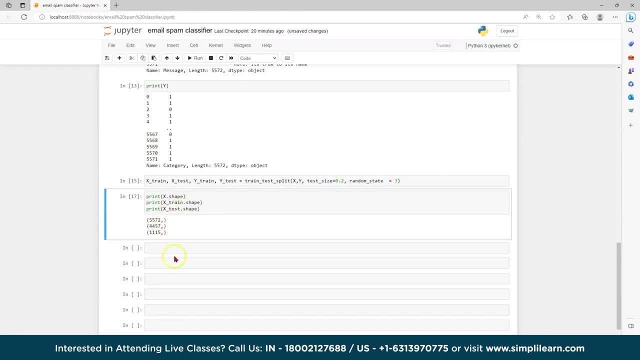 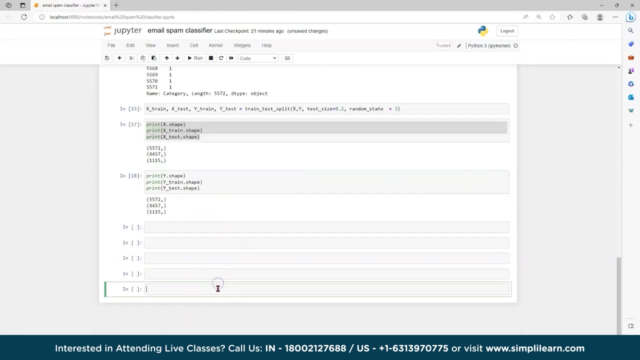 test is that the tョ g кол我們 one triple one, five. same goes for the y. so moving forward, okay, let me show you for the y also, so i will copy paste it here. so let's y, y, y. see, same goes for the y also. okay, so now what i will do. 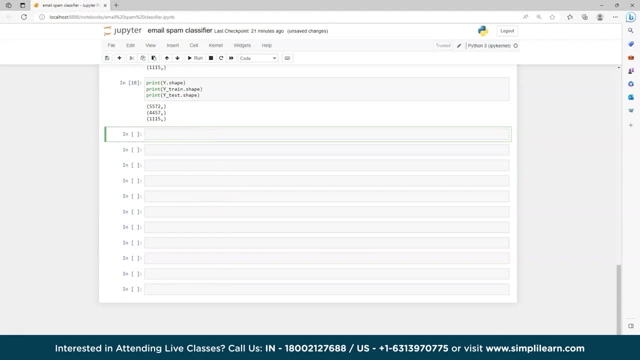 here i will transform the text data to feature vectors that can be used as input to the logistic regression. so feature extraction equals to t f id vectorizer: okay, the minimum difference will be one comma stop words. okay, stop words equals to english and lowercase. okay, here i am transforming the test data to the feature vector. 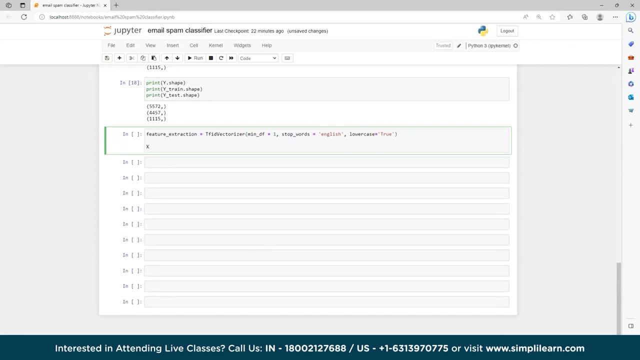 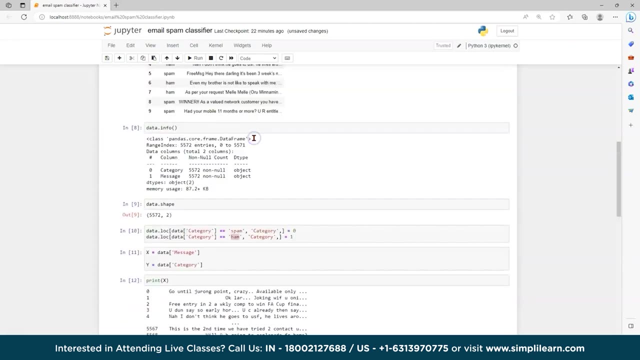 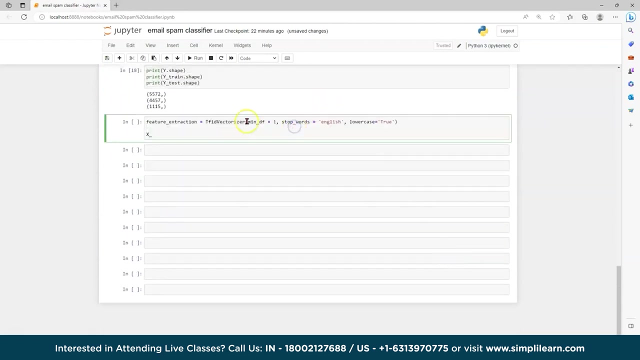 and okay. so here x. okay, let me tell you. so this is a feature extension. we are using tf devectorizer. okay, we have import here, as you can see, for the feature extension of the text, and this is the minimum difference, equal to one. and then, what is the stop word? the stop words are: 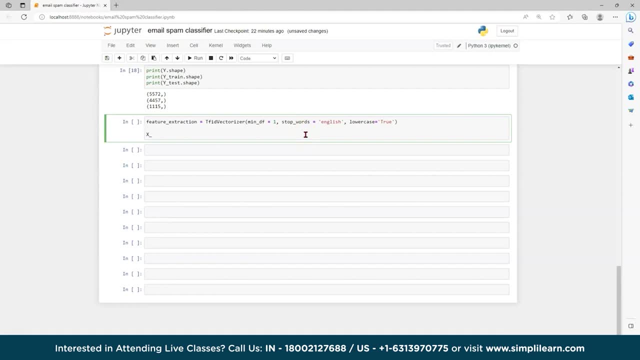 the english words which does not add much meaning to the sentence, they can safely being ignored without sacrificing the meaning of the sentence. okay, like, for example: you can see the words like the. he have such words already computerized and the captured. this is a corpus name and the corp. 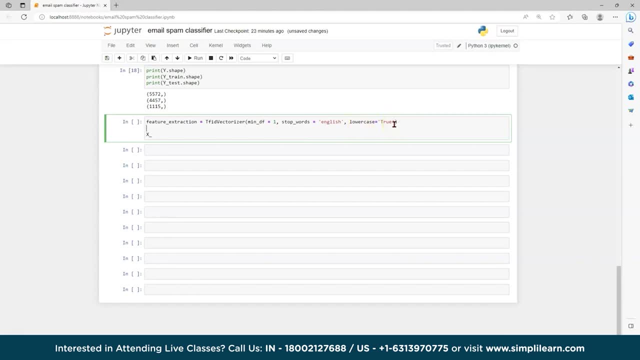 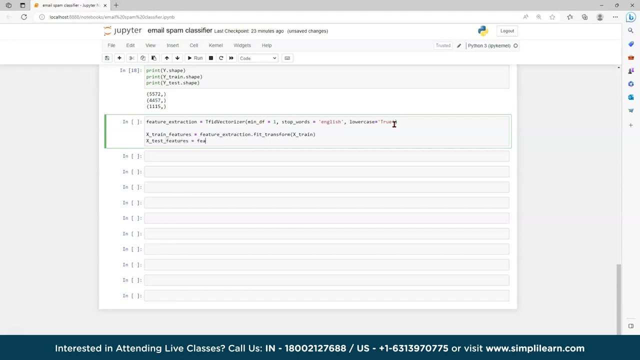 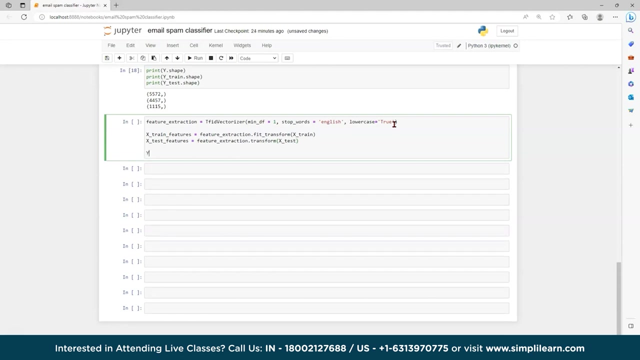 okay, and this lowercase equals to two. true, so here i will write: x- train features- question features. feature extraction dot. fit. transform. x underscore. x underscore test features: feature extraction dot. transform to the x text: okay, yeah, so moving forward, i will convert y train and y test values as an integer. okay, y train. 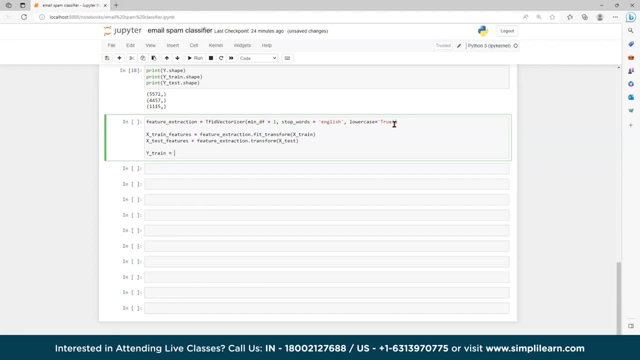 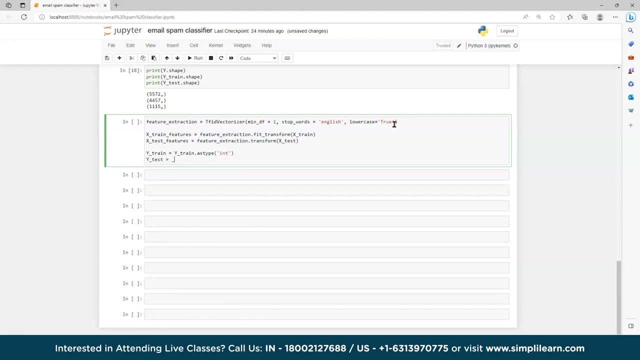 because they are zero. one zero and zero train equals to y train dot a style. okay, and okay, then y test equals to y test dot as type. y test dot as type is equal to y train dot as type. okay, then y test is equal to y test dot as type. 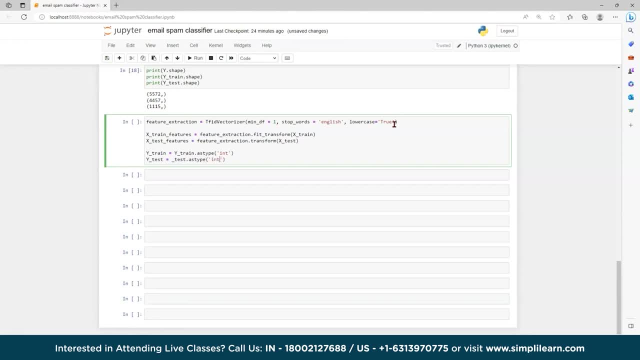 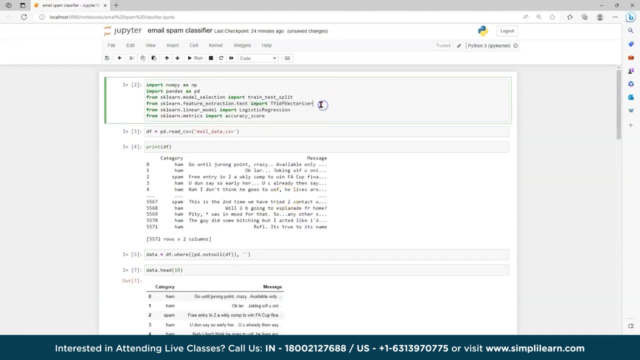 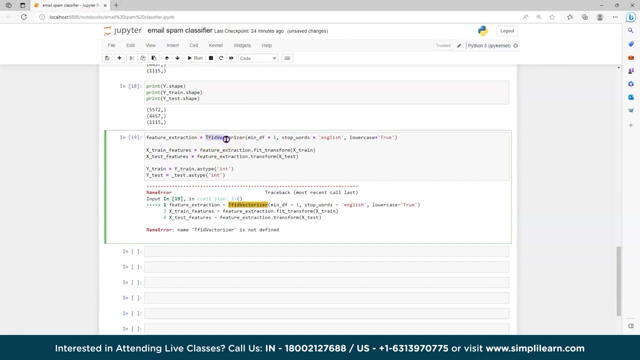 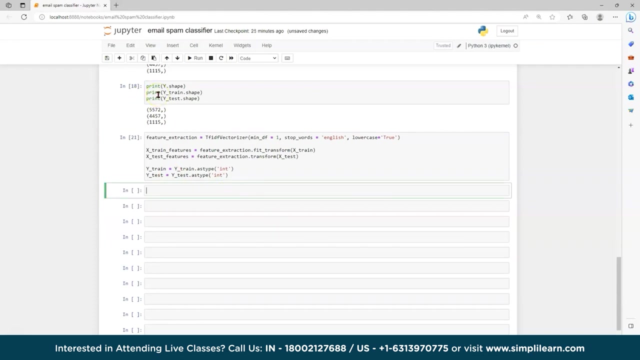 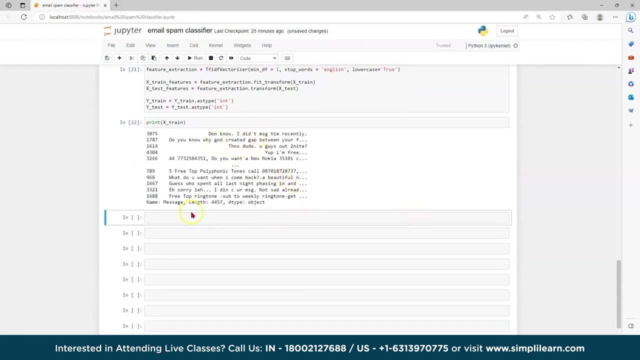 so, okay, spelling mistake. will copy from here, paste it here. okay, then i will run it. okay, y test it is. yeah, it's running. so now what i will do. i will print the x train train, as you can see the x train. so these are the messages and if i will print. 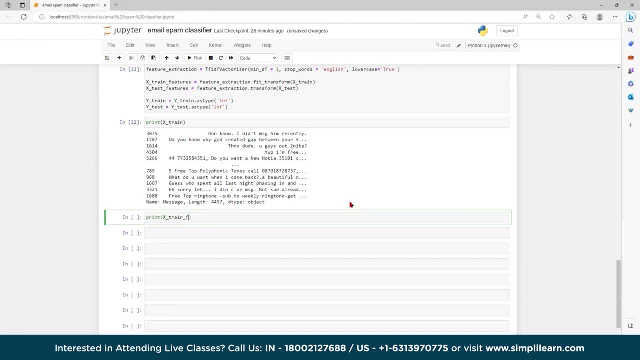 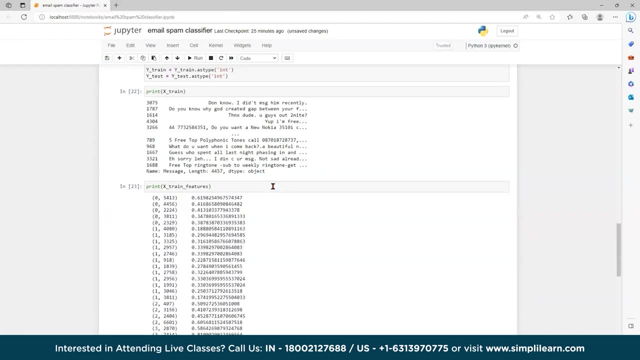 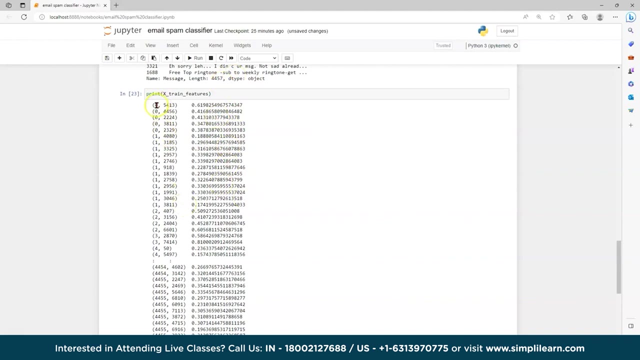 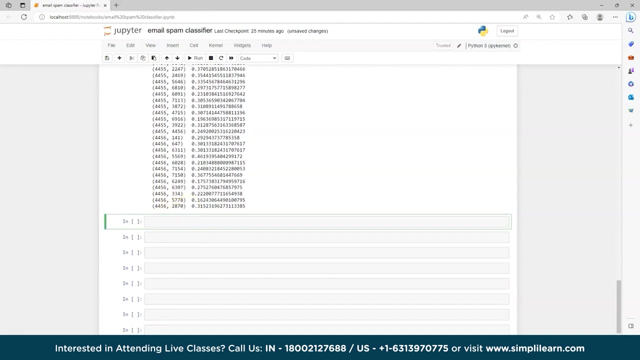 x train features we created here. now see extend features. okay, then you can see. so these are the features. accuracy: okay, since zero, zero, zero means spam, one, one mean m. okay, so moving forward, what i will do? i will now train the model. okay, logistic regression. so i will write here: model equals to okay, logistic. 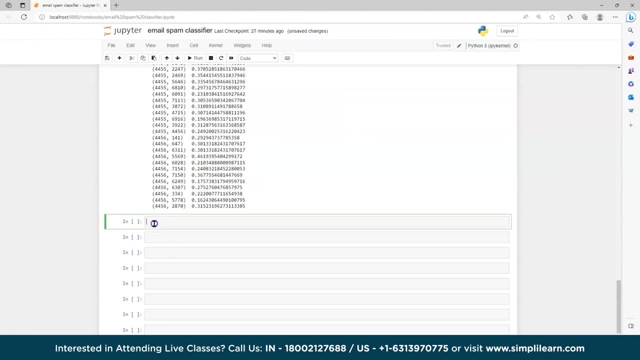 regression. so now we will, you know, train the model. so here i will write: model equals to logistic regression. okay, so we don't want to write again and again, again and again logistic reaction. so i am here assigning model to it, so let me run it. so here i will train the logistic. 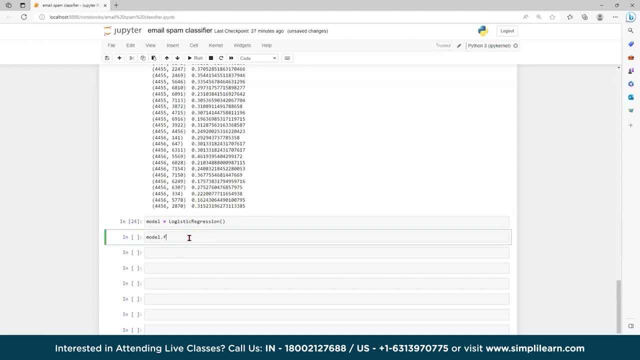 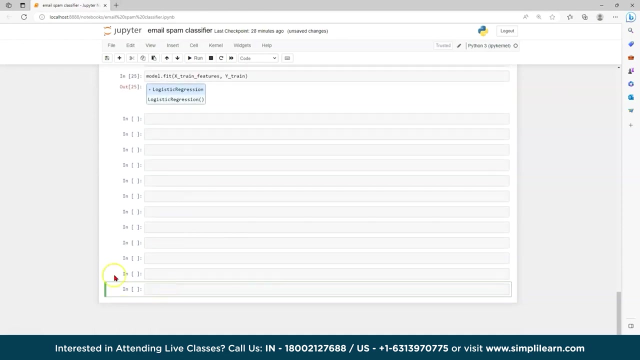 regression model with the training data. so here i will like model dot fit x train features, comma y train. okay, here we are training the logistic regression model with the training data. let me run it. yeah fine, it's running fine. so moving forward, we will do the evaluating of the training model, train model and the 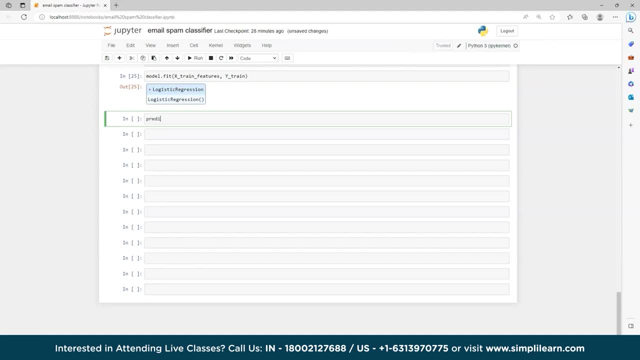 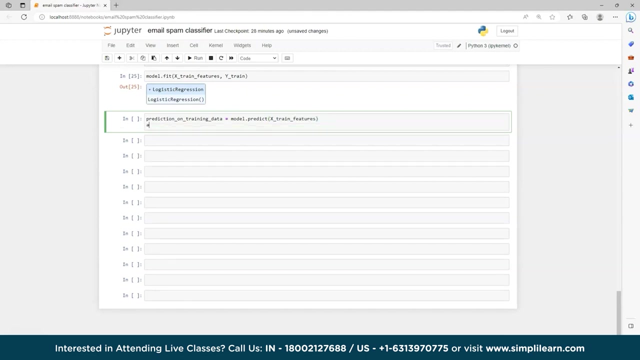 prediction of the training data. so for that i will add here prediction on training data. model: dot predict x train features. okay, then i will write here: accuracy training data, accuracy score. y train comma prediction. okay, i will write from here. okay, let me run it. so now we will see the prediction, so i'll write here prediction. 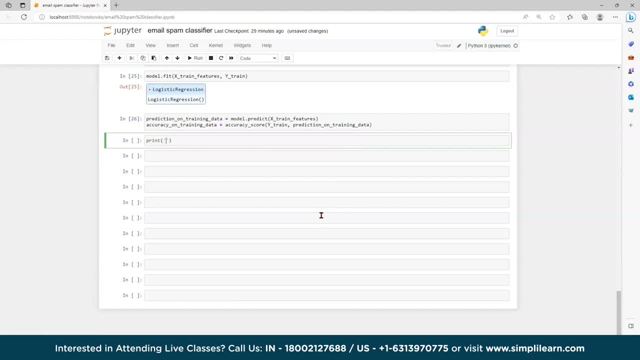 or simply i will write print: accuracy, patter comma, accuracy, data commitment. so, as you can see, accuracy on training data is 0.96 means this x is always rushed like normal training. so you may find that, or you, you may, maybe cumin and bl tama. you can at least find this one, but if you apply it, yaa. 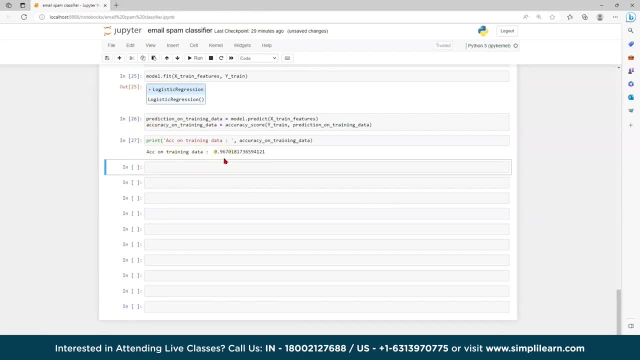 so, as you can see, accuracy on training data is 0.96. main see accuracy on training data is 0.9- is also to make sure that is working. règckament Einal mean: it is correct: in86 10 less than 6. if it works outside the current time and Let me do this so, as you can see, accuracy on training data is 0.96 means. 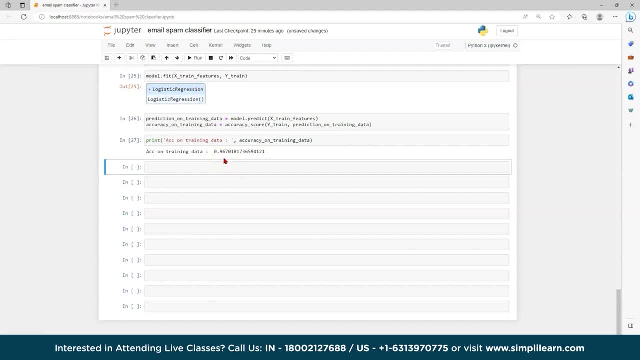 almost 97%, which is not bad, very, very good. okay, we will see print. okay, now we have to do for the testing data. this is for the training data and let's see the accuracy for the testing data. so for that I like same prediction test data. 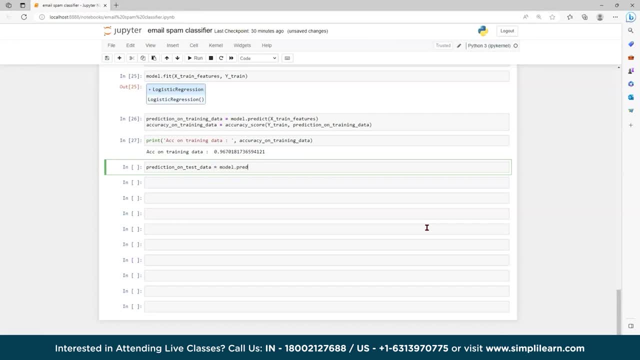 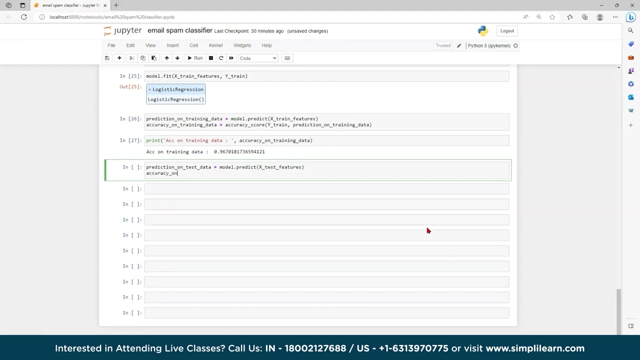 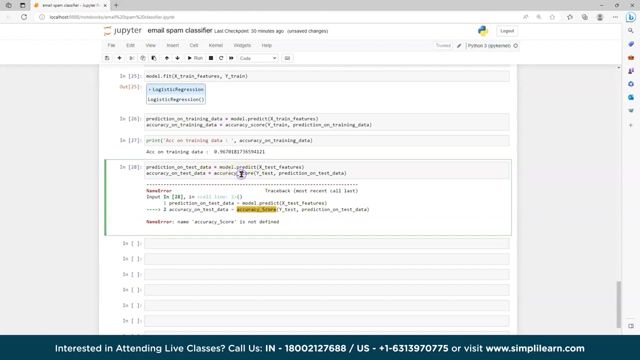 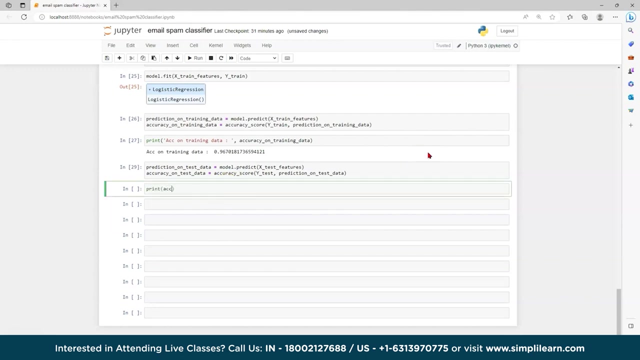 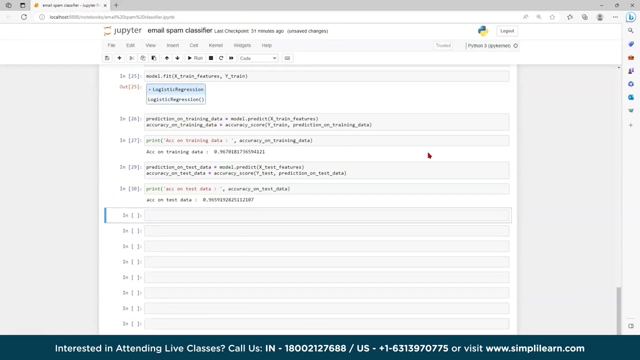 equals to model dot: predict X test features. accuracy on test data equals to accuracy score, then y test score, then y test prediction on test data. okay, so here I will write: print the accuracy on test data, comma. then I will write the accuracy on test data, okay. so, as you can see, the accuracy on test data is almost same as the training. 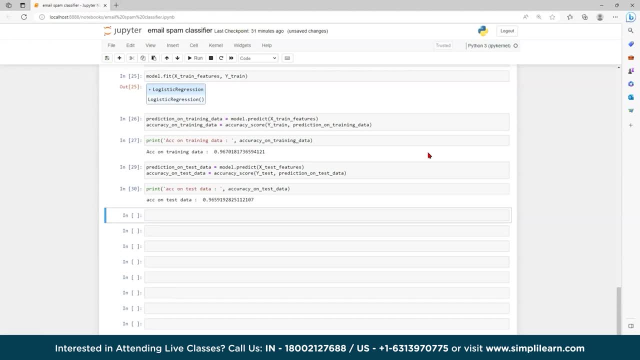 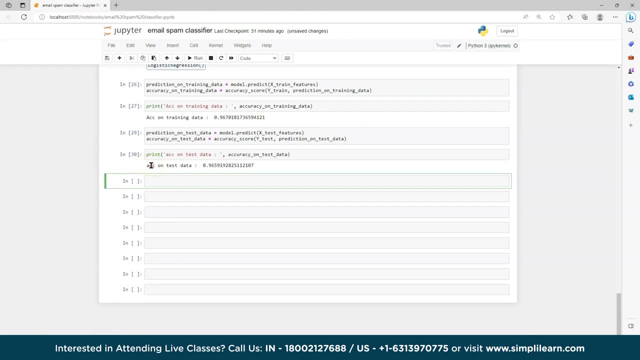 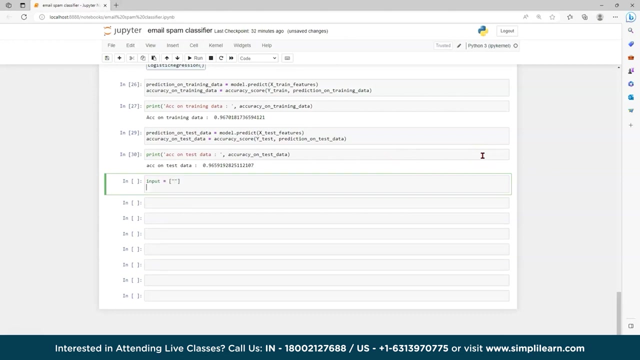 data: okay, almost 95 percent, 97 percent, sorry. so now what we will do. we will make a predictive system now, okay. So I will write here like input: okay, you have to input the mail here. okay, we will input later and we will now write the line for the convert text to feature vector. 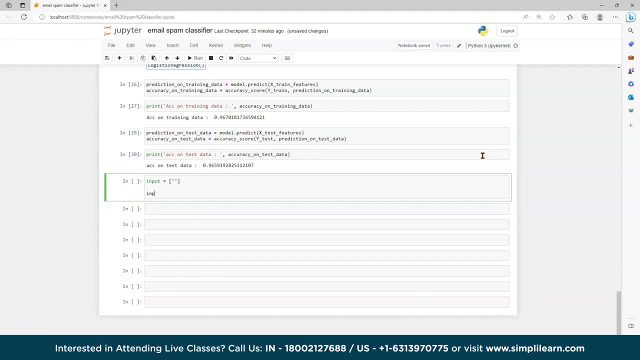 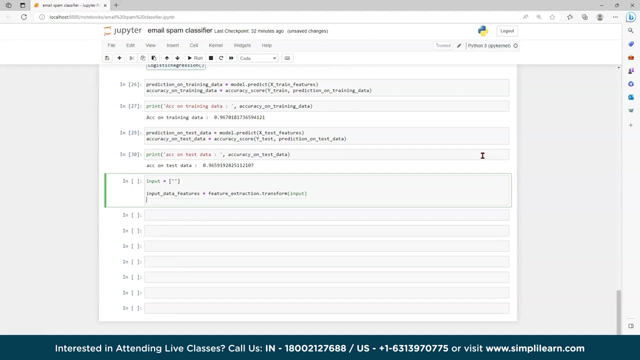 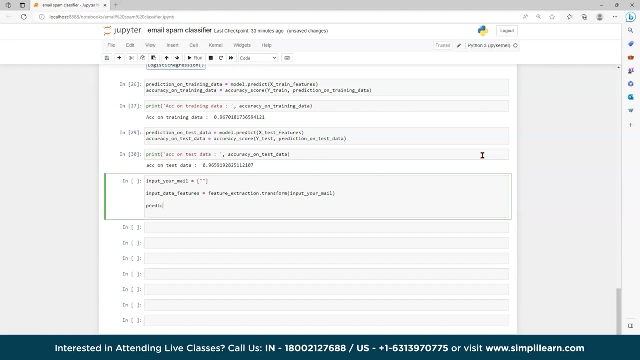 So for that I will write here: input data features: pursue feature extraction dot. transform input: okay. Okay, this is a function, so I will write here: input: Input your mail. input your mail. okay, So here we will make the prediction. okay, I will write the prediction. pursue model dot. 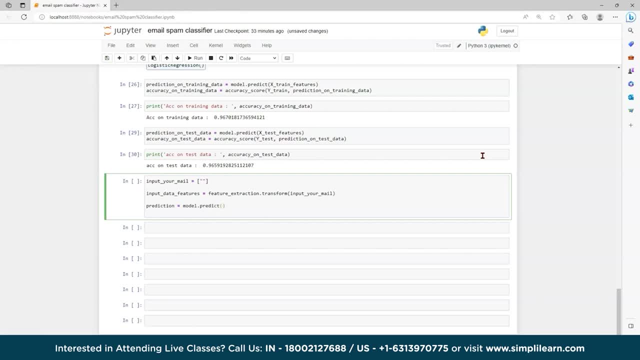 predict Okay, Okay. Okay, Input data features okay. So I have some spam mails with myself, so I will try to copy them and let's see. okay, I have some mail, so I will copy it, Okay, And put the let's see okay. 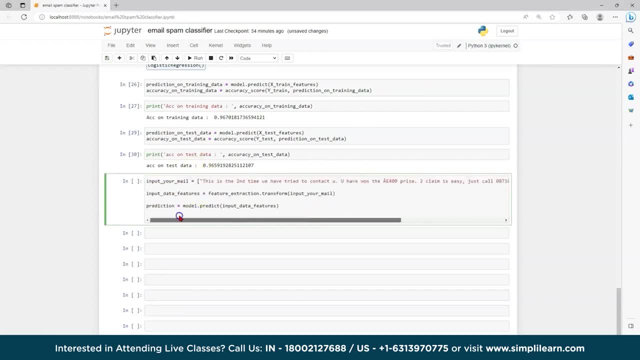 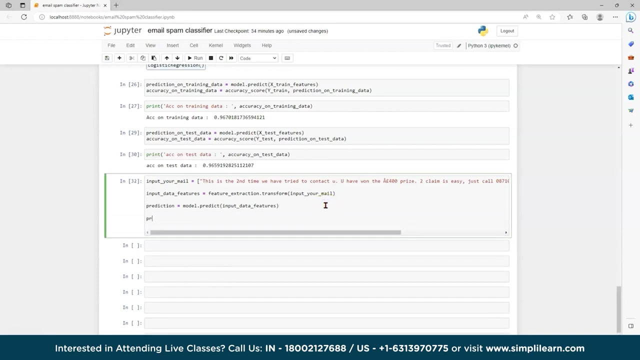 i will paste it here. okay, this is the second time we have tried to contact you. you have won this, this, this. these type of mails are spam actually, like you also know, so i will try to run it. let me run it. okay, i forgot to write print. print prediction, okay. 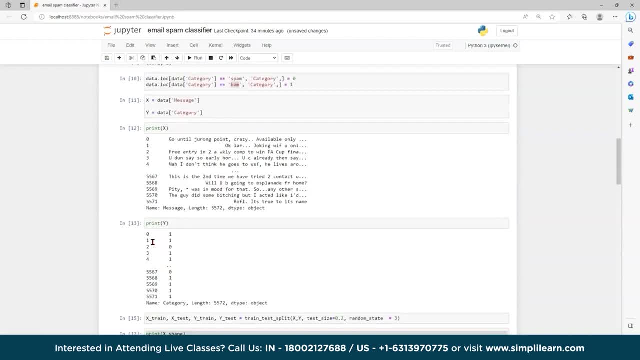 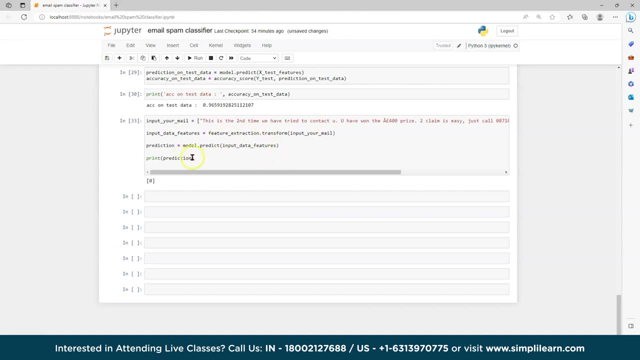 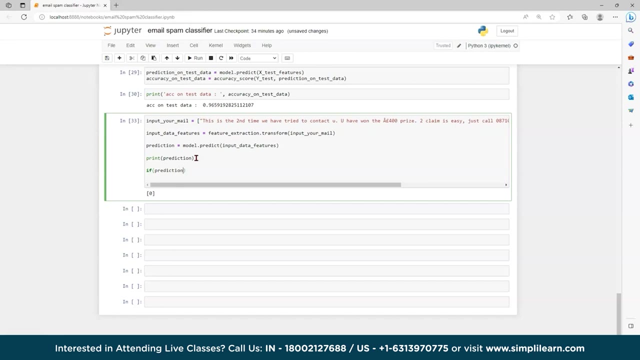 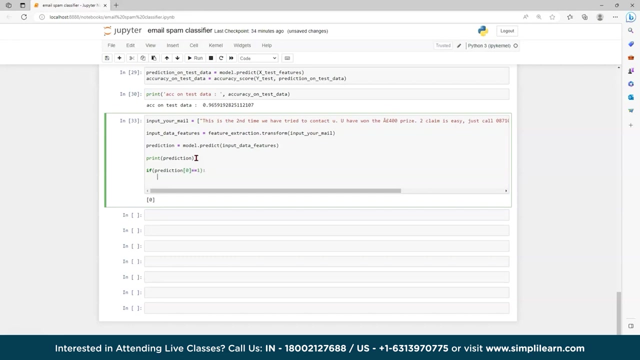 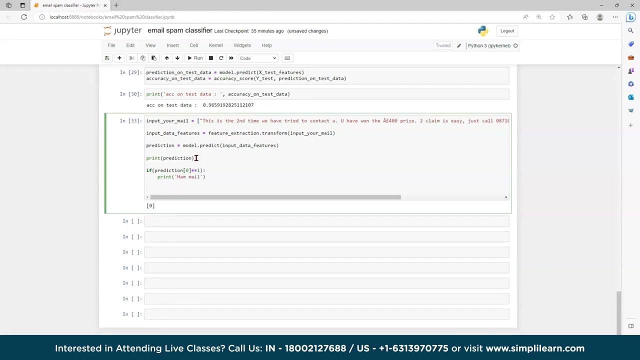 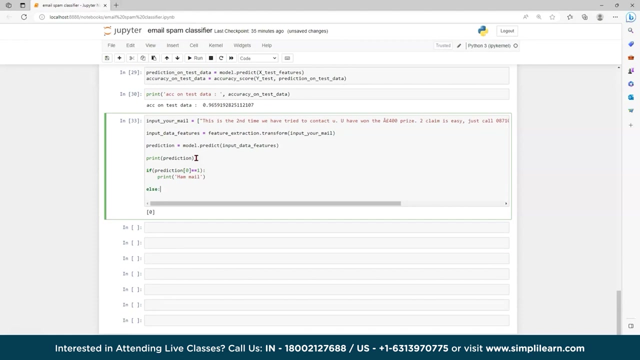 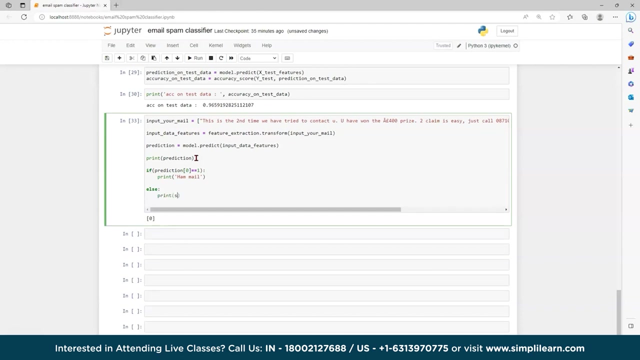 so zero. so here, as you can see already, zero means spam. okay, so this is a spam mail. actually, this is a spam mail. so, okay, wait, let me write here: if prediction is showing zero equals equals to true, then print this and as then print spam spam, okay. 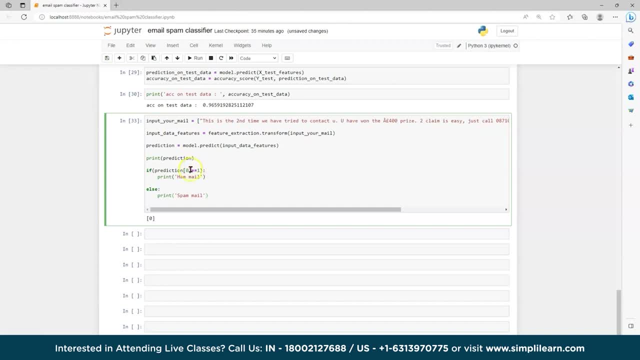 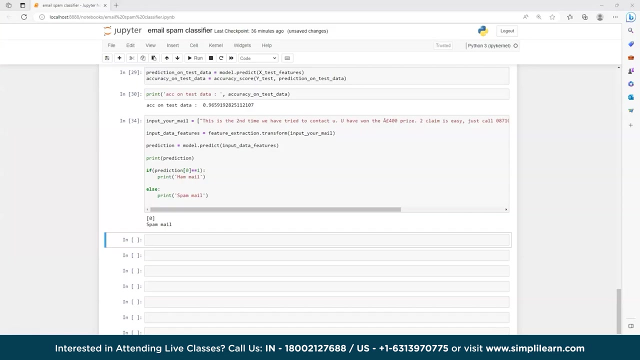 the prediction will be zero. it's not equals to one, okay, so it will show the ham mail or else the spam mail. very simple, pretty simple. see zero spam mail. okay, i will try to put it. put here one ham mail, okay. okay, let me copy it, paste it here. 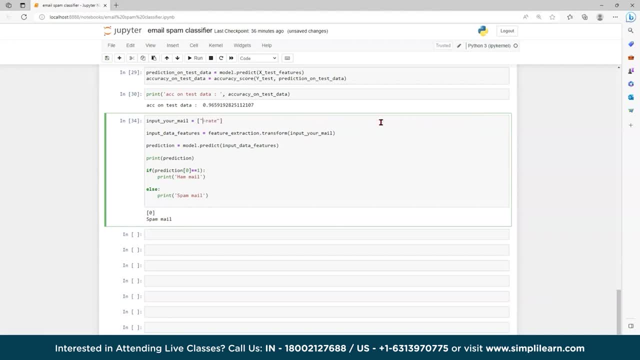 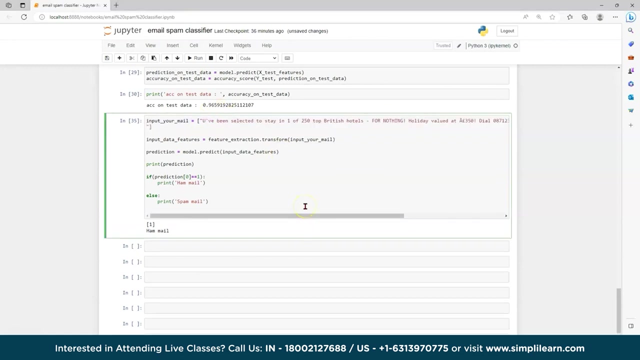 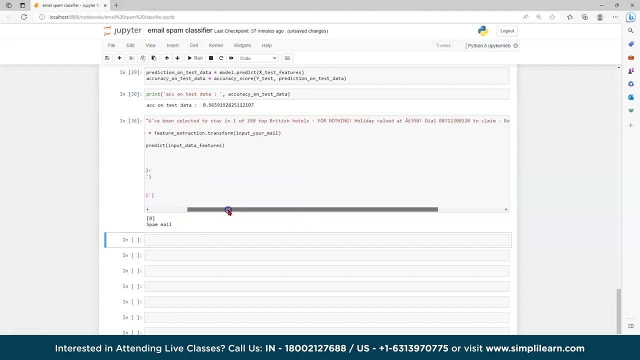 okay, let me delete this quickly. okay, let me run this so it is showing. ham mail means not spam. so quickly, let me run one more spam mail. okay, okay, copy this and paste it here. you can try with your own, like own email that you got. okay, so let me run this. so it is a spam mail. okay, see, you can see you have been selected to stay. 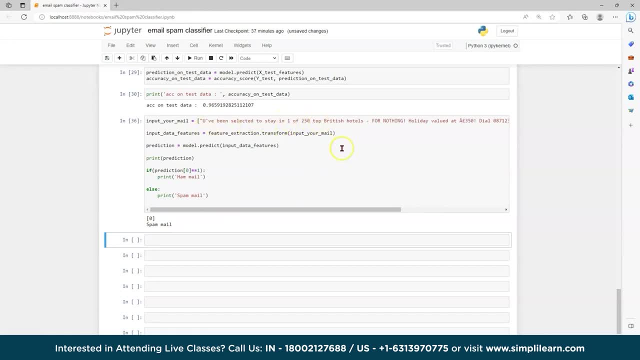 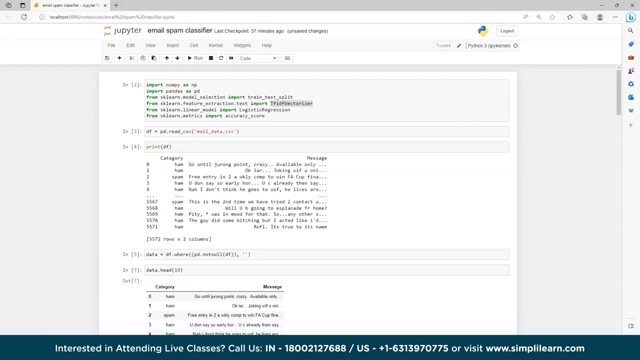 in marketing. okay, see in. so these type of mails are, like you know, these and the vouchers. this type of mails are the known as a spam mail, see: holiday value, this dial, this and this. okay, so here we are. we have done with our email spam classifier, as you can see. if you want this code, so you can. 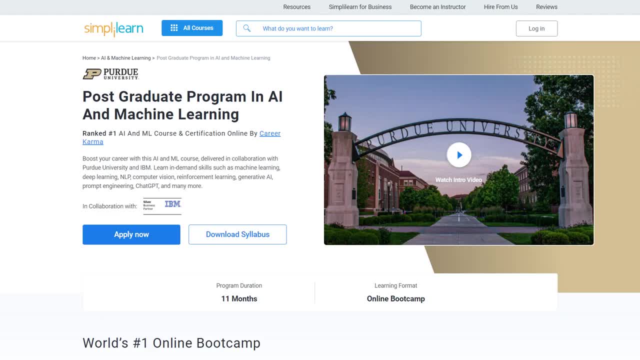 comment down below. if you're looking for a course that covers everything from the fundamentals to advanced techniques, then accelerate your course or start. if you're looking for a course that covers everything from the fundamentals to advanced techniques, then accelerate your course, and then you need to know the course based on your knowledge. 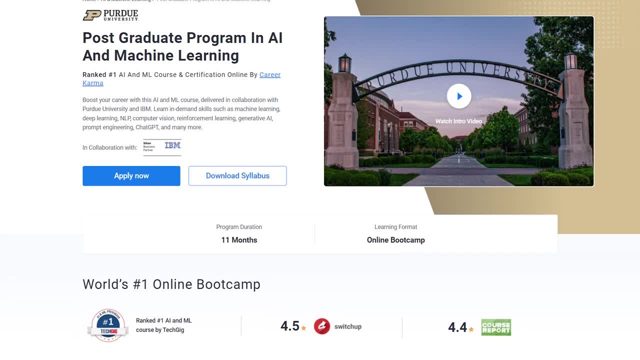 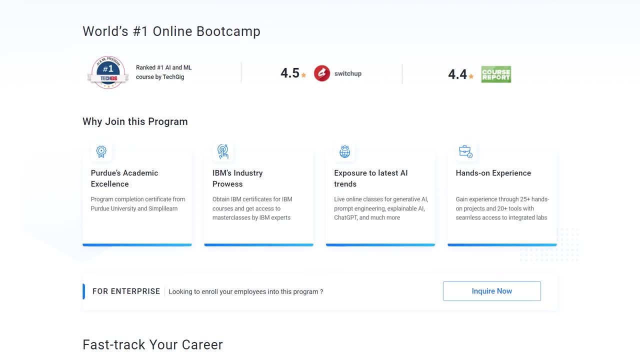 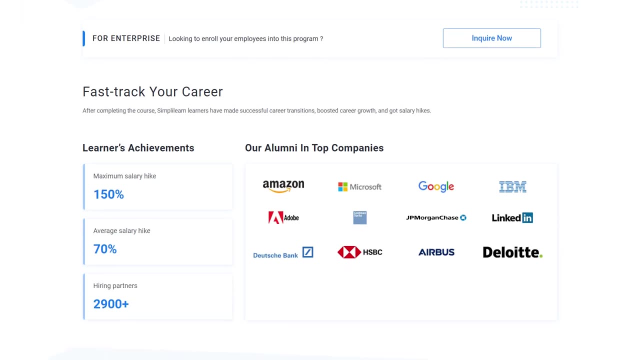 Then accelerate your career in AI and machine learning with a comprehensive postgraduate program in AI and machine learning. Boost your career with this AI and ML course, delivered in collaboration with the Purdue University and IBM. Learn in-demand skills such as machine learning, deep learning, NLP, computer vision reinforcement. 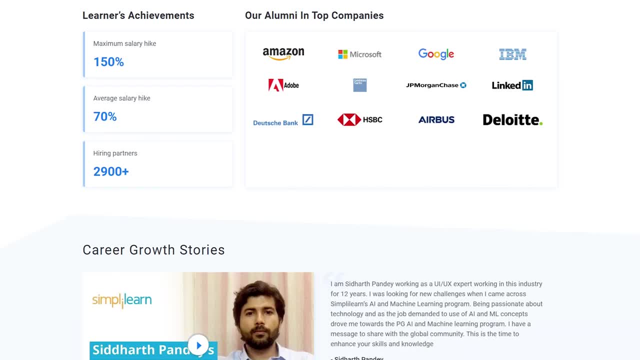 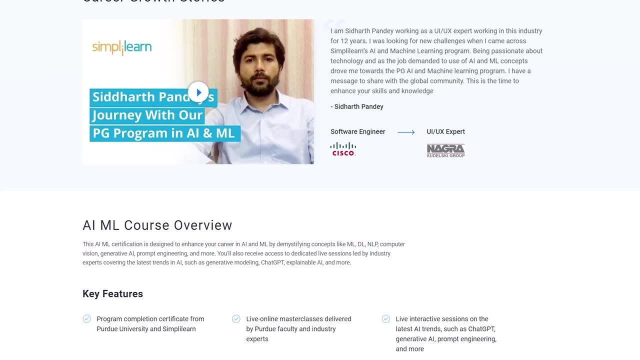 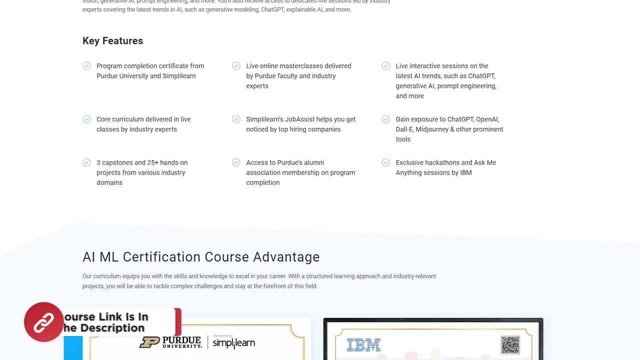 learning, generative, AI, prompt engineering, chat, GPT and many more. You'll receive a prestigious certificate and Ask Me Anything. sessions by IBM With 5 capstones in different domains, using real datasets: you'll gain practical experience. Masterclasses by Purdue faculty and IBM experts ensure top-notch education. 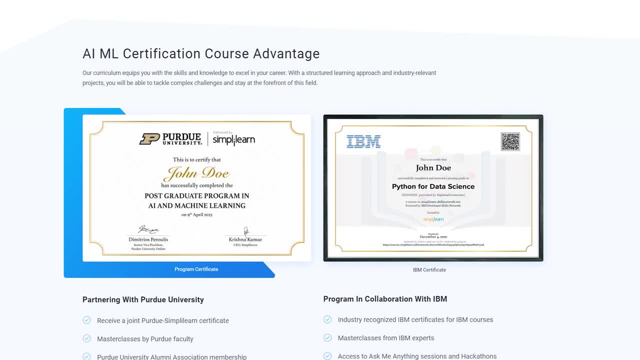 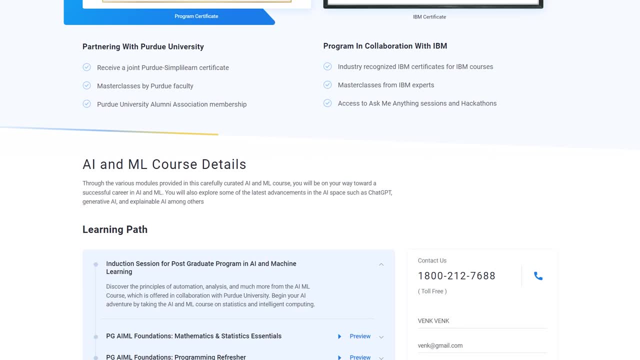 Simply Learn's job assists. help you get noticed by leading companies. This program covers statistics, Python, supervised and unsupervised learning, NLP, neural networks, computer vision, GANs, Keras, TensorFlow and many more such skills. 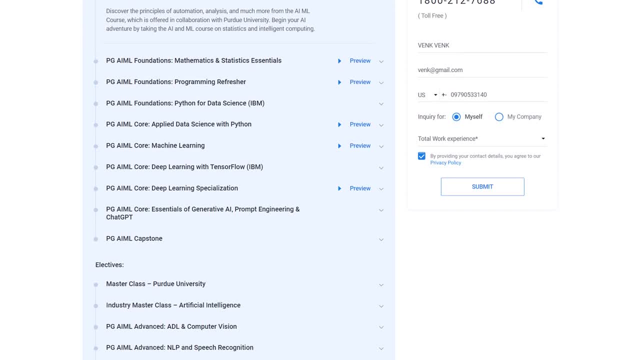 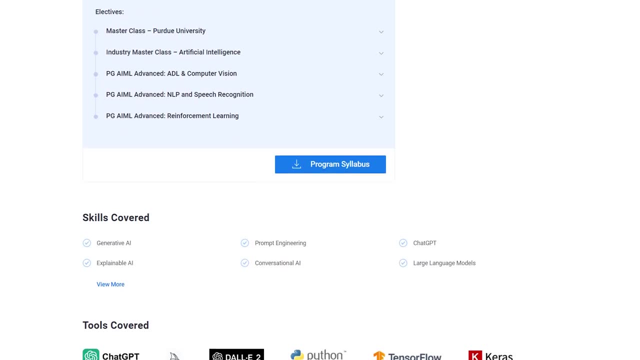 Admission to this postgraduate program in AI and machine learning requires a bachelor's degree With an average of 50% or higher marks, along with the basic understanding of programming concepts and mathematics, And candidates with 2 plus years of work experience are preferred to enroll in this course. 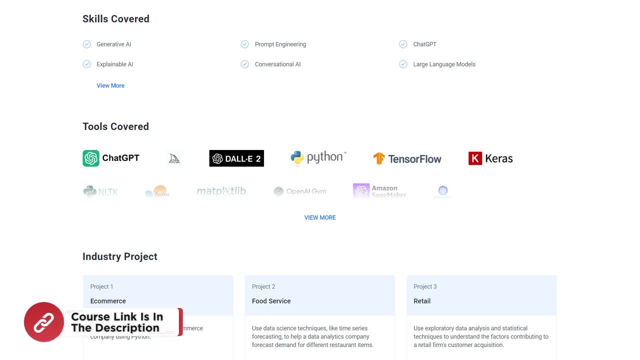 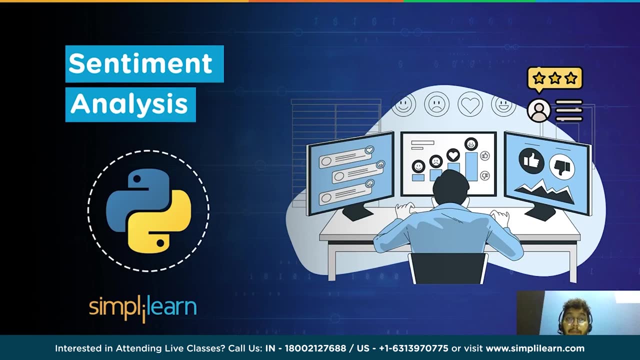 So enroll now and unlock exciting AI and machine learning opportunities. The link is mentioned in the description box below. We will take you through the hands-on lab demo of how you can do the Sentimental Analysis of Amazon Customer Reviews Before we start. I hope the screen is clearly visible and the audio is fine. 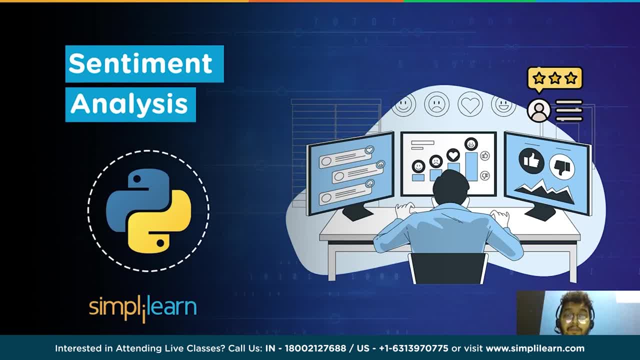 If yes, please type in yes. If there are any issues, do let us know in the chat section so that we can resolve them. Let's wait for some more minutes to let other people join. Let me tell you, guys, that we have regular updates on multiple technologies. 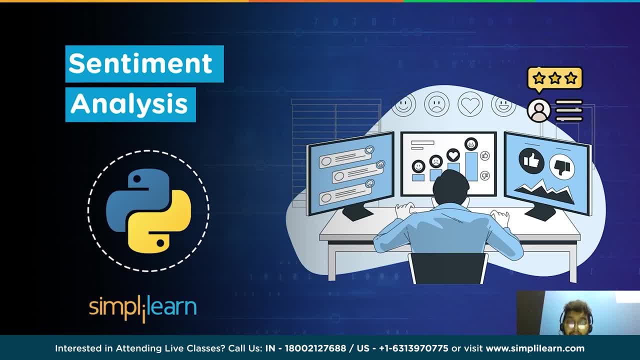 If you are a tech geek on a continuous hunt for the latest technological trends, then consider subscribing to our channel. Thank you, And don't forget to click the bell icon to never miss any update from Simply Learn Great, I think we can get started. 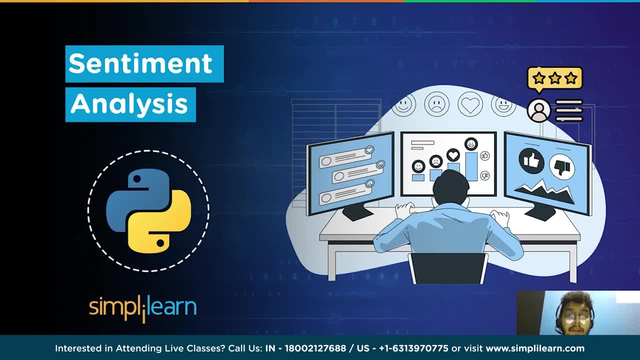 So in today's session we will go through what is Sentimental Analysis. After that we will see types of Sentimental Analysis, We will see some application of Sentiment Analysis And at the end we will see hands-on lab demo like how to implement Sentiment Analysis using. 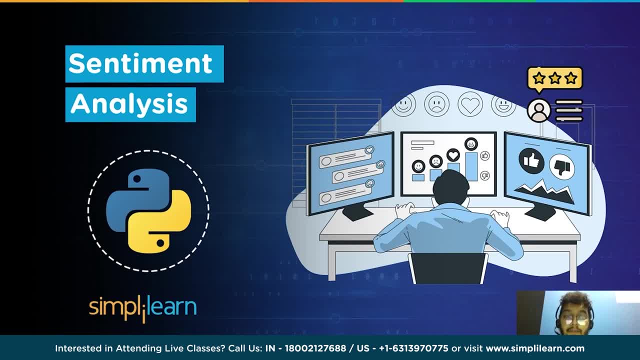 Python in detail. We already have Amazon Customer Dataset with us. We will perform different functions and analyze data for Sentimental Analysis using Python. You can download the dataset from the description box below. So before we move on to the programming part, let's discuss what Sentimental Analysis actually. 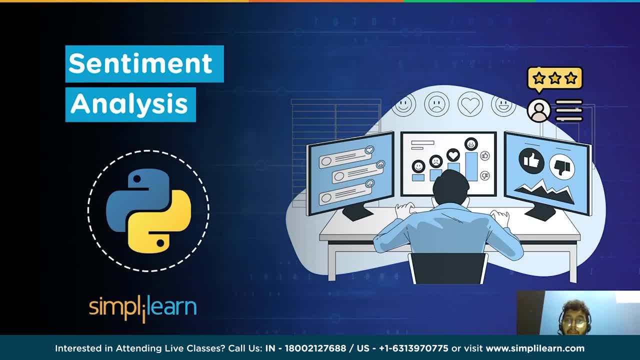 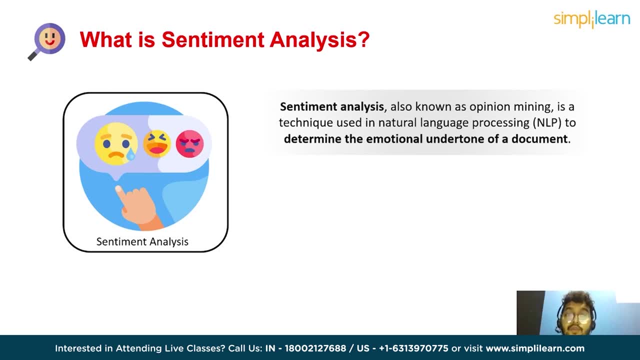 is and proceed further for the same. Sentimental Analysis, sometimes known as opinion mining, is a technique used in Natural Language Processing and LLP to determine the emotional undertone of a document. This is a common method used by organizations to identify and group ideas regarding a certain good service or concept. 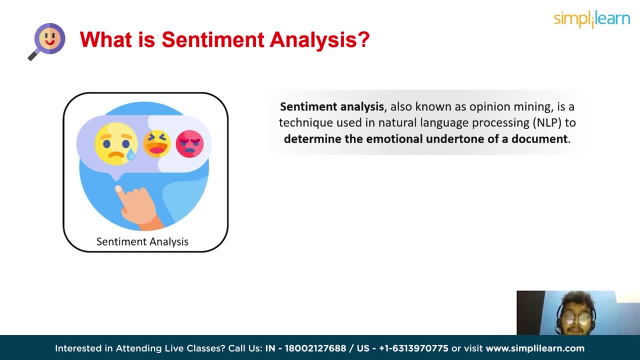 Text is mined for sentiment and subjective information using data mining, Machine learning and artificial intelligence. Tools for sentiment analysis assist businesses in extracting information from unstructured, unorganized language found in online sources like emails, blog posts, support tickets, web chats, forums and comments. 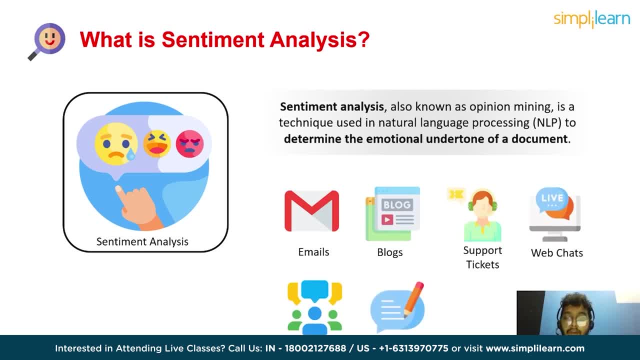 Algorithms use rule-based automatic or hybrid technology to replace manual data processing. While automatic systems use machine learning to learn from their data, rule-based systems execute sentiment analysis. Sentiment analysis uses predetermined lexicon-based rules. combining the two methods result in hybrid sentiment analysis. 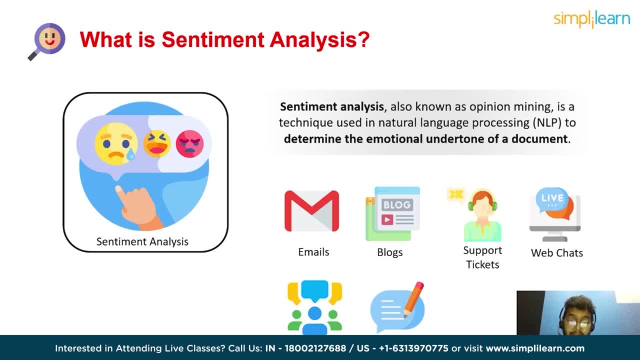 Sentiment analysis or opinion mining can extract the subject, opinion holder and polarity or the degree of positivity and negativity from the text and identify sentiment. Additionally, other scopes, including document, paragraph, sentence and sub-sentence level, can be used for sentiment analysis. 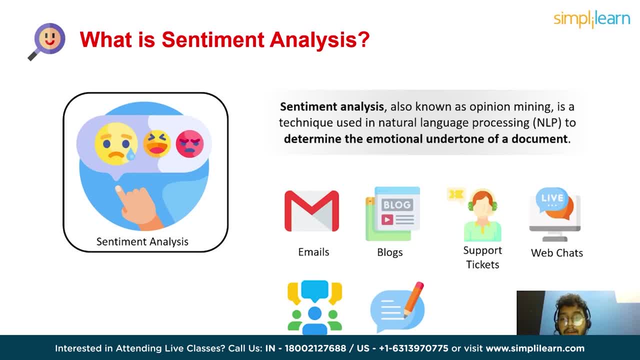 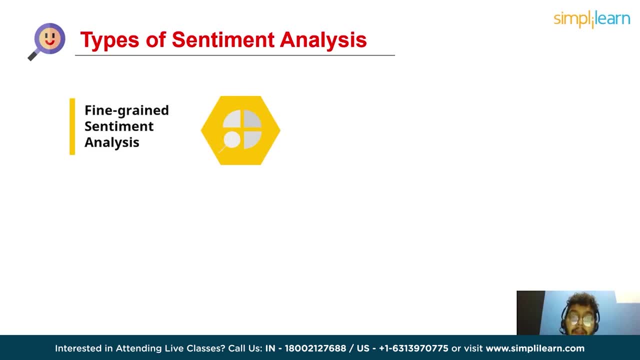 After seeing what is sentiment analysis, let's discuss some types of sentiment analysis. 1. Fine-grained sentiment analysis. By segmenting sentiment, each phrase or clause in a sentence is broken down and examined in relationship to others. Simply said, you can tell who reviews a product and what topics a person specifically discusses in their feedback. 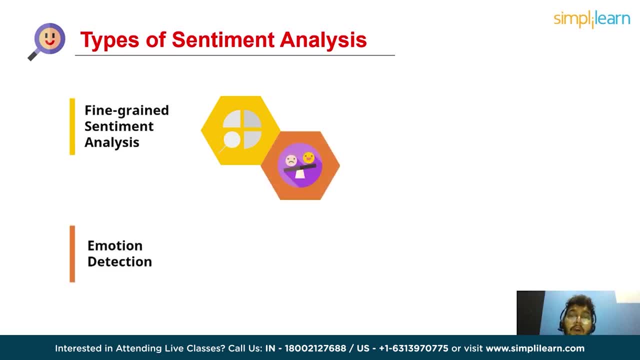 2. Emotion detection: Instead of identifying positivity and negativity action, recognize particular emotions. eg could include shock, rage, grief, frustration and happiness. Intent-based analysis: In addition to identify opinions in a text, the intent-based analysis also identifies behaviors. 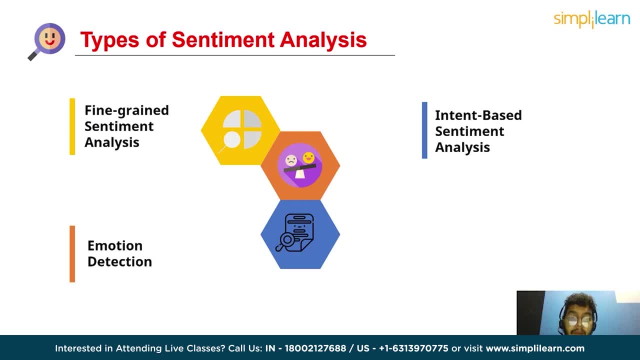 For instance, a frustrated online comment about changing a battery can motivate customer care to get in touch to address that particular problem. Sentiment-based analysis collects the precise component that is being mentioned, either favorably or unfavorably. For instance, a client may write in a product review that the battery life is too short. 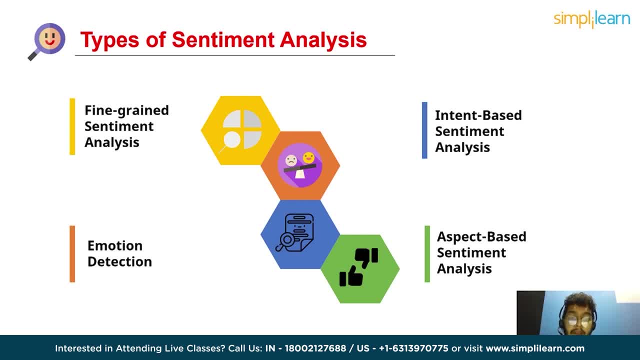 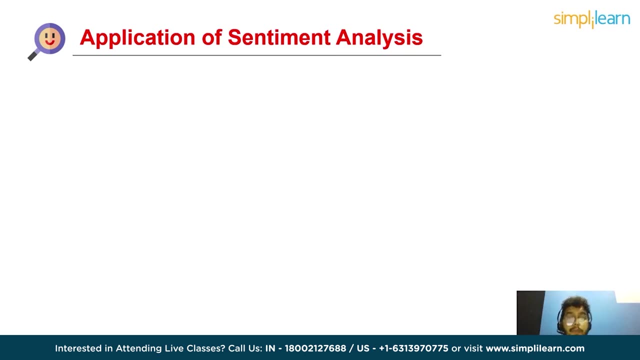 The system will then respond that the battery life is the main complaint and not the product as a whole. So after seeing types of sentiment analysis, let's see some application of sentiment analysis. Organization can employ sentiment analysis technologies for a number of purposes: 1.. 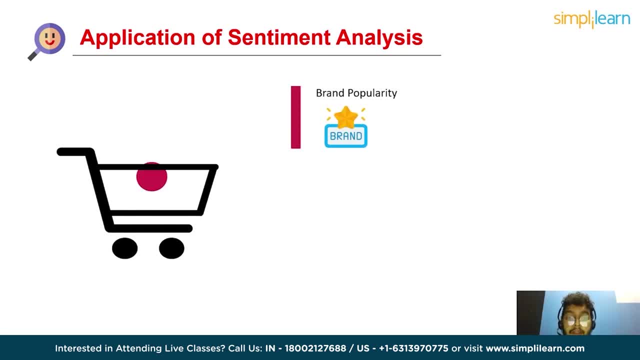 Determining brand popularity, reputation and awareness at a particular period or over time. 2. Customer service requests into categories. 3. Monitoring consumer response to new improvements or products. 4. Identifying the demographics or target market. 5. Determining the effectiveness of a marketing effort. 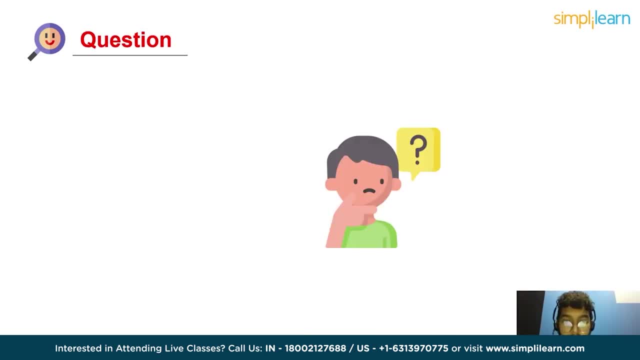 6. Identifying the demographics or target market. 7. Determining the performance of a product or service. Here is one question for you guys. I will give you one minute for this. You can comment or you can give answers in chat section. 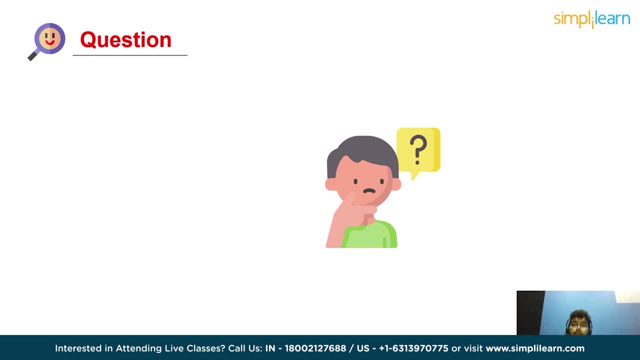 So I can see if the answers given by you are right or wrong. So the question is: is text analytics also refers to as text mining? I am repeating again: is text analytics also refers to as text mining? The options are true or false. 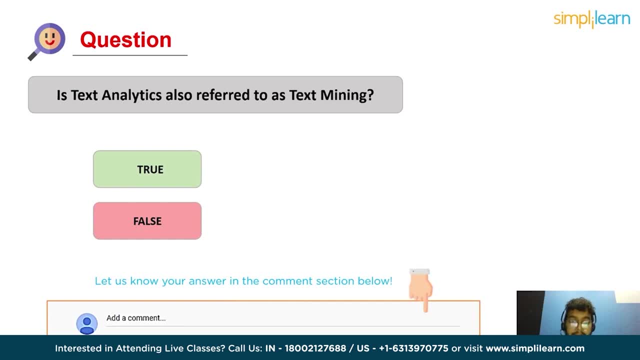 So let us know your answer in comment section below Or in chat section. I am starting timer of 1 minute. Just type your answer in comment section or in chat section. Do, let me know your answer. So I am starting timer of 1 minute. 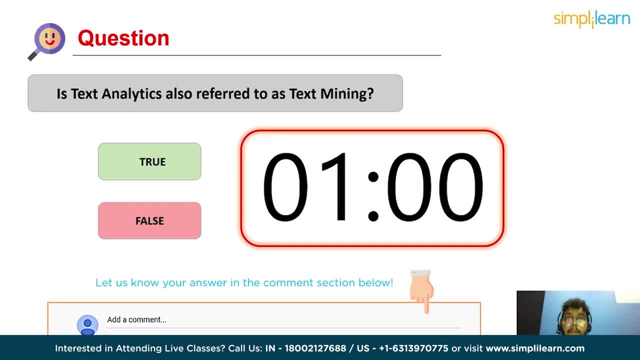 I kindly ask that everyone take part in this to make live session exciting. Share it to your friends. See you next time, Bye. So the question is: is text analytics also refers to as text mining? 35 seconds are left. Do let me know your answers. 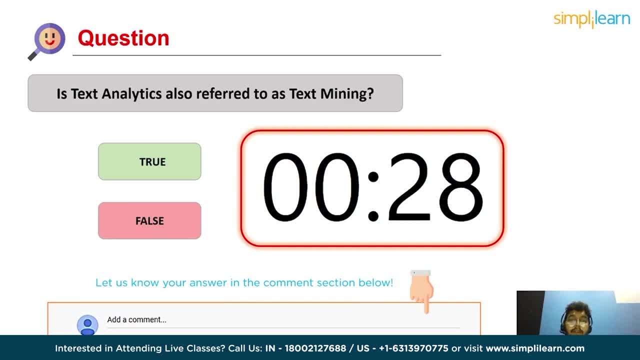 I currently ask that everyone take part in this to make the live session exciting. 20 seconds left. You can comment or you can give your answer in chat section so I can see if the answers given by you are right or wrong. So time up, guys. 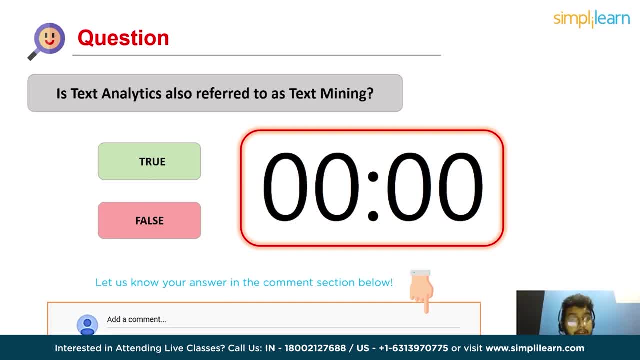 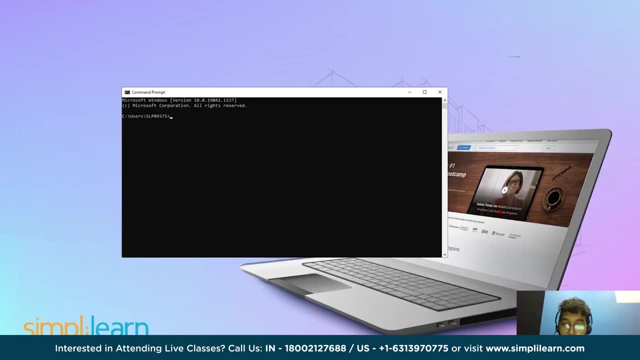 So, after the allotted time has passed, Those who provided the correct response Will receive a response and those who provided the incorrect response will receive one. Okay, now let's move to our programming part to perform sentiment analysis using Amazon customer data set. So first we will open command prompt to write command to open Jupyter Notebook. 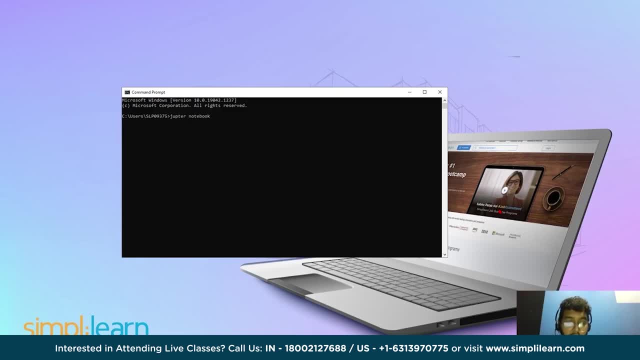 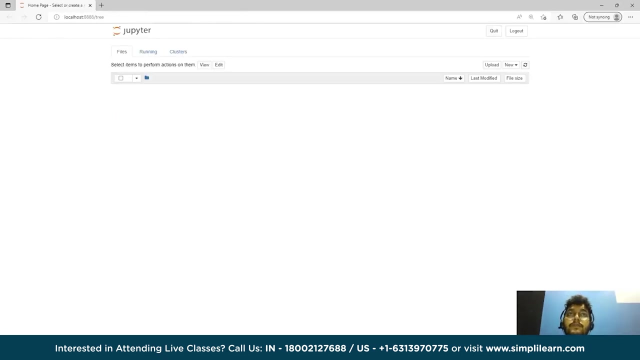 So here we will write Jupyter Notebook. Press enter: Okay, it's Jupyter Notebook. Okay, it's Jupyter Notebook. Okay, It's Jupyter Notebook, Okay. Okay, here we will write a command prompt to open Jupyter Notebook. 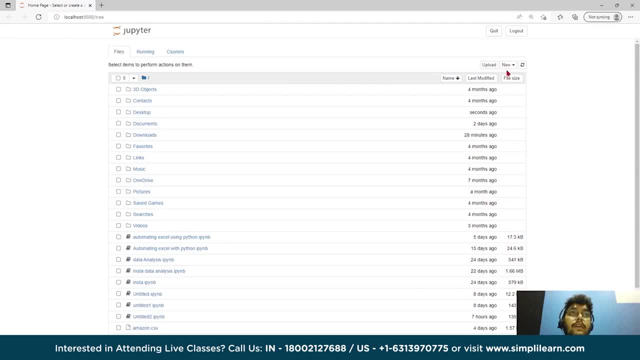 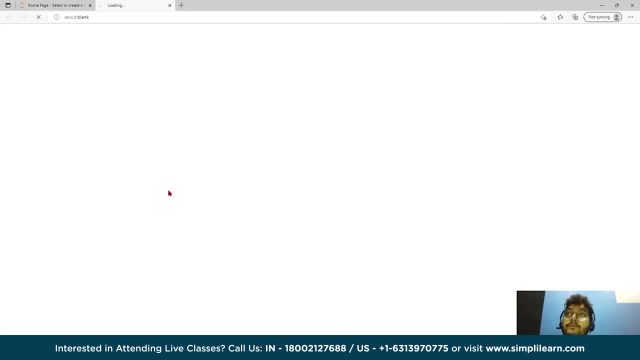 So this is the landing page of Jupyter Notebook, And here you can select new Python file. It's loading, Okay. So this is how the jupyter UI looks like. so at first we will import some bunch of major libraries of python which will help us in mathematical functioning. 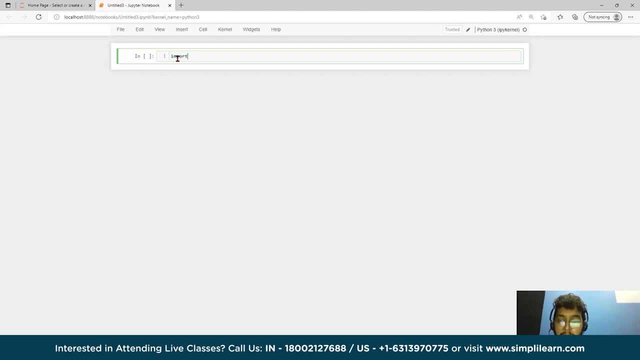 So the first one is numpy. so first I will write numpy, import, numpy, snp. numpy is a python library used for working with arrays. It also has functions for working in the domain of linear algebra and matrices. It is an open source project and you can use it freely. numpy stands for numerical python. 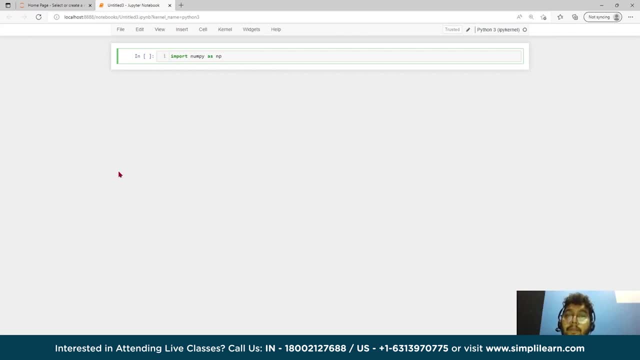 So the next one is pandas. I will write here: import pandas spd. So pandas is a software library written for a python programming language for data manipulation and analysis. In particular, it offers data structures and operations for manipulating numerical tables and time series. After that we will import nltk, so the natural language toolkit. nltk is a python programming. 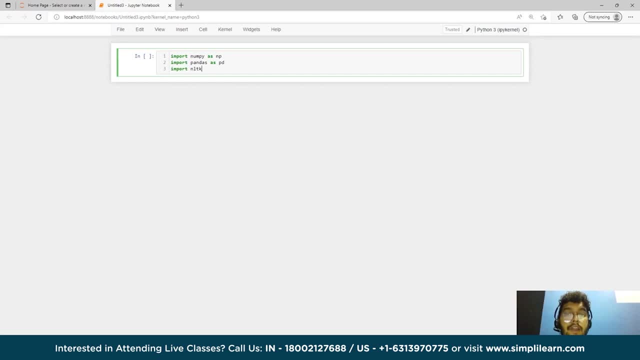 environment for creating applications for statical natural language processing. So we will import nltk For parsing, classification, stemming, tagging and semantic reasoning. it includes text processing libraries, So after that we will import from nltksentimentwdr. import nltksentimentwdr. 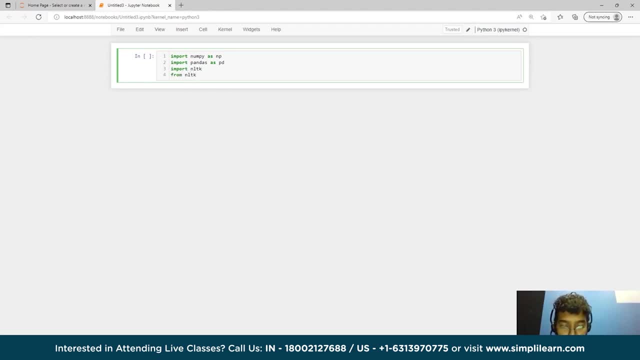 So after that we will import from nltksentimentwdr, import nltksentimentwdr, import nltksentimentwdr. So that section was also done. You now have nltksentiment入 golpeux. As you can see, list is filled with inside. 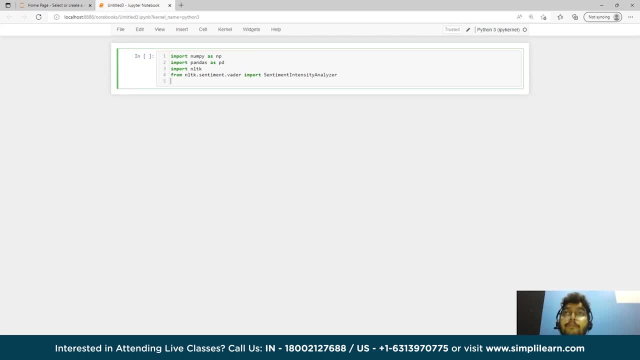 the column to understand the essence of these arguments. So let's try that. tell script realname Anyway. so in this panel we will have the lesson. There is no column. Yeah, Lunch. Yeah, Tell script realname Apparently erstmal. 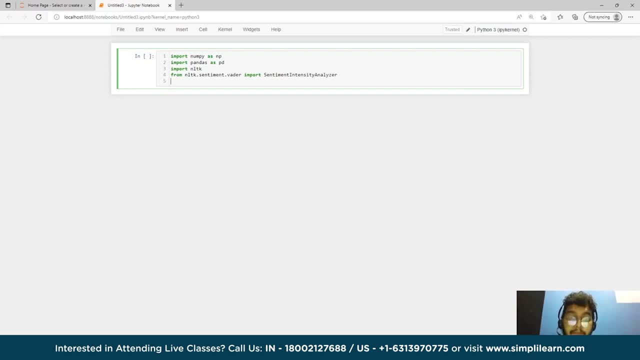 Valence Aware Dictionary and Essential Reasoning is customized precisely to sentiments expressed on social media. Wader makes use of a variety of sentiment lexicons as a collection of lexical elements such as words that are often classified as either positive or negative, depending on 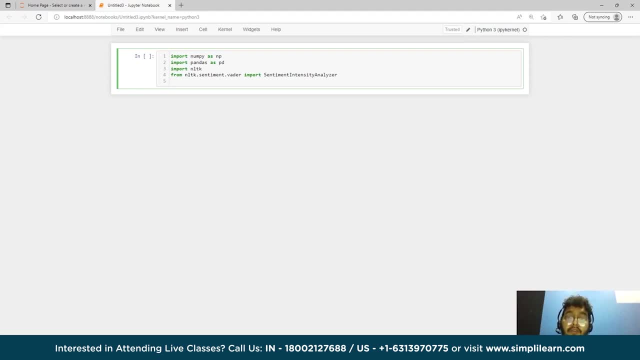 their semantic orientation. Wader not only informs us of the positivity and negativity scores, but also of the sentimentality of each score. So the next one is import re. Python re module fully supports regular expressions similar to those in Perl. If a regular expression, compilation or use error occurs, the re module raises the expression. 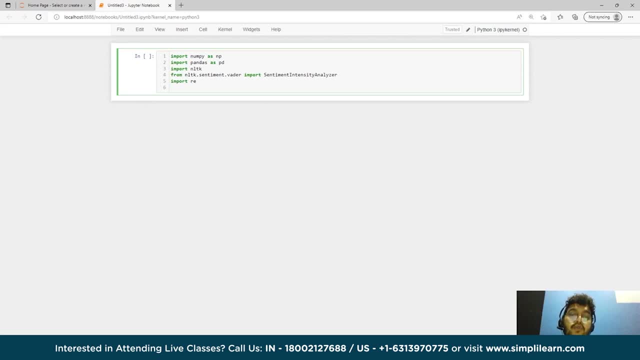 re. Two key functions that are used to manage regular expressions will be covered. So re means regular expressions. So the next one is from TextBlob- import TextBlob, So a Python 2 or 3 package called TextBlob, is used to process textual data. 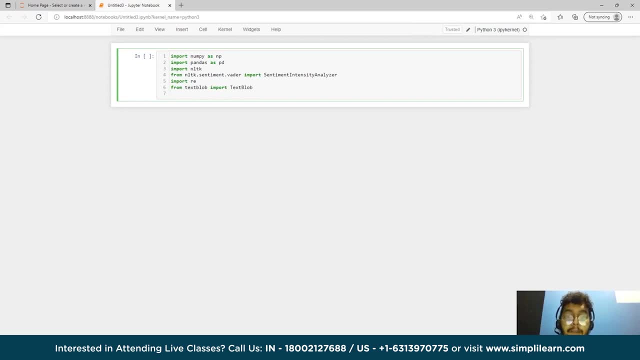 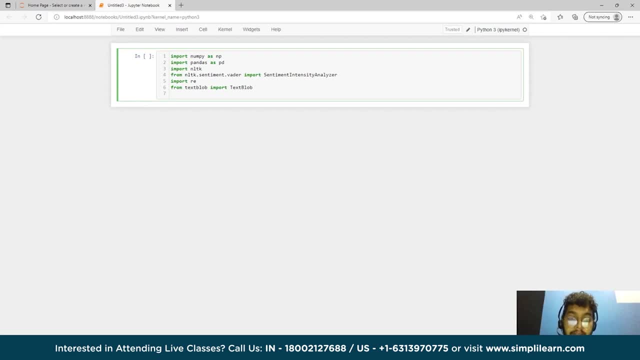 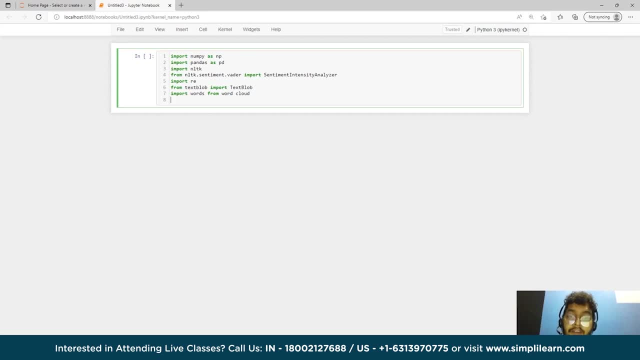 of words. popular words and phrases are highlighted using cloud creators, depending on their frequency and importance. They give you immediate, straightforward visual insights that can inspire more through analysis. So, like an open source Python library based on matplotlib is called seaborn, It is utilized. 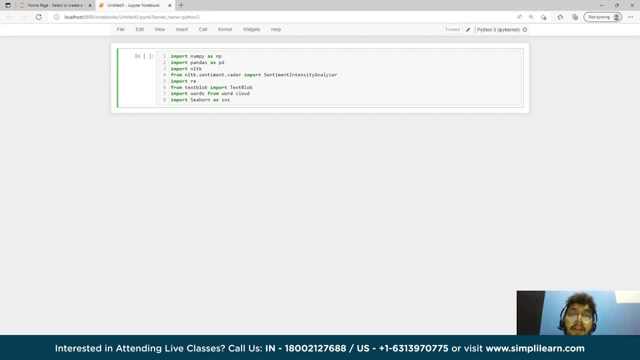 for data exploration and data visualization, where data frames and the pandas library seaborn function with ease. So the next one is import matplotlib dot pyplot as plt. okay, yeah, seems good for python and its numerical expression numpy. matplotlib is a cross-platform data visualization and graphical charting package. 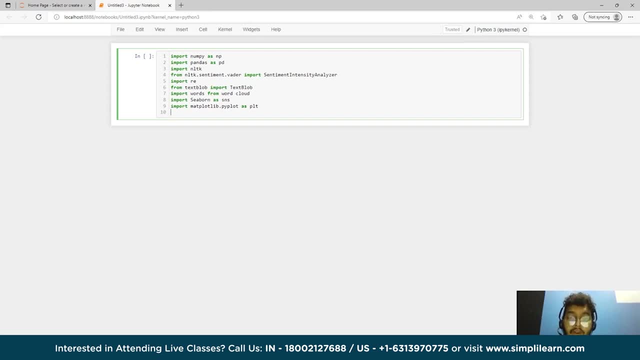 as a result, it presents a strong open source substitute for matlab. the apis for matplotlib allow programmers to incorporate graphs into gui applications, and the next one is import matplotlib cufflinks c, u, f, f, l, i, n, k, s as cf perfect. another python module called cuff link links plotly with: 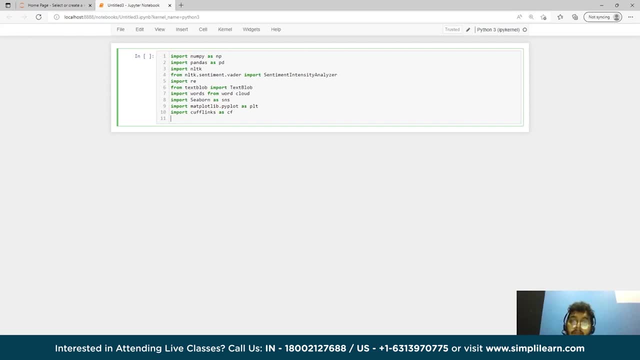 pandas, so that charts can be easily created on data frames. in essence, it function like a plugin. so next inline at plotlib- matplotlib, so you can enable inline plotting by using the magic function %matplotlib inline, which causes the plots and graphs to appear below the cell where you plotting commands are entered. similar to a jupyter notebook, it offers back. 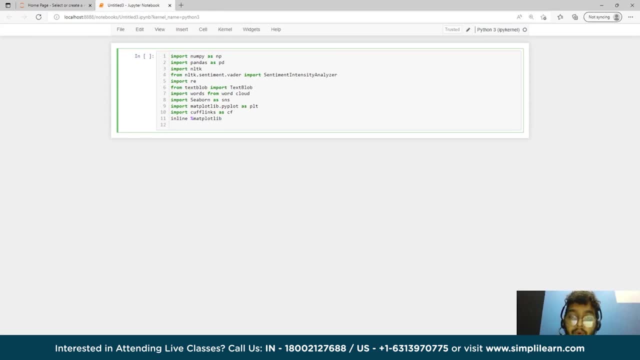 an interactivity in frontend. so next we will import what you can like. we can import. ok, from plotlyoffline import init: underscore, notebook, underscore mode, comma, iplot. ok, so we can import from plotlyoffline import init: underscore, notebook, underscore mode, comma, iplot. 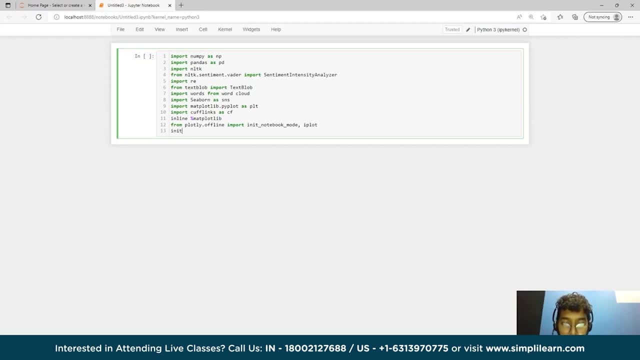 ok in it. underscore notebook notebook mode go. okay, it's true. yeah, pf dot. go underscore offline. ok, So in order to display the plot inside the notebook, you need to initiate plotly notebook mode as follows like this: Keep rest of the script as it is, like it and run the notebook cell by pressing you can. 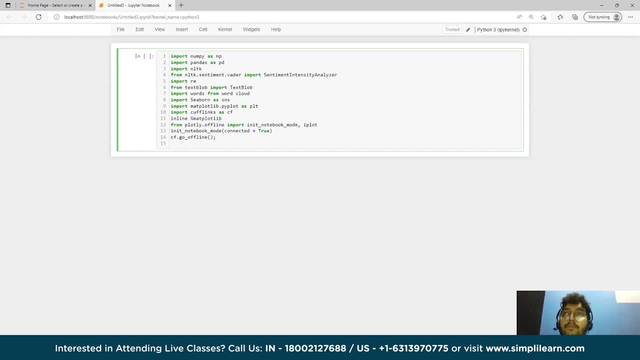 shift plus enter graph will be displayed offline inside the notebook. so basically it is used for the offline graphing. you can see, okay. so next we will import arm plotly dot subplots. The non-leaf nodes in this figure schema are represented by a hierarchy of python classes. 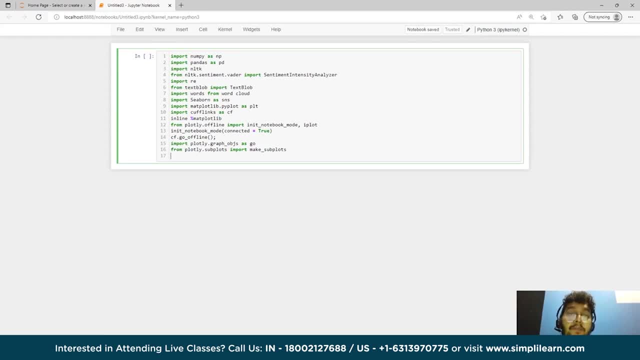 that was automatically constructed and is found in the plotly dot graph objects which is normally imported as go. These class instance are refers to as graphplotlygraph: The graph object, the plotly defined fundamental classes. So here we will import some like warnings, you can say like to get not error. 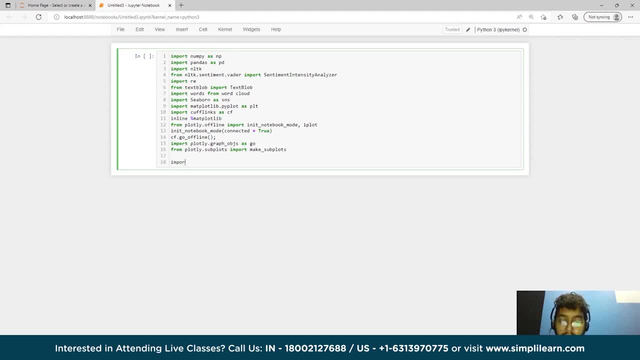 So we will import. let me give a line: space import warning warnings, Yeah, Warnings, Dot Filter, Warning, Ignore. Warnings, Dot Warn. And This Like will not show, So Don't worry, I am not going to show this. 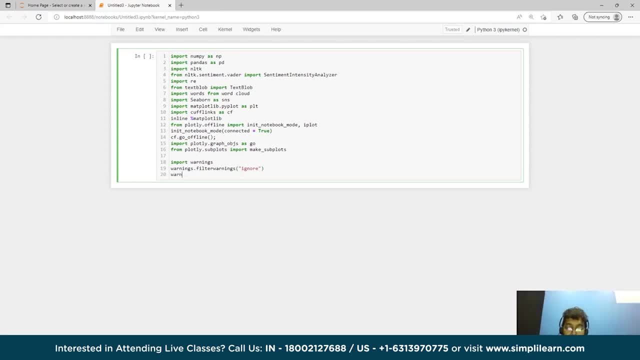 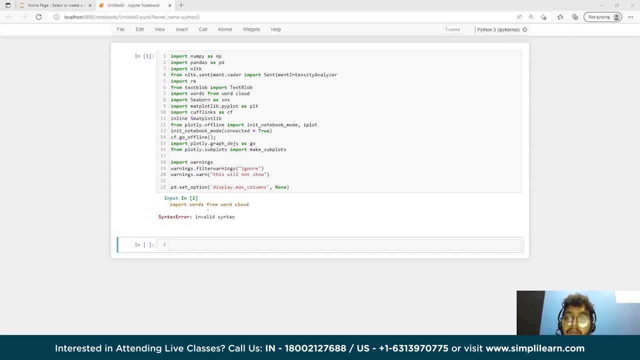 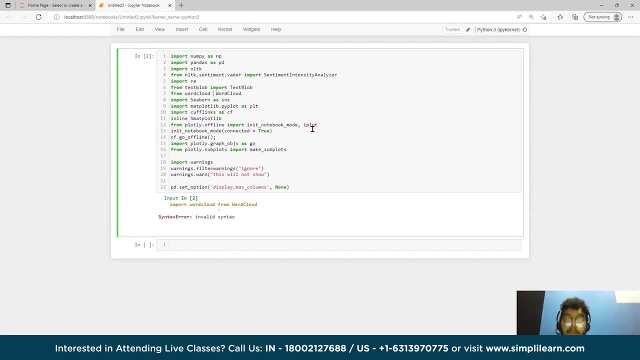 from word cloud import word cloud. okay, yeah, seems good. so wherever we, yeah, in warnings, despite the notification, the software continues to execute to display warning messages, utilize the one found in the warning module. the python built-in class inspection is a subclass of the warning module, which is used to display warning messages. 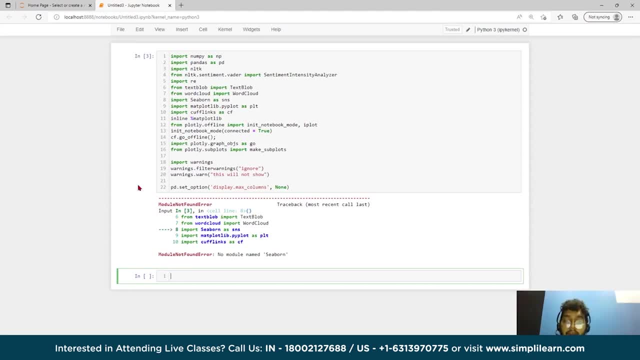 import warnings. okay for seeing full data, every single columns like: okay, there is error c born. no module has c born, so s will be small. dot okay in line. dot okay in line is only like like that line. any error, any error, i guess no error. 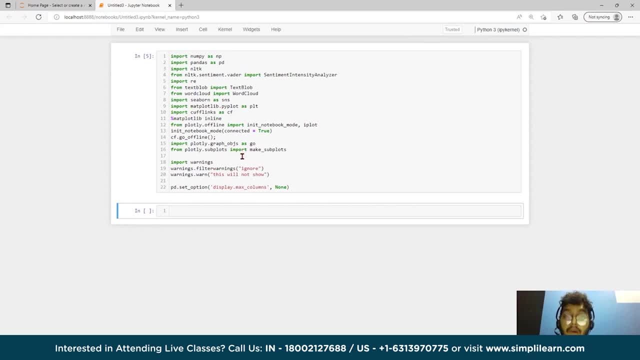 okay, yeah, for seeing full data, like every single columns or pd of pd. so here we are using this pd dot set option so we can use for it. so, moving forward, let's import data set. so for importing data set, we will write here: uh, like df equals to pd dot. read. 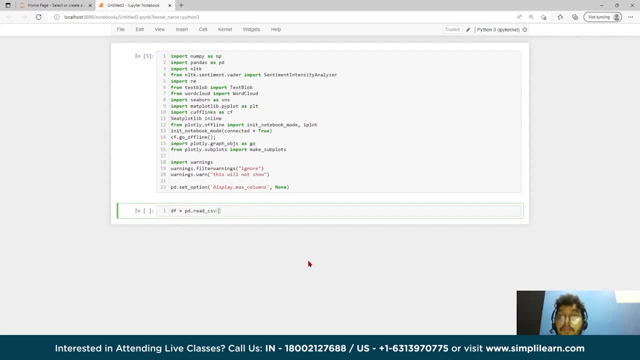 csv- okay, a data set name. so so you can download data set from the description box below. so no worries of for that. so let me run this. okay, so like here is: pd is for pandas library, read is used for reading the data set from the machine and csv is used for the type of file which you want to read. so let's see our data. 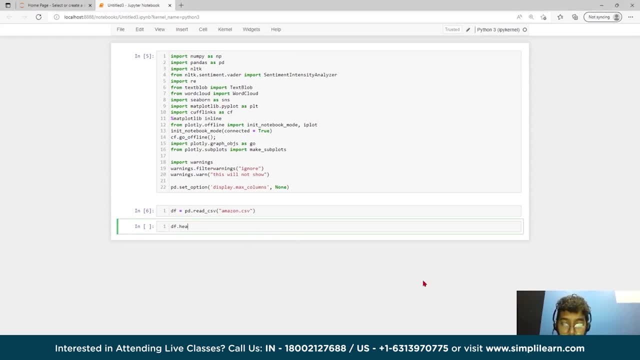 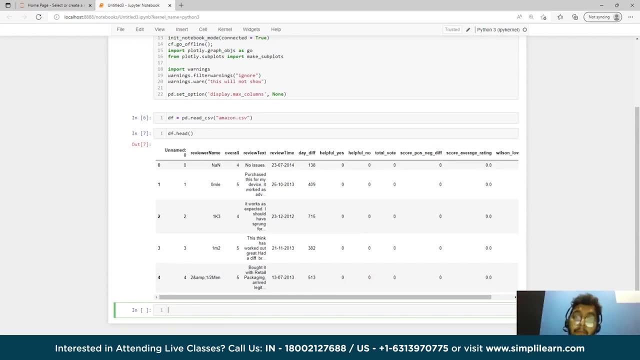 so here i will write df dot. so if you want to like, if you want to see top five rows of your data set, you can use head, and if you want to uh like see five rows of your data set, you can use tail insert instead of head. 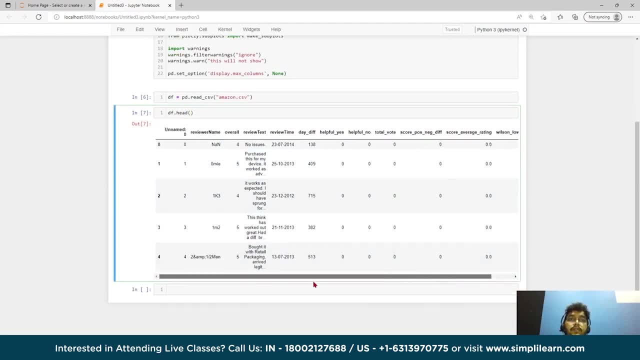 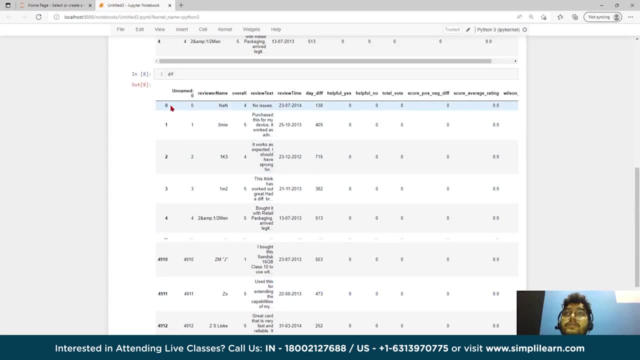 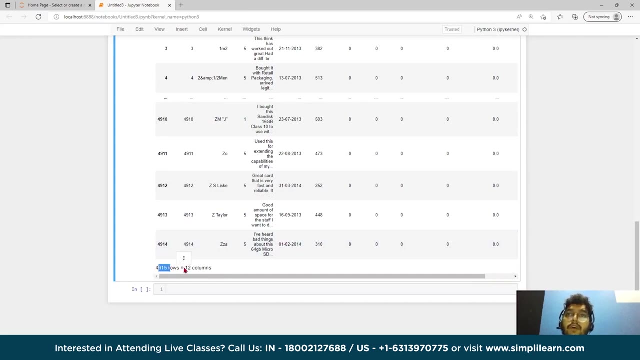 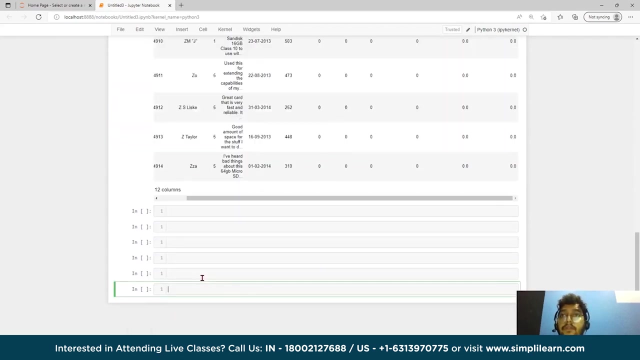 this one, okay. so this is our data set, with only five rows. if you want to see full data set, you can like i'm starting from zero and ending it. four, nine one, four rows, okay. four, nine one one, five rows and twelve columns eight. so let me give something like this for the better visual. yeah, 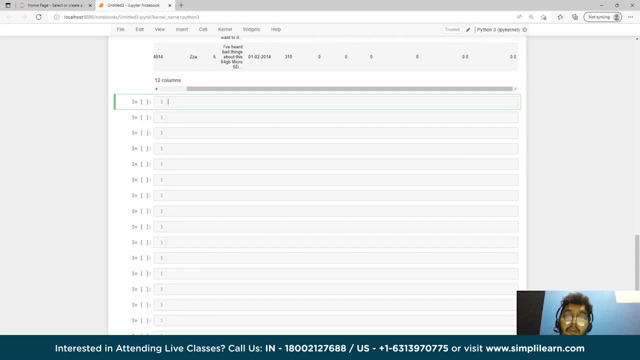 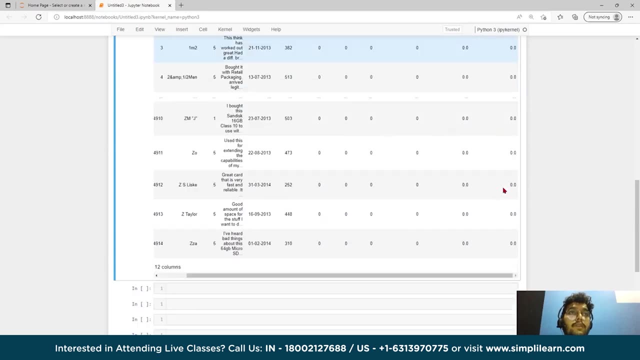 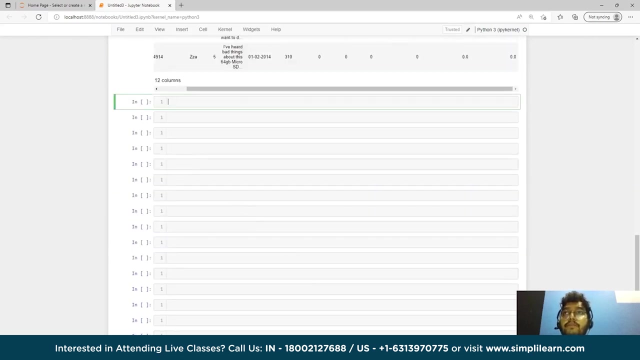 okay, so moving ahead, let's sort this wilson bound column to ascending order for better analysis. so i am talking about this wilson lower bound column, this one. well, it's not zero, zero, zero, like you know all the rows, so let me show you. so here you have to write like df equals. 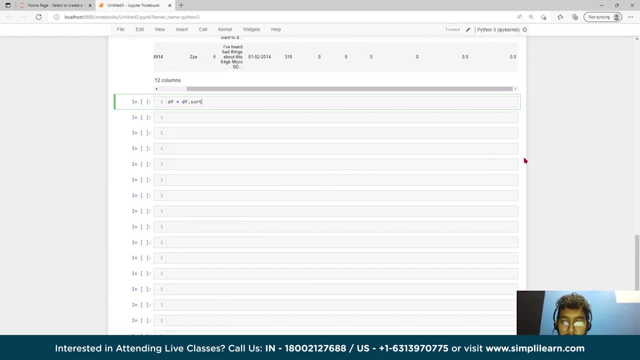 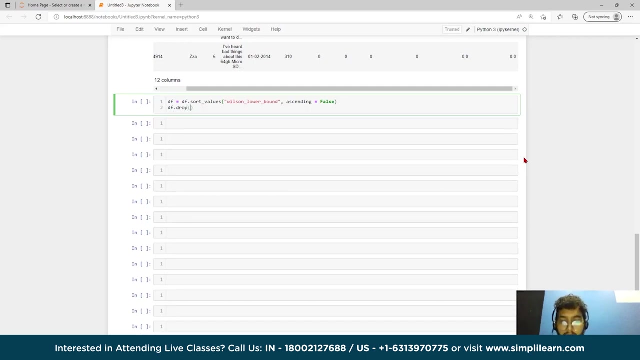 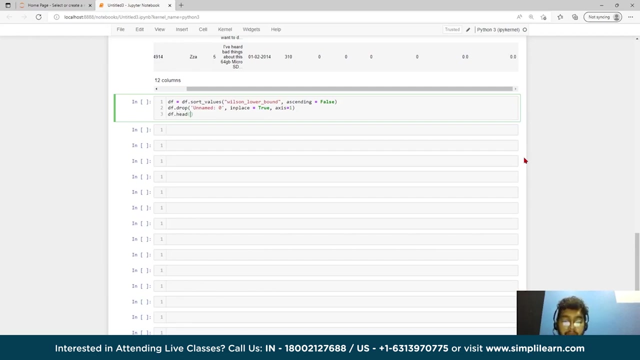 to df dot sort values. wilson spelling should be correct: lower pound. i'll make it to ascending order- ascending, sorry, descending order. so bf dot drop named unnamed colon zero. okay, in place it is equals to true comma. x is equals to one, okay, so let's see your data. 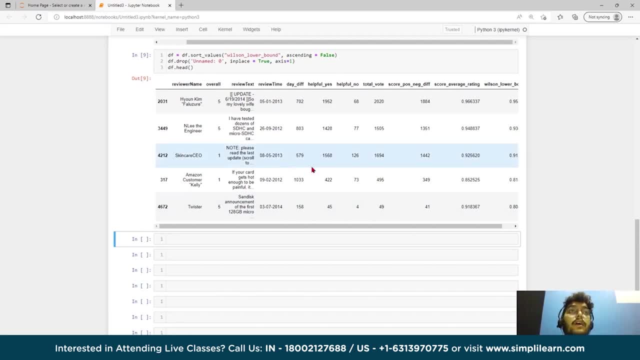 so here you can see. the data is sorted in as in ascending order. okay, the provided row or column is eliminated via the drop function. the draft method eliminates the specified column when the column accesses is specified. so in the Hey, where are you go into the landing page? here you go back to the, the last in the data elements. 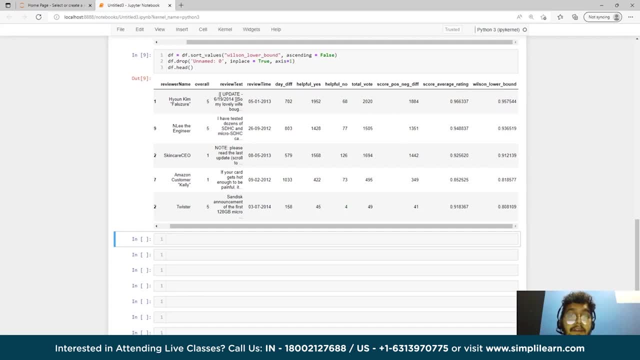 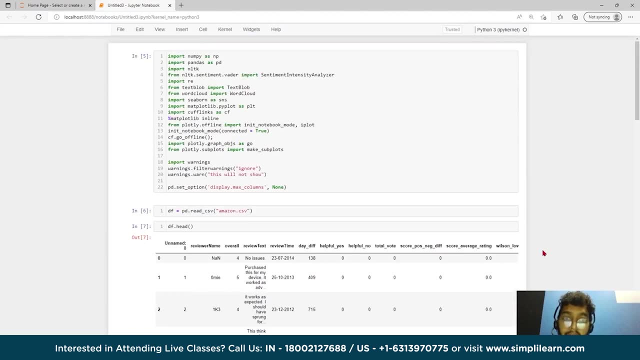 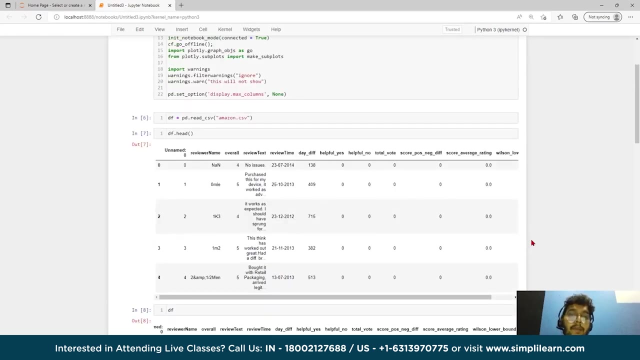 is specified. The drop method eliminates the designated row when the row access is supplied. So I hope you guys understand till here. If you have any queries or like any queries regarding any code or there is something question till here, just put as in comments. our team will. 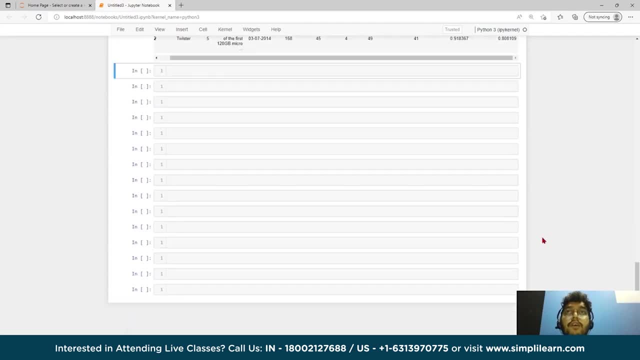 shortly provide you the correct solution. So, moving forward, let's make a function for missing values. So I will write here like df: missing values analysis analysis. okay, it's df for missing values. So I will write here like df: missing values analysis analysis. okay, it's df for missing. 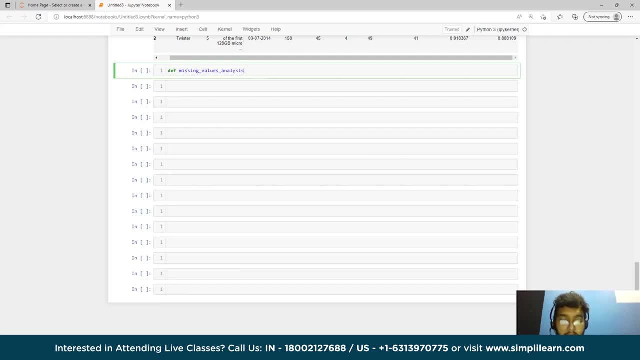 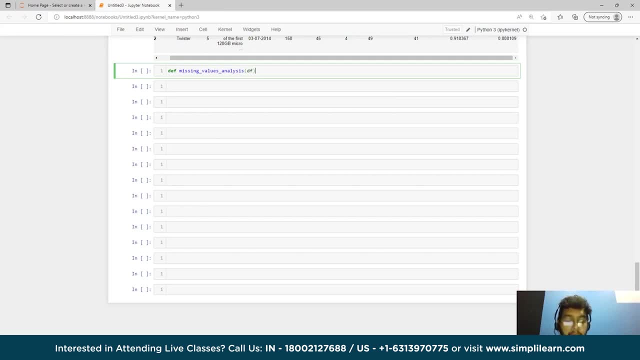 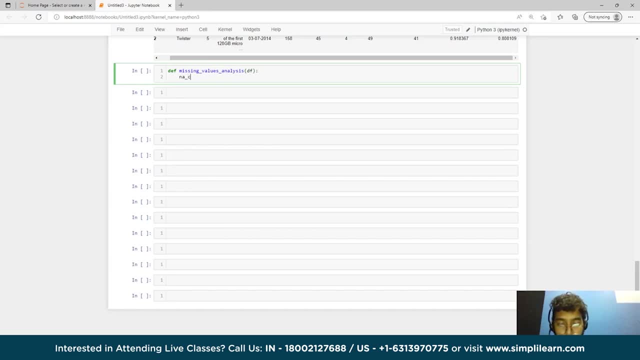 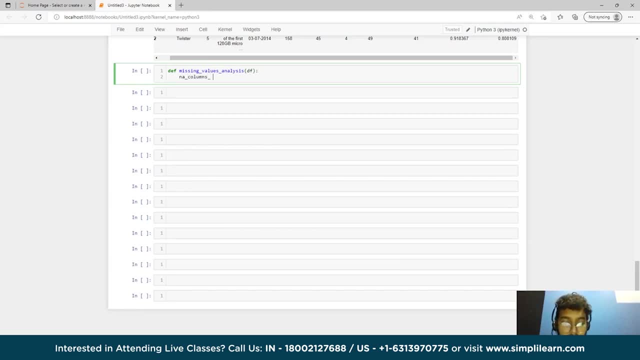 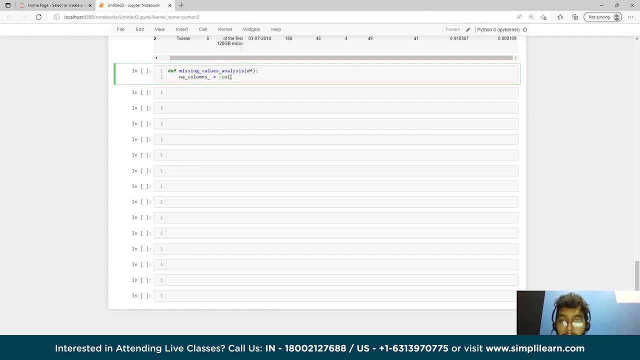 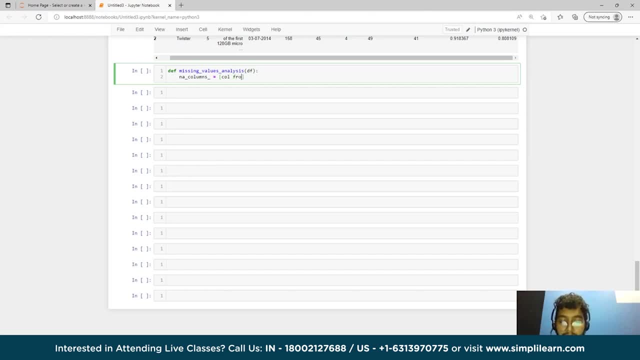 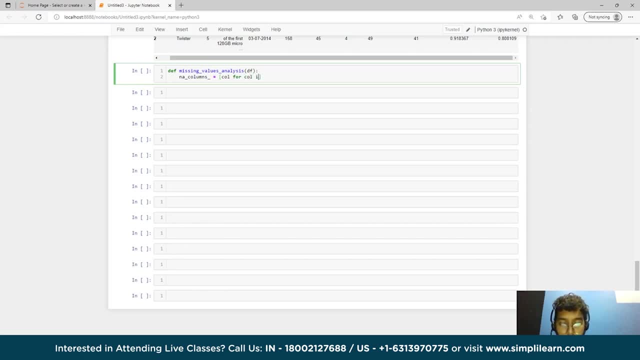 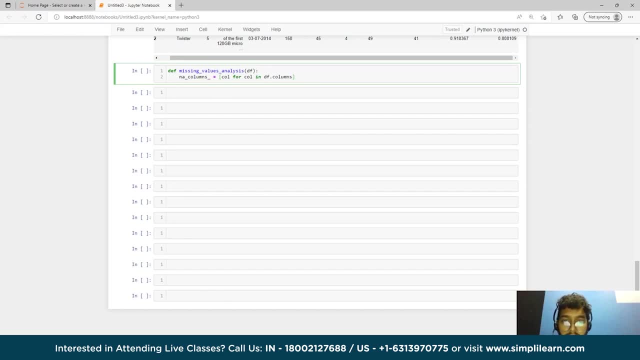 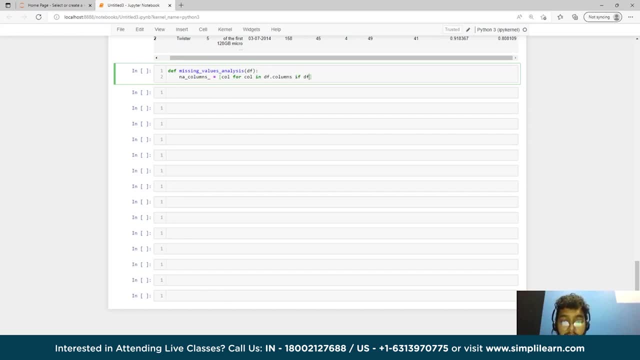 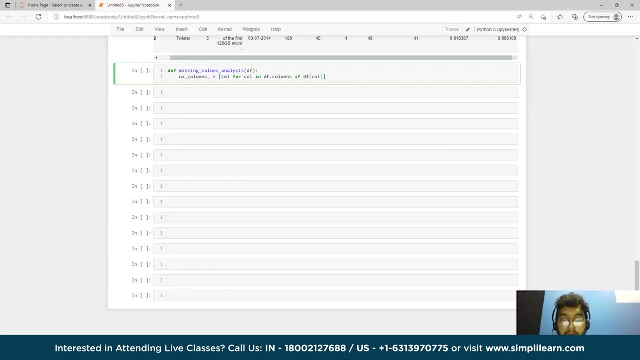 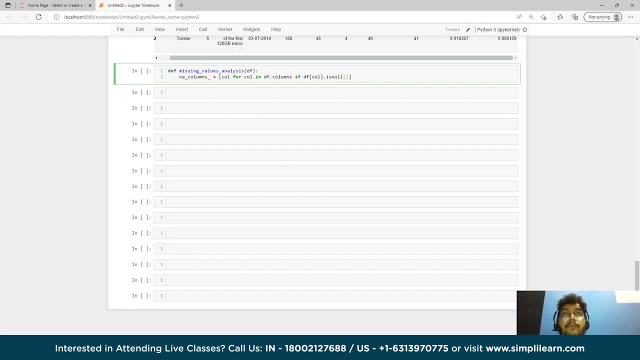 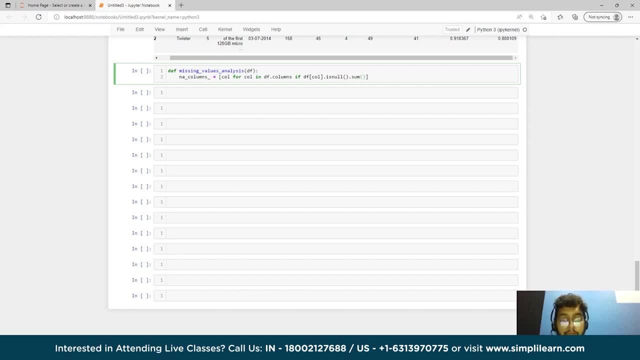 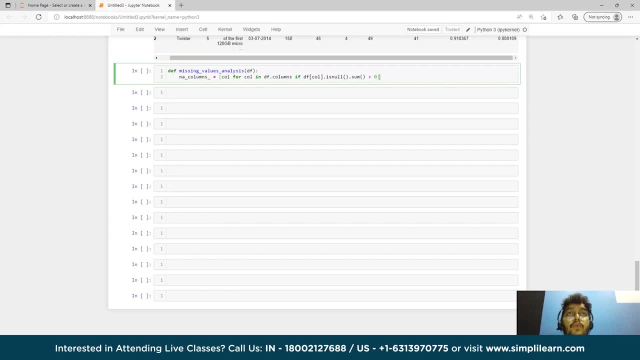 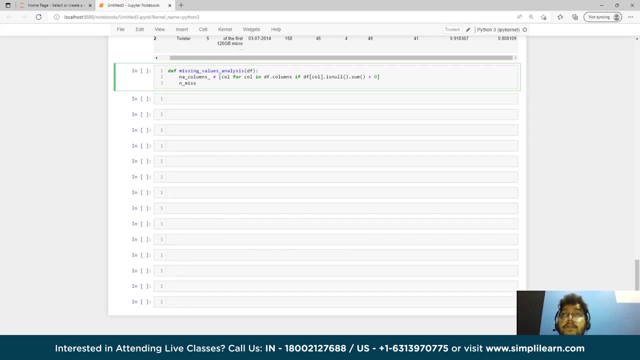 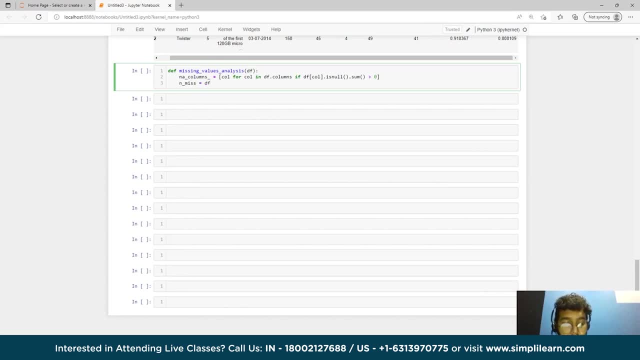 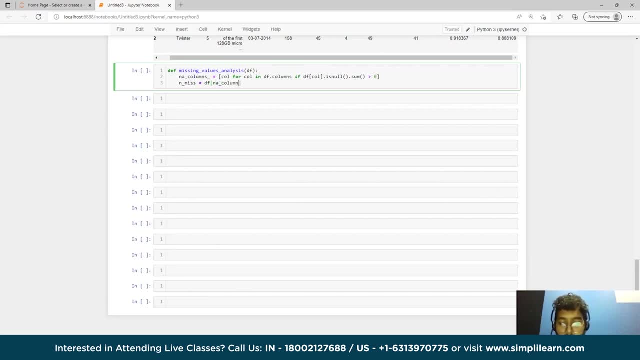 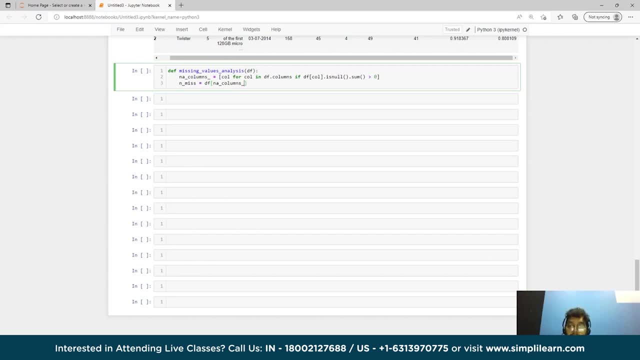 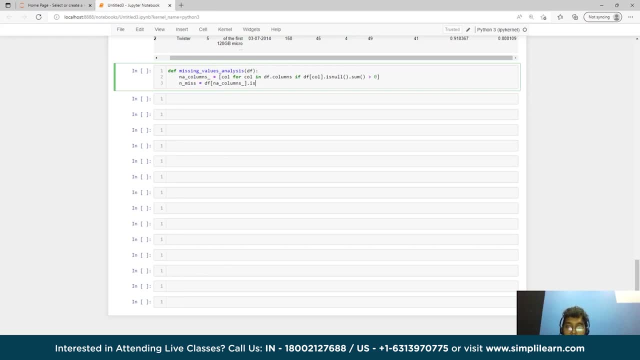 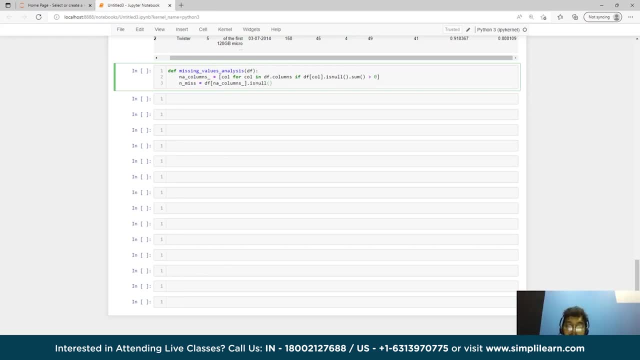 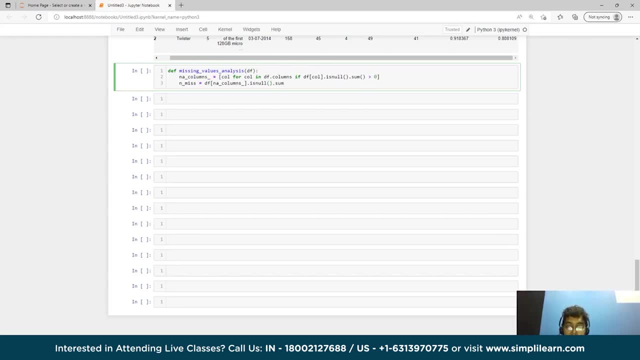 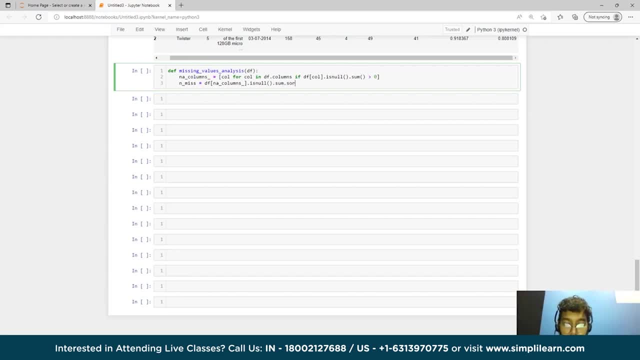 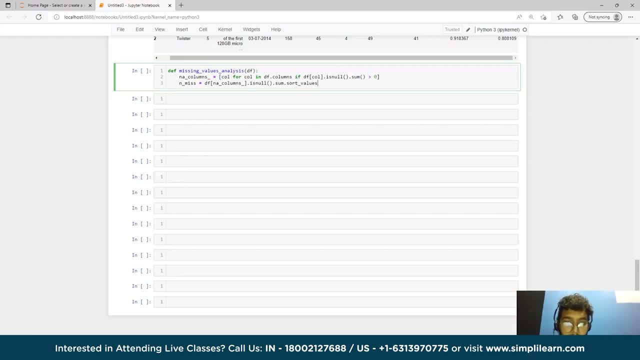 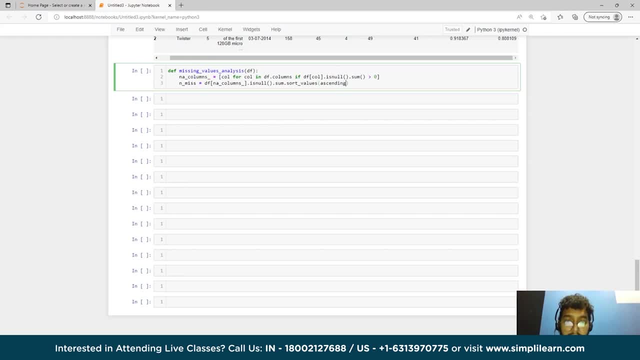 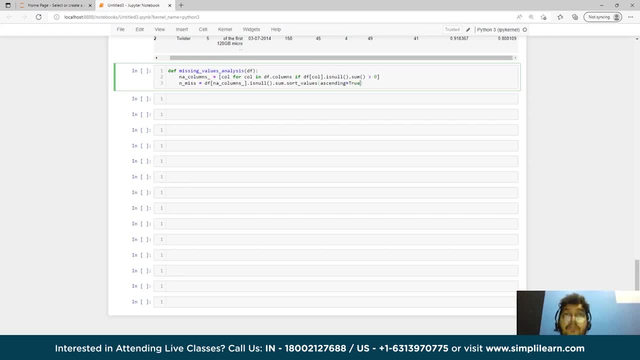 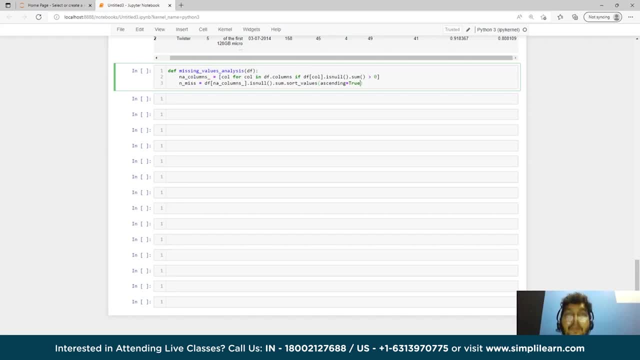 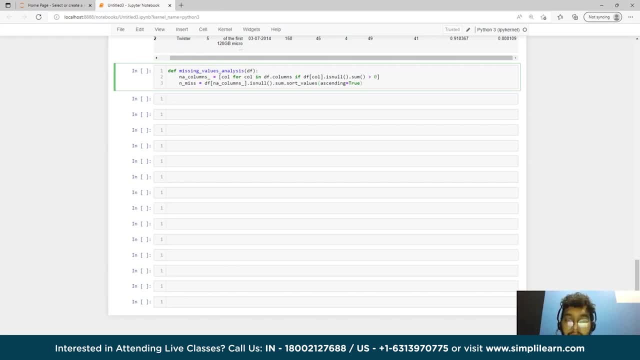 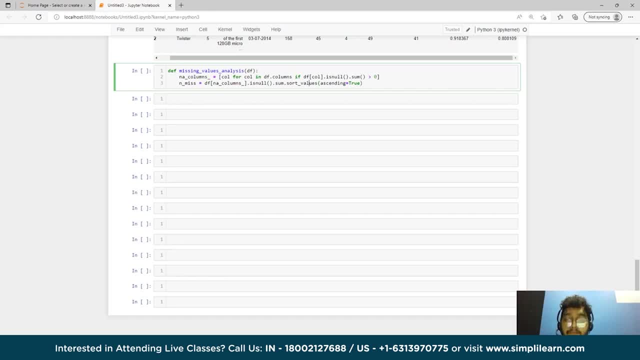 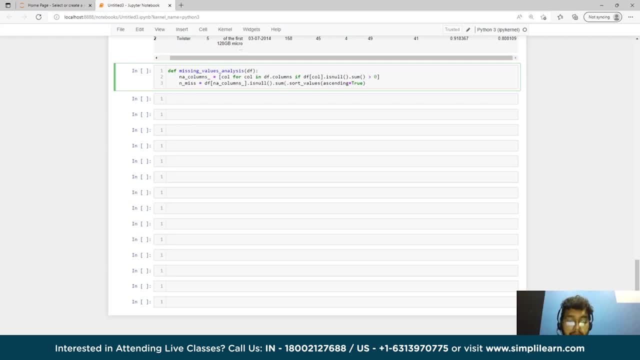 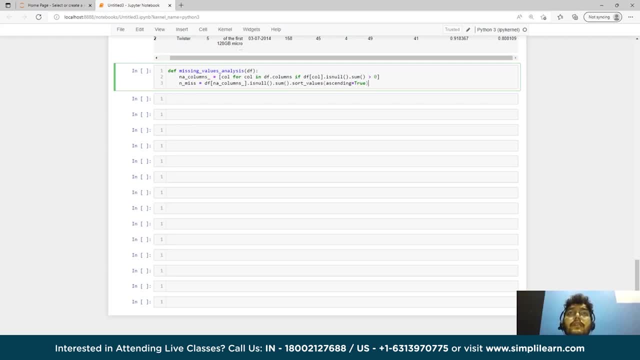 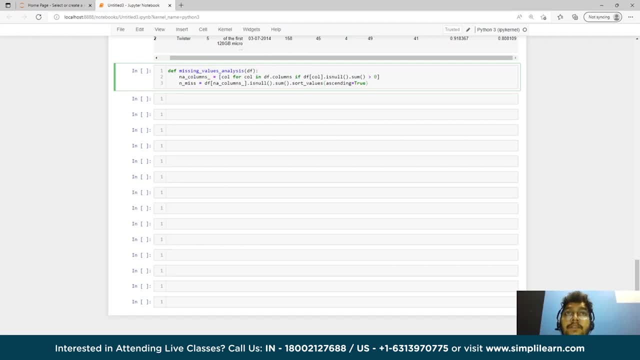 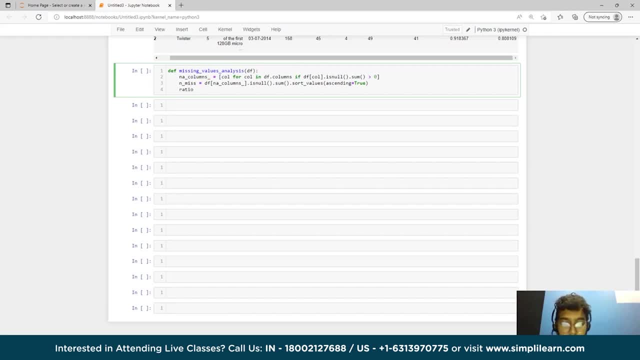 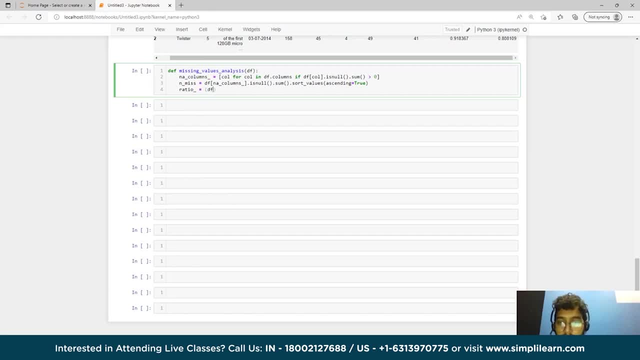 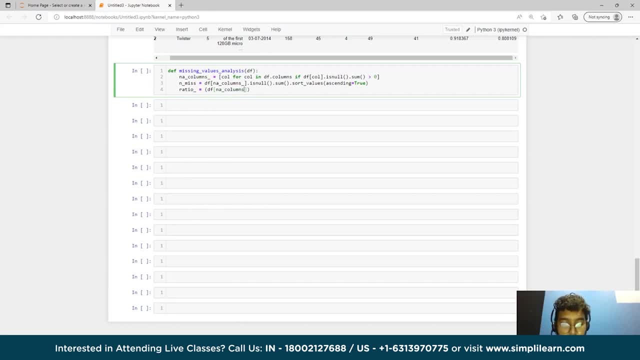 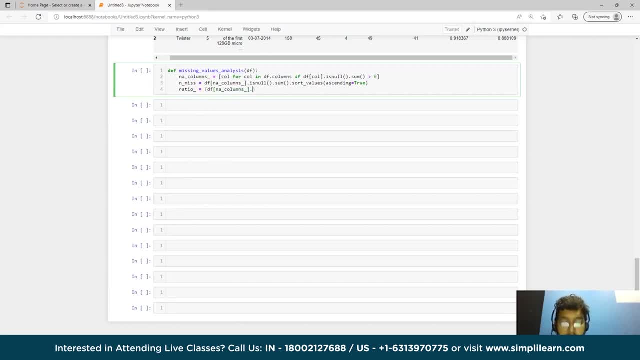 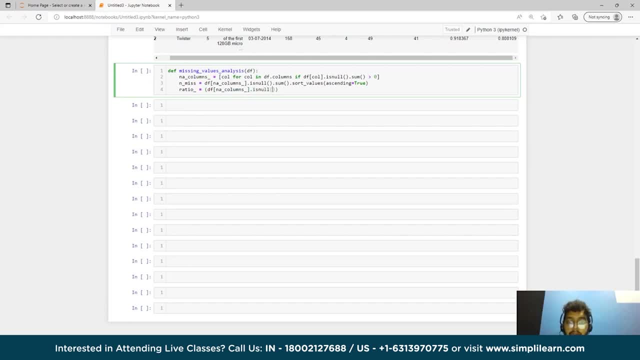 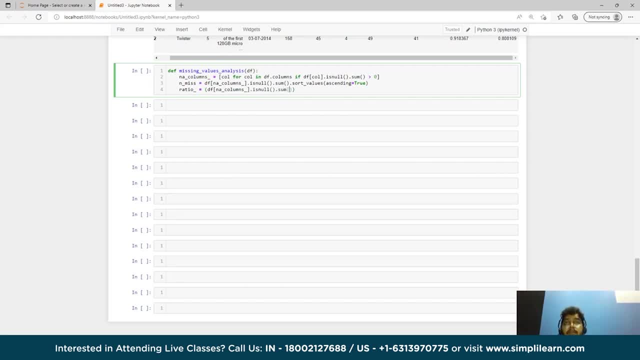 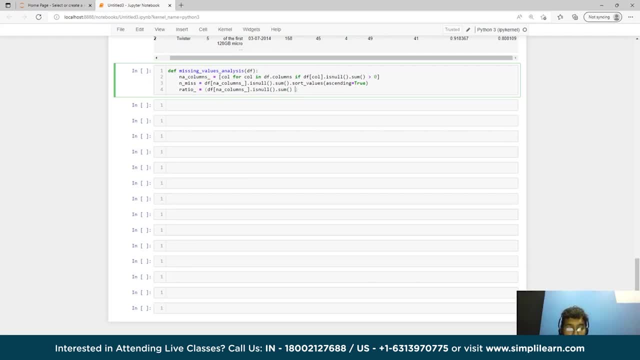 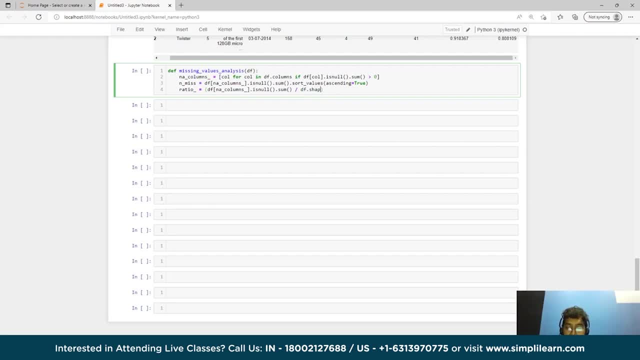 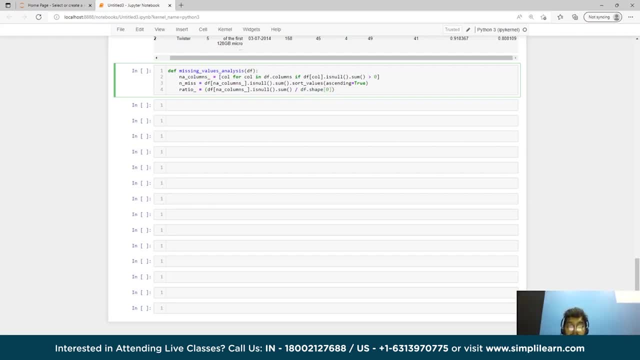 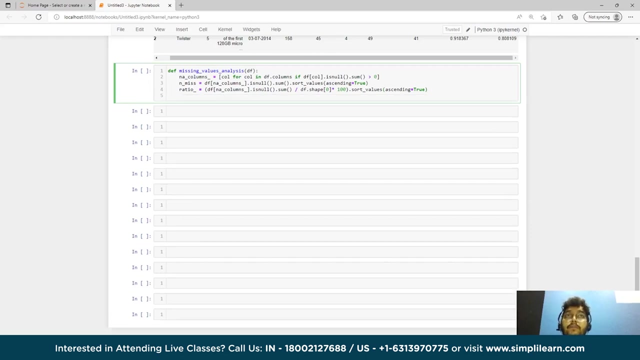 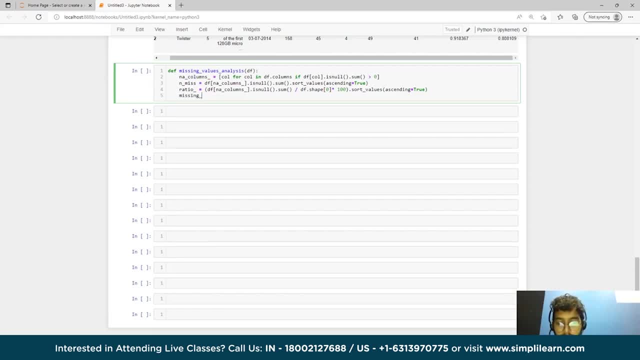 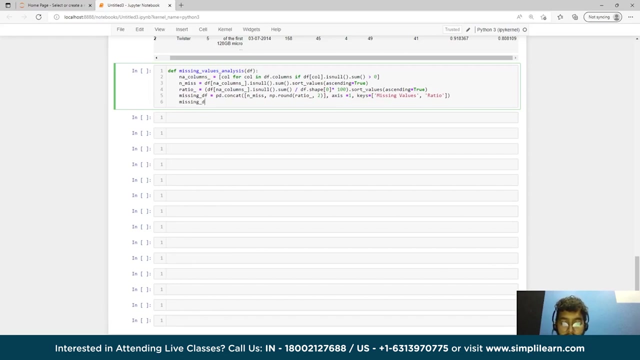 we will write missing underscore. DF goes to PD dot. CONCAT dot round issue underscore. comma to the perfect axis will be one: okay is equals to. I will give like total. I will write missing values: missing values: okay, comma ratio. you thing DF equals to PD dot. data frame. 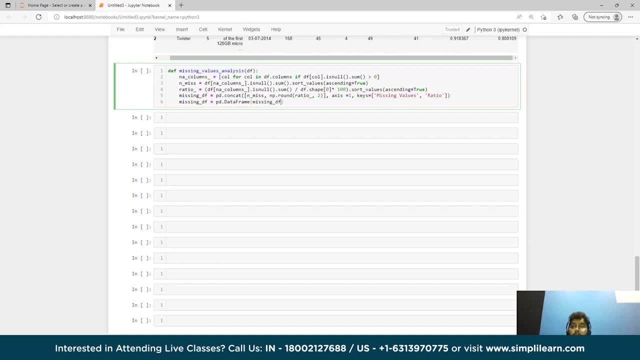 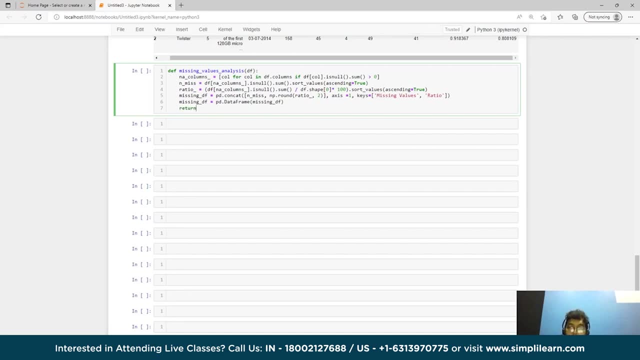 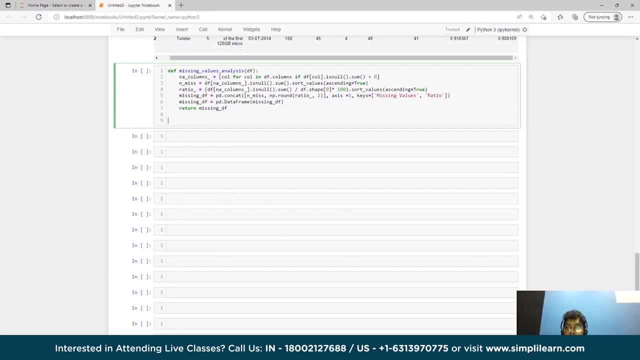 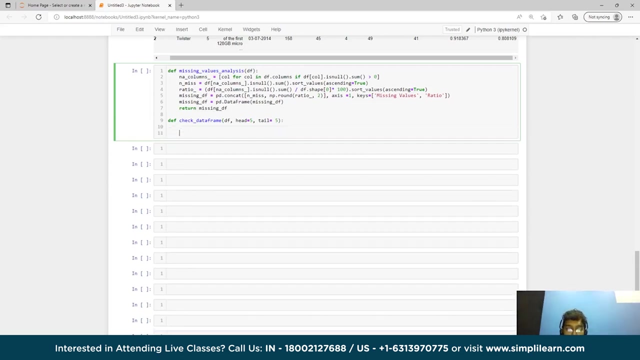 score DF. yeah, so let me return DF. let me create one more function for, like chat data frame. so be a that underscore data frame. okay, it equals to five comma tail equals to five you. so here I will write: print, print a. okay three, cida, center again for Rose print. 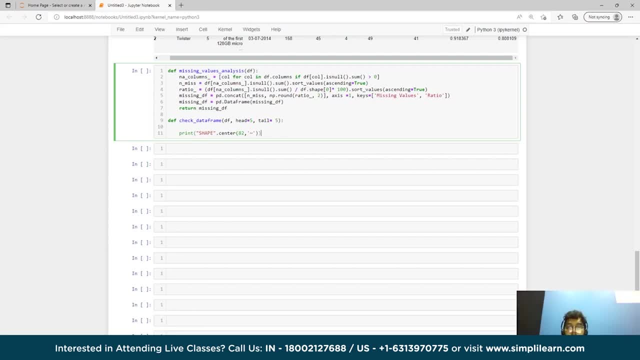 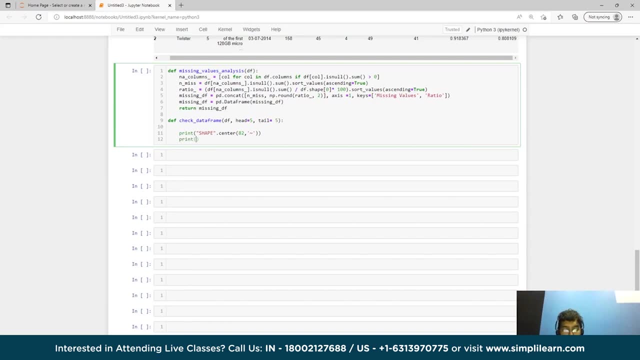 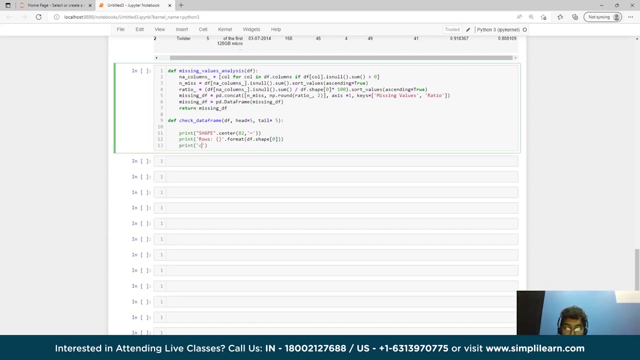 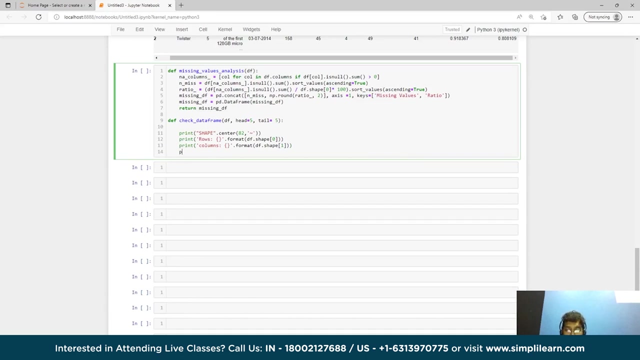 in for Rose print and you should get. the reference part is given. here goes curly braces, format, format. 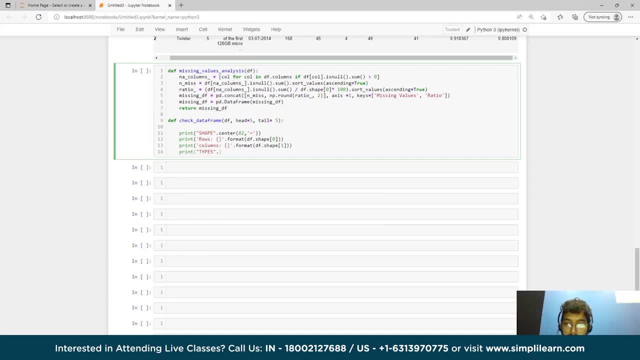 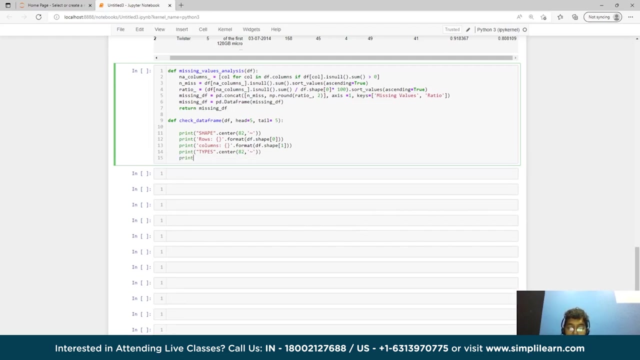 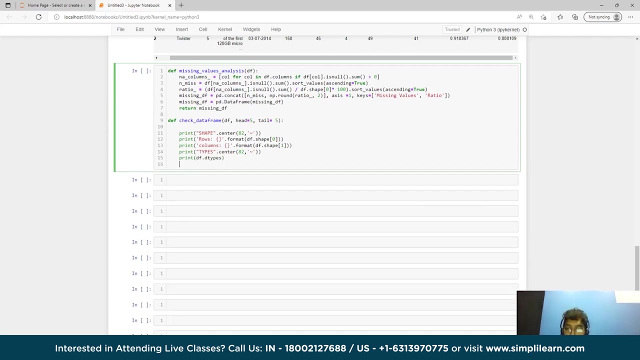 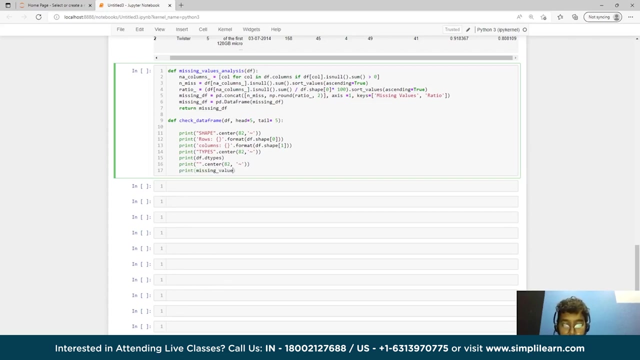 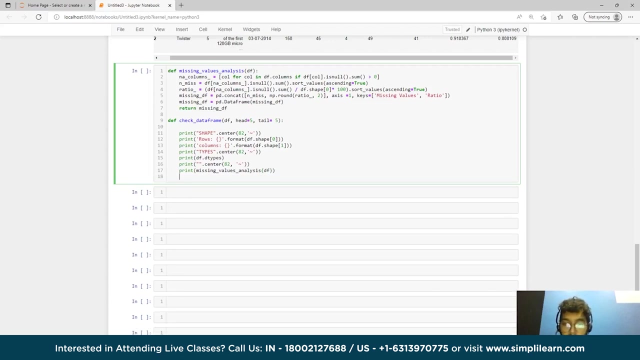 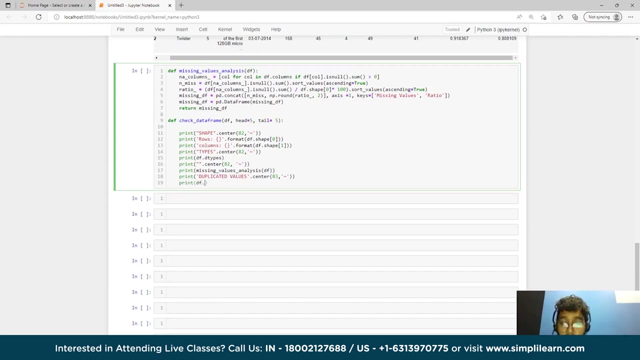 and the. in this end you have dot duplicated. don't worry, i will explain you like line by line. just stay with me, let me write the whole. 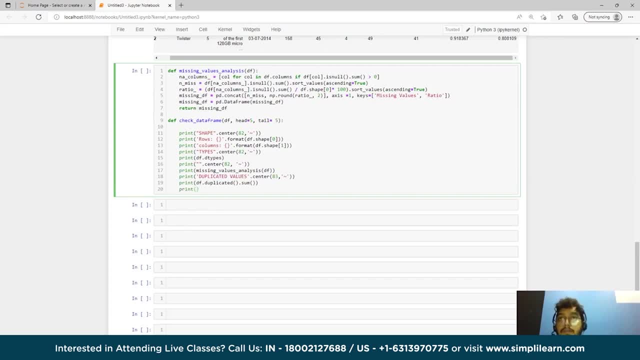 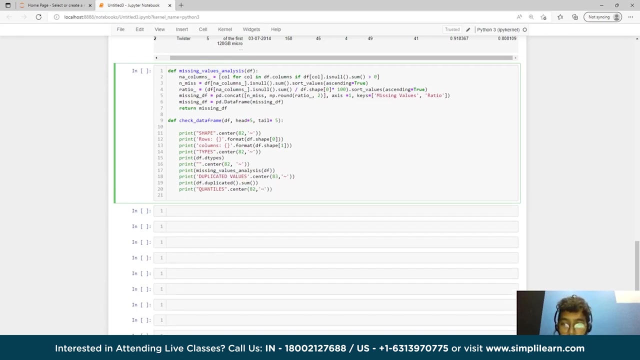 code: first print: guys like i'm printing multiple of things, so just be with me, enter, okay, okay. 82 pf dot one tile: 05 06 07 08 09 010, 011, 012, 013, 014, 015, 016, 017. 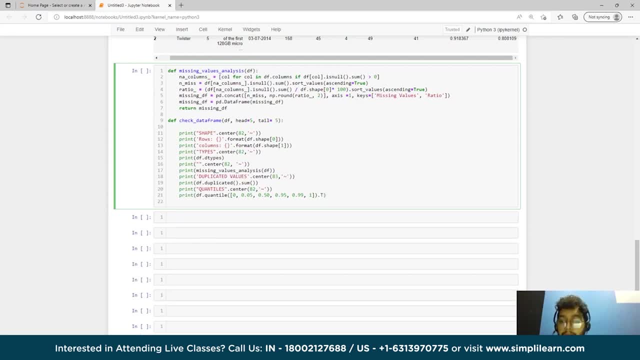 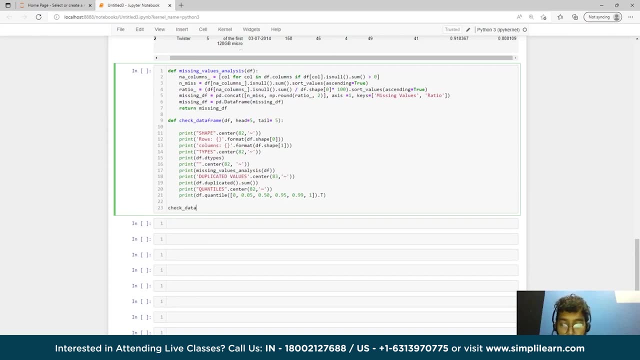 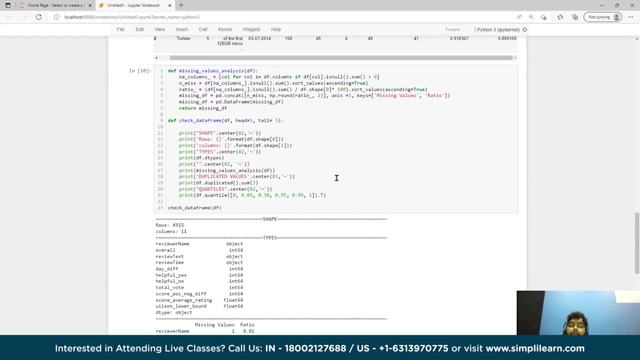 019, 020, 022, 023, 024, 025, 026, 027, 029, 030, 031, 033, 034, 035, 036, 037, 039, 040, 041, 042, 043, 044, 045, 046, 047 048. 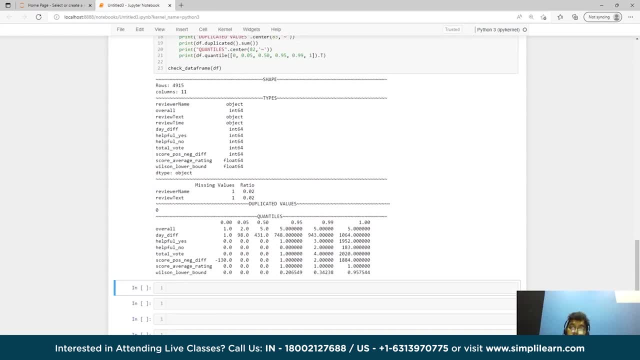 049, 051, 052, 053, 054, 055, 056, 057, 058, 059, 059, 059, 060, 061, 062, 063, 063, 064, 064, 064, 065, 067, 068, 068, 069, 069. 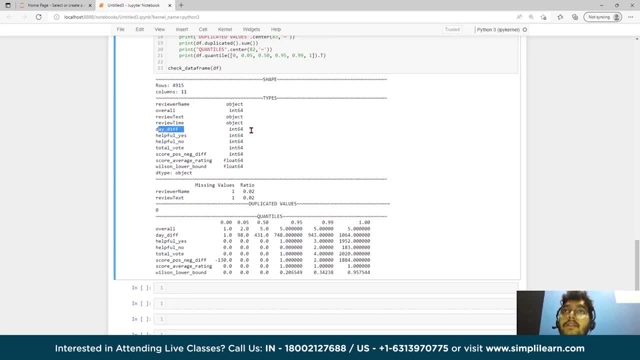 070, 071, 072, 072, 073, 073, 074, 074, 075, 076, 076, 078, 079, 079, 080, 090, 091, 092, 093, 093, 094, 095, 096, 096, 097, 098. 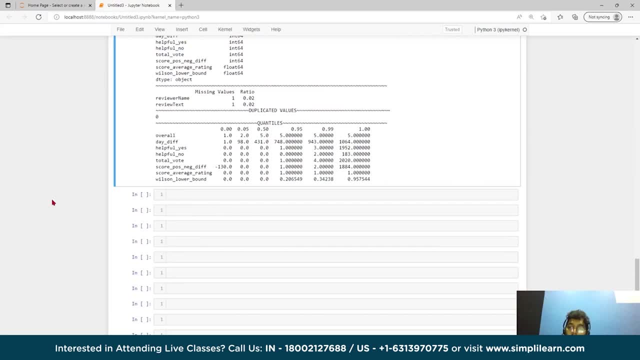 098, 099, 099, 099, 090, 090, 099, 099, 010, 011, 012, 013, 014, 015, 016, 016, 017, 019, 020, 023, 024, 026, 027, 028, 028, 029. 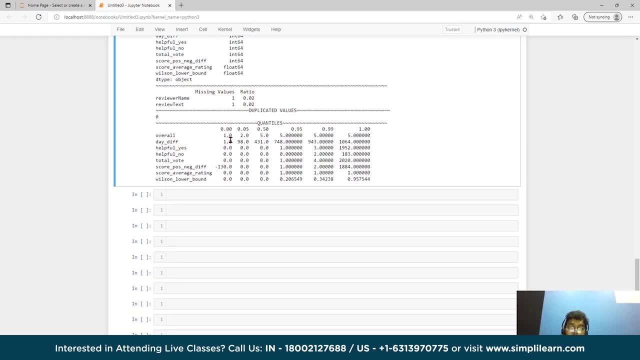 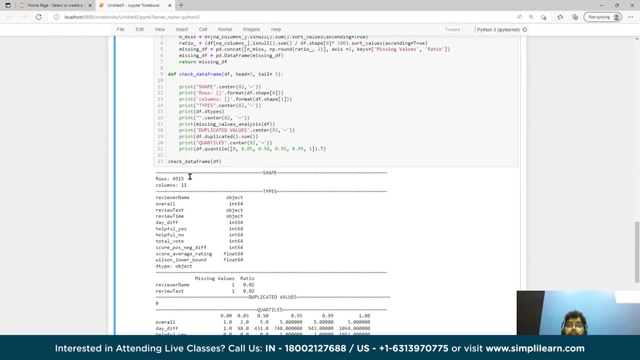 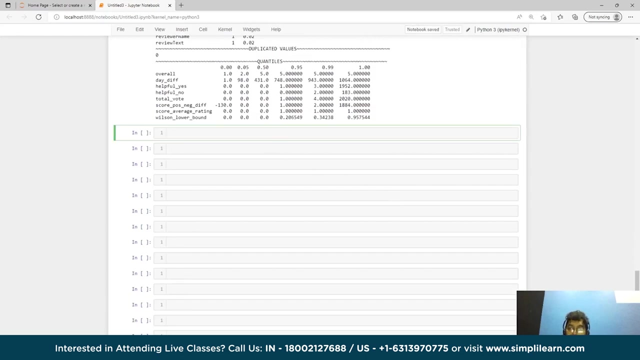 030 032, like quarter or the- you can say the fifth one. so why i wrote this 83, 82 and this for this purpose, for making this something look cool. that is why, okay, and so, moving forward, let's see unique values, and in each column. okay, so i will write def. 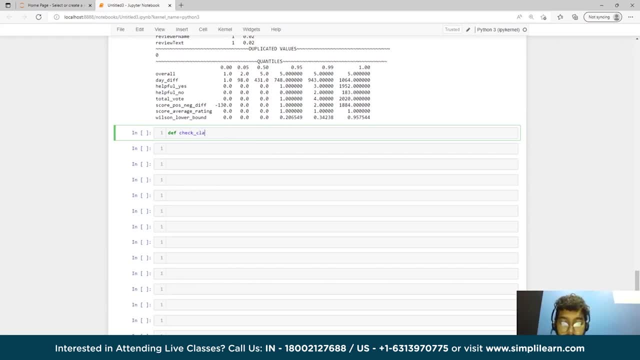 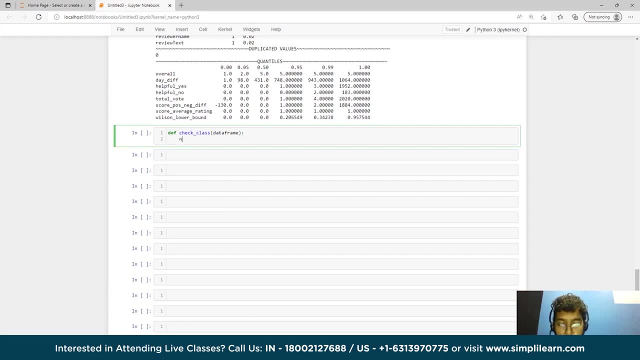 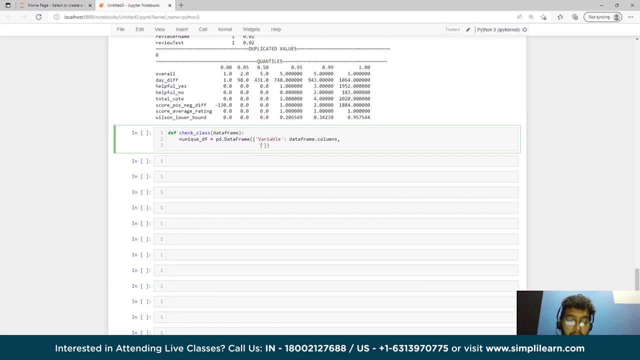 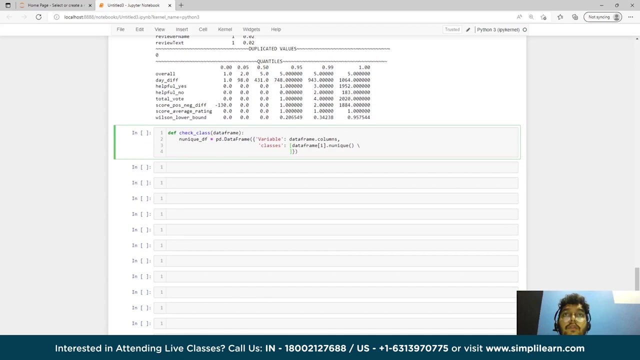 check class frame unique: f equals to pd dot data a frame variable variable. the frame columns, comma, classes, colon data frame i. i will write like n unique unique to ue or i in data frame dot columns. like n unique, unique data frame dot columns. like n unique, unique. 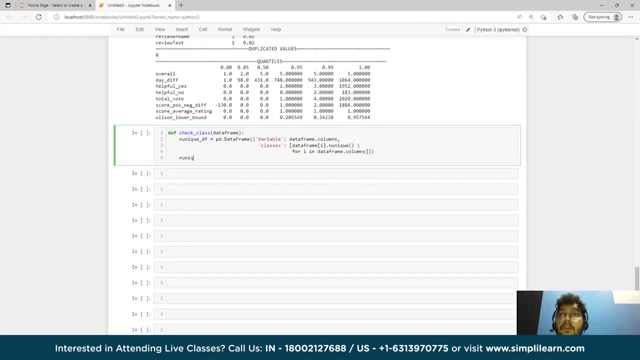 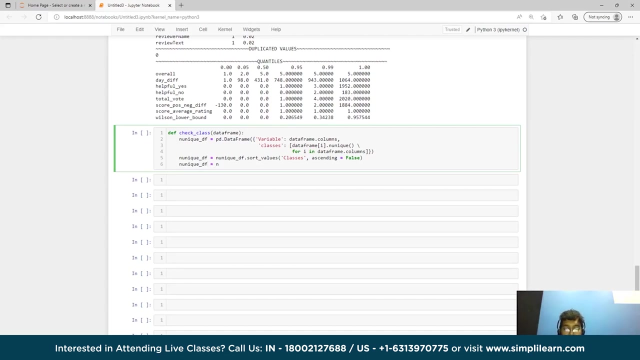 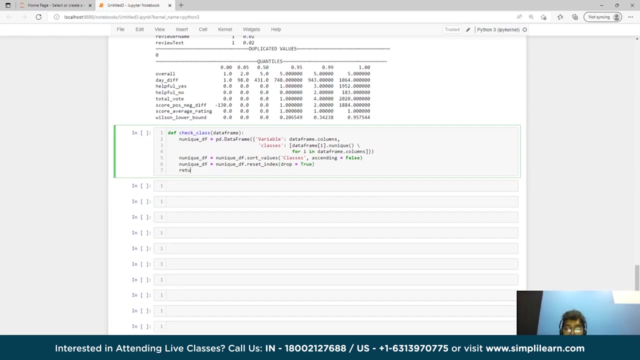 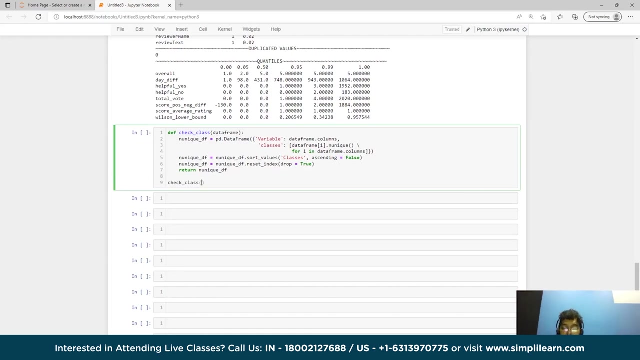 data frame dot columns like this: and unique for df equals to dot sort values. passes comma. ascending question: false. okay, and unique. unique underscore df equals to n. unique df dot reset index drop equals to true return. and unique check que. and unique df check underscore class which one df. 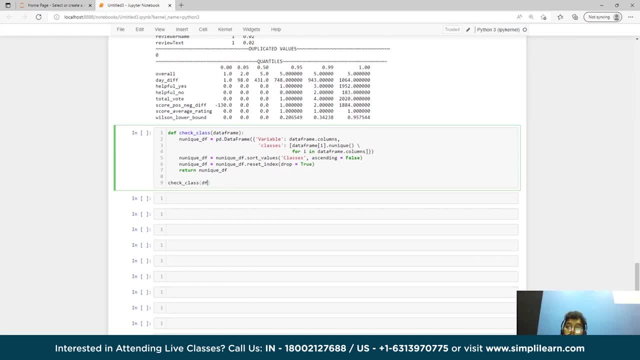 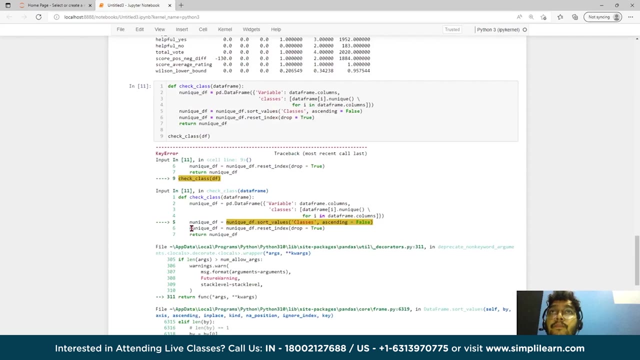 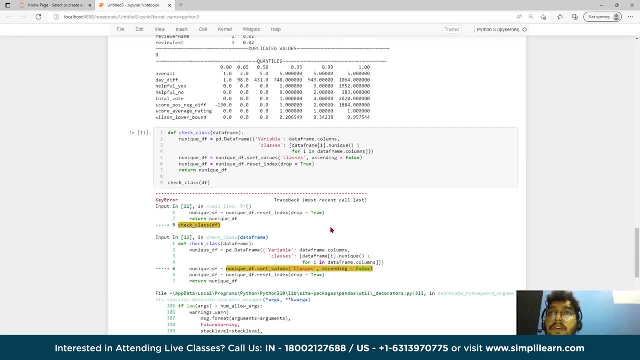 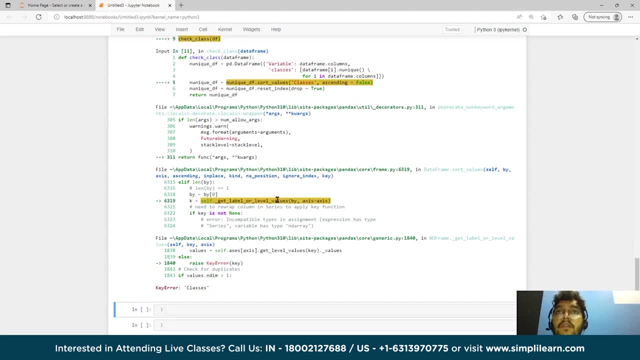 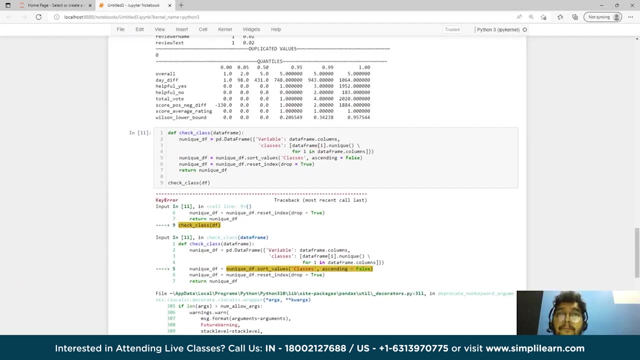 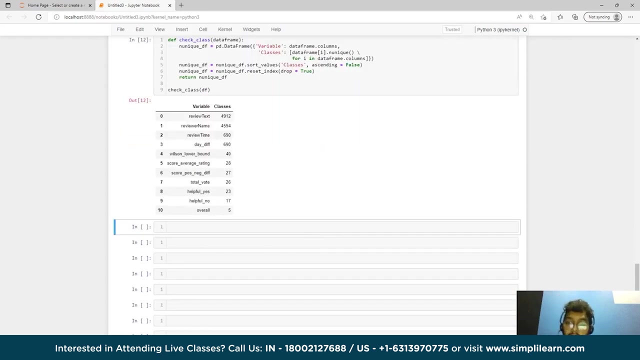 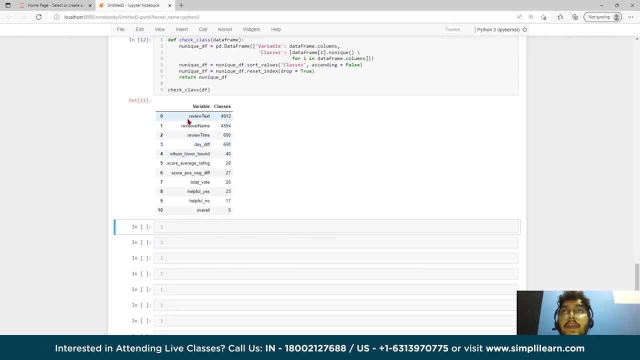 so here you can see the every column. so here you can see the every column. having unique values are sorted in. having unique values are sorted in. having unique values are sorted in descending order: descending order: descending order: like review tags have like more unique. like review tags have like more unique. 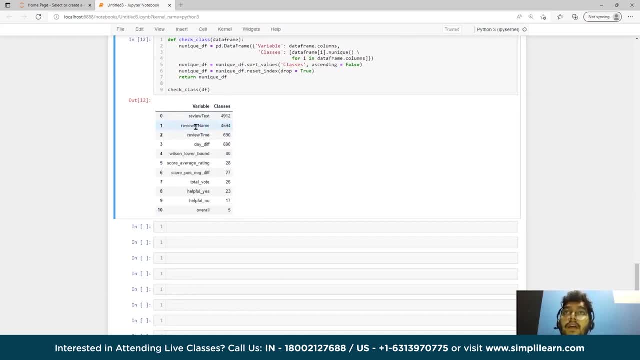 like review tags, have like more unique values, values, values. so it come first and then review your. so it come first and then review your. so it come first and then review your name. review time day difference. wilson name review time day difference. wilson name- review time day difference. wilson- lower bound. 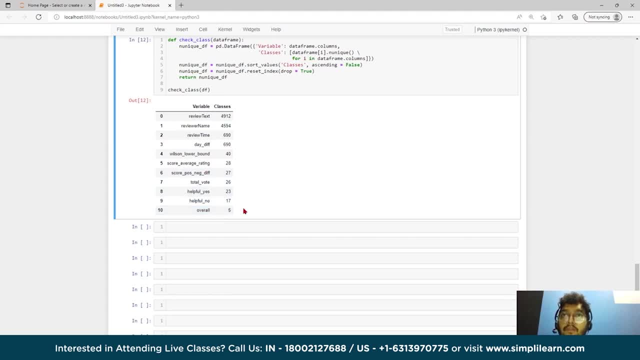 lower bound. lower bound score average. then goes to overall score average, then goes to overall score average, then goes to overall. okay, moving forward, let's do some. okay, moving forward, let's do some. okay, moving forward, let's do some categorical variable analysis for overall. categorical variable analysis for overall. 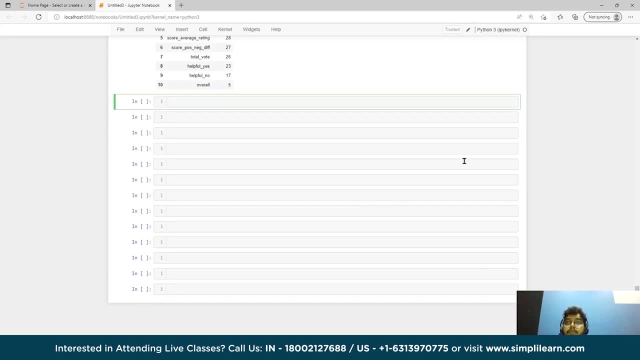 categorical variable analysis for overall. yeah, so this will be like amazing. yeah, so this will be like amazing. yeah, so this will be like amazing. something amazing is going to be happen. something amazing is going to be happen. something amazing is going to be happen. so constraints equal, so, so i am giving here. 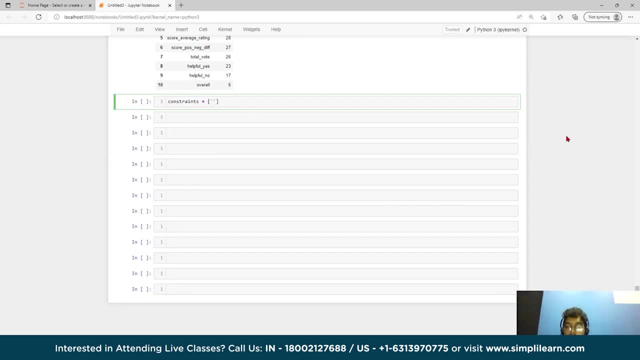 constraints equal. so so i am giving here constraints equal. so so i am giving here like some, like some, like some color values. so v34, v34, v34, d, d, d, 22, e, b, e, b e b, 00c, 00c, 00c. okay. 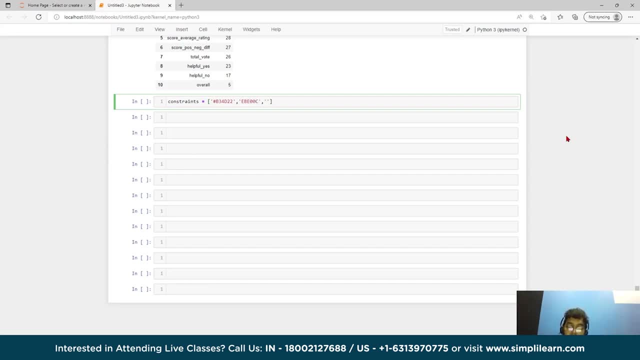 okay, okay, so you can change. you can like. so you can change. you can like. so you can change. you can like write whatever you want: color hashtag: oh i didn't write hashtag. yeah, hashtag. oh i didn't write hashtag. yeah, hashtag. oh i didn't write hashtag. yeah, hashtag. 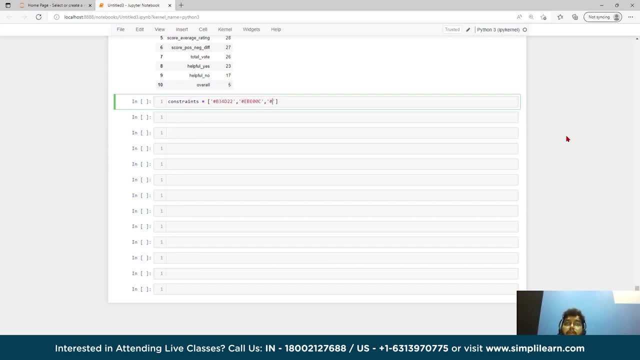 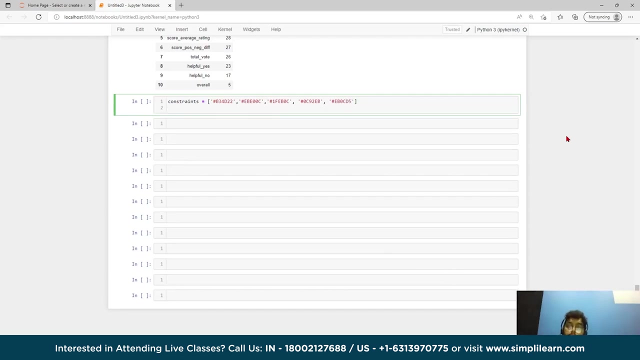 three, three, three come three, three, three, one done one, zero c, zero c, zero c. nine two, nine two, nine two, tb, e, be, e, be, e, be zero, zero, e be zero, see, see, see, see, and then and then d, you like five, right, okay, so df, let's make function, okay, small df. categorical variable. 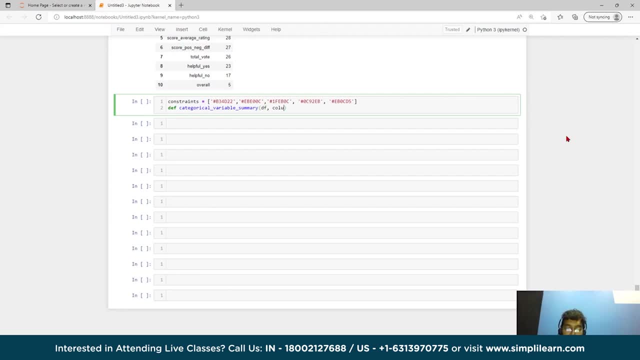 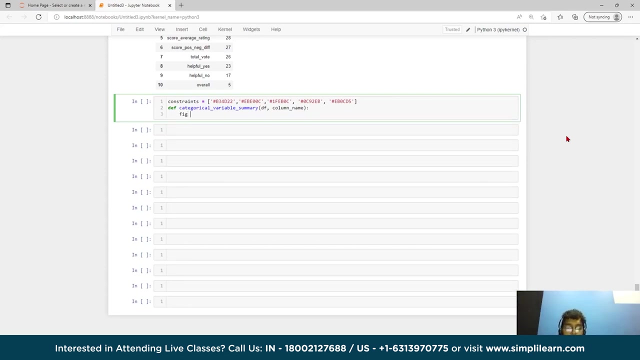 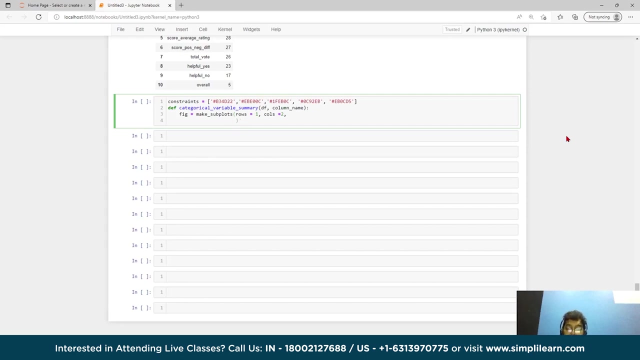 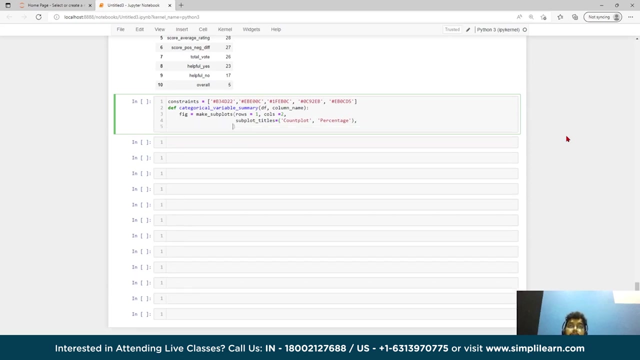 okay, df comma column: okay. categorical variable summary: yeah, perfect. so let's make some figures, so make subplots. odds rows equals to one, comma calls equals to two. let me write from here: like: subplot titles goes to count plot like one for percentage percentage: okay, so specs. speech goes to. 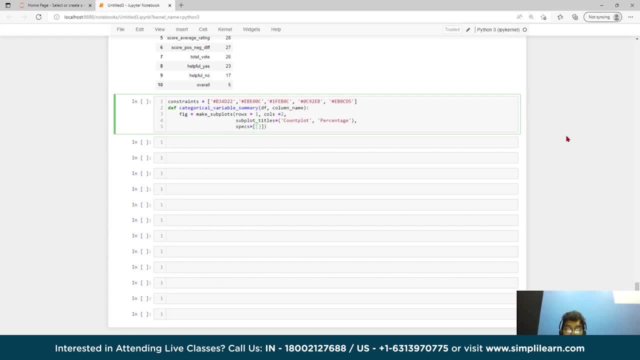 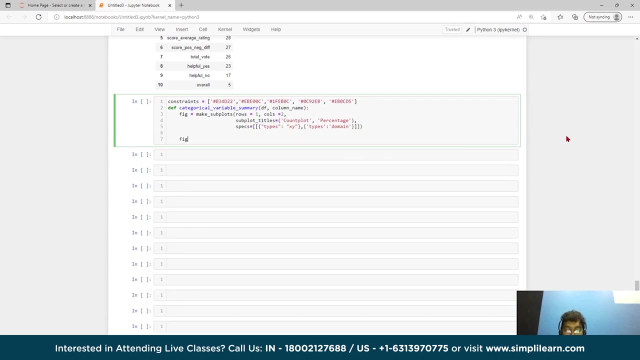 okay, like that. so let's make some figures. okay, okay like that, okay like that type colon, colon. that's why, okay, same type column here, domain figure, dot add and then trace dot bar, one bar and one that pie chart. okay, y opposed to df columns, column name. 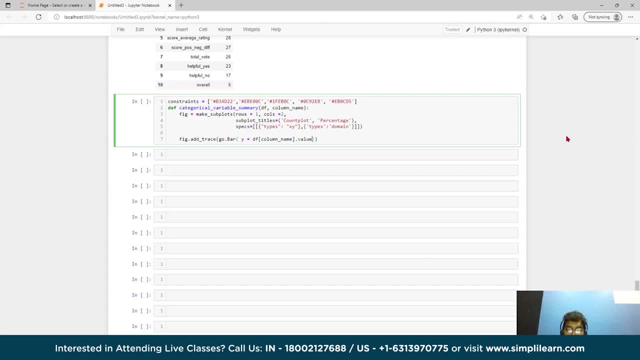 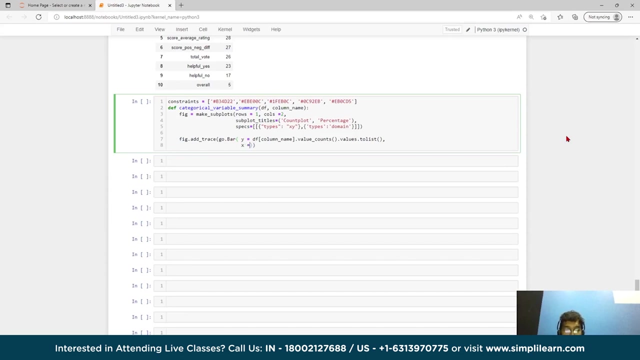 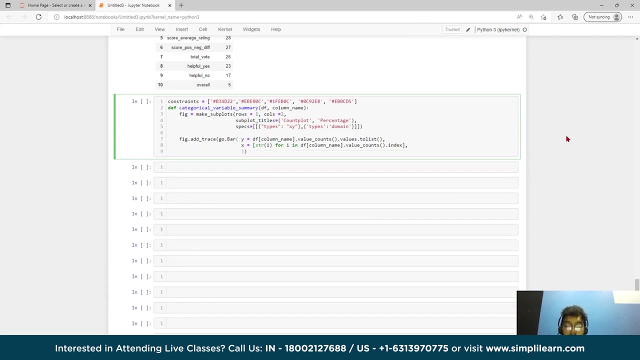 value values. dot to list values. dot to list values for x. you can link string string for x. you can link string string string string string. Yeah, str i for i in column name dot value dot counts. Next next equals to df column name dot value counts and then bracket dot values. 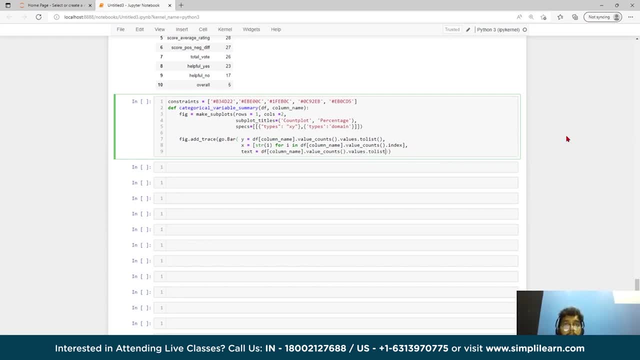 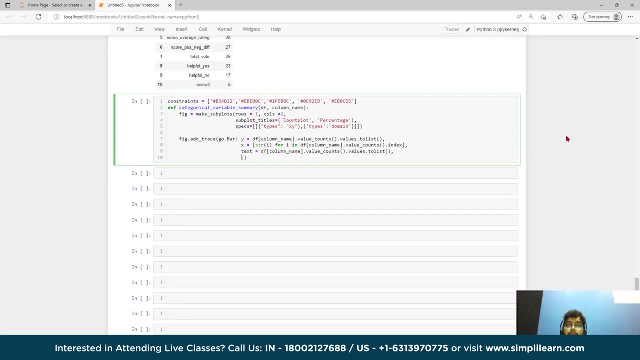 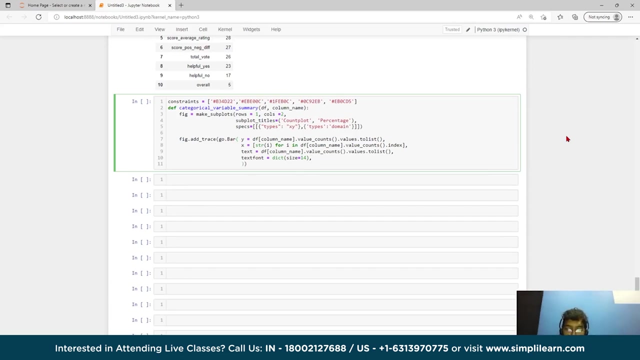 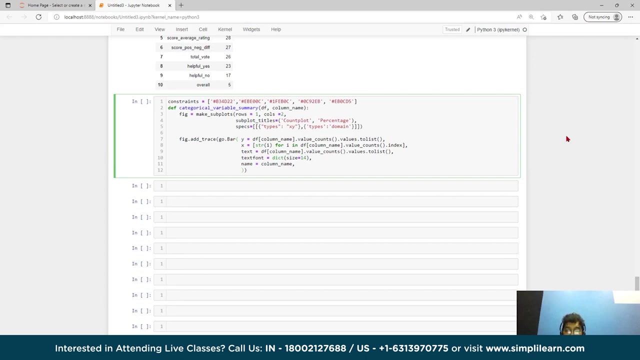 dot to list. Okay, Go for text font. The size should be 14 is enough, I guess, Okay. Okay, Just do column. Let's go name Exposition. So I'm doing for, like making chart. So stay with me to see that amazing chart. 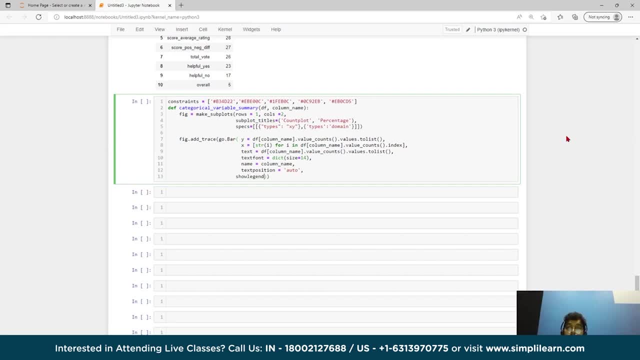 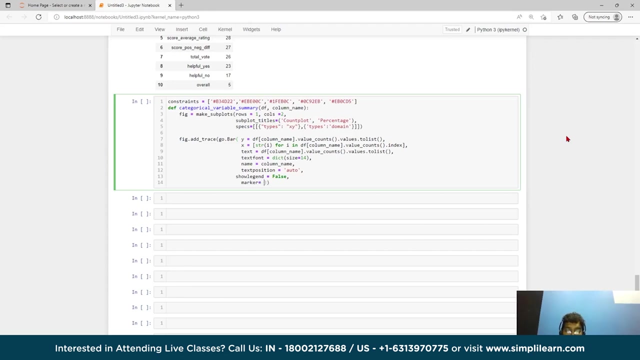 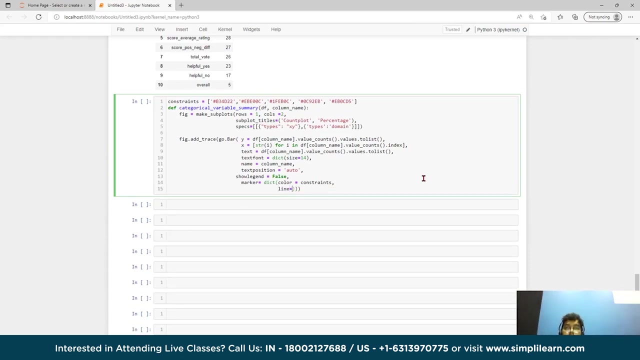 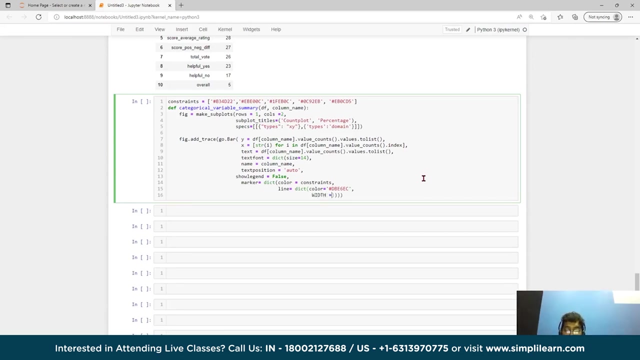 Okay, So show legend. so these are the like colors. so I'm giving a value like very variable name cost trends on my line because to hashtag db e6: easy mama one, okay, small you, you, hey, let me just like go over to. everything is correct or not for the 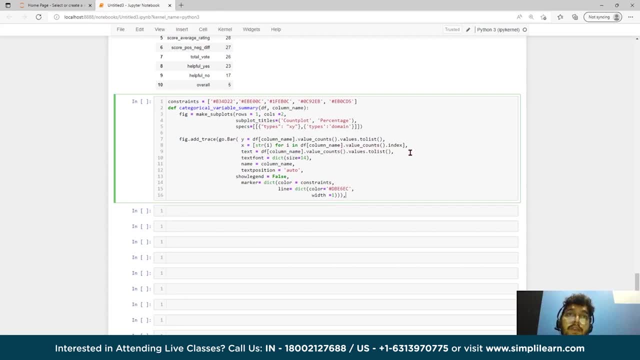 column really counts. index- yeah, it's fine. text equals to DF column name. dot value counts that values to list? okay. text font equals to take size, then okay for them. size is enough. name equals to column name and text position equals to auto and show legend falls and mark dict like: 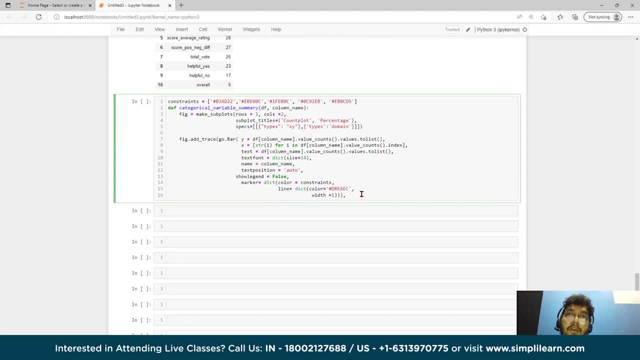 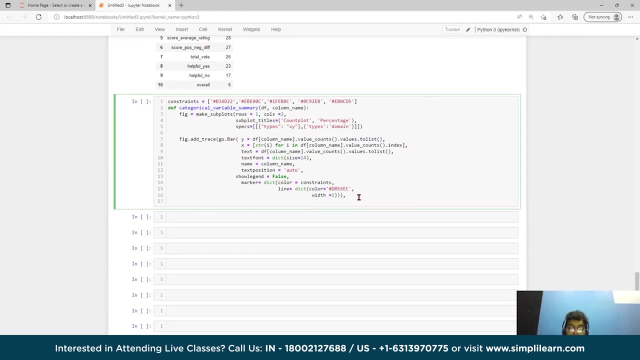 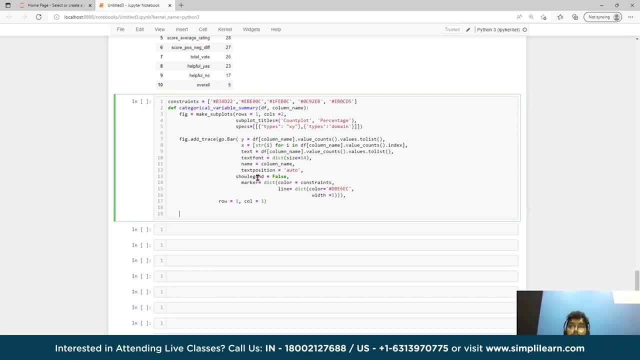 color equals to constant. okay, fine, line equals to color. and this, yeah, this, okay, cool, Oh, equals to 1. comma column equals to 1. seems good like for pie chart. we will make figure dot add. so this is done for the light line chart, not line chart, that bar chart, and this I'm doing for the pie chart. 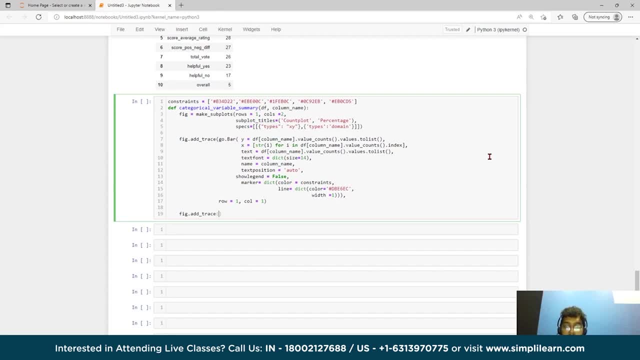 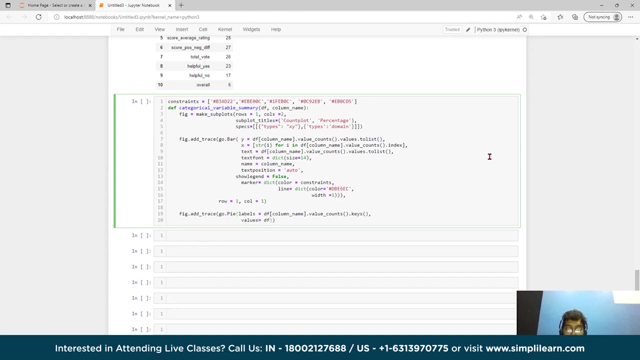 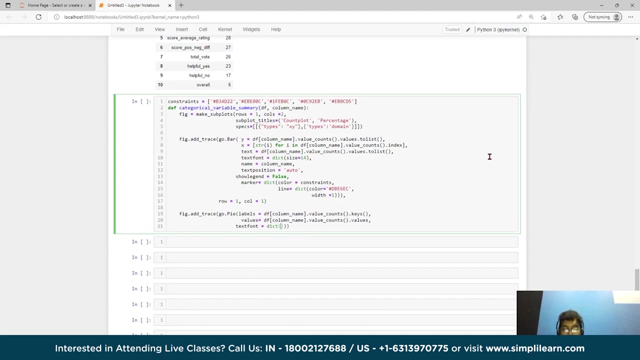 okay, trace, go dot. I, you, you, you, you, ok, yes, okay, ok, yeah, yes, go to DR again that column name value, count, counts and dot values, text font, text size: I will prefer 18 is enough. exposition: auto is fine legend, legend or legend also. no need of legend. 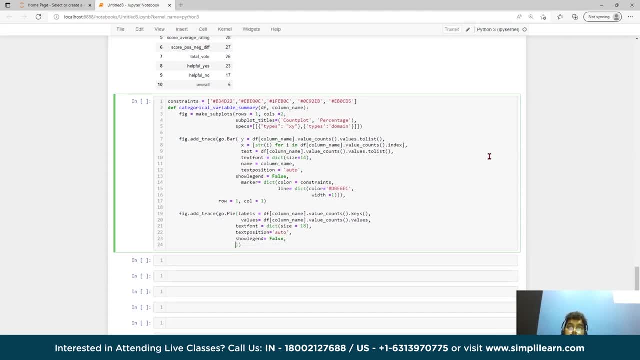 false name equals to column name. name equals to help me column name. ask quick Ashe first. oh, my date and colors goes to constraints because one column was you to like in second. okay, you will see and you will get to know, don't worry. so figure dot, update the out. 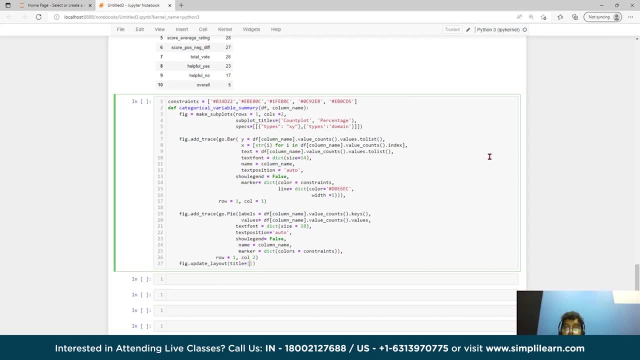 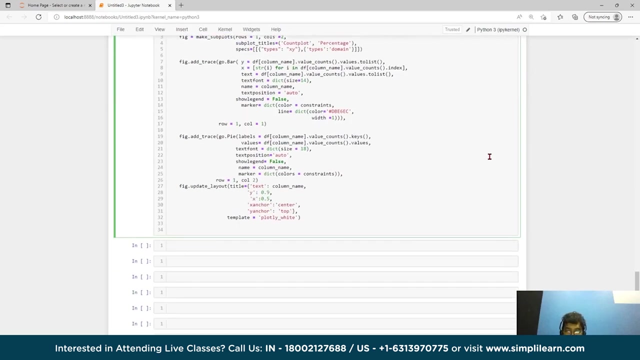 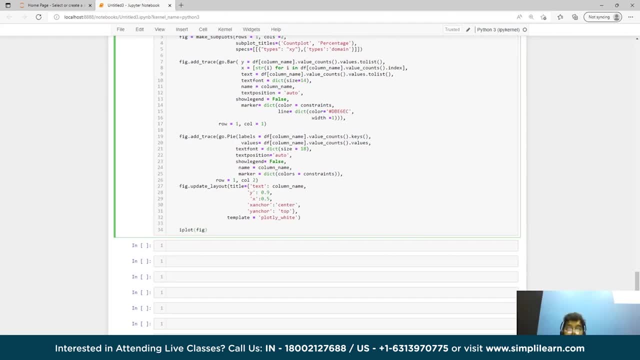 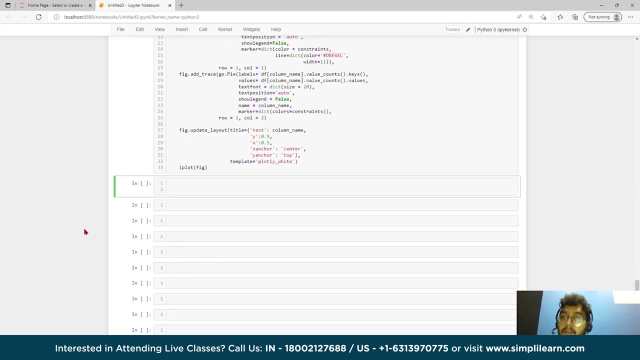 let me run this. okay, like: call equals to two. now let's see the chart of like: column: overall: one. so we will write here: categorical, okay, variable, variable summary, and then data frame: name: df, comma, overall. okay, let's run this. okay, it's loading here. it's loading. 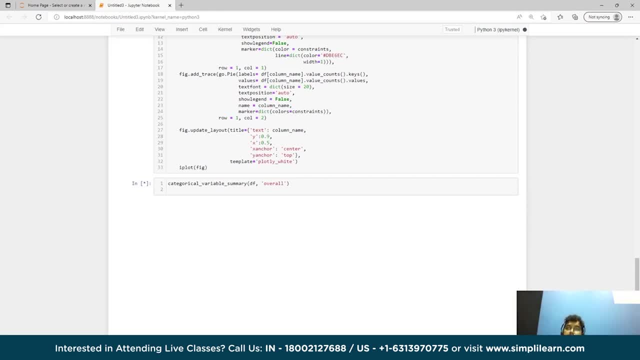 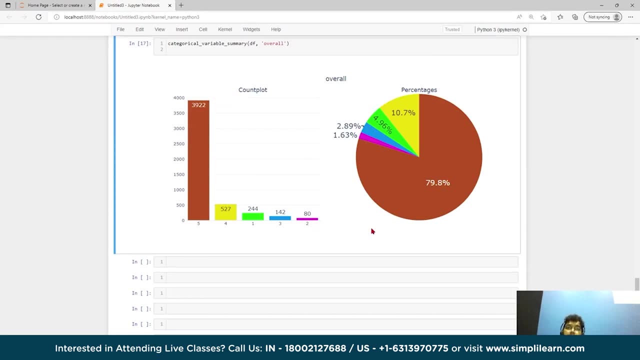 yeah, you can see, this is this is our bar plot and this is our pie chart. so like this is overall. uh, from overall, you can say that column, so like percentage bar and that bar plot. so this is how our like pie chart and bar chart looks like. i hope you. 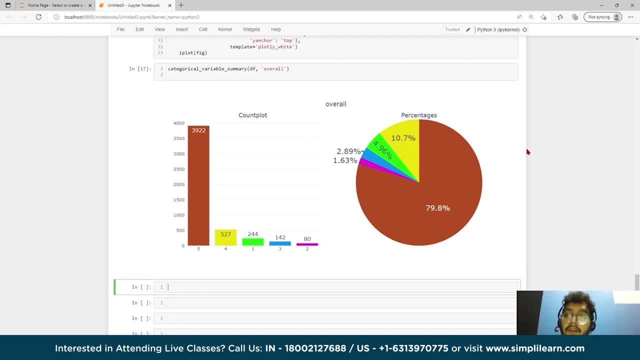 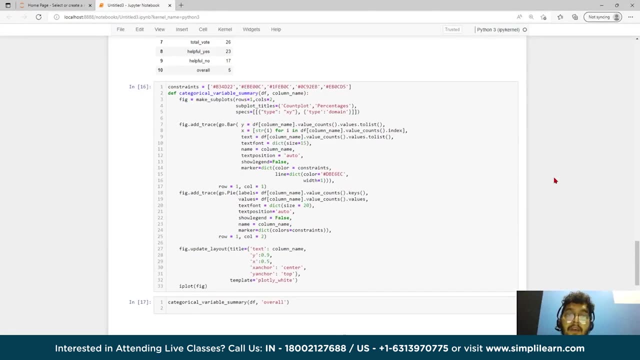 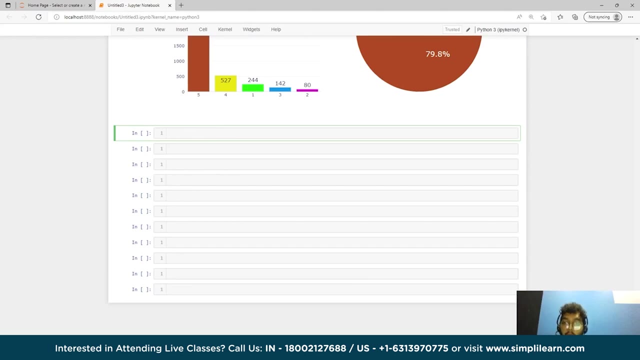 guys understand till here. if you have any questions or any query regarding any code, okay, like any code, any sort of code, you can write it down in the comment section. so just put as in comments. our team will shortly provide you and the correct solution. so, moving forward, our goal is to rank the com comments by the sentiment analysis, so we don't get. 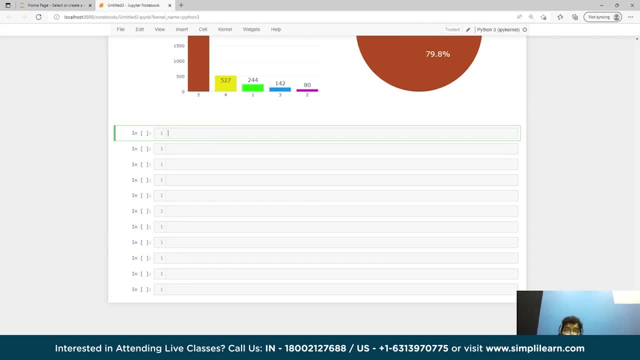 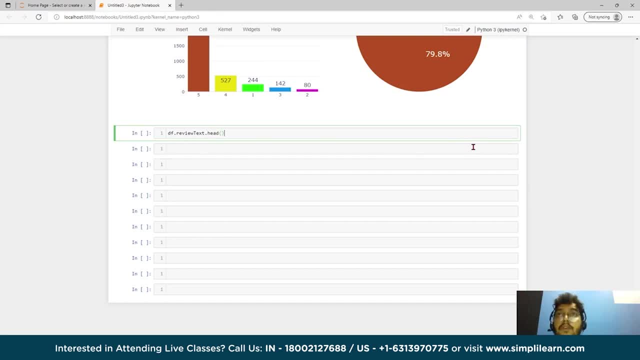 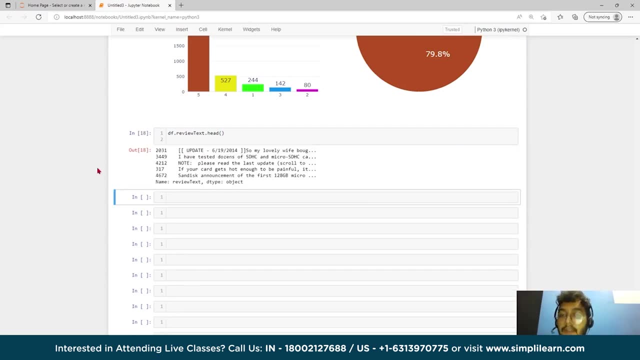 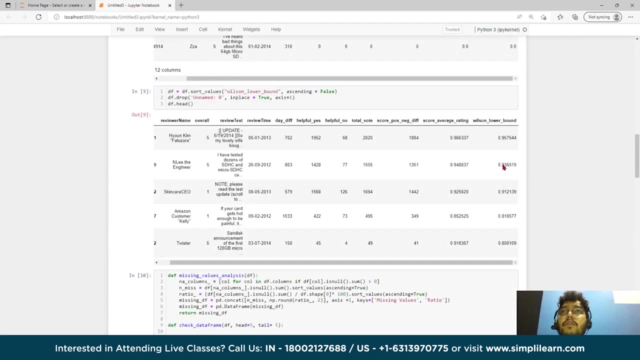 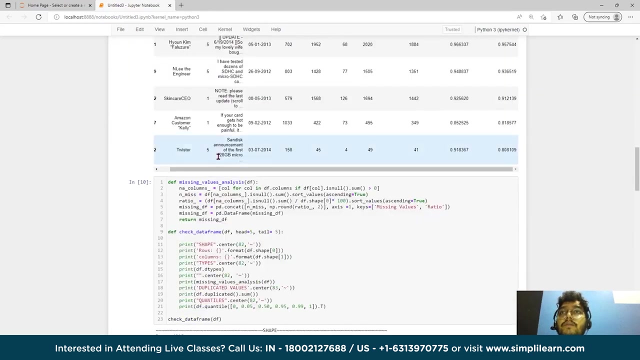 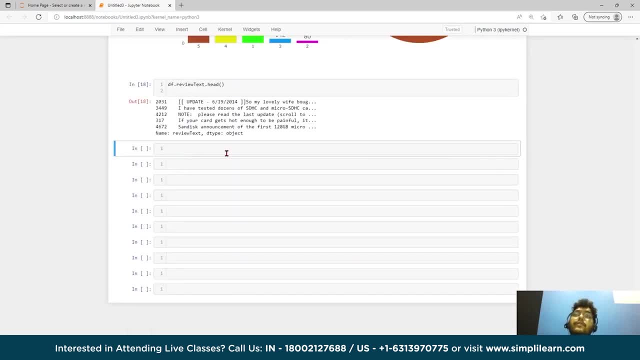 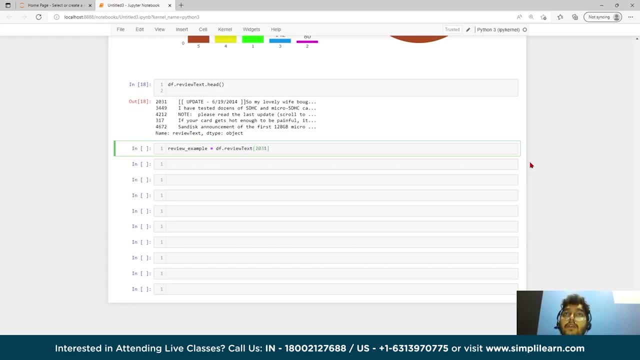 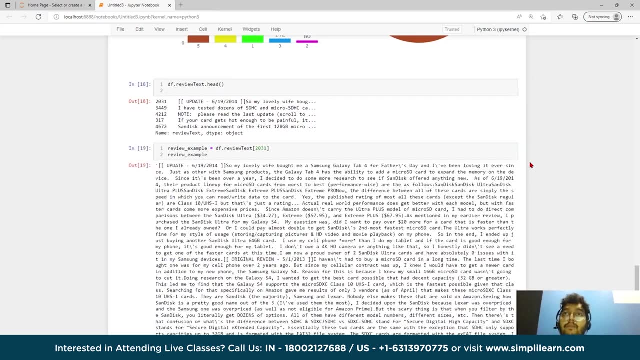 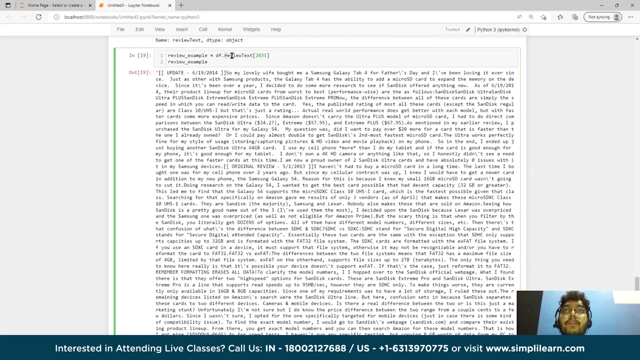 df, dot, df, dot, df, dot. okay, so review underscore example. so this is like at 2031, there is one review text. okay, so in that the whole data is here, like like. so my lovely wife bought me a samsung galaxy tab for father. this, this, this, this, like to find the exact model number. this is a long 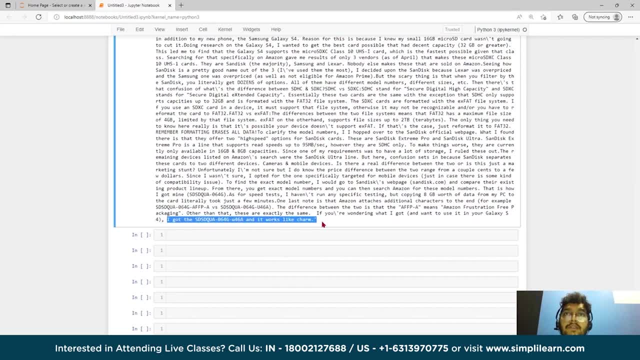 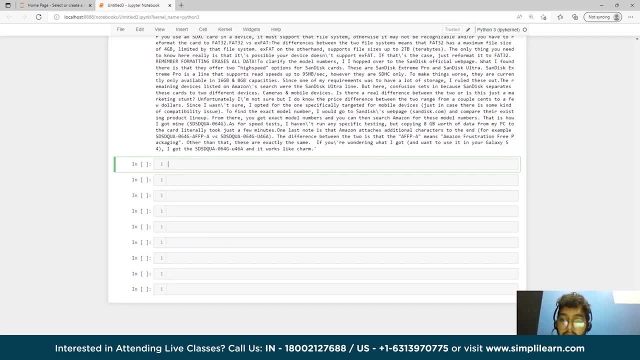 you know, comment: i got the this, this, this. it works like a charm, okay. so after seeing this data, what we're gonna do is like we will clean it from punctuation and numbers using regex. regex, what a regular expression. okay. so here i will write review underscore example. 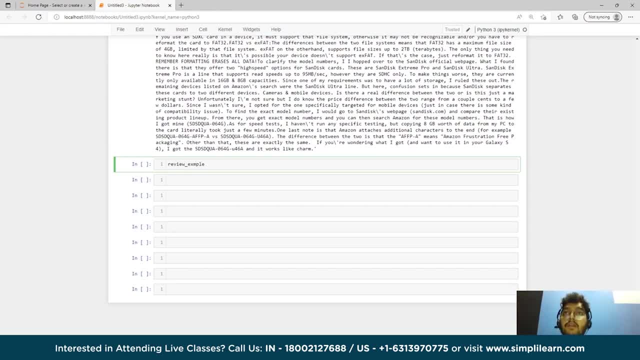 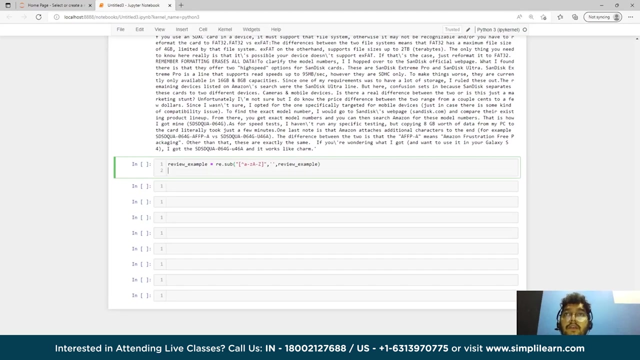 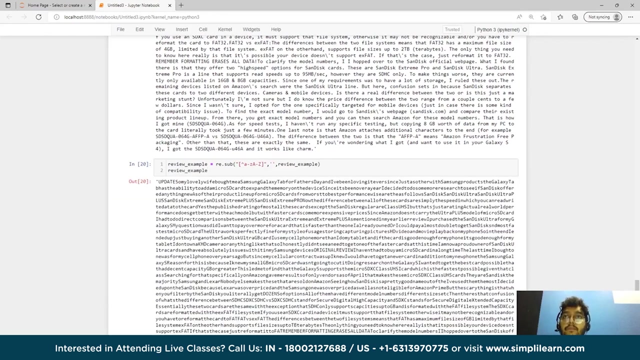 example: okay, okay, so, so, so. so it was to aree dot sub 号 and what i will do is okay, i will explain, don't worry, small late to capital in a to z: okay, comma, then space 05 06. So here we used re for regular expression. 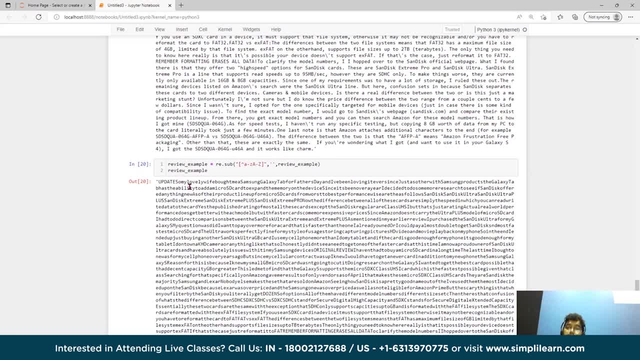 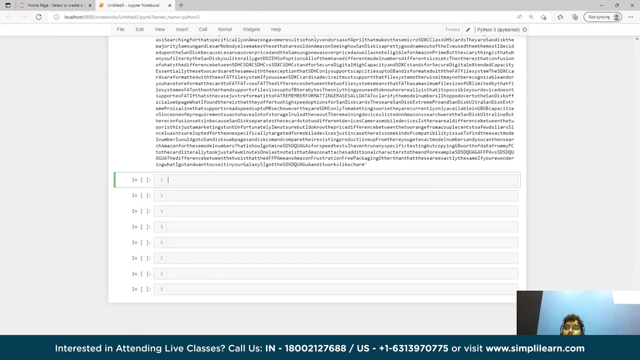 Okay, and so all the punctuation and numbers are removed from particular data. So let me check first This a to z, then a to z. okay, fine. So, like, all the punctuation and numbers are removed from particular data. I will now convert the text. 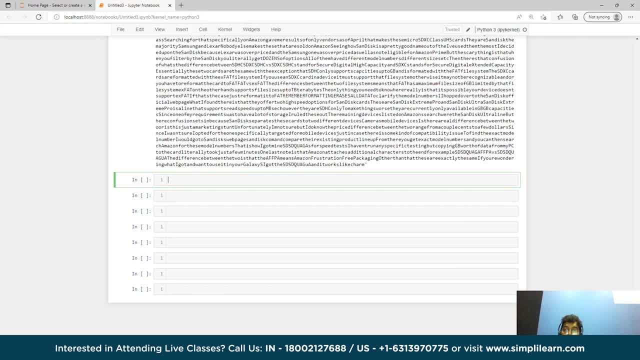 So To all lowercase, our machine learning algorithm recognize words that start with a capital letter as a different word and we will convert them to lowercase. So thus our machine learning algorithm will not perceive words that start with a capital letter as a different word. 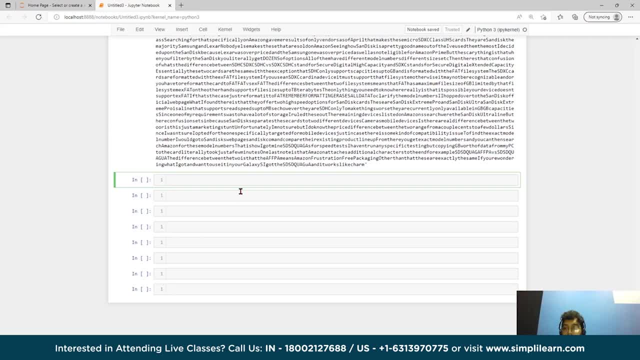 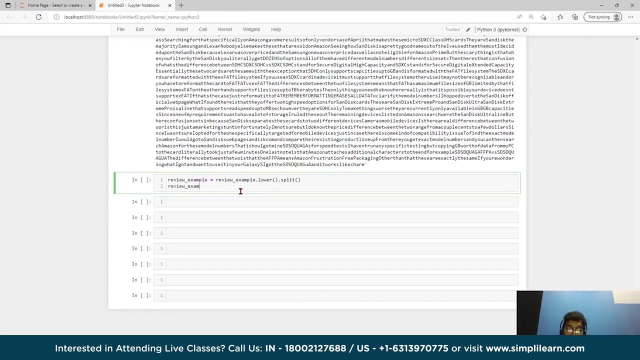 So what I will do is here I will write review. Scample- sample equals to review And sample lower. I will split, split, Okay, sample. So here you can see. we have converted all the words in the lowercase letter by using lower function. 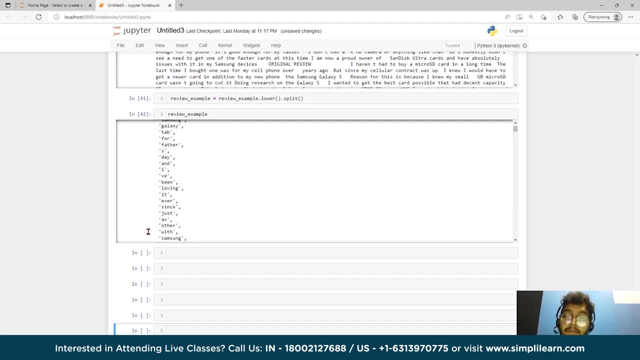 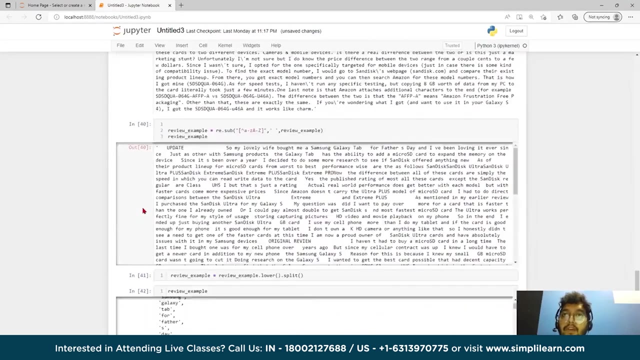 And why they are coming in new lines? Because we are using the lower function for the word Okay are splitting them using split function? okay, if you see, only did lowercase for single row, like we did for the like 2, 0, i guess 2, 0, 3, 1, okay, yeah, so let's make all rows same in lowercase. 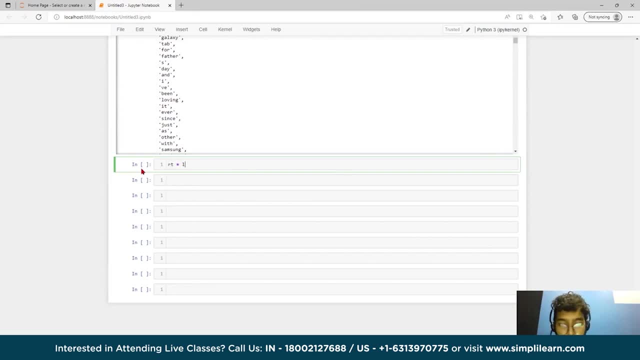 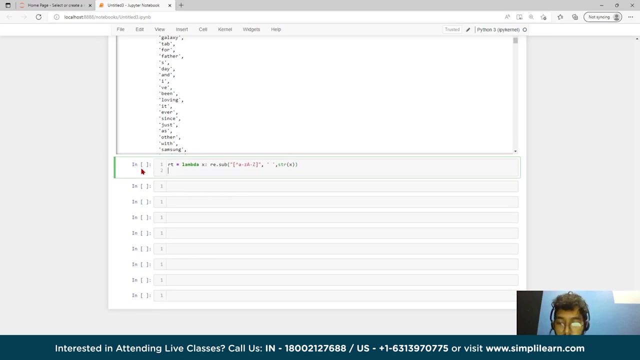 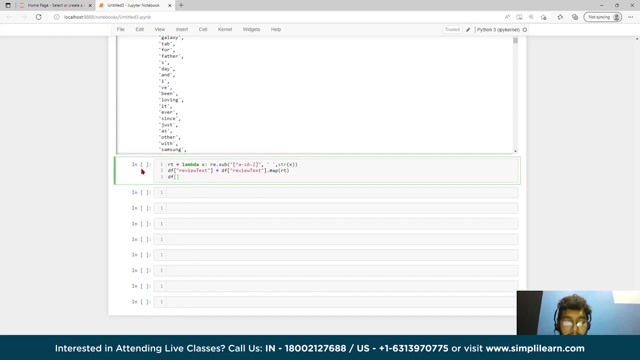 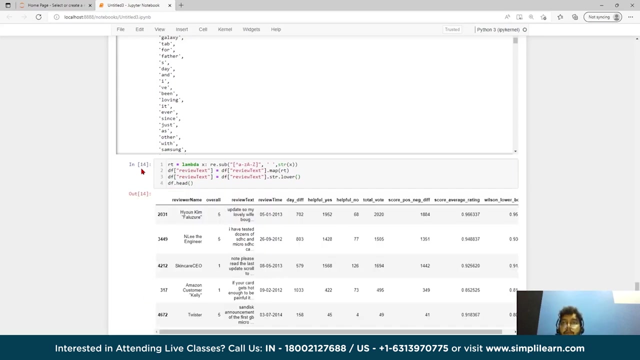 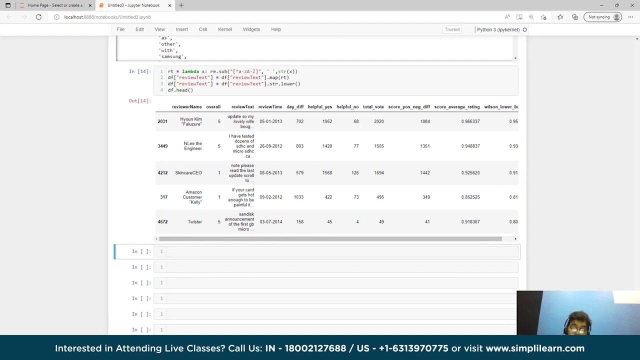 so i will write here: rt equals to lambda, x, sdr, er, x, df? u text: east capital text: df? u text df. df text text, df text text text text: x, x, x, x, x, x. see, all the data is in like lowercase, so i printed just top 10 rows and in like in reviews. 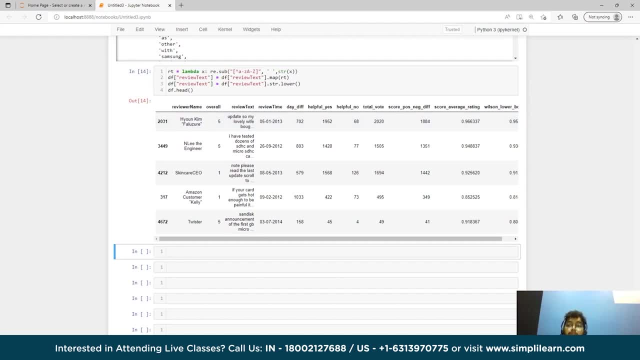 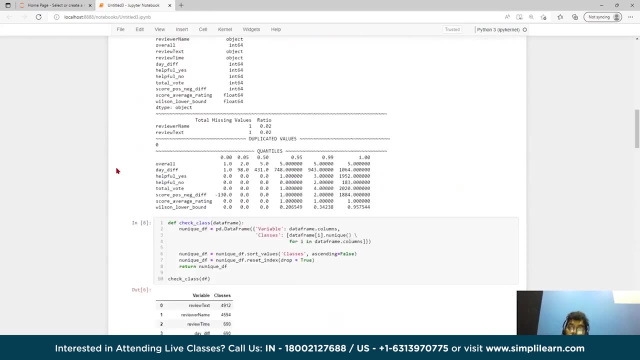 text column. all the are in the lowercase now, so i hope you guys understand till here. if you have any question or any query regarding any code or question till here like any code, just put as in comments. our team will shortly provide you the correct solution and if you 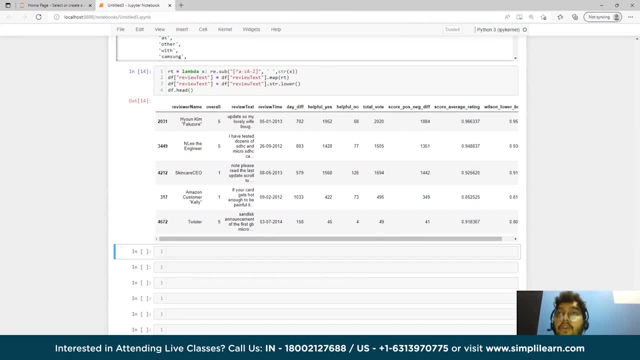 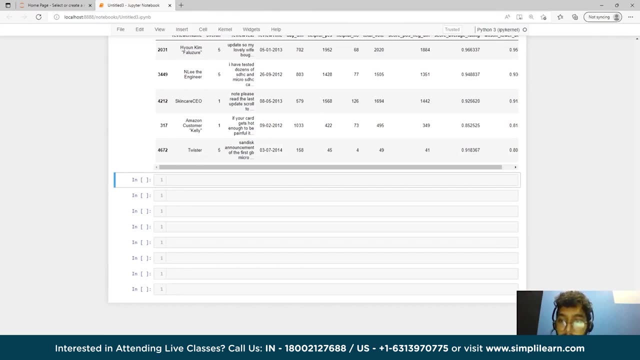 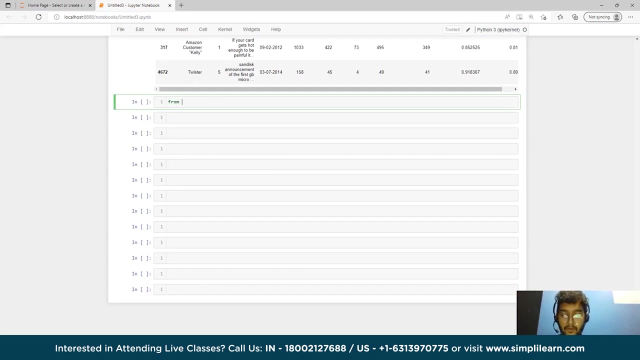 need this full code. you can comment down below. okay, so now the time is come to do sentiment analysis, because all the data is sorted. so what will i write here? let me put little bit up. yeah, so i will write from: yeah, from vader, sentiment dot vader. 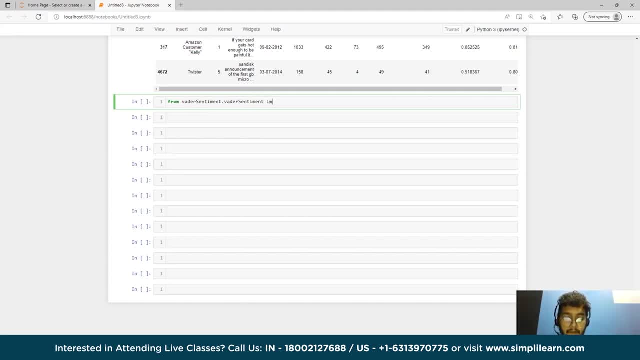 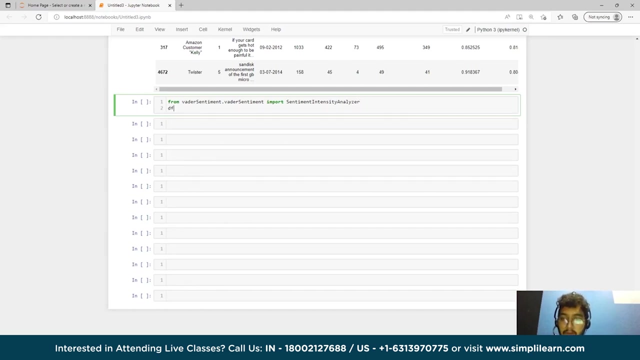 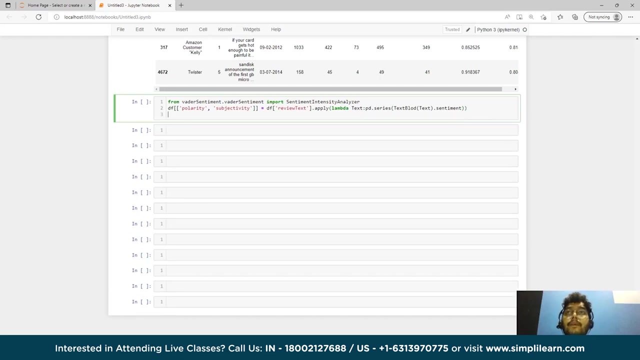 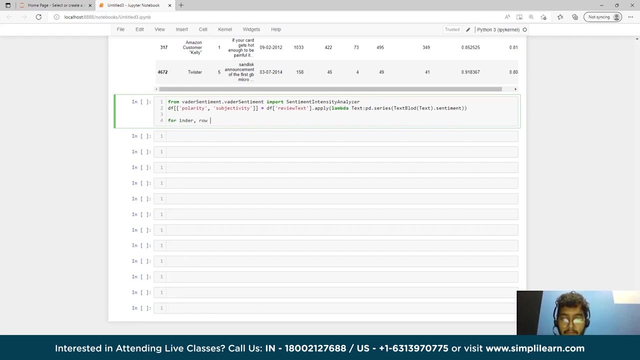 and report sentiment intensity analyzer. yeah, df, polarity subjectivity. subjectivity is to df. if you text not apply honda, next pd dot series. okay, here we'll write text blob. then again, text text dot like sentiment. let me run for loop for index comma row in df. let me run for loop for index comma row in df. 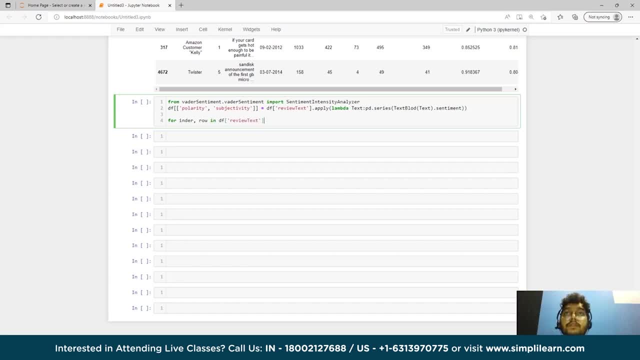 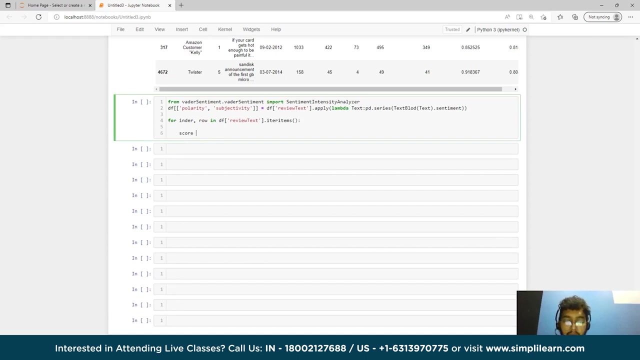 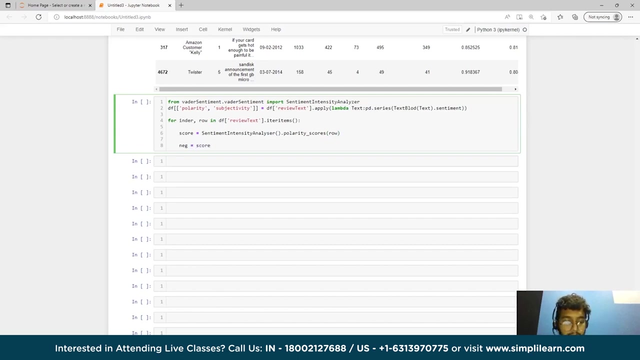 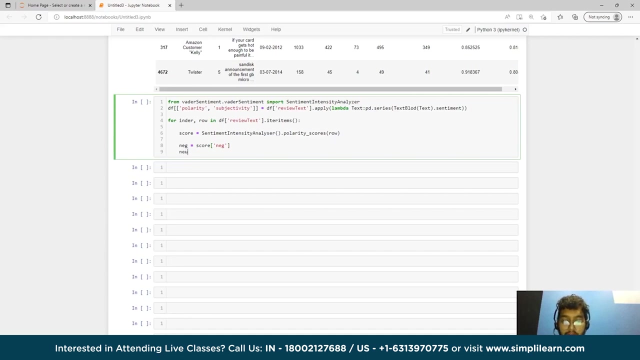 give you text, give you text, give you text. what item items? what item items go to go to sentiment intensity analyzer or polarity or polarity scores or polarity scores or polarity scores. row negative and score negative and score or neutral. i will write score or neutral. i will write score. 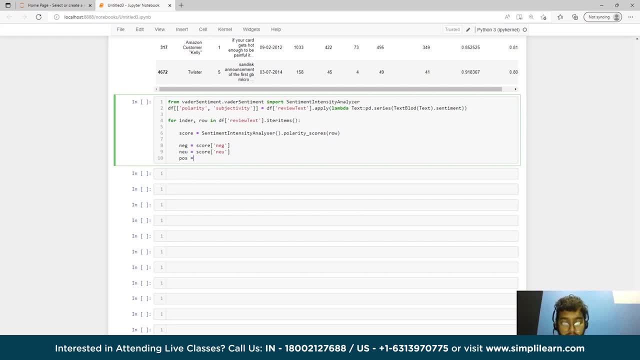 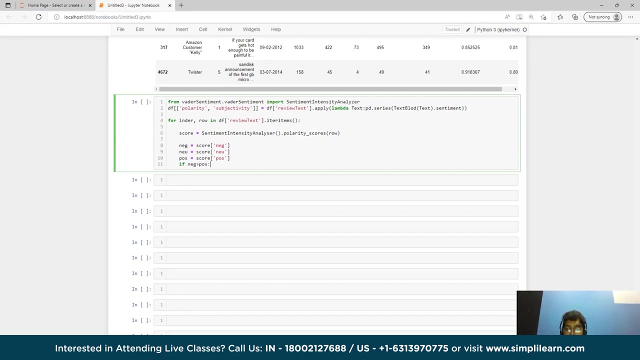 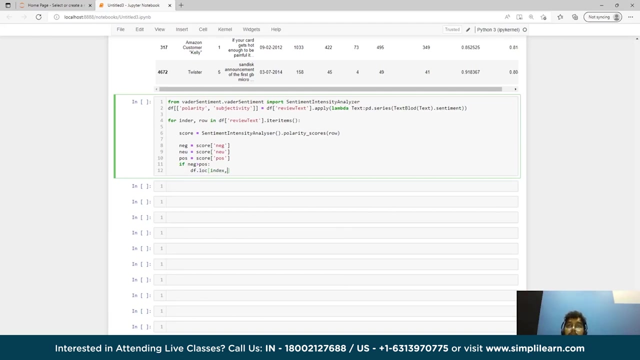 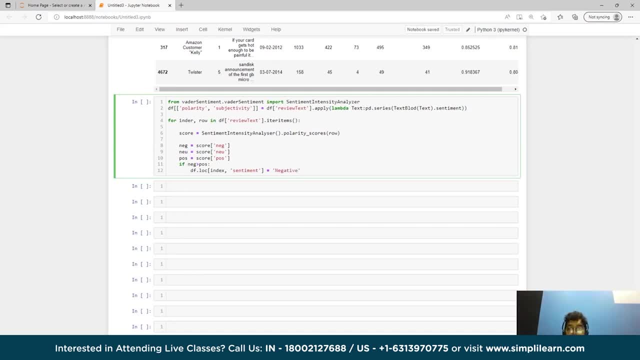 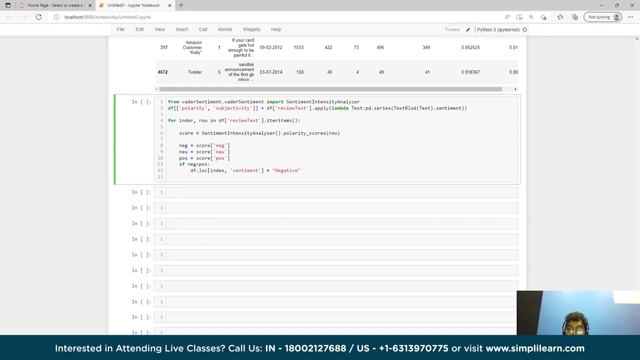 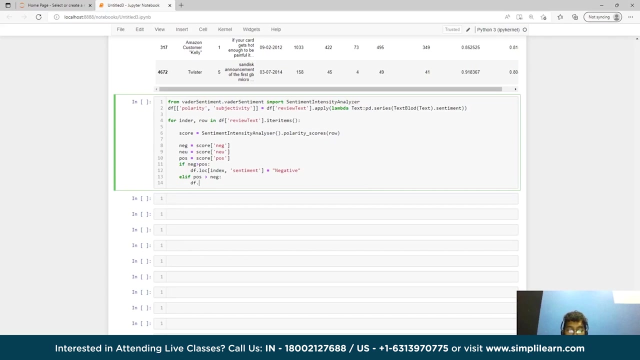 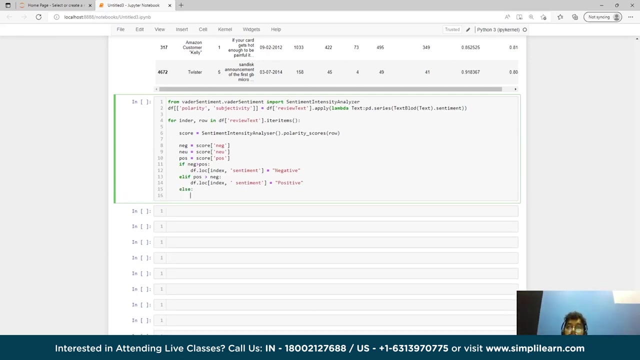 negative. positive is greater than negative, then in this case, df dot log index comma, sentiment was to positive P capital, else EF dot LLC X intimate neutral. yeah, so like this is for sentiment analysis and text blog, this thing like text blob, this blob, okay, X blob, will return polarity and subjectivity. 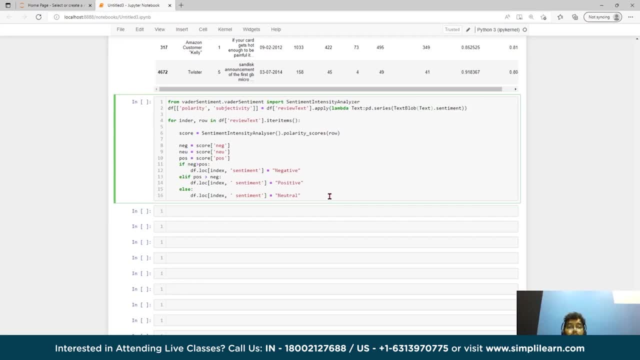 polarity indicates your mood, that is, whether it is positive or negative or neutral. it returns a value between 0 and 1. the closer to 1 the more positive, and the closer to 0 is more negative. okay, let me run this. it will take a little. 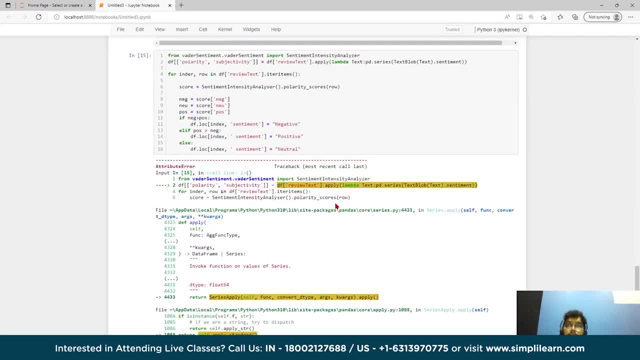 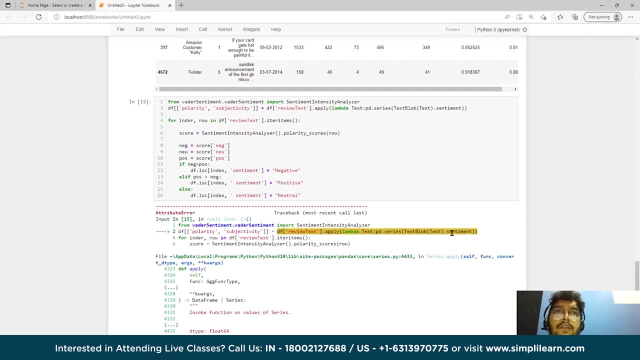 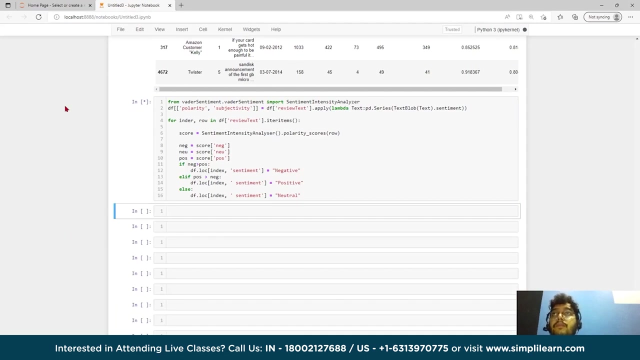 bit time because the sentiment: okay, it is getting error. like module panda has no attribute series. okay, which one X sentiment: okay here. what is the thing? s is, captain, let me run now. it is executing like fade for a while wait. so it will take time to run because, like, because of this. 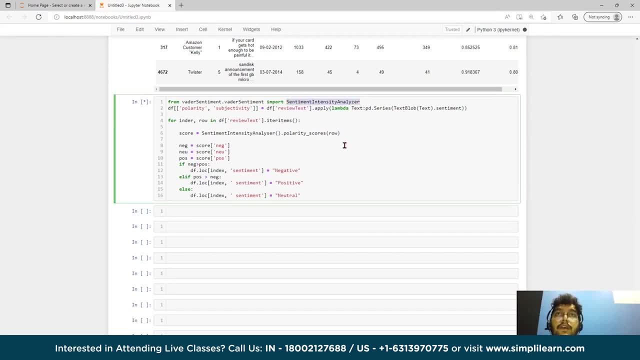 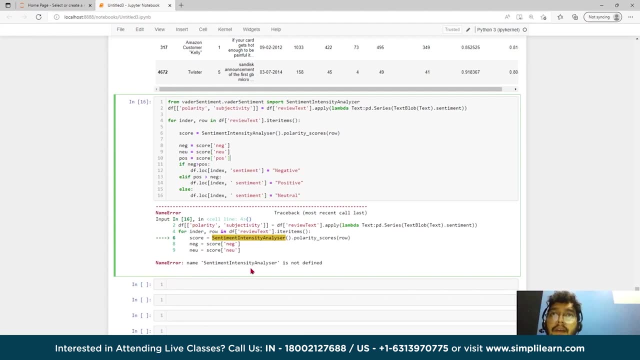 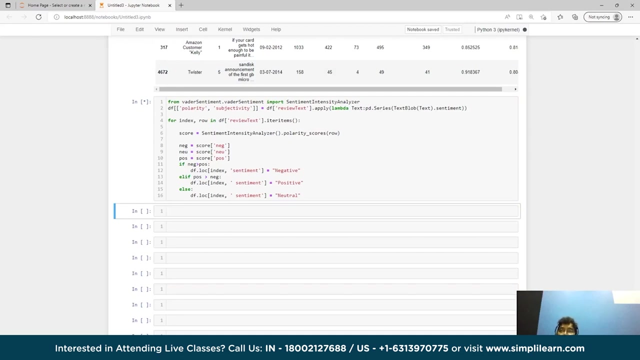 sentiment intensity analyzer. it takes times, can sentiment intensity analyzer. I don't see what it needs right now, so that's why I created the in the. I have added okay, spelling mistake again: Y index. index is not defined text. it will run, i guess, because everything seems good, negative, positive and this else. 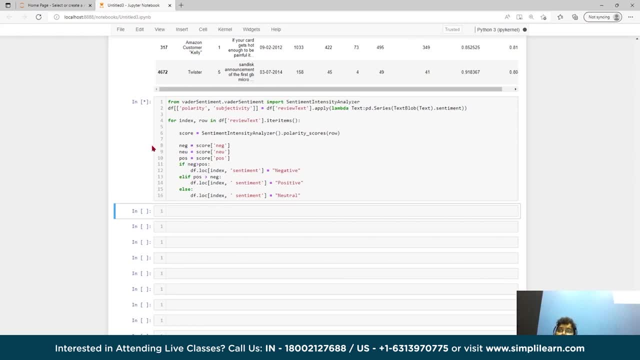 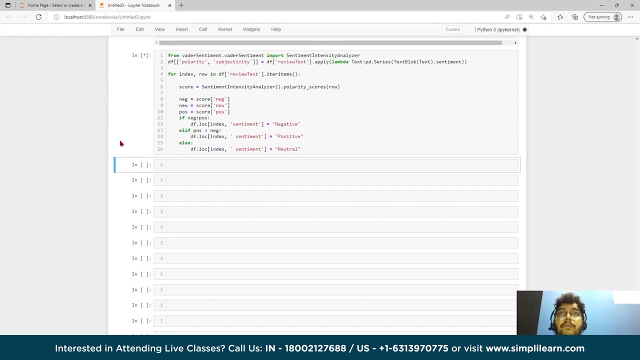 loading. so i have to wait like for like two minutes more. i guess loading guys, i take time. sentiment intensity analyzer: you, you. So let me tell you again: sentiment analysis: like this text blob will return polarity and subjectivity. so polarity indicates your mood, that is, whether it is positive, it is negative. 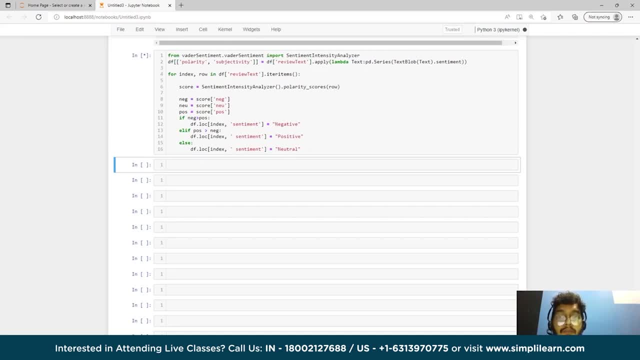 or it is. it will be neutral. it returns a value between zero and one. the closer to one, the more positive. the closer to zero, more negative. okay, I guess it's still running, so it will take time, so let me write code for that 20 interpretation. I repeat: moving forward, let's. 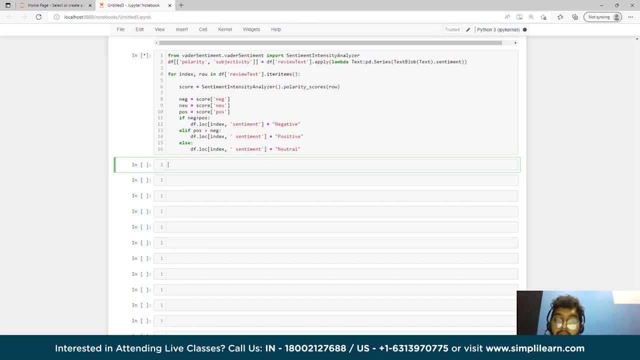 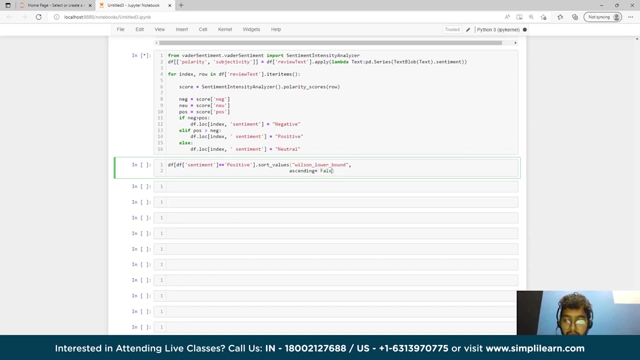 identify the 20 interpretation. now we can include the positive, negative and neutral status of the command. okay then, df, df. sentiment, which equals to positive thought. lose lower ending equals to false dot head. it's five. if I will run, it may give errors to me, because it's still running. 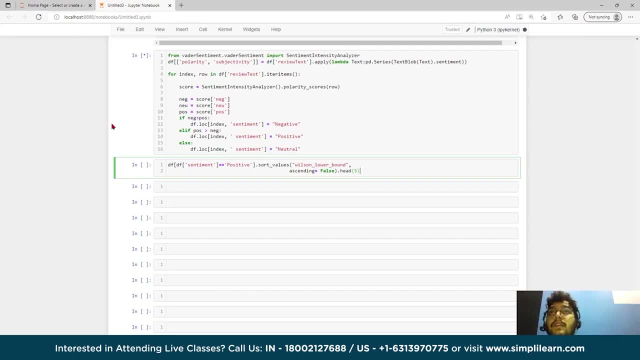 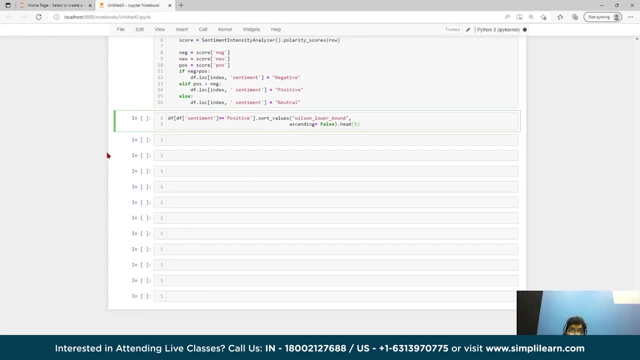 still running here, it's still loading, so so, so, so, so, so, so we will do it as well. so let let me write code for that unbalanced data problem, so like we will. So let let let me write code for that unbalanced data problem, so like we will. 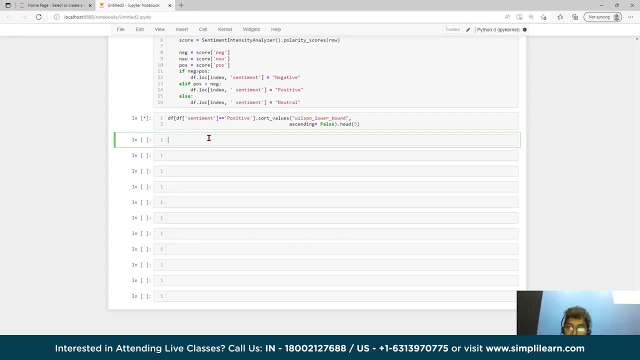 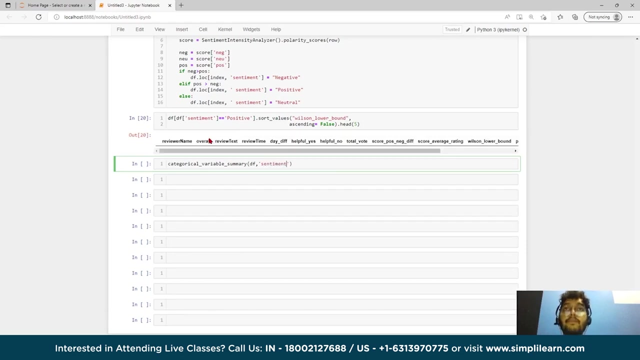 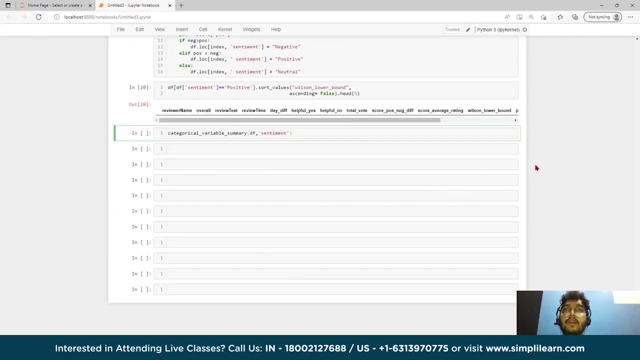 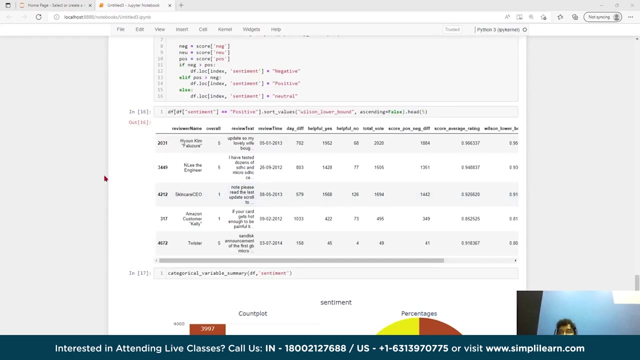 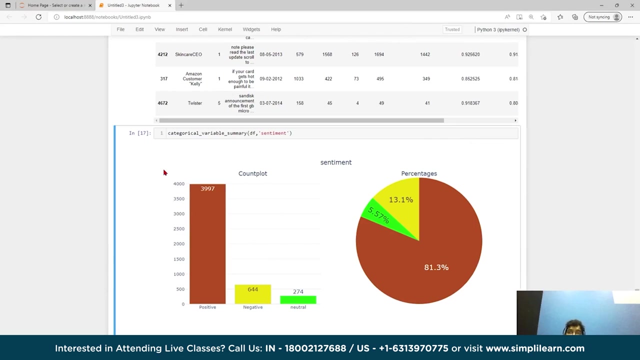 categorize that data into positive, negative and neutral. okay, so categorical, It came like this. because of this wait, I will tell you. Yeah, so here you can see the pie chart distributed in negative, positive and neutral emotions. Okay, or you can say ratings. and here you can see the bar chart also. 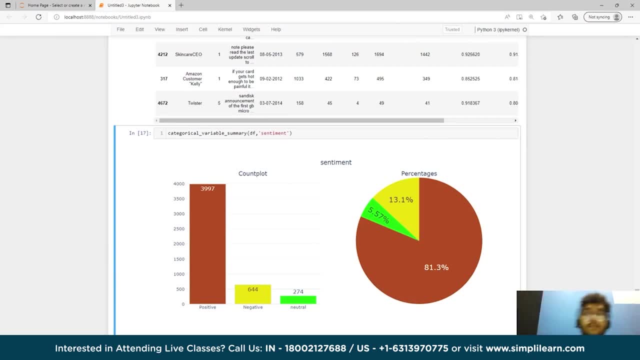 so, and You can see the percentage distributed in each like in positive, negative and neutral one. So I hope you guys must understood the concept of sentiment analysis, how we can implement it using python, If you're looking for a course that covers everything from the fundamentals to advanced techniques. 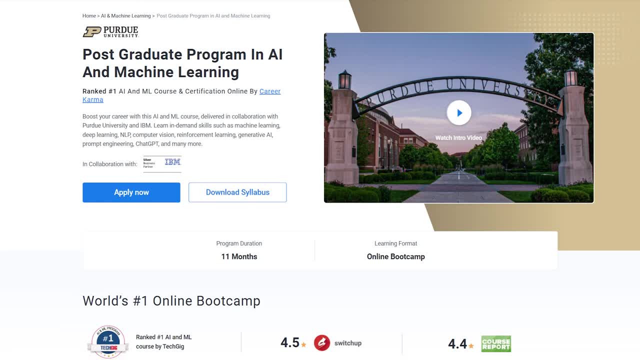 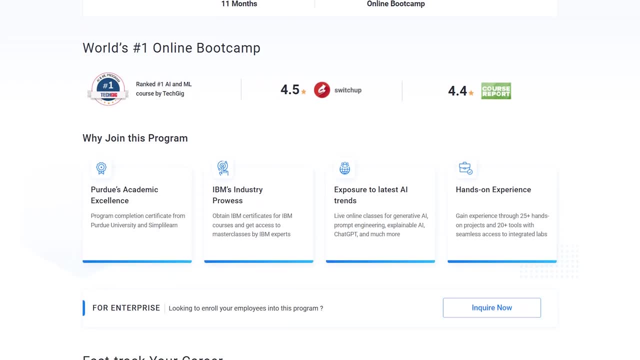 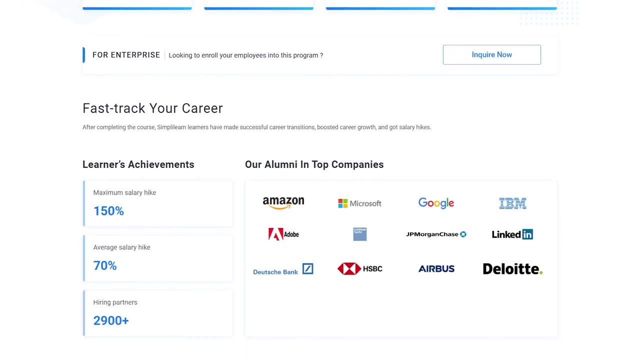 Then accelerate your career in AI and machine learning with a comprehensive postgraduate program in AI and machine learning. Boost your career with this AI and ML course, delivered in collaboration with the Purdue University and IBM. Learn in-demand skills such as machine learning, deep learning, NLP, computer vision. 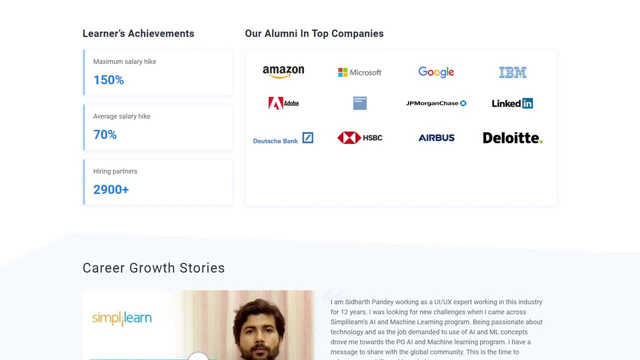 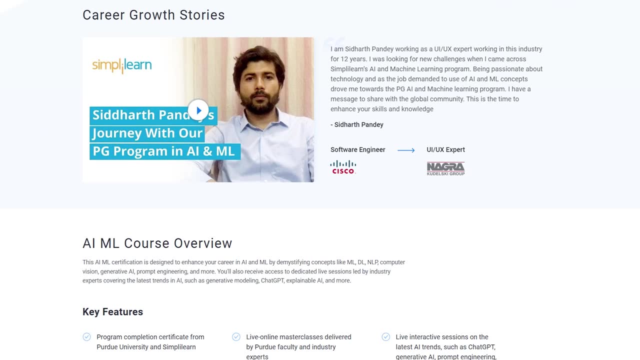 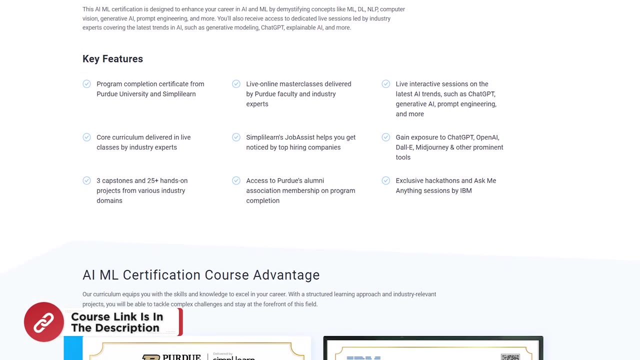 reinforcement learning, generative AI, prompt engineering, chat, GPT and many more. You'll receive a prestigious certificate and- ask me anything- sessions by IBM with five capstones in different domains, using real data sets. You will gain practical experience. masterclasses by Purdue faculty and IBM experts ensure top-notch education. 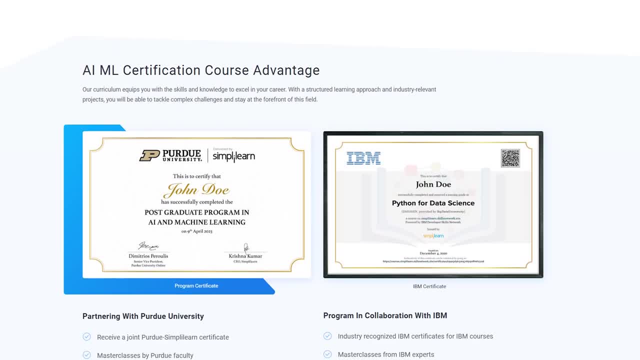 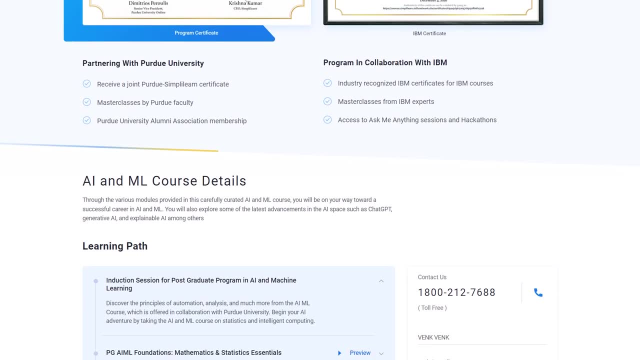 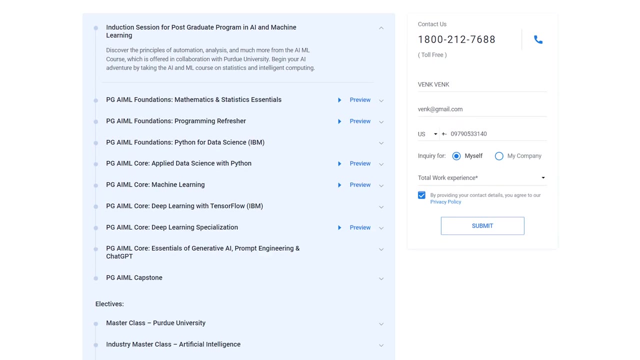 Simply learns job assist. help you get noticed by leading companies. this program covers statistics, Python, supervised and unsupervised learning and MLP, neural networks, computer vision, G and scarif, stanza flow and many more such skills. admission to this postgraduate program in AI and machine learning requires a bachelor's degree with an average of 50 percent or higher marks. 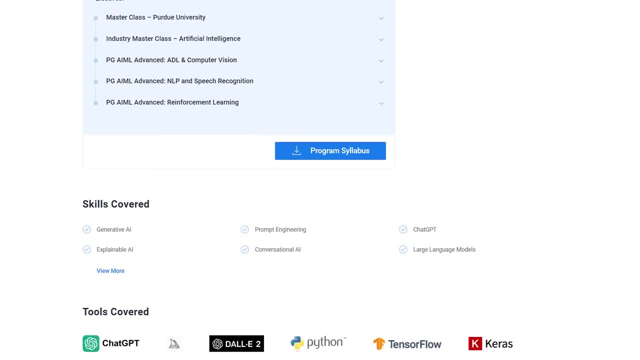 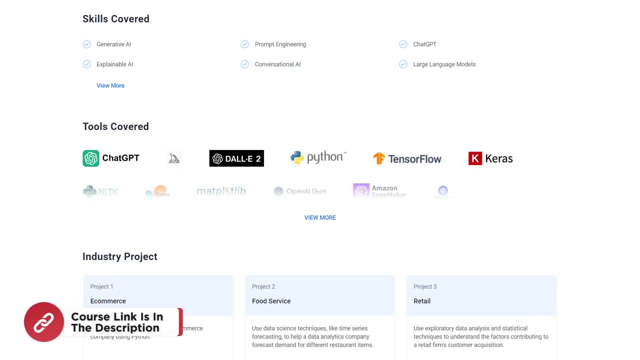 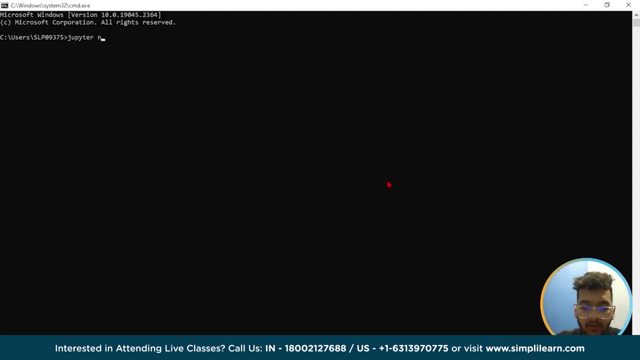 along with the basic understanding of programming concepts and mathematics, and Candidates with two plus years of work experience are preferred to enroll in this school. So enroll now and unlock exciting AI and machine learning opportunities. The link is mentioned in the description box below Jupiter Notebook and press enter. 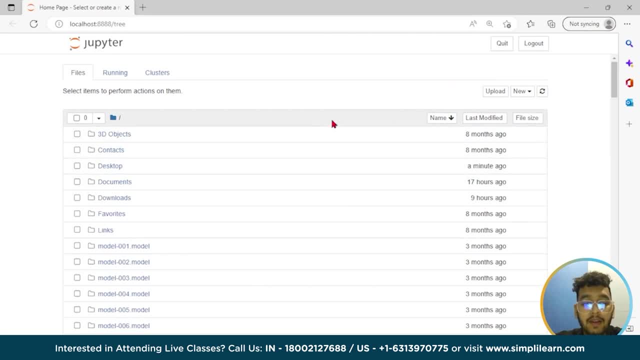 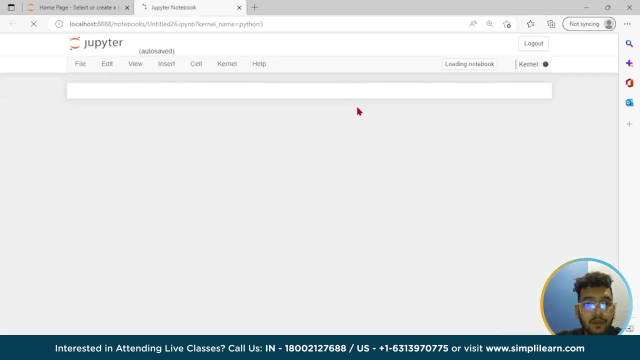 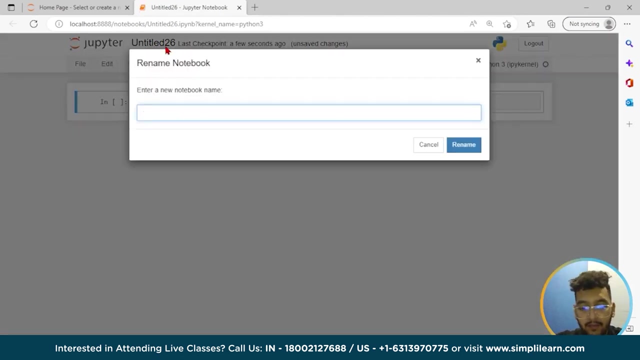 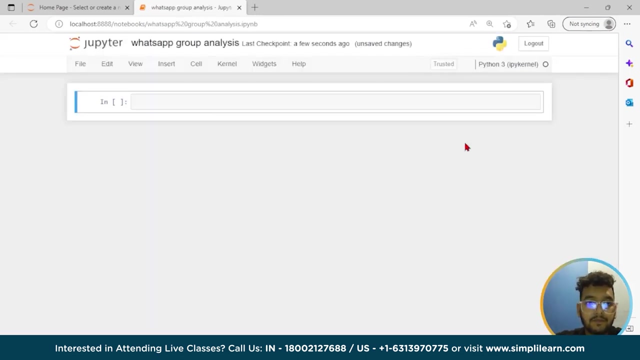 This is the landing page of Jupiter notebook and it select open new Python file. here we will go new button file. This is how the Python gonna look likes: Jupiter Python gonna look like. so here was. we Will change the name What's up group And yes, Here first we will import some major libraries. 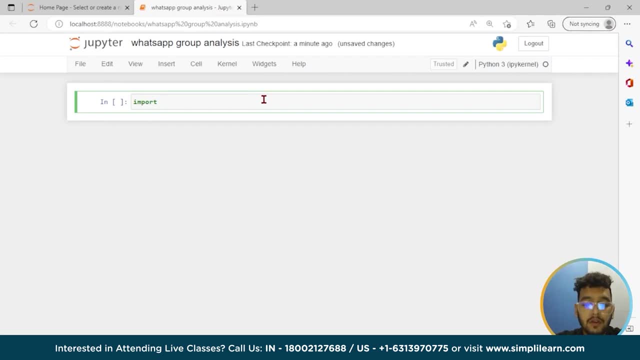 First we will import, import re regular expression and then import Dex. I will explain one by one. so very import One does Ed Report numpy and and P, and the fifth one is import Or Or express As PX. Okay then, from collection import Pounder And import My plot live dot by plot. 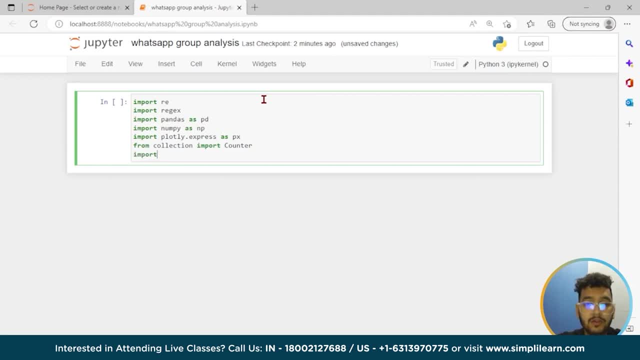 And import My plot live dot by plot. And import My plot live dot by plot, My plot, live dot by plot, My plot live dot by plot. lol At all. And okay, this is for the graph and from os import log field And the next one is from PIL import. 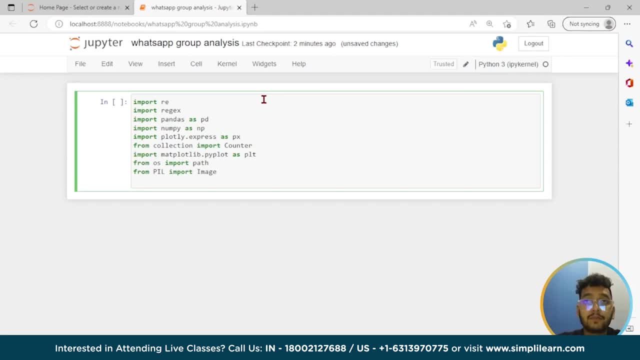 The next one is the maal, Then this is theавis. I am going to import The next major one: IMPORT DATE PACKET. This is the there supply type of key that we've did 아까 time and this one is the bottom word cloud. quote word cloud. 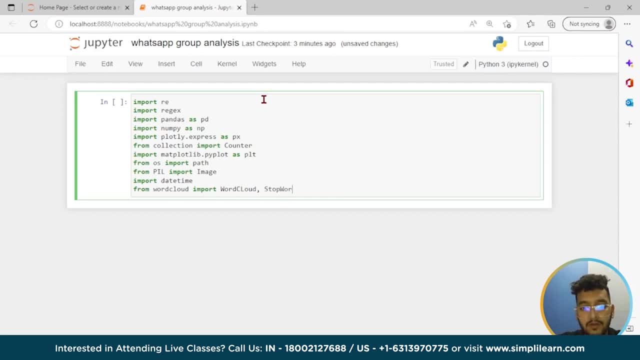 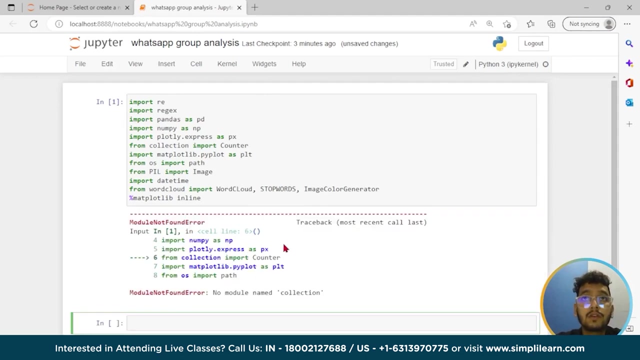 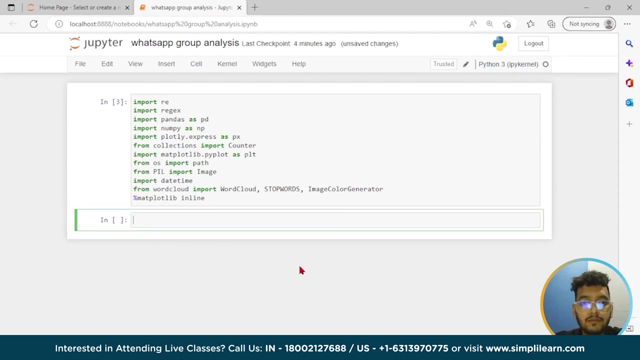 top words upwards and then image color editor. okay, then person matplotlib. then press enter. let's see selection. okay, should be collections from word cloud. import word cloud, stop words. image color generator. yeah, so cannot import name but cloud. okay, sorry, it should be small. so okay, so rest is fine. so numpy is a python library. 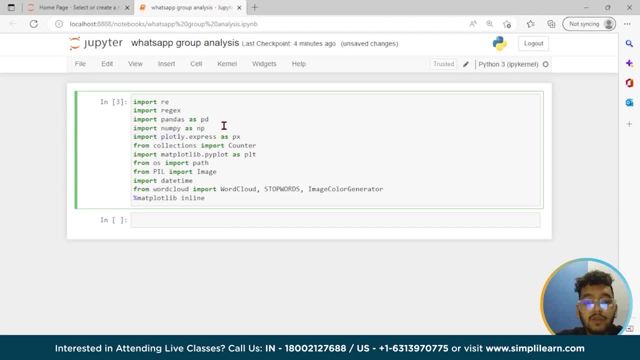 used for this one, numpy, with the python library used for working with arrays. it also has the functions for working in the domain of lelian algebra and matrices. it is an open source project and you can use it freely. numpy stand for numerical python and the panda. panda is a software library written for the python. 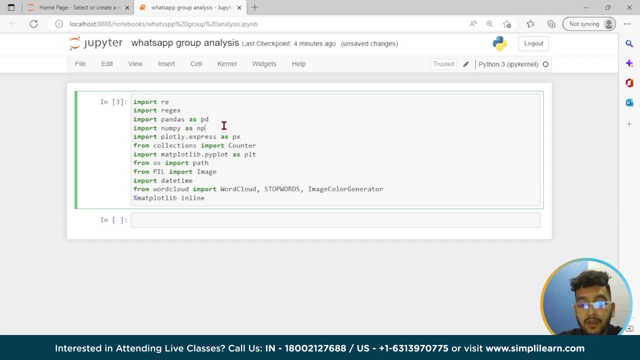 programming language for data manipulation and analysis. in particular, it offers data structure and operations for manipulating numerical tables and time series. this matplotlib, by plot for python and its numerical extension numpy matplotlib, is a cross-platform data visualization and graphical charting package. as a result, it represents a strong open source substitute. 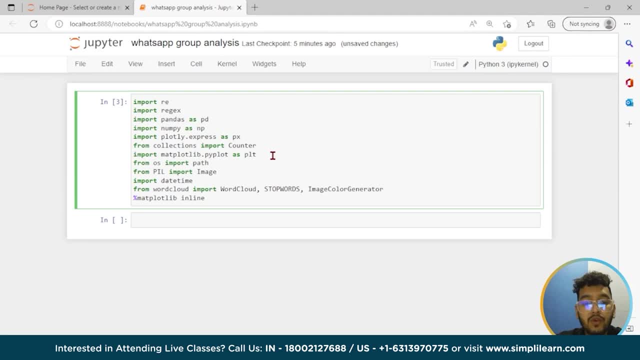 for matplotlib. the application programming interface for matplotlib. allow programmers to incorporate graphs into giu application. okay, then this re regular expression. so a regular expression: specify a set of string that matches it. the function in this module let you check if a particular string matches a given regular expression or not. or you can say if a given 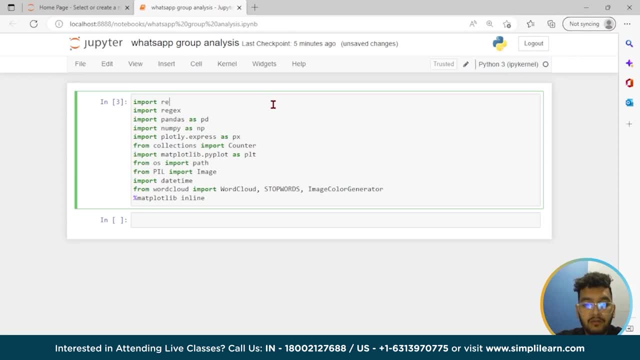 regular expression matches a particular string, which come down to the same thing. okay, then rejects a regex. or regular expression is a sequence of character that forms a search platform, okay, or you can say search pattern, that can be used to check if a string contains a specified search pattern or not. and this px, okay, totally express this plotly express module usually. 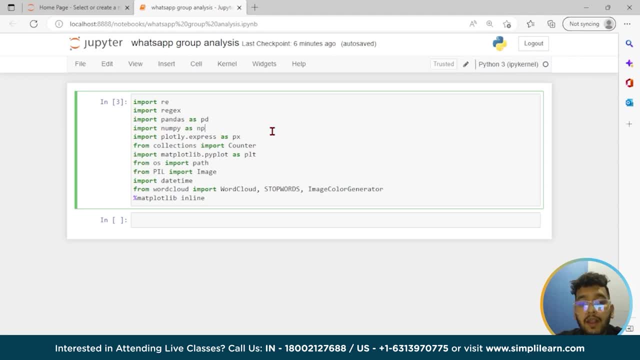 imported as px. contains functions that can create entire figure at once- okay- and is refers to as a distance that the string will activate or delete for everyegtucker, and the spacing class can be aligned in and, if autonomous, so the search-track will activate during that time. 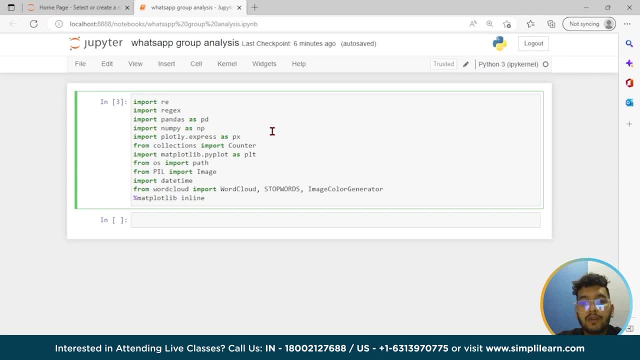 and the specifying property cannot beету or Prom Essection file. as it is, GamesX is a blasted folder. so when schoolsprepar заг금으로 is built-in part of the daily library and it is recommended starting point for creating the most common figures, 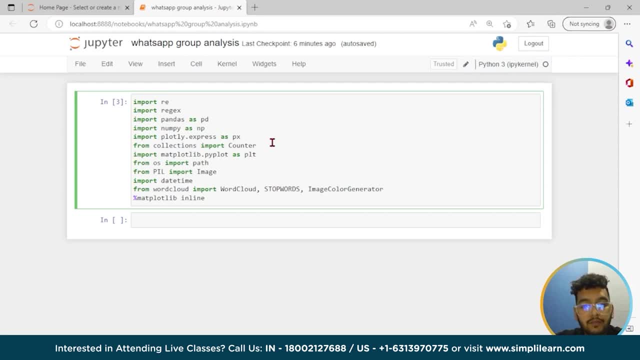 okay, then there is one more, this counter library. so the counter is a dict subclass for counting integer value including zero or negative counts. okay, then there is one more, this word cloud. okay, this is the kind of major one to visualize, so not major one, but it looks good at the end. 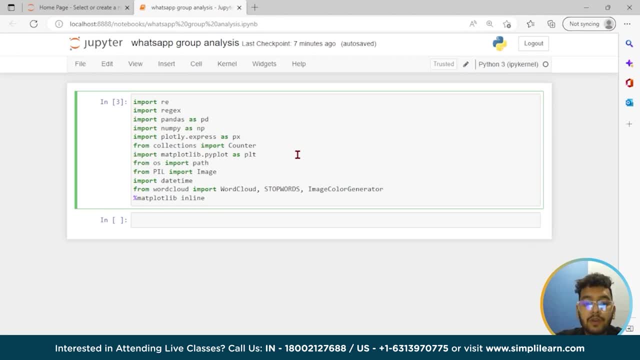 you will see. so word cloud is a data visualization technique used for representing text data, in the which size of each word indicate its frequency or importance. significant textual data points can be highlighted using word cloud. word clouds are widely used for analyzing data from social network websites. okay then, stop words. a stop word is a commonly used word, such as. 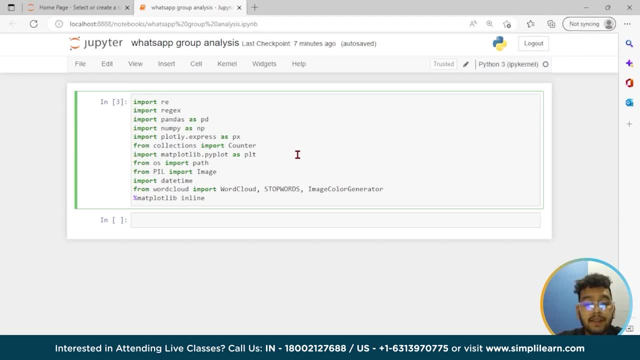 the uh and in, so that a search engine has been programmed to ignore both indexing entries for searching and when retrieving them as a result in a search query. okay, so let's proceed further and create the various function for the author, for the date and time for the get data time for the. 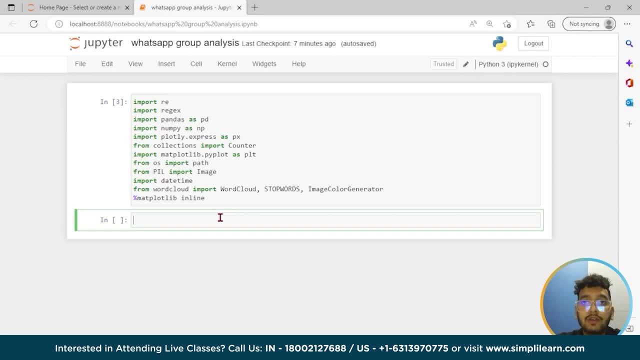 you know data point for the android and for the ios, like things like that. okay, so here i will add def arts with it and i will write here pattern. i will start with data and time. okay, i will write here pattern. i will write here pattern. okay, okay. 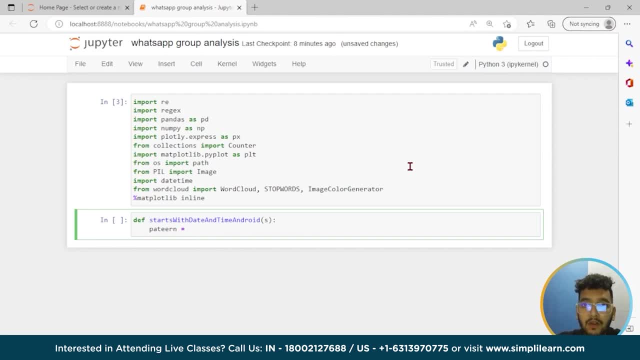 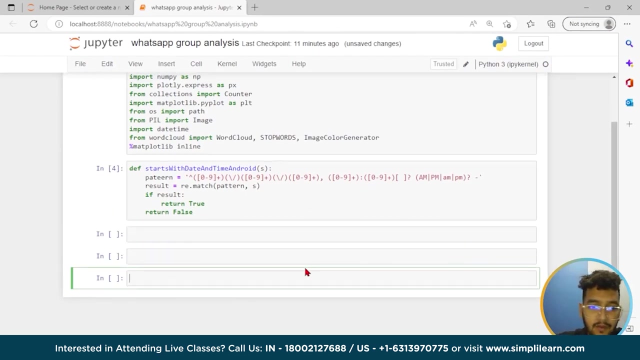 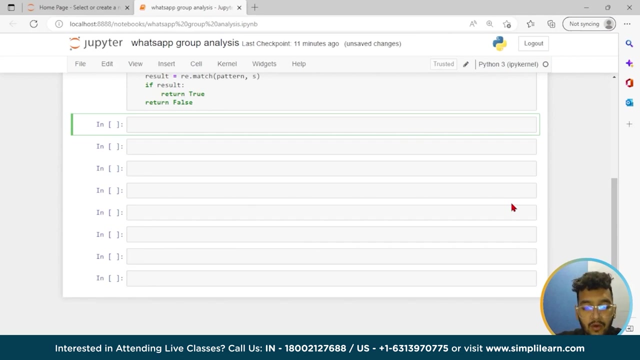 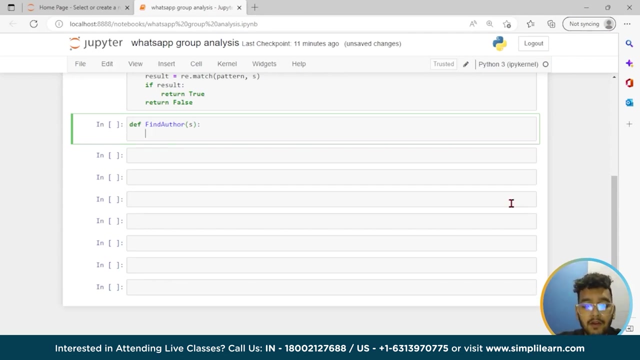 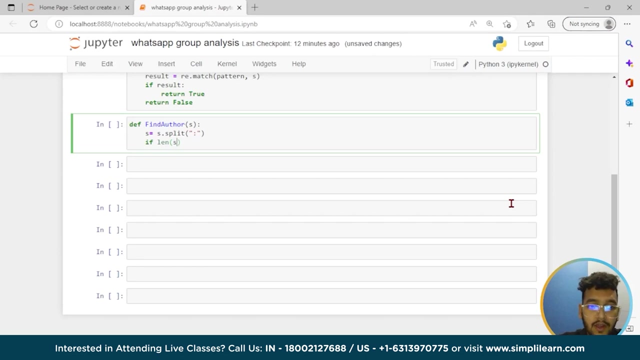 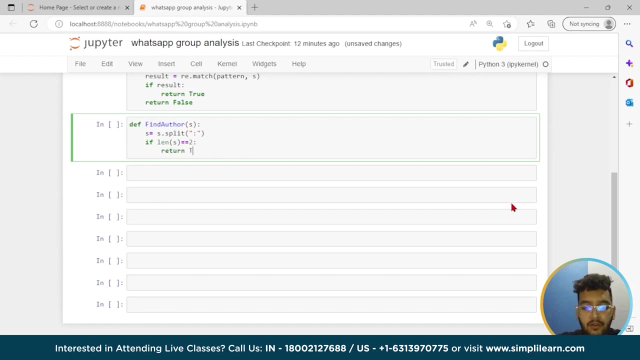 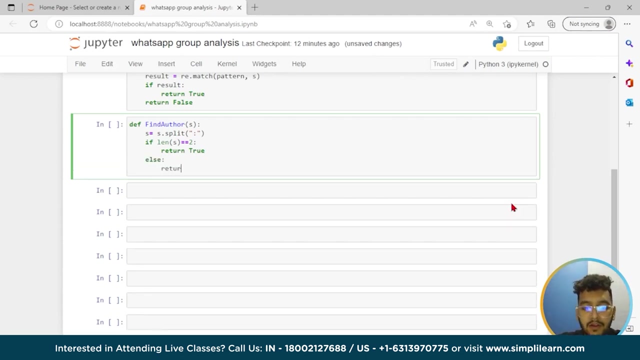 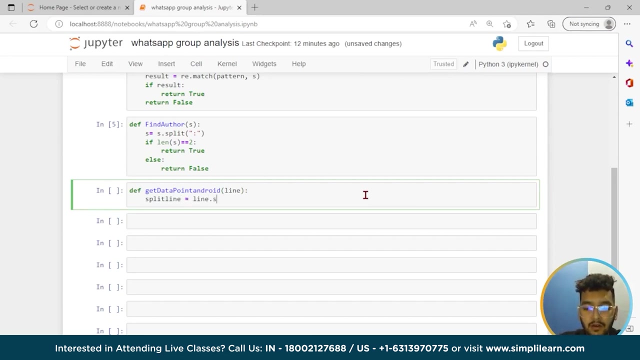 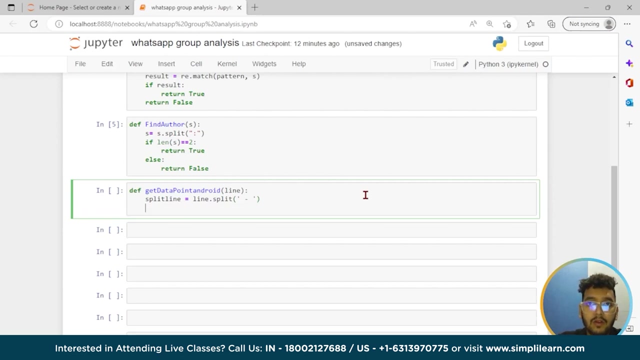 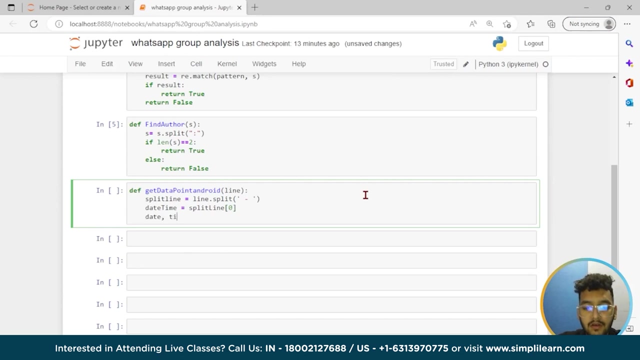 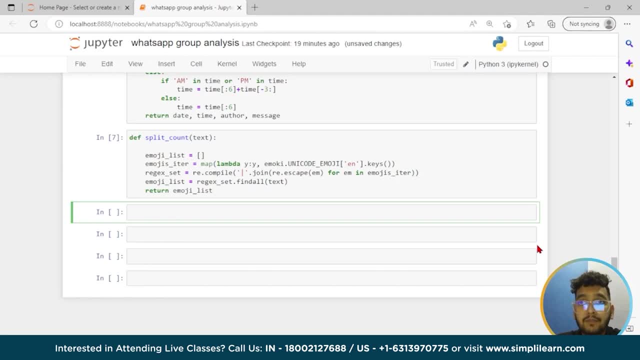 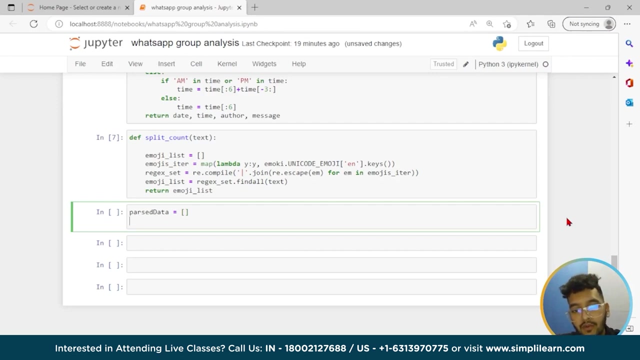 so it can be used for the Pandas DataFrame. We will create a separate every column for the date, time, author and messages. okay, so the major thing is: okay, let's import data first, then I will tell you. okay. so this is the list to keep a track of data it so it can be used for the 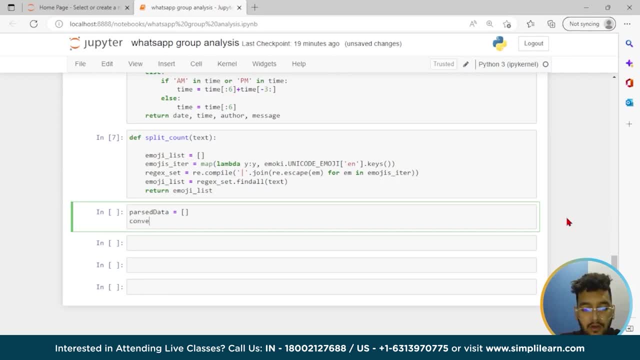 data frame on a database. okay, so let's converse conversation path. so my file name is whatsapp. that is captain it BIT and placed to rent in 22. this is my file, so how you can export your chat from your whatsapp group. okay, so this is the data. this is my personal data, so I can't give you. so how you can. 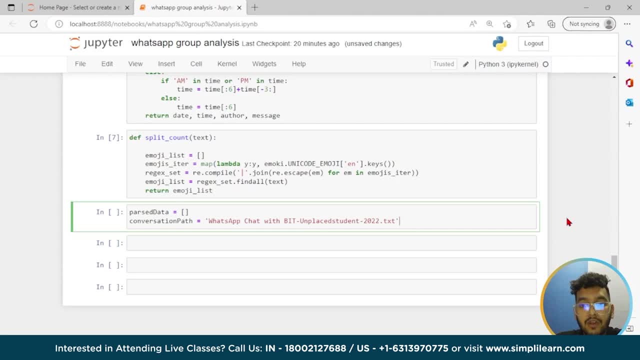 import your text, your chat. okay, so open any group. just click on the top right corner. okay, three dots. then you can go into mode and then you can explore chat including media and excluding media, your wish. okay, so you can download, you can send to the mail, you can upload in the drive. then you can. 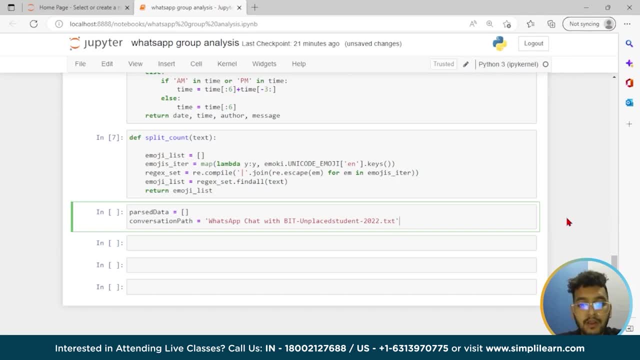 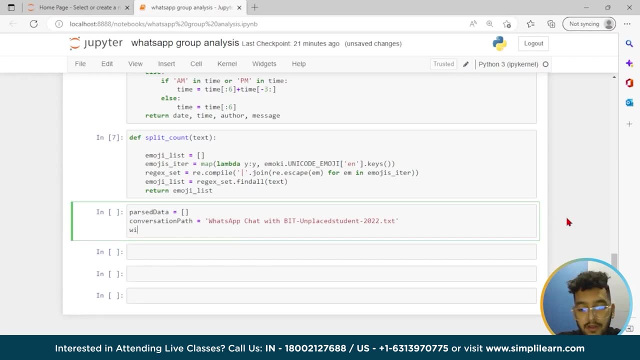 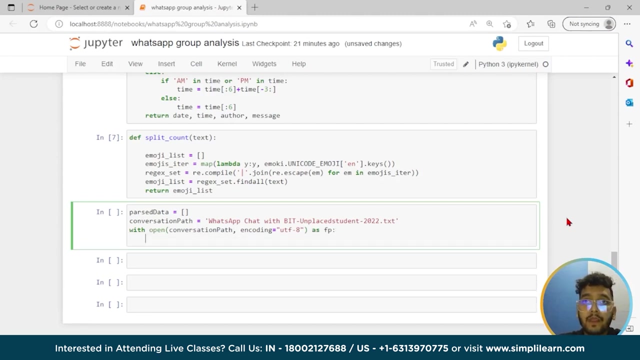 use in your machine learning project. okay, so I will write these, all these steps, in the description box below, so don't worry. going forward, let's do a quick test of my interface. now it's run, but I'm not going to show the statistics yet. okay, so we will talk about the data that we have on the website. so a minute is. 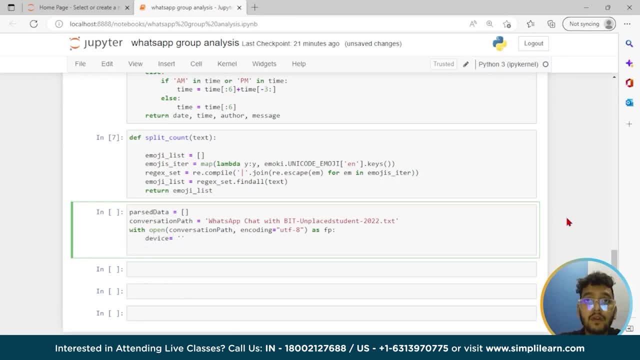 okay, so we will talk about the data that we have on the website. so I will talk about the data that we have on the website. so a minute is, and first is to fp dot read line. print first, if you, or else twice supposed to p dot read line. 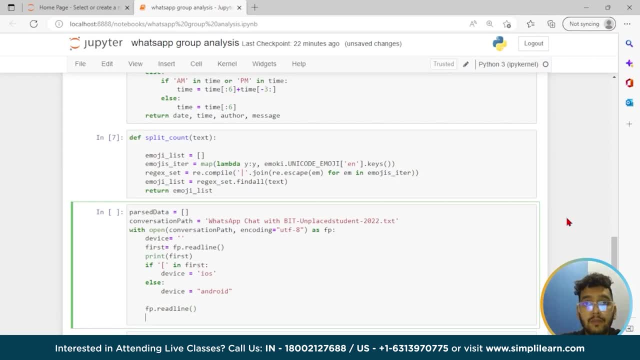 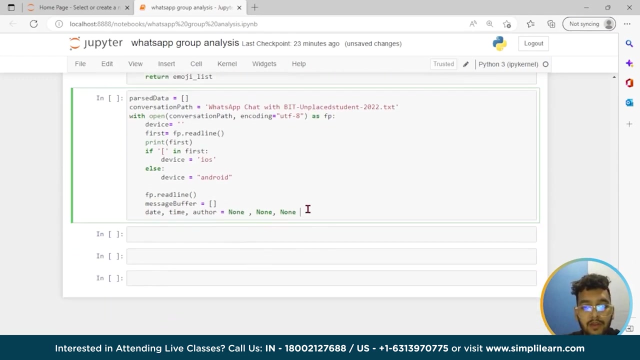 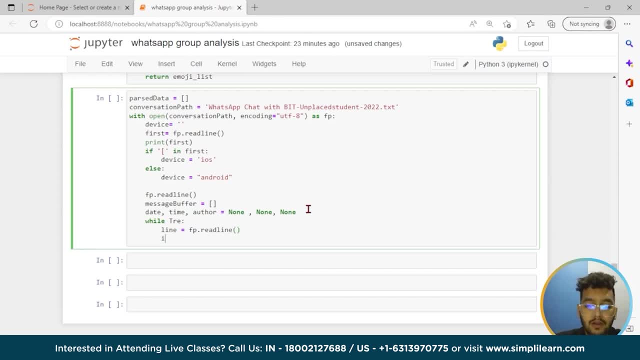 dot read line dot read line dot line line line devices devices devices ios ios ios ios ios now, now, now, now, now, correct, correct, I'm? I was fine, that would date. I'm, I was lying, so here I will asked: data dot it, you okay? so this is the long. 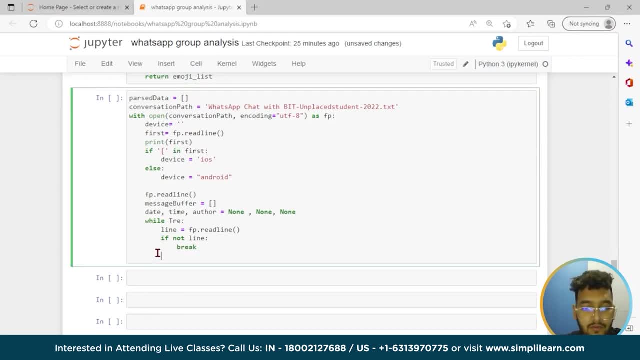 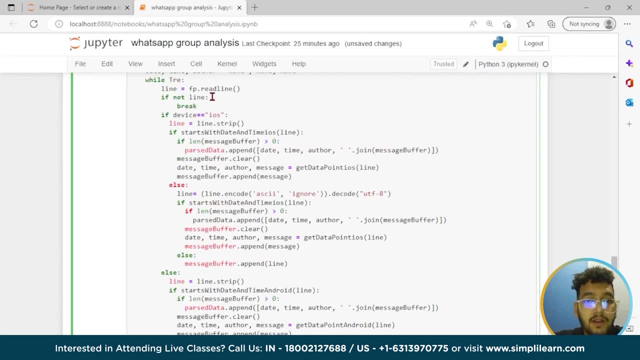 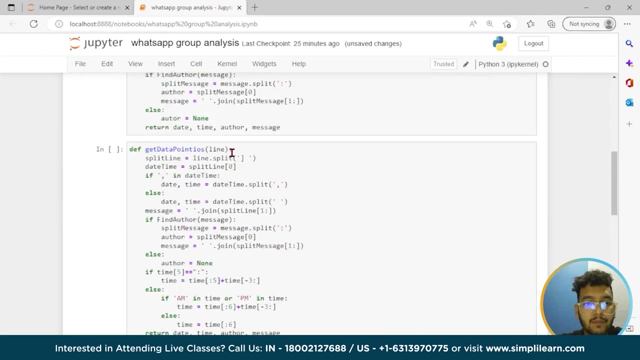 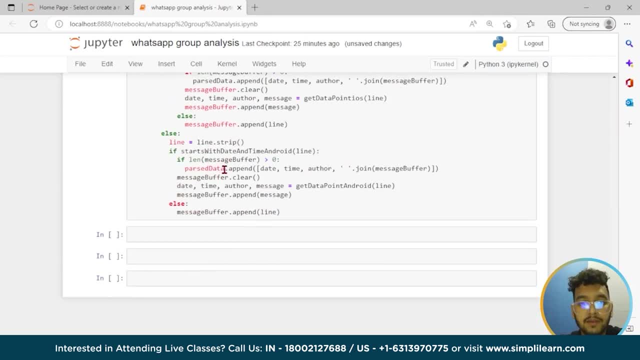 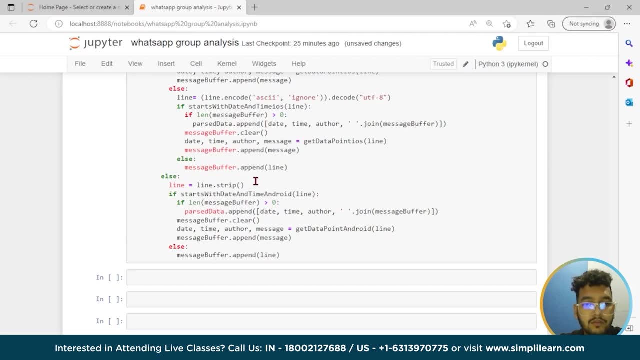 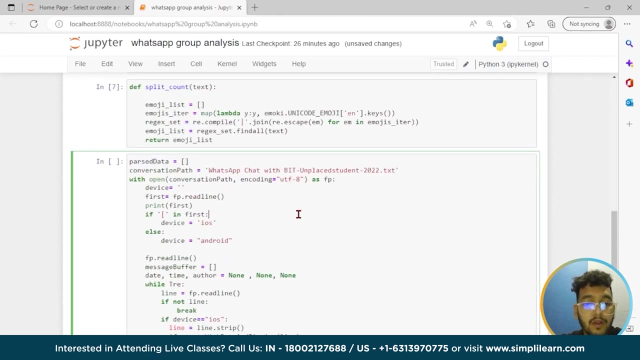 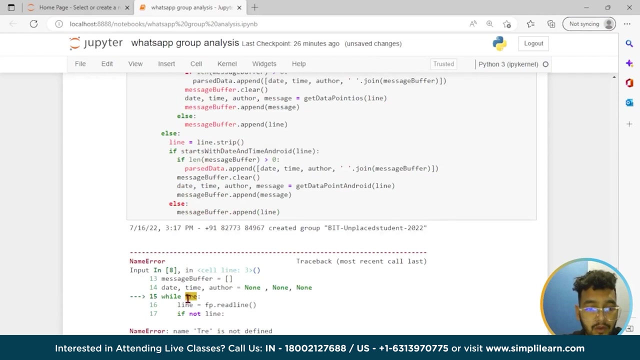 okay, it will capture the date, time, author and messages. okay, then at the end the message buffer will append: okay for the both. okay, this pass data is for the. we created for the data frame panda's data frame okay list, so let's go ahead and see. okay, while TRE. 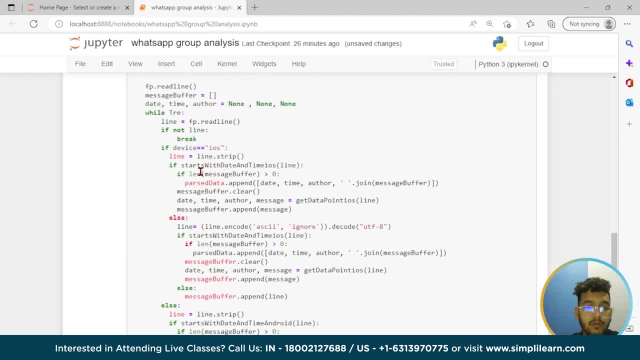 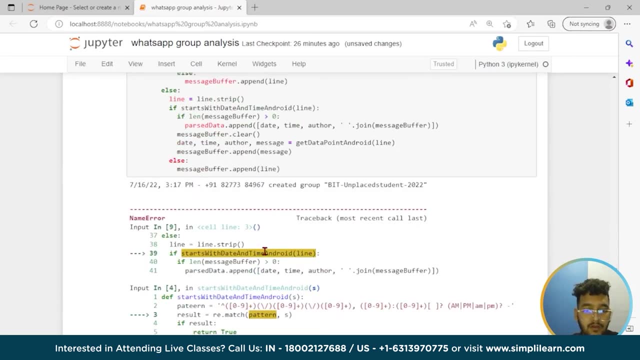 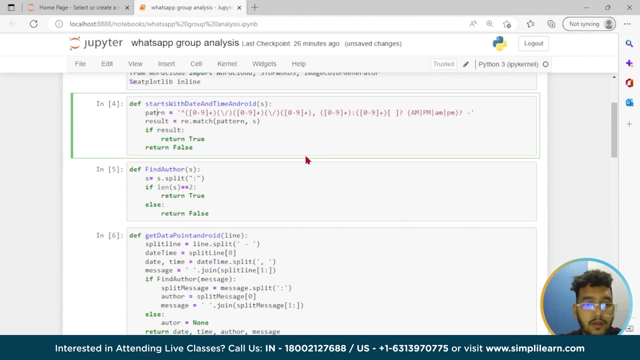 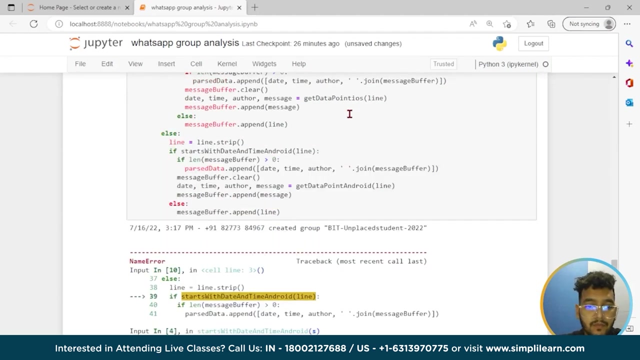 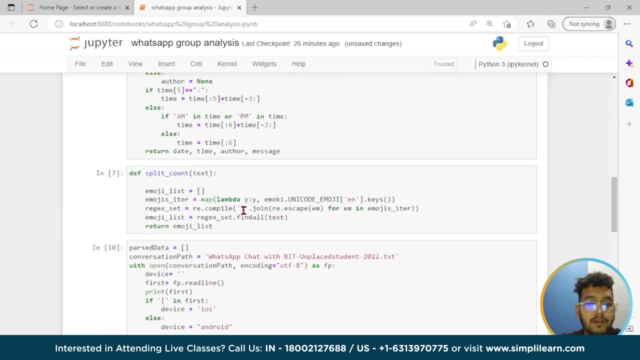 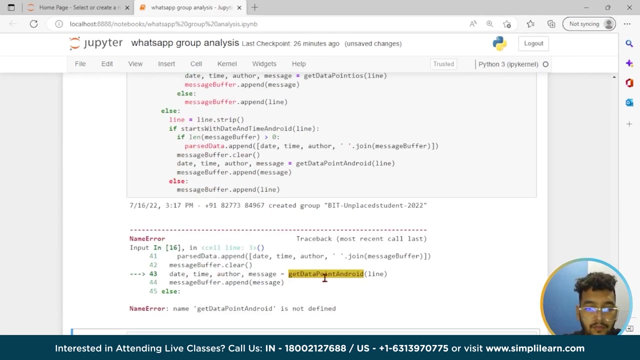 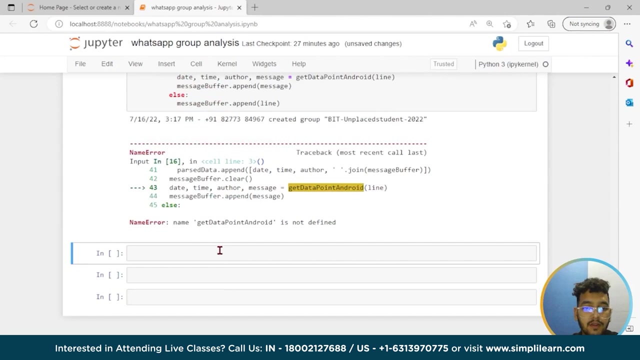 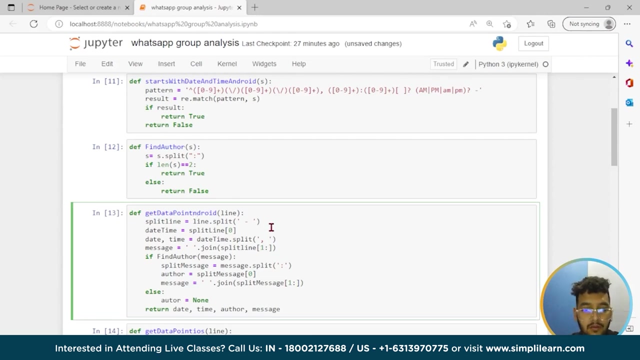 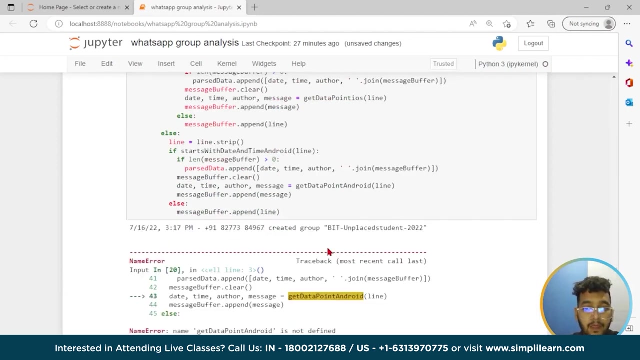 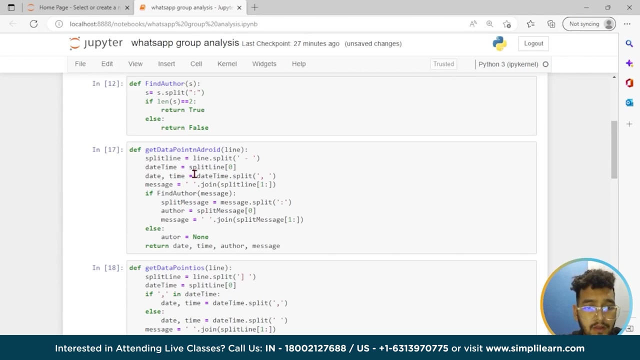 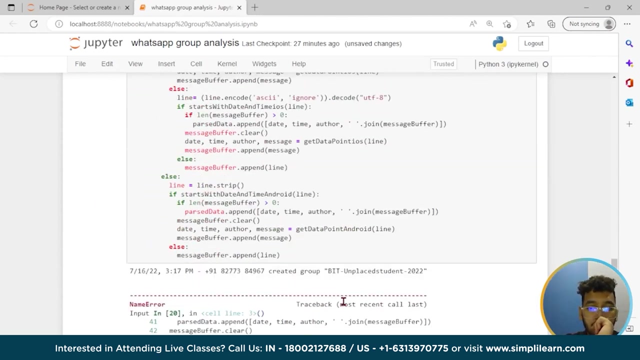 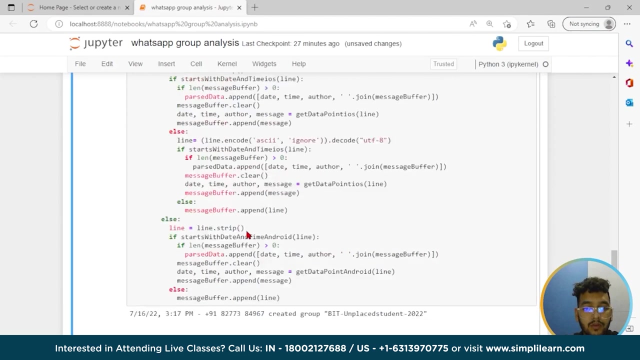 okay, okay, start with. pattern is not defined here in pattern, so at data point Android line- maybe the spelling mistake, as you can see- point get: data point Android is capital and this, what did she like? get it appointed right, we copy it from here. copy, copy, copy, copy. 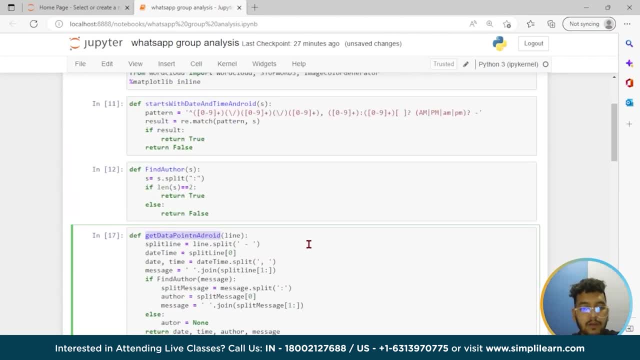 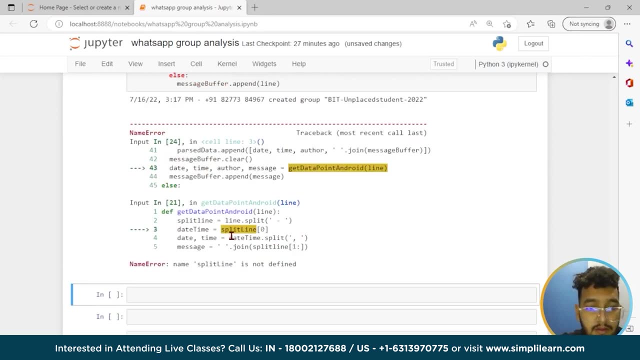 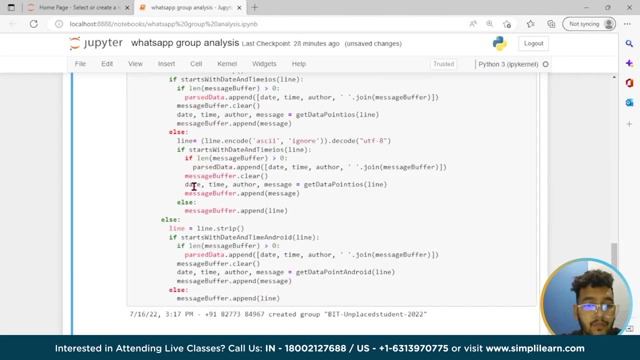 and then let me run it hit line. okay, the split line. split line is not defined. okay, let me get back to you so, as you can see, everything is sorted. so so here you can see. this is the group name. okay, bit and play this from 2022. 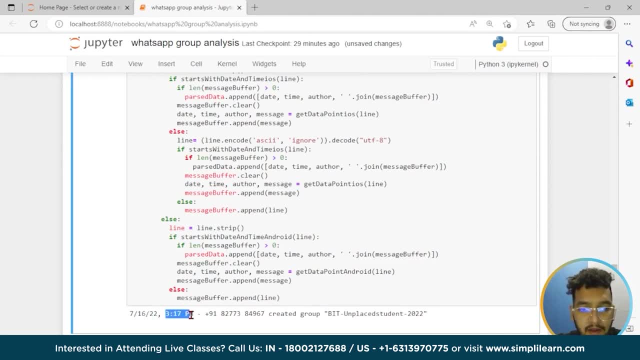 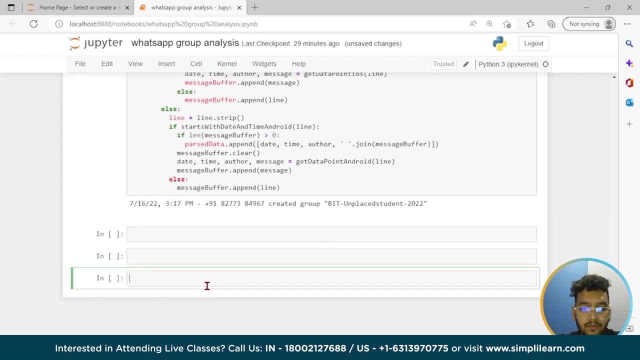 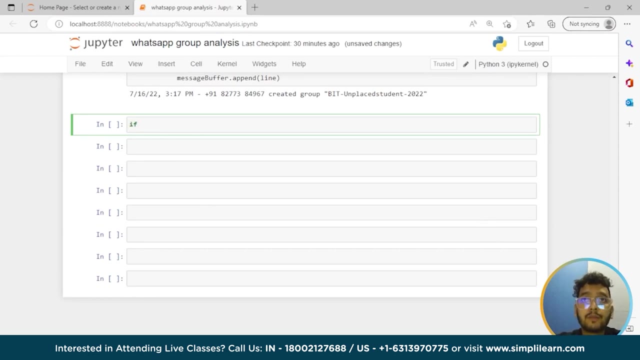 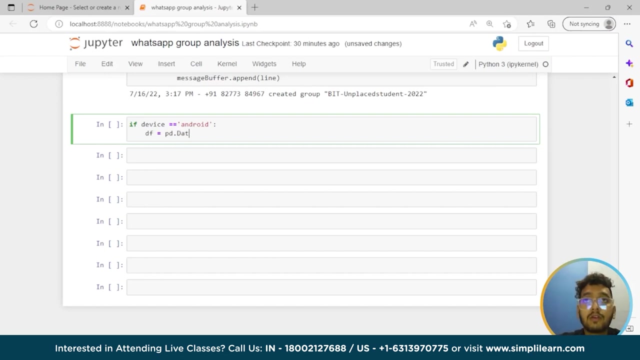 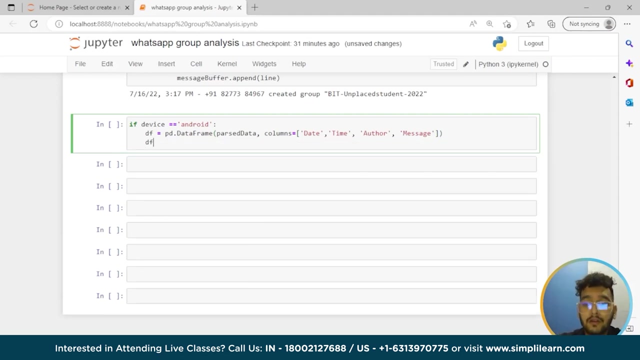 and this is date and this is time and this is the guy who created the group. okay, so here i will write: if device plus you go to android, okay and df equals to pd dot data frame pass data columns. question it okay. x and df eight. i'm setting the columns pd dot two. 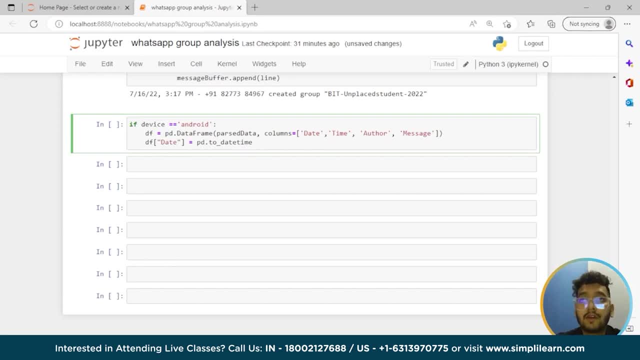 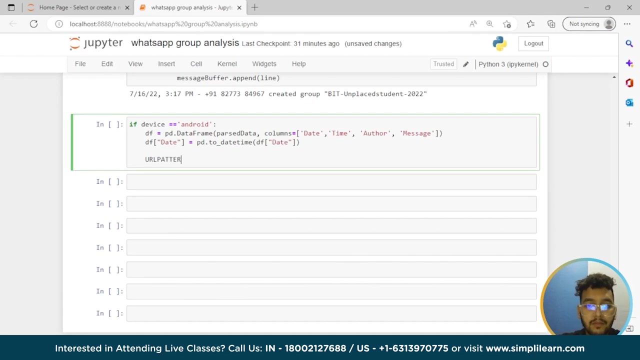 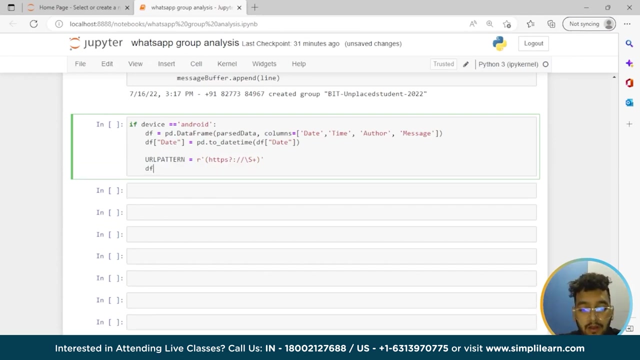 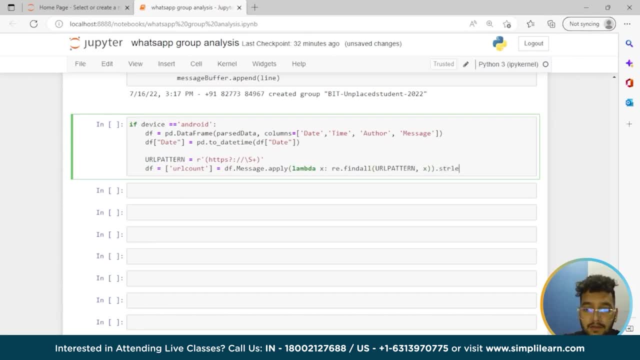 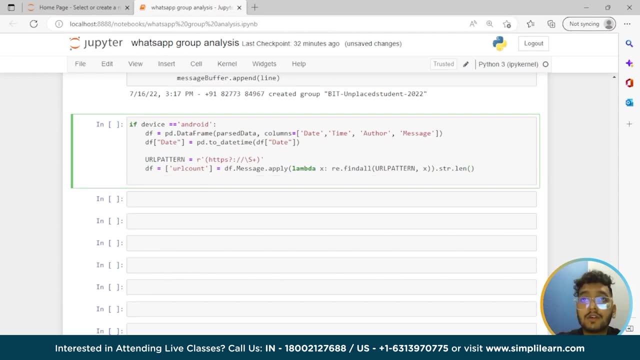 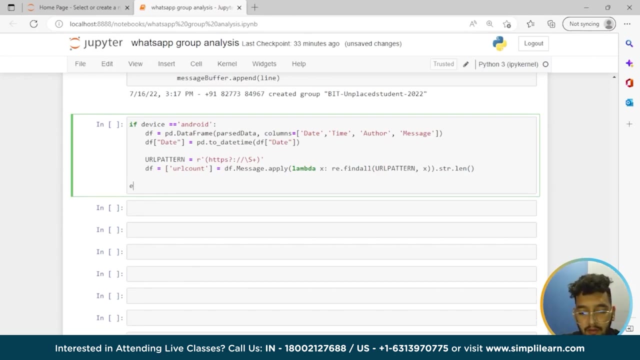 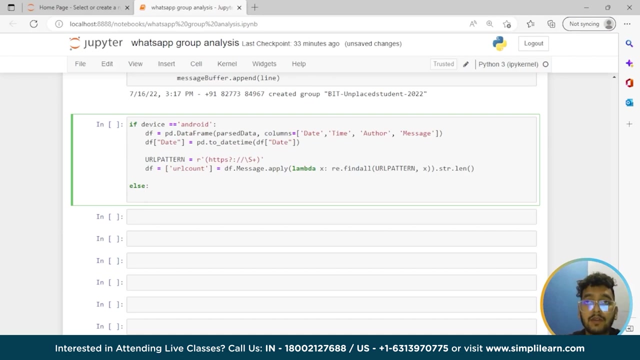 you are a string length, so is fine after it. else, here we are, like initializing the data frame under data frame. so DF equals to PD dot data frame. was it a comma columns? was date comma? I'm mother, yeah, so this is the pandas data frame where eN Lichthardt the what's your? 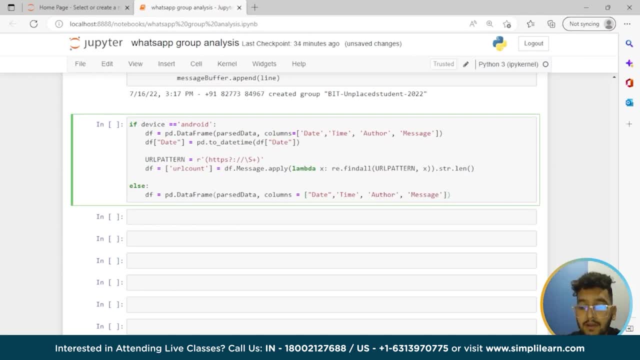 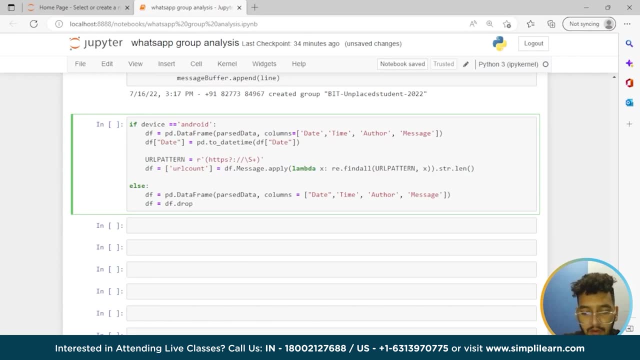 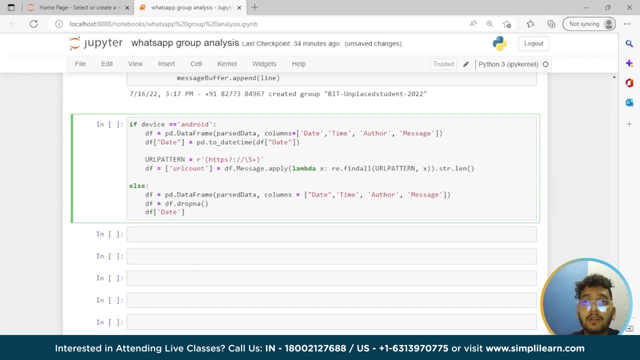 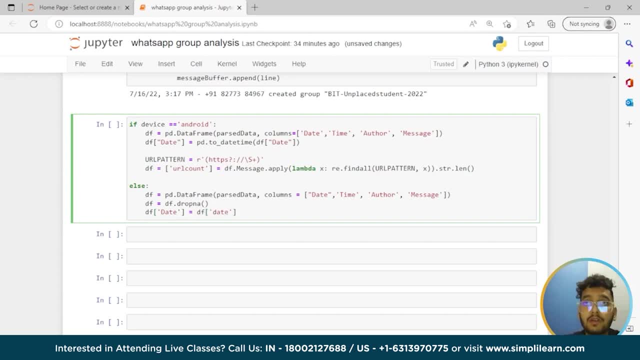 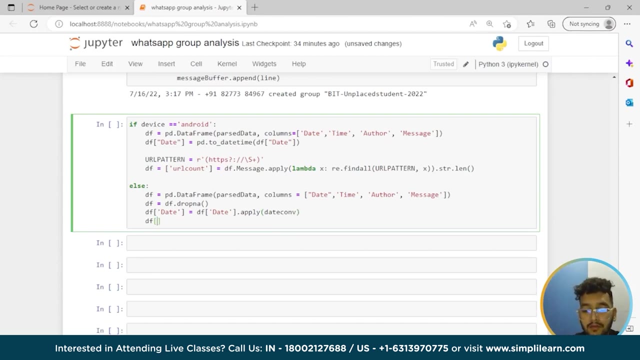 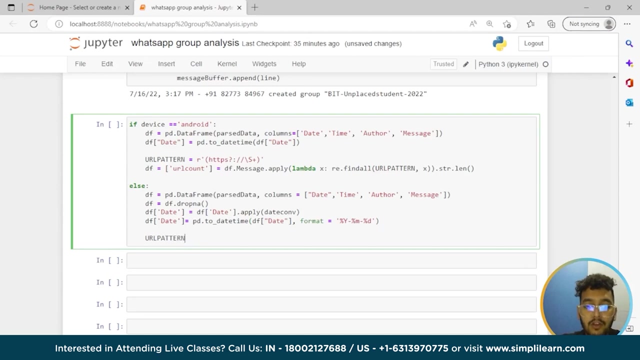 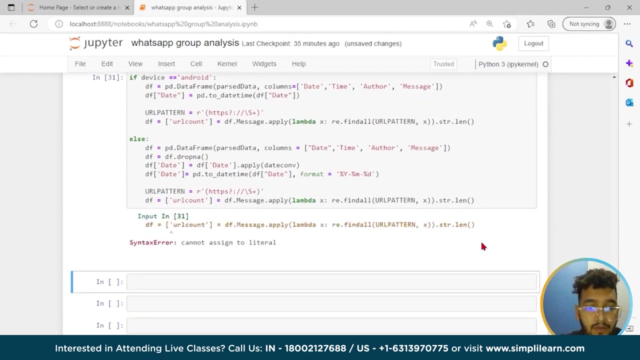 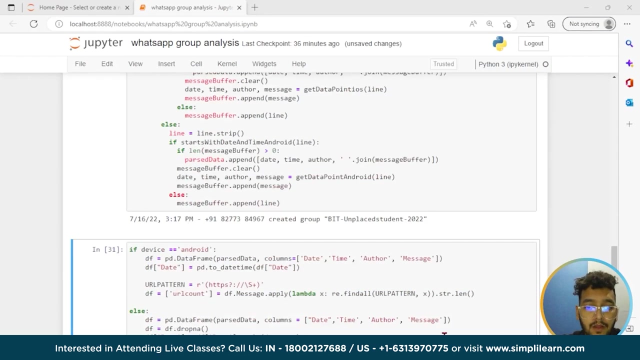 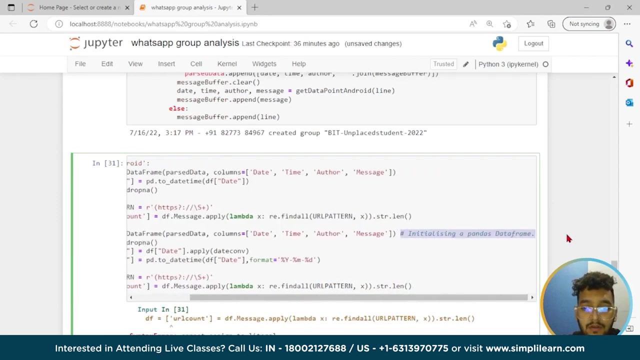 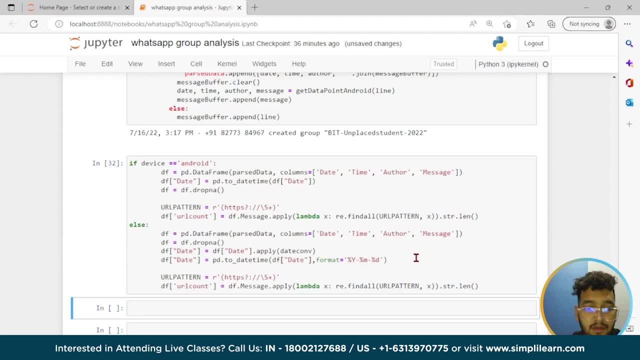 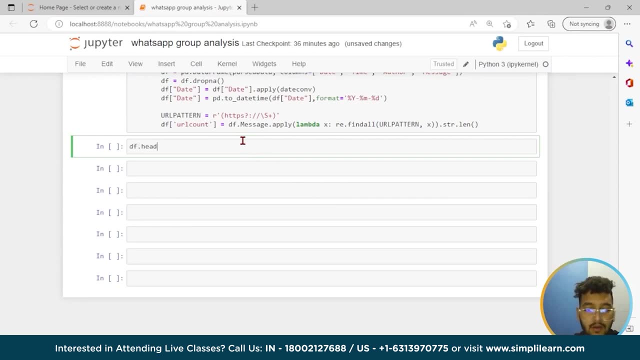 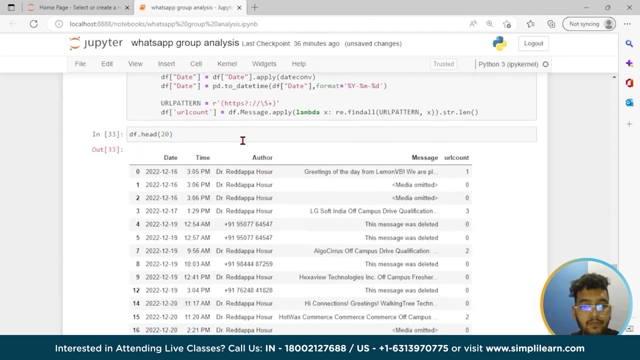 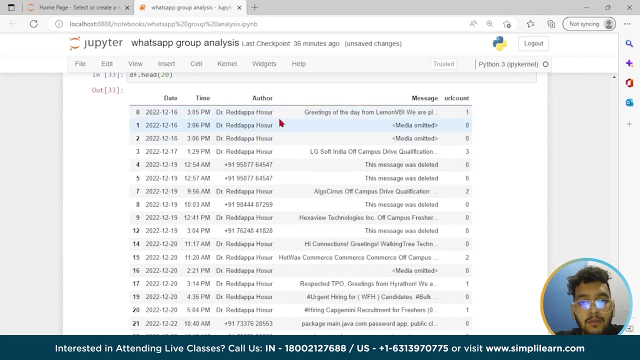 not assigned to little well. it is not assigned to little well. this the answer. this is the answer. yes, that is the answer. that is. this answer is correct. so this is time when he sent or when she sent. okay, so this. there are three links in this, two links. 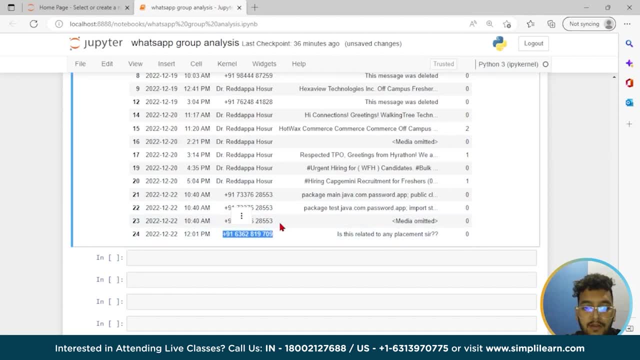 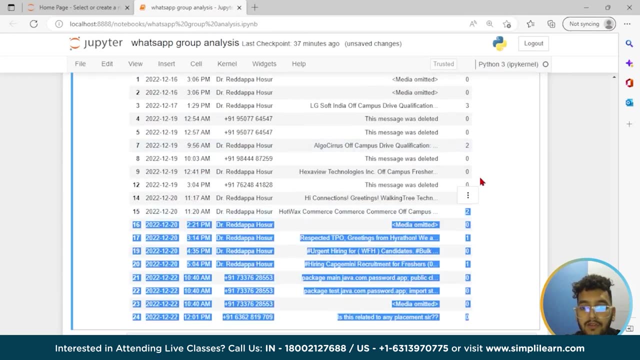 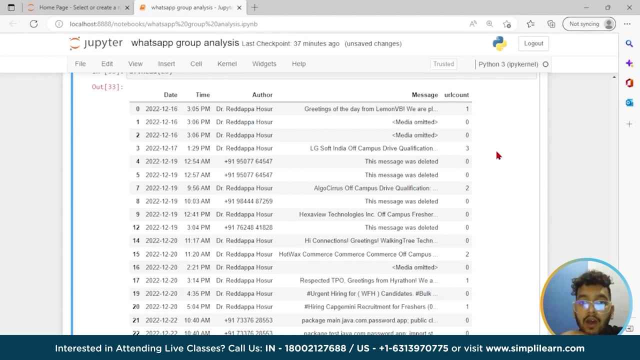 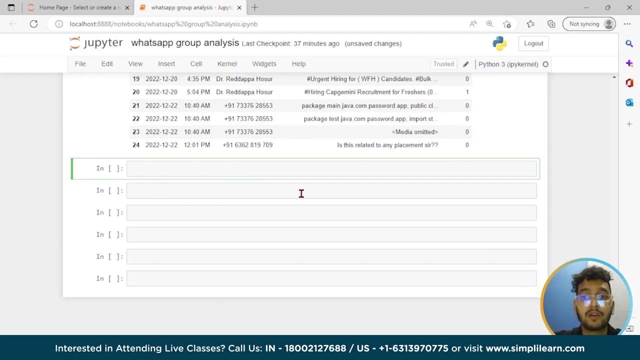 okay, is this related to placement? this guy sent? okay, so these are the top 20, the number of links you can see in the particular message: two, three and then the zero, zero. this is the media. okay, so i downloaded, uh, the chat without media. okay, you can chat. you can come using media. 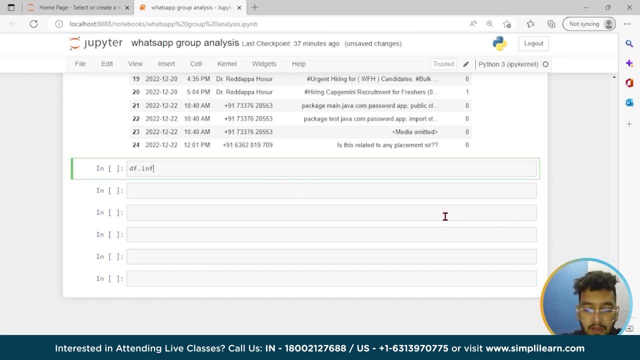 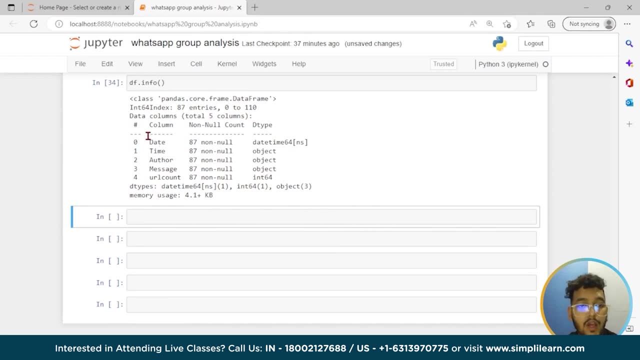 let's see the information data. so this is. you can see we have five column: name: date time, author message: url count. okay, so, okay, url count date time. this is object and this is object and url count as n64. okay, let's see all the author names, only author names. so here i will write df dot dot. unique. 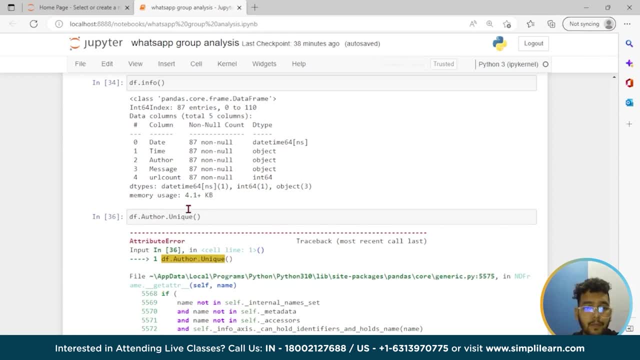 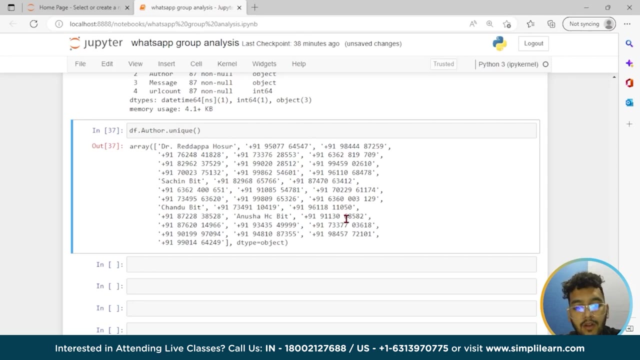 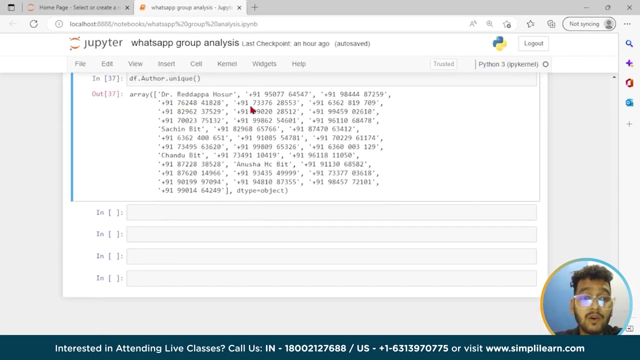 my bad. so these are the authors, all the authors. number of members you can say in particular, uh, group, okay, these all are the unique authors. so, moving forward, let's see the you know like, let's drop all the null values. so for that we have to write df. dot equals to df dot drop and. 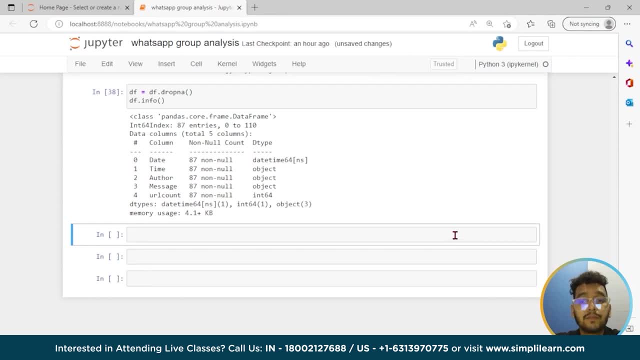 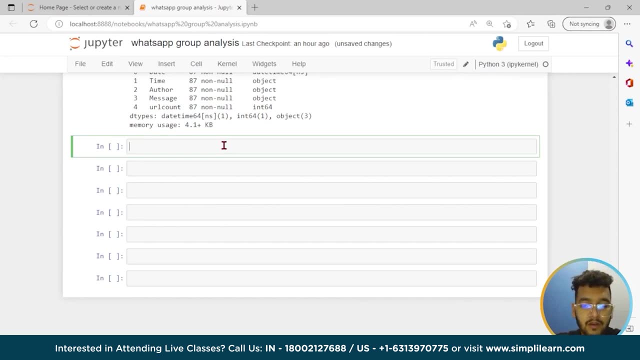 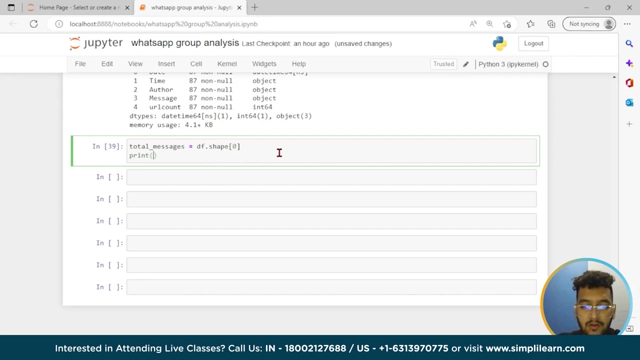 oh, top n is done and so these are the some basic. you can say the function of machine learning and python. okay, and moving forward, let's see the total messages. total, this first two df dot shape i'm going to print and so we can say that this is. 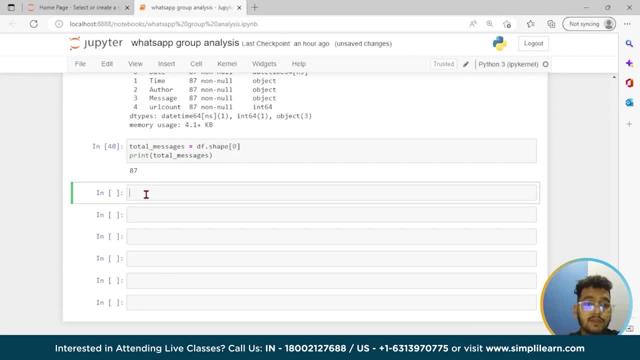 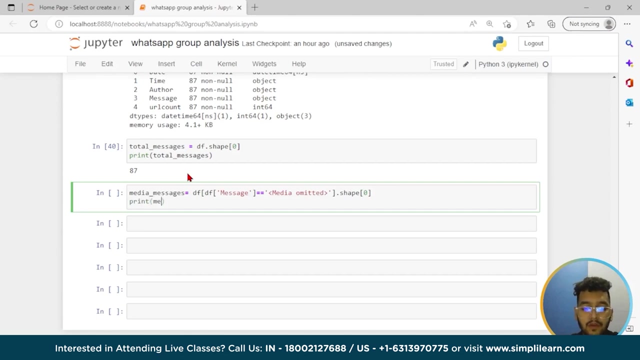 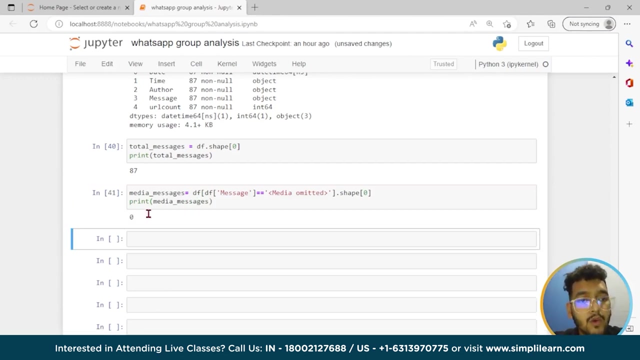 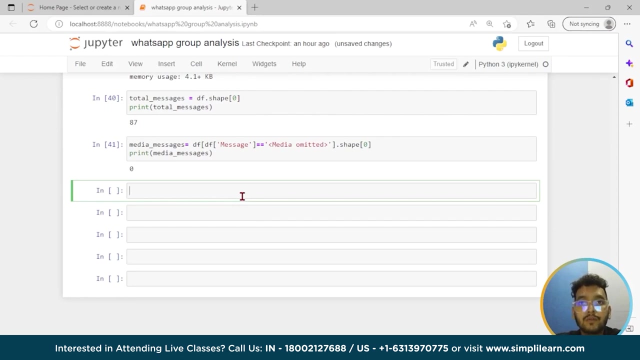 a custom text. oh so, uh, such a good, uh, a very good. either you are specific, random, um ask practice. single mean three reasons, and omit it if you know. and media, why this is zero. I already told you like I export chat without media. okay, so you can export with media too. okay. so right, here you are then and done. 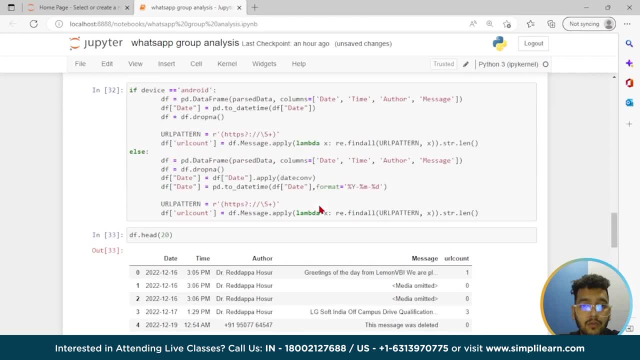 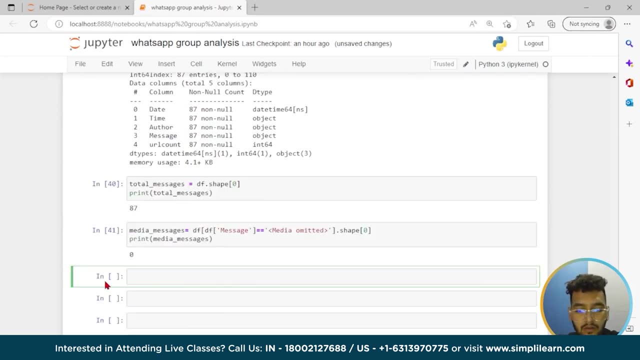 you, okay. so this is the you can say the rejects pattern. this one: okay, this is the rejects pattern and with the start with the STL HTTPS. and second one: this: this URL, count written URL which matches with pattern and counts it through the all the lambda function. okay, now I will write one more. 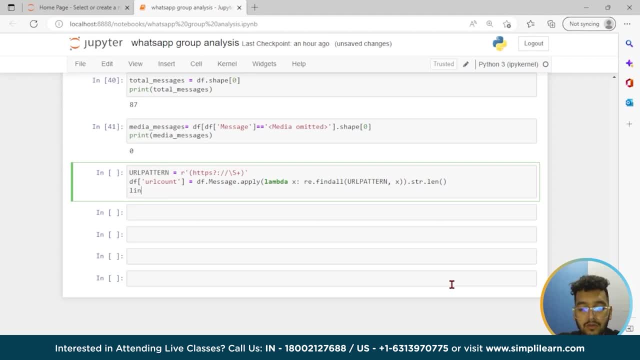 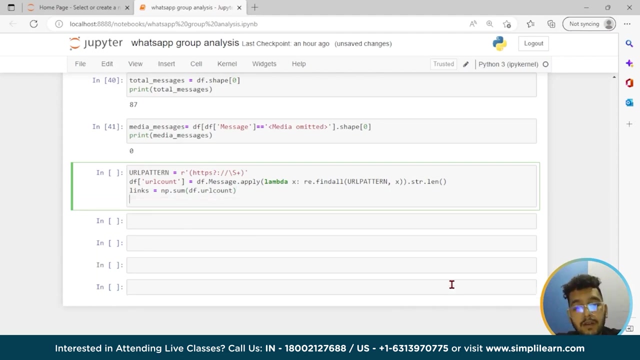 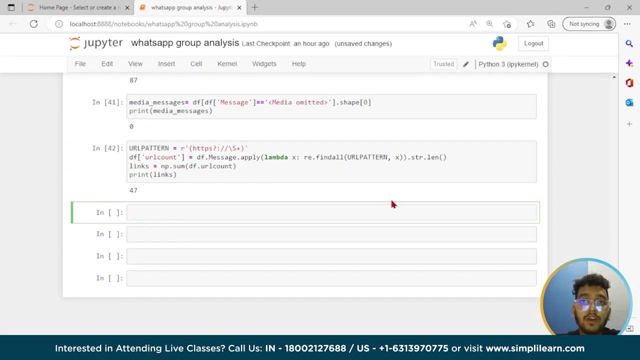 thing was you and the dots some. yeah, what this will do this is sum up all the links. okay, so print links. as you can see, there are 47 links in the group chat. group chat information. okay, so moving forward, let's let us separate. and media messages. 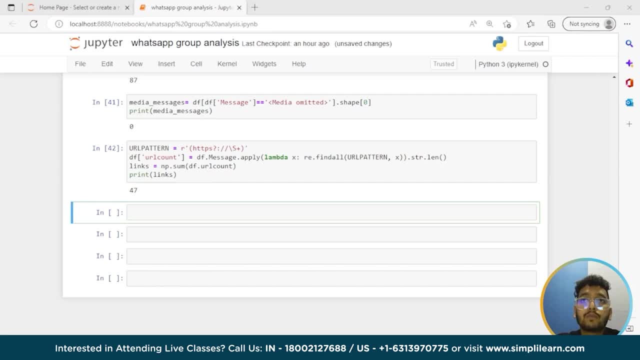 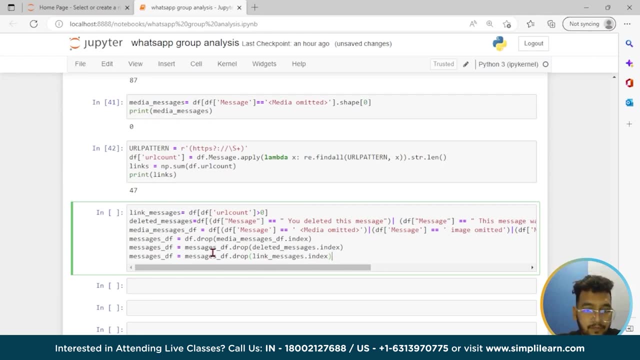 and the text message. okay, so this is the. it is the code for that. so link message go to URL count. okay, deleted messages and this message was deleted. okay, both the statement and this media Omitted this image. okay, this video, for the video and a text message that used to contain: this is the messagereally don't we need Михailo? 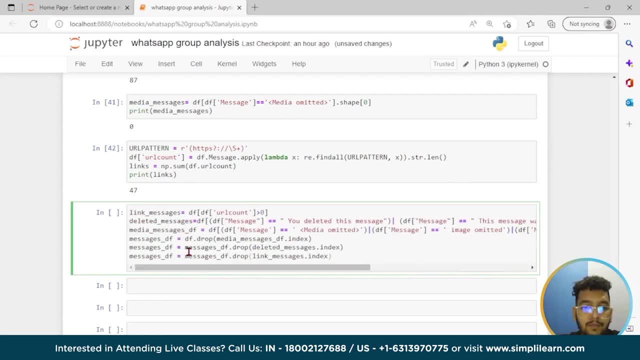 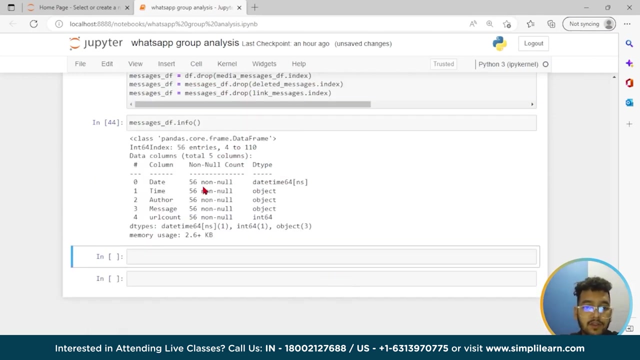 for the video and there is stickers you send. we send. okay, then the drop and a deleted message and the link message. okay, so for that let's press enter and message under so DF dot. okay, so now you can see we deleted, dropped all the. you can say the deleted. 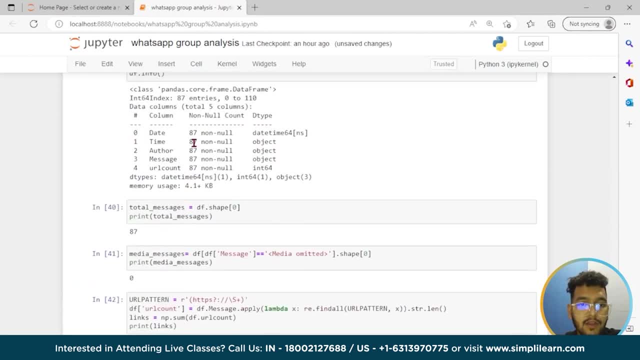 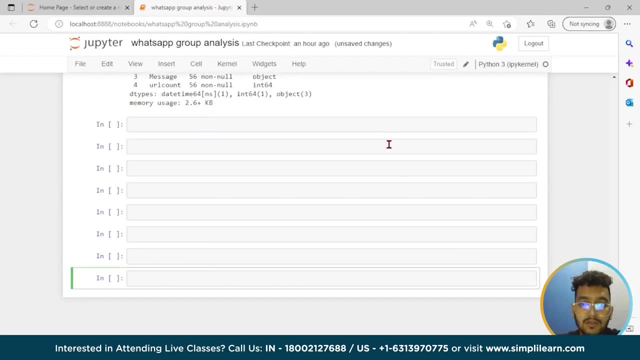 messages or the link messages. okay, as you can see, 87, now 56 only. okay, so let's calculate words and letters. okay, for that I have like messages. let's go DF, then let account. let account then equals to messages here message. right, like you can, I will write here messages. 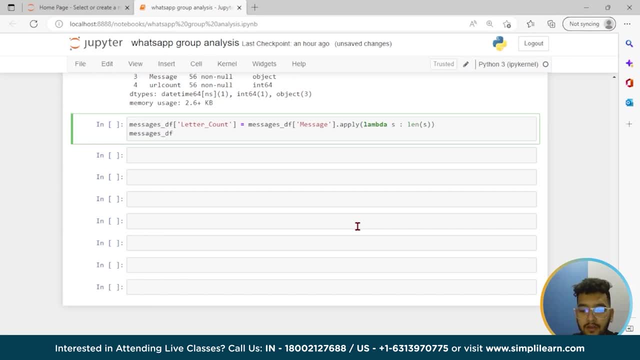 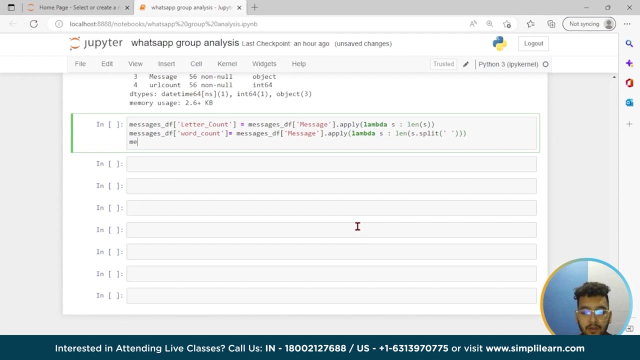 who DF? then what come you? you, yes, underscore, dear you, which dot dot you guys it you, yes, messages, yes, messages, yes, messages, yes, yes, the message count 1. okay, so here you can see. I wrote here: split, so word count will be count as like the space. you can see space between the words. okay, splitting sometimes with the. 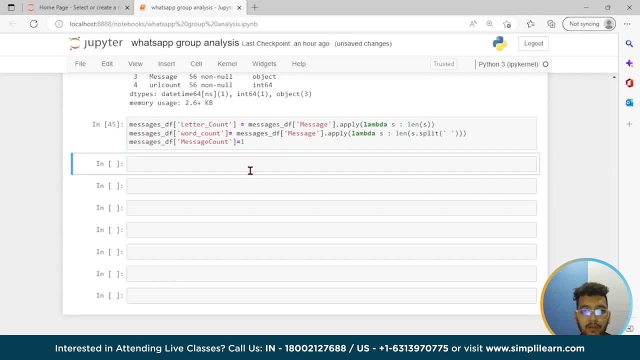 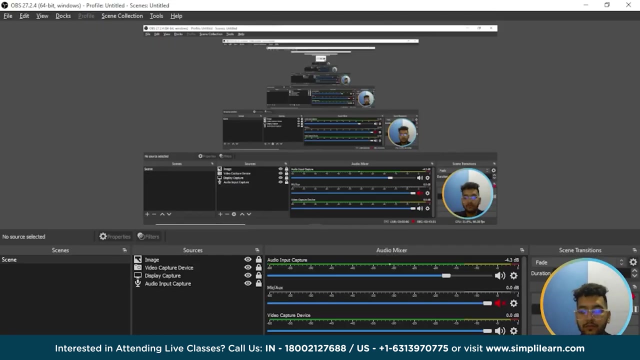 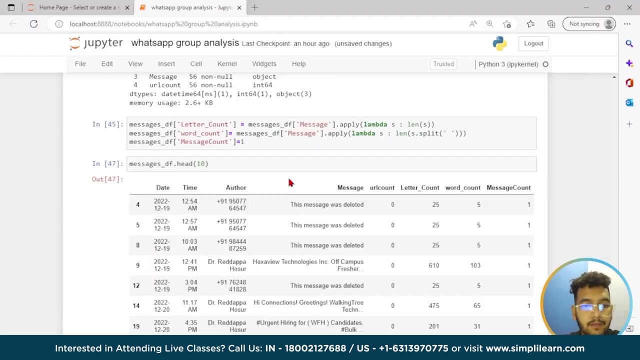 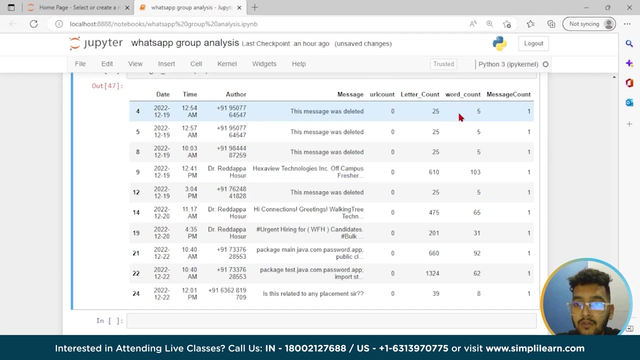 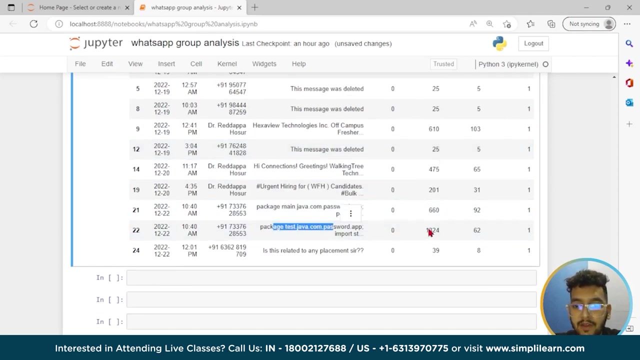 white space, you can say: okay, let's see as it underscore DF dot at 10 present. here I have to write messages. yeah, now you can see this author saying this letter, count 25 and the word count is this and the message count is one only. so this package test dot things and this is things. this doctors, this urgent hiding work from home. 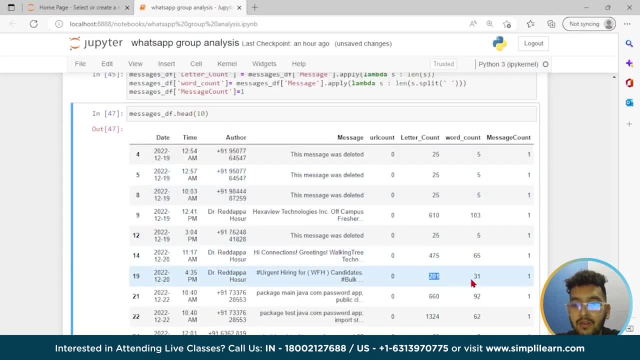 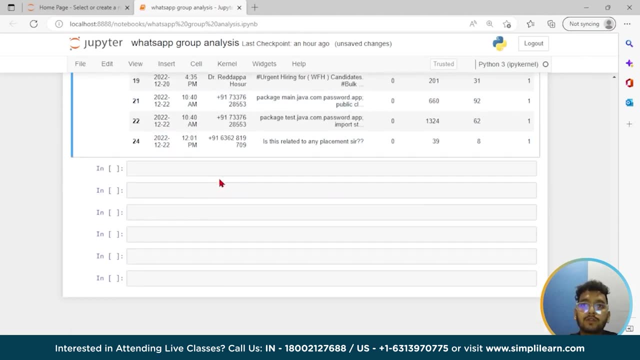 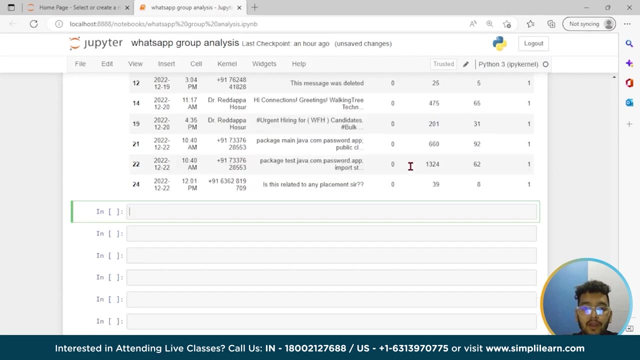 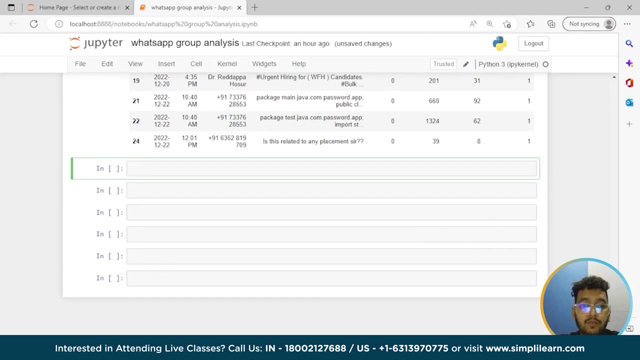 kind of things. and the word letter count is 2, 0, 1, then 1 counted 31. okay, and this is something hexa view things, and okay. so these are the words and letters we calculate. okay, now we will see the like author wise. okay for that. I will write the code and we'll get back to you after that. 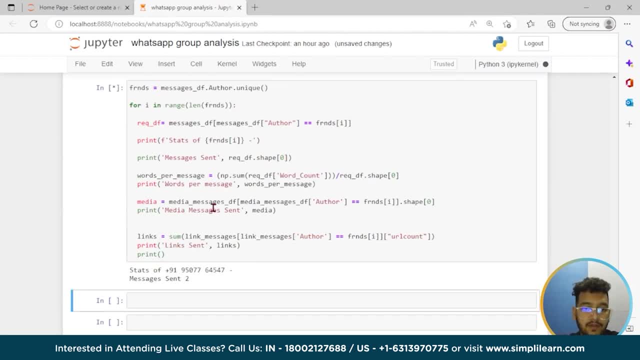 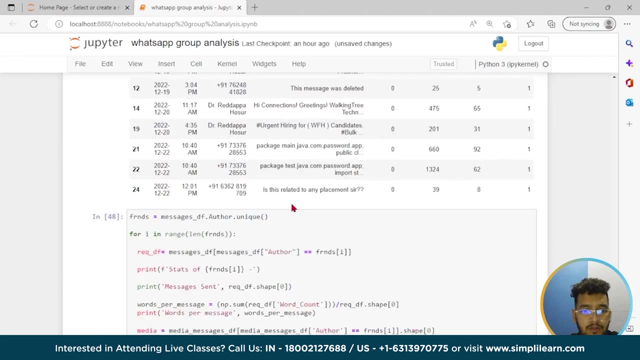 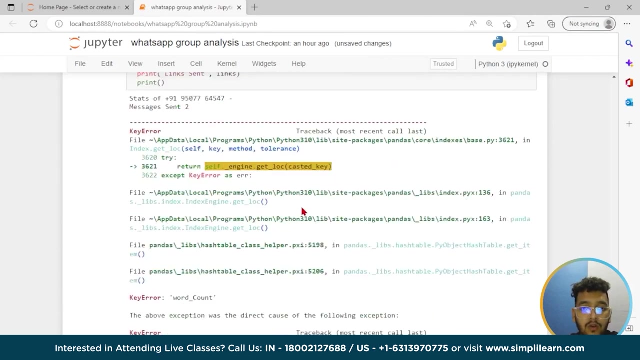 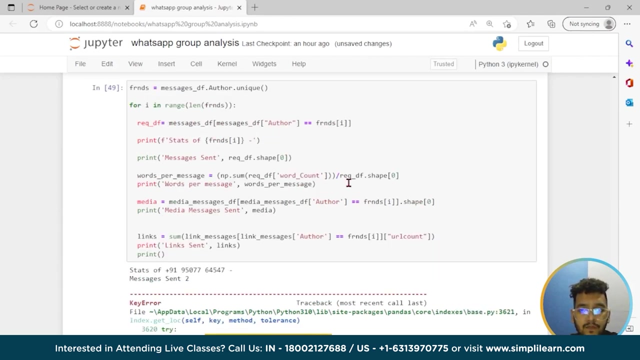 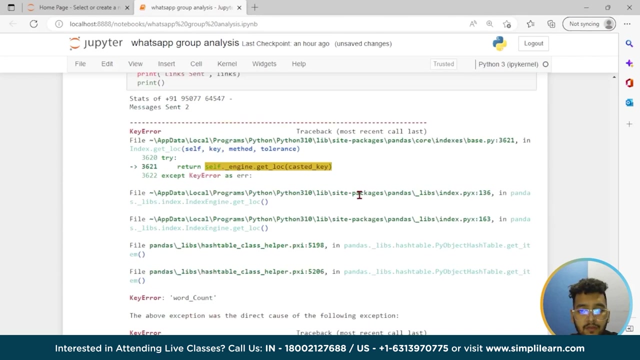 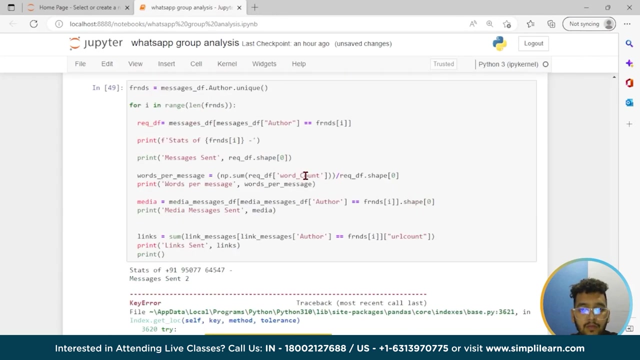 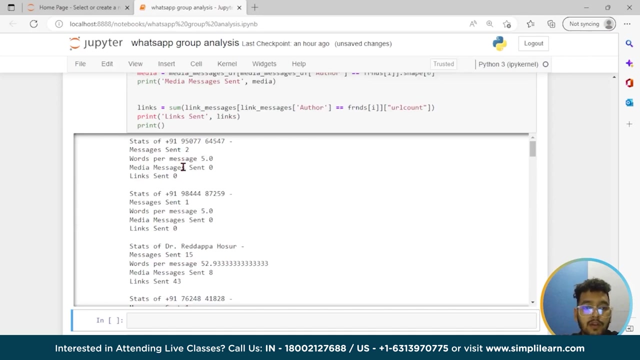 so this is the code for the. you can say stats: okay, there's an error. word count where? where? What is the word count? Okay, so these are the all the stats per user, per author. you can say message sent and words per message and media. media sent is zero because, like I haven't, you know, included. 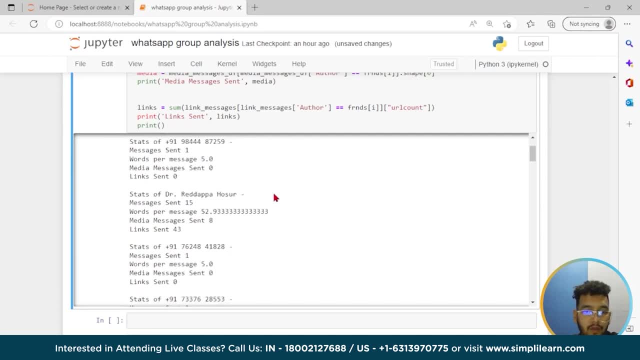 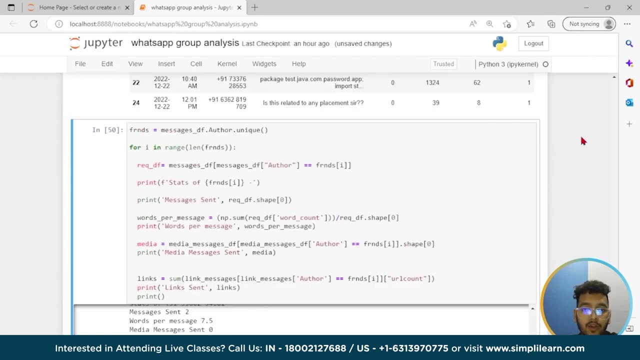 media in my chat. So that's fine. Okay, words per message. this is all the stats you can see And let me explain you the code. So this is for the like filtering, you know, filtering out the message for the particular. 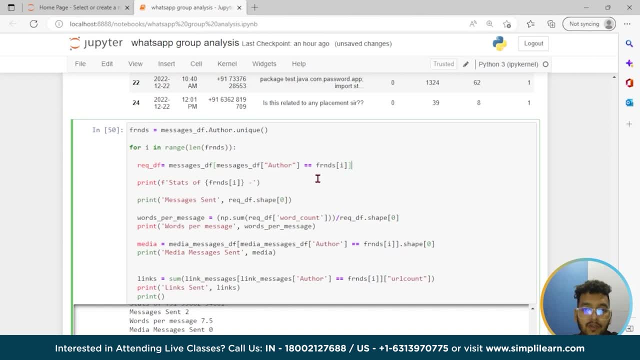 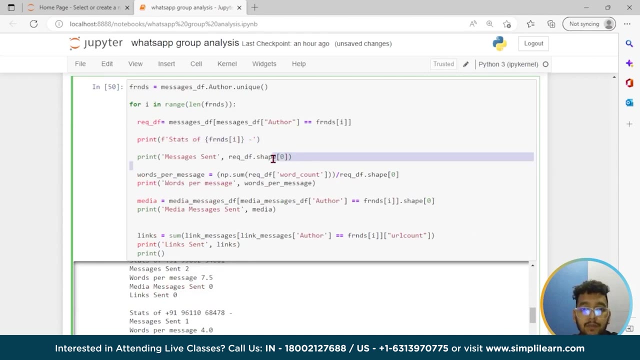 user, This message df, message df, author, friends, And for this, like req, df will contain messages of only one particular user. So we are printing that, okay, and this shape this one. so shall we print the number of rows which indirectly mean the number of messages, okay. 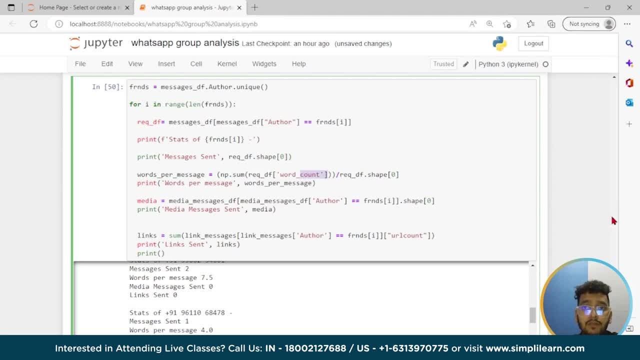 So this word count, this word count, so word count contains all the total words in one message. sum of all the words divided by total messages will yield words. words per message. Okay, so this is for the media messages. this is zero. 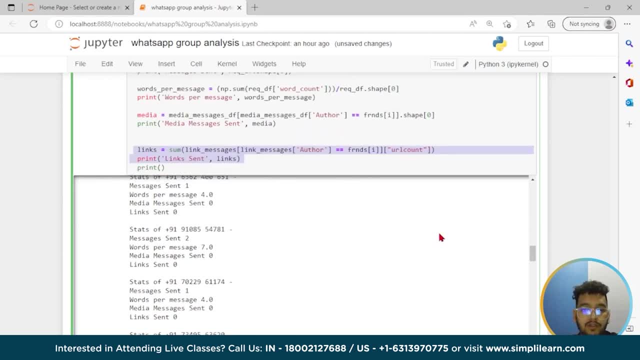 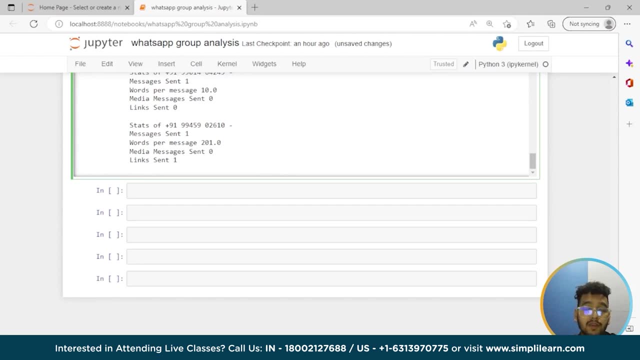 And this is where the link consists of the total links. Okay, so this is all the data. So moving forward, So let's see the times of the day. Let's see the times of the day. So in this time, the most messages gone like this: 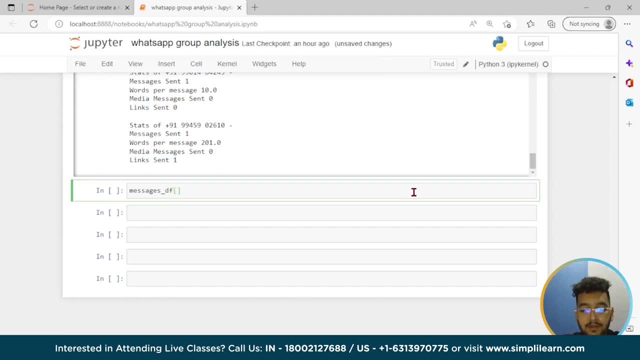 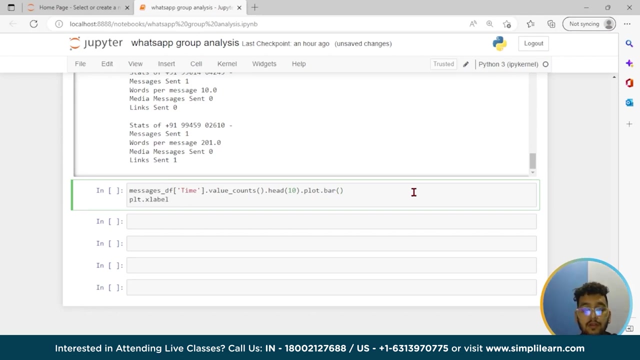 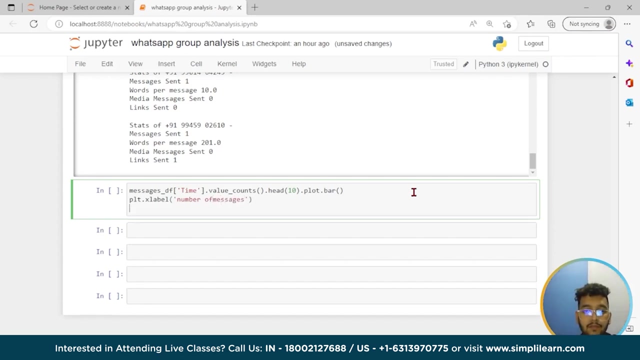 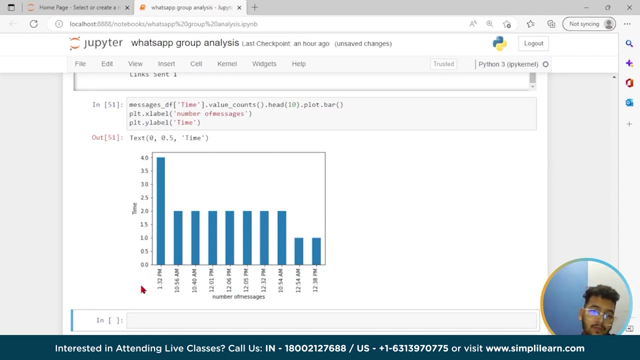 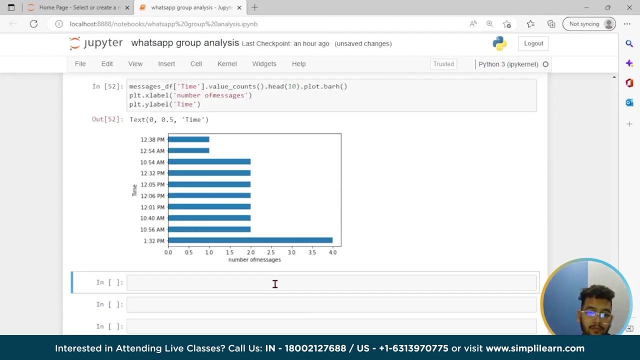 So messages df. That is timevalue, Okay, Okay, and thought paragraph: okay, horizontal. then PLT dot X label: yes, and PLT dot Y level- you. and times of the day at which the most number of message sent: okay, this is top ten. okay, so because of okay, let me do like this: now it's good time, a number of 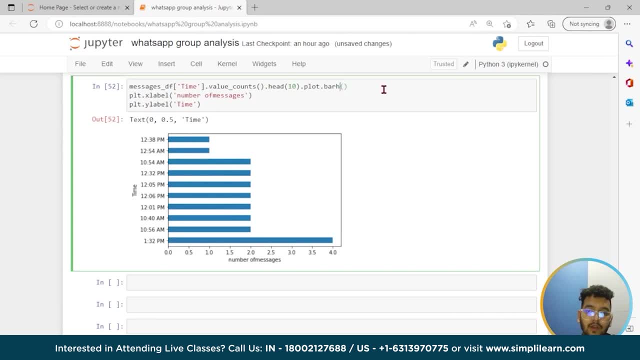 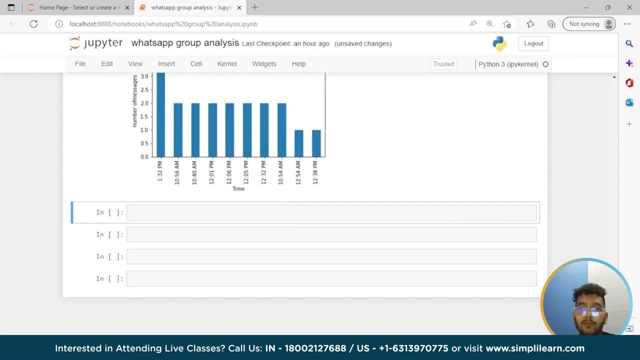 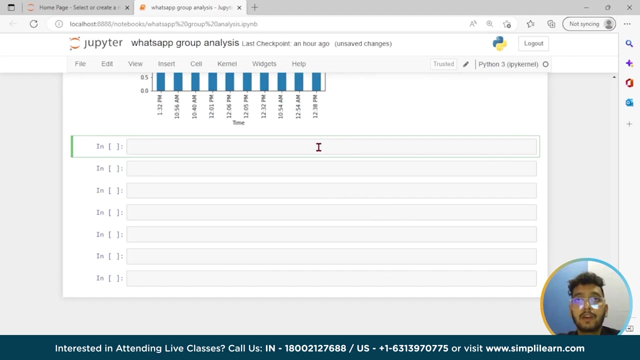 message. okay, this is it what I can do. number of messages and the top ten time: most number of message. now the time is came to see the word cloud. okay, now we'll make the word cloud. so for that I will you text pursue or join. join you can say review. 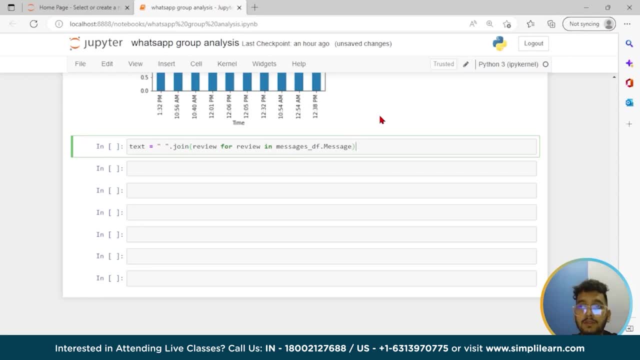 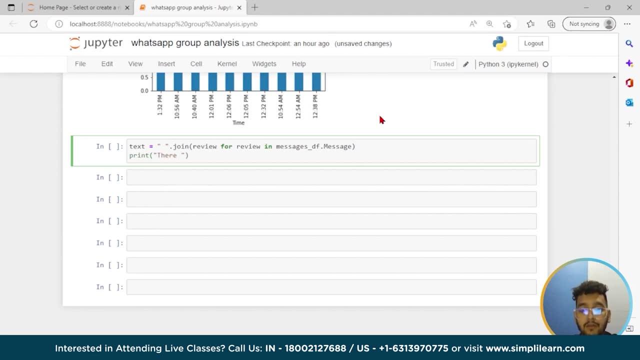 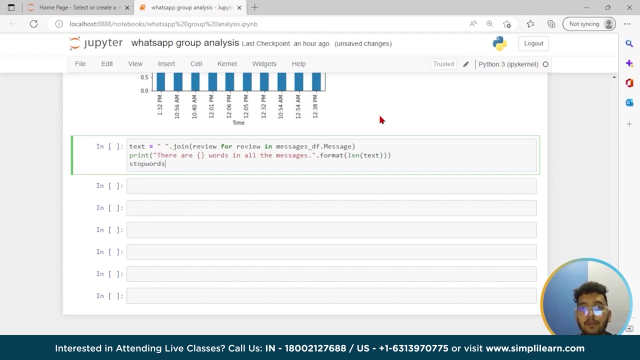 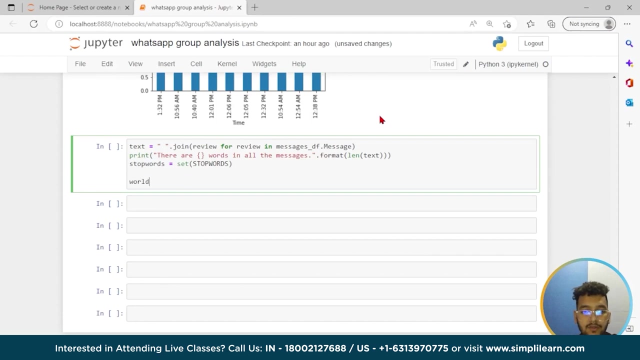 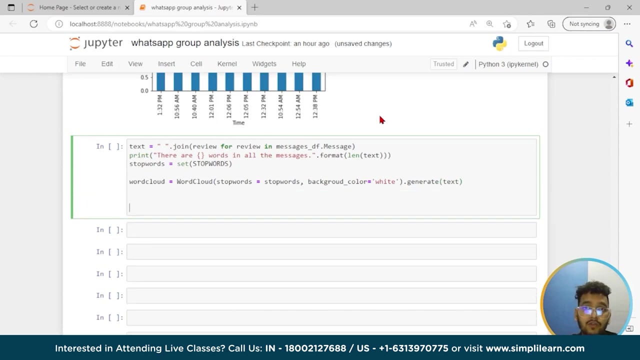 print. print as much words. the okay dot dot for format will be length and then stop words, one of my favorite set. stop words then will generate the word cloud. this is to generate the word cloud. okay, sorry, word cloud. now upwards and ground white dot red. yes, so will display the generated image and the plot using the, you know, matplotlib way. so 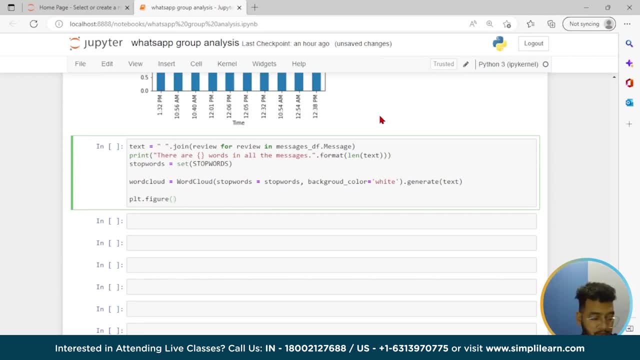 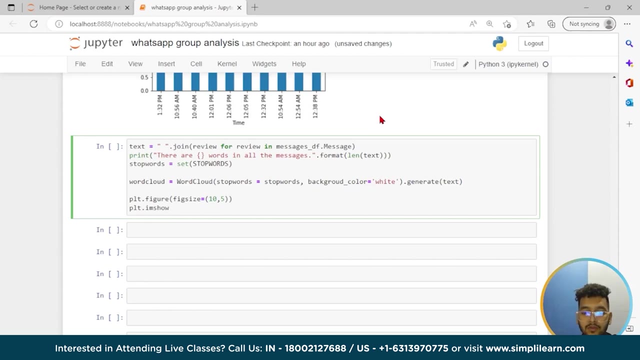 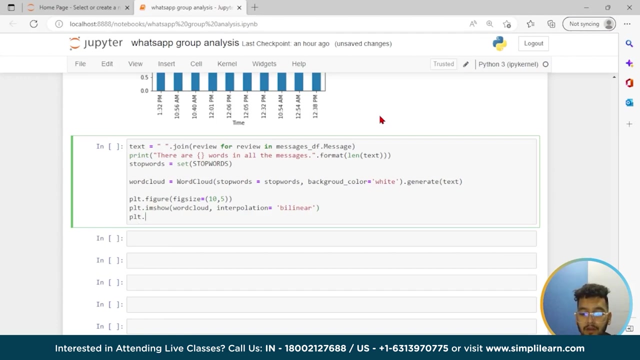 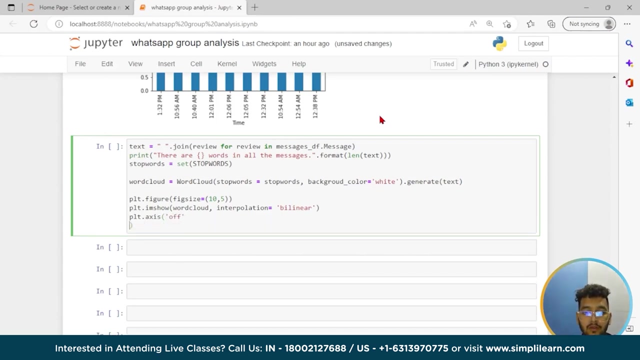 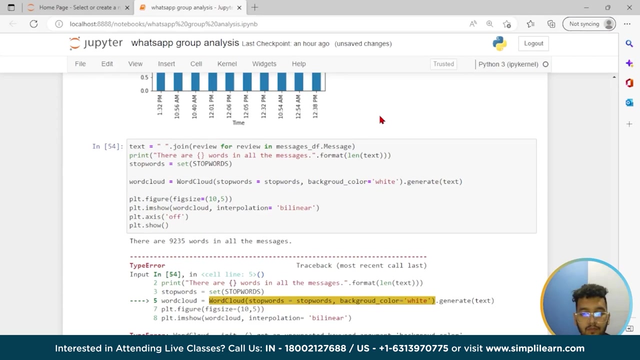 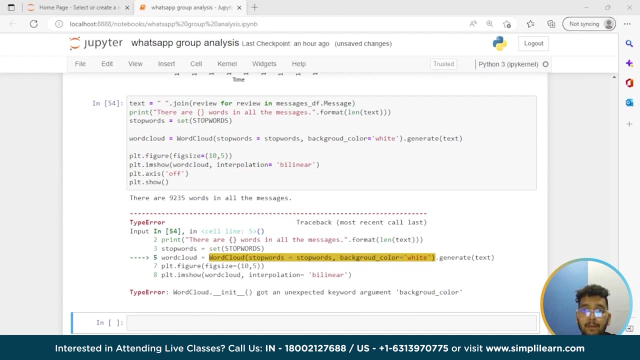 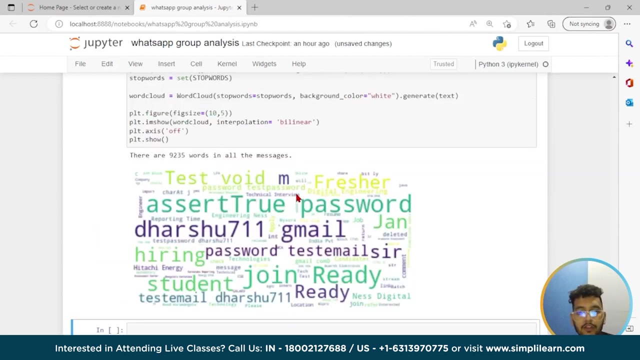 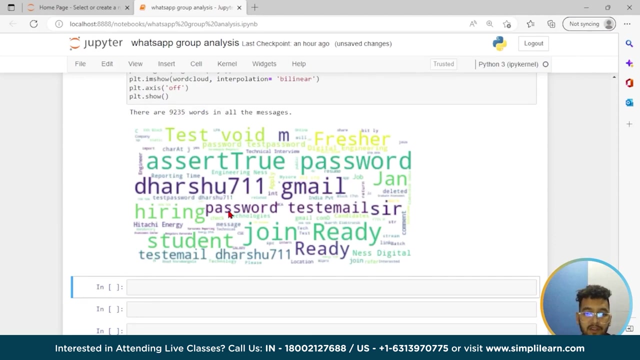 here the dot figure size size, then corner relation equation equals to set it to bilinear and then erd dot axis. You can see there are 9 to 3, 5 words in all the messages. So these are the some gmail password pressure ready test email student and see something. 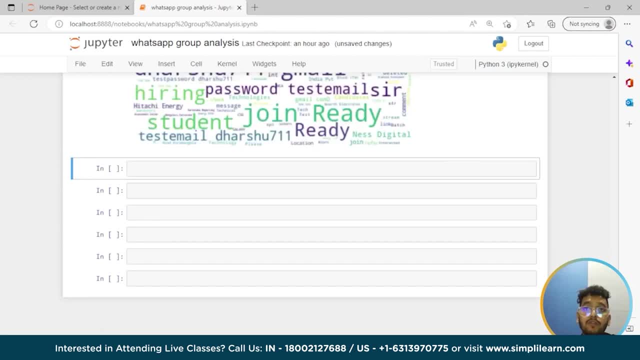 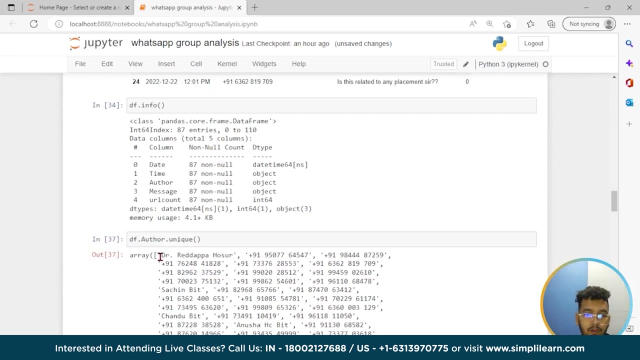 like this: These are the worldcloud. So what if I want to see the particular author name worldcloud, Like how many messages he sent and all like this. So this is the doctor I took from here, See doctor Redappa, And this Chandu something. and this Anusha. 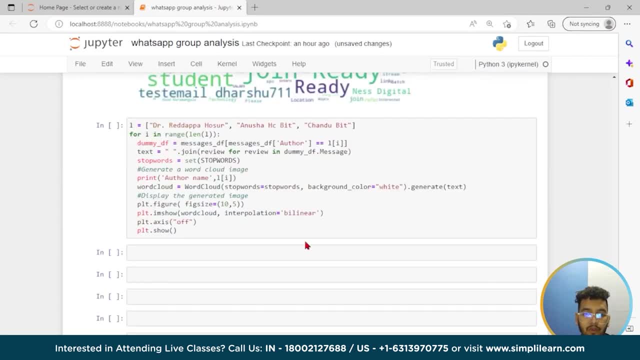 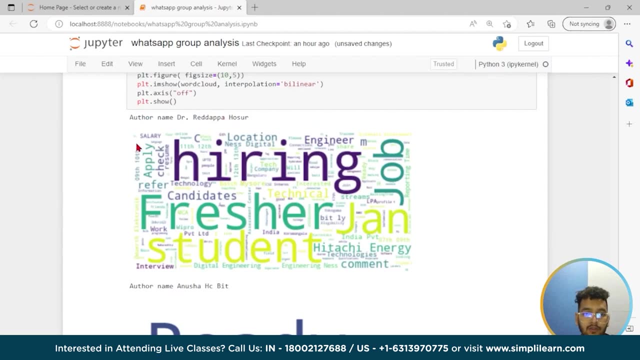 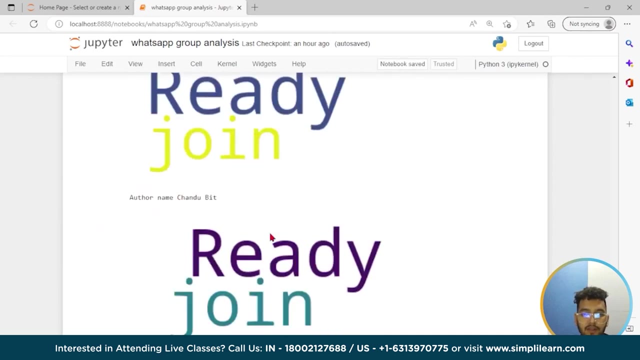 You can take the number also, no issues. So let's see. This is author doctor Redappa. He sent hiring job freshers student and this is Anusha. ready join and save the Chandu video: ready join. 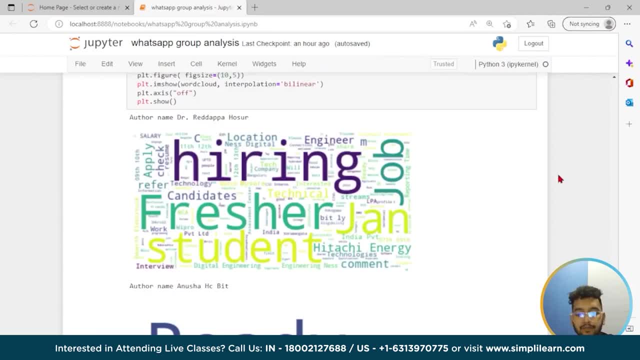 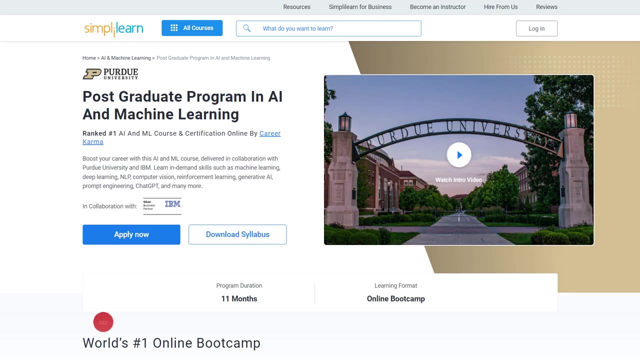 So this is how you can analyze and you can see Data. you can analyze your whatsapp group data. Okay, I will add all the you know steps how you can explore the chat If you are looking for a course that covers everything from the fundamentals to advanced. 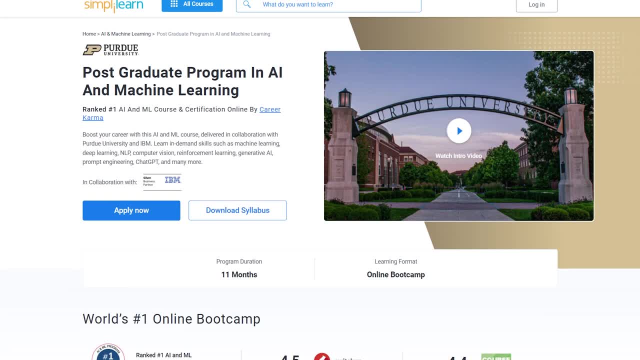 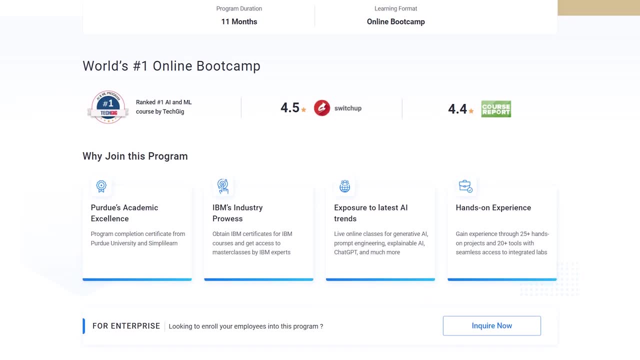 techniques, then accelerate your career in AI and machine learning with a comprehensive postgraduate program in AI and machine learning. Boost your career with this AI and ML course, delivered in collaboration with Purdue University and IBM. Learn in demand skills such as machine learning. Learn in demand skills such as machine learning. 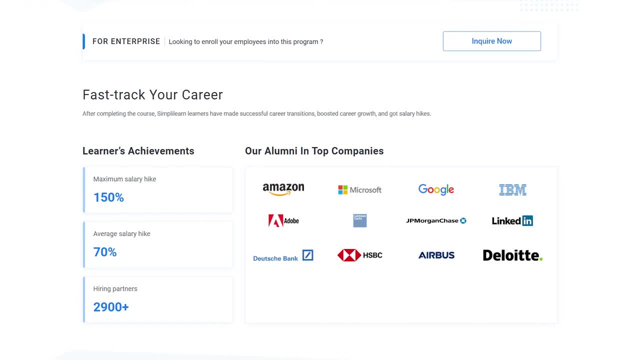 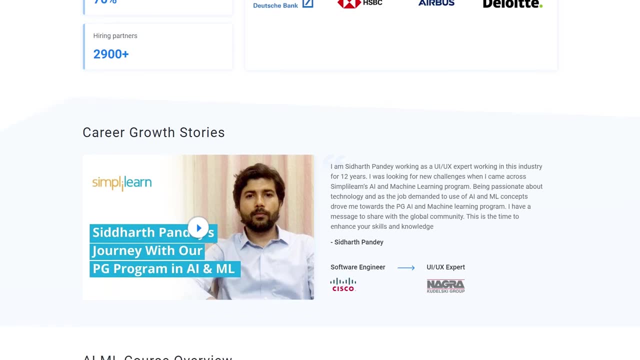 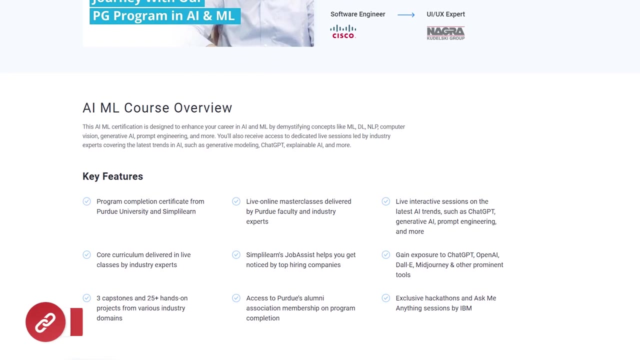 Deep learning, Deep learning, NLP, Computer vision, Reinforcement learning, Generative AI, Prompt engineering, Chat, GPT And many more. You will receive a prestigious certificate and ask me anything. sessions by IBM With five capstones in different domains, using real data sets. you will gain practical experience. 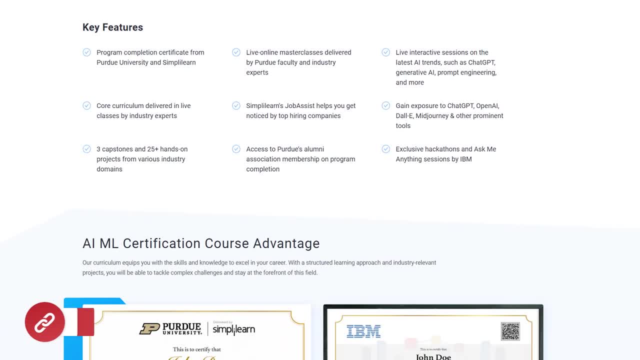 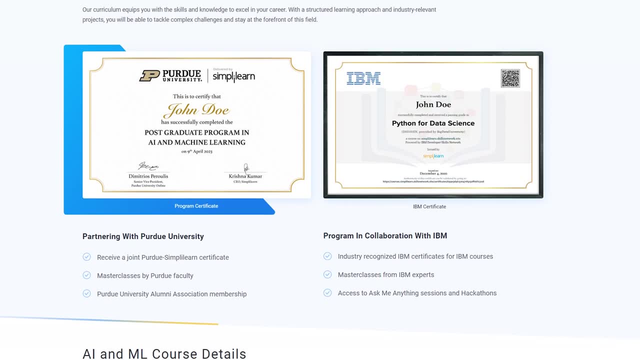 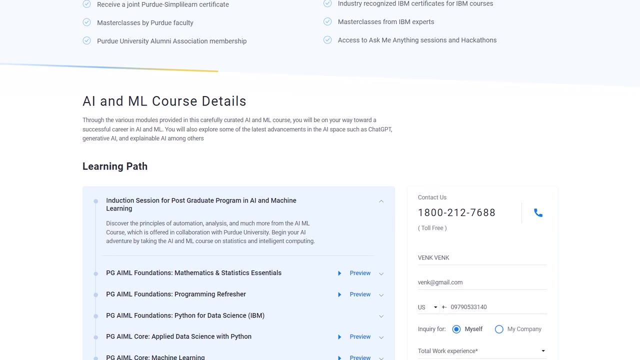 Masterclasses by Purdue faculty and IBM experts ensure top notch education. SimplyLearn's job assist help you get noticed by leading companies. This program covers Statistics, Python, supervised and unsupervised learning, NLP, neural networks, computer vision, GANs, Keras. 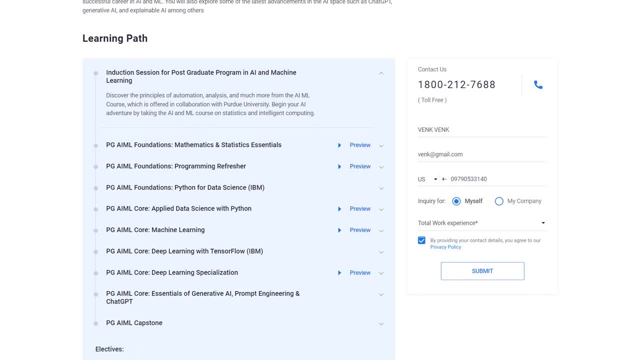 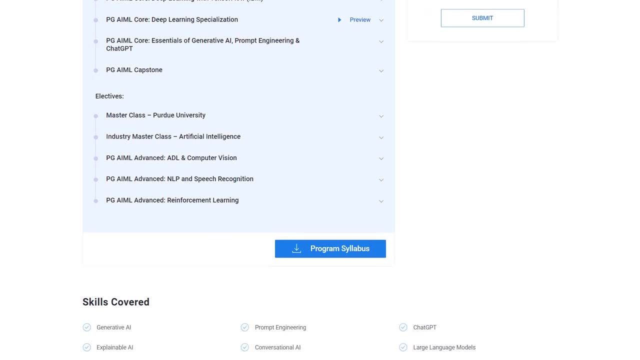 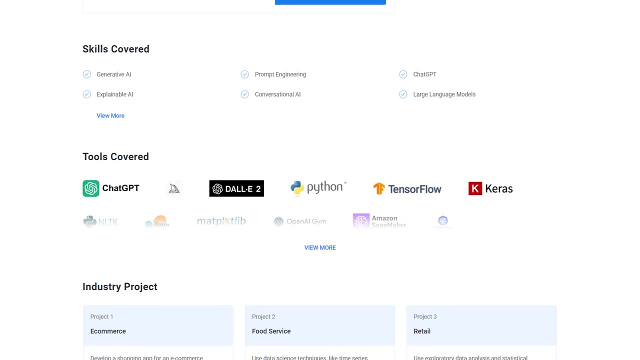 TensorFlow and many more such skills. Admission to this postgraduate program in AI and machine learning requires a bachelor's degree with an average of 50% or higher marks, along with the basic understanding of programming concepts and mathematics, And candidates with 2 plus years of work experience are preferred to enroll in this school. 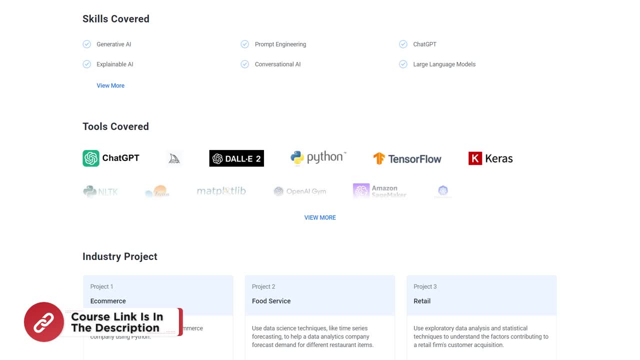 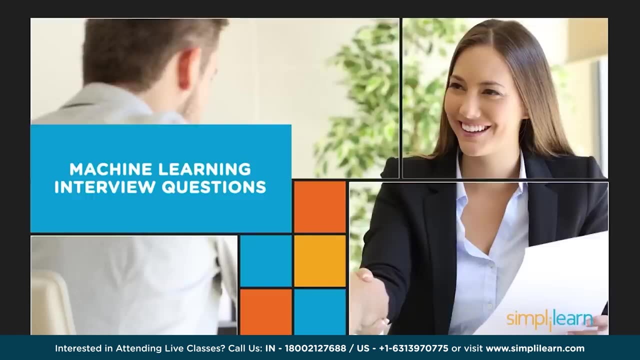 So enroll now and unlock exciting AI and machine learning opportunities. The link is mentioned in the description box below. Hello everyone, welcome to the session. I'm Mohan from Simply Learn, and today we'll talk about interview questions for machine learning. Now. this video will probably help you when you're attending interviews or machine learning. 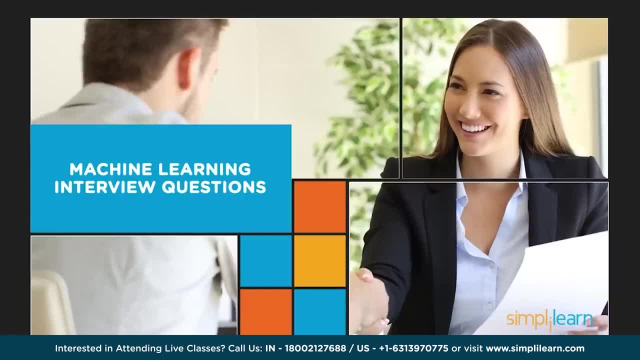 positions, and the attempt here is to probably consolidate 30 most commonly asked questions and to help you in answering these questions. We tried our best to give you the best possible answers, but of course what is more important here is, rather than the theoretical knowledge you need to kind of add to the answers, or 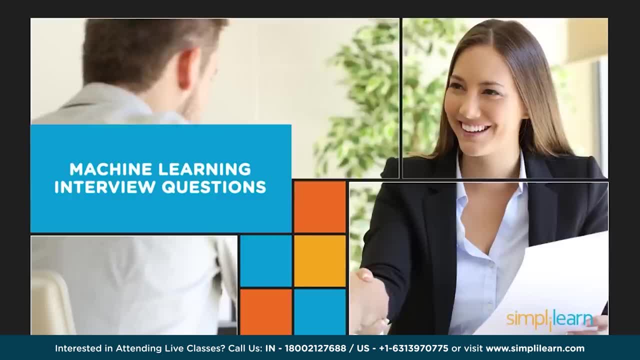 supplement your answers with your own experience. So the responses that we put here are a bit more generic in nature, so that if there are some concepts that you are not clear, this video will help you in kind of getting those concepts cleared up. But what is more important is that you need to supplement these responses with your own. 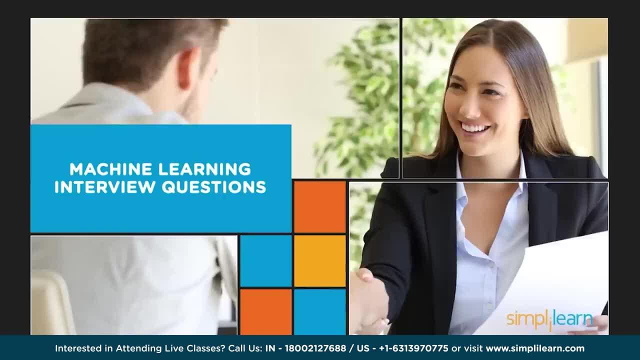 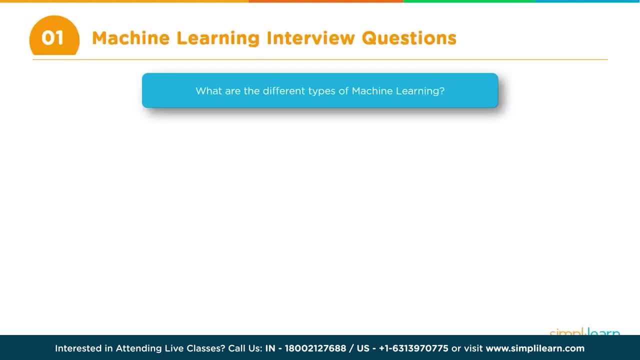 practical experience. So with that let's get started. So one of the first questions that you may face is: what are the different types of machine learning? Now, what is the best way to respond to this? There are three types of machine learning. if you read any material, you will always 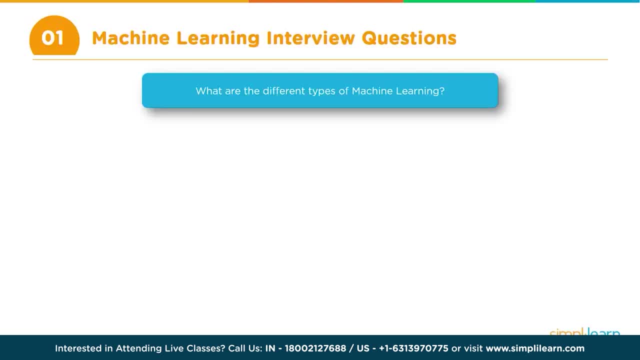 be told there are three types of machine learning, But what is important is, You would probably be better off emphasizing that there are actually two main types of machine learning, which is supervised and unsupervised, And then there is a third type, which is reinforcement learning. 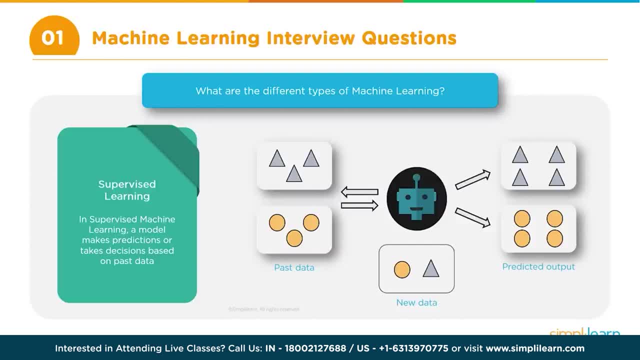 So supervised learning is where you have some historical data and then you feed that data to your model to learn. Now you need to be aware of a key word that they will be looking for, which is labeled data, Right, Right. So if you have some statistical data, the impact may not be so much. you need to emphasize. 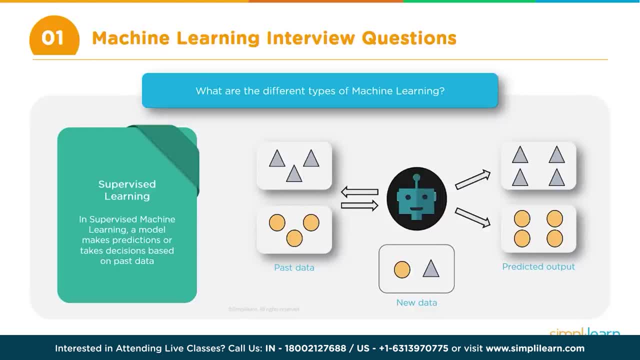 on labeled data. So what is labeled data Basically? let's say, if you're trying to do training model for classification, you need to be aware of all your existing data which class each of the observations belong to right. So that is what is labeling. 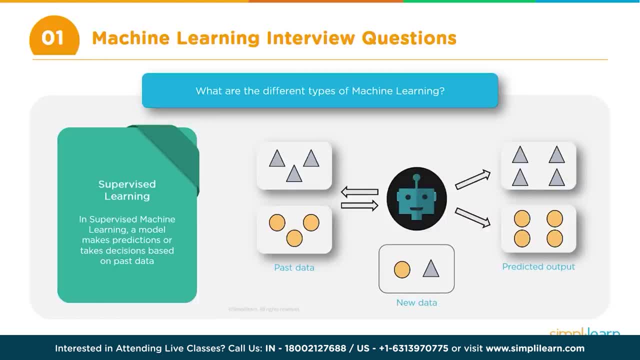 So it is nothing but a fancy name. you must be already aware, but just make it a point to throw in that keyword labeled, So that will have the right impact. Okay, So that is what is supervised learning: when you have existing labeled data which you 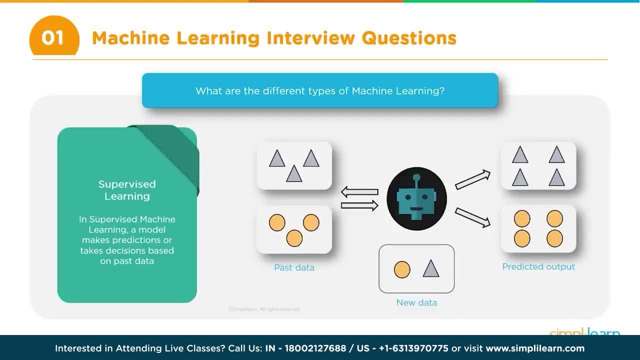 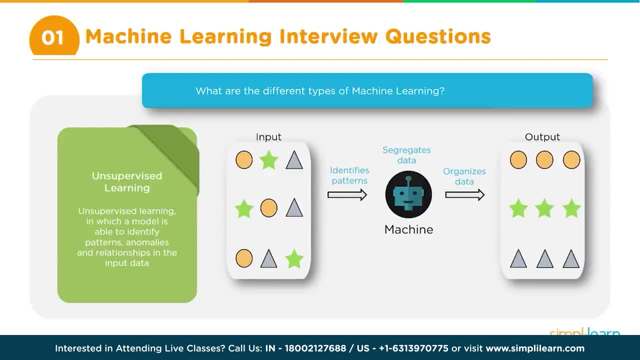 then use to train your model. that is known as supervised learning, And unsupervised learning is when you don't have this labeled data. So you have data. it is not labeled, So the system has to figure out a way to do some analysis on this. 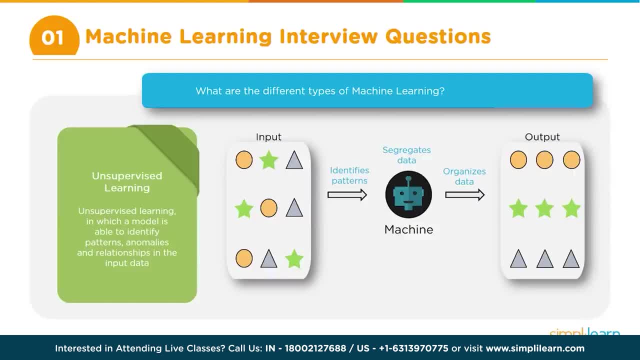 So that is unsupervised learning, And you can then add a few things like what, what are the ways of performing a supervised learning, Supervised learning and unsupervised learning, or what are some of the techniques? So supervised learning we perform or we do regression and classification, and unsupervised 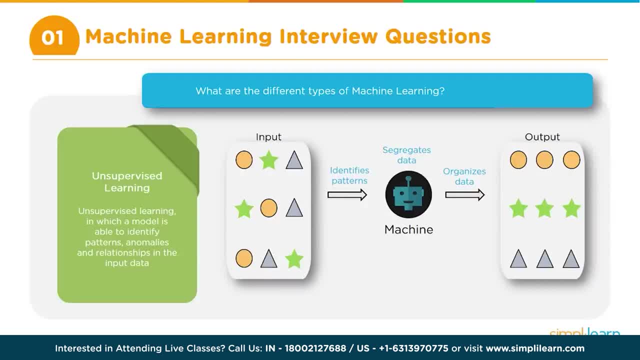 learning, We do clustering, and clustering can be of different types. Similarly, regression can be of different types. but you don't have to probably elaborate so much if they are asking for just the different types. you can just mention these, and just at a very high level. 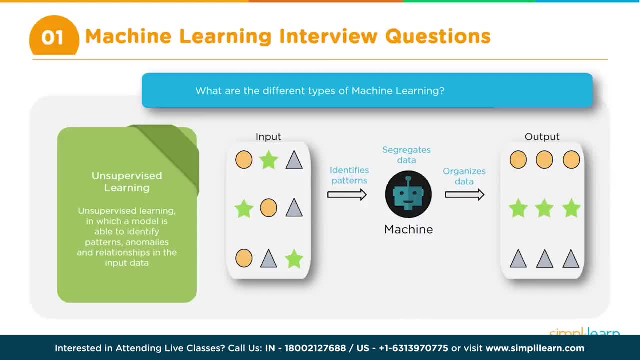 But if they want you to elaborate, give examples, then of course you can do it. So that is what is supervised learning. Okay, And of course I think there is a different question for that. We will see that later. Then the third: so we have supervised, then we have unsupervised, and then reinforcement. 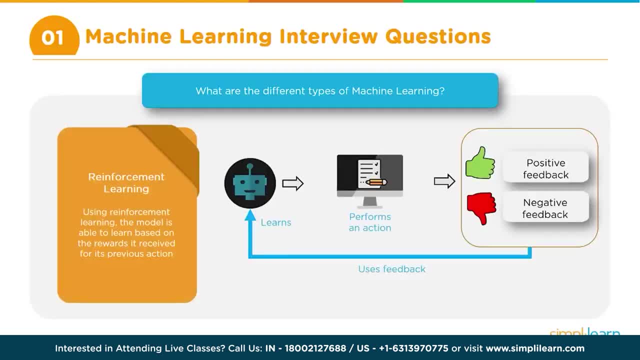 you need to provide a little bit of information around that as well, because it is sometimes a little difficult to come up with a good definition for reinforcement learning, So you may have to a little bit elaborate on how reinforcement learning works, right? So reinforcement learning works in such a way that it basically has two parts to it. 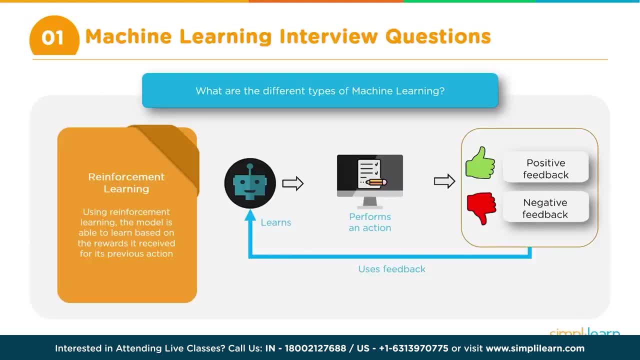 One is the agent and the environment. Okay, So the agent basically is working inside of this environment and it is given a target that it has to achieve and every time it is moving in the direction of the target. so the agent basically has to take some action and every time it takes an action which is 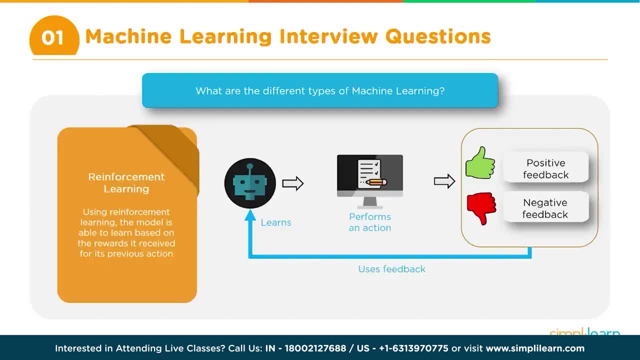 moving the agent towards the target, towards a goal- a target is nothing but a goal- then it is rewarded- Okay. And every time it is going in a direction where it is away from the goal: Okay. And every time it is going in a direction where it is away from the goal, then it is punished. 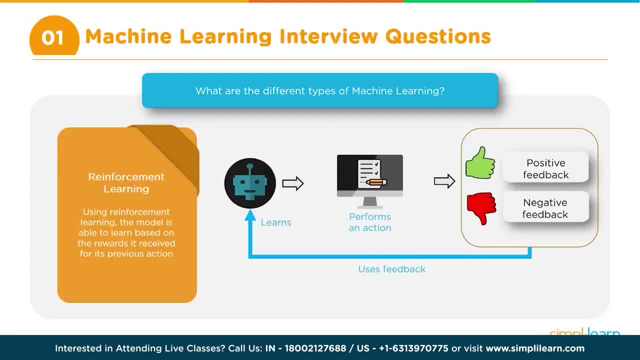 So that is the way you can a little bit explain. And this is used primarily or very, very impactful, or teaching the system to learn games and so on. Examples of this are basically used in AlphaGo- You can throw that as an example- where AlphaGo used reinforcement learning to actually learn. 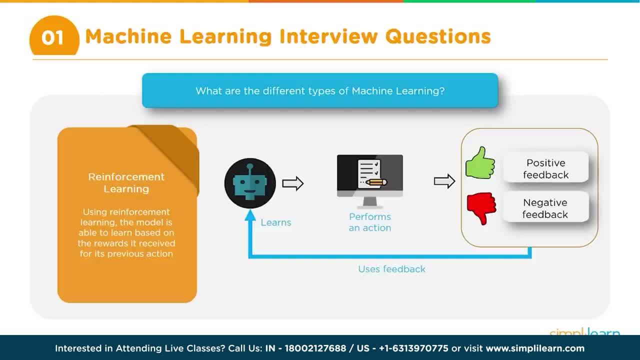 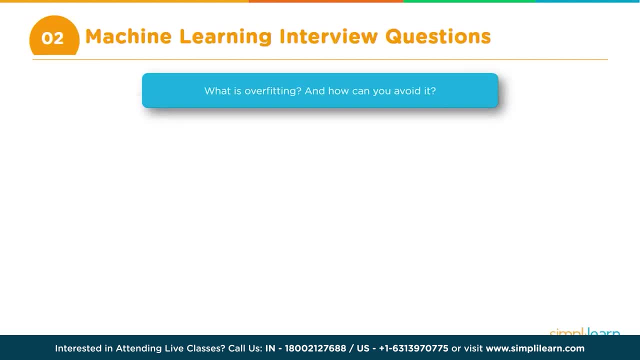 to play the game of Go and finally it defeated the Go world champion, Right? So there's a bunch of information that would be good enough. Okay, Then there could be a question on overfitting. So the question could be: what is overfitting and how can you avoid it? 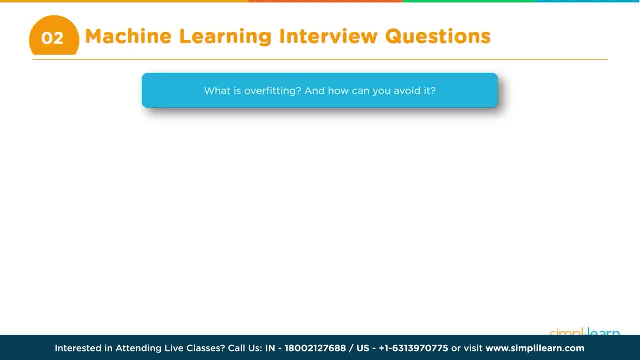 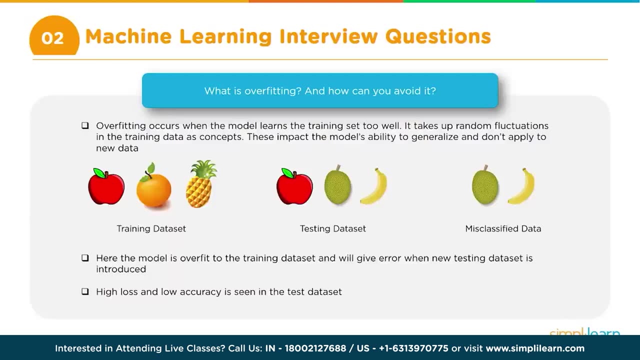 So what is overfitting? Let's first try to understand the concept, because sometimes overfitting may be a little difficult to understand. Overfitting is a situation where the model has kind of memorized the data. So this is an equivalent of memorizing the data. 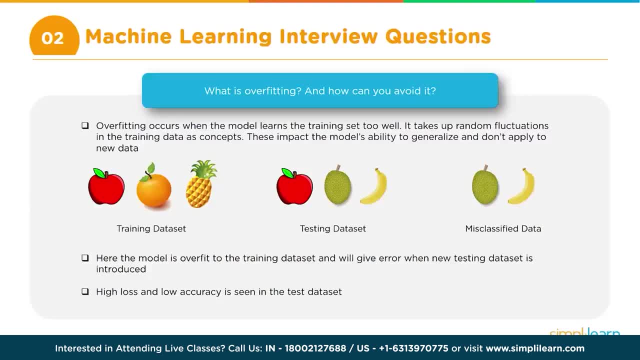 So This is an analogy, so that it becomes easy to explain this. Now, let's say you're teaching a child about recognizing some fruits or something like that. Okay, And you're teaching this child about recognizing, let's say, three fruits: apples, oranges and 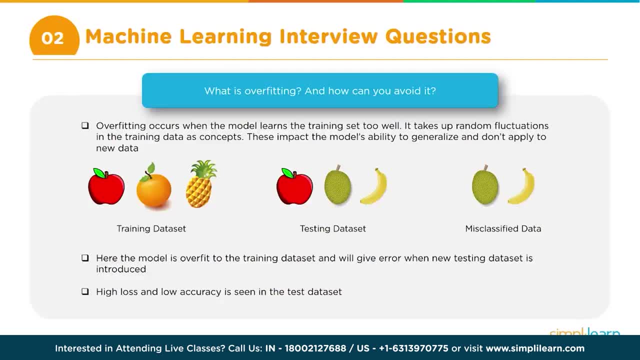 pineapples. Okay, So this is a small child And for the first time you're teaching the child to recognize fruits, then So what will happen? So this is very much like that is your training data set. So what you will do is you will take a basket of fruits which consists of apples, oranges, 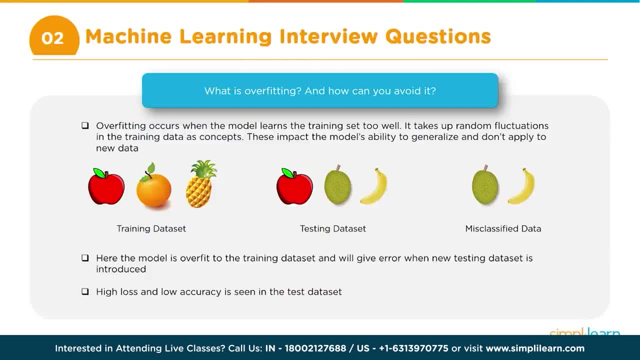 and pineapples, Okay, And you take this basket to this child and there may be, let's say, hundreds of these fruits. So you take this basket to this child and keep showing each of this fruit And then, first time, obviously, the child will not know what it is. 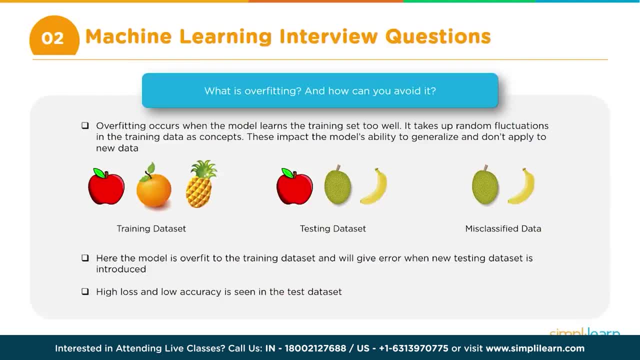 So you show an apple and you say: Hey, this is apple. Then you show maybe an orange and say: this is orange, and so on and so forth, And then again you keep repeating that, Right? So until that basket is over. 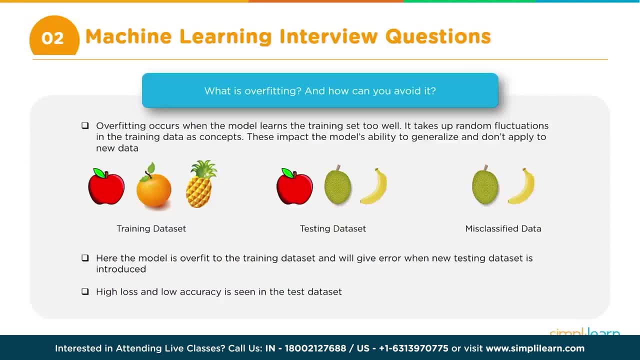 This is basically how In machine learning also. that's how training works. So till the basket is completed there may be a hundred fruits. You keep showing this child in the process What has happened. The child has pretty much memorized these. 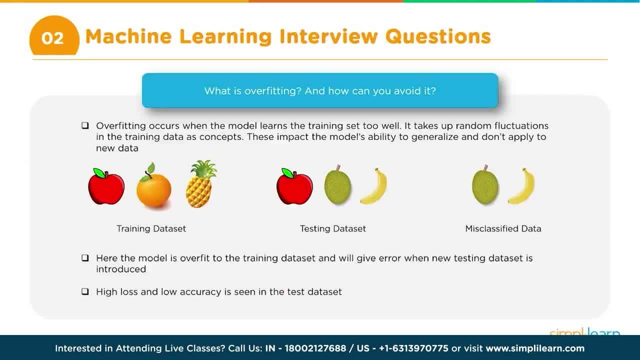 So even before you finish that basket right By the time you are halfway through, the child has learned about recognizing the apple, orange and pineapple. Now what will happen after? halfway through? initially you remember it made mistakes in recognizing, but halfway through now it has learned. 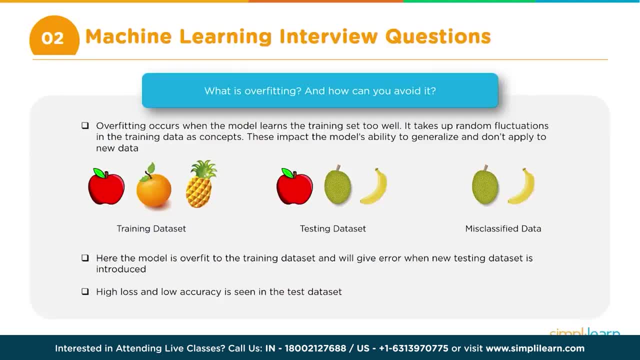 So every time you show a fruit, it will exactly a hundred percent accurately it will identify it. It will say: the child will say: this is an apple, this is an orange, And if you show a pineapple it will say: this is a pineapple, right. 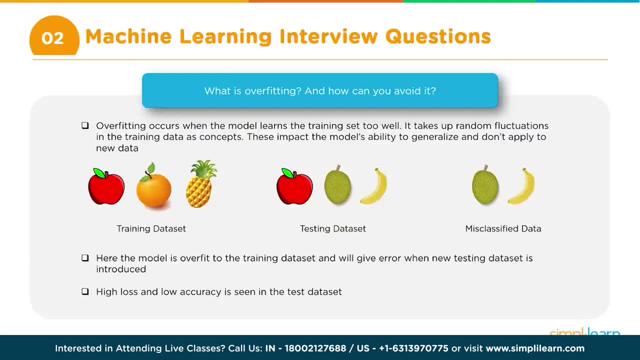 So that means it has kind of memorized this data. Now, let's say you bring another basket of fruits and it will have a mix of maybe apples, which were already there in the previous set, but it will also have in addition to apple. 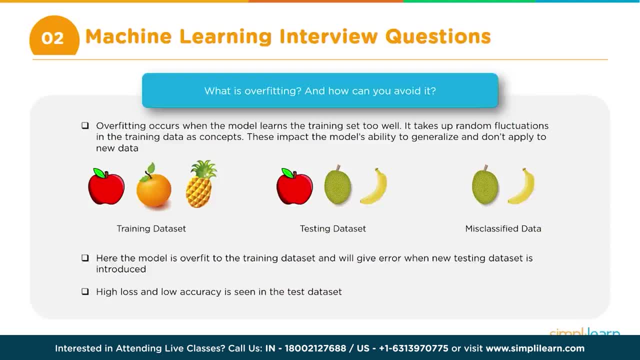 it will probably have a banana Or maybe another fruit like a jackfruit, right? So this is an equivalent of your test data set, which the child has not seen before. Some parts of it it probably has seen, like the apples it has seen, but this banana and 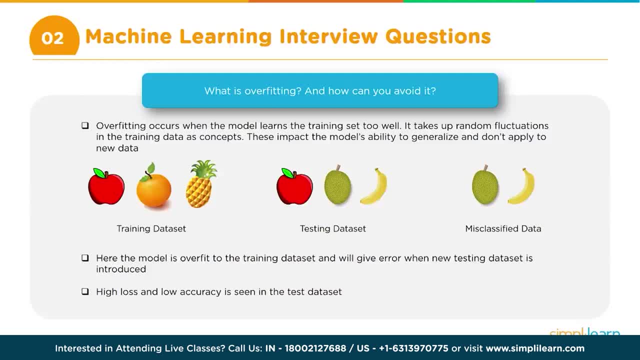 jackfruit it has not seen. So then what will happen in the first round, which is an equivalent of your training data set towards the end? it has a hundred percent. It was telling you what the fruits are. right, Apple was accurately recognized. 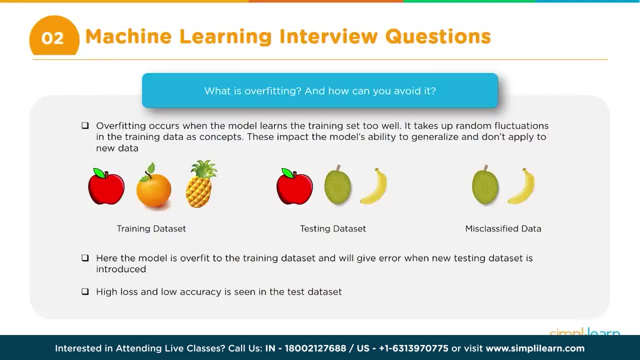 Orange was accurately recognized And pineapples were accurately recognized, Right. So that is like a hundred percent accuracy. But now, when you get another, a fresh set, which we're not a part of the original one, what will happen? All the apples maybe it will be able to recognize correctly, but all the others, like the jackfruit. 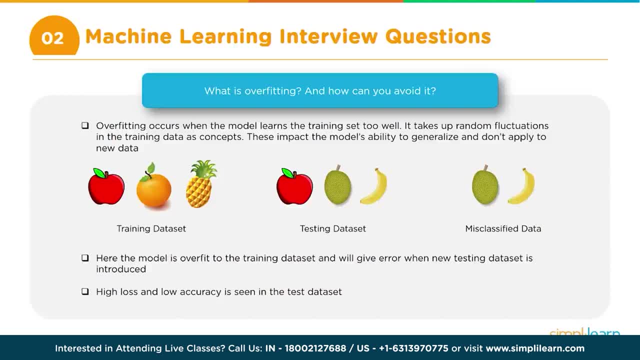 or the banana will not be recognized by the child, right? So this is an analogy. This is an equivalent of overfitting. So what has happened during the training process? It is able to recognize or reach a hundred percent accuracy, maybe very high accuracy. 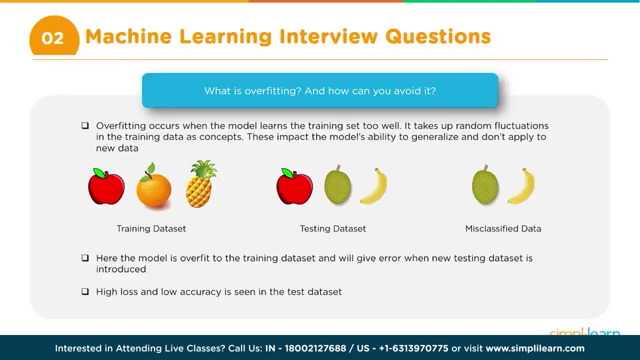 Okay, Or maybe very low loss, right? So that is the technical term. So the loss is pretty much zero and accuracy is pretty much a hundred percent, Whereas when you use testing there will be a huge error, which means the loss will be. 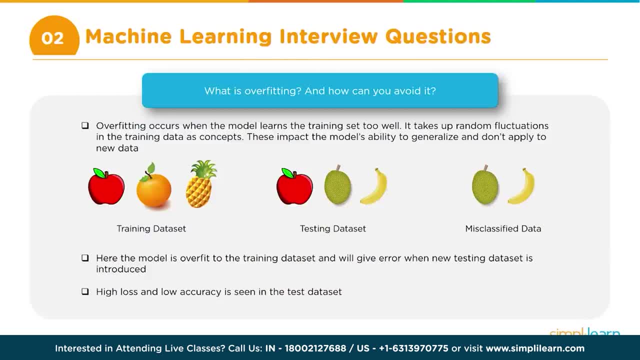 pretty high And therefore the accuracy will be also low. Okay, This is known as overfitting. This is basically a process where training is done. Training processes it goes very well, almost reaching a hundred percent accuracy, but while testing it really drops down. 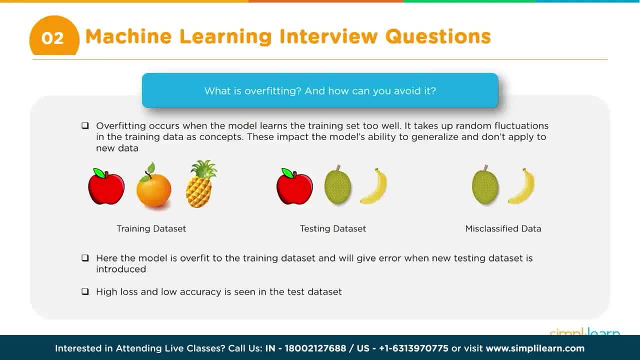 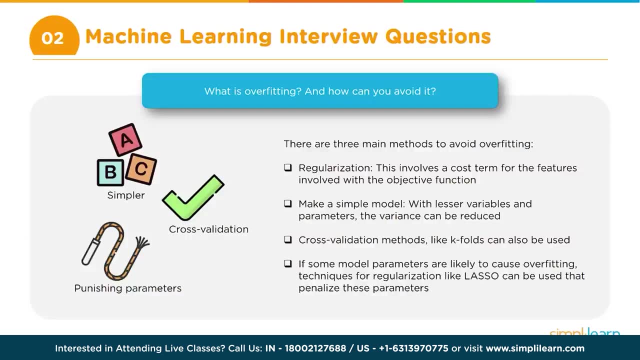 Now, how can you avoid it? So that is So, as an extension of this question, there are multiple ways of avoiding overfitting. There are techniques like what you call regularization. That is the most common technique that is used for avoiding overfitting. 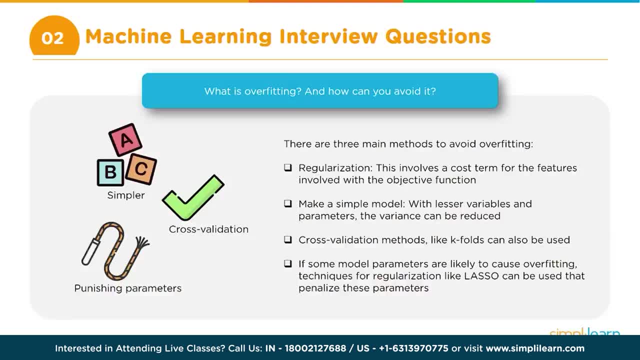 And within regularization there can be a few other subtypes, like dropout in case of neural networks and a few other examples. But I think if you give example or if you give regularization as the technique, probably that should be sufficient. So so there will be some questions where the interviewer will try to test your fundamentals. 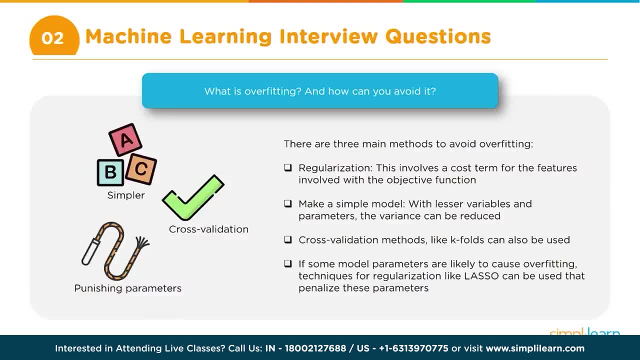 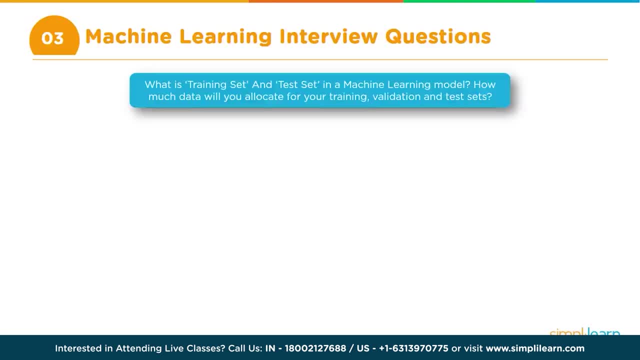 and your knowledge and depth of knowledge and so on and so forth, And then there will be some questions which are more like quick questions, that will be more to stump you. Okay, Then the next question is around the methodology. So when we are performing machine learning training, we split the data into training. 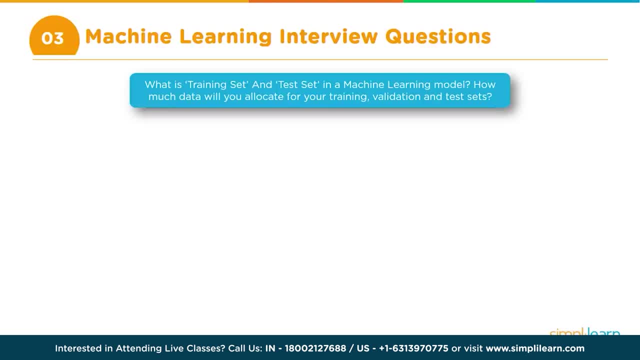 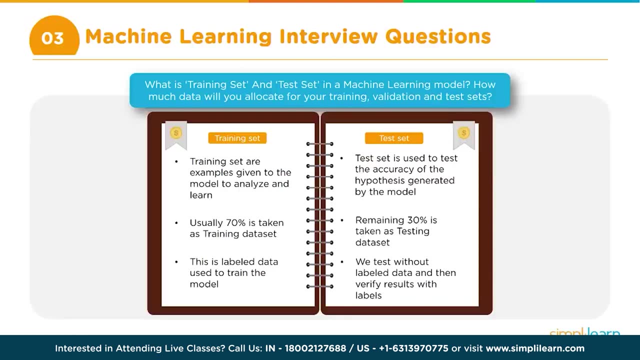 and tests, right. So this question is around that. So the question is: What is the training set and test set in machine learning model and how is the split done? So the question can be like that: So in machine learning, when we are trying to train the model, so we have a three step. 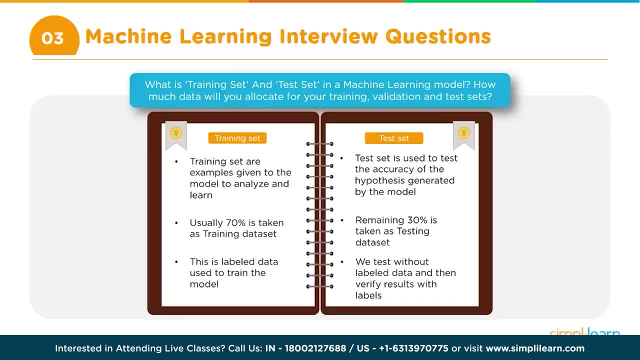 process. We train the model and then we test the model And then, once we are satisfied with the test, only then we deploy the model. So what happens in the train and test is that you remember the labeled data. So let's say you have. 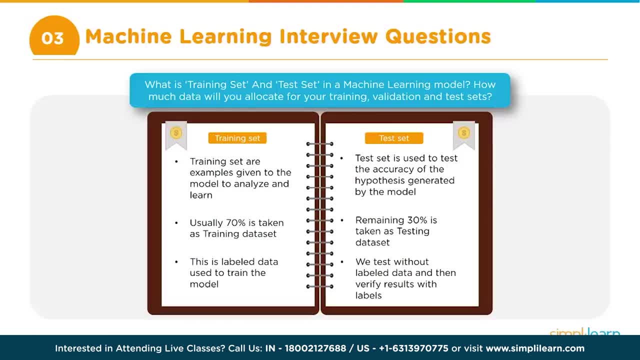 1000 records with labeling information. Now, one way of doing it is you use all the thousand records for training and then maybe right, which means that you have exposed all this thousand records during the training process, And then you take a small set of the same data and then you say, okay, I will test it. 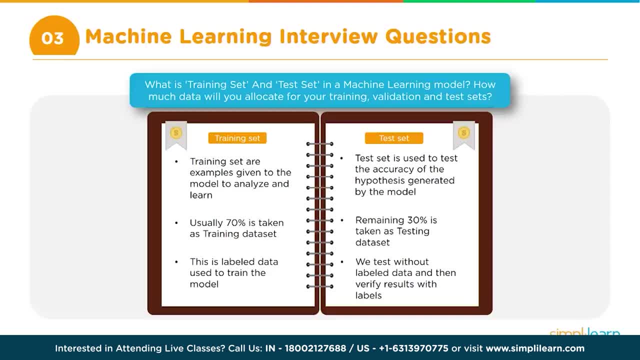 with this, Okay, And then you probably what will happen? You may get some good results right, But there is a flaw there. What is the flaw? This is very similar to human beings, It is. We are showing this model, the entire data, as a part of training. 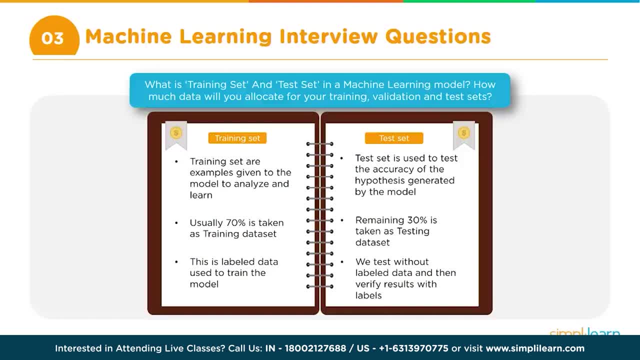 Okay, So obviously it has become familiar with the entire data. So when you're taking a part of that again and you're saying that I want to test it, obviously you will get good results. So that is not a very accurate way of testing. 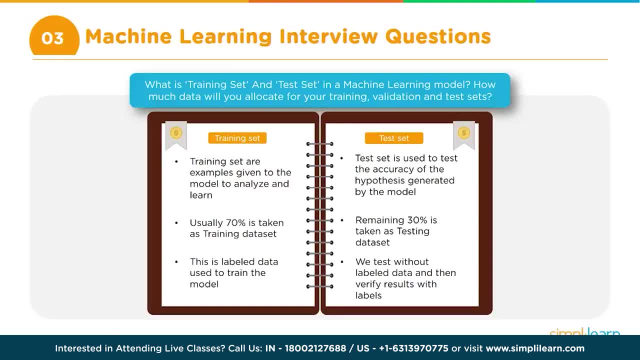 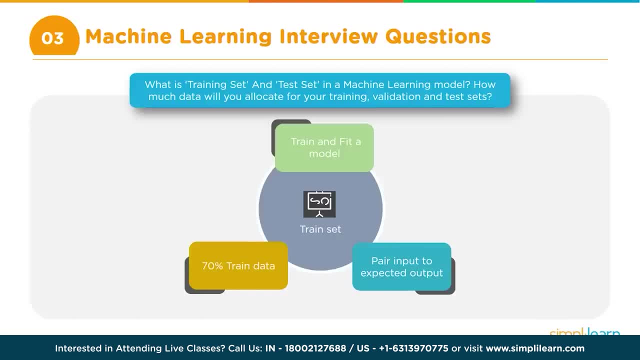 So that is the reason. what we do is we have the label data of this thousand records or whatever We set aside before starting the training process. we set aside a portion of that data. Okay, We call that test set and the remaining we call this training set. 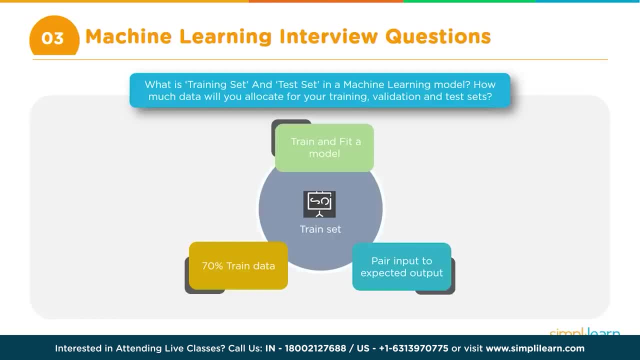 And we use only this for training, our model. Now, the training process, remember, is not just about asking one round of this data set. So let's say now your training set has 800 records. It is not just one time you pass this 800 records. 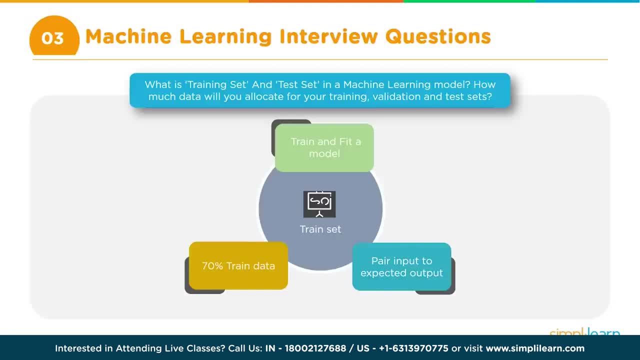 What you normally do is you actually, as a part of the training, you may ask this data through the model multiple times. So this thousand records may go through the model, Maybe 10,, 15,, 20 times, till the training is perfect, till the accuracy is high, till the 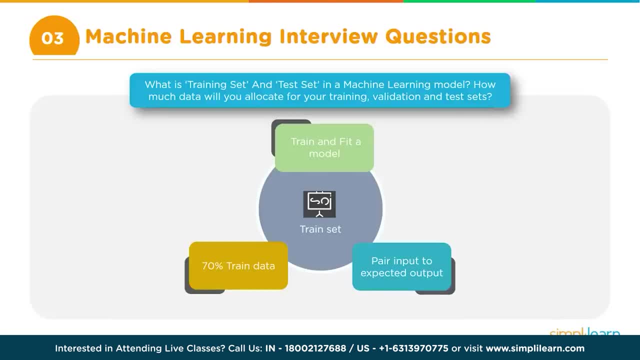 errors are minimized. Okay Now so, which is fine, which means that you are. that is what is known as the model has seen your data and gets familiar with your data. And now, when you bring your test data, what will happen is: this is like some new data. 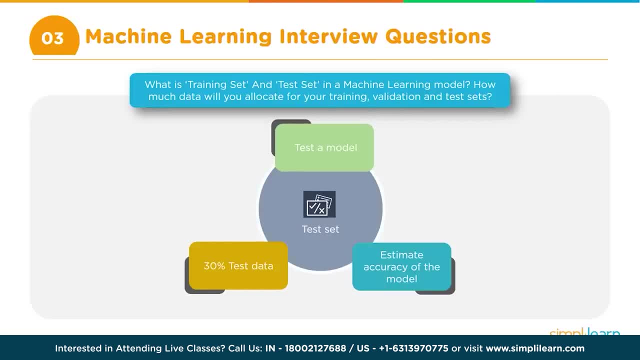 because that is where the real test is. Now you're trained the model and now you are testing the model with some data which is kind of new. That is like a situation. That like a realistic situation, because when the model is deployed, that is what will happen. 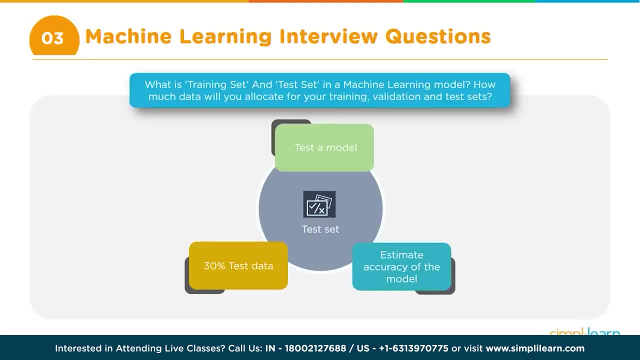 It will receive some new data, not the data that it has already seen, right. So this is a realistic test. So you put some new data. So this data which you have set aside is for the model. It is new And if it is able to accurately predict the values, that means your training has worked. 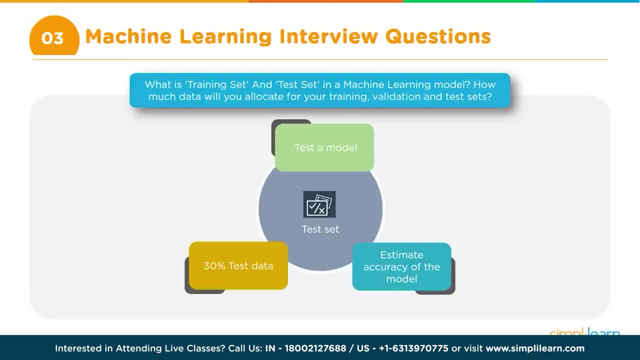 Okay, The model got trained properly. but, let's say, while you're testing this with this test data, you're getting a lot of errors. That means you need to probably either change your model Or retrain with more data and things like that. 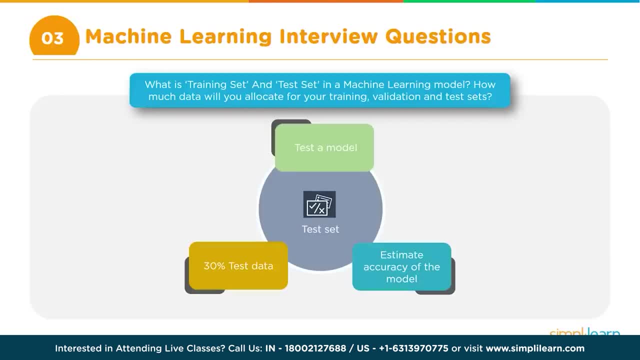 Now coming back to the question of how do you split this? What should be the ratio? There is no fixed number. again, This is like individual preferences. Some people split it into 50, 50,, 50% test and 50% training. 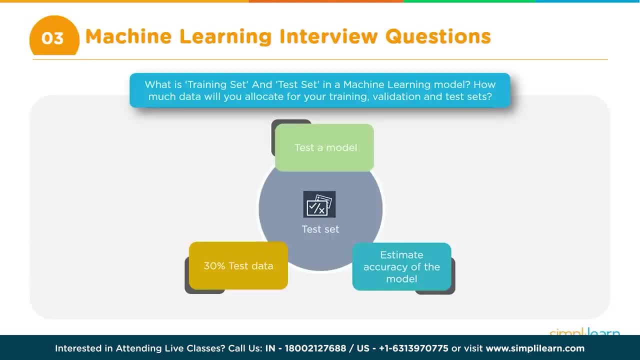 Some people prefer to have a larger amount for training and a smaller amount for test, So they can go by either 60, 40 or 70, 30, or some people even go with some odd numbers like 65, 35 or 63.33 and 33,, which is like one third and two thirds. 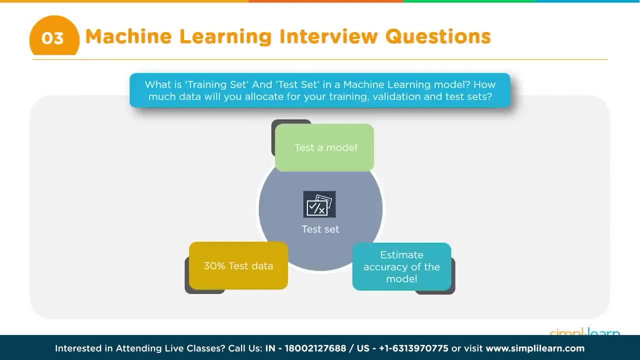 So there is no fixed rule that it has to be something. that ratio has to be this. You can go by your individual preferences, All right. Then you may have questions around data handling, data manipulation, or what do you call data management or preparation. 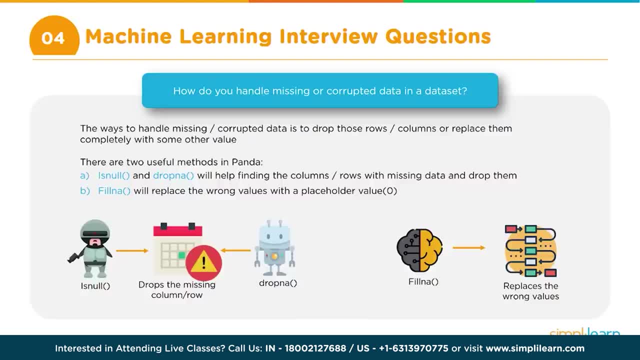 So these are all some questions around that area. There is, again, no one answer, one single good answer to this. It really varies from situation to situation and depending on what exactly is the problem, what kind of data it is, how critical it is, what kind of data is missing and what is the 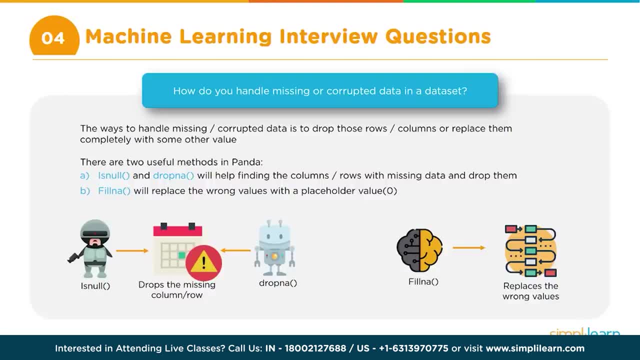 type of corruption. So there are a whole lot of things, which is a very generic question and therefore you need to be a little careful about responding to this as well. So probably have to illustrate this again, if you have experience in doing this kind. 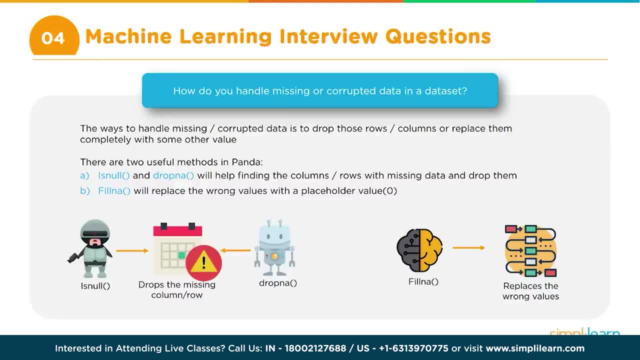 of work in handling data. you can illustrate with examples, saying that I was on one project where I received this kind of data. These were the columns where data was not filled, or these were the this many rows where the data was missing. That would be, in fact, a perfect way to respond to this question. 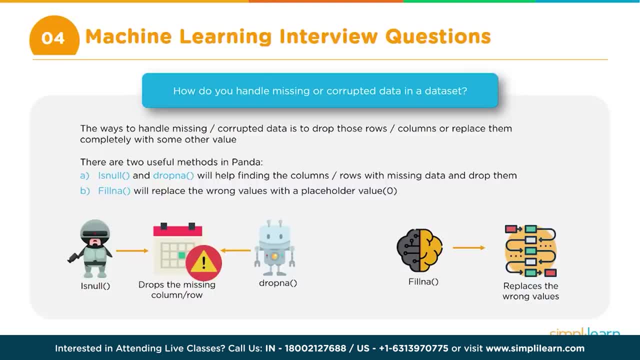 But if you don't have that, obviously you have to provide some good answer. I think it really depends on what exactly the situation is, And there are multiple ways of handling the missing data or corrupt data. Now let's take a few examples. 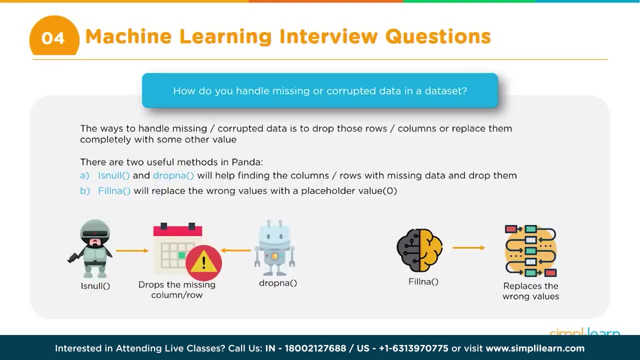 Now, let's say you have data where, Okay, The values in some of the columns are missing and you have pretty much half of your data having these missing values in terms of number of rows. Okay, That could be one situation. Another situation could be that you have records or data missing. but when you do some initial 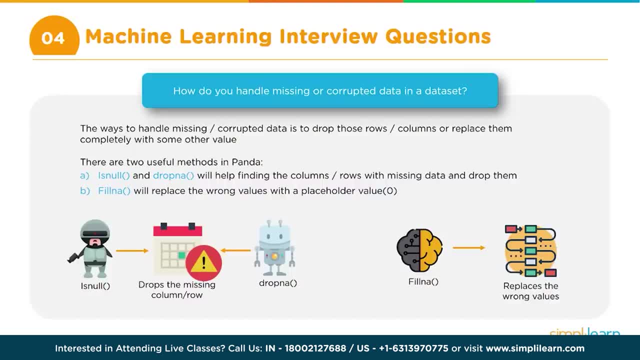 calculation how many records are corrupt, or how many rows or observations, as we call it, has this missing data? Let's assume it is very minimal, like 10%. Okay, Now, between these two cases, how do you So? let's assume that this is not a mission critical situation. 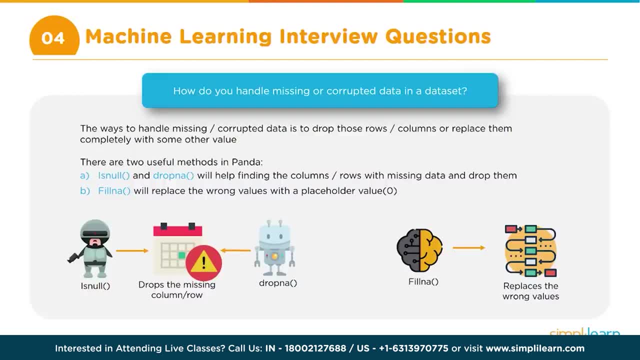 And in order to fix this 10% of the data, the effort that is required is much higher, And obviously effort means also time and money, right? So it is not so mission critical and it is okay to, let's say, get rid of these records. 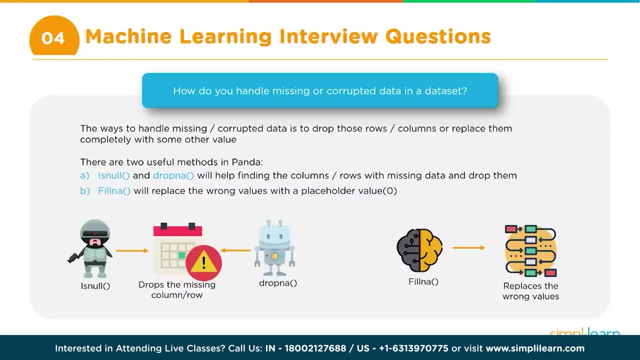 So obviously one of the easiest ways of handling the data part or missing data is remove those records or remove those observations from your analysis. Okay, So that is the easiest way to do, But then the downside is, as I said in, as in the first case, if, let's say, 50% of your 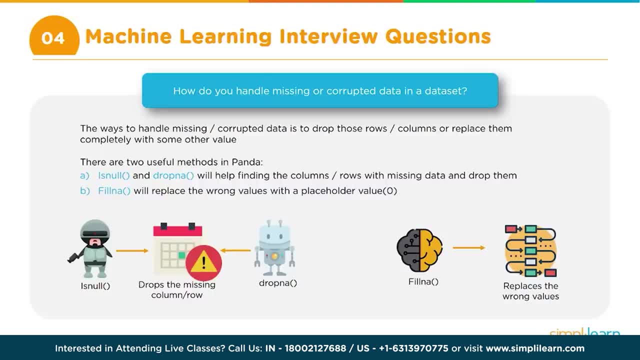 data is like that, because some column or the other is missing, So it is not like every in every place in every row, the same column is missing. but you have in maybe 10% of the records column one is missing and another 10%- column two. 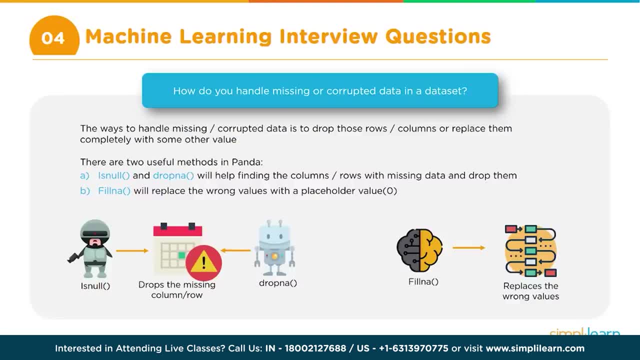 is missing, another 10%. column three is missing, and so on and so forth. So it adds up to maybe half of your data set. So you cannot completely remove half of your data set. Then the whole purpose is lost. Okay, So then how do you handle? 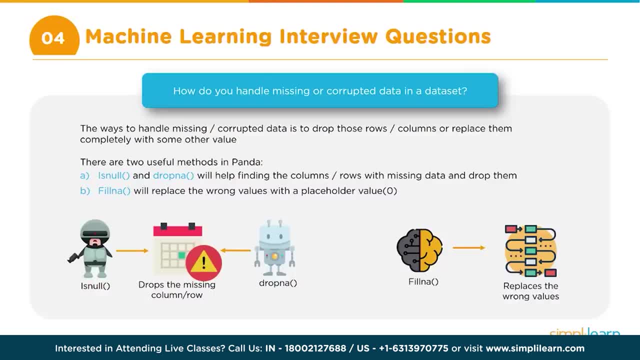 Then you need to come up with ways of filling up this data with some meaningful value. right, That is one way of handling. So when we say meaningful value, what is that meaningful value? Let's say, for a particular column. you might want to take a mean value for that column. 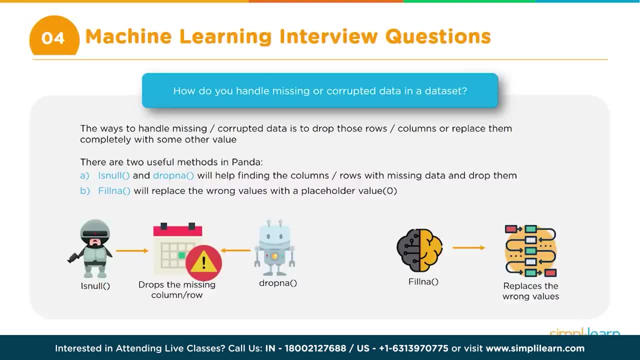 and fill wherever the data is missing. fill up with that mean value So that when you're doing the calculations your analysis is not completely way off. So you have values which are not missing. First of all, Your system will work. Number two: these values are not so completely out of whack that your whole analysis goes. 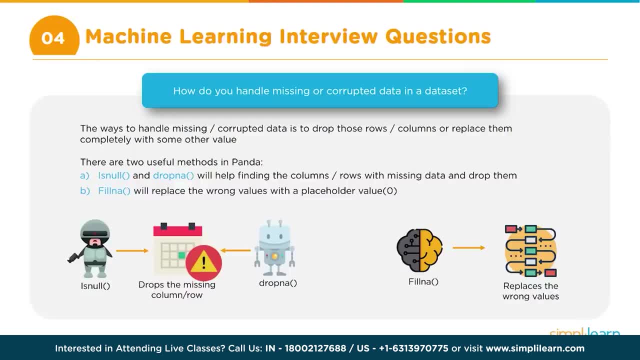 for a toss right. There may be situations where, if the missing values, instead of putting, mean maybe a good idea to fill it up with the minimum value or with a zero. So on with the maximum value again. as I said, there are so many possibilities. 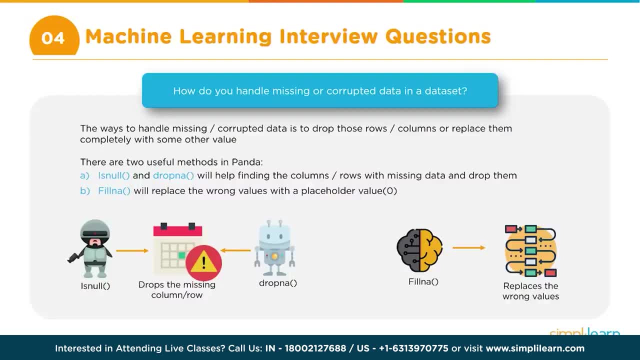 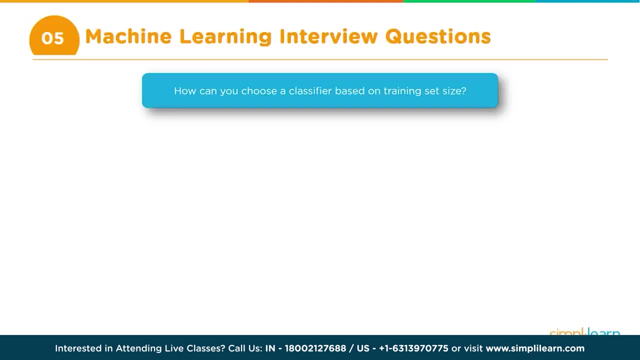 So there is no like one correct answer for this. You need to basically talk around this and illustrate with your experience, As I said, that would be the best. Otherwise, this is how you need to handle this question. Okay, So then the next question can be: how can you choose a classifier based on a training? 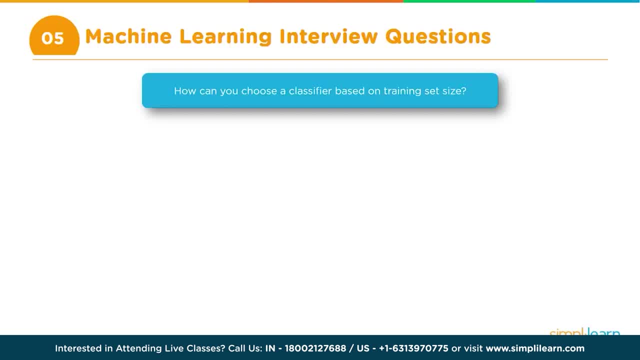 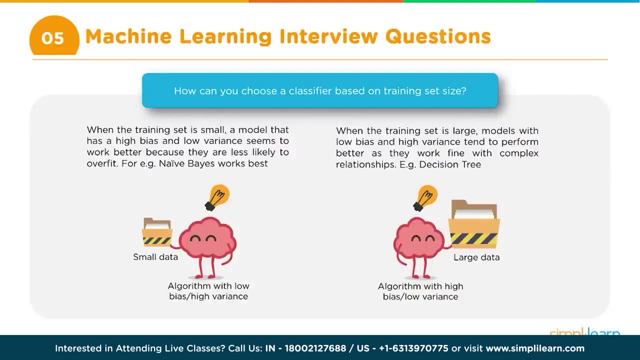 set data size. So, again, this is one of those questions where you probably do not have like a one size fits all answer. First of all, you may not, let's say, decide your classifier based on the training set size. Maybe not the best way to decide the type of the classifier. 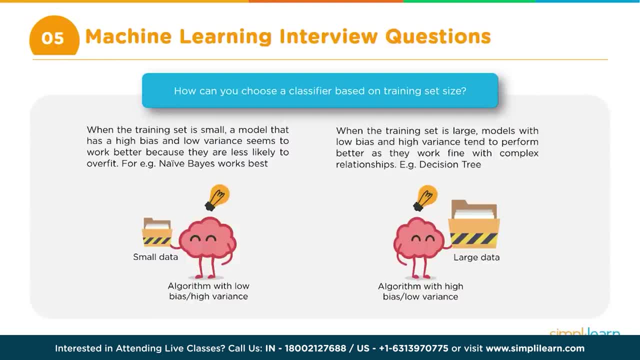 Okay, And even if you have to, there are probably some thumb rules which we can use, But then again every time. so, in my opinion, the best way to respond to this question is: you need to try out a few classifiers, irrespective of the size of the data, and you need to then. 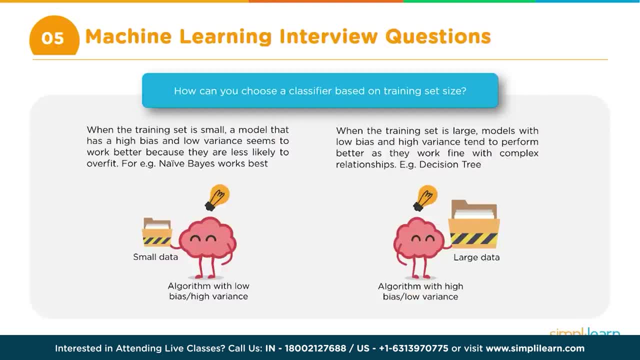 decide on your particular situation which of these classifiers are the right ones. This is a very generic issue, So you will never be able to just by if somebody defines a problem to you and somebody, even if they show the data to you or tell you what is the data or even the size of the data. 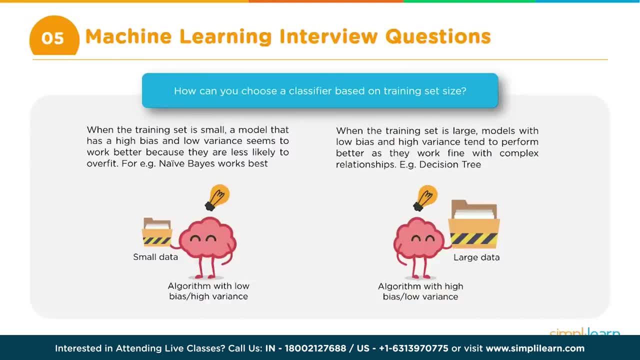 I don't think there is a way to really say that, yes, this is the classifier that will work here. No, that's not the right way, So you need to still, you know, test it out, get the data, try out a couple of classifiers. 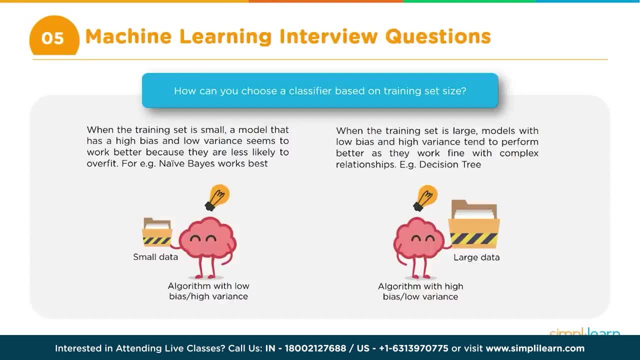 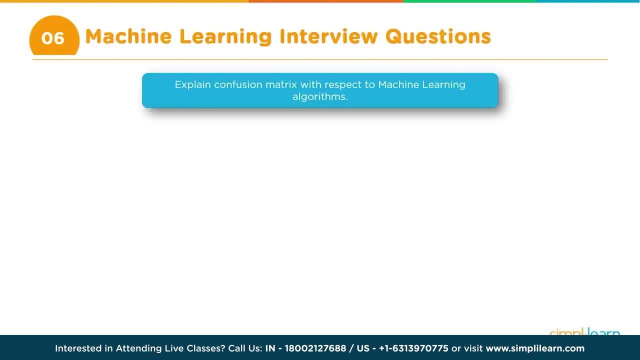 and then only you will be in a position to decide which classifier to use. You try out multiple classifiers, see which one gives the best accuracy, and only then you can decide. Okay, So let's move around Confucian matrix, So the question can be explained. Confucian matrix, right? 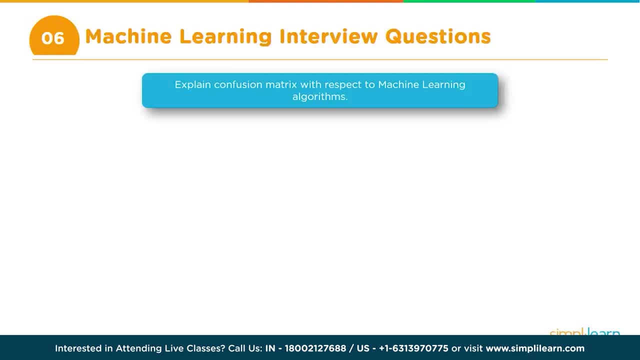 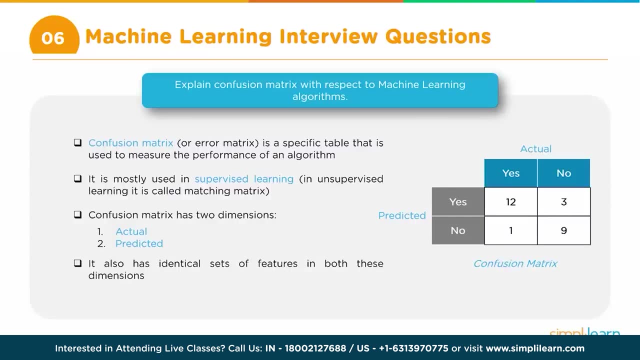 So Confucian matrix. I think the best way to explain it is by taking an example and drawing like a small diagram. otherwise it can really become tricky. So my suggestion is to take a piece of pen and paper and explain it by drawing a small. 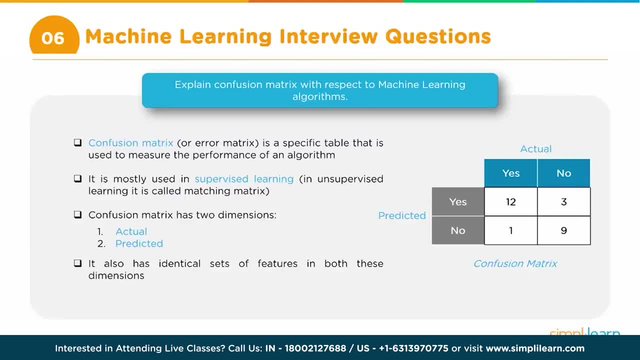 matrix And Confucian matrix is about to find out. this is used especially in classification learning process And when you get the results, when the model predicts the results, you compare it with the actual value and try to find out what is the accuracy. okay, 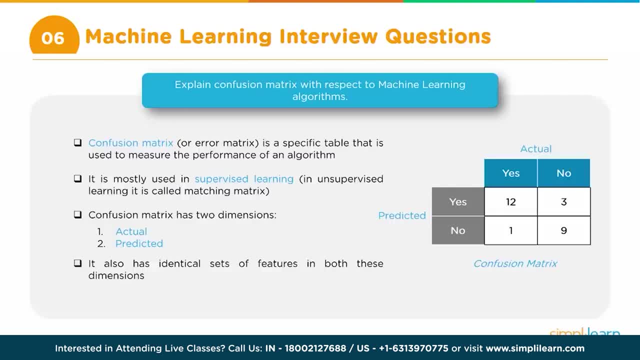 So in this case, let's say this is an example of a Confucian matrix and it is a binary matrix. So you have the actual values, which is the labeled data right And which is so you have how many yes and how many no. so you have that information. 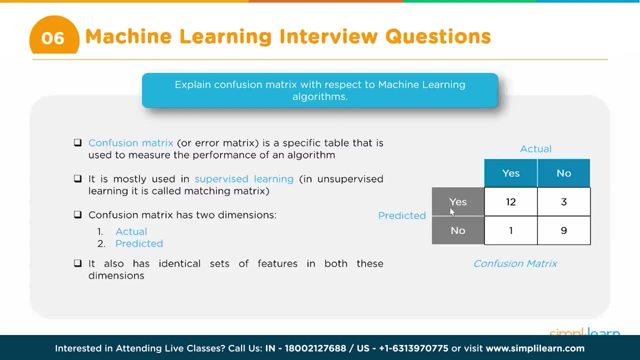 and you have the predicted values. Okay, How many yes and how many no? right? So the total actual values: the total yes is 12 plus 1, 13,, and they are shown here. And the actual value no's are 9 plus 3, 12,. okay, 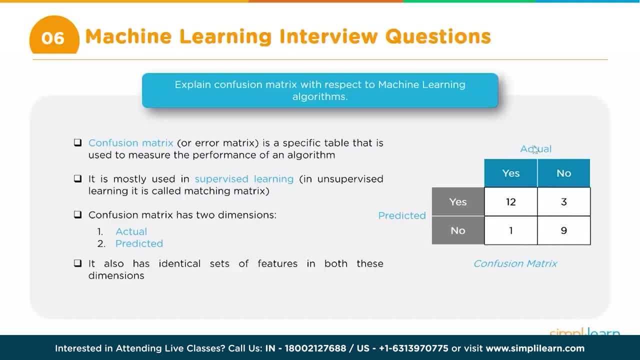 So that is what this information here is. So this is about the actual and this is about the predicted. Similarly, the predicted values there are: yes are 12 plus 3, 15 yeses and no are 1 plus 9, 10 no's. okay, 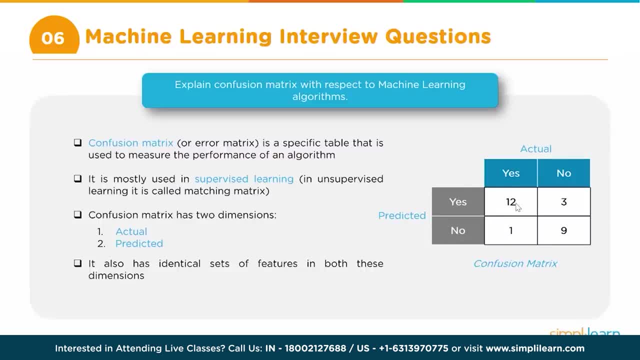 So this is the way to look at this Confucian matrix. Okay, And out of this, what is the meaning conveyed here? So there are two or three things that needs to be explained outright. The first thing is for a model to be accurate, the values across the diagonal should be high. 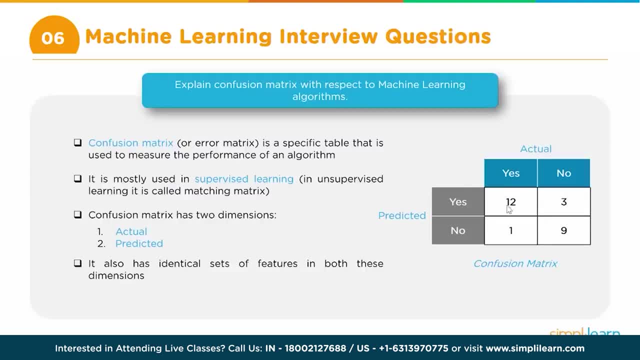 like in this case. right, That is one Number two. the total sum of these values is equal to the total observations in the test data set. So in this case, for example, you have 12 plus 3, 15 plus 10, 25, so that means we have 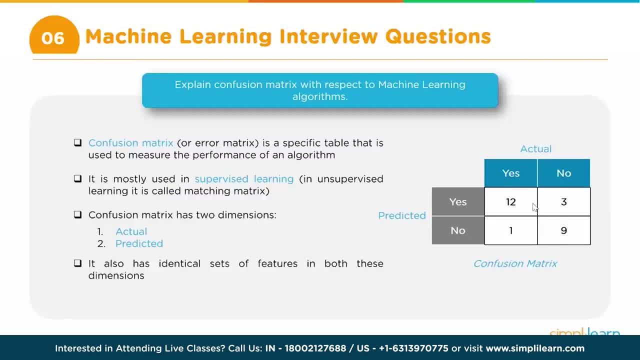 25 observations in our test data. Okay, So these are the two things. you need to first explain that the total sum in this matrix, the numbers, is equal to the size of the test data set and the diagonal values indicate the accuracy. So by just by looking at it, you can probably have a idea about is this an accurate model? 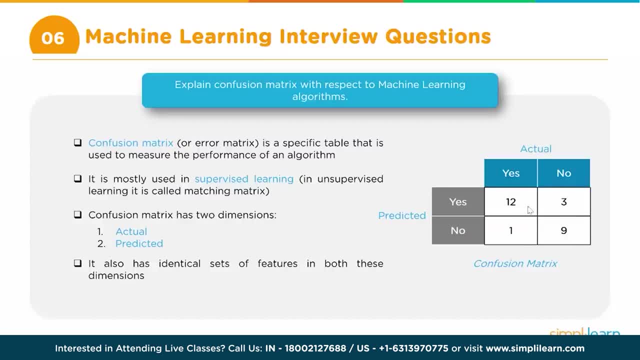 Is the model being accurate If they're all spread out equally in all these four boxes, that means probably the accuracy is not very good. Okay, So how do you calculate the accuracy itself? right, How do you calculate the accuracy itself? So it is a very simple mathematical calculation. 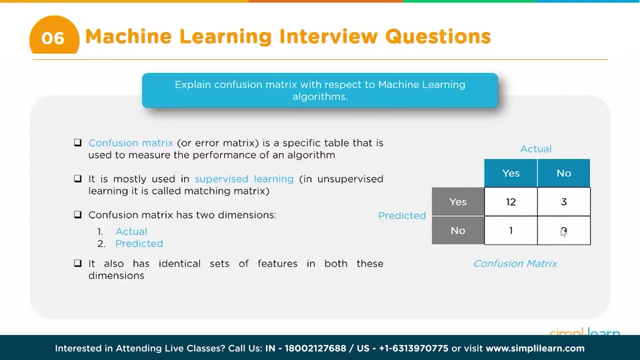 You take some of the diagonals right. So in this case, it is nine plus 12, 21, and divide it by the total. So in this case, what will it be? Let's me take a pen. So your, your diagonal values is equal to. if I say D is equal to 12 plus nine. 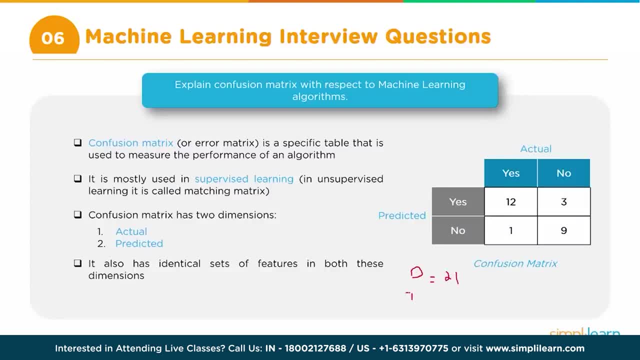 So that is 21,, right, And the total data set is equal to right. We just called it. Okay, We just calculated it is 25.. So what is your accuracy? It is 21 by your accuracy is equal to 21 by 25.. 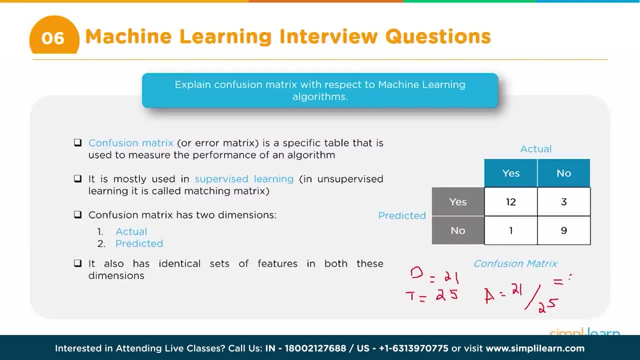 And this turns out to be about 85%, right? So this is 85%. So that is our accuracy. Okay, So this is the way you need to explain draw diagram. give an example, and maybe it may be a good idea to be prepared with an example so that it becomes easy for you. 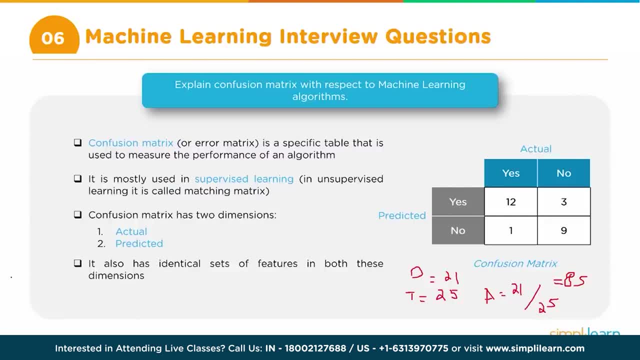 You don't have to calculate those numbers on the fly, Right? So a couple of uh hints are that you take some numbers which are with, which add up to a hundred. That is always a good idea, So you don't have to really do this complex calculations. 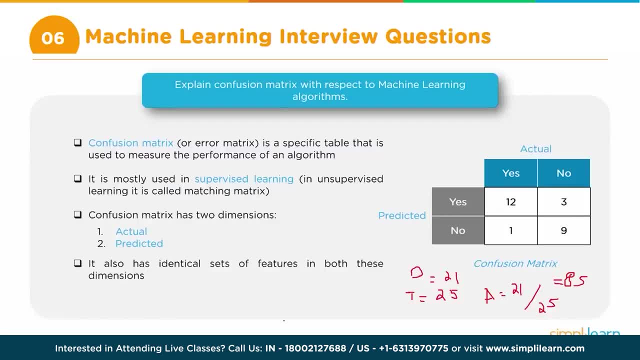 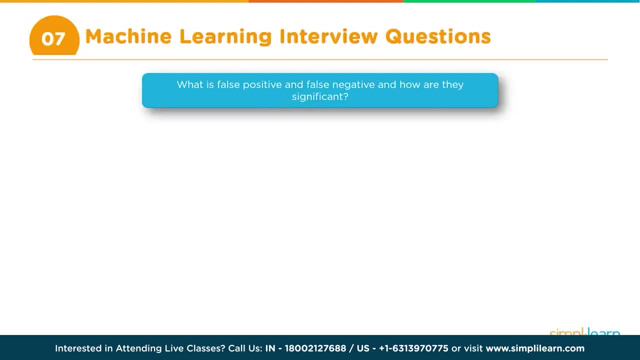 So the total value will be a hundred and then diagonal values. you divide. once you find the diagonal values, that is equal to your percentage. Okay, All right. So the next question can be a related question about false positive and false negative. So what is false positive and what is false negative? 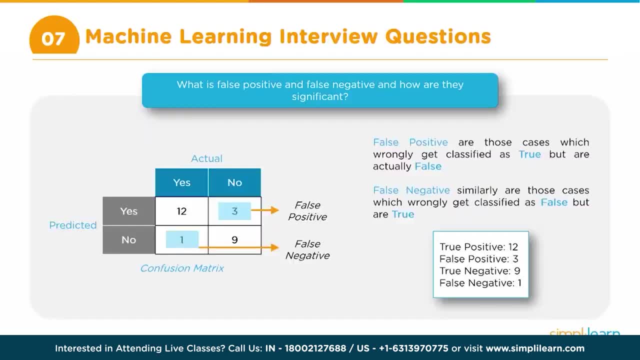 Now, once again, the best way to explain this is using a piece of paper. Okay, A piece of paper and pen, otherwise it will be pretty difficult to explain this. So we use the same example of the confusion matrix and, uh, we can explain that. 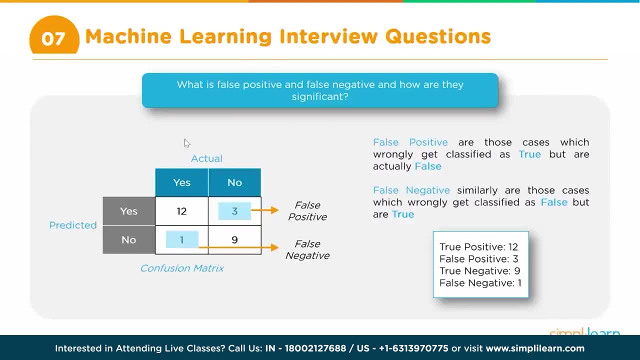 So a confusion matrix looks somewhat like this and, um, when we just take a yeah, it looks somewhat like this. and we continue with the previous example, where this is the actual value, This is the predicted value And, uh, in the actual value we have 12 plus one 13.. 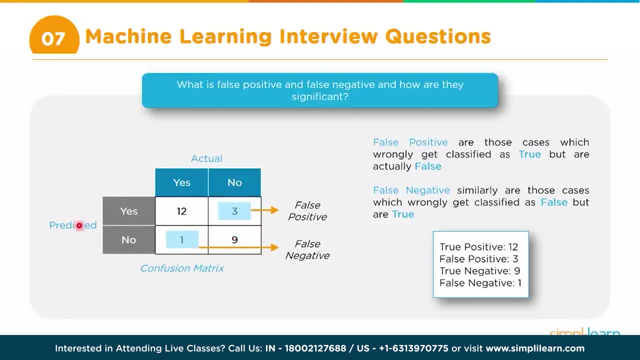 Yes, And three plus nine, 12 knows, and the predicted values there are 12 plus three, 15 yeses, and a one plus nine, 10 knows. Okay, Now this particular case, which is the false positive. what is a false positive? 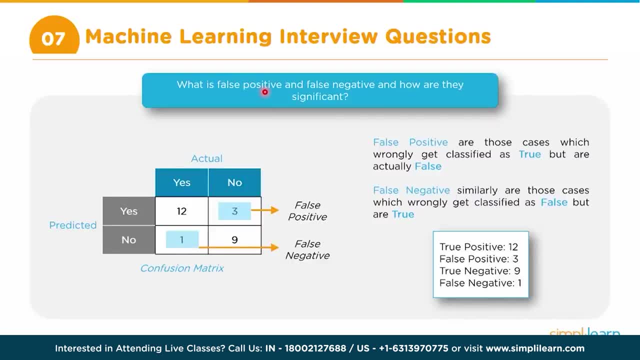 First of all, the second word, which is positive, okay, is referring to the predicted value. So that means the system has predicted it as a positive, but the real value? so this is what The false comes from, but the real value is not positive. 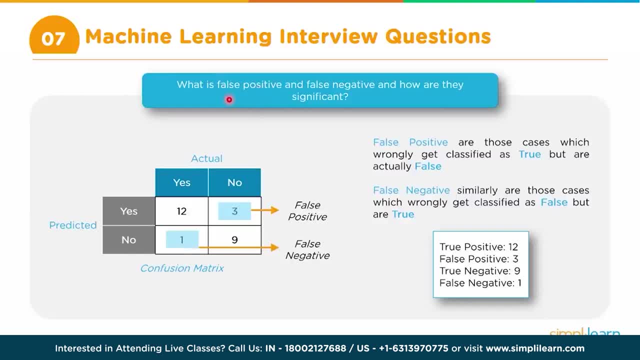 Okay, That is the way you should understand this term: false positive or even false negative. So false positive, So positive is what your system has predicted. So where is that system predicted? This is the one. positive is what? Yes, So you basically consider this row. 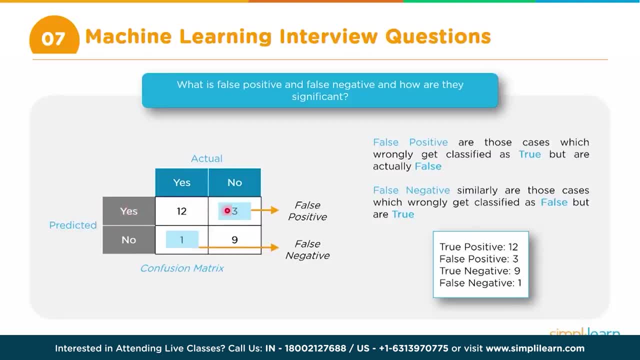 Okay, Now, if you consider this row, so this is, this is all positive values. This entire row is positive values. Okay, Now, the false positive is the one with where the value Okay, The actual value is negative. predicted value is positive, but the actual value is negative. 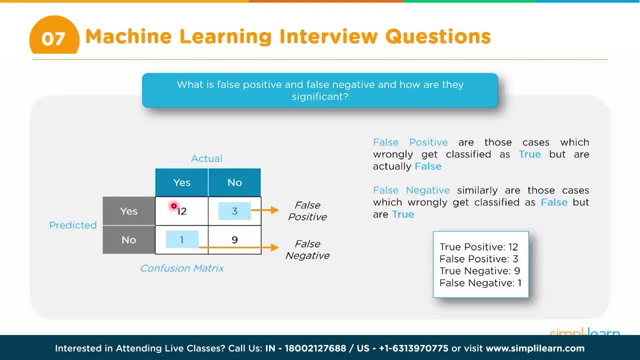 So this is a false positive right, And here is a true positive. So the predicted value is positive and the actual value is also positive. Okay, I hope this is making sense. Now let's take a look at what is false negative, false negative. 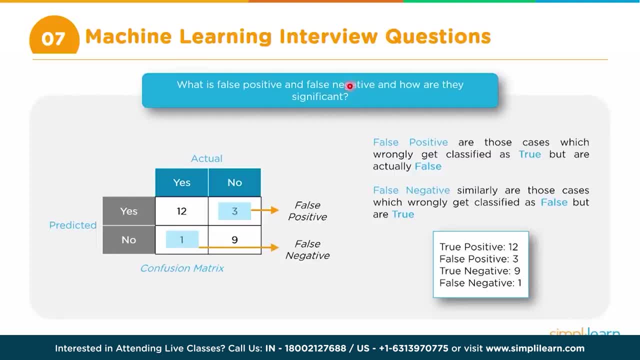 So negative is the second term. That means that is the predicted value that we need to look for. So which are the predicted negative values? This row corresponds to predicted negative values. All right, So this row corresponds to predicted negative values and what they're asking for: false. 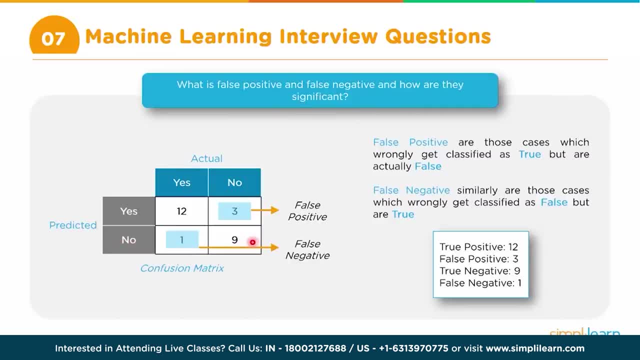 So this is the row for predicted negative values and the actual value is this one right. This is predicted negative and the actual value is also negative. Therefore, this is a true negative. So the false negative is this one predicted is negative but actually is positive right. 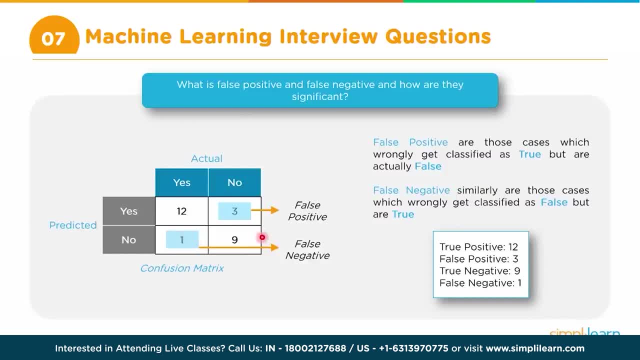 So this is the false negative. So this is the way to explain, And this is the way to explain. This is the way to look at false positive and false negative. Same way, there can be true positive and true negative as well. So, again, positive, the second term you need to use to identify the predicted row, right. 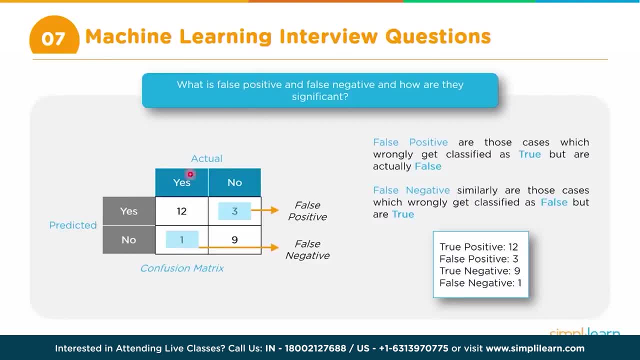 So if we say true, positive, positive you need to take for the predicted part. So predicted positive is here Okay. And then the first term is for the actual. So true, positive, So true. in case of actual is yes, Right. 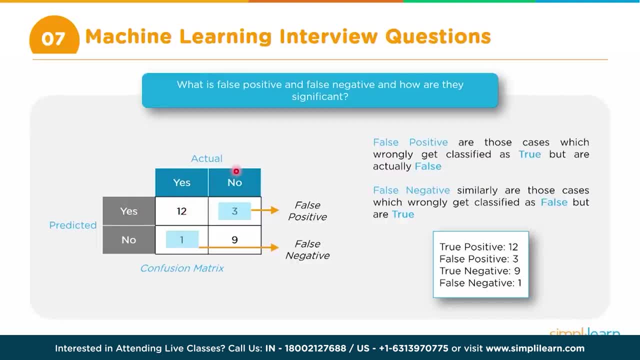 So true, positive is this one, Okay. And then, in case of actual the negative now we are talking about, let's say true, negative, true, negative, negative is this one and the true comes from here. So this is true, negative, right. 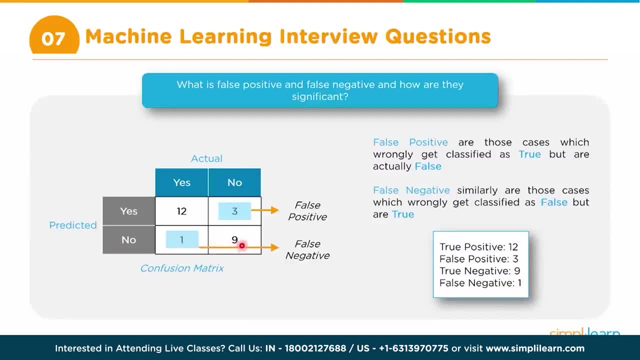 Nine is true, negative, The actual value is also negative and the predicted value is also negative. Okay, So that is the way you need to explain this: the terms false positive, false negative and true positive, true, negative. Then you might have a question like: what are the steps? 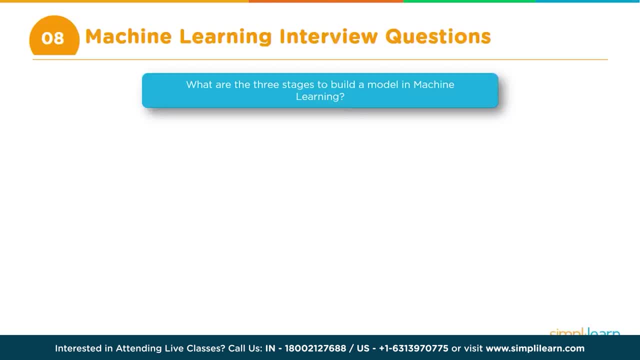 Okay, What are the steps involved in the machine learning process, or what are the three steps in the process of developing a machine learning model? right, So it is around the methodology that is applied. So basically, the way you can probably answer in your own words, but the way the model development, 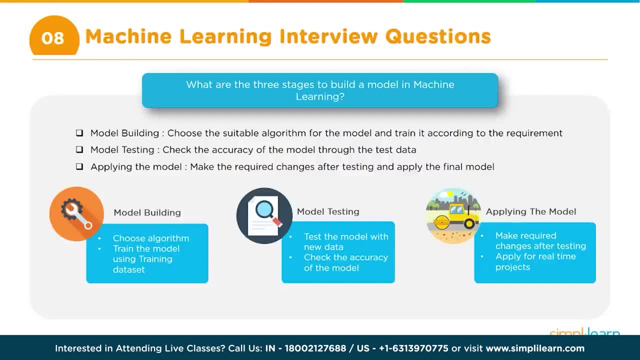 of the machine learning model happens is like this. So first of all, you try to understand the problem and try to figure out whether it is a classification problem or a regression problem. Based on that, you select a few- Okay, You select a few algorithms and then you start the process of training these models. 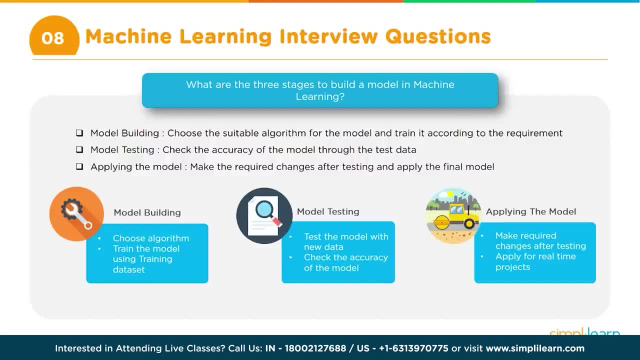 Okay. So you can either do that or you can. after due diligence, you can probably decide that there is one particular algorithm, that which is most suitable. Usually it happens through trial and error process, but at some point you will decide that, okay, this is the model we are going to use. 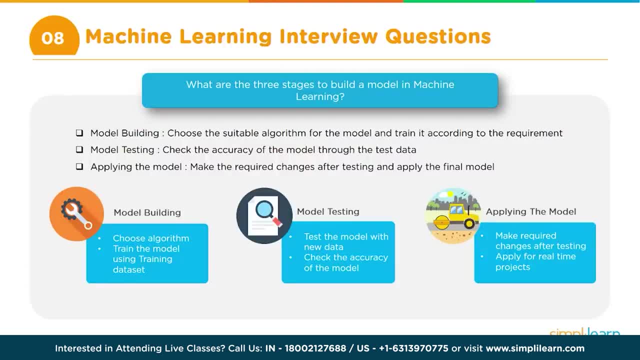 Okay, So in that case we have the model algorithm and the model decided and then you need to do the process Of training the model and testing the model, And this is where, if it is supervised learning, you split your data, the label data, into training. 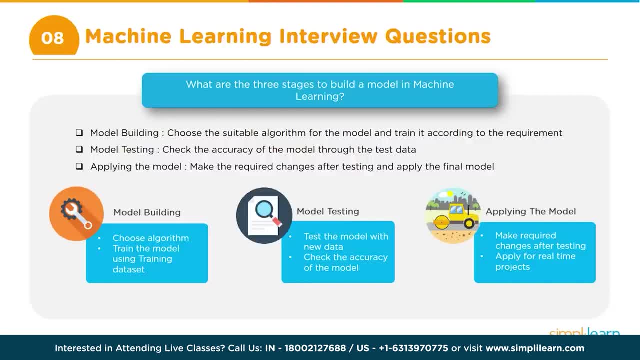 data set and test data set and you use the training data set to train your model And then you use the test data set to check the accuracy, whether it is working fine or not. So you test the model before you actually put it into production, right? 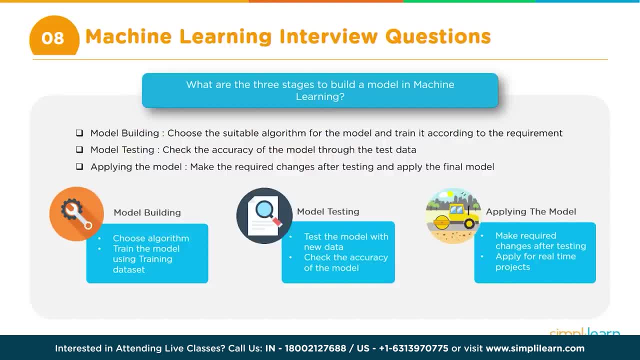 So once you test the model, you're satisfied it's working fine. Then you go to the next level, which is putting it for Production, and then in production obviously new data will come and the inference happens. So the model is readily available and only thing that happens is new data comes and the 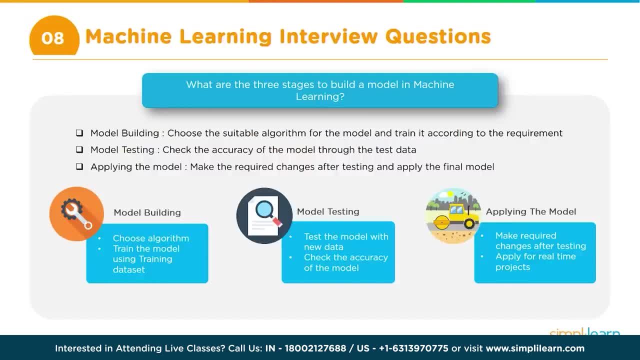 model predicts the values, whether it is regression or classification now. So this can be an iterative process. so it is not a straightforward process where you do the training for the testing and then you move it to production now. So during the training and test process there may be a situation where, because of either 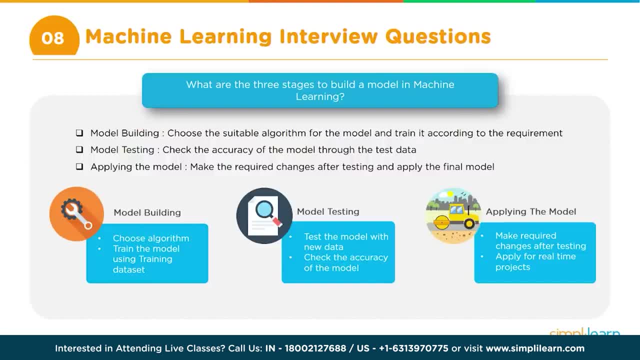 overfitting or things like that, The test doesn't go through, Which means that you need to put that back into the training process, So that can be an iterative process. Not only that, even if the training and test goes through properly and you deploy the model, 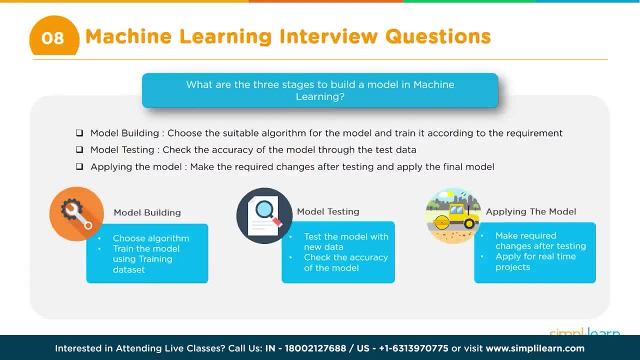 in production, there can be a situation that the data that actually comes, the real data that comes with that, this model is failing, So, in which case you may have to once again go back to the drawing board, or initially it will be working fine, but over a period of time, maybe due to the change in the nature, 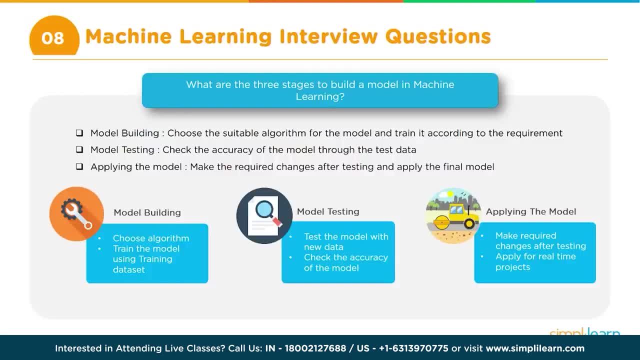 of the data. once again, the accuracy will deteriorate. So that is again a recursive process. So once in a while you need to keep checking whether the model is working fine or not And, if required, you need to tweak it and modify it, and so on and so forth. 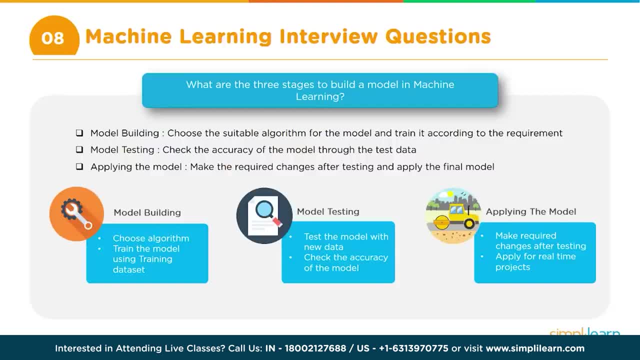 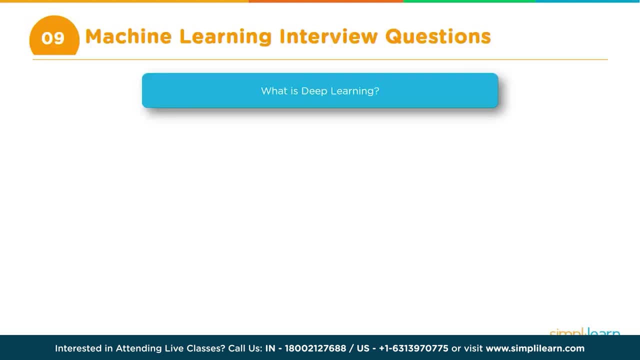 So this is a continuous process of tweaking the model and testing it and making sure it is up to date. Then you might have question around deep learning. So, because deep learning is now associated with AI, artificial intelligence and so on, So can be as simple as what is deep learning? 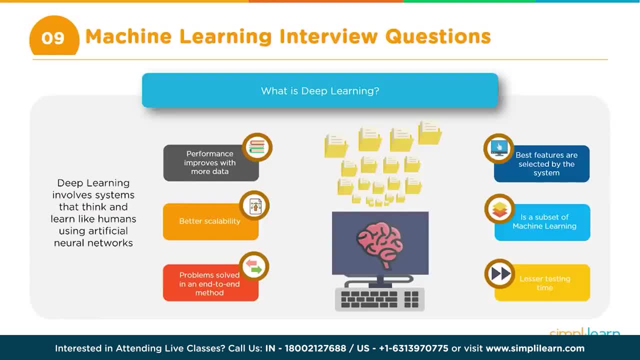 I think the best way to respond to this could be: deep learning is a part of machine learning, and then, obviously, the question would be: then what is the difference? right, So deep learning. you need to mention there are two key parts that interviewer will be. 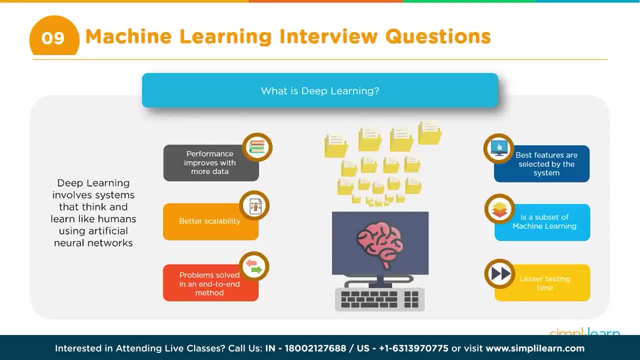 looking for when you are defining deep learning. So first is, of course, deep learning is a subset of machine learning. So machine learning is still the bigger, let's say, scope, and deep learning is one part of it. So then, what exactly is the difference? 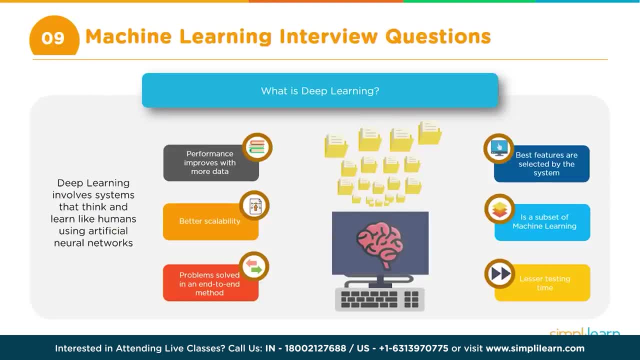 Deep learning is primarily when we are implementing these algorithms or when we are using neural networks for doing our training and classification and regression and all that right. So when we use neural network, then it is considered as deep learning, And the term deep comes from the fact that you can have several layers of neural networks. 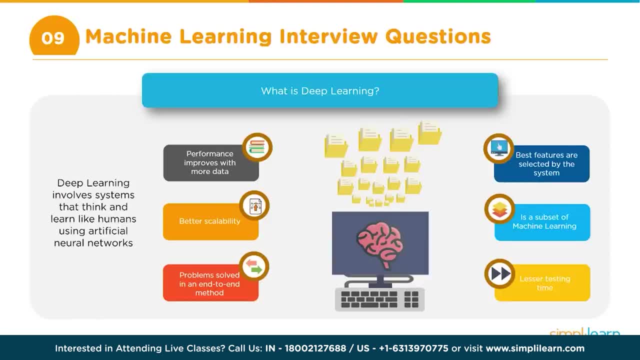 and these are called deep neural networks and therefore the term deep deep learning. The other difference between deep learning and deep learning is that deep learning is a deep learning. Deep learning is a deep learning. The difference between machine learning and deep learning, which the interviewer may be, 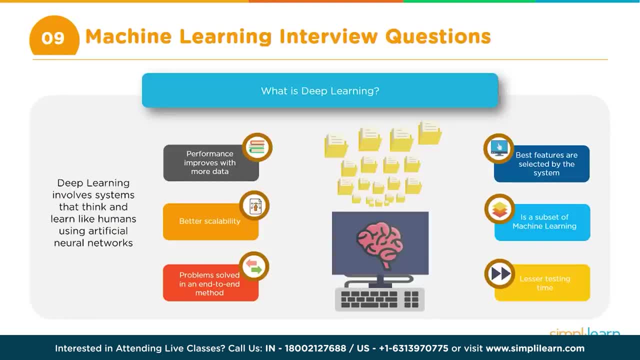 wanting to hear is that, in case of machine learning, the feature engineering is done manually. What do we mean by feature engineering? Basically, when we are trying to train our model, we have our training data right. So we have our training label data and this data has several- let's say, if it is a regular. 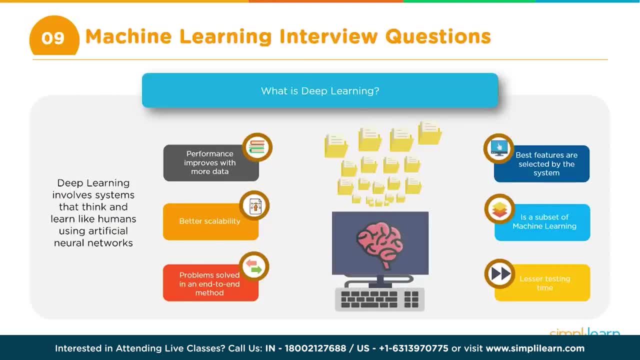 table. it has several columns. Now, Each of these columns, Each of these columns, actually has information about a feature, right? So if we are trying to predict the height, weight and so on and so forth, So these are all features of human beings. 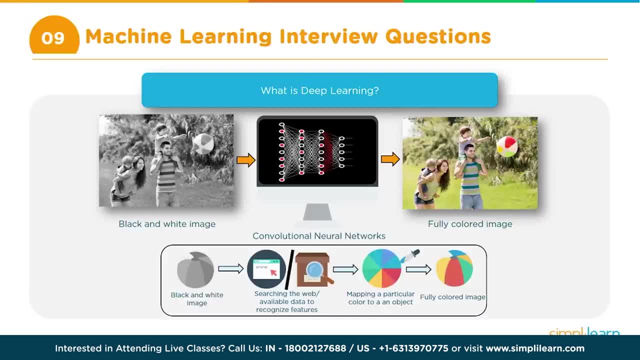 Let's say we have census data and we have all this. So those are the features Now. there may be probably 50 or a hundred. in some cases there may be a hundred such features. Now all of them do not contribute to our model, right. 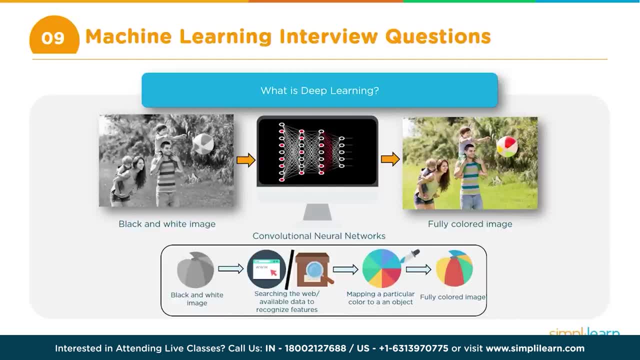 So we, as a data scientist, we have to decide whether we should take all of them, all the features, or we should throw away some of them. Because, again, if we take all of them, number one, of course your accuracy will probably. 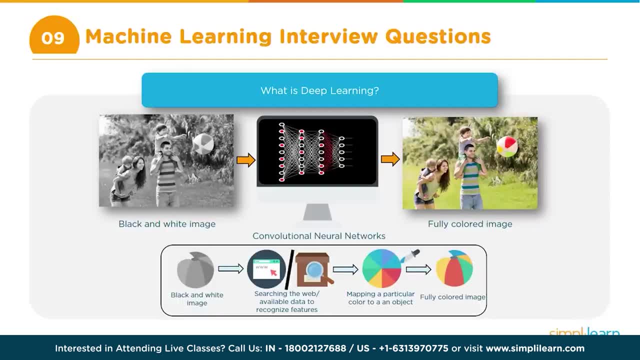 get affected. but also there is a computational part. So if you have so many features and then we have so much data, it becomes very tricky. So in case of machine learning, we manually take care of identifying the features that do not contribute to the learning process, and thereby we eliminate those features and 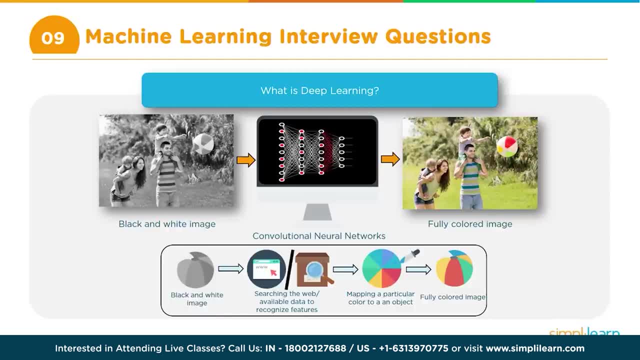 so on. So this is known as feature engineering, and in machine learning we do that manually, Whereas in deep learning, Where we use We use neural networks, The model will automatically determine which features to use and which to not use, And therefore feature engineering is also done automatically. 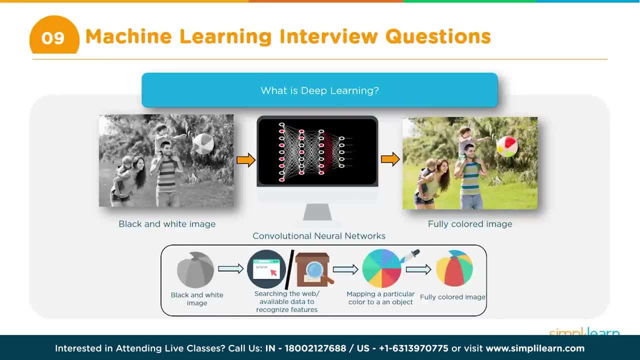 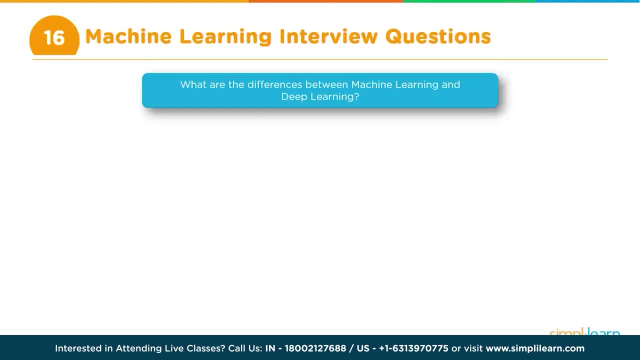 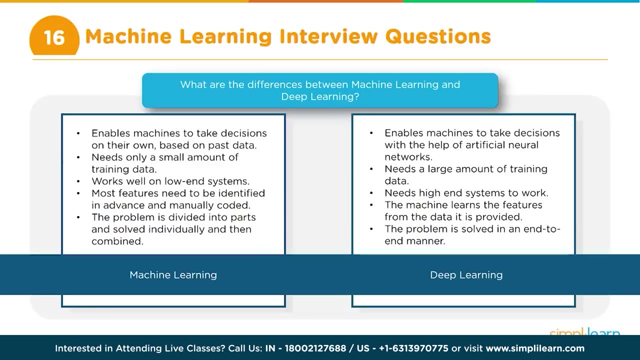 So this is a explanation. These are two key things probably will add value to your response. All right, So the next question is: what is the difference between, or what are the differences between, machine learning and deep learning? So here this is a quick comparison table between machine learning and deep learning. 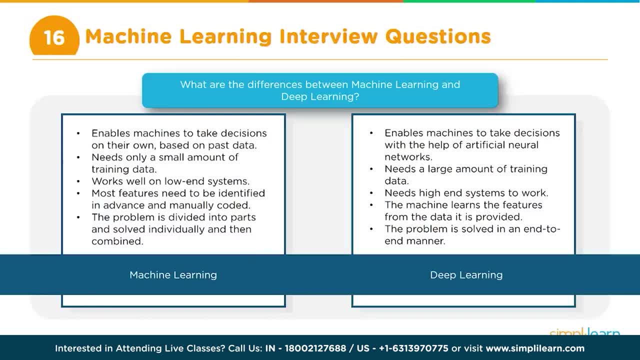 In machine learning. machine learning enables machines to take decisions on their own based on past data. So here we are talking primarily of supervised learning, and it needs only a small amount of data for training and then works well on low end systems. So you don't need large machines and most features need to be identified in advance. 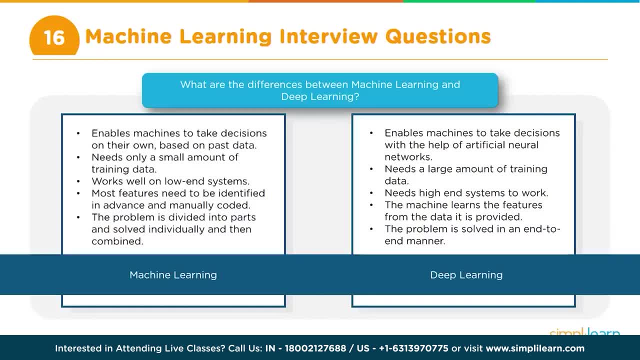 and manually coded. So basically the feature engineering part is done manually and the problem is divided into parts and solved individually And then combined. So that is about the machine learning part In deep learning. deep learning basically enables machines to take decisions with the 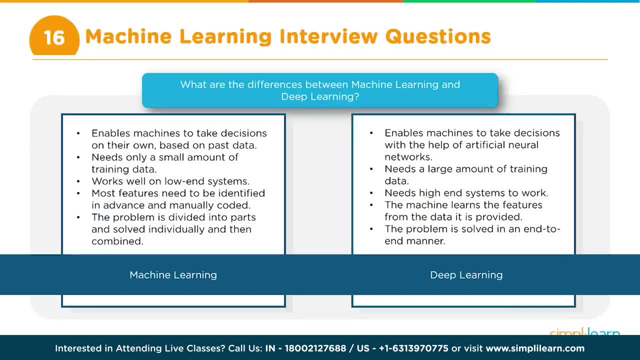 help of artificial neural networks. So here in deep learning we use neural networks. So that is the key differentiator between machine learning and deep learning. And usually deep learning involves a large amount of data And therefore the training also requires- usually the training process requires- high 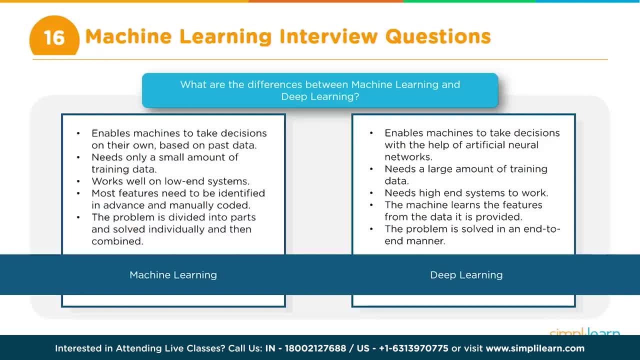 end machines because it needs a lot of computing power and the machine learning features are, or the feature engineering is, the most important part. So in deep learning, deep learning requires a large amount of data, So the machine learning is done automatically, So the neural networks takes care of doing the feature engineering as well. 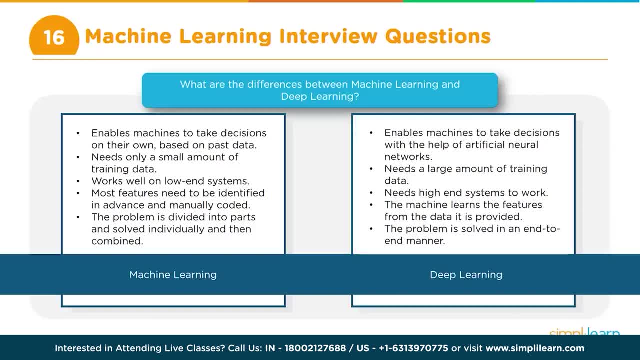 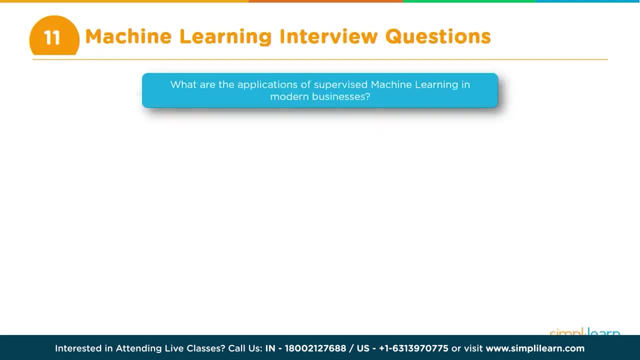 And in case of deep learning, therefore, it is said that the problem is handled end to end. So this is a quick comparison between machine learning and deep learning. in case you have that kind of a question, Then you might get a question around the uses of machine learning or some real life applications. 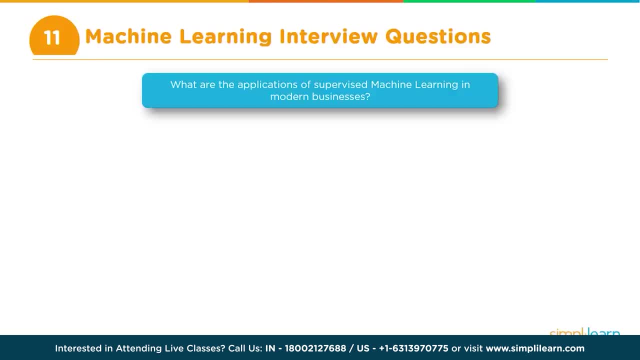 of machine learning in modern business. The question may be worded in different ways, But the meaning is: How exactly is machine learning used, or actually supervised machine learning? It could be a very specific question around supervised machine learning, So this is like give examples of supervised machine learning. use of supervised machine. 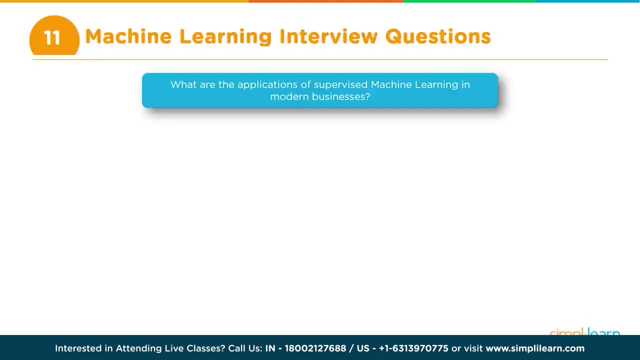 learning in modern business. So that could be the next question. So there are quite a few examples, or quite a few use cases, if you will, for supervised machine learning. The very common one is email spam detection. So you want to train your application. 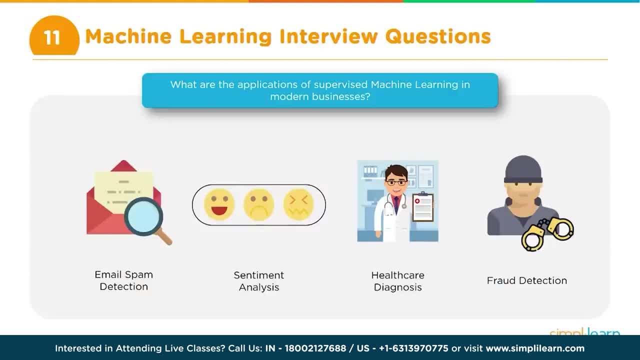 You want to train your application, You want your system to detect between spam and non-spam. So this is a very common business application of supervised machine learning. So how does this work? The way it works is that you obviously have historical data of your emails and they are 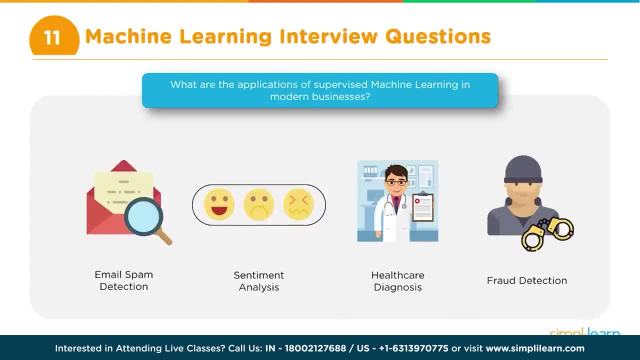 categorized as spam and not spam. So that is what is the labeled information. And then you feed this information or all these emails as an input to your model Right And the model will then get trained to detect which of the emails are, to detect which is. 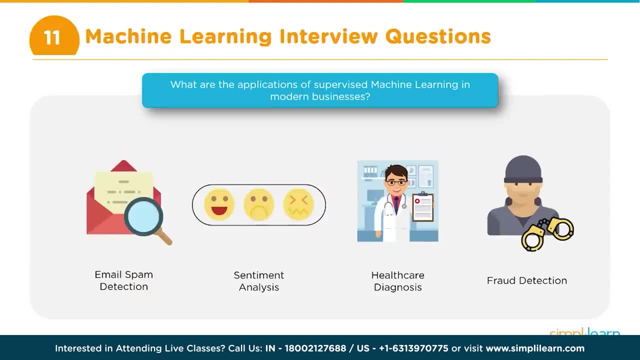 spam and which is not spam. So that is the training process, And this is supervised machine learning, because you have labeled data, You already have emails which are tagged as spam or not spam, And then you use that to train your model, Right? 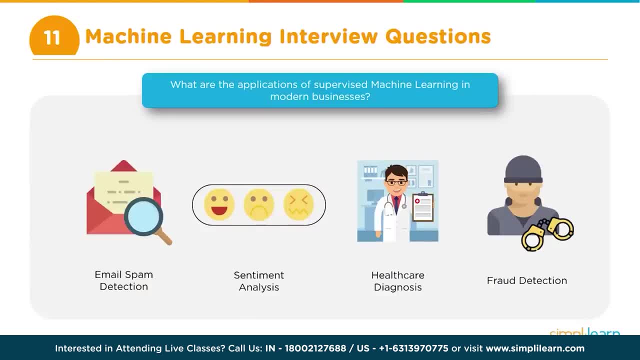 So this is one example. Now there are a few industry specific applications for supervised machine learning. One of the very common ones Is a health care diagnostics. in health care diagnostics You have these images and you want to train models to detect whether, from a particular 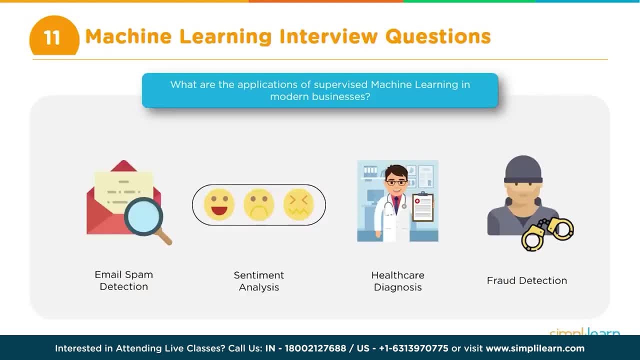 image whether it can find out if the person is sick or not, whether a person has cancer or not, Right? So this is a very good example of supervised machine learning. here The way it works is that existing images- it could be X-ray images, MRI or any of these- 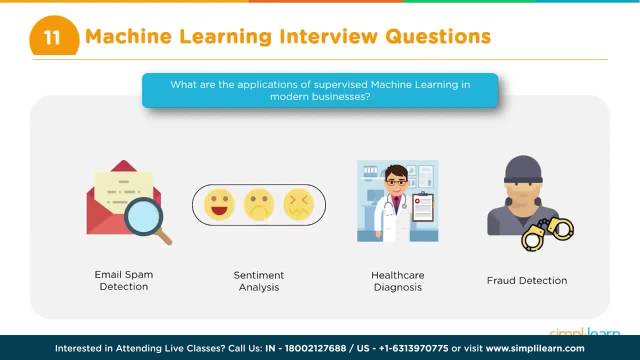 images Are available and they are tagged saying that, OK, this X-ray image is defective, or the person has an illness, or it could be cancer, whichever illness, right? So it is tagged as defective or clear or good image and defective image, something like that. 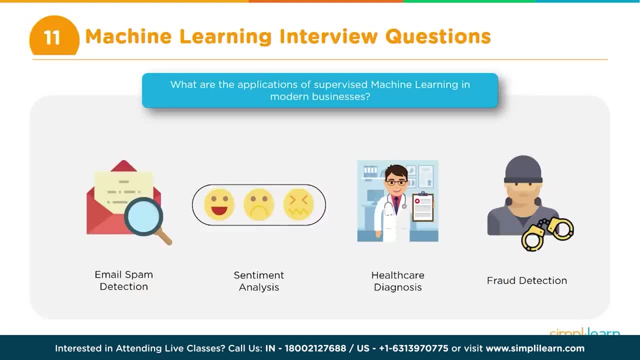 So we come up with the binary- or it could be multiclass as well- saying that this is defective to 10 percent, this is 25 percent, and so on. But let's keep it simple. You can give an example of just a binary classification. that would be good enough. 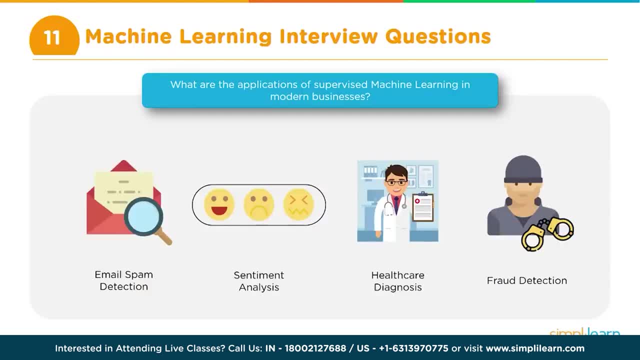 So you can say that In health care diagnostics using image, we need to detect whether a person is ill or whether a person is having cancer or not. So here the way it works is you feed labeled images and you allow the model to learn from. 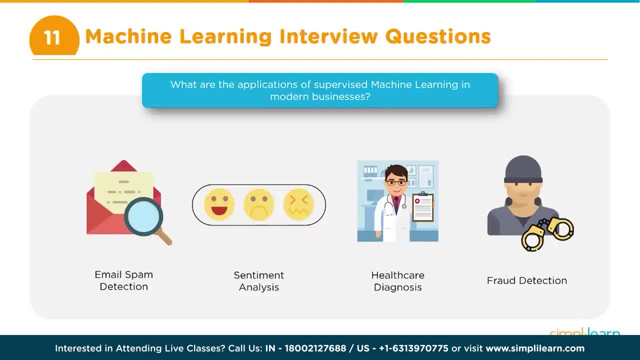 that, so that when new image is fed, it will be able to predict whether this person is having that illness or not, having cancer or not, Right? So I think this would be a very good example for supervised machine learning in modern business, All right. 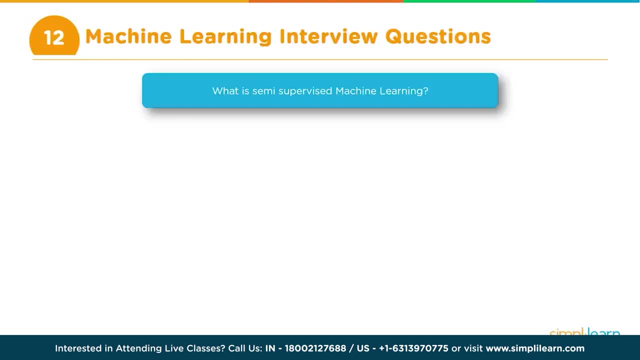 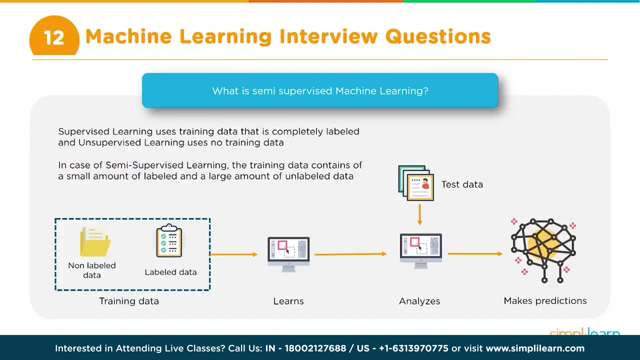 So we can have a question like: so we've been talking about supervised and unsupervised, and so there can be a question around semi-supervised machine learning. So what is semi-supervised machine learning? Now, semi-supervised learning, as the name suggests, it falls between supervised learning. 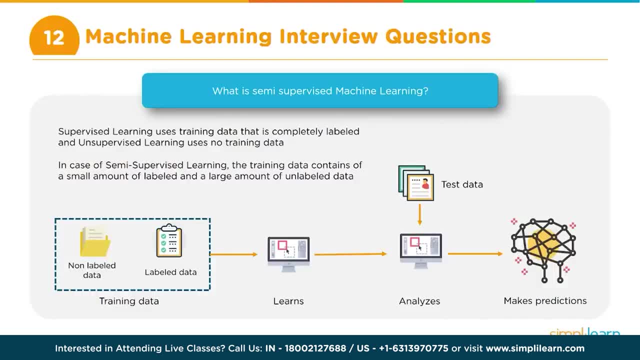 and unsupervised learning, But for all practical purposes it is considered as a part of supervised learning, And the reason this has come into existence is that In supervised learning you need labeled data. so all your data for training, your model, has to be labeled. 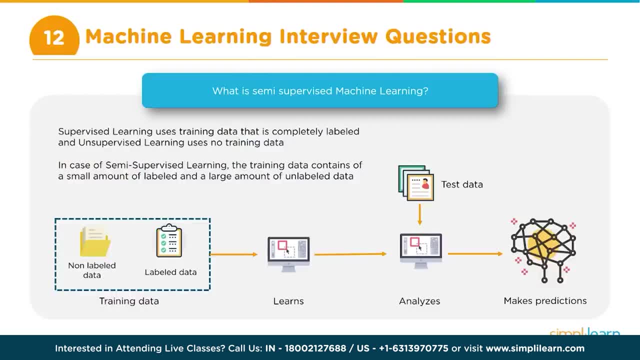 Now this is a big problem in many industries, or in many under many situations. Getting the label data is not that easy, because there's a lot of effort in labeling this data. Let's take an example of diagnostic images. We can just, let's say, take X-ray images, and there are actually millions of X-ray images. 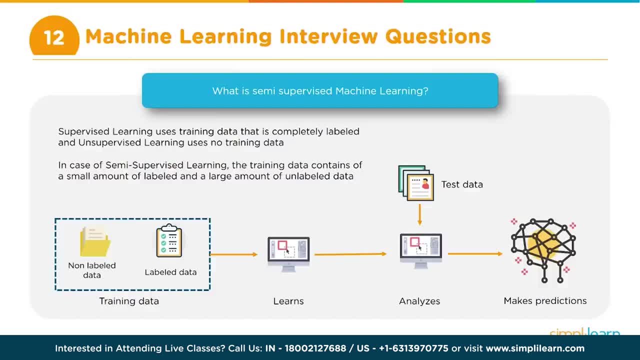 available all over the world, But the problem is they are not labeled. so the images are there, But whether it is effective or whether it is good that information is not available along with that right in a form that it can be used by a machine, which means that somebody 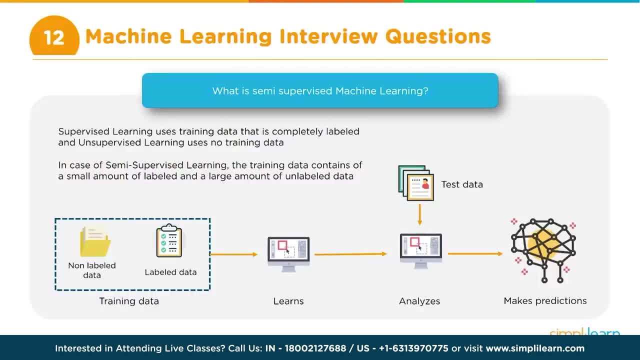 has to take a look at these images, and usually it should be like a doctor and then say that, OK, yes, this image is clean and this image is cancerous, and so on and so forth. Now that is a huge effort by itself. 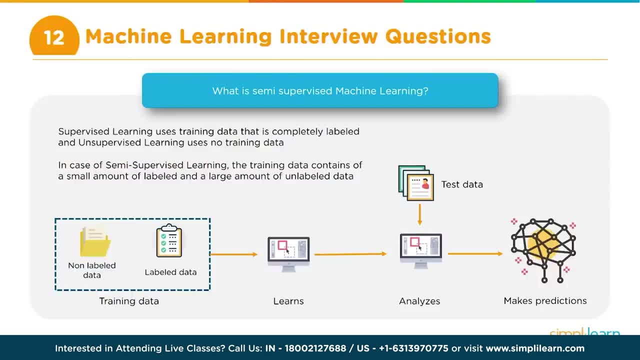 So this is where semi-supervised- Okay, Semi-supervised- learning comes into play. So what happens is there is a large amount of data, maybe a part of it is labeled. Then we try some techniques to label the remaining part of the data so that we get completely. 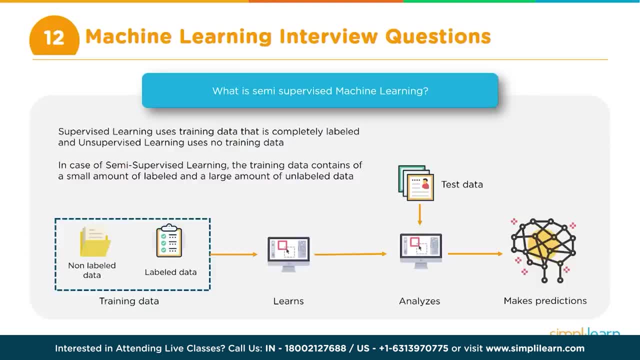 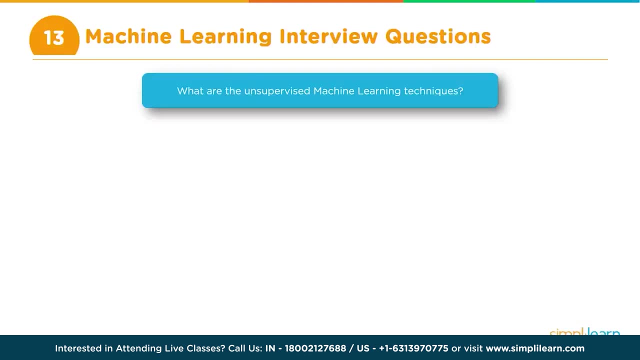 labeled data and then we train our model. So I know this is a little long winding explanation, but unfortunately there is no quick and easy definition for semi-supervised machine learning is the only way probably to explain this concept. We may have another question, as what are unsupervised machine learning techniques or what are some? 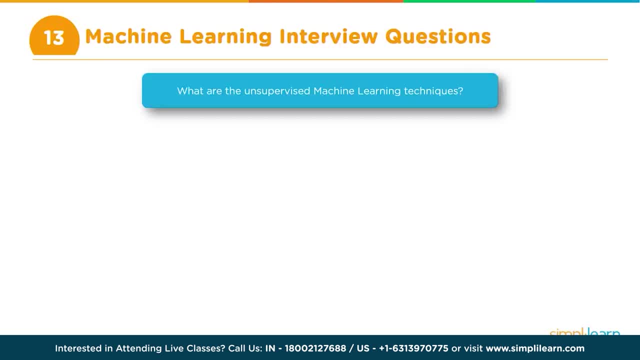 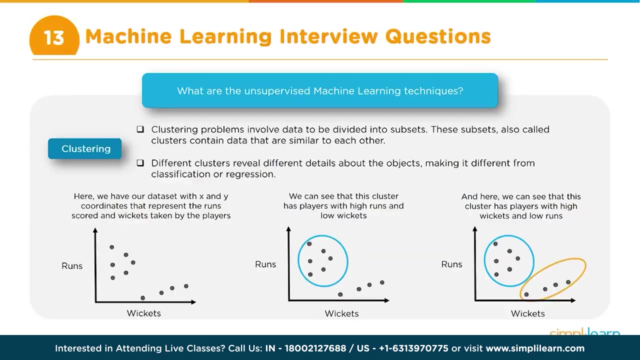 of the techniques used for performing unsupervised machine learning, So it can be worded in different ways. So how do we answer this question? So, unsupervised learning, you can say that there are two types: clustering and association. And clustering is a technique where similar objects are put together. 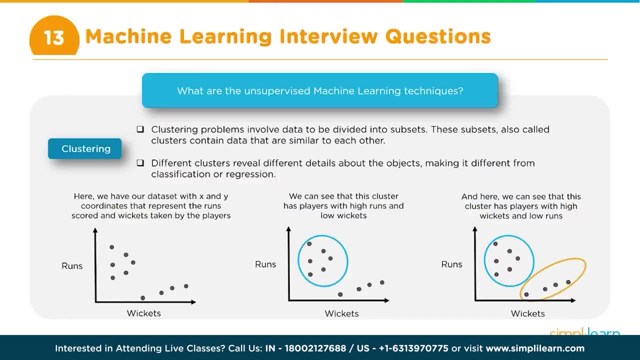 There are different ways of finding them, So there are different ways of finding them, So there are different ways of finding similar objects. So their characteristics can be measured and if they have most of the characteristics, if they are similar, then they can be put together. 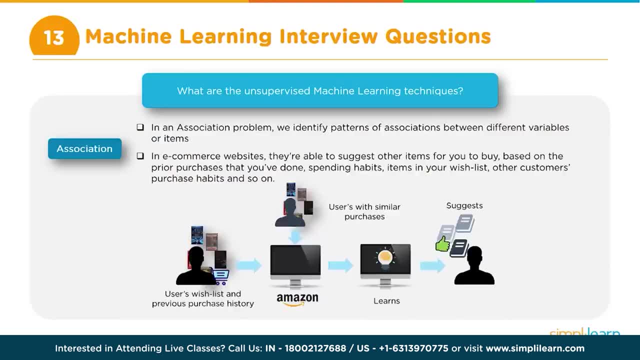 This is clustering, Then association you can. I think the best way to explain association is with an example. In case of association, you try to find out how the items are linked to each other. So, for example, if somebody bought, maybe, a laptop, the person has also purchased a mouse. 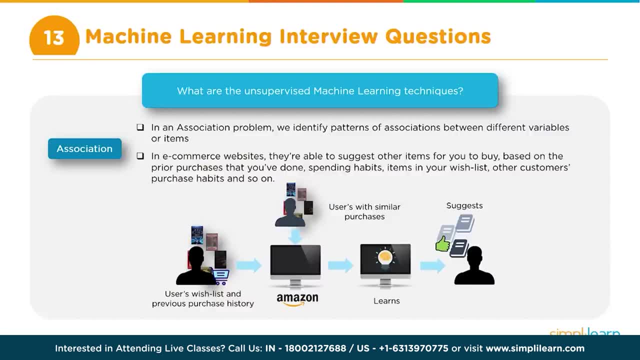 So this is more in an e-commerce scenario, for example, so you can give this as an example. So people who are buying laptops are also buying a mouse, So that means there is an association between laptops and mouse. or maybe people who are 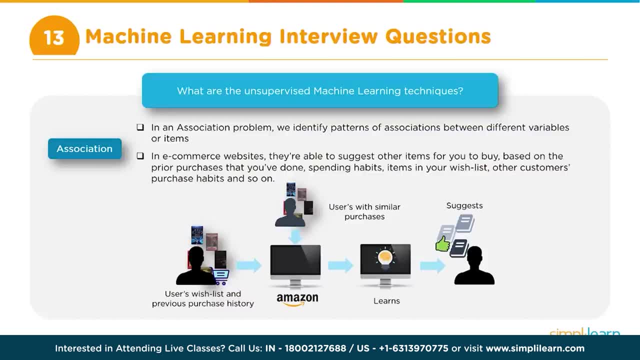 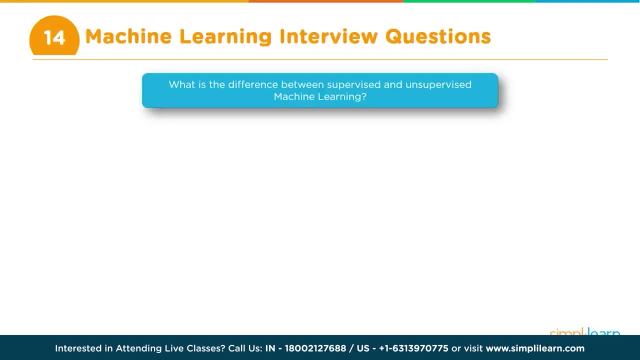 buying bread are also buying butter, So that is a association that can be created. So this is unsupervised learning one of the techniques. Okay, All right. Then we have a fundamental question: What is the difference between supervised and unsupervised? 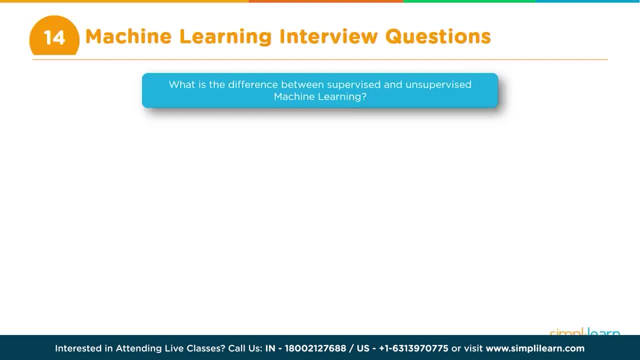 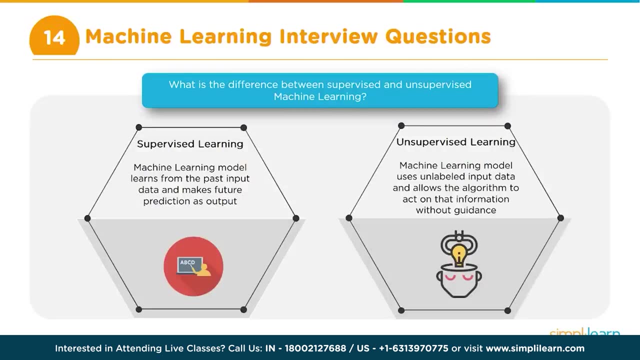 What is supervised machine learning? So, machine learning, these are the two main types of machine learning: supervised and unsupervised. And in case of supervised- and again here, probably the key word that the person may be wanting to hear is labeled data. 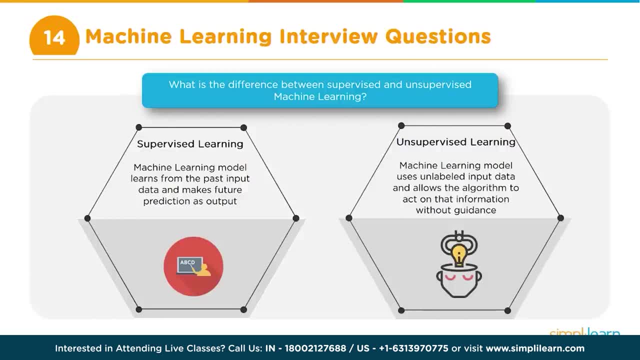 Now, very often people say: we have historical data and if we run it it is supervised. And if we don't have historical data, yes, but you may have historical data, but if it is not labeled, then you cannot use it for supervised learning. 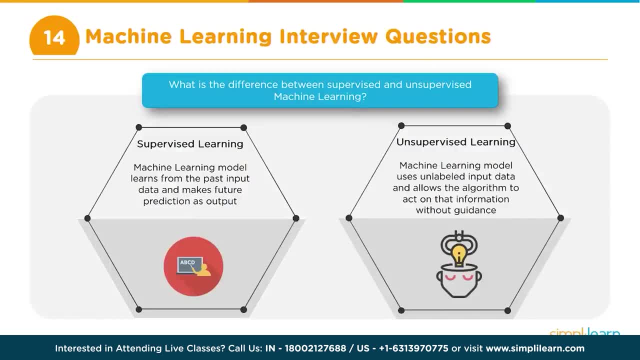 So it is. it's very key to understand that. So we put in that keyword labeled okay. So when we have labeled data for training our model, then we can use supervised learning, And if we do not have labeled data, then we use unsupervised learning. 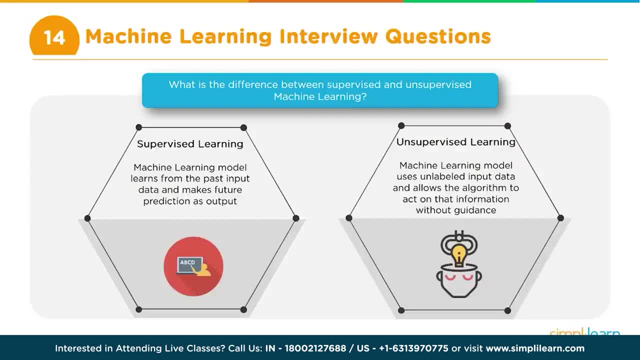 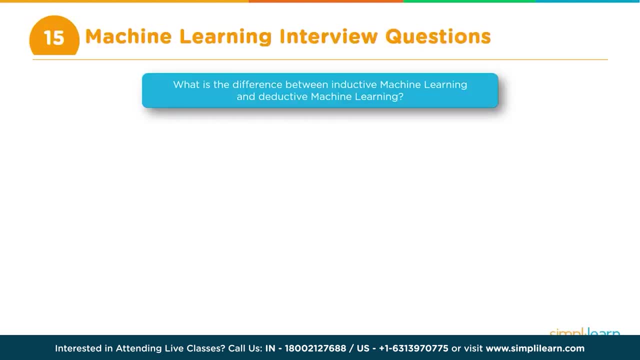 And there are different algorithms available to perform both of these types of trainings. So there can be another question a little bit more theoretical and conceptual in nature. This is about inductive machine learning, Okay, And deductive machine learning. So the question can be: what is the difference between inductive machine learning and deductive? 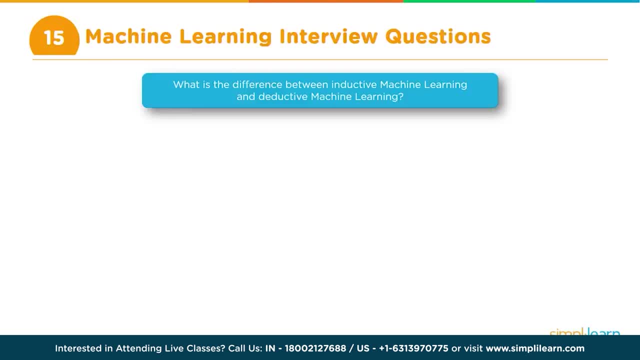 machine learning or somewhat in that manner, so that the exact phrase or exact question can vary and they can ask for examples and things like that. but that could be the question. So let's first understand what is inductive and deductive training. 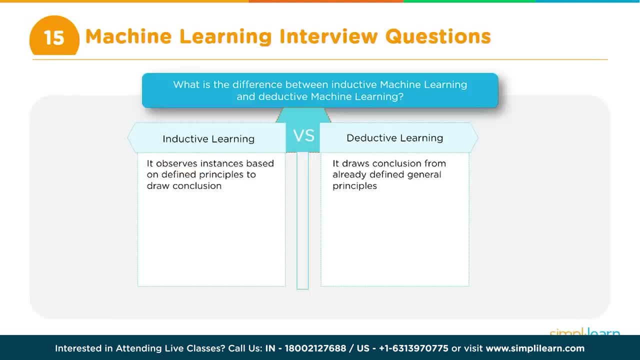 Inductive training is induced by somebody and you can illustrate that with a small example. I think that always helps. So whenever you're doing some explanation, try as much as possible, as I said, to give examples from your work experience or give some analogies. 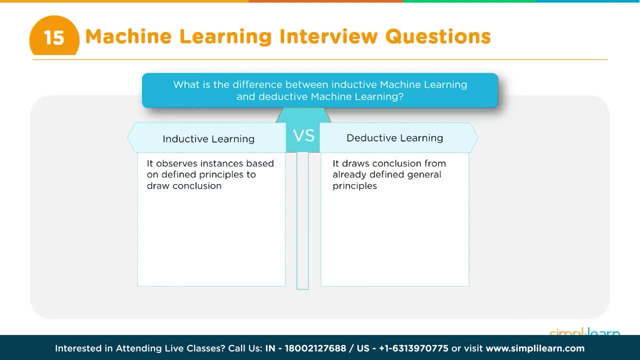 And that will also help a lot in explaining as well and for the interviewer also to understand. So here we'll take an example, or rather we will use an analogy. So inductive training is when we induce some knowledge or the learning process into a person. 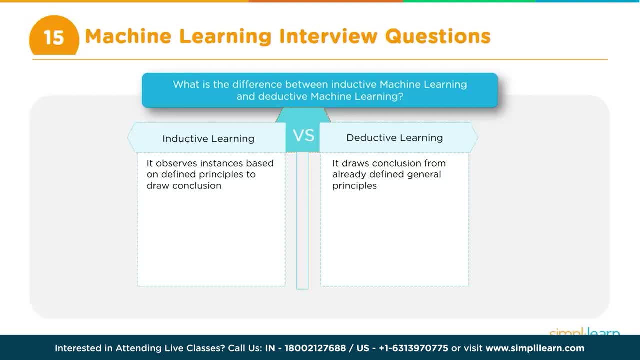 without the person actually experiencing it. What can be an example? So we can probably tell the person or show a person, Okay. Okay, So the person is a video that fire can burn the thing, burn his finger or fire can cause damage. 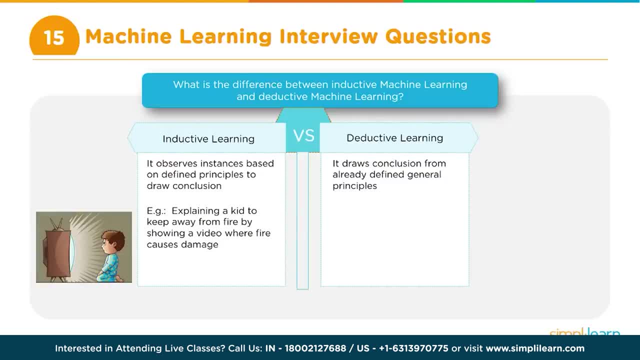 So what is happening here? This person has never probably seen a fire or never seen anything getting damaged by fire, but just because he has seen this video, he knows that, okay, fire is dangerous And if a fire can cause damage, right. 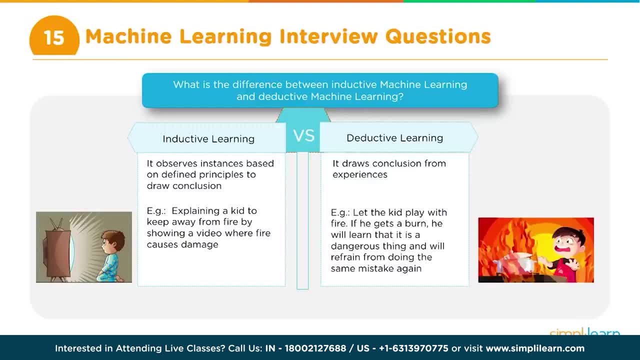 So this is inductive learning compared to that, What is deductive learning? So here you draw conclusions. The person draws conclusion out of experience, So we will stick to the analogy. So, compared to the showing a video, let's assume a person is allowed to play with fire. 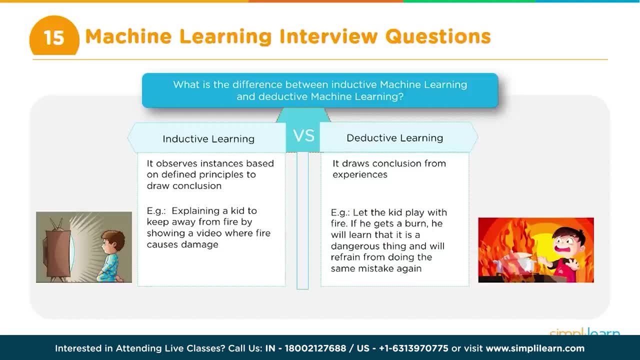 right. And then he figures out that if he puts his finger, it's burning, or if throw something into the fire, it burns. So he is learning through experience. So this is known as deductive learning. Okay, So you can have applications or models that can be trained using inductive learning or 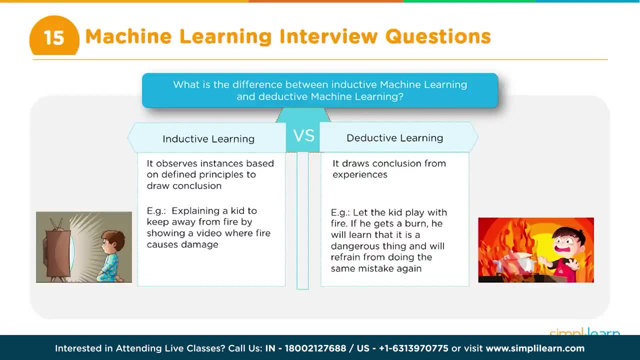 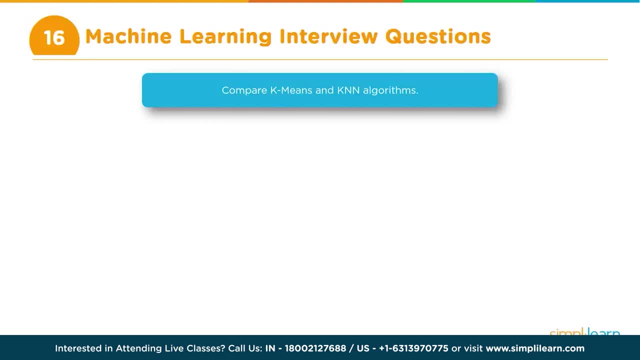 deductive learning. All right, I think probably that explanation will be sufficient. The next question is: are KNN and K-means clustering similar to one another or are they same right, Because the letter K is kind of common between them okay? 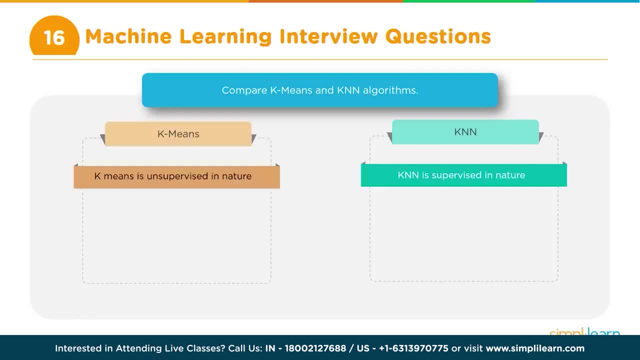 So let us take a little while to understand what these two are. One is KNN and another is K-means. KNN stands for K- nearest neighbors- and K-means, of course, is the clustering mechanism. Now, K and N are completely different, except for the letter K being common between them. 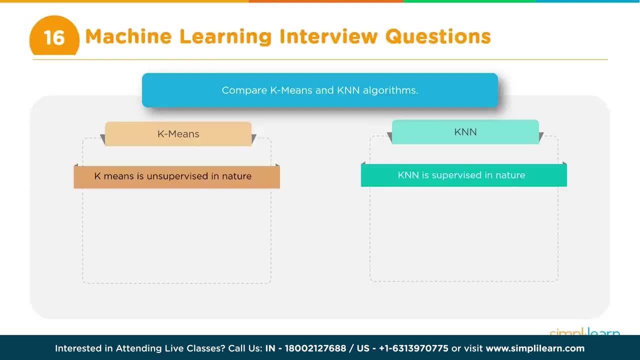 KNN is completely different. K-means clustering is completely different. KNN is a classification process and therefore it comes under supervised learning, whereas K-means clustering is actually unsupervised. okay, When you have KNN, when you want to implement KNN, which is basically K- nearest neighbors- 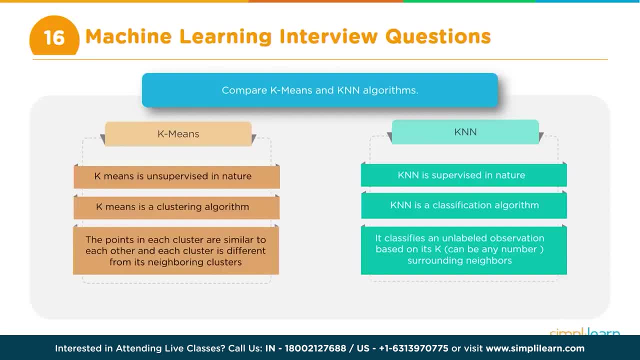 the value of K is a number, So you can say K is equal to 3.. You want to implement KNN with: K is equal to 3. So which means that it performs the classification in such a way that how does it perform the? 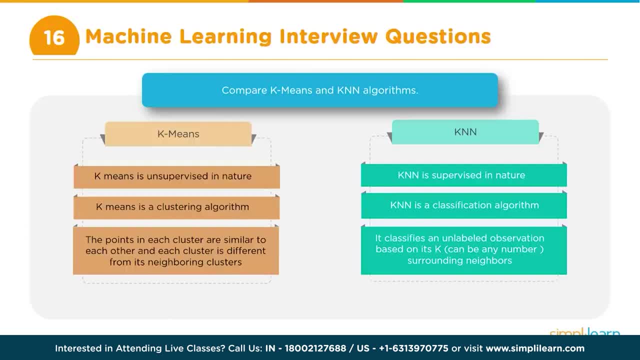 classification. So it will take three nearest objects and that is why it is called nearest neighbor. So basically, based on the distance, it will try to find out its nearest objects, that are, let us say, three of the nearest objects, and then it will check whether the class they. 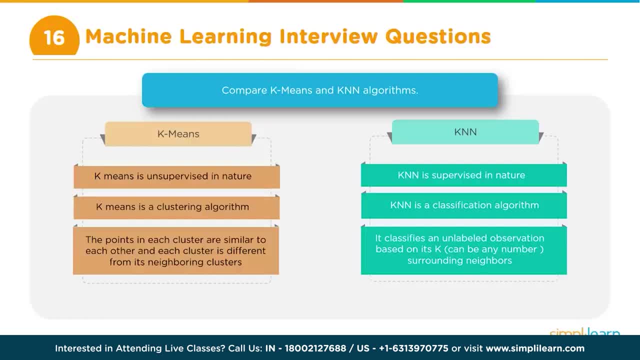 belong to which class, right? So if all three belong to one particular class, Obviously The object is also classified as that particular class. but it is possible that they may be from two or three different classes. Okay, So let's say they are from two classes and then if they are from two classes, now, usually 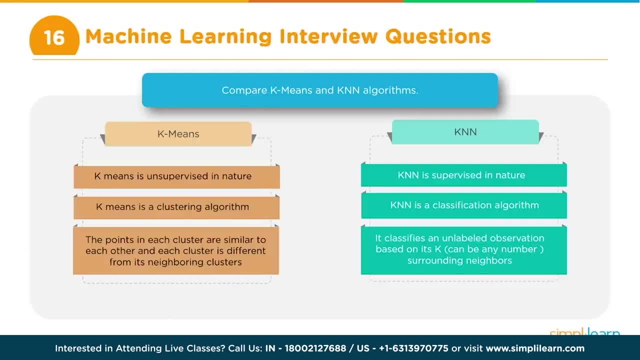 you take an odd number. you assign an odd number to say, if there are three of them and two of them belong to one class and then one belongs to another class, So this new object is assigned to the class to which the two of them belong. 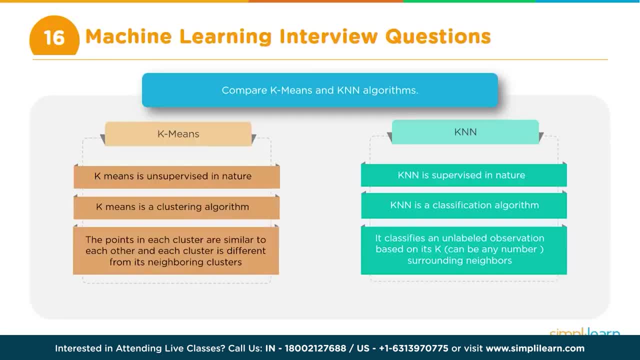 Now, the value of K is sometimes tricky: Whether should you use three, Should you use four, Should you use five, Should you use seven? That can be tricky because the ultimate classification can also vary. So it's possible that if you're taking K as three, the object is probably in one particular. 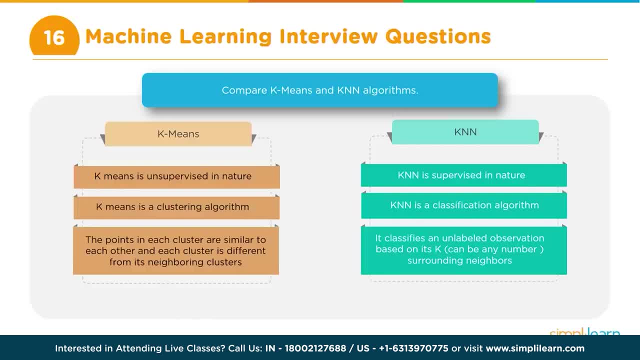 class. But if you take, K is equal to five, maybe the object will belong to a different class, because when you're taking three of them, probably two of them belong to a class one and one belong to class two, Whereas when you take five of them, it is possible that only two of them belong to class two. 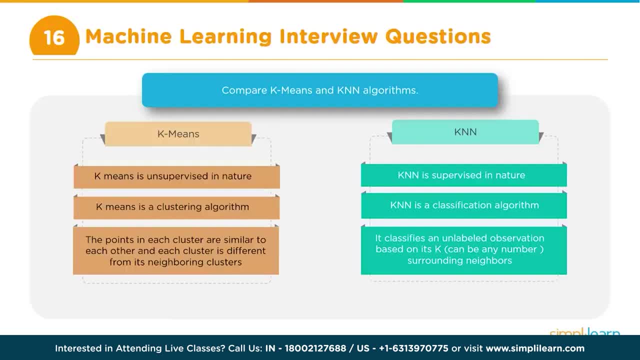 Okay, So basically, two of them belong to class one and three of them belong to class two, So which means that this object will belong to class two, right? So you see that. So it is. the class allocation can vary depending on the value of K. Now, K means on the other. 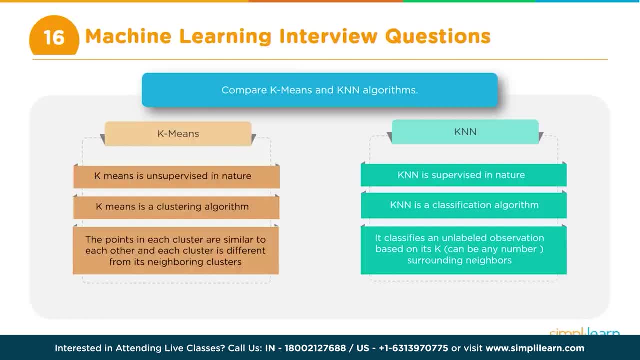 hand, is a clustering process and it is unsupervised, where what it does is the system will basically identify how the objects are, how close the objects are with respect to some of their features. Okay, And, but the similarity, of course, is the, the letter K, And in this case the system will. 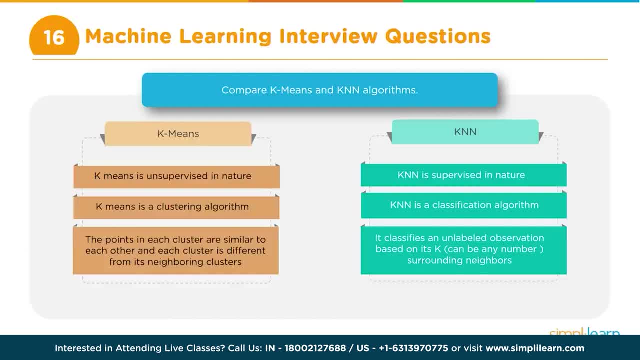 basically identify how the objects are, how close the objects are with respect to some of their features. Okay, And in case of K means also, we specify its value, and it could be three or five or seven. There is no technical limit as such, but it can be any number of clusters that you can. 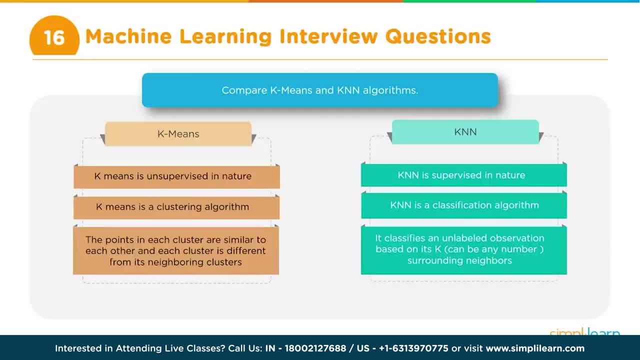 create. Okay, So based on the value that you provide, the system will create that many clusters of similar objects. So there is a similarity to that extent that K is a number in both the cases, but actually these two are completely different processes. 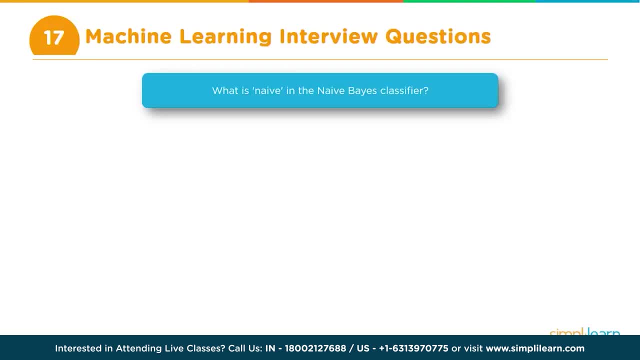 We have what is known as Naive Bayes cluster. So the name of the person who found this classifier or who developed this classifier, which is not a hundred percent true, Bayes, is the name of the person. B-A-Y-E-S is the name of the person. 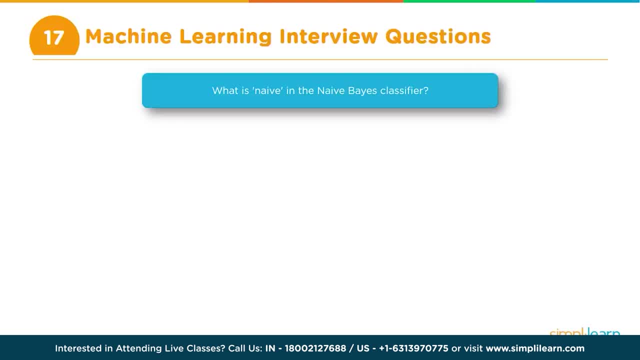 But Naive is not the name of the person, Right? So Naive is basically an English word and that has been added here. because of the nature of his particular classifier, Naive Bayes classifier is a probability based classifier, Okay, and it makes some assumptions that presence of one feature of a class is not related to the 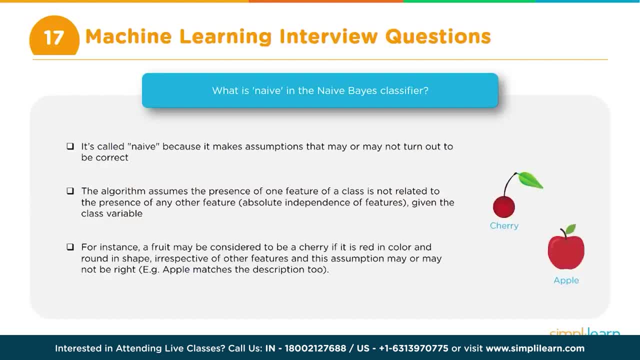 presence of any other feature of maybe other classes, right, So which is not very strong or not a very- what do you say? accurate assumption, because these features can be related and so on. But even if we go with this assumption, this whole algorithm works very well. 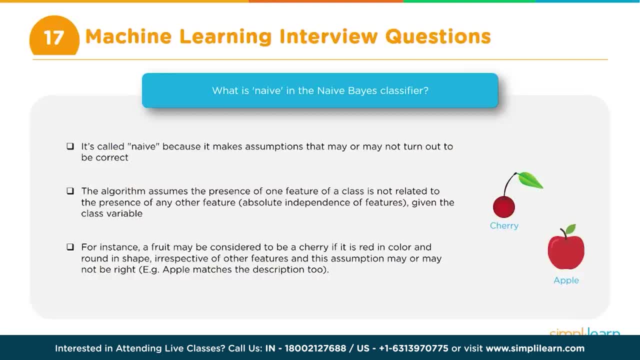 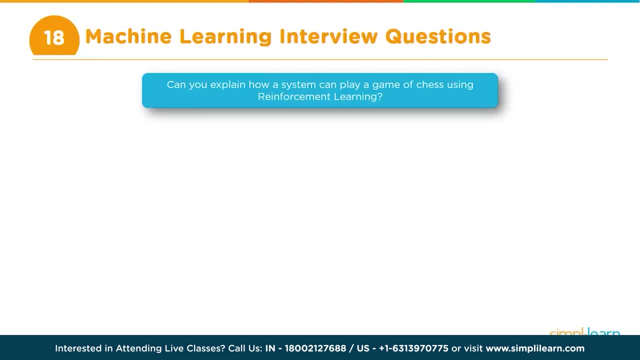 even with this assumption, and that is the good side of it, but the term comes from that, So that is the explanation that you can get. Then there can be question around reinforcement learning. It can be paraphrased in multiple ways. One could be: can you explain how a system can? 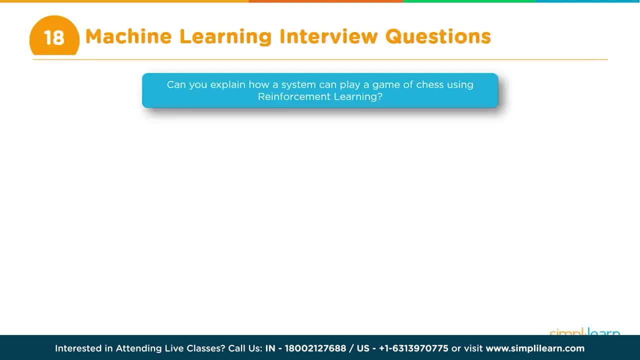 play a game of chess using reinforcement learning, or it can be any game. So the best way to explain this is again to talk a little bit about what reinforcement learning is about and then elaborate on that to explain the process. So, first of all, reinforcement learning has an environment and an 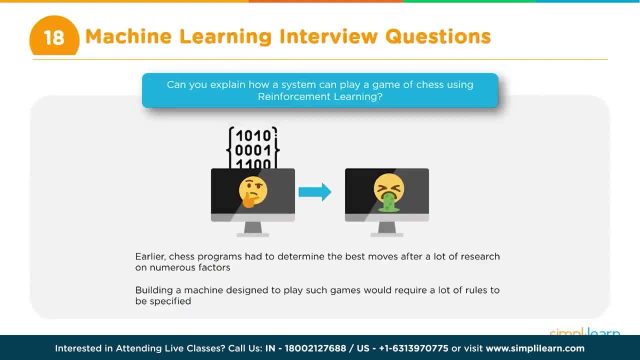 agent. The agent is basically performing some actions in order to achieve a certain goal, and these goals can be anything either. if it is related to game, then the goal could be that you have to score very high score, a high value, high number, or it could be that your number of lives should be as high as 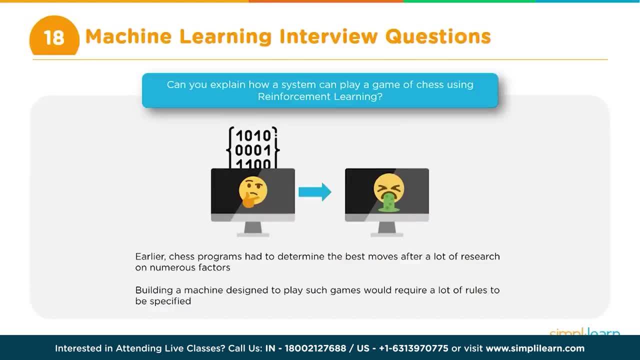 possible, Don't lose life. So these could be some of them. More advanced examples could be for driving in the automotive industry: self-driving cars. They actually also make use of reinforcement learning to teach the car how to navigate through the roads. 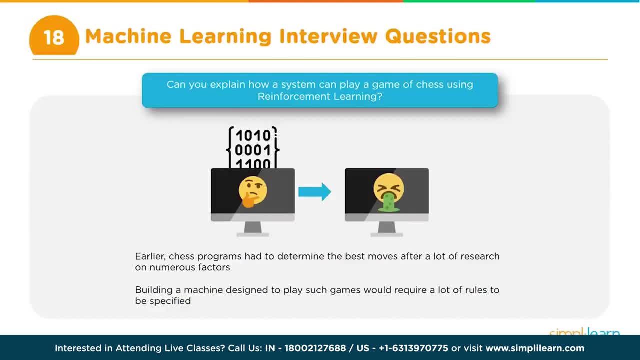 and so on and so forth. That is also another example. Now how does it work? So if the system is basically there is an agent and environment, and every time the agent takes a step or performs a task which is taking it towards the goal, the final goal, let's say, to maximize the score, or 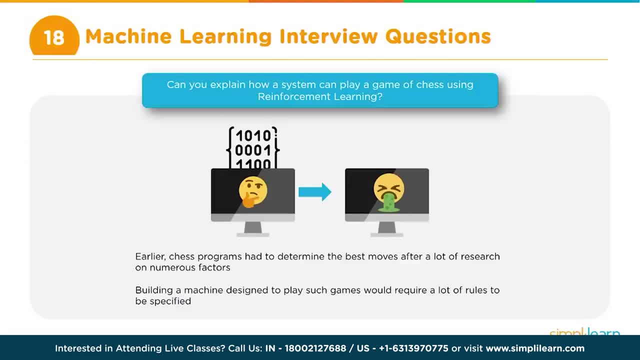 to minimize the number of lives and so on, or minimize the debts, for example, it is rewarded and every time it takes a step which goes against that goal and contrary or in the reverse direction, it is penalized. So it is like a carrot and stick system. Now how do you use this to create a game? 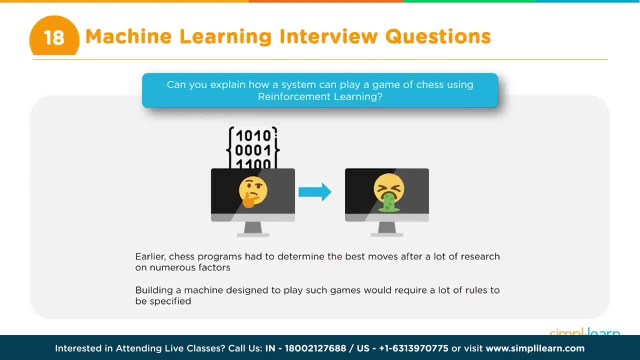 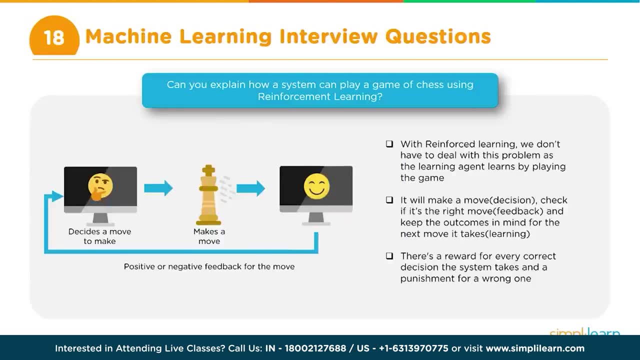 of chess or to create a system to play a game of chess. Now, the way this works is- and this could probably go back to this AlphaGo example, where AlphaGo defeated a human champion- So the way it works is in reinforcement learning, the system is allowed, for example. in this case, we are talking. 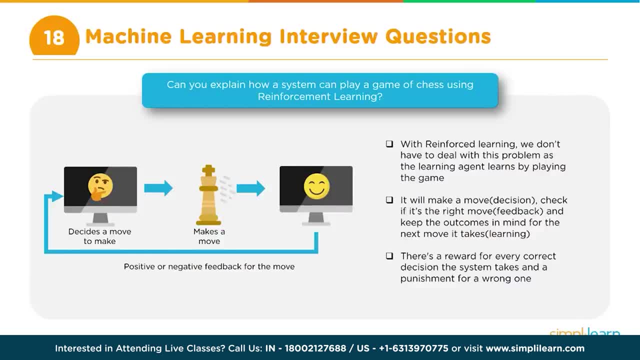 about chess. so we allow the system to first of all watch playing a game of chess. so it could be with a human being, or it could be the system itself. there are computer games of chess right, so either this new learning system has to watch that game or watch a human being play the game. 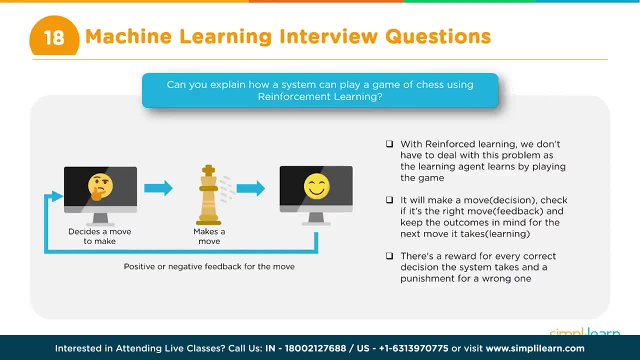 because this is reinforcement. learning is pretty much all visual. so when you're teaching the system to play a game, the system will not actually go behind the scenes to understand the logic of your software, of this game or anything like that. it is just visually watching the screen. 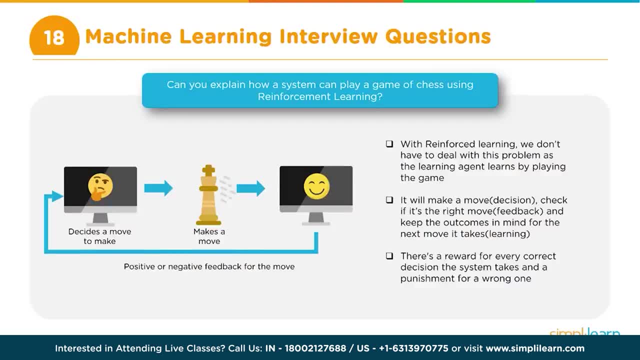 and then it learns. okay, so reinforcement learning to a large extent works on that. so you need to create a mechanism whereby your model will be able to watch somebody playing the game and then you allow the system also to start playing the game. so it pretty much starts from scratch. 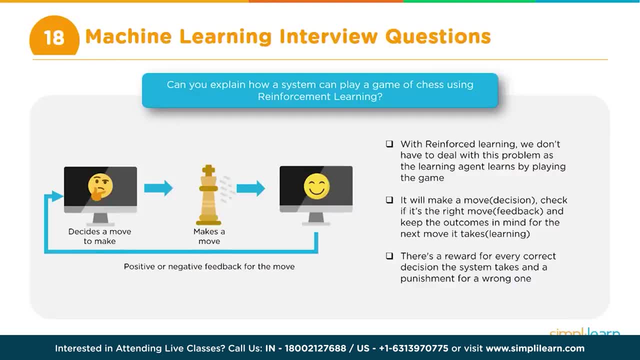 okay, and as it moves forward it it's like, right at the beginning, the system really knows nothing about the game of chess. okay, so initially it is a clean slate. it just starts by observing how you're playing, so it will make some random moves and keep losing badly. but then what happens? 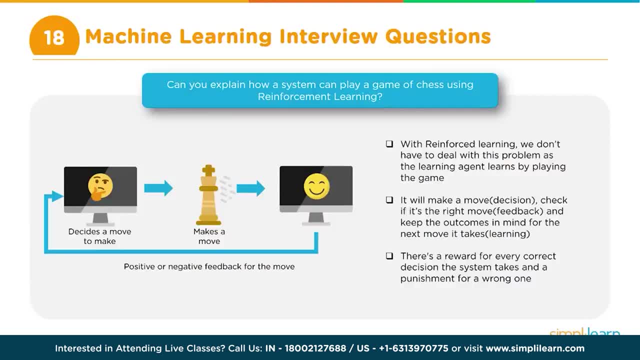 is over a period of time, so you need to now allow the system or you need to play with this system, not just one, two, three, four or five years times, but hundreds of times, thousands of times, maybe even hundreds of thousands of times. and that's exactly how AlphaGo has done. It played millions of games between itself and the system. 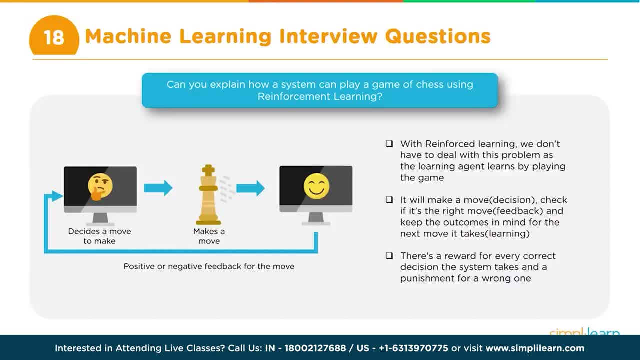 right. So for the game of chess also, you need to do something like that. You need to allow the system to play chess and then learn on its own over a period of repetition. So I think you can probably explain it to this much to this extent, and it should be sufficient. Now this is another. 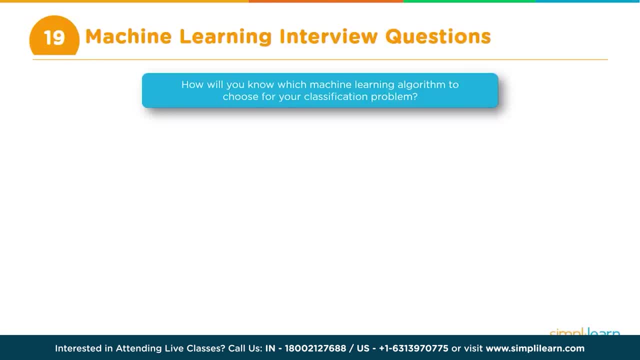 question which is again somewhat similar, but here the size is not coming into picture. So the question is: how will you know which machine learning algorithm to choose for your classification problem? Now, this is not only classification problem, It could be a regression problem. I 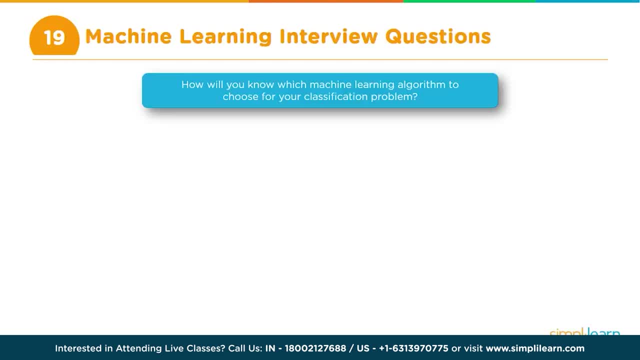 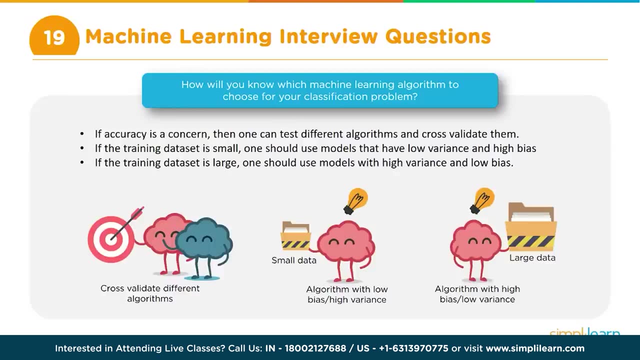 would like to generalize this question. So if somebody asks you, how will you choose, how will you know which algorithm to use, The simple answer is: there is no way you can decide Exactly saying that this is the algorithm I am going to use In a variety of situations there. 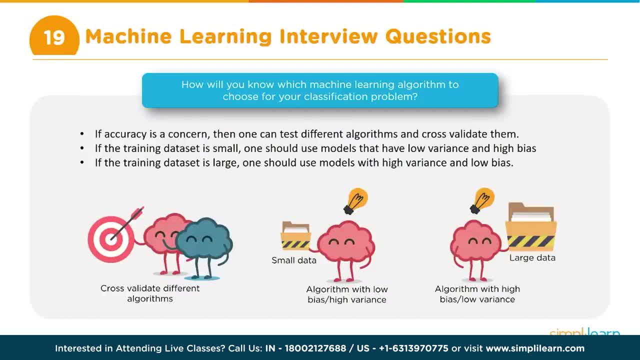 are some guidelines like, for example: you will obviously, depending on the problem, you can say whether it is a classification problem or a regression problem and then, in that sense you are kind of restricting yourself to: if it is a classification problem there are, you can only apply a classification algorithm right To that extent. you can probably, let's say, limit the number. 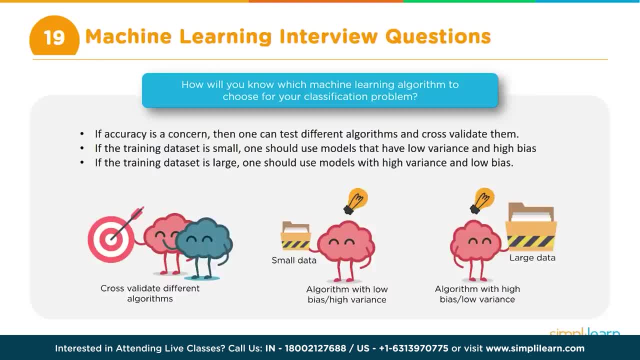 of algorithms, but no, Within the classification algorithms, you have decision trees, you have SPM, you have logistic regression. Is it possible to outright say yes for this particular problem? since you have explained this? Now, this is the exact algorithm that you can use. That is not possible, Okay so. 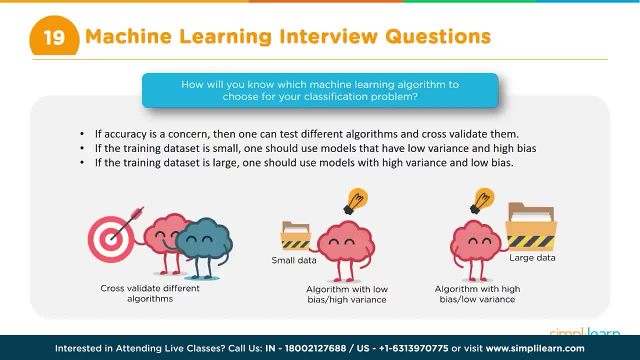 we have to try out a bunch of algorithms, See which one gives us the best performance and best accuracy, and then decide to go with that particular algorithm. So in machine learning a lot of it happens through the classification algorithm. So you have to try out a bunch of algorithms. 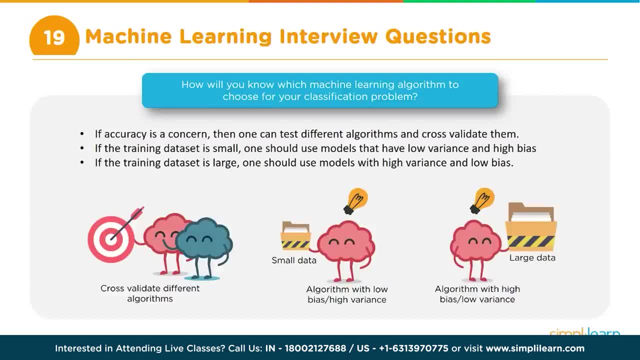 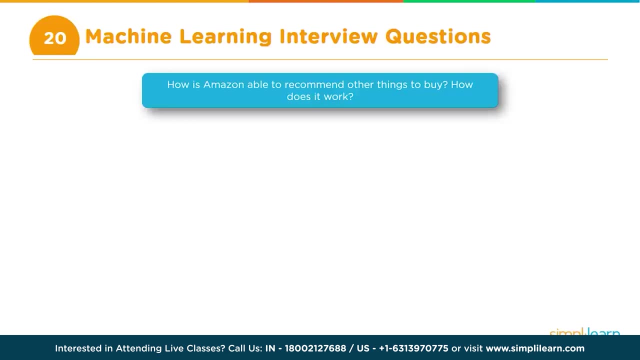 There is no real possibility that anybody can, just by looking at the problem or understanding the problem, tell you that okay, in this particular situation, this is exactly the algorithm that you should use. Then the questions may be around application of machine learning, and this question is specifically around how Amazon is able to recommend other things to buy. So this is around 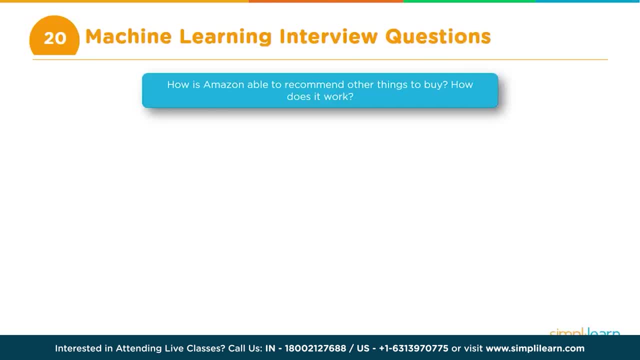 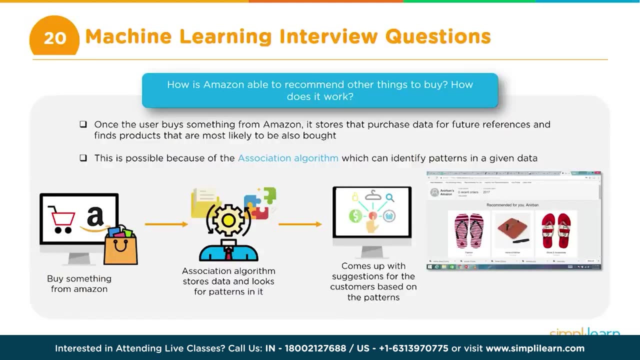 recommendation engine. How does it work? How does the recommendation engine work? So this is basically the question is all about. So the recommendation engine again works based on various inputs that are provided. Obviously, something like you know Amazon website or e-commerce site like Amazon collects a lot of. 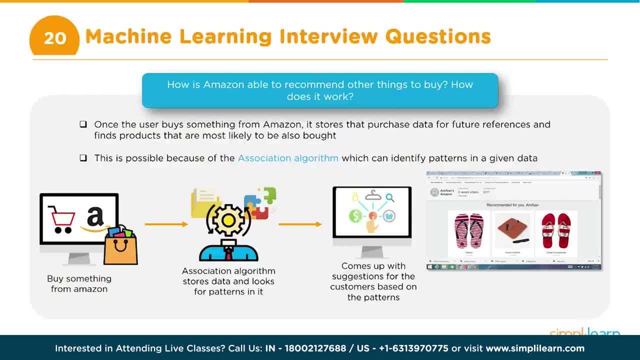 data around the customer behavior- Who is purchasing what, and if somebody is buying a particular thing, they are also buying something else. So this kind of association, right. so this is the unsupervised learning we talked about. They use this to associate and link or relate. 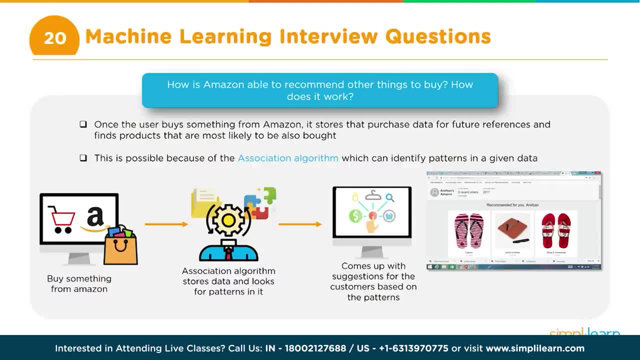 and that is one part of it. So they kind of build association between items, saying that somebody buying this is also buying this. That is one part of it. Then they also profile the users right based on their age, their gender, their geographic location. They will do some profiling and then 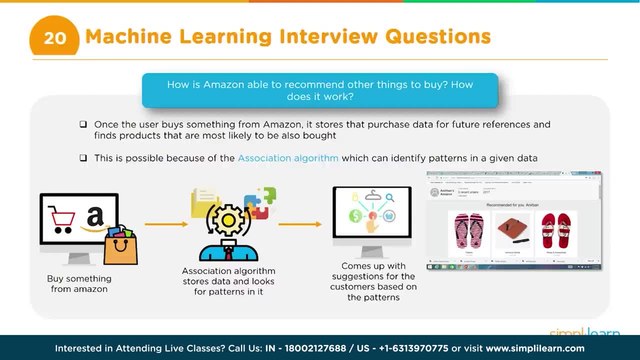 when somebody is logging in and when somebody is shopping, kind of the mapping of these two things are done. They try to identify. obviously, if you have logged in, then they know who you are and your information is available So they can identify who you are and what you are doing. So 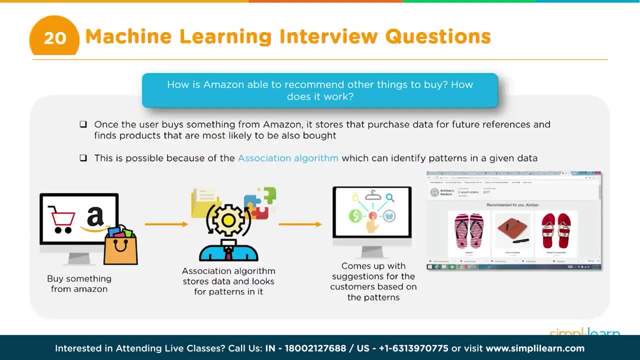 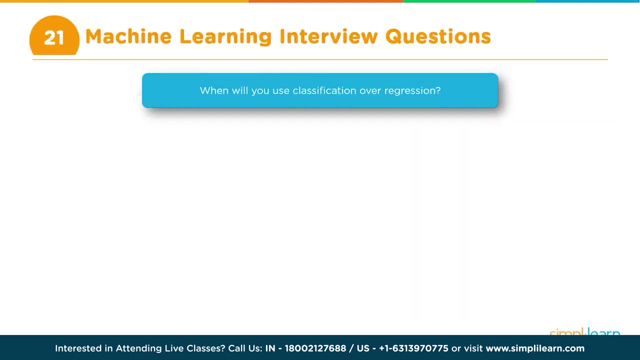 for example, your age may be, your gender and where you are located, what you purchased earlier, right. So all this is taken and the recommendation engine basically uses all this information and comes up with recommendations for a particular user. So that is how the recommendation engine works. All right, then the question can be something very basic like: when will you go for? 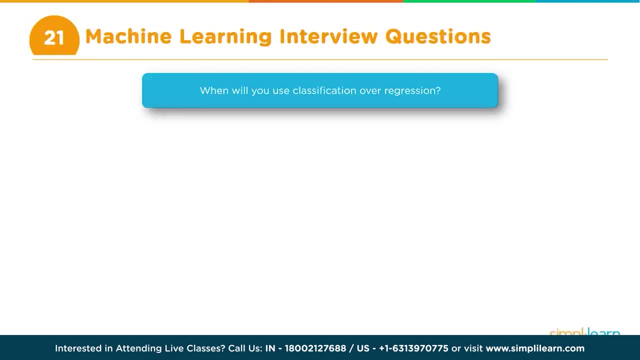 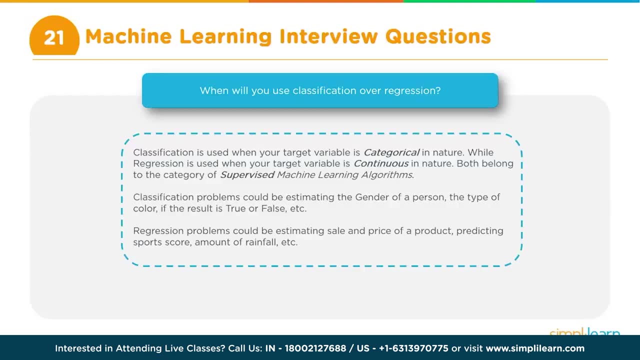 classification instead of regression, or when will you use classification instead of regression? Now, yes, so this is basically going back to the understanding of the basics of classification and regression. So classification is used when you have to identify or categorize things into discrete classes. So the best way to respond to this question is to take up some examples and use 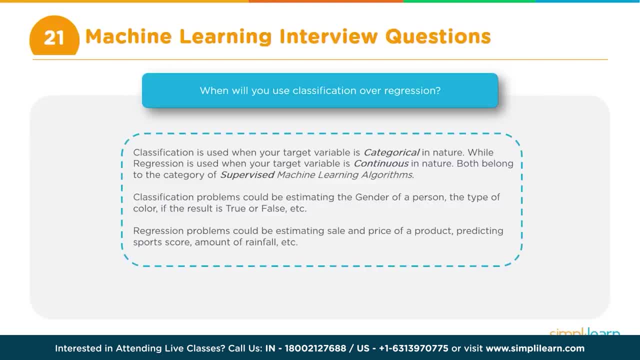 it, Otherwise it can become a little tricky. The question may sound very simple, but explaining it can sometimes be very tricky. In case of regression. we use, of course there will be some keywords that they will be looking for, So just you need to make sure you use those keywords. One is the discrete values and other is the 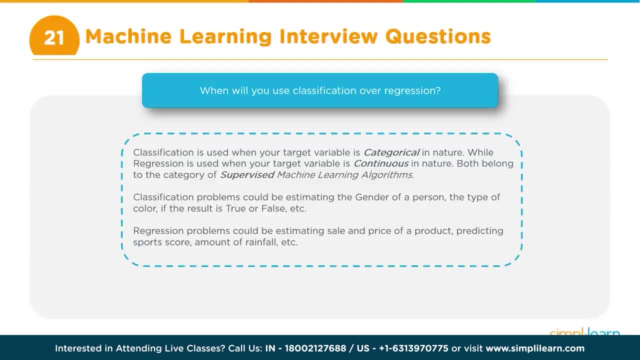 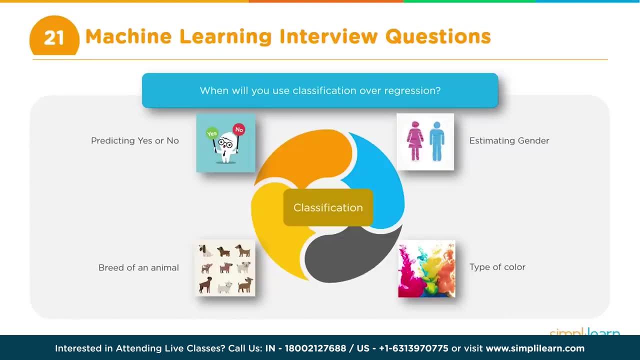 continuous values. So for regression, if you are trying to find some continuous values, you use regression, whereas if you are trying to find some discrete values you use classification. And then you need to illustrate what are some of the examples. So classification is like, let's say, 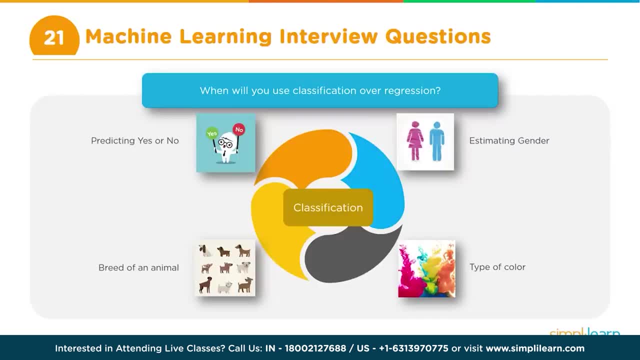 there are images and you need to put them into classes like cat, elephant, tiger, something like that. So that is a classification problem, Or it can be that is a multi-class classification problem. It could be binary classification problem, like, for example, whether a customer will buy or he will not buy. That is a classification, binary classification. 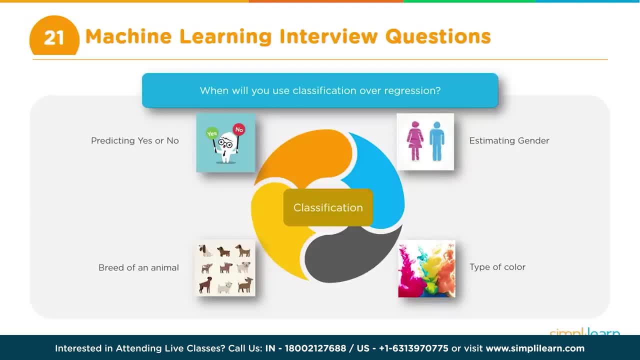 It can be in the weather forecast area. Now, weather forecast is again combination of regression and classification, because on the one hand, you want to predict whether it's going to rain or not rain. However, you also have to predict what is going to be the temperature tomorrow. 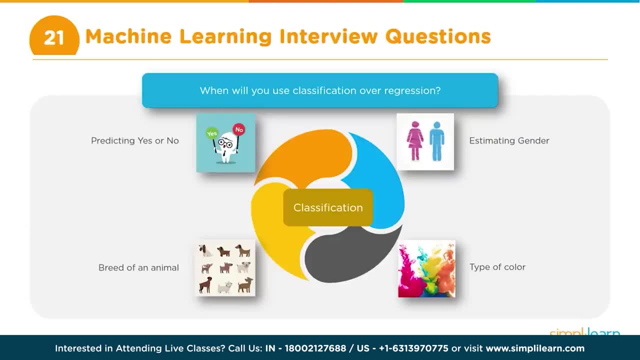 Now, temperature is a continuous value. You can't answer the temperature in a yes or no kind of a response. So what will be the temperature tomorrow? So you need to give a number which can be like 20 degrees, 30 degrees or whatever. So that is where you use regression. One more example is stock price. 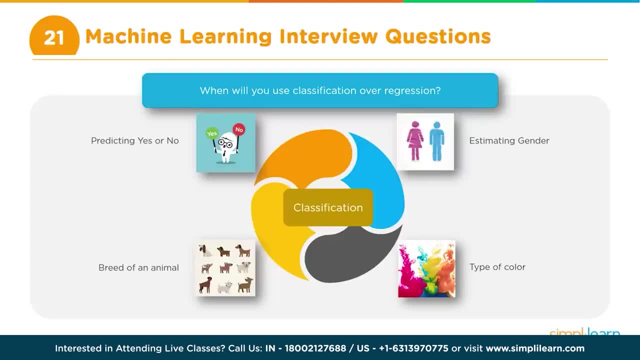 prediction. So that is where, again, you will use regression. So these are the various types of examples. So you need to illustrate with examples and make sure you include those keywords like discrete and continuous. So the next question is more about a little bit of a design related. 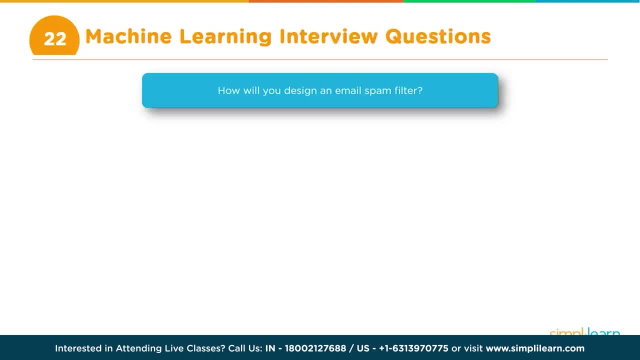 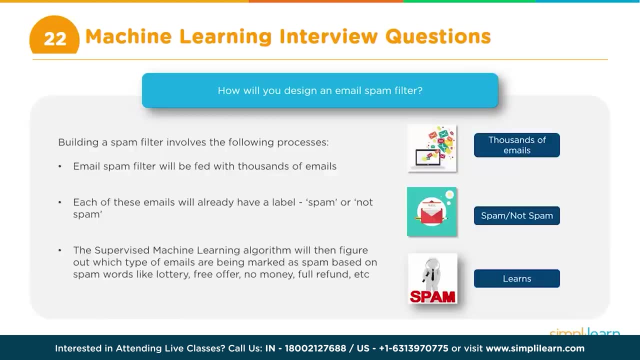 question to understand your concepts and things like that. So it is: how will you design a spam filter? So how do you basically design or develop a spam filter? So I think the main thing here is he is looking at probably understanding your concepts in terms of what is the algorithm you? 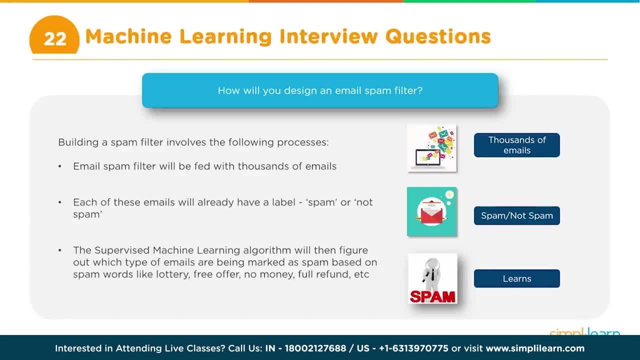 will use or what is your understanding about difference between classification and regression and things like that, And the process, of course, the methodology and the process. So the best way to go about responding to this is we say that, OK, this is a classification problem because we want 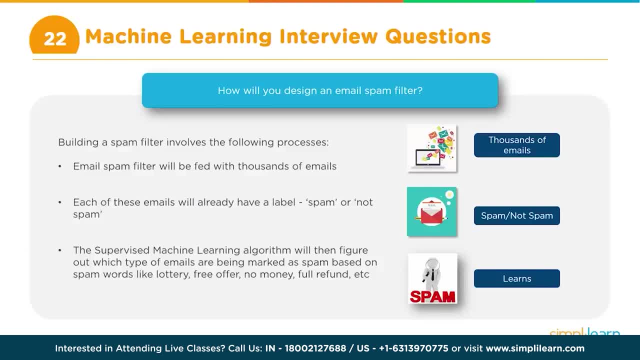 to find out whether an email is a spam or not spam, so that we can apply the filter accordingly. So first thing is to identify what type of a problem it is. So we have identified that it is a classification. Then the second step may be to find. 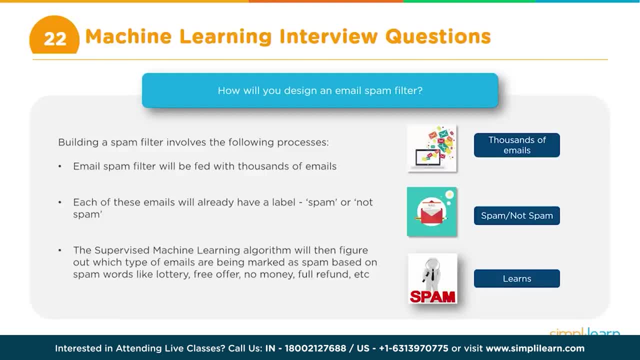 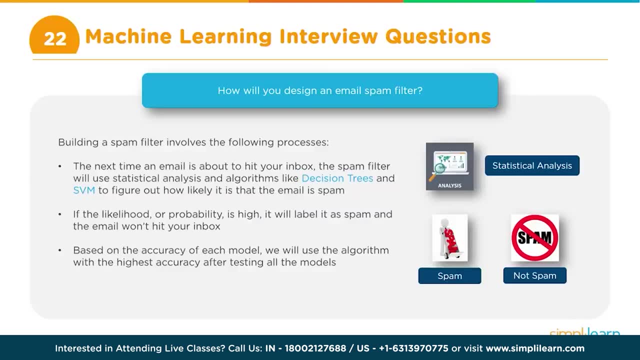 out what kind of algorithm to use Now, since this is a binary classification problem. logistic regression is a very common, very common algorithm, But however, as I said earlier also, we can never say that OK, for this particular problem, this is exactly the algorithm that we can use. So we can. 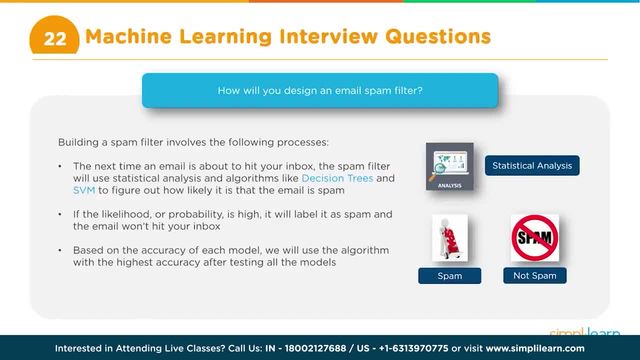 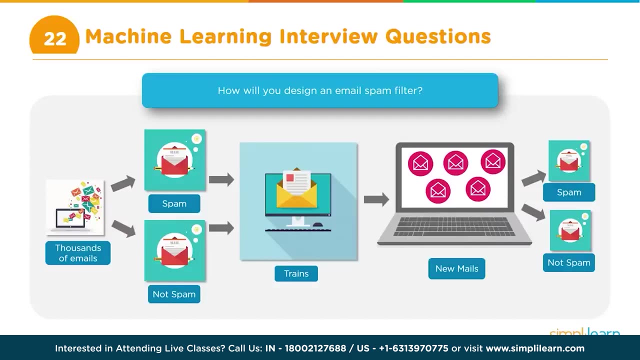 also probably try decision trees or even support vector machines, for example SVM. So we will kind of list down a few of these algorithms and we will say, OK, we want to, we would like to try out these algorithms, and then we go about taking your historical data, which is the 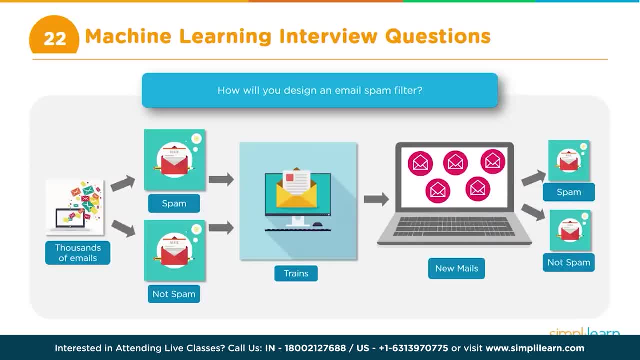 labeled data which are marked. so you will have a bunch of emails and then you split that into training and test data sets. You use your training data set to train your model, that or your algorithm that you have used, or rather the model actually. So, and you actually will have three models. Let's 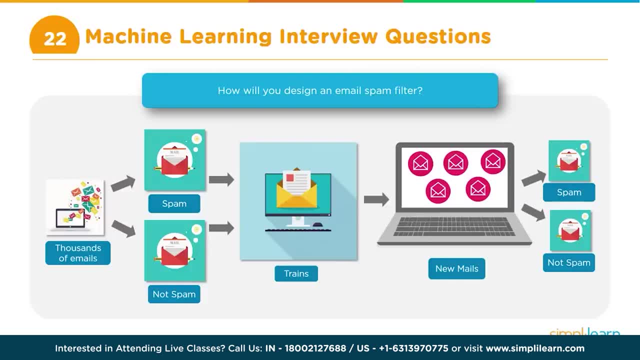 say: you are trying to test out three algorithms. So you will obviously have three models. so you need to try all three models and test them out as well, See which one gives the best accuracy, and then you decide that you will go with that model. OK, so training and 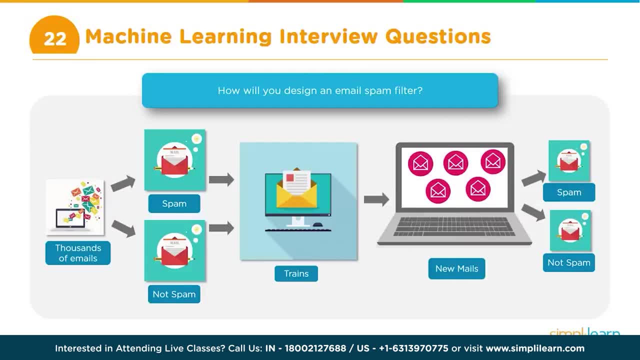 test will be done, and then you zero in on one particular model and then you say, OK, this is the model we will use. we will use and then go ahead and implement that or put that in production. So that is the way you design a spam field. The next question is about random forest. What is random? 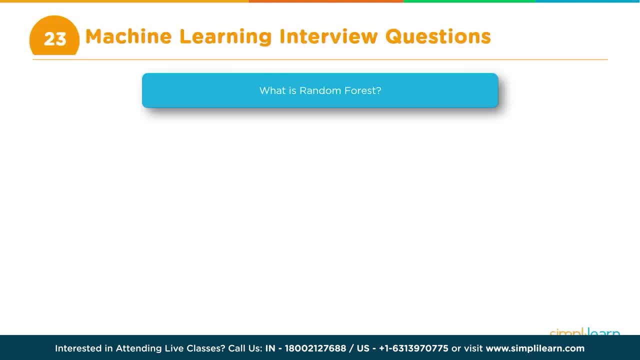 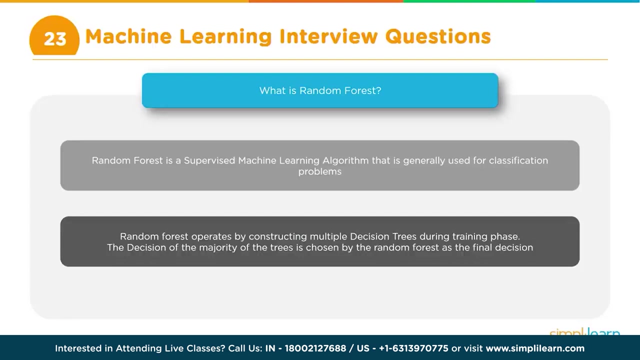 forest. So this is a very straightforward question. However, the response: you need to be again a little careful. while we all know what is random forest, explaining this can sometimes be tricky. So one thing is: random forest is kind of, in one way, it is an extension of decision trees, because it is basically nothing but you have multiple decision. 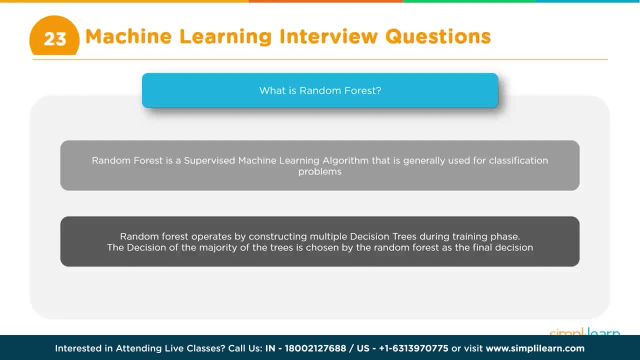 trees and trees will basically you will use for doing if it is classification- mostly it is classification- you will use the trees for classification and then you use voting for finding that the final class Underlines. but how will you explain this? How will you respond to this? So, first thing, obviously, 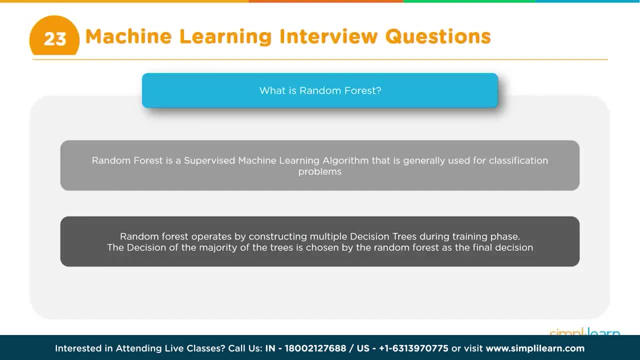 you will say that random forest is one of the algorithms and the more important thing that you need to- probably the interviewer is is waiting to hear- is ensemble learner right? So this is one type of ensemble learner. What is ensemble learner? Ensemble learner is like a combination of 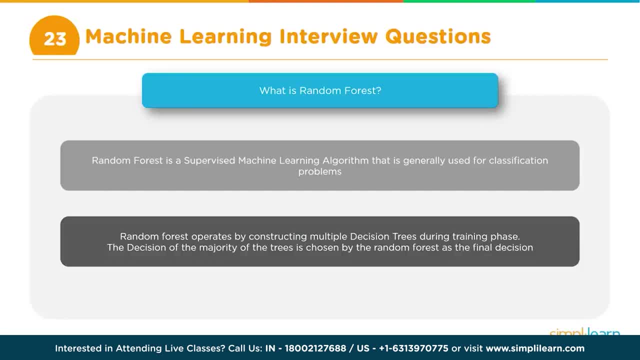 algorithms, So it is a learner which consists of more than one algorithm or more than one, maybe more than one instance of it. but in the case of random forest, the algorithm is the same, But instead of using one instance of it, we use multiple instances of it, and we use so in a way. 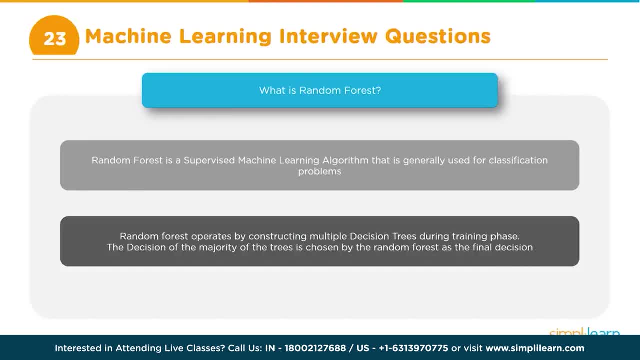 that is, a random forest, is an ensemble learner. There are other types of ensemble learners where we have, like we use different algorithms itself, So you have one, maybe logistic regression and a decision tree combined together, and so on and so forth. Or there are other ways, like, for example, 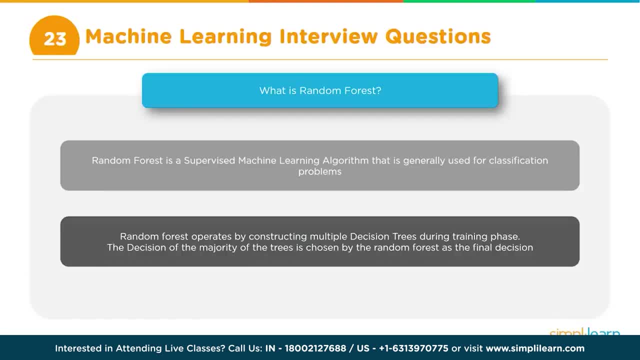 splitting the data in a certain way and so on. So that's all about ensemble. We will not go into that. but random forest is said- I think the interview will be happy to hear this word- ensemble learner. And so then you go and explain how the random forest works. So if the random forest is, 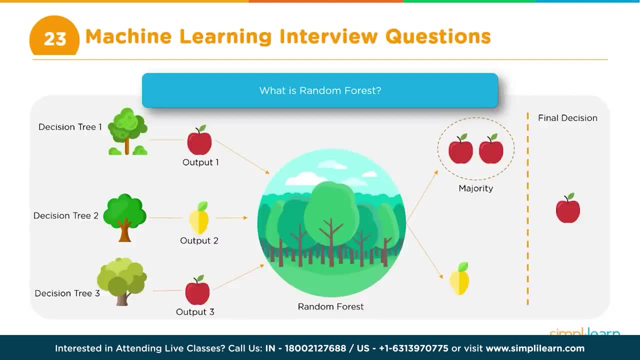 used for classification, then we use what is known as a voting mechanism. So, basically, how does it work? Let's say your random forest consists of 100 trees and each observation- you passed through this forest- and each observation. let's say it is a classification problem, binary classification, zero. 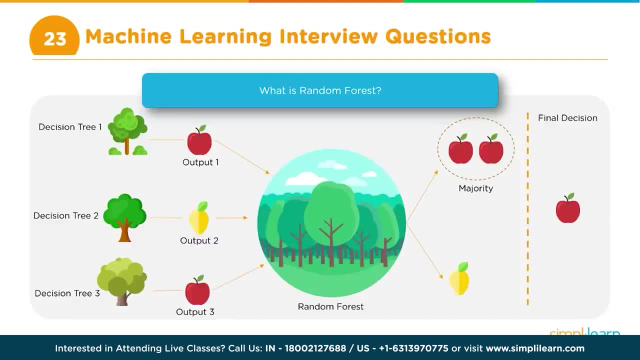 or one, and you have 100 random forest and if the classification problem is not also toxic and you 100 trees. now, if 90 trees say that it is a 0 and 10 of the trees say it is a 1, you take the majority, you may take a vote and since 90 of them are saying 0, you classify this as 0. then you take. 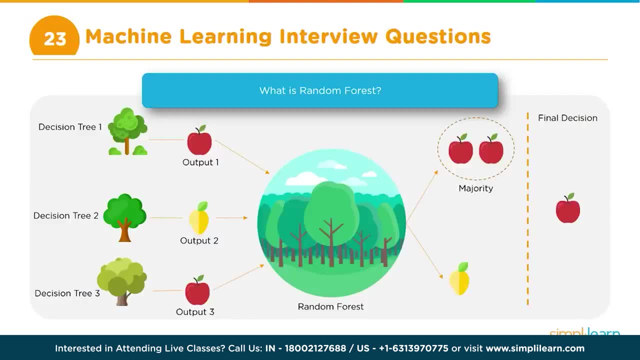 the next observation, and so on. so that is the way random forest works for classification. if it is a regression problem, it's somewhat similar, but only thing is, instead of vote, what we will do is so, in regression, remember what happens. you actually calculate a value, right? so, for example, you're 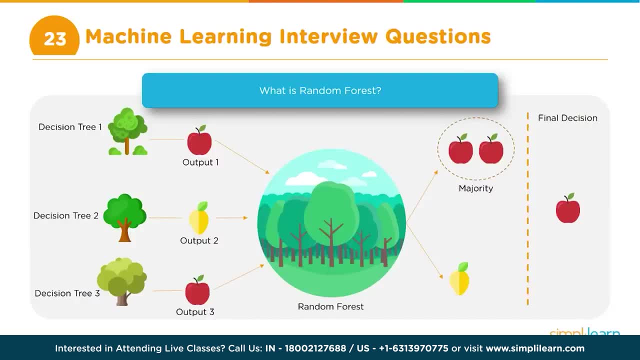 using regression to predict the temperature, and you have 100 trees and each tree obviously will probably predict a different value of the temperature. they may be close to each other but they may not be exactly the same value. so these 100 trees. so how do you now find the actual? 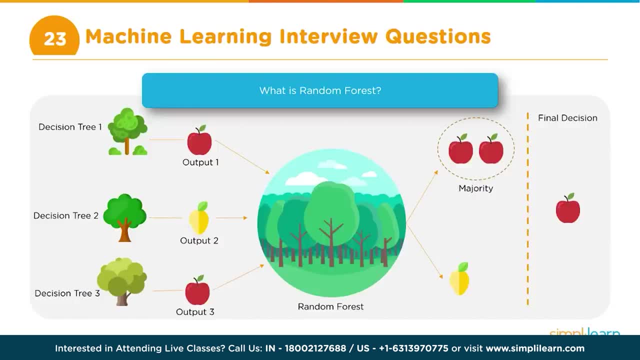 value the output for the entire forest, right? so you have outputs of individual trees which are a part of this forest, but then you need to find the final output of the forest itself. so how do you do that? so in case of regression, you take like an average or the mean of all the 100 trees, right? so this is also a way of reducing. 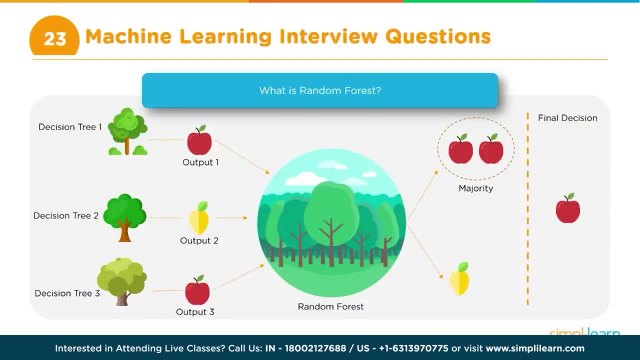 the error. so maybe if you have only one tree and if that one tree makes a error, it is basically 100 wrong or 100 right, right. but if you have, on the other hand, if you have a bunch of trees, you are basically mitigating that error, reducing that error. okay, so that is the way. random forest. 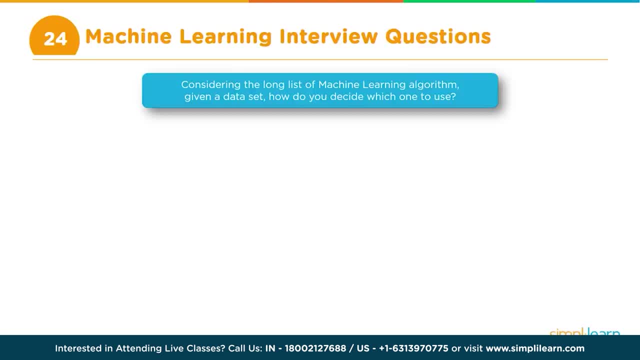 works. so the next question is: considering the long list of machine learning algorithms, how will you decide on which one to use? so once again here, there is no way to outright say that this is the algorithm that we will use for a given data set. this is a very good question, but then the response. 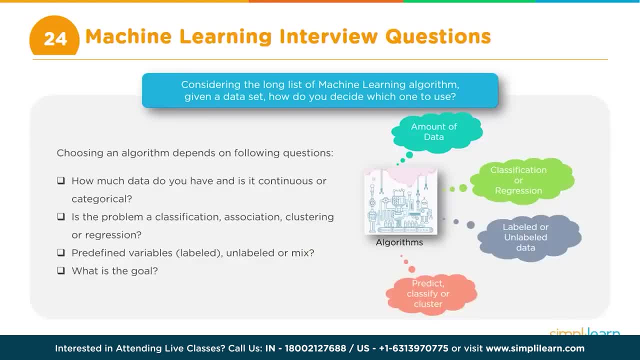 has to be like again. there will not be a one size fits all, so we need to. first of all, you can probably shorten the list in terms of by saying, okay, whether it is a classification problem or it is a regression problem, to that extent you can probably shorten the list. 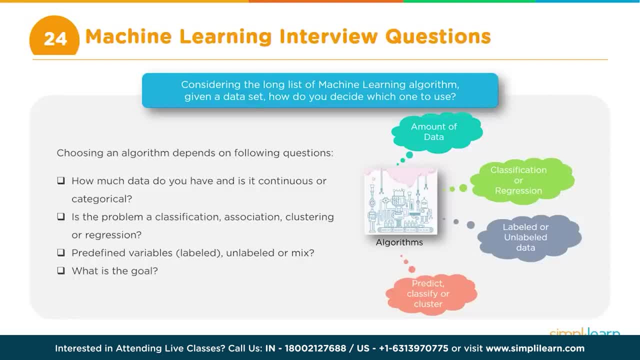 because you don't have to use all of them. if it is a classification problem, you only can pick from the classification algorithms, right. so, for example, if it is a classification, you cannot use linear regression algorithm, or if it is a regression problem you cannot use svm, or maybe, no, you can. 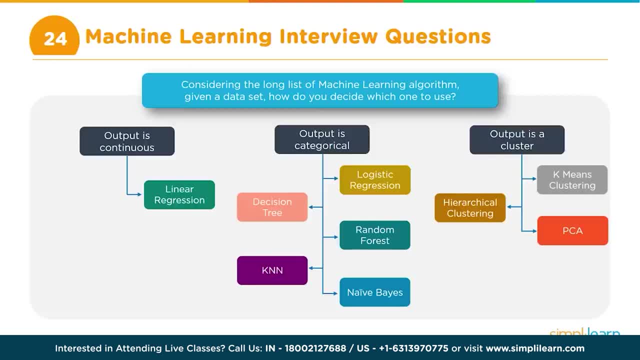 use svm, but maybe a logistic regression right. so to that extent you can probably shorten the list, but still you will not be able to 100 decide on saying that this is the exact algorithm that i am going to use. so the way to go about is you choose a few algorithms based on what the problem is. you try out your data, you train some. 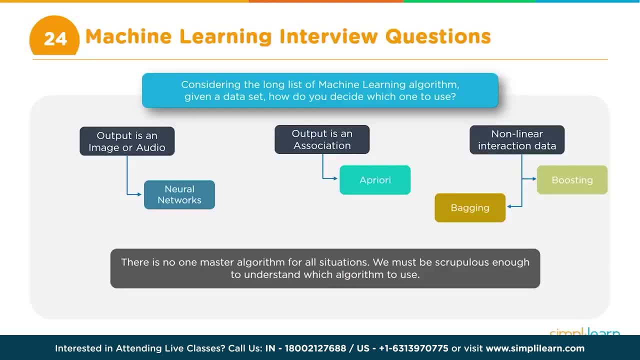 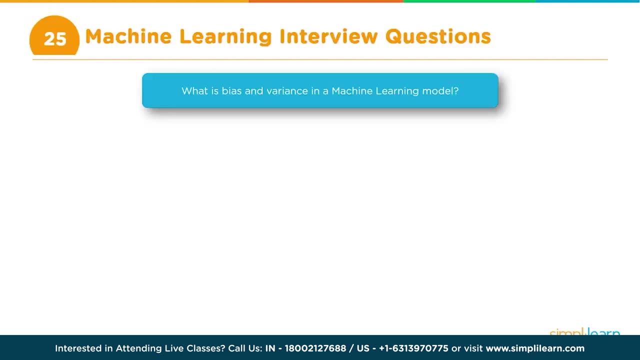 models of these algorithms, check which one gives you the lowest error or the highest accuracy, and based on that, you choose that particular algorithm. okay, all right. then there can be questions around bias and variance. so the question can be: what is bias and variance in machine learning? so you just need to give out a definition for each of these, for example. 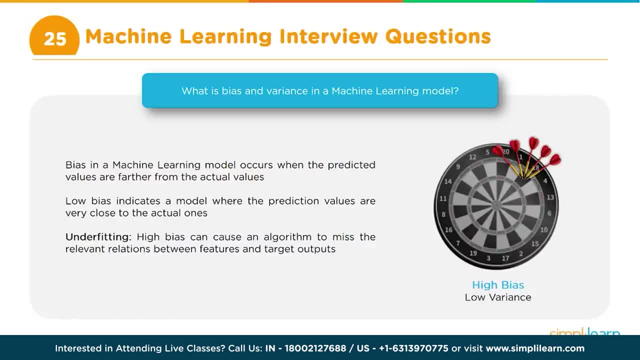 in machine learning it occurs when the predicted values are far away from the actual value. so that is a bias, okay, and whereas they are all, all the values are probably. they are far off, but they are very near to each other, though. the predicted values are close to each other, right while they 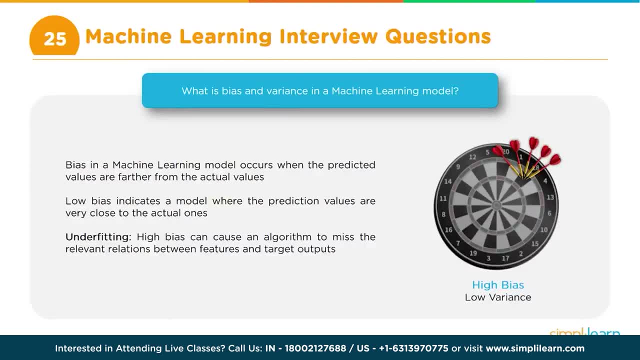 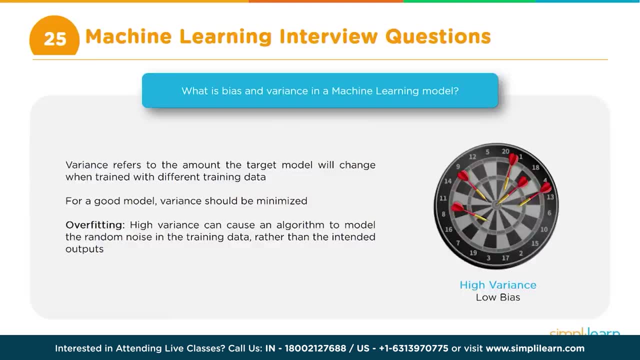 are far off from the actual value, but they are close to each other. you see the difference. so that is bias. and then the other part is your variance. now, variance is when the predicted values are all over the place, right. so the variance is high. that means it may be close to the target, but it is kind of very scattered. so 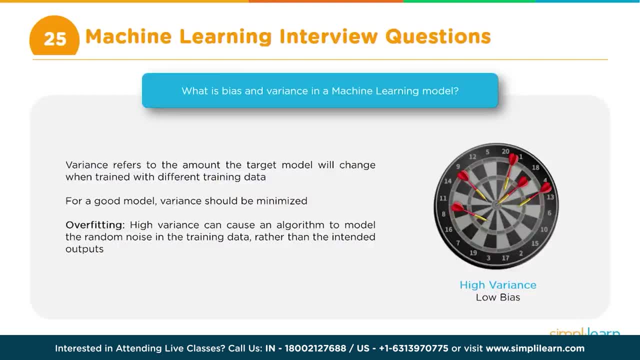 the point, the predicted values are not close to each other. right in case of bias, the predicted values are close to each other, but they are not close to the target. but here they may be close to the target, but they may not be close to each other. so they are a little bit more scattered. so 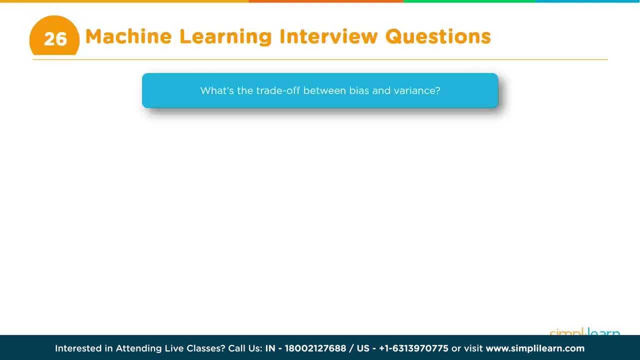 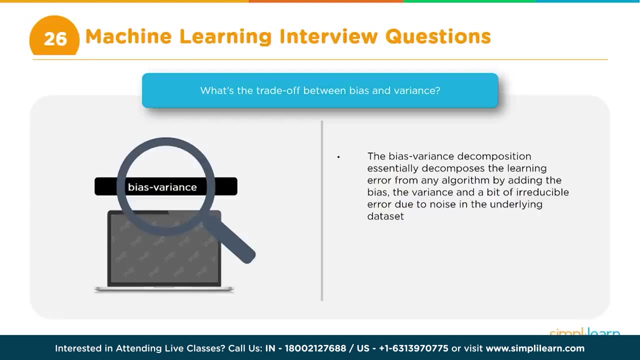 that is what in case of a variance. okay, then the next question is about, again related to bias and variance. what is the trade-off between bias and variance? yes, i think this is a interesting question because these two are heading in different directions. so, for example, if you try to minimize the bias, variance will keep going high, and if you 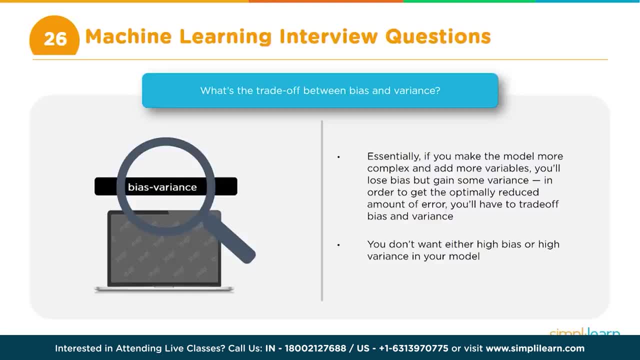 try to minimize the variance bias will keep going high and there is no way you can minimize both of them. so you need to have a trade-off saying that, okay, this is the level at which i will have my bias and this is the level at which i will have variance. so the trade-off is that, pretty much that. 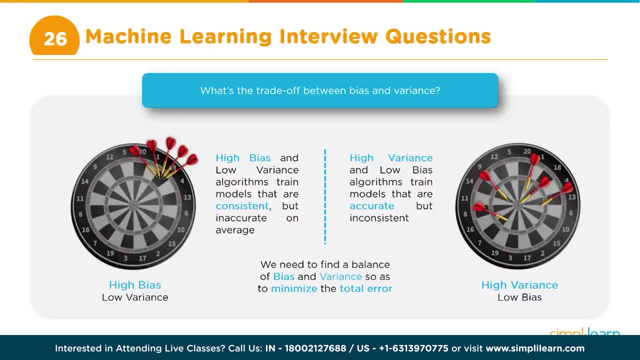 if i try to minimize bias and variance at the same time, the price and change at the same time. so to put it in this way, that you can mean at leastCom built both these values, separate to anime and anime are effectively one, and it does not work critically but they help get figures. 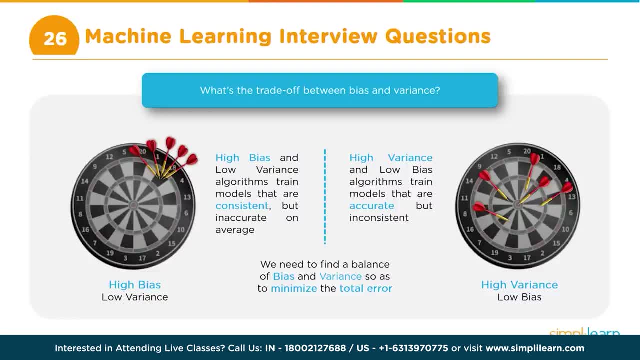 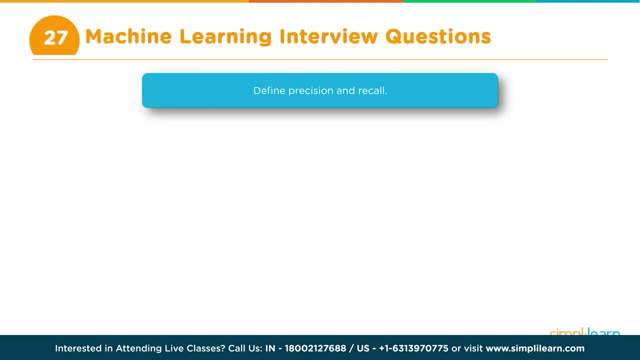 later in the general explanation. what not so for sunrise, which is who will beblemost? just to, Ok, let's go to it. in parameters, whichever 김, each one that's right, let's go to it of them will go off the track. Define precision and recall. Now again here, I think it would be. 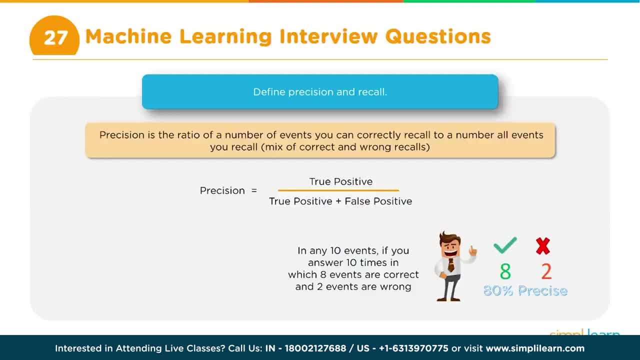 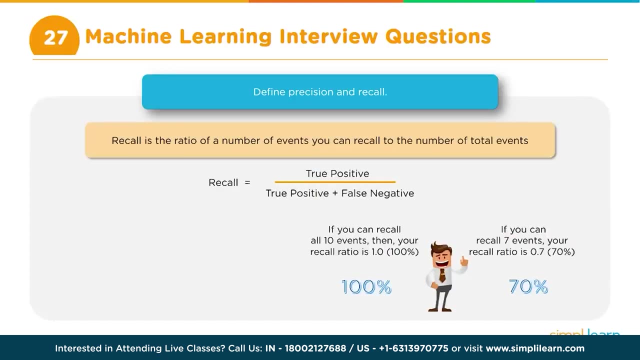 best to draw a diagram and take up the confusion. matrix, and it is very simple. The definition is like a formula. Your precision is true positive by true positive plus false positive and your recall is true positive by true positive plus false negative. So that's, you can just show it. 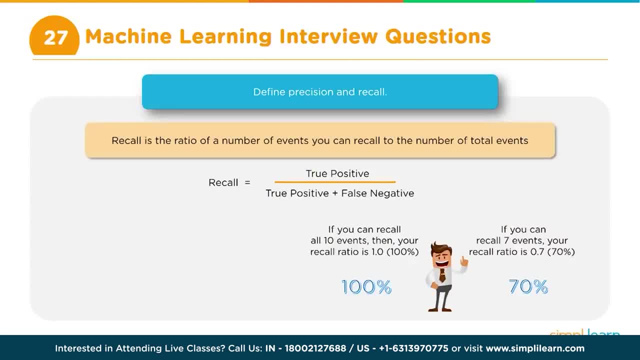 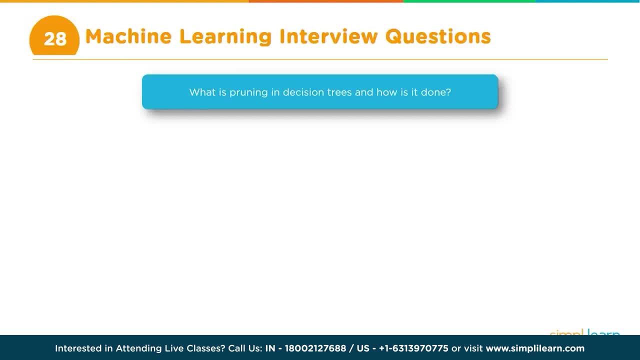 in a mathematical way. That's pretty much you know. that can be shown. That's the easiest way to define. So the next question can be about decision tree. What is decision tree pruning and why is it So? basically, decision trees are really simple to implement and understand, but 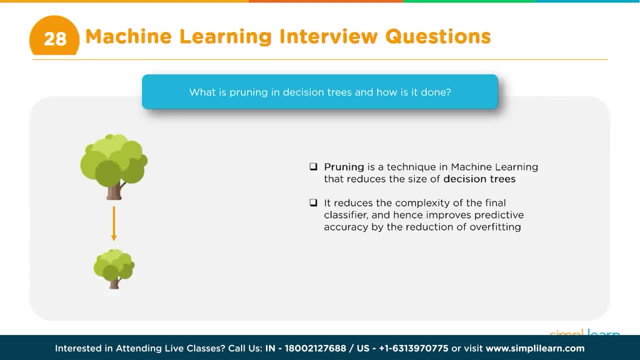 one of the drawbacks of decision trees is that it can become highly complicated As it grows right and the rules and conditions can become very complicated, and this can also lead to overfitting, which is basically that during training you will get 100% accuracy, but 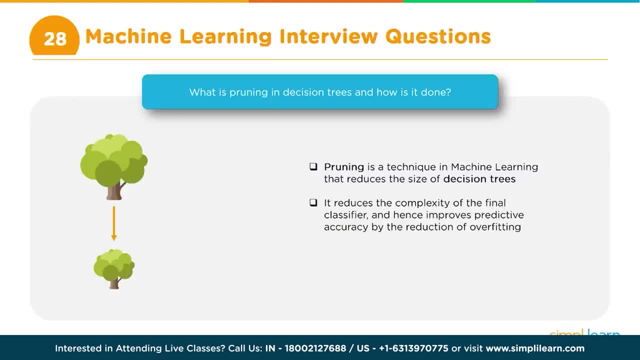 when you're doing testing, you'll get a lot of errors. So that is the reason pruning needs to be done. So the purpose or the reason for doing decision tree pruning is to reduce overfitting or to cut down on overfitting. and what is decision? 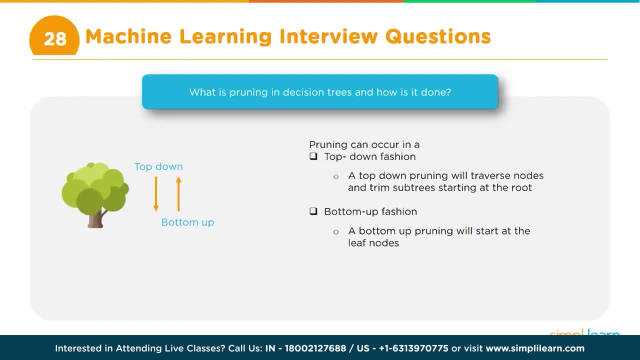 Decision. tree pruning. it is basically that you reduce the number of branches because, as you may be aware, a tree consists of the root node and then there are several internal nodes and then you have the leaf nodes. Now, if there are too many of these internal nodes, that is when you face the problem. 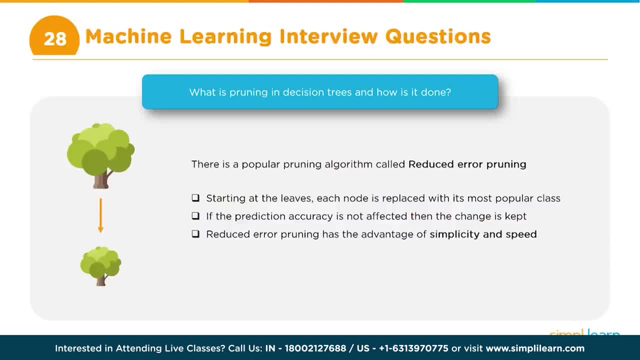 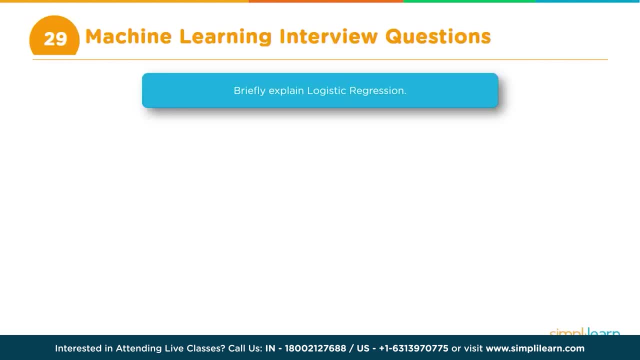 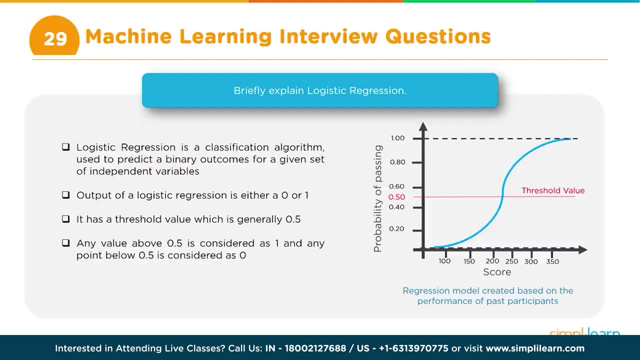 of overfitting and pruning is the process of reducing those internal nodes. Alright, so the next question can be: what is logistic regression? So, basically, logistic regression is one of the techniques used for performing classification, especially binary classification. Now there is something special about logistic regression, and there are a couple. 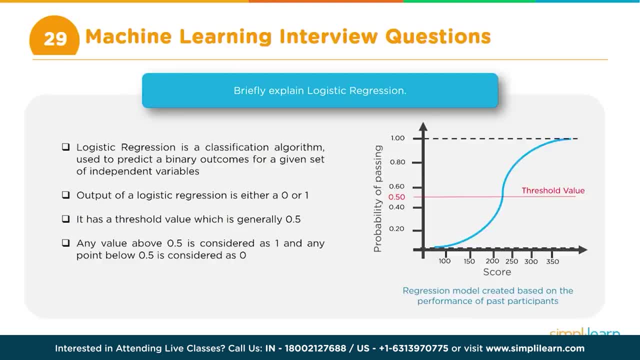 of things you need to be careful about. First of all, the name is a little confusing. It is called logistic regression but it is used for classification, So this can be sometimes confusing. so you need to probably clarify that to the interviewer if it's really you know. 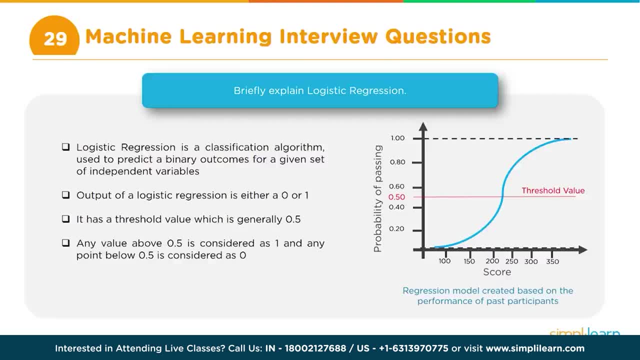 if it is required, and they can also ask this like a trick question, right? so that is one part. Second thing is the term logistic has nothing to do with the usual logistics that we talked about, but it is derived from log, so that the mathematical derivation involves log and therefore the 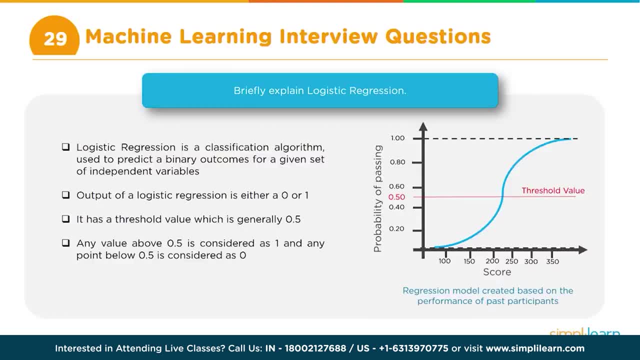 name logistic regression. So what is logistic regression and how is it used? Logistic regression is used for binary classification and output of a logistic regression is either a zero or and it varies. so it's basically. it calculates a probability between 0 and 1 and we can set a. 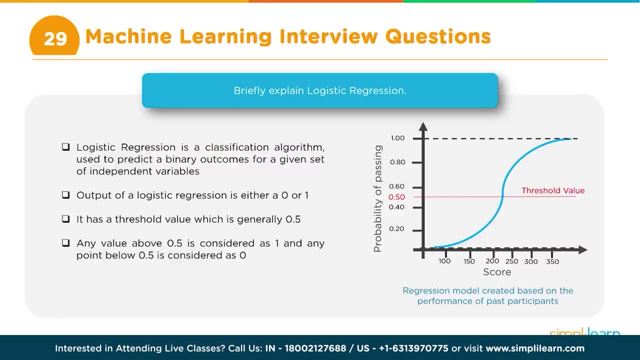 threshold that can vary. typically it is 0.5, so any value above 0.5 is considered as 1 and if the probability is below 0.5 it is considered as 0. so that is the way we calculate the probability, or the system calculates the probability and, based on the threshold, it sets a value of 0 or 1, which. 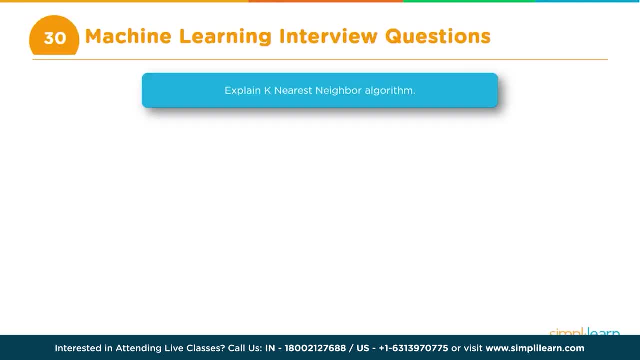 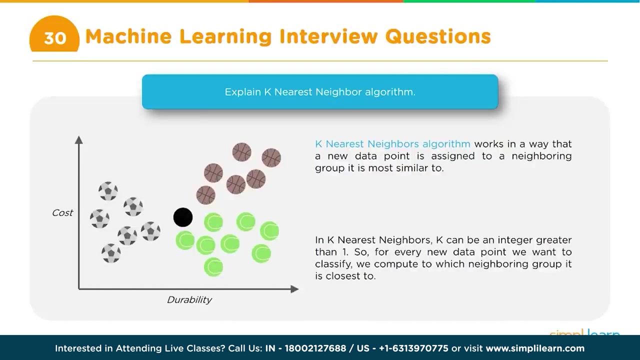 is like a binary classification- 0 or 1.. Okay, then we have a question around k nearest neighbor algorithm. so explain k nearest neighbor algorithm. So, first of all, what is a k nearest neighbor algorithm? this is a classification algorithm, so that is the first thing we need to mention and 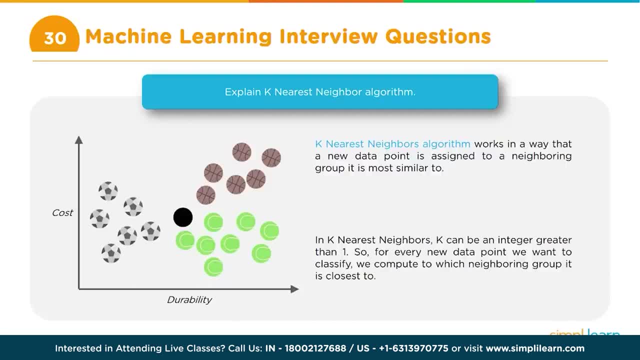 we also need to mention that the k is a number, it is an integer, and this is variable and we can define what the value of k should be. it can be 2,, 3,, 5,, 7,, 8,, 9,, 10,, 11,, 12,, 13,, 14,, 15,, 16,, 17,, 18,, 19,, 20,, 21,, 22,, 23,, 23,, 24,, 25,, 26,, 27,, 28,, 29,, 30,, 31,. 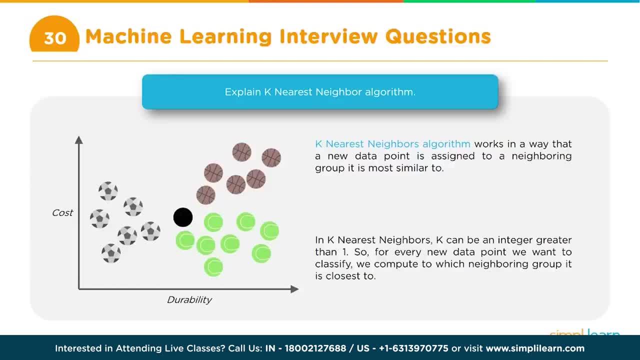 32,, 33,, 34,, 35,, 36,, 37, and usually it is an odd number. so that is something we need to mention. technically it can be even number also, but then typically it would be odd number and we will see. 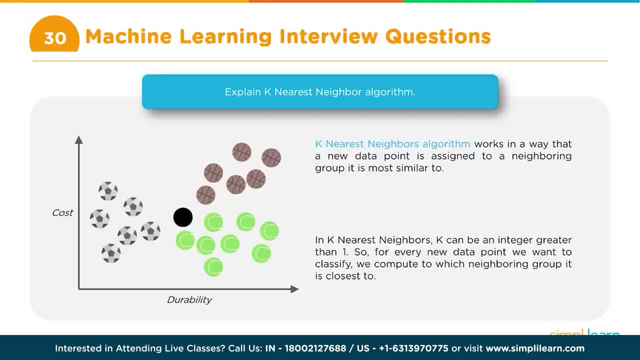 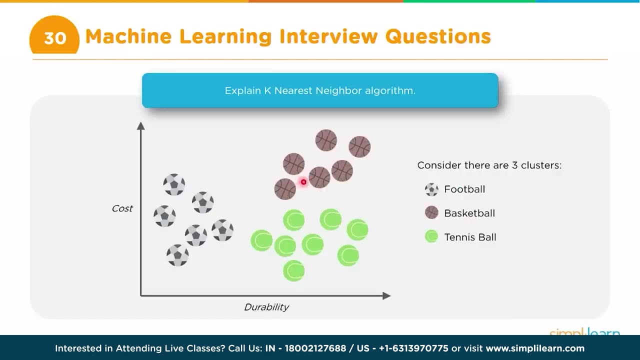 why. that is okay. so, based on that, we need to classify objects. okay, we need to classify objects. so, again, it will be very helpful to draw a diagram. you know, if you are explaining, I think that will be the best way. so draw some diagram like this: and let's say we have three clusters or three. 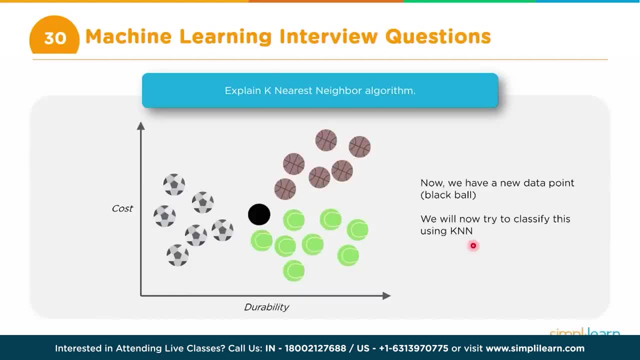 classes existing and now you want to draw a diagram. and you want to draw a diagram and you want to find for a new item that has come, you want to find out which class this belongs to. right, so you go about, as the name suggests. if you go about finding the nearest neighbors, right the points. 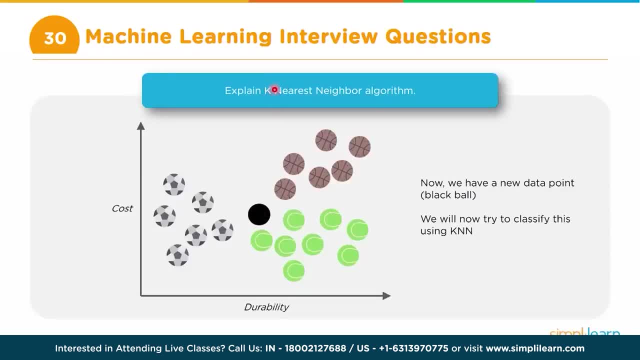 which are closest to this and how many of them you will find. that is what is defined by k. now, let's say our initial value of k was 5, so you will find the k the five nearest data points. so in this case, as it is illustrated, these are the five nearest. 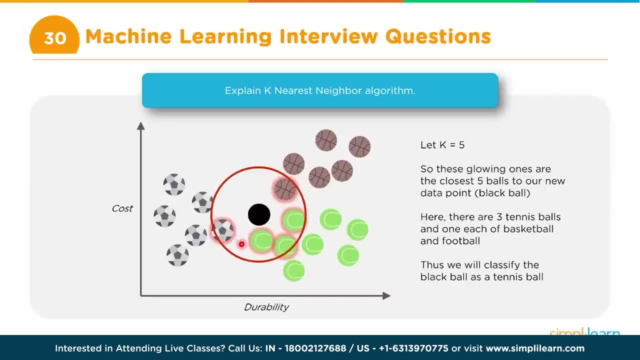 data points, but then all five do not belong to the same class or cluster. so there are one belonging to this cluster, one, the second one belonging to this cluster, two, three of them belonging to this third cluster. okay, so how do you decide? that's exactly the reason we should. 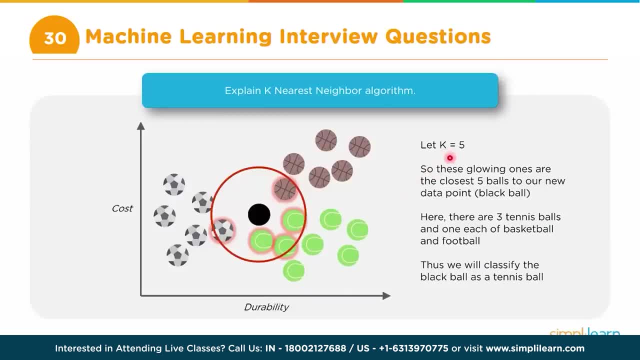 as much as possible, try to assign an odd number so that it becomes easier to assign this. so in this case, you see that the majority. actually, if there are multiple classes, then you go with the majority. so since three of these items are the same, then you should try to assign an odd number. 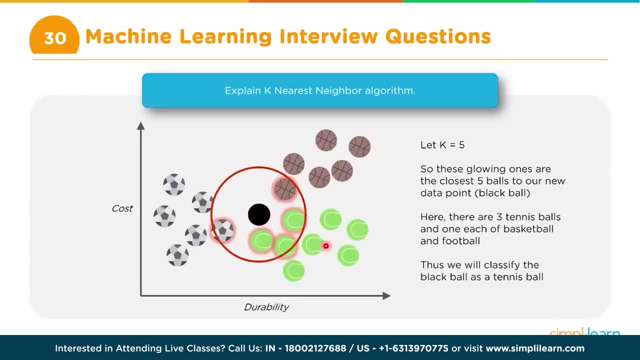 which will then make you understand how this class will change. so all these items belong to this class. we assign, which is basically the in, in this case the green or the tennis or the third cluster, as i was talking about, right, so we assign it to this third class. so in this case it is uh. 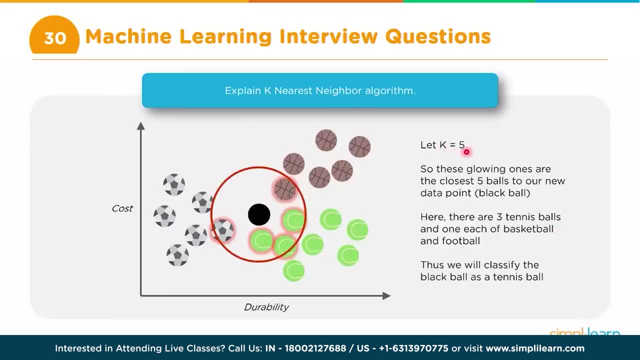 that's how it is decided. okay, so k: nearest neighbors. the first thing is to identify the number of neighbors that are mentioned as k. so in this case it is k is equal to 5, so we find the has the maximum number in that, and then the new data point is assigned to that class. 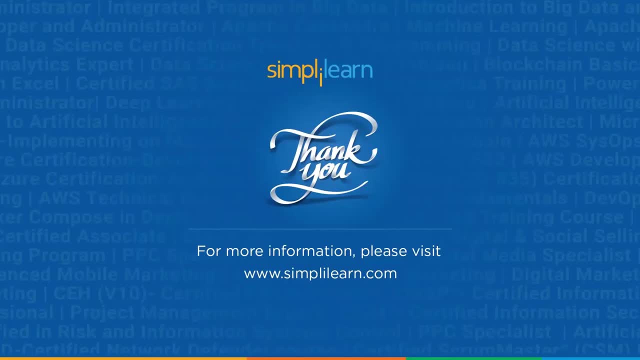 And with that we have come to the end of this NLP full course. I hope you found it valuable and entertaining. Please ask any questions about the topics covered in the video in the comment box below and a team of experts will assist you in addressing your